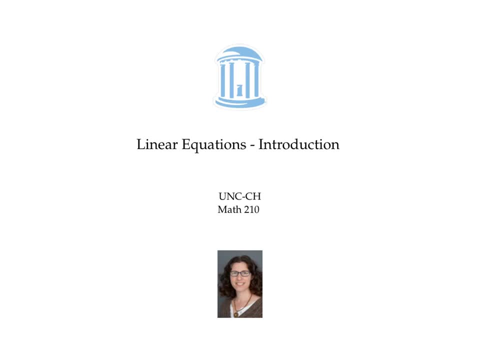 This video gives an introduction to systems of linear equations. The equation for x minus five, y plus 7.3, z equals 27 is an example of a linear equation, And in general, a linear equation is an equation that can be written as the sum of a bunch of numbers called the. 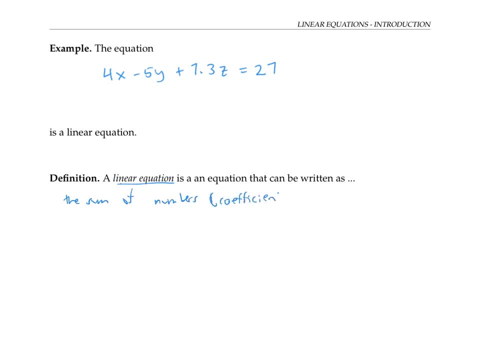 coefficients times variables, I'll add it up to equal another number. Okay, so in this example, above the numbers four, negative five and 7.3 are the coefficients And letters x, y and z are the variables And the products of coefficients times. the. 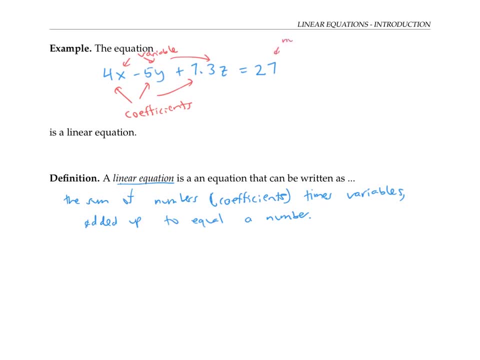 variables get added up to equal another number. So which of these three examples qualify as linear equations? The first one does not, Because the four is multiplied by x squared, the square of a variable, not just a single variable. The second equation is also not a linear equation because the 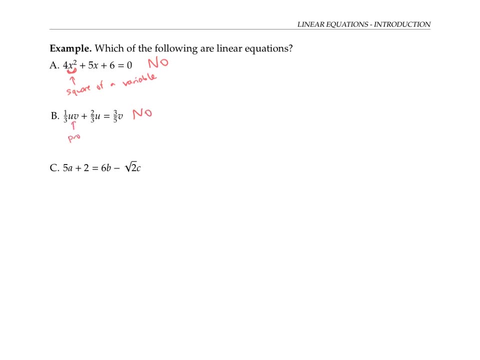 one third is multiplied by a product of variables, not just a single variable. The third equation does qualify as a linear equation Because if I rewrite it as five a minus six B, plus the square root of two c equals negative two, then it is a sum of coefficients, x variables, all added up to equal a number, A system of. 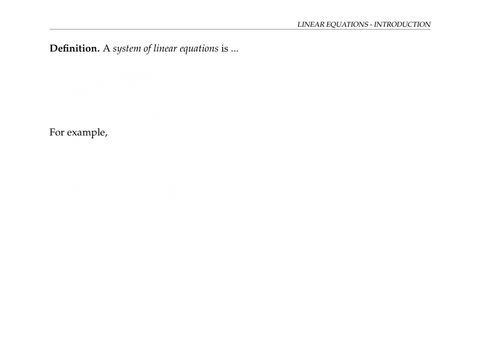 linear equations is just a set or collection of linear equations involving the same sum, the same variables. Here's an example. This example involves four equations and three variables are s and t. Notice that not every equation has to contain all the variables. A solution to a system of linear equations is a set of values for the variables, So that 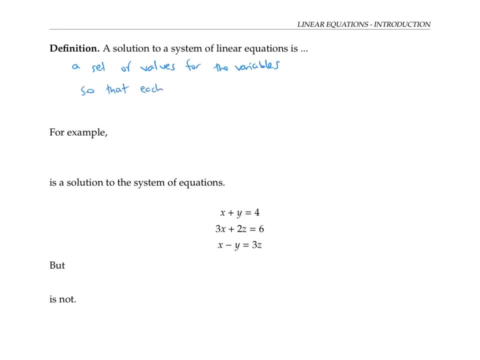 each equation in the system is satisfied. For example, x equals two, y equals two, z equals zero is a solution to this system of equations, because we plug in two for x and two for y and zero for z. This satisfies the first equation, the second equation and the third equation. 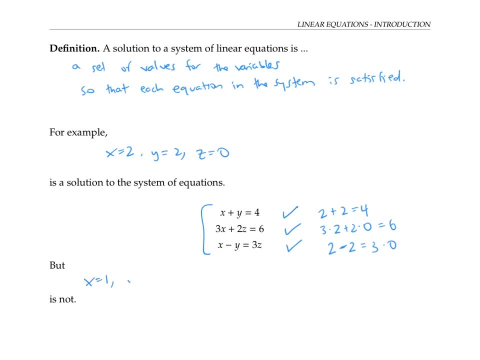 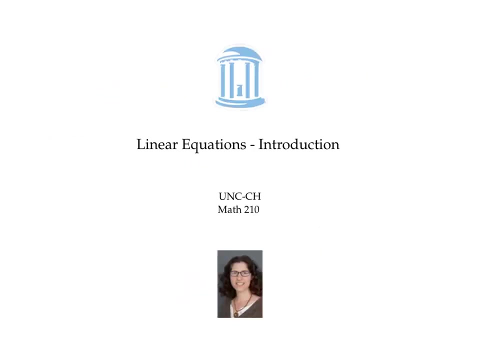 On the other hand, x equals one, y equals three and z equals three. halves is not a solution. You can check that these values satisfy the first equation and the second equation, but not the third one. This concludes the brief introduction to systems of linear equations. If you've ever heard, 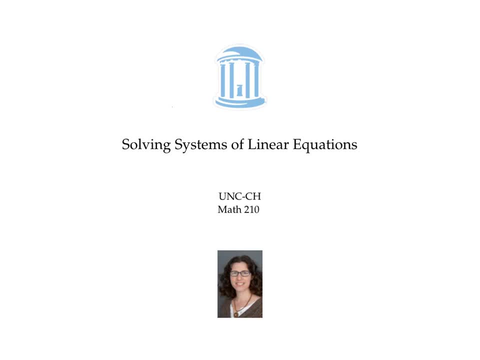 the expression there's more than one way to skin a cat. it definitely applies to solving systems of linear equations. In this video, I'll demonstrate two standard methods: the method of substitution and the method of elimination. If we want to solve the system of linear equations using the method of substitution, the basic 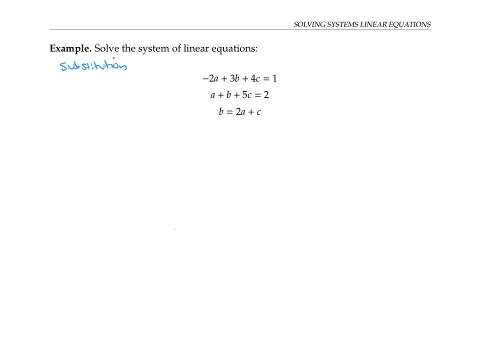 idea is to use one of the equations to solve for a variable in terms of the other variables and then substitute in to the other equations. In this example, I noticed that in equation three I already have B solved for in terms of two A plus C. So 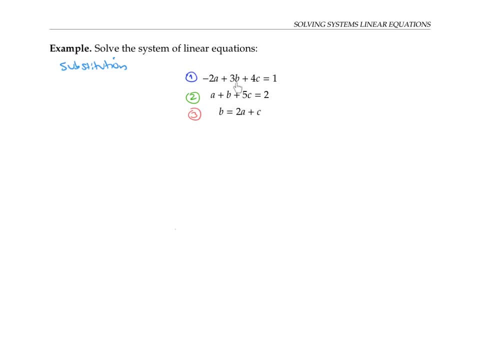 that makes it easy to substitute in two A plus C everywhere I see a B in the other equations to get rid of the variable there. So my first equation becomes negative. two A plus three times two a plus C plus four, c equals one. And my second equation becomes: 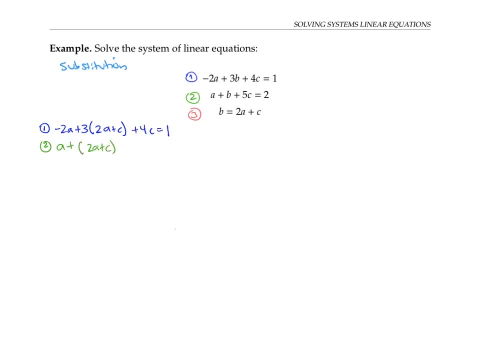 a plus two, a plus c plus five c equals two. I'll just carry down my third equation. Now let me simplify my first equation a bit. I'll distribute and group like terms: minus two, a plus six, a is for a, three c plus four c is seven c, and that equals one. I'll also 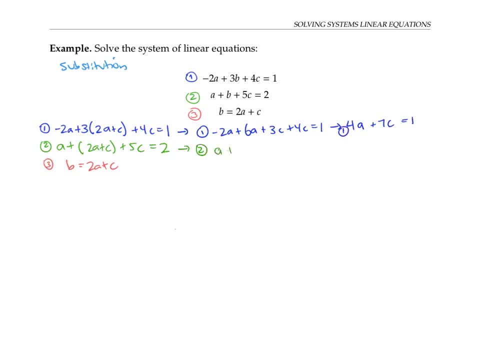 simplify the second equation by getting rid of the unnecessary parentheses and combining like terms. Once again, I'll just carry over the third equation. Notice that my first two equations now have only the variables a and c in them. Once again, I'll solve for one variable, say a, in one of the equations, say the first one. 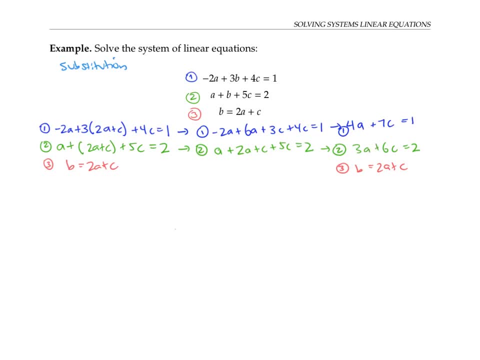 and then substitute that into the second equation. So in the first equation I have four a equals one minus seven C. so a equals one fourth minus seven fourths C, And I'll plug that in to the second equation. So everywhere I see an A I'm going to put in one fourth minus. 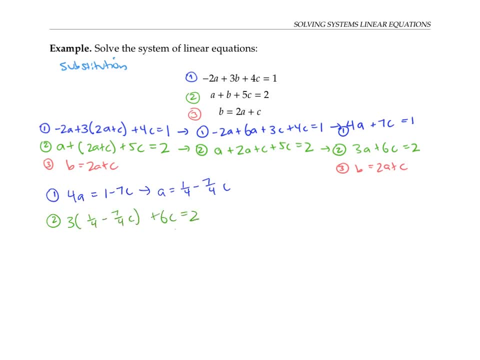 seven fourths C. Okay, once again I'll simplify by distributing, combining like terms. Let's see: six C is the same as 24 fourths C, and 24 fourths minus 21 fourths is three fourths C. So that's equal. 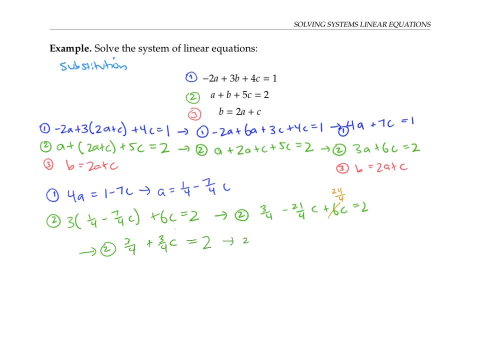 to two. I can subtract the three fourths to the other side, So I get three four. C equals one. So two minus three fourths. so two is eight fourths. So eight fourths minus three fourths is five fourths. So that means that C is equal to five fourths divided by three fourths. 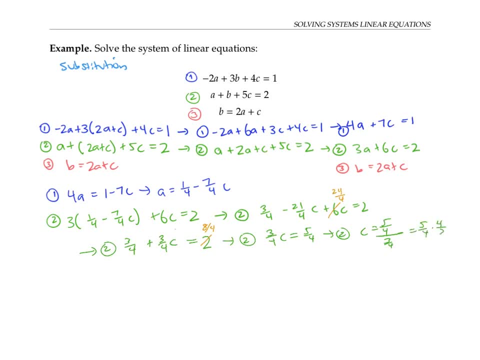 the same thing as five fourths times four thirds, or five thirds. So I now have a numerical value for C. C is equal to five thirds. Poor equation. three gets carried along for the ride yet again. Well, I've made huge progress. 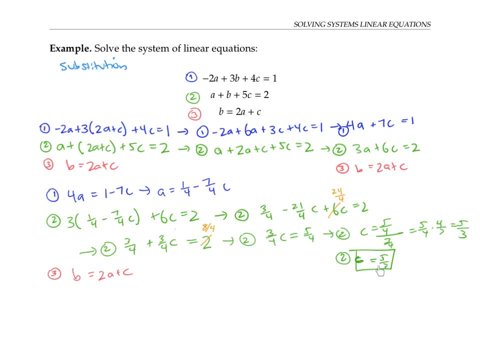 here. Now that I have a numerical value for C, I can plug that number into this version of the first equation and get a number for a. So my first equation is now going to be: a equals one fourth minus seven fourths times five thirds. So that's one fourth minus 35.. 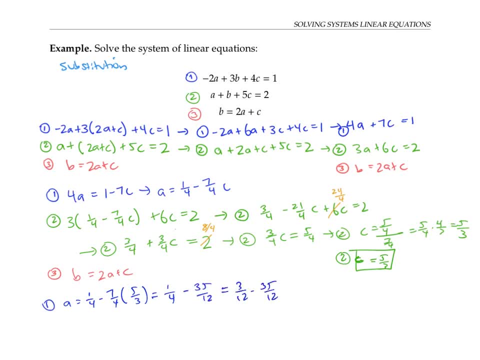 That's three, 12th minus 35, 12th, which is minus 32, 12th, which is minus eight thirds. So I have that a equals minus eight thirds. Now I can plug A and C into the third equation to get B. Let me just copy the second equation over for completeness. And now the third equation. 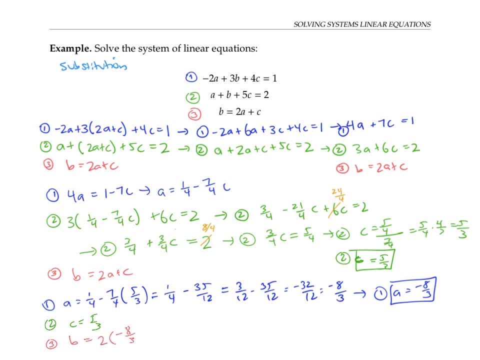 becomes: B equals two, Two times negative, eight thirds plus five thirds. So that's negative 16 thirds plus five thirds or negative 11 thirds. C: B equals negative 11 thirds. And I found the solution to the system of linear equations. I can check my work by plugging in these values into each. 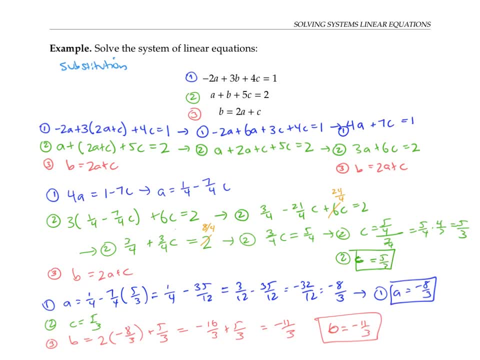 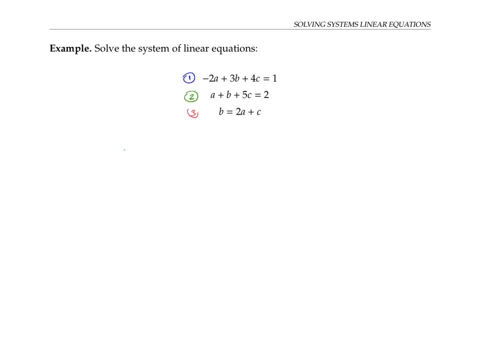 of the three equations to make sure that they do in fact satisfy all three equations. Now I'm going to attack the same system of three linear equations using the method of elimination. The idea behind this method is: I add or subtract multiples of equations. 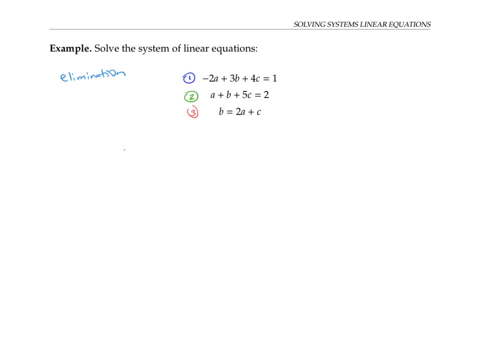 together to get rid of variables. Before I start, though, I'm going to write my equations in the standard form, where all the variables are on the left and all the constants are on the right. The first two equations are already in this standard form, So I'll just 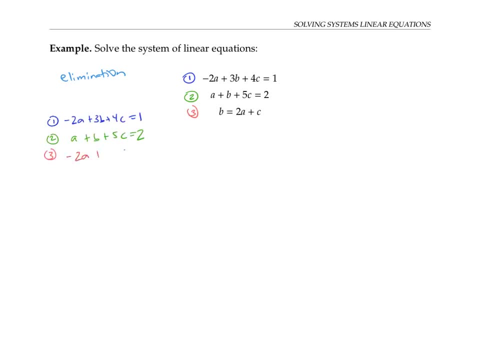 rewrite the third one, I'll put negative two a plus b minus c equals zero as an equivalent equation and standard form. I'm going to try to eliminate my variable a from some of the equations. first, Notice that if I added together equation one and equation two, I wouldn't eliminate the 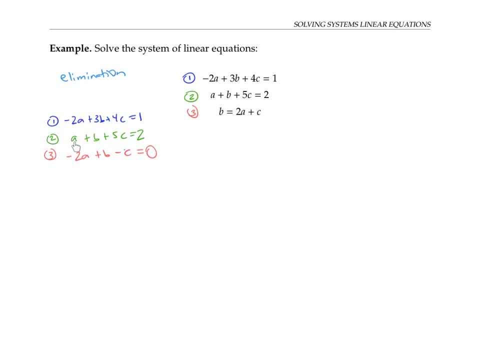 variable a, because I have negative two copies of a here and only one copy of a here, so they wouldn't cancel out. However, if I take my equation one and add twice equation two to it, then I'll have two copies of a to cancel, exactly with these negative two copies of. 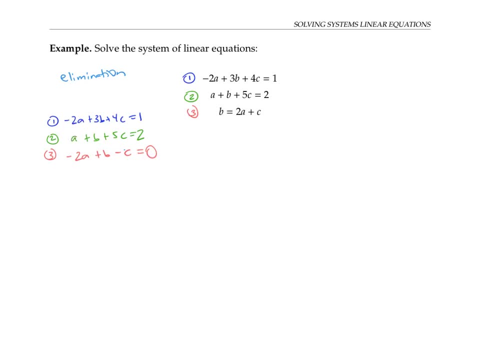 a. So that's what I'm going to do. I'm going to take equation two, twice equation two And once equation one, add them together and put that in the place where I I currently have equation two. So I'll do this over on the side. So I'll just write down my equation one. That's negative. 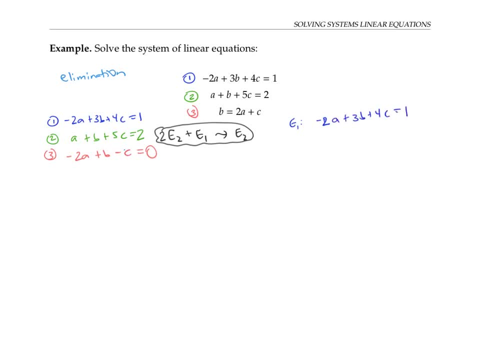 two, a plus three, b plus four, c equals one. And then I'm going to write down twice equation two. So that's two, a plus two, b plus 10.. c equals four, because I had to multiply everything by two. And now I'm going to add these together And I'll get zero copies of a, five copies. 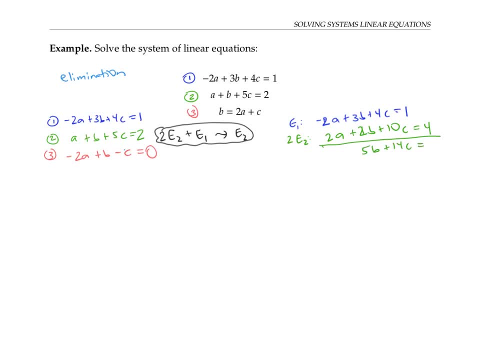 of b, 14 copies of C, and that's going to equal five. So this is what I'm going to put as my new equation to here. I'll write it down here: Five b plus 14 c equals five. My equation one I'm just going to copy down. Now I can do the same trick to replace equation three. 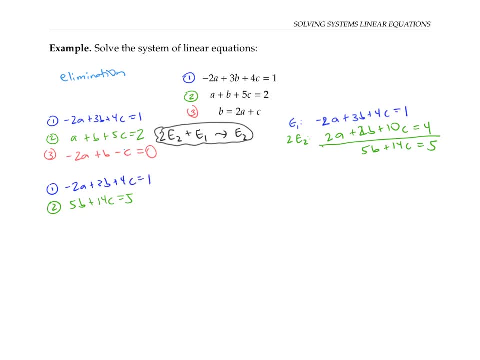 with something where variable a is eliminated. So for example, I could take equation one and subtract equation three and put that where equation three is. there are other things i could do too. For example, I could take twice equation two plus equation three. 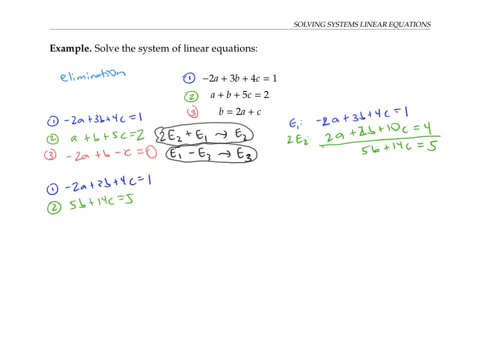 But I'll just do it this way. So that means I'm taking equation one. So equation one negative two a plus three, b plus four c equals one. and I'm going to take equation three Negative: two a plus b minus C equals. 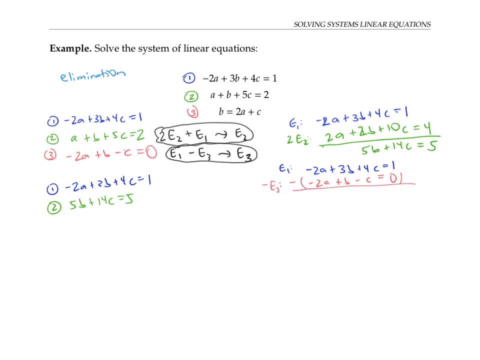 equals zero and I'm going to subtract my A's will cancel. three B minus B is to be four C minus negative C is four C plus C, So that's five C, and one minus zero is one. So this is my new equation: three, two B plus five C equals one. So, as desired, I've gotten rid. 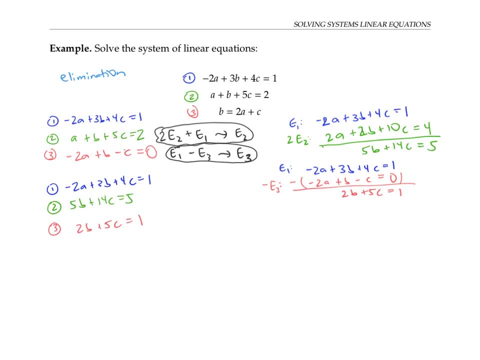 of variable A in the second and third equation. Now I'm going to try to use equation two and three to eliminate another variable, say B. the second equation B has a coefficient of five and the third equation a coefficient of two. So if I take twice equation two, twice, 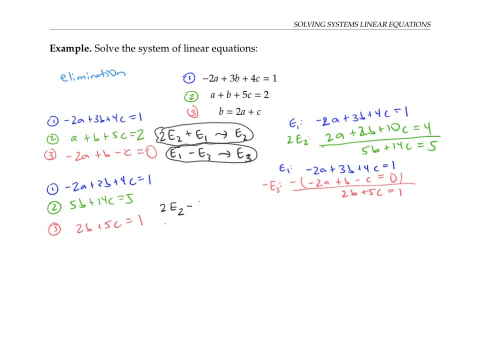 equation two and then subtract five times equation three. those coefficients on B should change. They cancel out. Let's try that. So twice equation two, that's going to be multiplying everything by two. So 10 B plus 28 C equals 10.. And now five times equation three, that's. 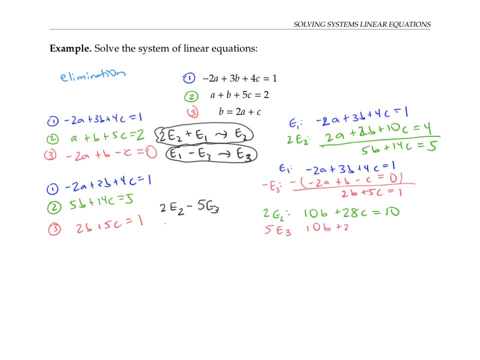 going to be 10 B plus 25 C equals five, but I'm going to subtract that And that's going to give me the B's cancel, as I want three C, because 28 minus 25 is 310, minus five is five, Huh. So I'll copy down my equations From here. it's easy to find: C is just five. 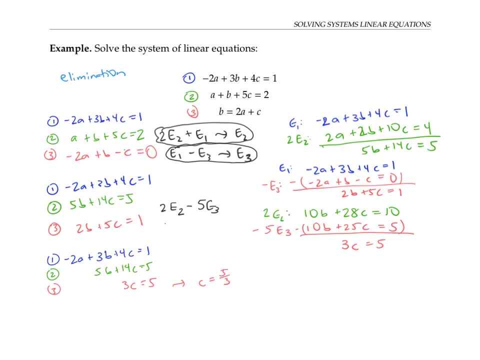 thirds, same as before, And once again I can plug in that number into the second equation to solve for B: 5B plus 14, times five thirds equals five, means that five B is five minus 70 thirds. So that means that 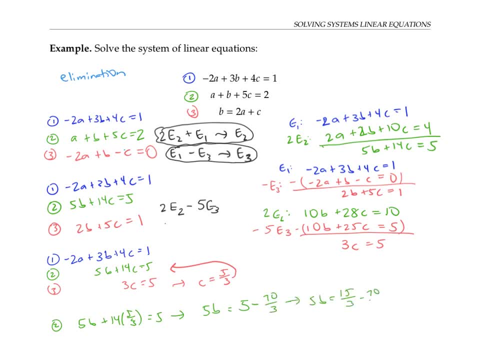 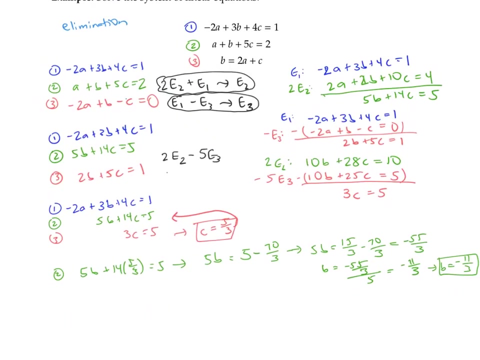 five. B is 15 thirds minus 70 thirds, which is negative 55 thirds. So B is negative 55 thirds divided by five, which is minus 11 thirds. And finally I can plug in both the value of C and the value of B into equation one to solve: for a I have minus two, a plus. 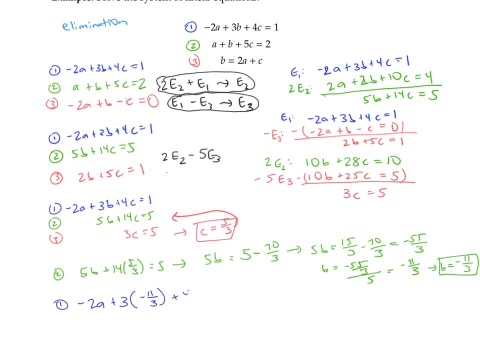 three times minus 11 thirds plus four times five thirds equals one, And when the dust clears, that gives me the value of a as minus eight thirds. So I've finished solving this system of equations using the method of elimination In this video. 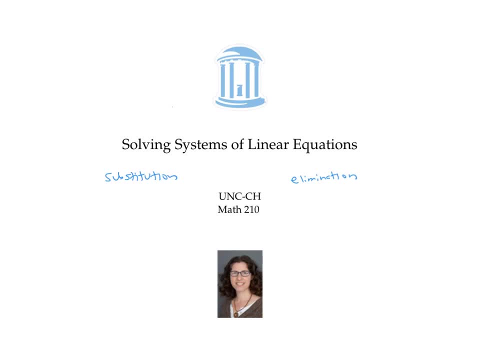 we solve the same system of linear equations in two different ways: First using substitution and then using elimination, And thankfully we got the same answer both times, because math is wonderful like that. So in another video I'll solve the same system of linear 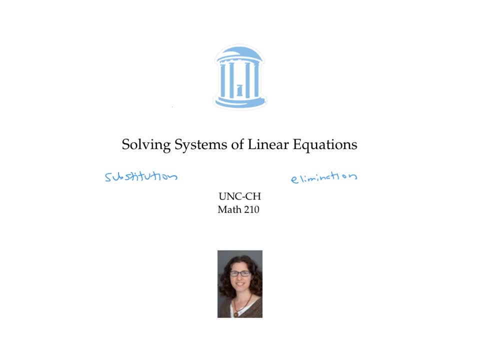 equations yet again in a third way. In this video, we'll code a system of linear equations into a matrix. We'll then solve the system of linear equations in a systematic way, using tricks like adding two equations together or multiplying an equation by a constant. As we solve the system of equations, 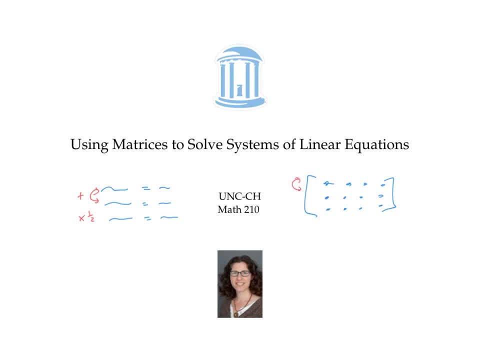 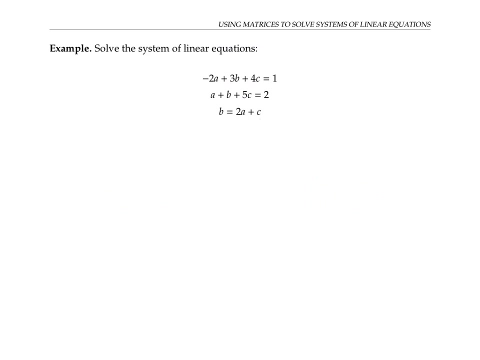 we'll perform equivalent manipulations on the rows of the matrix And we'll see that solving the system of linear equations is equivalent to getting the matrix in a particularly nice form. Here's the system of linear equations that we want to solve. We've got three variables. 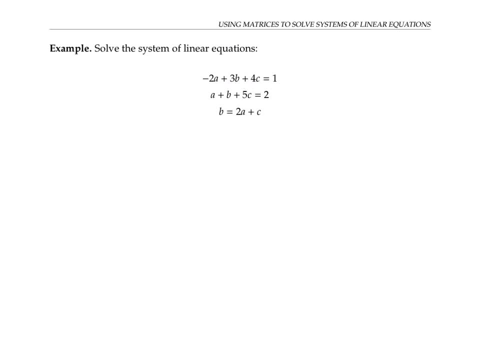 a, b and c and three equations. I'm going to start by rewriting the equations in a more standard form, by making sure the terms with the variables a, b and c are all on the left side in ABC order and the constants are all on the right side. The first two equations are: 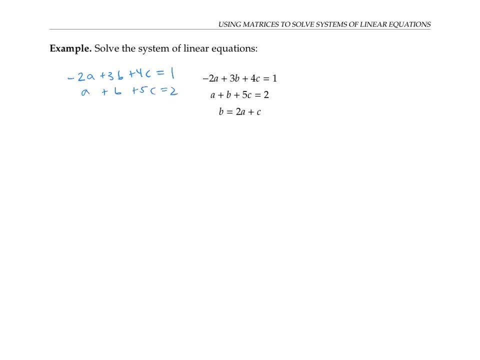 already in that order. But the third equation I'll rewrite as negative: two a plus b minus c equals zero. Now I could write that same information a little more concisely with an array or matrix of numbers, by just recording the coefficients of a, b and c and then the 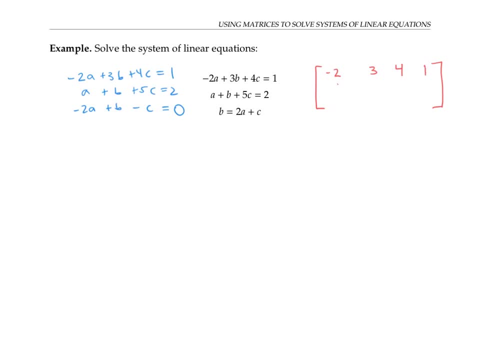 coefficients of a, b and c, And then the coefficients of a, b and c and then the constant term on the right. I'm omitting writing down the variable names themselves: a, b and c. but no information is lost because the order of the numbers, the order of the coefficients, 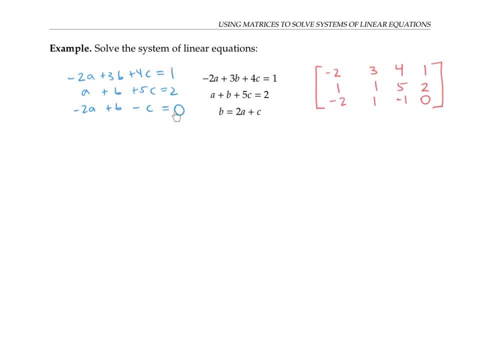 is in ABC order, with the constant terms on the right side of the equations, in the far right column of the matrix. To solve this system of linear equations I'm going to use tricks like adding multiples of one equation to another equation. But the arithmetic will. 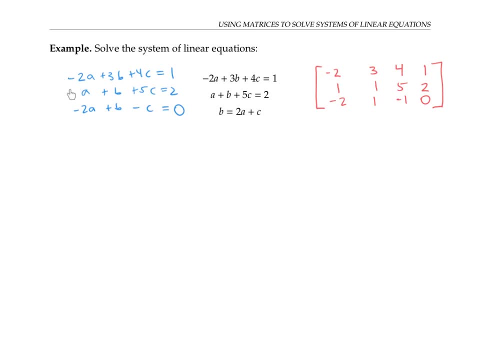 work out. It's a lot simpler if I make use of equations that have coefficients of one in front of my variables. To keep things better organized, I'm going to actually switch the order of these two equations, So I'll just copy down my equations Over on the matrix side. this: 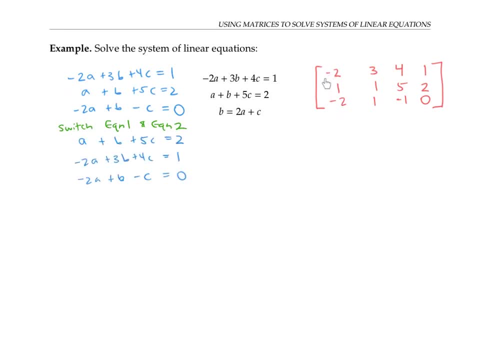 is equivalent to just switching the orders of row one and row two. Now I'm going to try to eliminate the variable a in the second and third equations. I can do this by adding twice the first equation to one time the second equation and then replacing equation two with this. 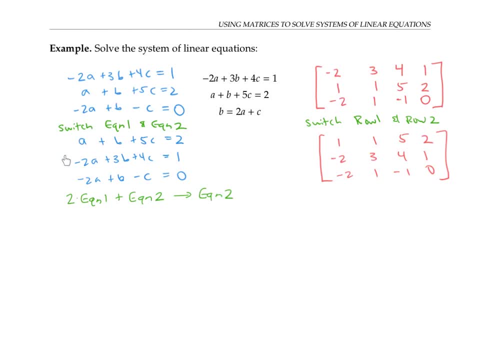 sum. Similarly I can add twice the first equation to equation three and replace equation three with that sum. So first I'll just copy down my equation one, because it's not changing. Now equation two gets replaced with- let's see: negative two a plus two a gives me zero. 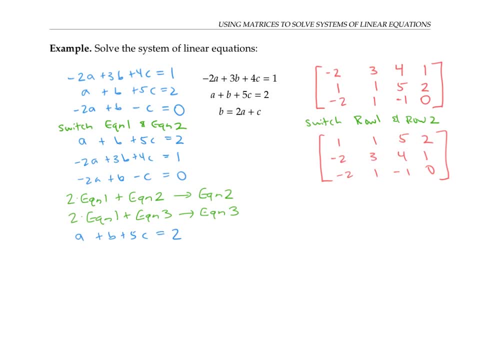 times a, so there's no a term which is equal to negative. two a plus two a times a, So there's no a term. Okay, Which is what I want. Twice b plus three times b is five times b. Twice five times c plus. 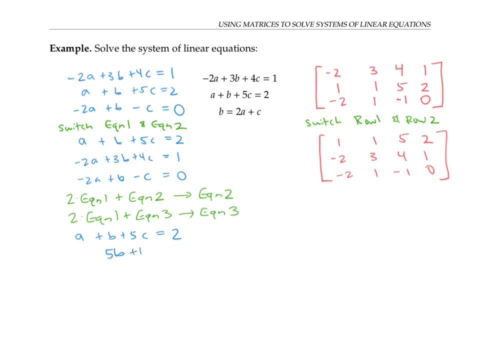 four times c gives me 14. c. And for the constant term, two times two plus one is five. Similarly, I'm going to add twice this first equation to the third equation. Again, that eliminates my a, 2b plus B, which is 3b, And twice five C minus C. that's 10 C minus C, which is nine C. And 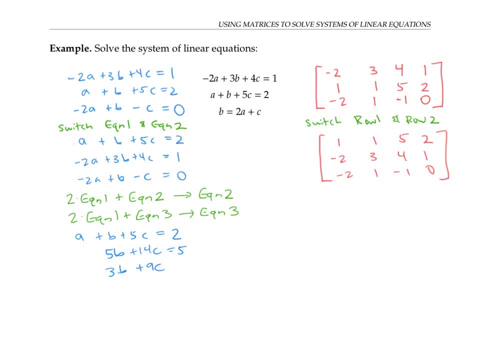 the constant term is twice two plus zero, which is four Over on the matrix side. the same thing would be to multiply twice row one and add that to row two and replace row two with that, And then twice row one plus row three and replace row three with that. 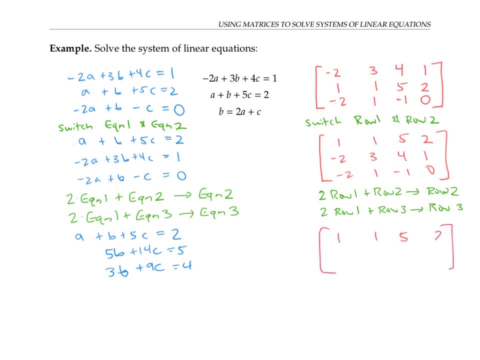 That gives me the first same row, one as before. the second row is going to have: two times one minus two is zero. Two times one plus three is four. Two times five. two times five plus four is 14.. Two times two plus one is five. Same idea. 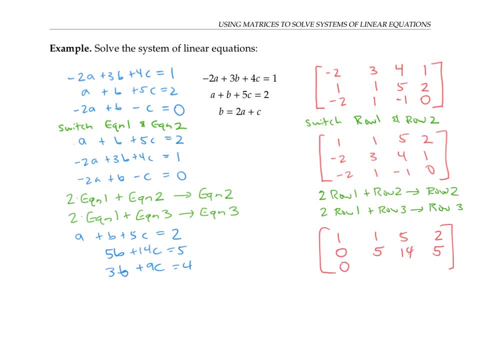 for twice the row one plus row three, zero, three, nine and four. Notice that I've really done the same thing with both the equations and the matrices, And so it makes sense that if I just read off the coefficients of the equations here, I get the numbers in my matrix. 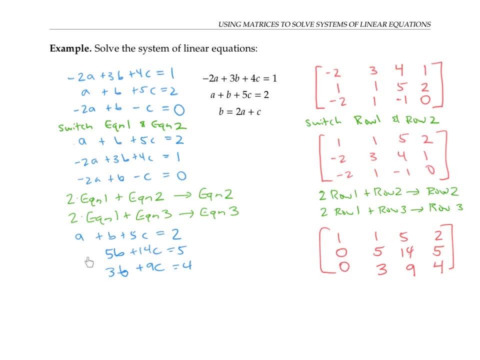 whereas I have zero, Where I'm missing the A altogether in the equations. Now I've eliminated the variable A from the second and third equations. Next, I'd like to use one of these two equations to eliminate variable B from an equation, If one of these equations happen to have a. 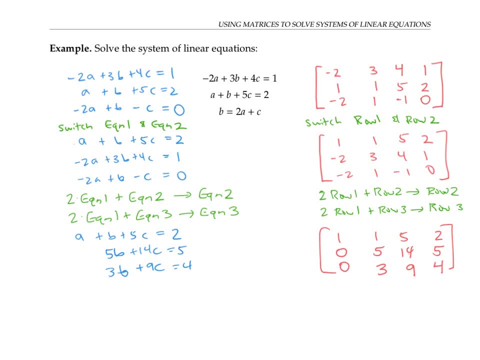 coefficient of one already. I would use that equation because it'd be easy to work with, But since they don't, I'll just use the second equation and make it have a coefficient of one in front of the B By multiplying it by one fifth. In other words, I'm going to take equation to multiply it. 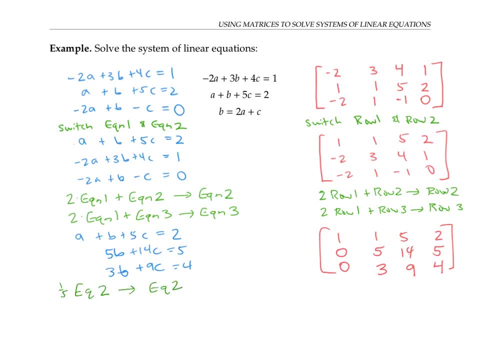 by one fifth and replace equation two with that. So I'll copy down the other two equations on changed and replace the second equation with a fifth of it. So that gives me B plus 14, fifth C equals one. of course I can do the same thing on the matrix side by taking 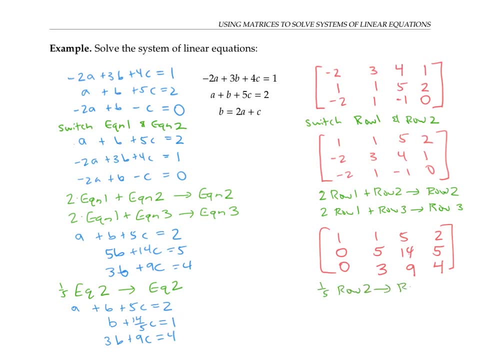 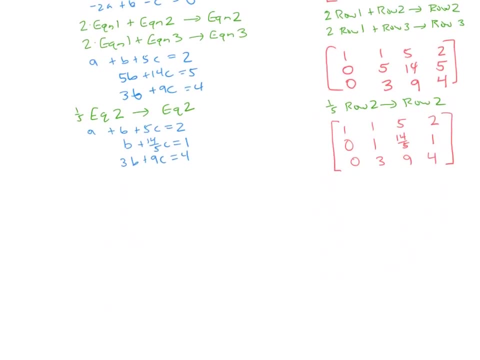 one fifth of row two. two and replacing row two with it. Now I'm in a position to use equation two to eliminate the variable B from equation three. I can do that by taking negative three times equation two, adding it to equation three and replacing equation three by it On the matrix side. 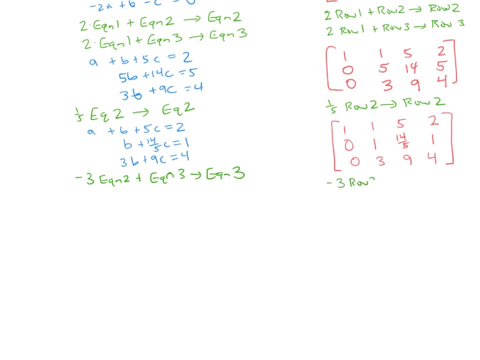 this corresponds to taking negative three times, row two plus row three, and replacing row three by it. For variety, I'm going to do the matrix side first. this time the first two rows just get copied as they are. then the third row gets replaced by negative three. 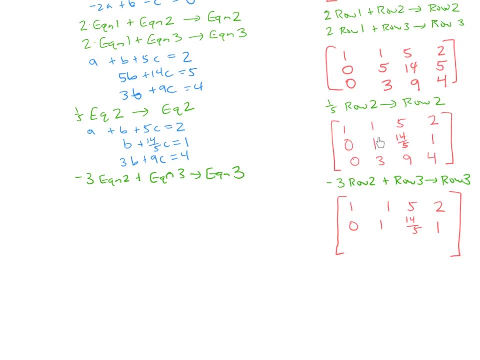 times the second row plus the third row, So negative three. well, the zeros just stay as zero, because negative three times zero equals negative three, Zero plus 00.. And then negative three times one plus three gives me zero, which was the. 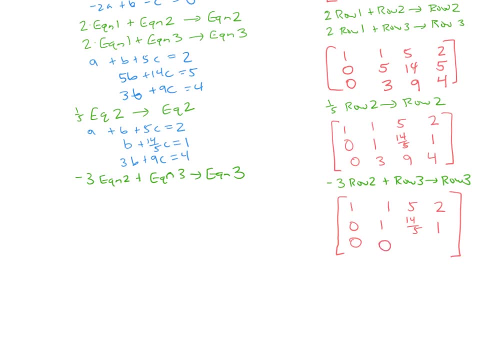 whole point to eliminate that B variable. Now I have negative three times 14 fifths plus nine, So that's a little tricky arithmetic. here Let's see negative three times 14 fifths plus nine, which is 45 fifths. I think this works out to negative 42 fifths plus 45 fifths. 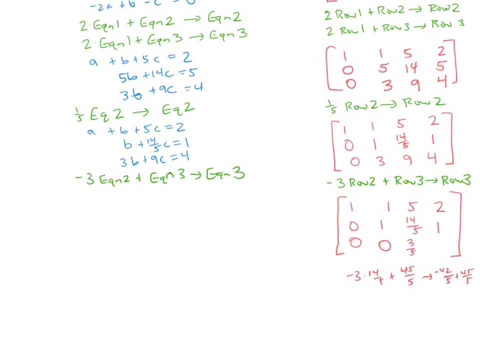 which is three fifths, And finally negative three times one plus four. that one's a little easier. that ups up to one. The work on the equation side is pretty similar, So I'll just write it down quickly. I'm making a lot of progress, because now I have an equation with just C in it. So 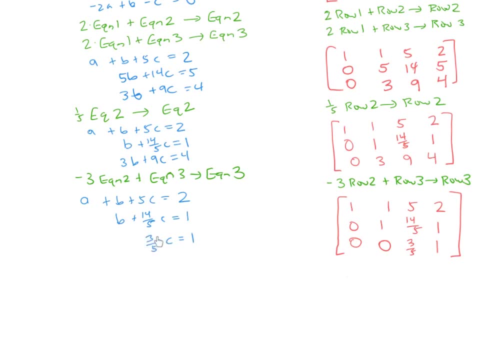 if I multiply that equation by the reciprocal, the coefficient, so by five thirds, I'll have isolated C and solve for C. The first two equations I'll just leave as is for now. I can also do this on the matrix end. Now I've got my system of equations in a nice. 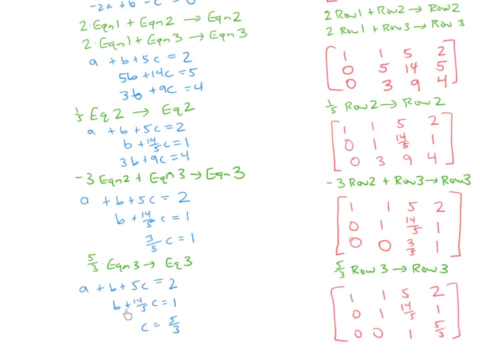 triangular form with all three variables in the first equation, only the last two variables in the second equation and only the last variable in the third equation, where the leading variables all have coefficients of one. Similarly, on the matrix side I've got a bunch of zeros. 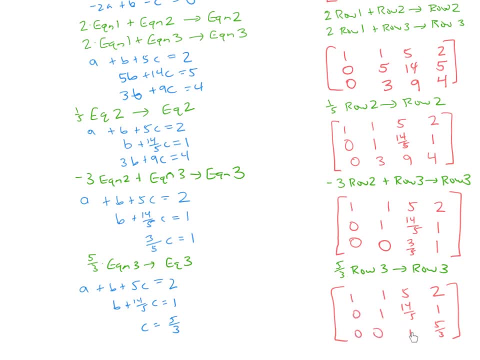 in the bottom left triangle with ones along this diagonal. In the next steps I'm going to work my way back up the equations by using this happy third equation to eliminate C from the first and second equations, and then using equation two to eliminate B from the first. 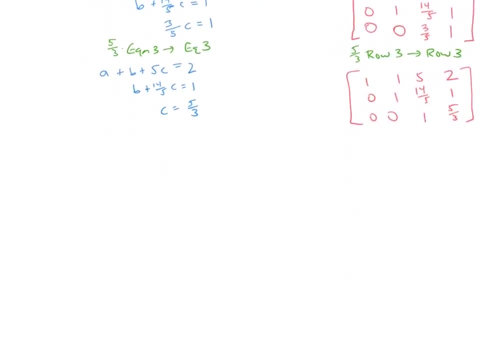 equation. Let me grab a little more space. To eliminate C from the second equation, I'll need to add the second equation to negative 14 fifths. a third equation that I'll make the coefficients match On the matrix side. I'll take row two minus 14 fifths row three and replace row two. 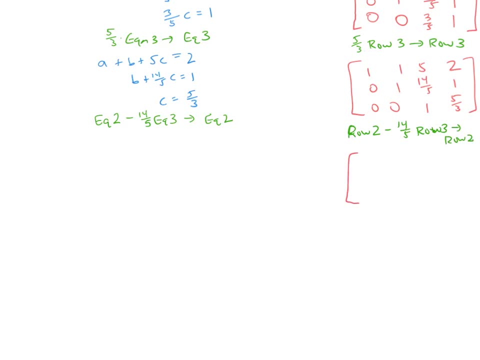 with that, I'll do the matrix side first. So row one and row three don't get changed. So I'll just copy those down, And now I'll fix up row two. So let's see zero minus 14 fifths, zero is still zero. 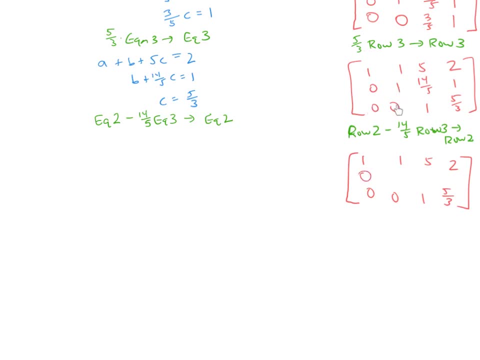 And if I do one minus 14 fifths zero, that's still one, So those haven't changed. The next piece: 14 fifths minus 14 fifths times one. that equals zero, like I wanted it to be. 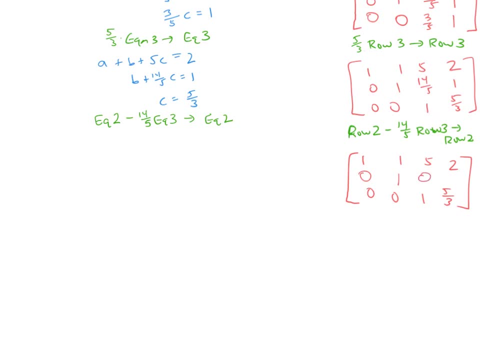 And finally, the real content here is that I'm going to take one minus 14 fifths times five thirds. So that is simplifies to one minus 14 thirds, which is three thirds minus 14 thirds Or minus 11 thirds. So that's what goes in this space here, If we did it with equations. 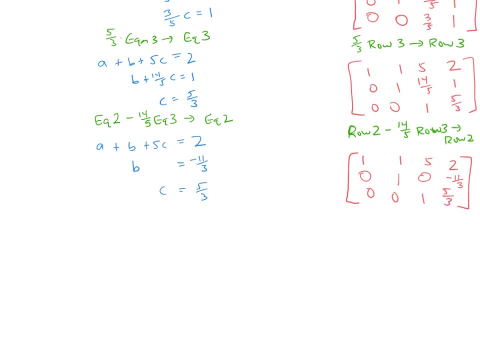 we'd be going through the same process. Now we've actually solved for both B and C And I still need to eliminate C from the first equation and B from the first equation to solve for A. eliminate C first by replacing equation one with equation one minus five. 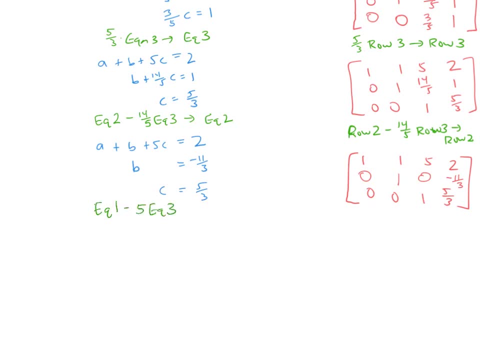 minus five, So that's going to be five times equation three, or the equivalent thing with matrix rows. So when I do equation one minus five times equation three, that's as far as the A terms, that's a minus five times no A's. So that's just a for the B's, it's B minus. 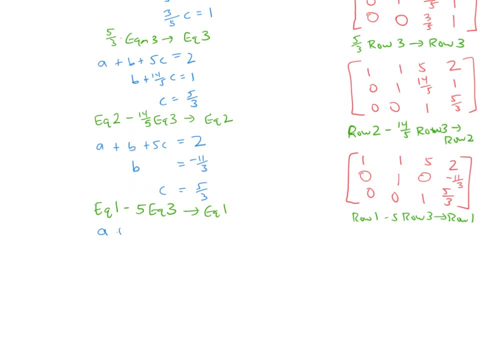 five times no B's, So that's going to be just the B. And here I have five C minus five times C, So that's no C's. I'll just leave a blank for the C's And for the constant term I. 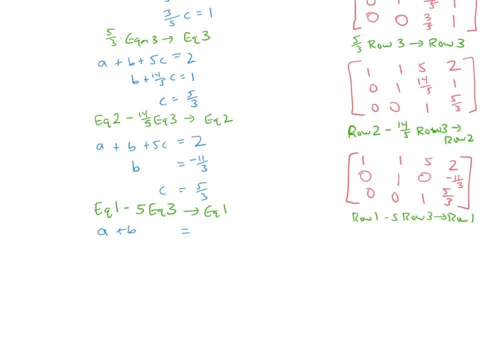 have two minus five times five thirds, That's the same as six thirds minus 25 thirds, which is minus 19 thirds. So minus 19 thirds here, and I can copy the other two equations down- The equivalent thing happens on the matrix side. 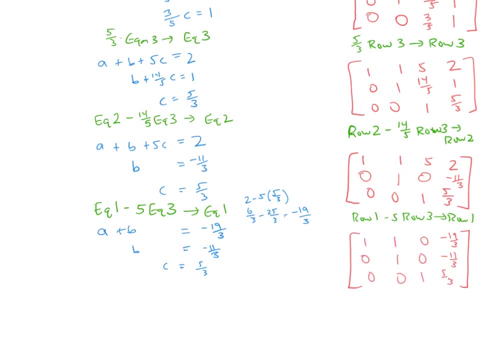 Then, finally, I'll eliminate B from the first equation by adding the first equation and minus the second equation. So let's see, I get A plus B minus B. that gets rid of the B and leaves just the A on the left side, And on the right side I'm going to do minus. 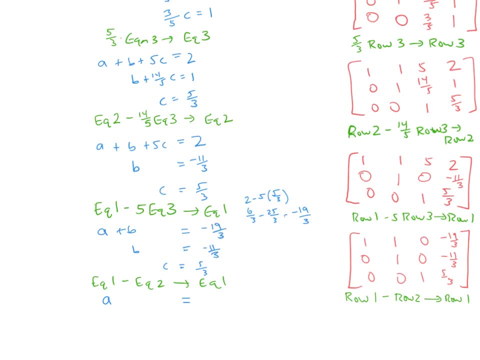 19 thirds minus negative 11 thirds. So that's minus 19 thirds Plus 11 thirds, which is minus eight thirds. on the right side, Same thing happens to the first row on the row side, 100 minus eight thirds, and the other rows or equations just get copied down, Notice. 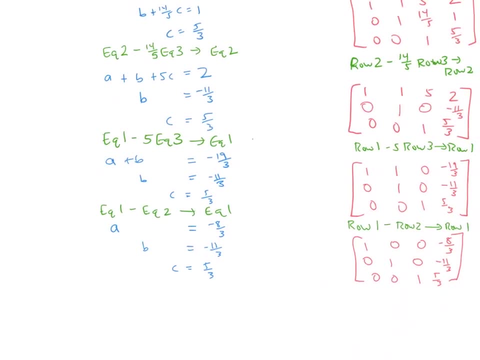 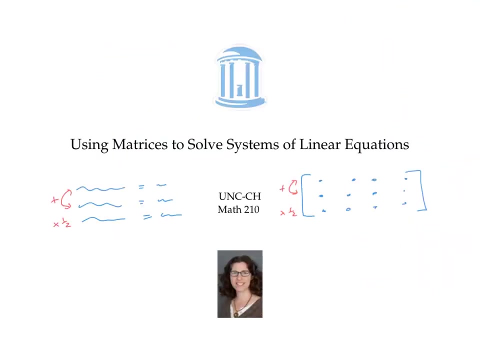 that now I can very easily read off my solution from my equations. But I can also read it off from my matrix: one times a equals negative eight thirds, one times B is negative 11 thirds and one times C is five thirds. To solve our system of linear equations we use three operations. 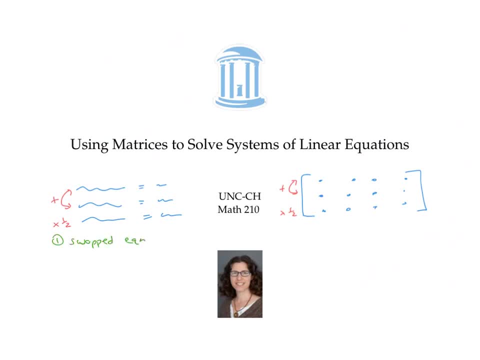 we swapped the order of equations. we added multiple- a multiple of one equation- to another equation And replace an equation with that, And we multiplied an equation by a constant. we can similarly use these operations on the matrix form of the system- equations- by swapping rows. 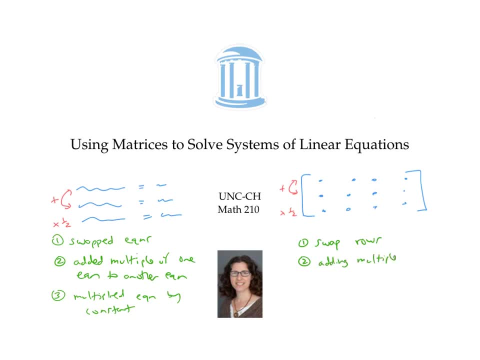 adding multiple of a row to another row and multiplying a row by a constant. By applying these operations systematically, we can end up with a matrix that just looks like ones and zeros, with the solution to the system over in the far right column. This corresponds to solving our system of equations and getting answers for A, B and 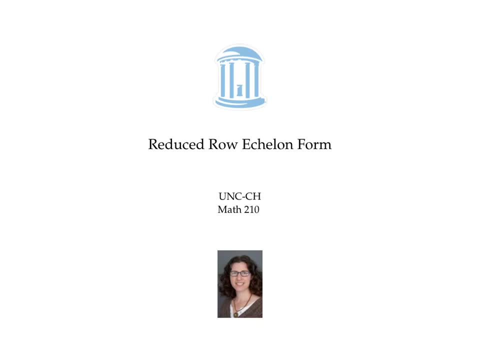 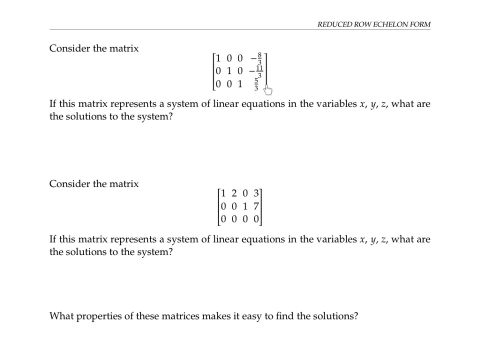 C. This video introduces a form of a matrix called reduced row echelon form that can be handy when using matrices to solve systems of linear equations. Consider this matrix that appeared in a previous video. If this matrix represents a system of linear equations in the variables x, y and z, then 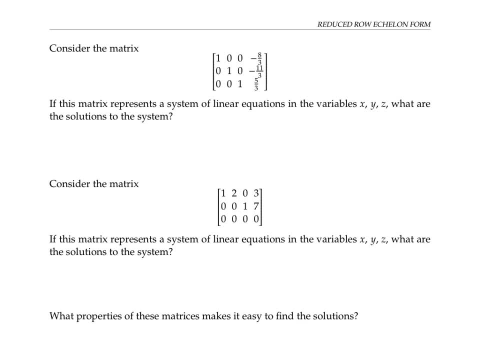 what are the solutions? Well, if it represents a system of equations, then this column represents the coefficients of x, this column is the coefficients of y and this column is the coefficients of z. The final right-nose column represents the constants that are on the right sides of. 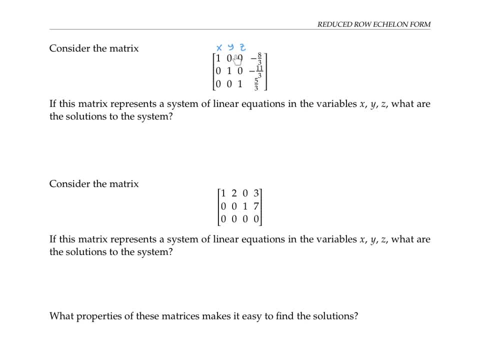 the equations. So if we write out the first equation in the first row, we get that 1 times x plus 0 times y plus 0 times z is equal to negative x. That's negative 8 thirds. In other words, x equals negative 8 thirds. 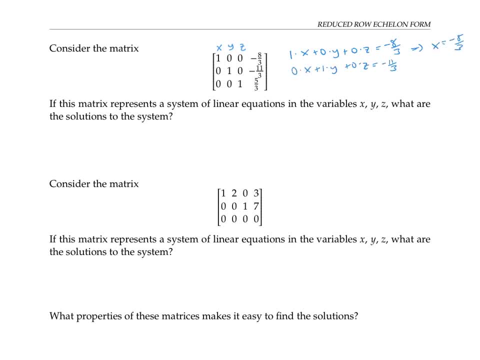 Similarly, if we write out the second equation, we get that y is equal to negative 11 thirds, And the third equation tells us that z is equal to 5 thirds. So this matrix makes it really easy to read off the solution to a system of linear equations. 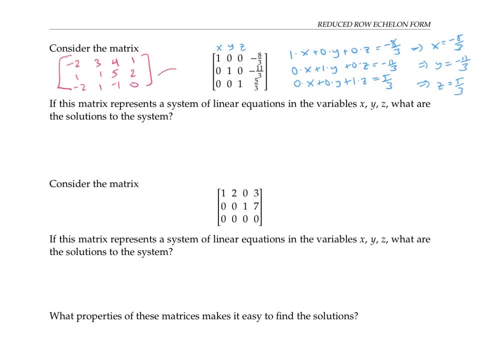 much easier than this other matrix that we transformed into the simpler matrix And that actually has the same solution. Next, let's consider this matrix. If it also represents a system of linear equations in the variables x, y and z, then what are? 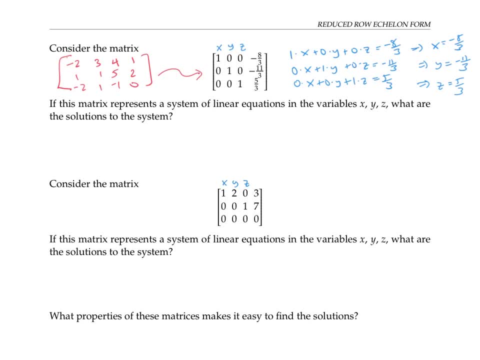 the solutions to the system of equations. If we write out the equations: 1 times x plus 2 times y plus 0 times z equals 3.. 1 times z equals 7.. And the last equation doesn't really give us any negative. 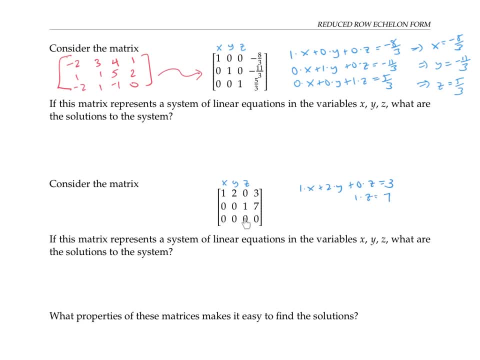 It just says if we use 0 coefficients for all the variables, that adds up to 0.. We can rewrite this equation a little more simply by saying that z equals 7 and x plus 2y equals 3.. There's no unique solution here. 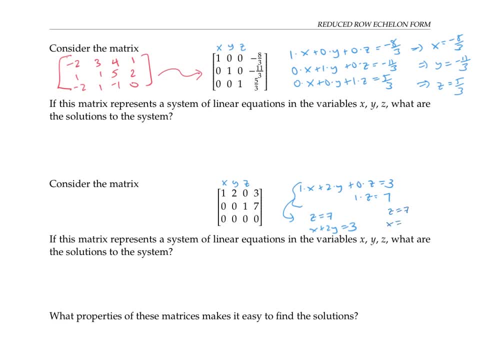 As long as z equals 7 and x is equal to 3 minus 2y, we can make y be anything we want. For example, if y equals 0, then x would be 3.. If y equals 1,, then x would be 1 also. 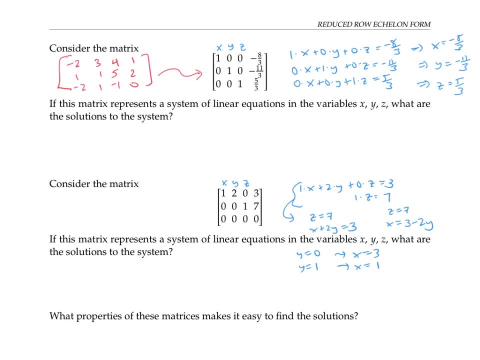 So we have infinitely many solutions. They're just all of the form 3 minus 2y, y, 7, where y can be anything. But it's still pretty easy to read off that information just from the matrix, Much easier than if we were given some other matrix like this one that turns out to actually 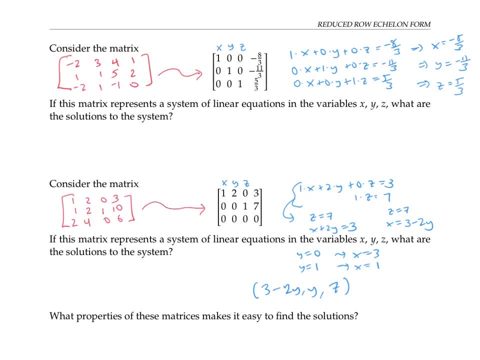 contain equivalent information and have the same solution set. So what properties of these two matrices makes it particularly easy to read off the solution to the associated system of linear equations? One property is the presence of all these leading 1s. The first number in each row, that's not entirely 0s, is a 1.. 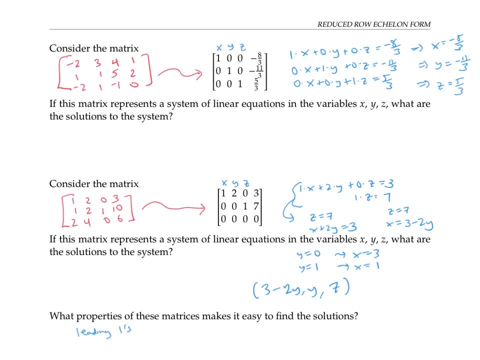 Another property is the presence of lots of 0s. Notice that when For each leading 1.. All the numbers above it in its column are 0s. We'll use these two properties: presence of leading 1s and the presence of lots of 0s. 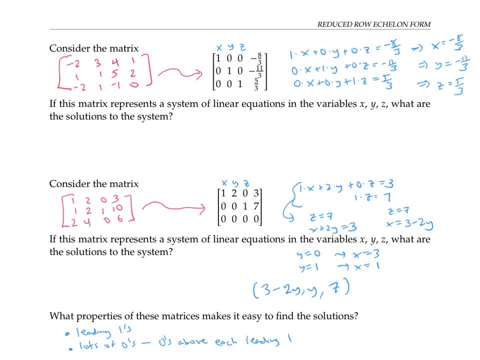 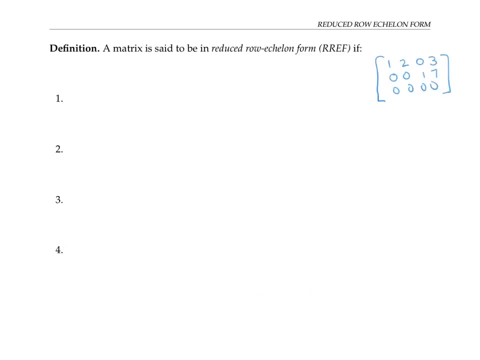 especially above the leading 1s, along with a couple other properties to define something called reduced row echelon form. This is the form of a matrix that makes it particularly easy to read off the solutions for its associated system of equations, A matrix like the ones on the previous page. 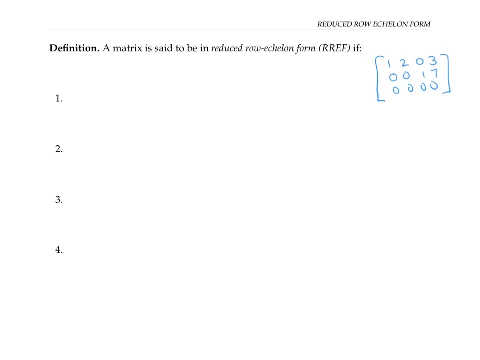 Are said to be in reduced row echelon form, abbreviated RREF, if, first of all, the first non-zero entry on each row that is not entirely 0s, is the number 1. These are called leading 1s. That's certainly true for this matrix. 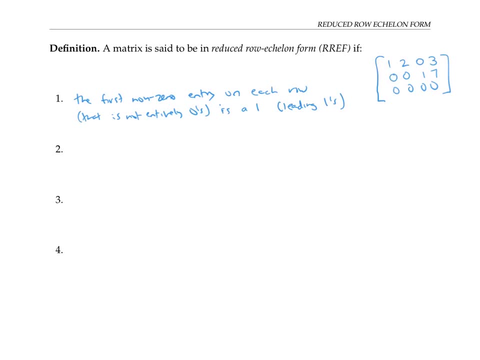 For the two rows that aren't entirely 0s, We're going to call them leading 1s. The first entry that's not 0 is a 1.. Second of all, the leading ones are in descending order. That means that each leading one is to the right of the leading ones in higher rows. 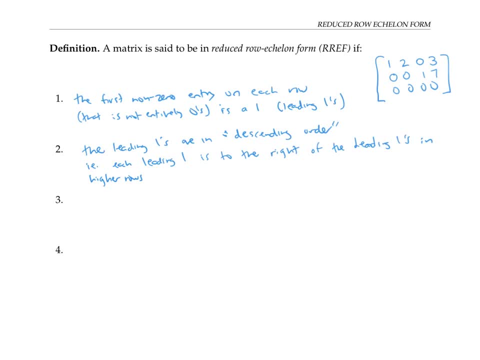 That's also true in this example. This, this leading one, has no higher rows, But this leading one is to the right Of the leading one in the higher row. If I switch the first and second row of this matrix, though, then this property would no. 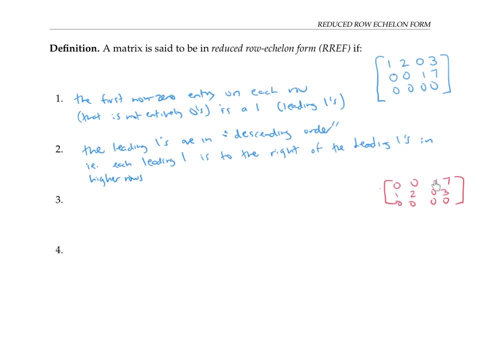 longer hold, because this leading one would be to the left of the leading one above it, not to its right. The third property is that each leading one has a column of zeros above it. In other words, it has a zero above it in every row above it. 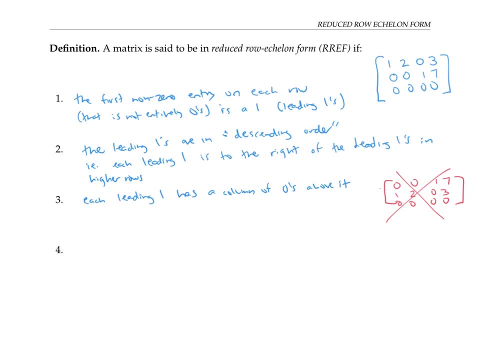 So in this example, This leading one doesn't have any zeros. So in this example, this leading one doesn't have any zeros Above it, and this leading one only has one row above it, but it does have a zero above it in that row. 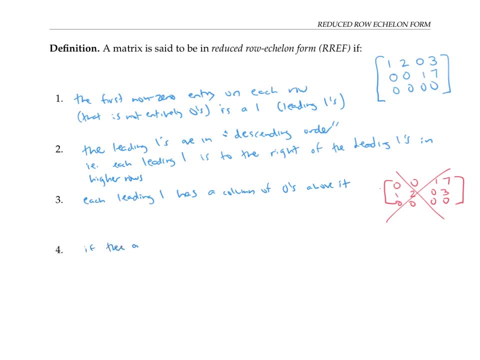 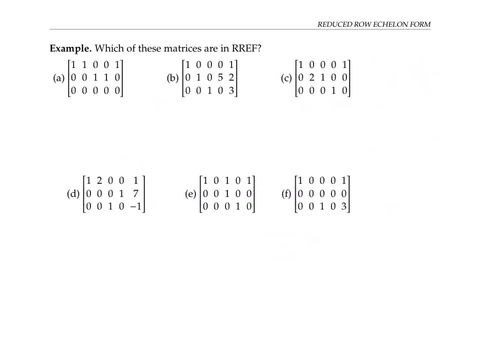 And the final condition is that if there are any rows that are entirely zeros, they must be at the bottom of the matrix, Definitely true in this example. So this example is an example of a matrix in reduced row echelon form. Please pause the video for a moment and see if you can figure out which of these six. 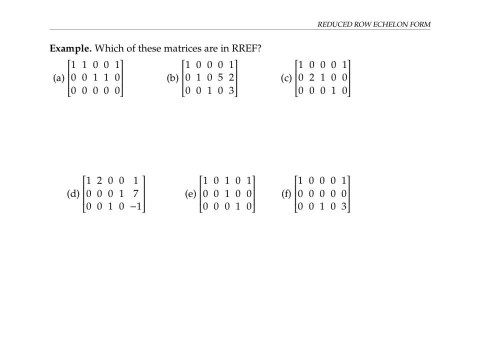 matrices are in reduced row: echelon form. Matrix A is in reduced row echelon form. It has a leading one in every row. that's not entirely zeros. The ones are in descending order. Above each leading one there's a zero column of zeros. 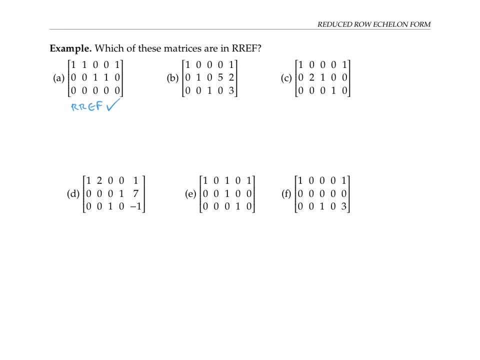 And the rows that are entirely zeros are at the bottom. Matrix B is also in reduced row echelon form. All three of its rows have leading ones. The ones are in descending order, And above each leading one there's a column of zeros. 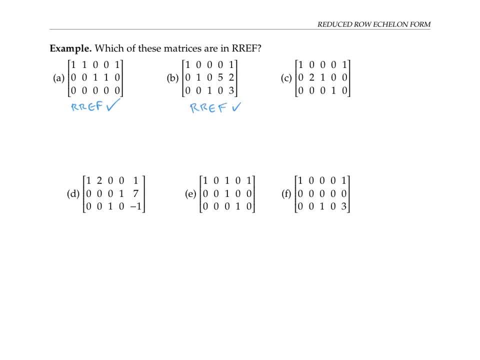 There are no rows that are entirely zero here to worry about. Matrix C is not in reduced row echelon form. Why not? Well, it doesn't have a leading one in the second row. The first nonzero entry of the second row is a two instead of a one. 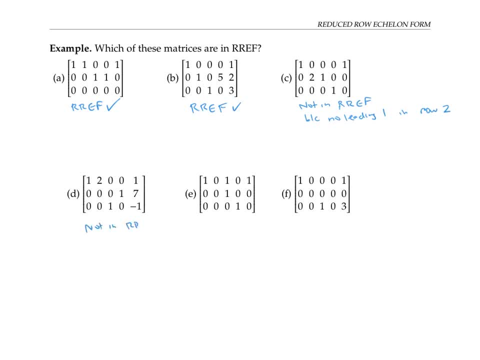 Matrix D is also not in reduced row echelon form. This time, the problem is that the leading ones are not in descending order. This leading one is to the right of the leading one in the row above it, as we want it to be. 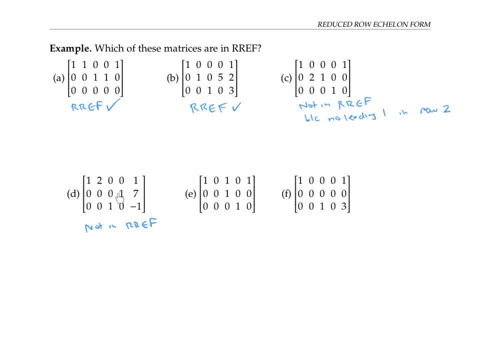 But this leading one is actually to the left of the one, the leading one in the row above it. Matrix E is not in reduced row echelon form. It does have the leading ones And they are in descending order, But we don't always have zeros above the leading ones. 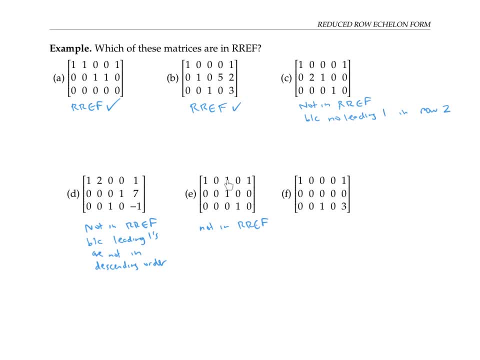 In particular, this leading one has a one above it, not a column of zeros. Finally, Matrix D is not in reduced row echelon form either. This time, it's the simple matter of the row that's entirely zeros is supposed to go at. 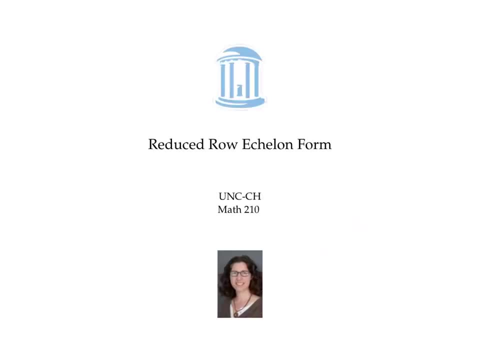 the bottom. In this video we introduced an especially nice form for a matrix called reduced row echelon form. To be in reduced row echelon form, a matrix has to have a leading one in each row that is not entirely zeros. The leading ones have to be in descending order. 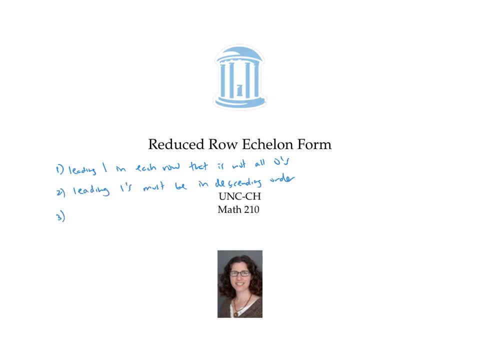 Matrix E is not in descending order. The leading ones have to be topped by columns of zeros, And any rows that are all zeros have to go at the bottom. In a future video we'll practice getting matrices into reduced row echelon form using 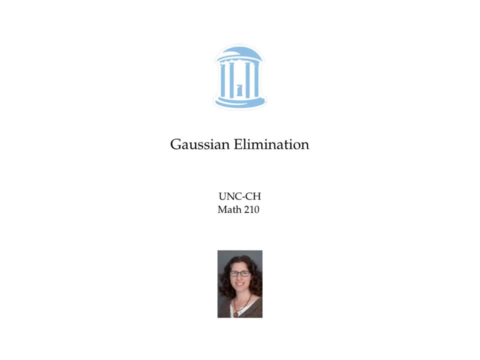 an algorithm called Gaussian elimination. In this video we'll practice converting matrices to reduced row echelon form using elementary row operations. Recall that elementary row operations consist of the following three things: swapping rows, multiplying a row by a constant and adding a multiple of a row to another row. 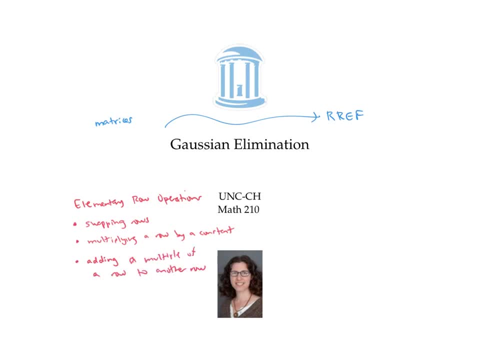 If we think of each row of the matrix as representing a linear equation, then these are exactly the steps we might take to solve the system of linear equations. Recall also that a matrix is in reduced row echelon form if there is a leading one in each. 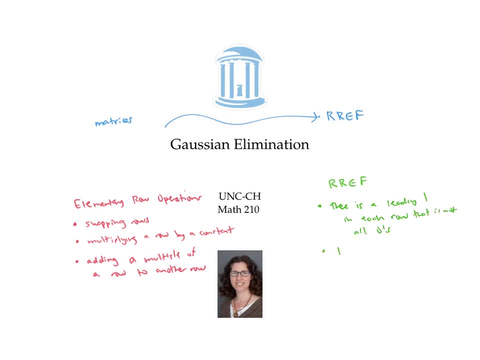 row that is not all zeros. The leading ones go in descending order kind of like a staircase, although there can be some uneven steps. The leading ones have columns of zeros above them And any rows that are all zeros are at the bottom. 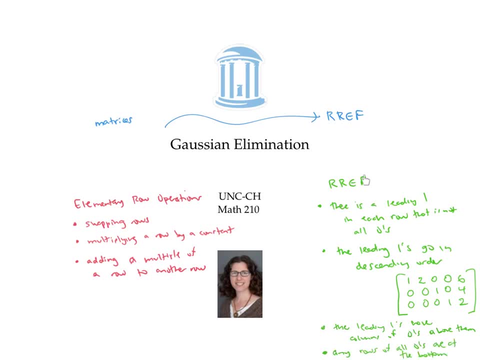 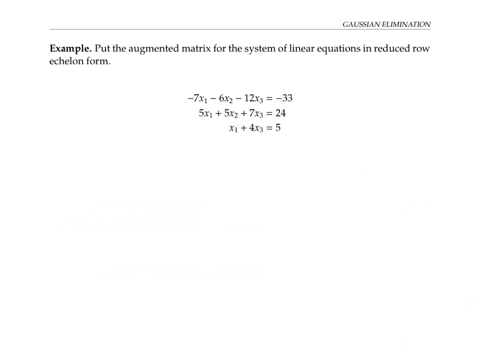 So this is our destination or our goal- reduced row echelon form- And this is our methods of getting there. We'll see, in fact, that any matrix can be transformed to reduced row echelon form using just these elementary row operations, And the algorithm that we'll use to get there is called Gaussian elimination. 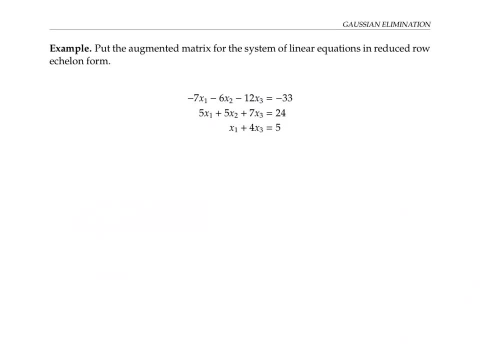 So let's put the matrix for this system of linear equations into reduced row echelon form. The instructions talk about an augmented matrix. All that means is that we're going to write the coefficients of the first variable, x one, in the far left column, followed by the coefficients of x two, the coefficients of x three. 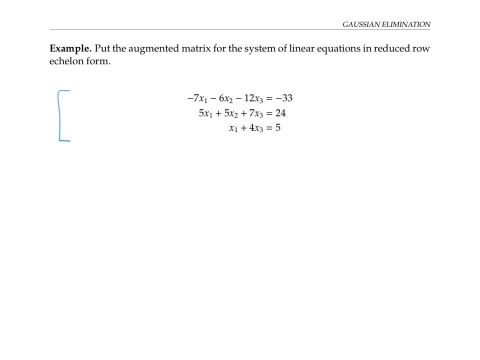 And finally, these constants on the right side of the equations will go in the far right column. The constants can be thought of the additional or augmented part of the matrix. So the first equation becomes the row negative seven, negative, six, negative 12, negative 33.. 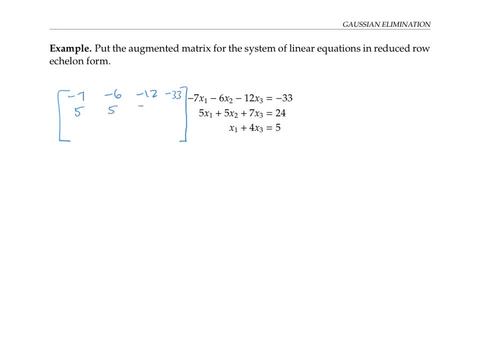 The next equation becomes 55724.. And the last equation becomes one. there's a zero as the coefficient of x two, since x two doesn't appear in this equation. And then four is the coefficient of x three and five is the constant term. 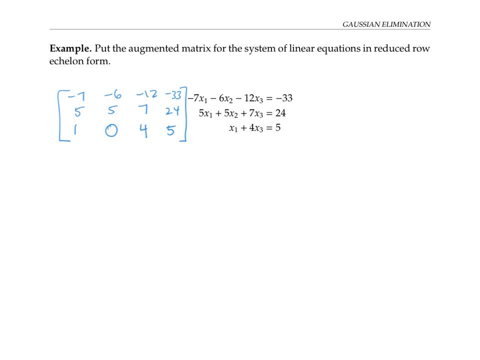 Two, To get this matrix in reduced row echelon form, I'm going to need a leading one in every row. that's not all zeros. Well, I could get a leading one in the first row just by dividing the whole row by negative seven. 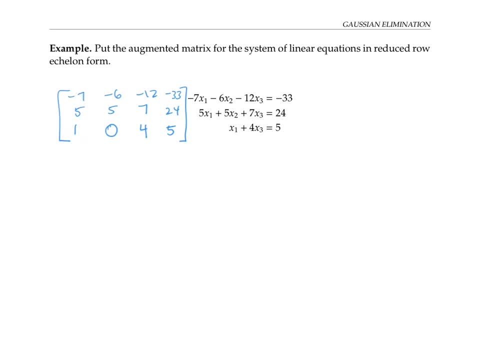 But I think it's going to be easier instead to just swap the first and the third rows, So that'll give me this new matrix. Now I'm going to try to get zeros in the column under this one so that the next leading ones. 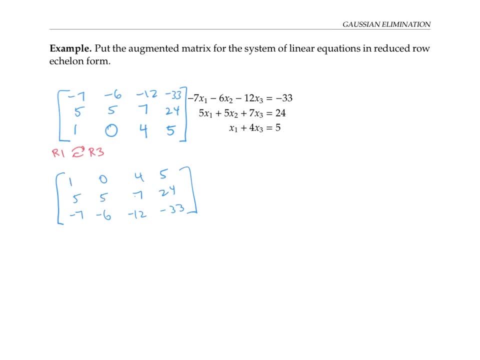 will be to the right Right of this leading one is they're supposed to be. to get a zero in this position, I'm going to take negative five times the first row plus the second row and replace the second row with that sum. So negative five times the first row plus the second row goes to where the second row. 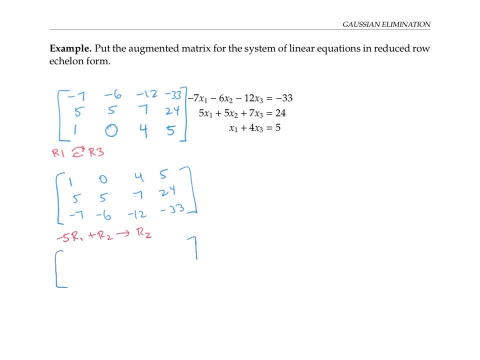 is The first row. I'll just copy over Now in the second row: negative: five plus five is zero. Negative. five times zero plus five is five Negative. five times four plus seven is negative: 20 plus seven. So that's going to be negative 13.. 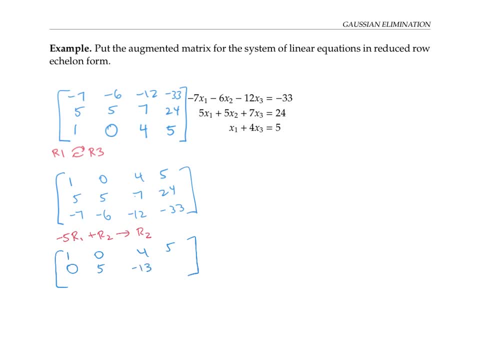 And negative five times five plus 24.. That's negative 25 plus 24.. So that's negative one. I can also get a zero in this position if I take seven times the first row and add it to the third row. 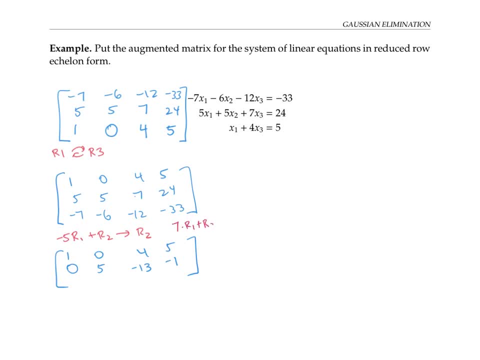 So that's seven times our one. One plus r three goes in the r three position. So that gives me zero negative six. Now, seven times four is 28 minus 12 is going to be 16.. And seven times five is 35 minus 33 is two. 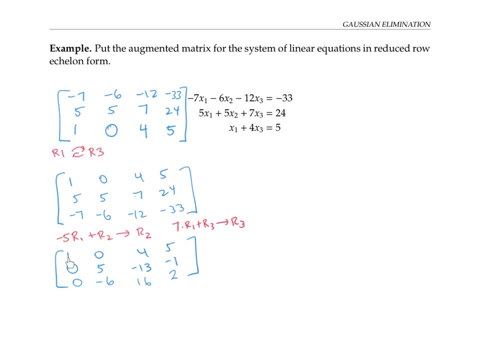 Now that I've got a leading one On the left side of the first row and zeros below it, it's time to worry about getting a leading one in the next column somewhere. There are a couple possible approaches. I could multiply the second row by one fifth. 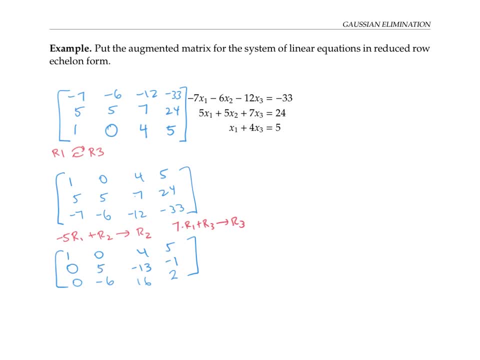 in order to turn that five into a one. But since that will create some nasty fractions, I think, instead I'd like to maybe add together these two rows and replace the The- The say the second row- with their sum. So that's r two plus r three goes in the r two position. 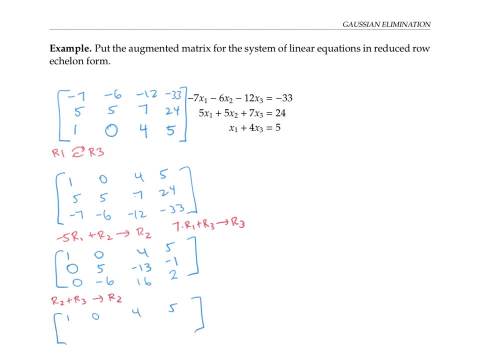 I'll just copy over the first row- I'm not going to change it- And the second row becomes the sums, that zero minus one, three and one. I'll copy the third row down for now too. Now I just have to multiply the second row. 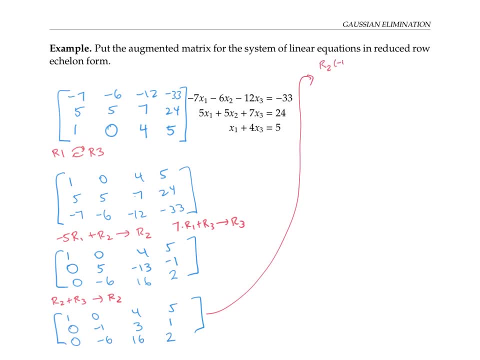 By negative one And I'll have my leading one in the second row. Now I'm going to work to get zeros below this leading one, So I want to get a zero here. So I can do that by taking six times row two and adding it to row 36, r two plus r three. 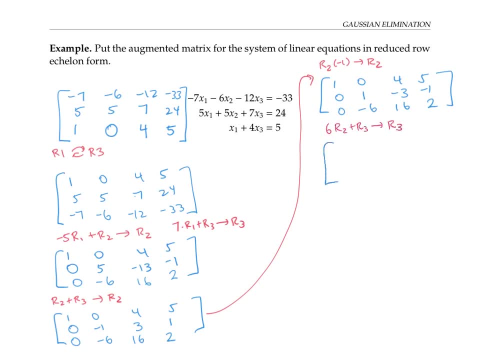 and I'll replace our three with that. I'll copy the first two rows over. And now in the third row, I'm going to copy the first two rows over, And in the third row I'll get six times zero plus. zero is zero six times one minus. 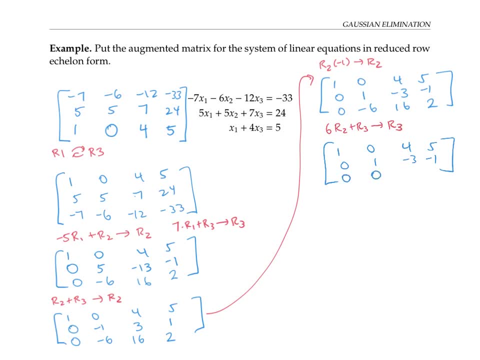 six is zero, like I want it to be. six times minus three plus 16 minus two. six times minus one plus two is minus four. So now I've got a leading one in the first row with zeros below it, a leading one in the second row with zeros below it. 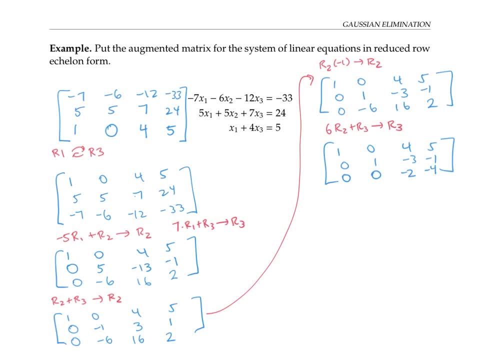 My next job is to get a leading one in the third row, And to do that, I'm going to multiply the third row by one over negative two. That gives me this matrix, which has a leading one in every row, And the leading ones are in descending order. 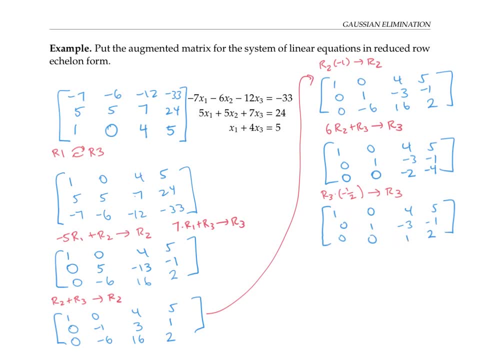 There are no rows of all zeros I have to worry about. But there is one more thing I have to fix. I need to have zeros above each of the leading ones. I'm fine here because there's nothing above it. fine here because there's a zero above. 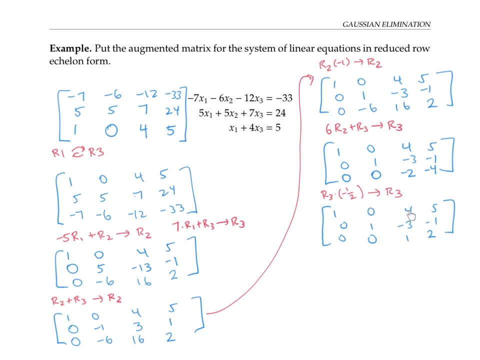 it, But I need to make zeros in these rows above this one. Now I can do that by adding a multiple of row three to each of row two and row one. To get rid of the negative three and row two, I'm going to take three times r three and 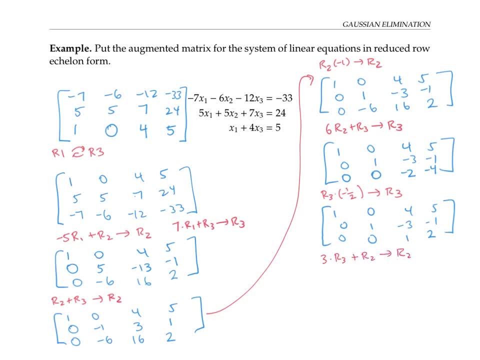 add it to our two and replace our two with that. to get rid of the four in row one, I'm going to take negative four times r three plus r one and replace our one with it. Notice that that won't mess up any of the progress we've made with these leading ones. 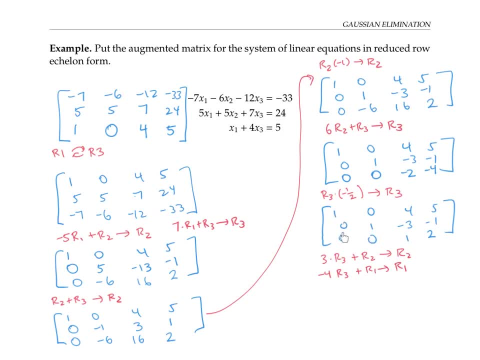 here and all these zeros, because row three just has zeros everywhere before that leading one. So adding a multiple of it to the previous rows won't mess up the the columns over here that have the zeros in them. Okay, so I'll copy the third row down. 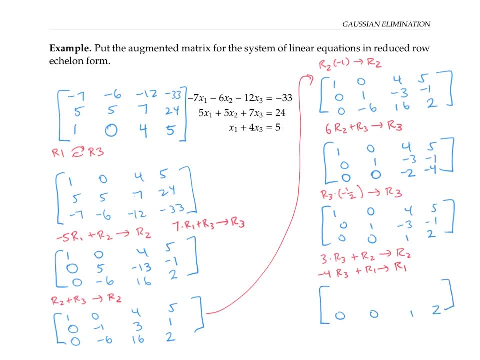 As it is now not making any changes to this. For the second row, I need three times row three plus row two. that's gonna give me 010.. And then three times two plus negative one is going to be six minus one, which is five. 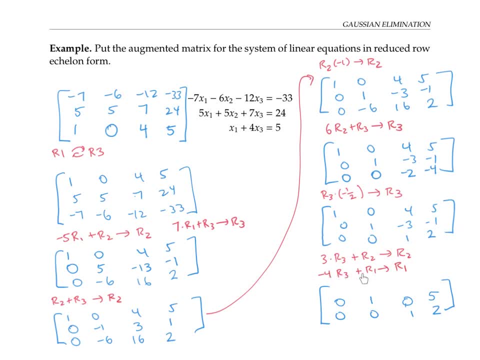 Now the first row gets replaced by negative four times r three plus r one. So that's just one zero zero here, And negative four times two is negative. eight plus five gives me negative three. I now have a matrix in reduced row echelon form. 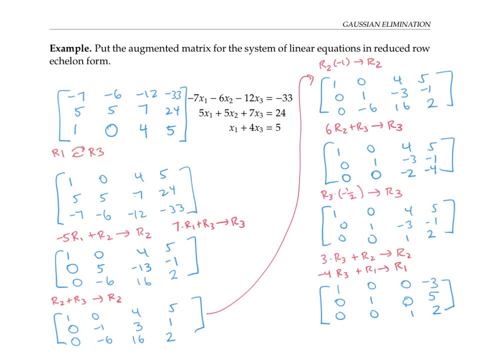 And I can use it to read off the solution to my system of equations. My solution is just: x one is negative, three x two, x one is five and x three is two. So before we leave this problem, let's just review some of the steps we took to get ourselves. 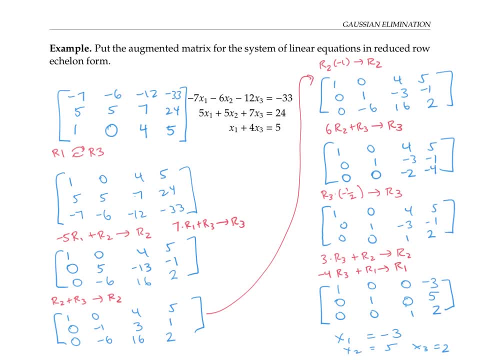 into reduced row echelon form. We first focused on getting a one in the top row and as far left as possible to get a leading one there. Then we got zeros below it By adding multiples of that first row to the first row. Then we kind of moved down and in a bit and focused on getting a one in this next position. 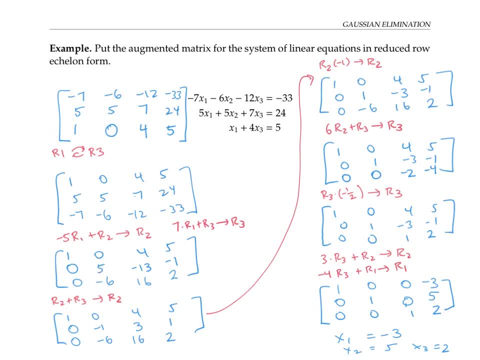 or at least in the second row, as far left as we could. Once we had the one there, we could use multiples of the second row to get zeros below it. Finally, we got a leading one in the third row, as far left as we could. 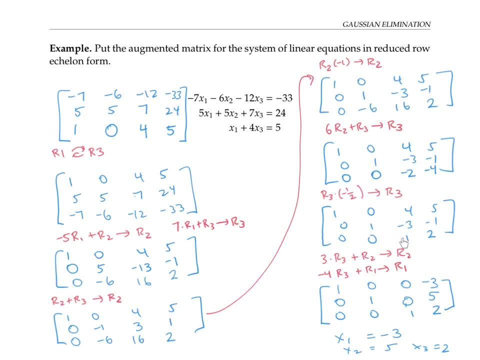 And once we had worked forwards like that to get our leading ones in descending order, we could go forward. We could go back up and get zeros above them, as needed by using multiples of the row to eliminate the numbers in the rows above it. This systematic process that we use is called Gaussian elimination. 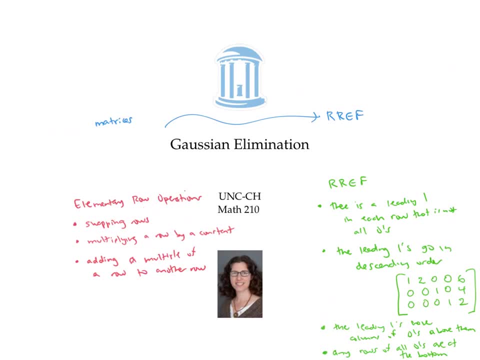 In this video we used elementary row operations to put a matrix into reduced row echelon form in a systematic process called Gaussian elimination. This process is complex and it takes a while to get adept at it, But once you do you'll have a powerful tool for solving systems of linear equations efficiently. 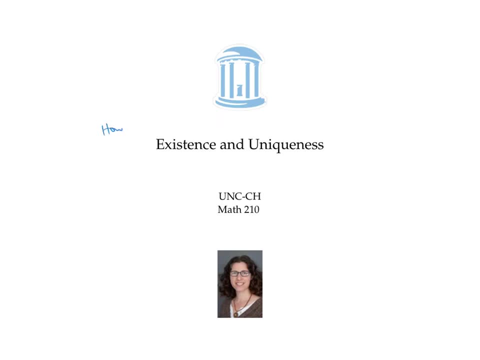 In this video, we'll address the question of how many solutions does a system of linear equations have, And how can we tell? Addressing this question can also be thought of as addressing the existence and uniqueness of solutions, since existence of solutions has to do with having at least one solution. 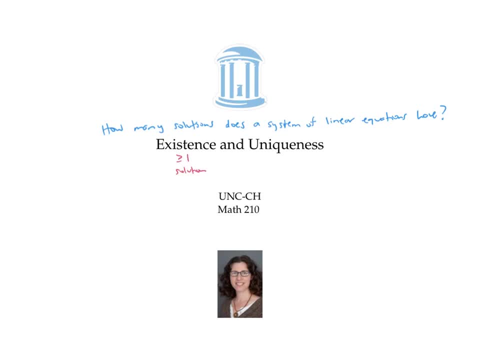 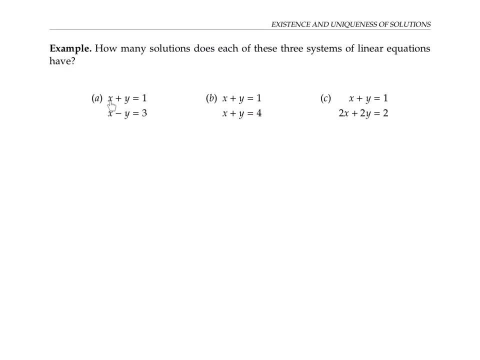 and uniqueness has to do with having no more than one solution. Let's start with some simple examples of systems of equations with two equations and two variables, How many solutions does each of these three systems have? In the first case, if we solve these two equations together by adding them up, we get two x equals. 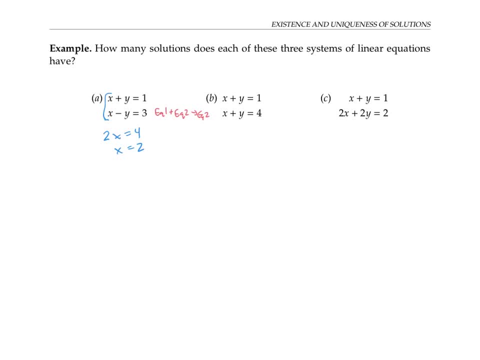 four. so x equals two, and plugging x equals two back into, say, the first equation, gives us two plus y equals one, which means that y is negative one. So here we have a solution: x equals two and y equals negative one and is unique. 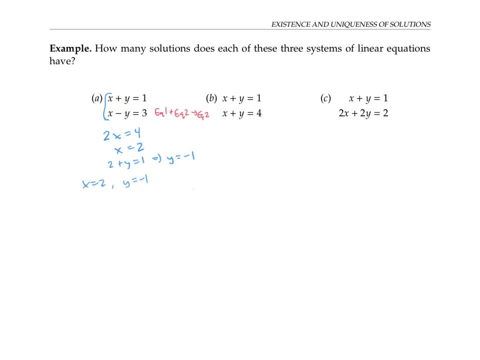 In the second system, it's not too hard to see that there's a problem. We have that x plus y should equal one, but x plus y should also equal four. Well, both of those can't be true, And in fact, if we try to solve these equations together, for example by taking the first, 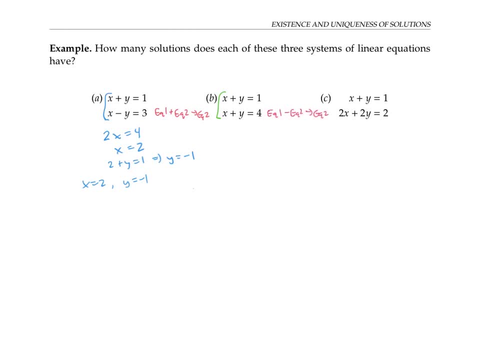 equation and subtracting the second one. By subtracting the second equation we get zero x, zero y equals one minus four negative three. So zero equals negative three, which is definitely impossible. So no solutions exist for this system of equations. 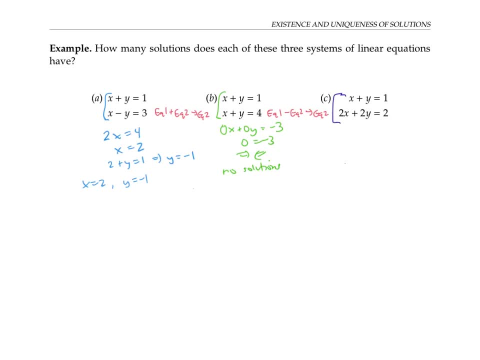 For the third system. you might notice that the second equation really just contains the same information as the first equation. It's just the first equation multiplied by two And in fact if we try to solve these equations together, we get zero x, zero y equals one. 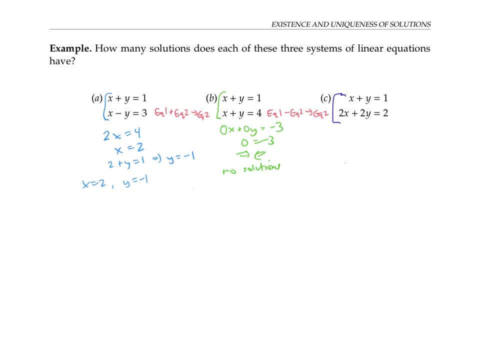 and is unique. So if we try to solve the equations together, for example by taking twice negative two times the first equation and adding it to the second equation, we'll get zero. x plus zero y equals negative two times one plus two is zero. 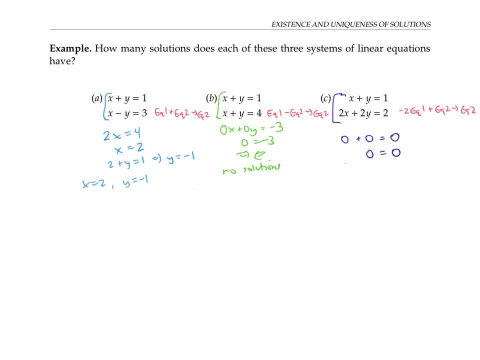 So you just get zero equals zero, which is always true. It doesn't contain any new information. So, in fact, any pairs of x and y that satisfy x plus y equals one will work. So we can think of y as being a double value equation. 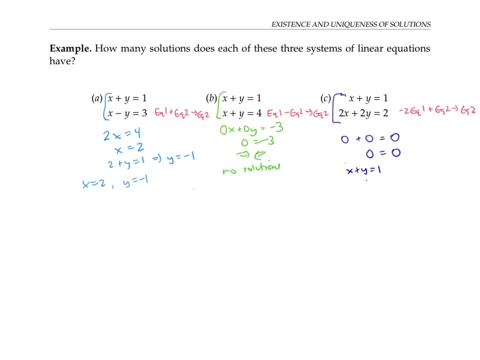 And it should be that way, a free variable. we can set y to anything and then we just need x to equal one minus y. So one way of writing the solution set it's all pairs x, y, where x equals one minus y. 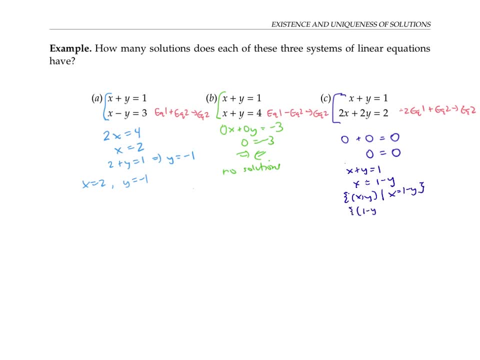 or you can write it as all pairs of the form one minus y, y. Particular examples of solutions might be, for example, if y equals one, then x will be zero, so zero one. or when y equals two, x will be minus one, so minus one, two would be another. 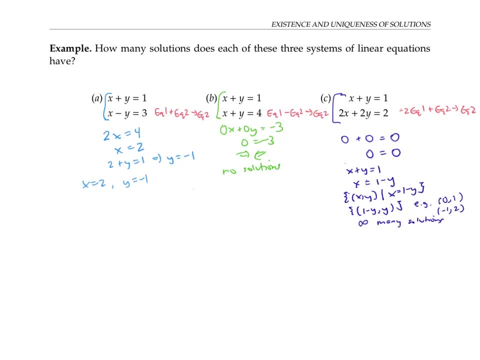 solution. There are infinitely many of these solutions. So we've observed three possible outcomes to solving a system of linear equations: one solution, no solutions and infinitely many solutions. Thinking about these equations as equations of lines in the plane can shed some light on what's going on in these three situations. 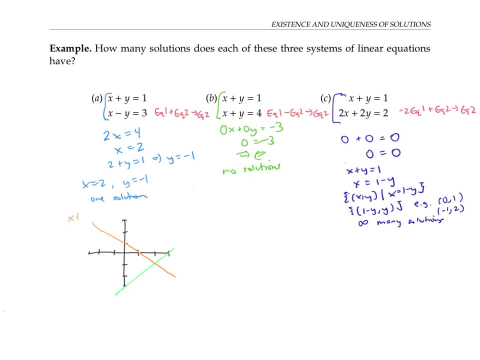 Here's a graph of the equation x plus y equals one, which can also be written as y equals negative x plus one, and a graph of x minus y equals three, which can also be written as y equals x minus three, And you'll notice that those two lines intersect in this unique. 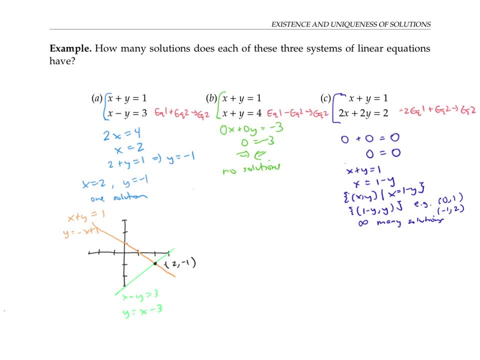 point with coordinates two, negative one. However, when we graph the second set of equations, we get two parallel lines, both of which have slope- negative one- but different y intercepts. therefore, the two lines have no intersection and the system of equations has no solution. 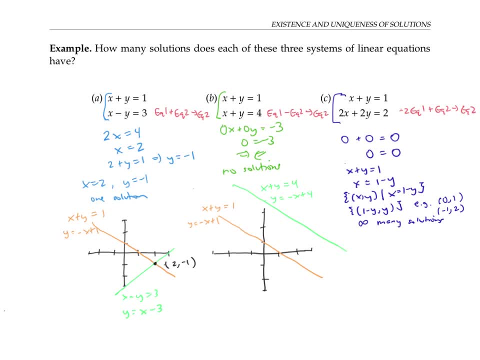 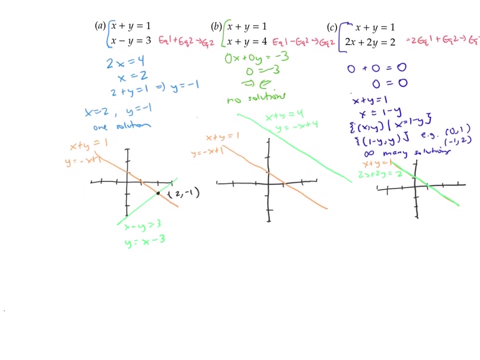 Finally, when we graph these two equations, our two lines are on top of each other, So any point on this line satisfies both equations and there's an infinite number of solutions to the system. Let's analyze these two equations, These three systems, from yet one more perspective. let's write down their augmented matrices. 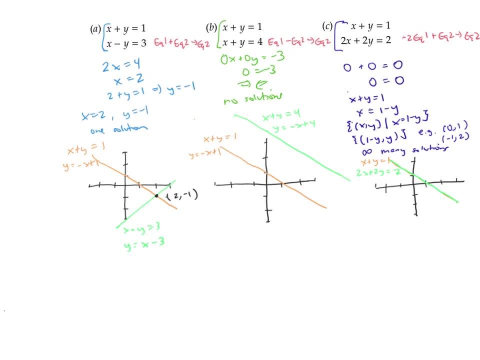 and row, reduce them. Here's the augmented matrix for the first system. Let's take negative one times the first row and add it to the second row, replace the second row with that. we can then multiply the second row by negative one half And finally get rid of this one. 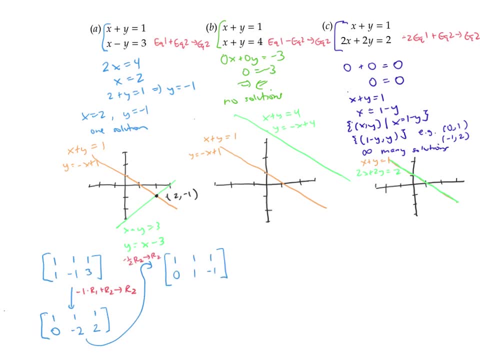 up here. Above that, leading one, by taking negative one times the second row and adding it to the first row, we get a nice matrix in reduced row echelon form where we can read off the solution: one times x equals two and one times y equals negative one. No surprises there, But let's. 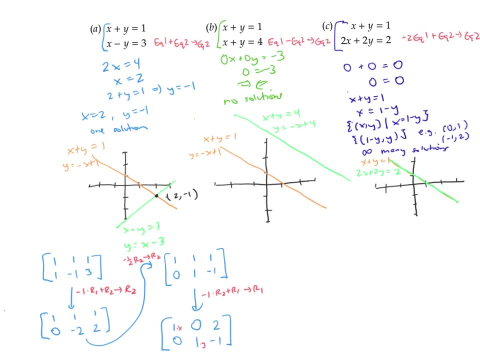 see what happens when we put the next system in matrix form and try to reduce it. So once again, we'll take negative one times the first row And replace the second row with that. we can continue to reduce by multiplying the second row by one third and then subtracting that second row from the first row. we've got something. 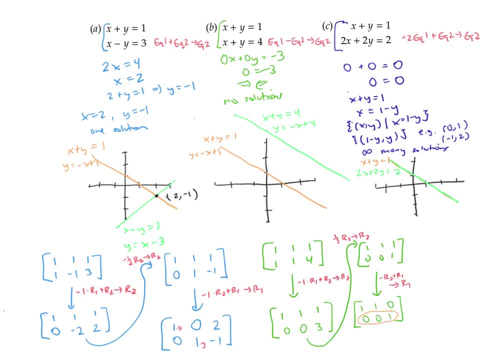 weird going on here. we've got a row that has all zeros in it except a one on the very far right. That's saying that zero times our variables x and y add up to one, So we can get a one, which is impossible. So this weird row with all zeros and a one on the far right. 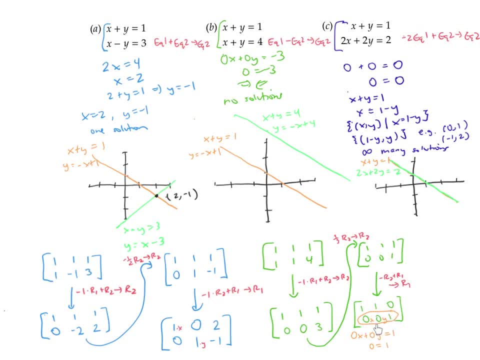 is a signal that we have a contradiction, that we have an impossible system of linear equations with no solution. Finally, if we write down and row reduce the third augmented matrix, notice that in addition to the far left column that has a leading one and the far right column. 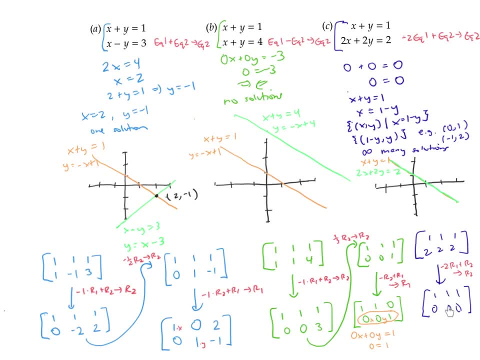 that just represents those constant terms. We have a column, this middle column, that doesn't have any leading ones in it. that's different from this first situation in which all the columns, besides the far right column of constants, all of those other columns had leading ones, Because this second column doesn't have a leading. 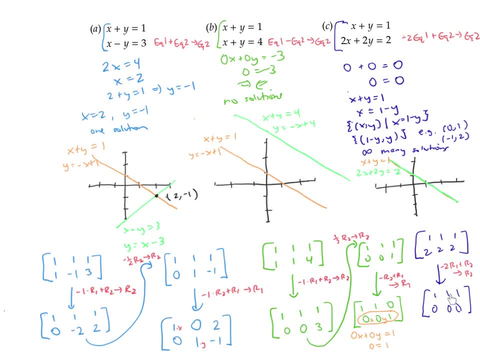 one in it. the variable that it represents, which here is y, is what's called a free variable. it can be anything. So we have no restrictions on y And the only restriction we have is y. The only restriction we have is that one times x plus one times y equals one. So y is free. 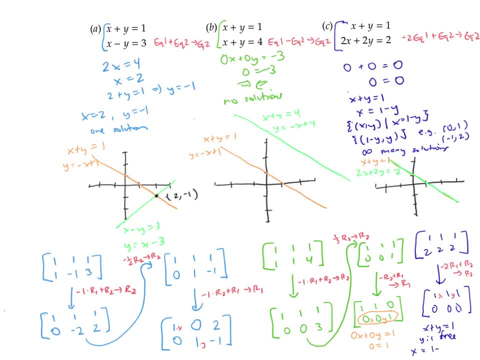 and independent, whereas x, we can say, depends on y. Of course we could have made x independent and y depend on x if we wanted to, But making y the free variable makes it easy to recognize it as coming from the column that doesn't have a leading one. 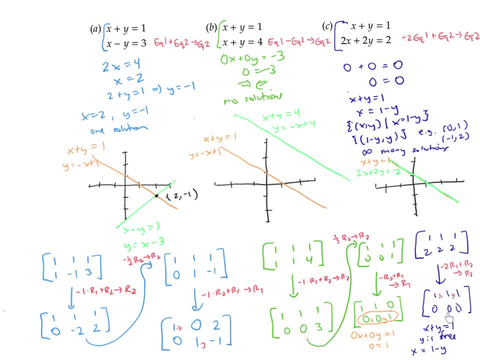 The absence of a leading one in a column is what we'll be looking for as a signal that our system has infinitely many solutions. In fact, the three situations that we see here are the only situations that we can have for any system of linear equations, even much. 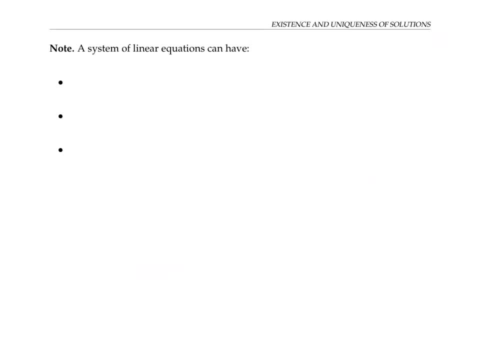 more complicated ones. A system of linear equations can either have one unique solution, or it can have no solutions, Or it can have infinitely many solutions. The systems that have no solutions are called inconsistent systems, while the systems with solutions are called consistent. Let's look. 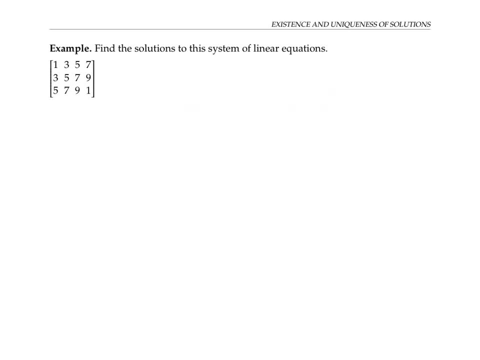 at some other examples. Here we're supposed to find the solutions to a system of linear equations, So we're supposed to interpret this matrix as the augmented matrix of a system of equations In three variables, say x one, x two and x three, with this last column being the constant terms. I'll 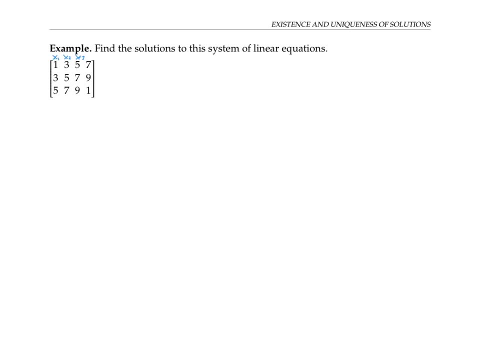 sketch out the row reduction process, but leave the details for you to work out separately. if you're interested Here, I've used the first equation, which already has a one in its leftmost column, to get rid of the coefficients underneath it by adding appropriate multiples. 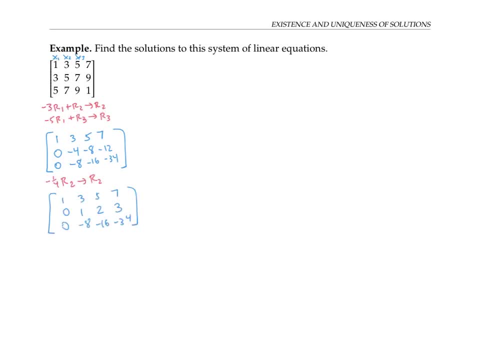 of this first equation to the other equations. Here I've turned this negative four into a leading one just by multiplying the second row by negative one. fourth: Now I use the second row to zero out the entries below this leading one And I turn this leading 10, negative 10, into a leading one by multiplying that row by negative. 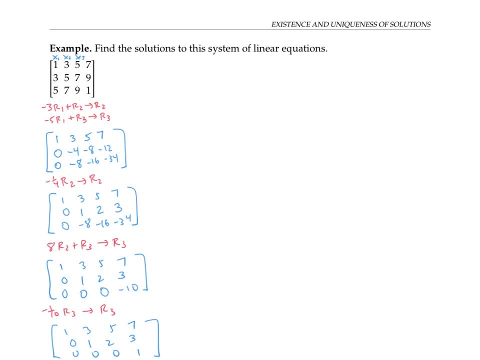 one 10.. Finally, I can zero out the entries above this leading one. Now, on the opposite end, if I tiles, i can output the number from ten to the number five. Well, there we go. here it is All of that công located. Ridley can convert it to negative. help And thanks. 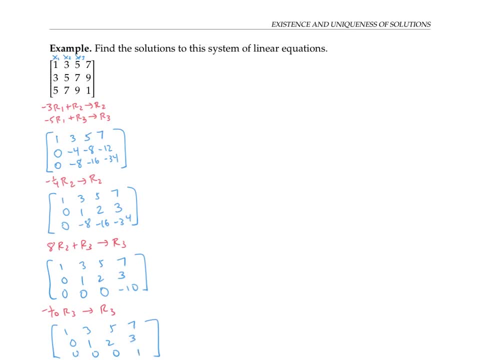 Take care by adding multiples of the third row to these two rows and use the second row to zero out the entries above its leading one. Now that I've got my matrix in reduced row echelon form, what kind of solution set does my system of linear equations have? 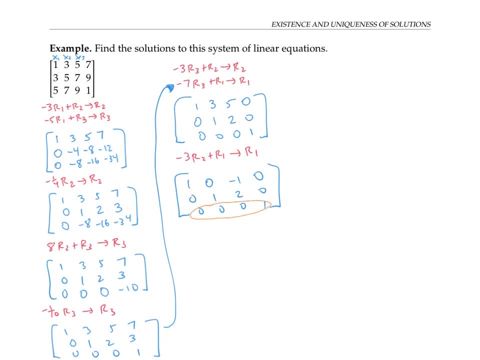 Well, because of this last row, in which all the coefficients of my variables are zero, but the constant term is one, I have a contradictory equation, And so I have no solutions. In fact, I could have predicted this even from this stage of reducing my matrix. 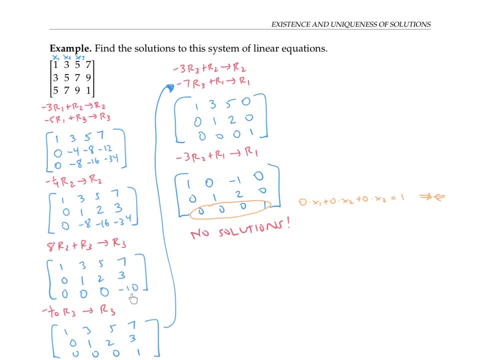 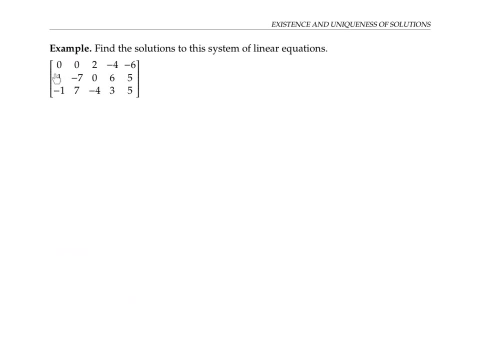 without completing the entire row reduction process. Let's try another example To row reduce. I'll start by swapping my first and second rows. Since I already have a leading one in the first row now, I'll use it to zero out the entries below it, namely this entry in the third row: 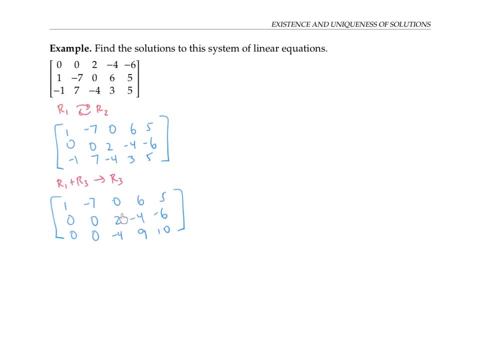 I'll make this leading to a leading one by dividing the second row by two and use the second row to zero out the entries below its leading one. Finally, I'll get rid of any nonzero entries above my leading ones. So my matrix is now in reduced row echelon form. notice that I don't. 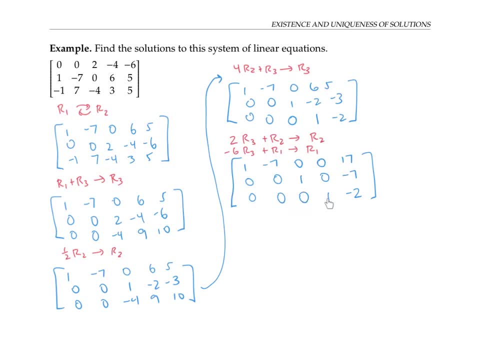 have any of those contradiction rows where I have all zeros and then just a one in my, in my constant column. I don't have any contradiction rows, But I do have some columns that don't have leading ones in them, In fact columns that correspond to variables. I don't. I don't care about this. 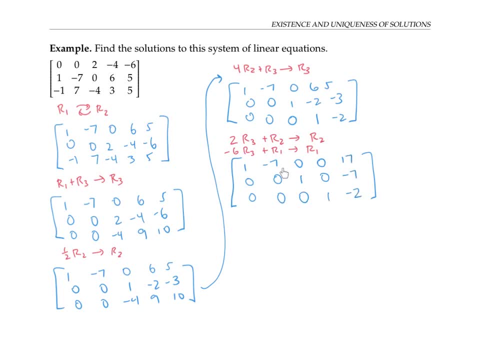 this far right constant term column. But over here I have a column corresponding to the variable x two that doesn't have a leading one in it. So that means that x two can be used as a free variable. I can set it to be any number I like- And x one has the relationship that x one minus. 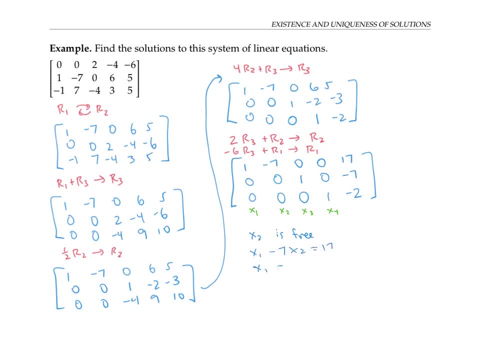 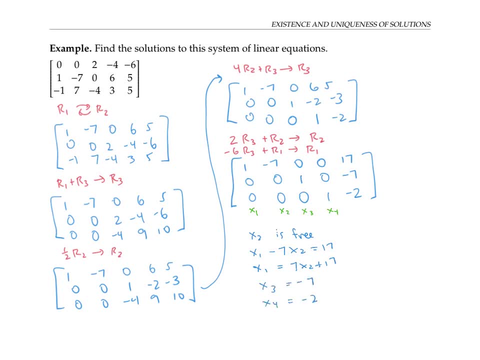 be equal to negative seven, and x four has to equal negative two. So I have infinitely many solutions that can all be written in terms of one free variable, That is, I can write them as x one, as seven, x two plus 17.. x two is just x two, And then 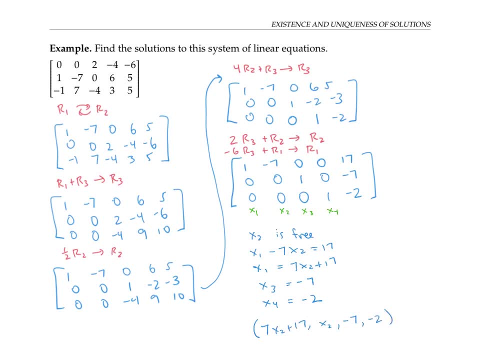 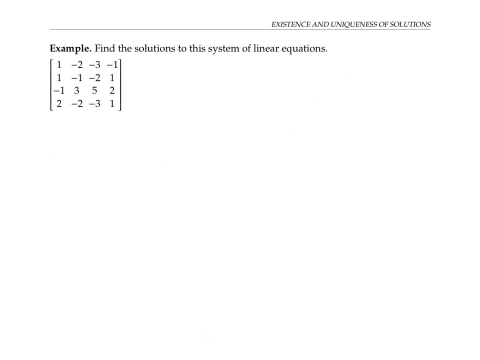 negative seven for x three and negative two for x four. these ordered quadruplets give my infinite family of solutions. For completeness, I'll give one more example that illustrates the third possibility of a unique solution, But I'll leave out even more of the details. 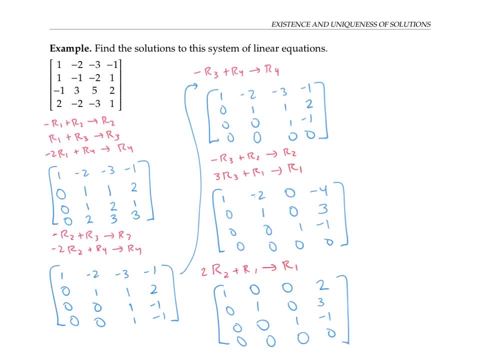 in the row reduction process. With my matrix in reduced row echelon form, I can analyze the solution set. I don't have any of those contradictory rows where I have all zeros as my coefficients and then a nonzero element for my constant term having all zeros as. 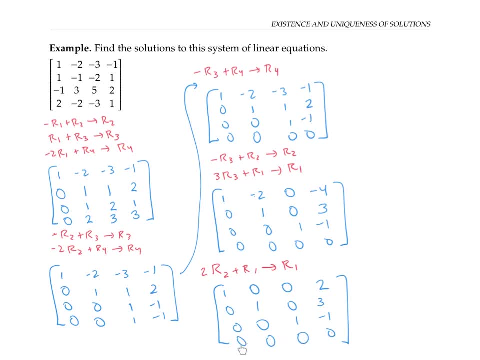 coefficients and then as zeros. my constant term is fine. That's just saying zero times x one plus zero times x two plus zero times x three is zero, which has to be true. it doesn't add any more information, So I can just ignore this row of entirely zeros And 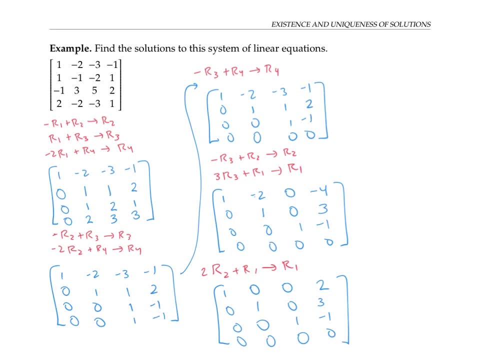 once I ignore it. I don't have any contradictory rows And I don't have any columns that don't have leading ones in them besides the the constant column, And therefore I'm going to have a unique solution. my solution will be that x one. 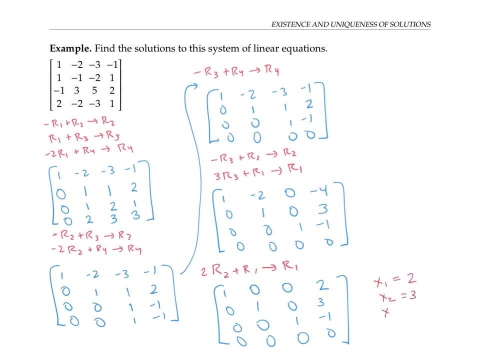 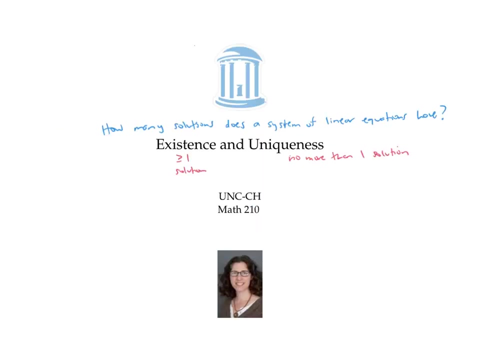 is equal to two, x two equals three and x three equals negative one. So here is an example of a system that has a unique solution. This video revealed the fact that there are three, and only three, possibilities for the number of solutions for a system: linear equations. 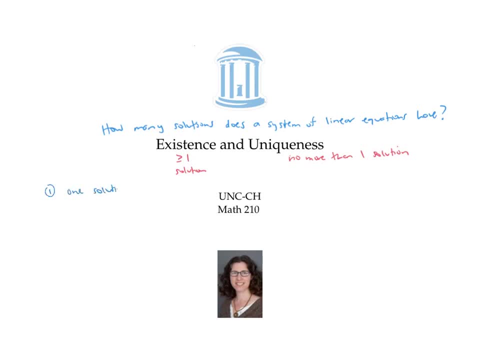 there could be one unique solution. There could be one unique solution. be one unique solution, be no solutions, Or there could be infinitely many solutions. We can observe which situation we're in by examining the augmented matrix for the system Once it's converted to reduced. 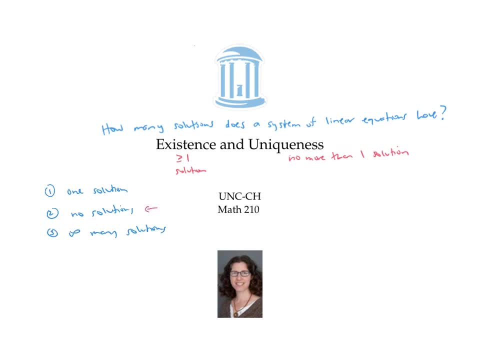 row echelon form. If the matrix has a contradictory row with all zeros and then a one in the constant column, then that tells us we have no solutions. If there's no such contradictory row, but there are columns corresponding to variables that don't have leading ones in them, then the 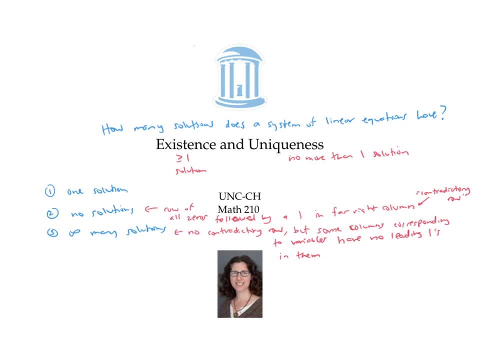 variables for those columns without leading ones can be used as free variables and their infinitely many solutions. Finally, if they're no contradictory rows and all columns corresponding to variables have leading ones and all columns corresponding to variables have leading ones, then the flip. 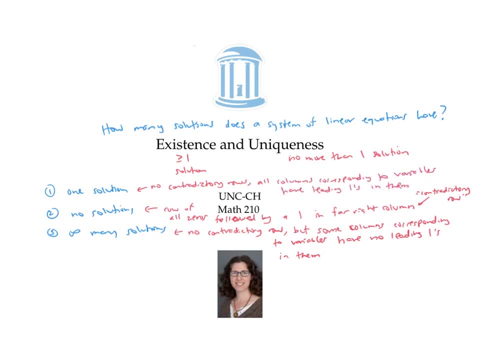 ones in them. Then we're in the situation where we have one unique solution, The columns corresponding to variables. by that I just mean the all the columns except for the far right column which corresponds to those, those constant terms. That concludes this video on existence and uniqueness of solutions. This video gives an example of setting up. 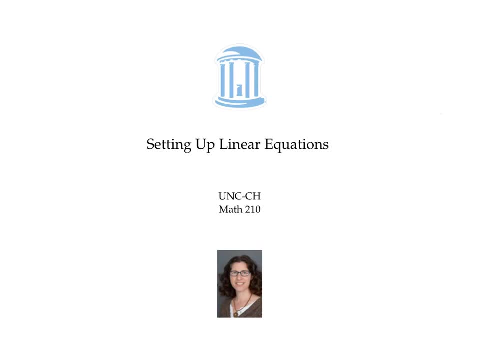 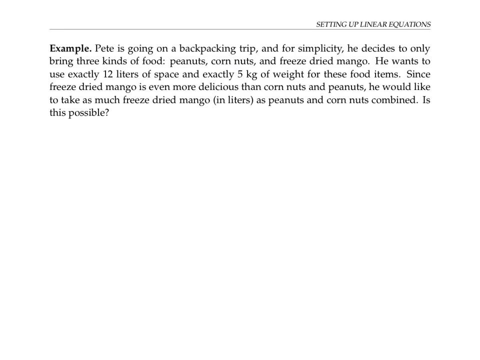 and solving a system of linear equations. So my friend Pete is going on a backpacking trip And for simplicity he decides to only bring three kinds of food: peanuts, corn nuts and freeze dried mango. He wants to use exactly 12 liters of space and five kilograms of 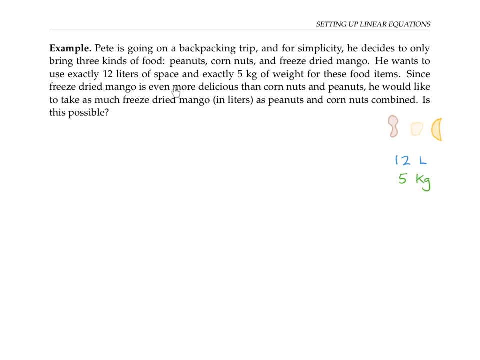 weight. Since freeze dried mango is so delicious, he'd like to take as much freeze dried mango in liters as peanuts and corn nuts combined. Is this possible? In order to describe this situation in equations, we're first going to need to decide on some variables to describe. 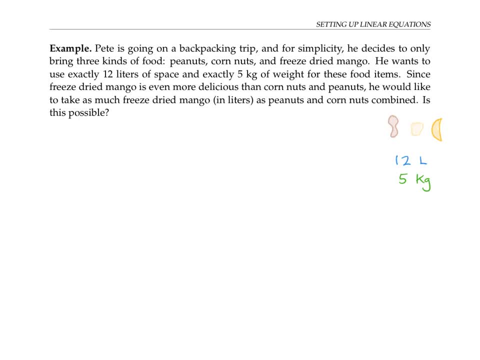 our unknowns. We don't know, and Pete would probably like us to tell him how much peanuts, corn nuts and freeze dried mango He should bring to satisfy these criteria. So I'm going to let p equal the amount of peanuts, c be the amount of corn nuts and m be the amount of mango. But hang on a second. 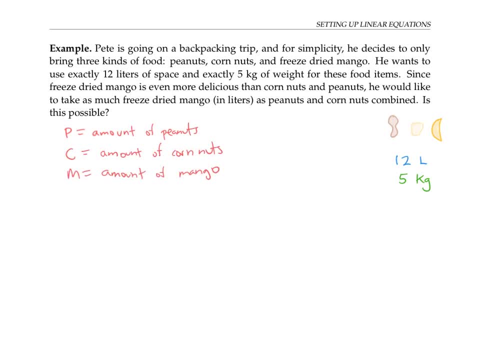 what should my units be here? I could describe the amounts in liters or in kilograms, or I suppose I could describe them in numbers like number of peanuts, corn nuts and mango in liters. But since this last condition has to do with liters, I think it'll be easiest for me to 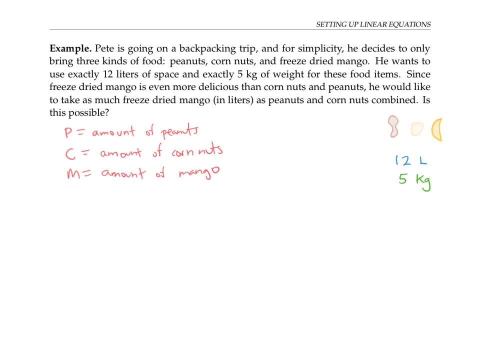 stick with liters, So I'll let these amounts be in terms of liters. Now, the fact that he wants to use exactly 12 liters of space for all this food already gives me one equation. I know that the amount of peanuts in liters plus the amount of corn nuts in liters, plus 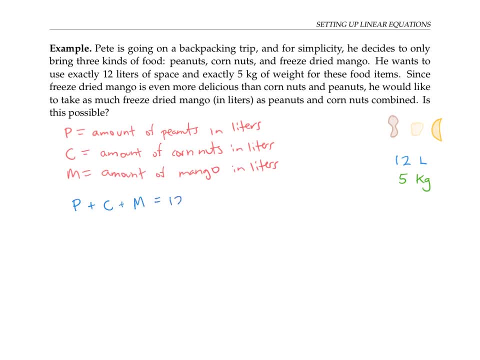 the amount of mango in liters has to add up to 12 liters. Now I also know that the amount of the weights of these food items need to add up to exactly five kilograms of weight. To write this condition as an equation, I'm going to need to know how much p liters of 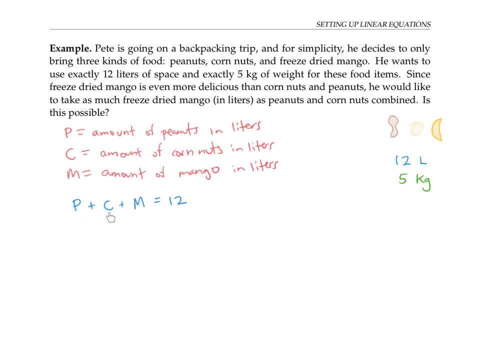 peanuts weighs in kilograms, And similarly for the corn nuts and the mango. A quick internet search brings me to an aquacom- or sorry, aqua calccom- website that has all these food volume to weight conversions And I find that for peanuts, shelled peanuts, one liter corresponds. 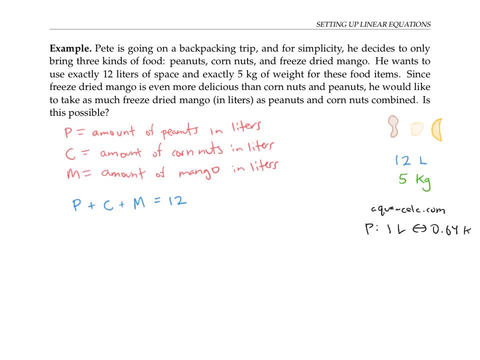 to 0.64 kilograms of weight. For corn nuts one liter is 0.36 kilograms And for freeze dried mango one liter is 0.1 kilogram. So therefore the p liters of peanuts: one liter will weigh 0.64 times p kilograms. The C corn nuts will weigh 0.36 times C kilograms. 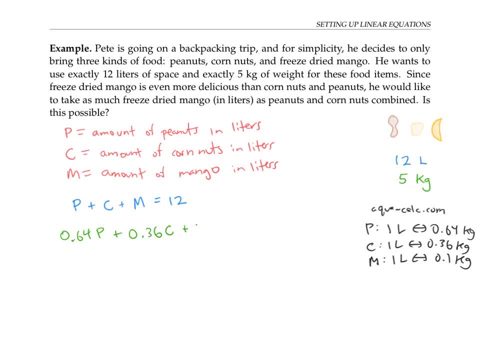 And the M liters of mango will weigh 0.1 times m kilograms, So that has to add up to five kilograms. The third and final condition is that Pete wants to take as much freeze dried mango in liters as peanuts and corn nuts combined. So to write that as an equation, I'm going to write that mango leaders is equal. 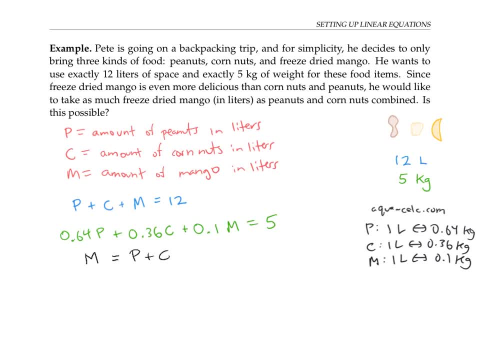 to peanut leaders plus coordinate leaders. So now I have three equations in three variables and I system of equations. And let's solve these: the system equations to find out how much peanuts, corn nuts and mango peach should bring. So I've copy: 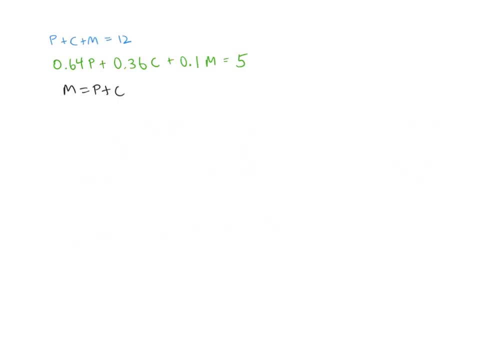 these three equations over to a new page where we can solve them. There are many ways of solving systems of linear equations, And in another video I show some systematic methods. But here I'm just going to use an ad hoc method. I'm noticing that since m is equal, 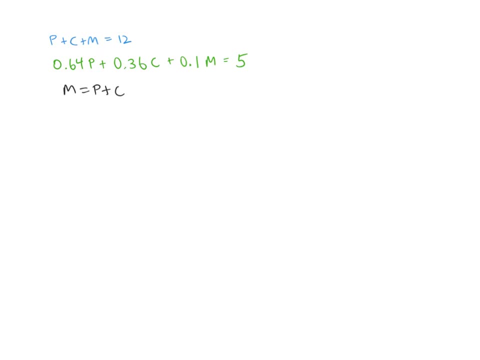 to P plus C. I should be able to just substitute in for the expression P plus C. that's the same thing as m. So that means that m plus m is equal to 12.. In other words, to m is equal to 12.. So m has to equal six. Now if I plug that number six in to the first and 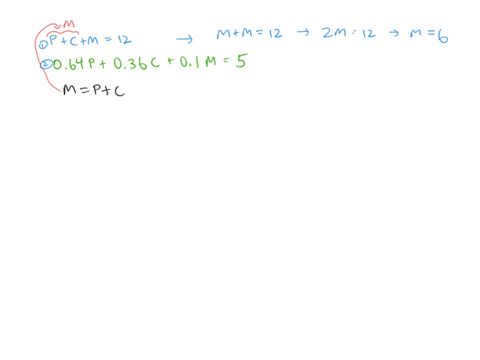 second equation: I get: P plus C plus six equals 12.. So in other words, P plus C equals six. And then the second equation equation: I get 0.64 P plus 0.36 C plus 0.1 times six equals five. That simplifies a little. 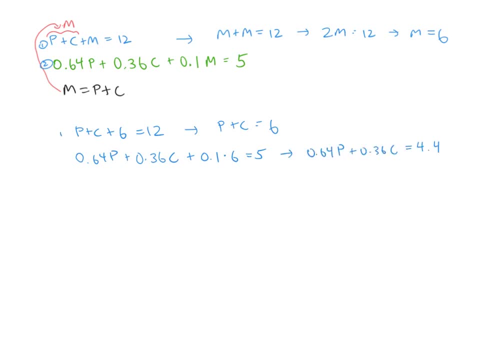 bit here Now from the new first equation. I can actually rewrite this to solve for P in terms of C and I can plug that in to the second equation: 0.646 minus C plus 0.36 C equals 4.4.. That simplifies to the following. Now my second equation involves only the variable. 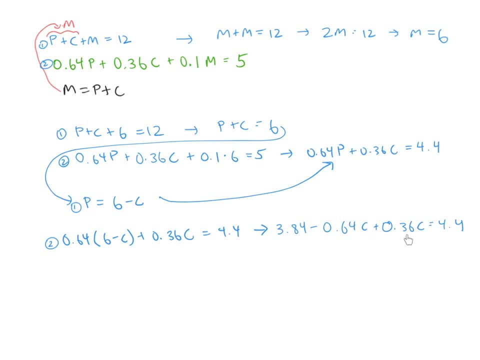 C. So I'll simplify a little further by combining C terms and moving my constant terms all the way to the right side. So now I can divide to get C equals 0.56 over negative 0.28, which is negative two. And finally, 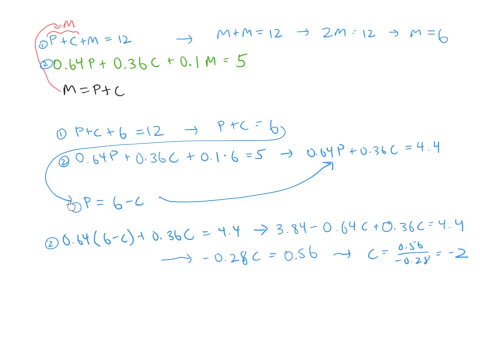 plugging that value C equals negative two into this version of equation one, I get that P equals six minus negative two, so P equals eight. So I found out that anything that satisfies these three equations must have P equals P equals eight. 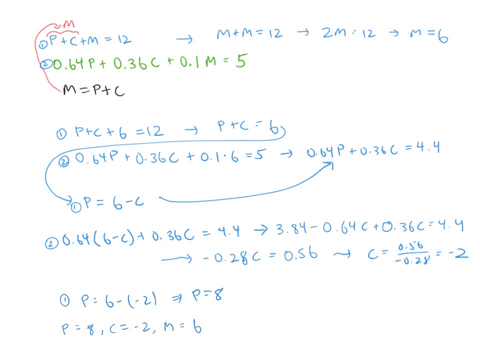 C equals negative two and m equals six. And I can verify the solution does in fact work by plugging back in to my original equations and seeing that it satisfies all three of them. So this is our unique solution to our system of equations. But this is this a solution to Pete's backpacking issue, Not 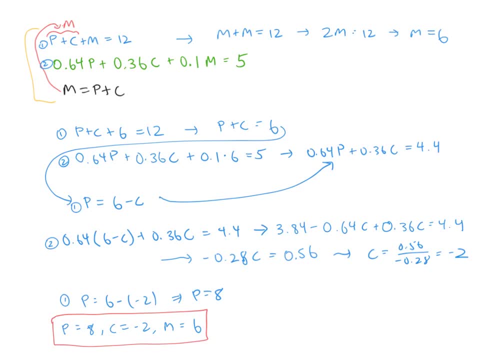 really, Because in order to satisfy all his criteria, we're going to have need to have negative two liters of corn nuts. So, in fact, in the real world application, where all these variables need to have non negative values, there is no solution. Sorry, Pete. And that concludes this example of setting. 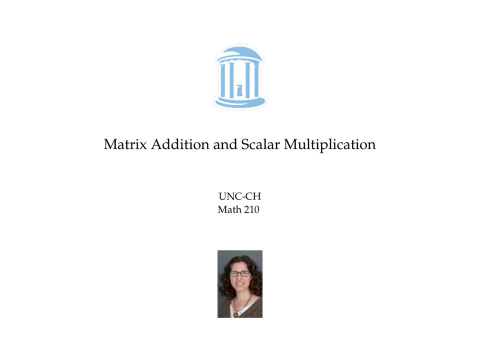 up and solving a system of linear equations. In this video, we'll talk about adding two matrices together. We'll also talk about multiplying a matrix by a scalar like the number five. The word scalar is just a fancy word for a number to distinguish it from from multiplying. 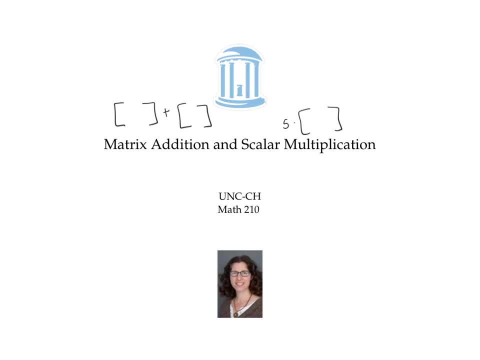 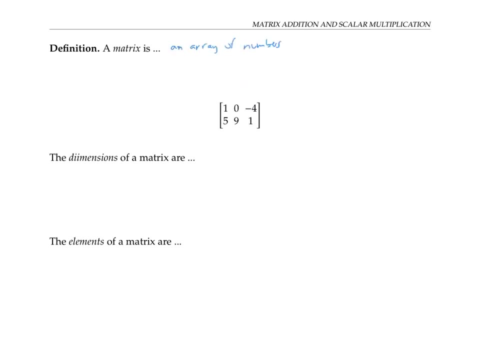 by a matrix. In a future video we'll talk about multiplying two matrices together, but not yet Recall that a matrix is just an array of numbers like this one. The dimensions of a matrix is just the number of larger or smaller matrices, So it's just the number of numbers. 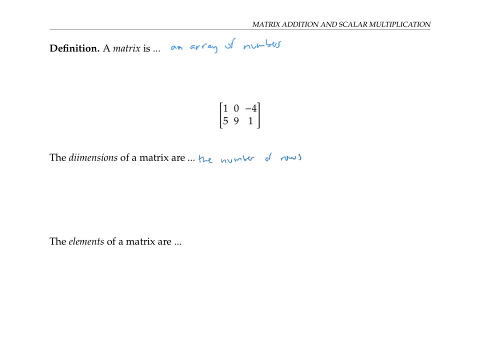 of the matrix. To summarize, a matrix is just a number of larger or smaller matrices. To matrix are the number of rows and the number of columns. For example, in this matrix above, we have two rows and three columns. So we say that this is a two by three matrix. The 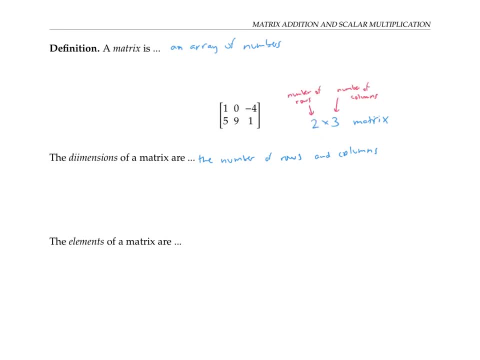 number of rows is always listed first. the elements of a matrix are just these individual entries. So this matrix has six elements. Sometimes these elements are indexed by their row number and column number. So, for example, if I want the element a to one, that would 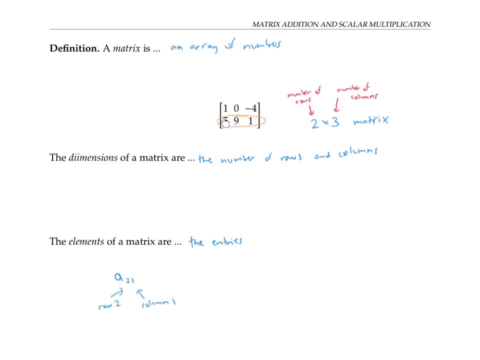 be the element in the second row and the first column, so that would be the number five. If, instead, I wanted the element a, one, two, that would be the first row And the second column, so that would be the number zero. Sometimes you'll see a whole matrix. 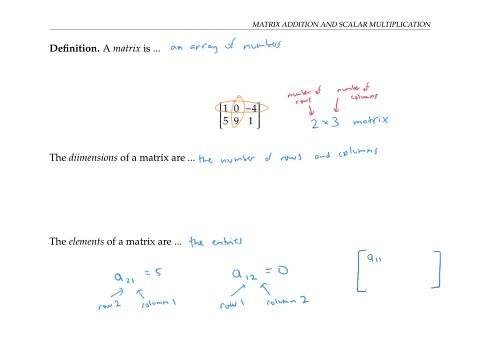 listed out with this abstract notation, So a 11,, a 12,, a 13,, a 21,, a 22,, a 23, is the correct ordering for the entries in this two by three matrix The first index in these. 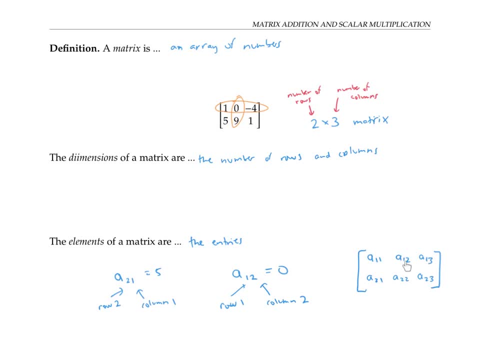 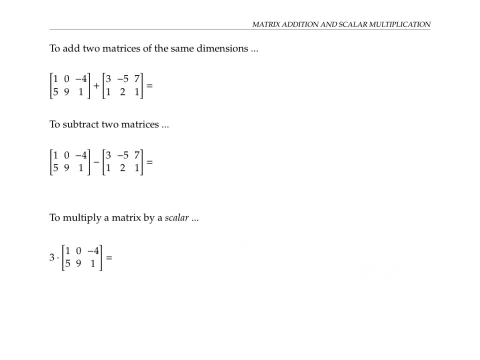 double indexes tells you the row number, So each of these numbers is in row one, and the second index tells you the column number To add together two matrices of the same dimensions. So here, dimensions two by three, we do just what you would think we would do: We add the corresponding elements together, So one plus. 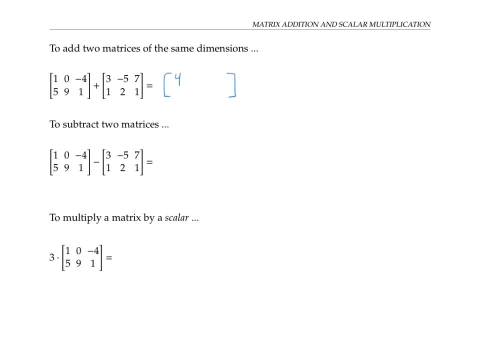 three is 40 plus negative five Is negative. five negative four plus seven is three, And similarly, if we add a corresponding elements in the bottom row, we get 611 to to subtract two matrices of the same dimensions, we subtract elements. So here we get negative 25, negative 1144.. 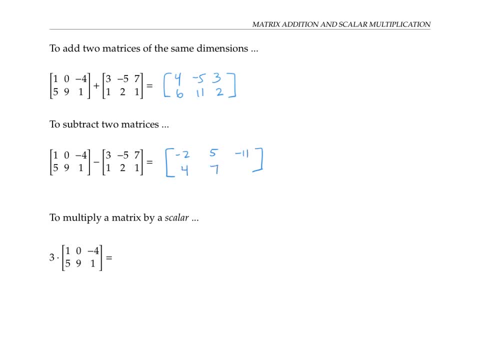 Okay, Okay, Okay. So we have a matrix of three, seven and zero. Note that it's not possible to add or subtract matrices with different dimensions, because we wouldn't be able to line up corresponding elements. To multiply a matrix by a scalar- it's just a number- we again do just what. 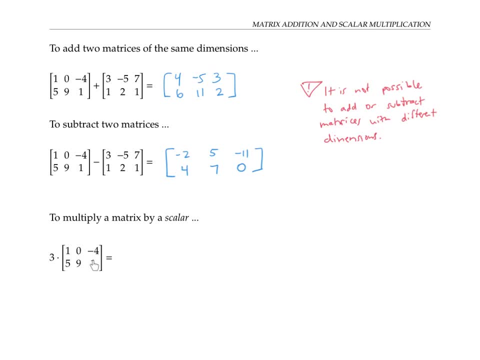 you think we do. we multiply each element by that number. So here we're multiplying three by this matrix, That just means we get three times one, which is three. three times zero is zero. three times negative, four is negative 12.. 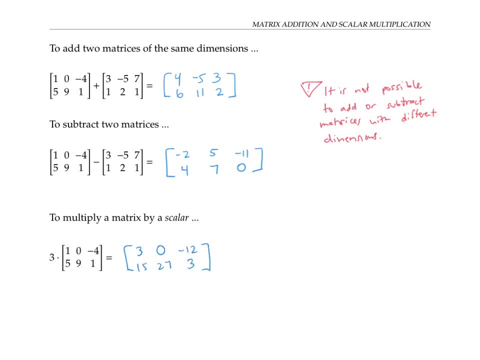 And similarly we get these numbers on the bottom row. It's most difficult to write scalar multiplication with the scalar on the left side, But it's also possible to write the scalar multiplication with the scalar on the right side And it means the same thing. One. 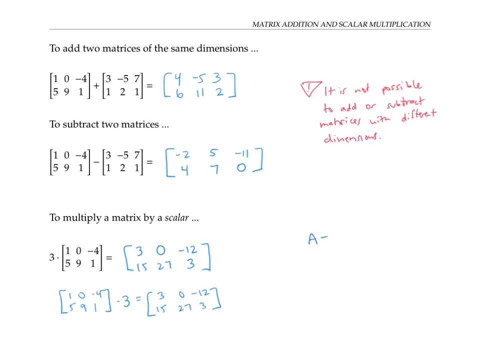 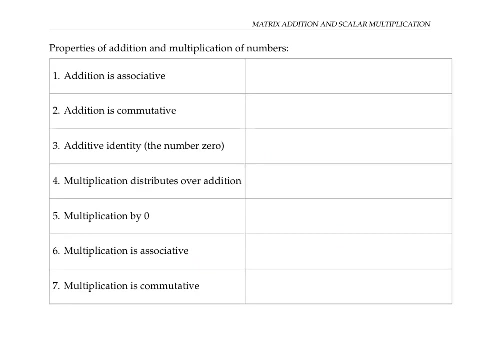 last point is that instead of writing subtraction of matrices, it's also possible to write the addition together with scalar multiplication by negative one. I'd like to go through some properties of matrix addition and scalar multiplication, But before I do that, I want to review some. 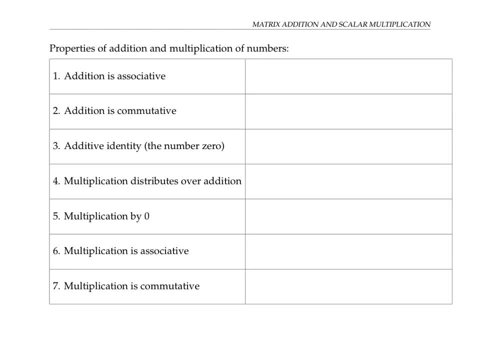 properties of just addition and multiplication of numbers. So we say that addition is associative. What this means is if you have numbers like, say, three plus four, and you add those together and add another number like seven, that's the same thing as three plus four plus seven. 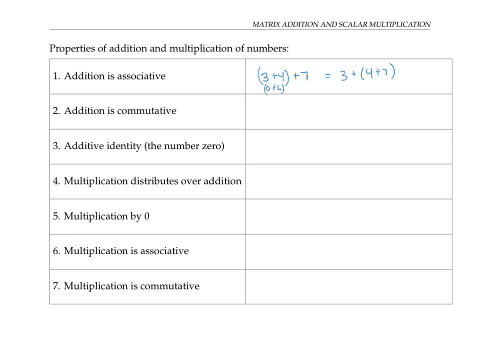 you can group these in other orders And, more generally, if you have A plus B grouped plus C, that's the same thing as adding A to the grouping B plus C. that's the associative property. Addition is commutative. That means it doesn't matter what order you add things in A plus. 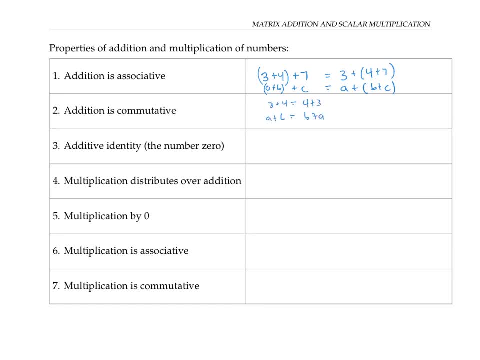 B is always the same as B plus A. There's something called an additive identity. we usually just call it the number zero. The key property of number zero with addition is that if you add zero to any number, you just get the same number you started with. We have this property called the distributive. 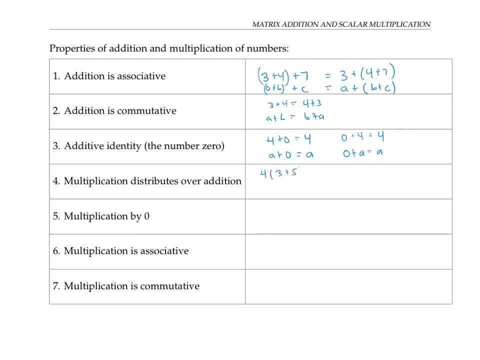 property. Multiplication distributes over addition. So if you have four times three plus five, that's the same thing as four times three plus four times five, And that's true no matter what numbers- A, B and C- You stick in the places of four, three and five When you multiply any number by zero. 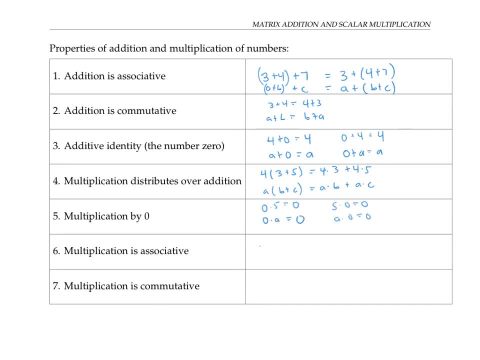 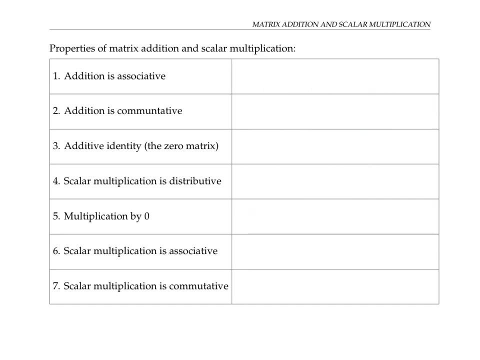 you just get zero. Multiplication is also associative. A times B times C, the same thing as doing A times B first and then multiplying that answer by C, And multiplication is commutative. A times B is the same as B times A. Well, guess what these same properties hold for? 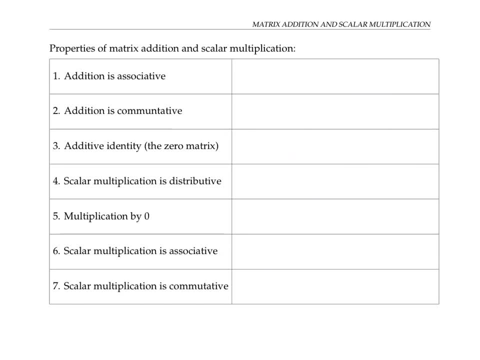 matrix addition and scalar multiplication. If you add matrices together, it doesn't matter if you first add the two matrices A plus B and then add that result to C, get the same thing if you group it the other way. And this follows really from the associative property for addition of numbers, Because when we're 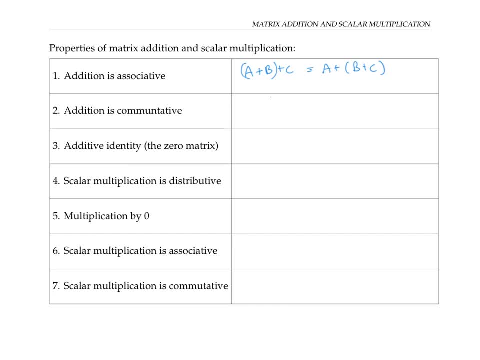 adding matrices. we're just adding numbers in each position of the matrix. Same thing for commutativity: You can add matrices in either direction. Okay, In either direction, you'll get the same answer, just because you can add numbers in either direction, and you'll get the same answer. Now, what about this additive identity? 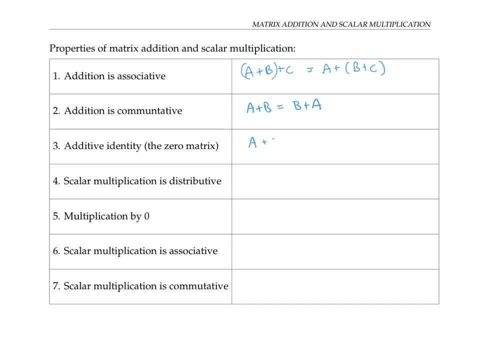 Is there such a thing as a zero matrix that you can add on to any other matrix and just get the same matrix? I'll write the zero with little brackets around it to emphasize that it's supposed to be a matrix, not the, not the scalar number zero. See, if you could guess. 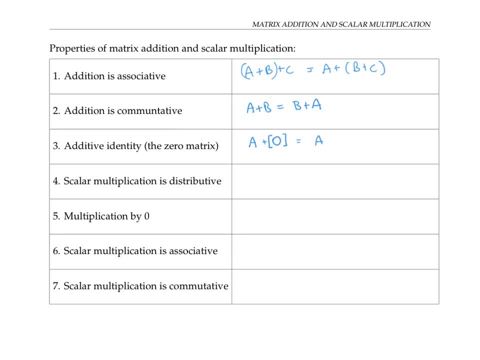 what that matrix would look like. If you're guessing that it would have all entries in every zero, you're exactly right, Because when you add zero to every single element of a matrix, you're just going to get the same matrix again. Notice that. to be precise, 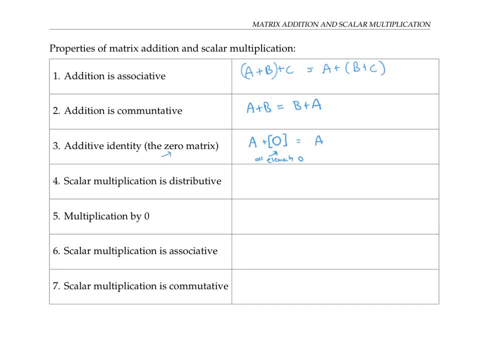 there's actually a lot of different zero matrices, One for every possible pair of dimensions, m by n. Just like for regular multiplication and addition of numbers, scalar multiplication over matrices is distributive. So if I have a scalar k and I multiply it by a number, 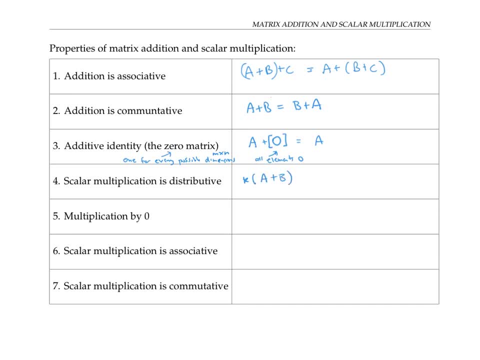 by the sum of two matrices, A and B. I could instead first multiply the first matrix by k and then multiply the second matrix by k and then add them up. Multiplication by the scalar zero is just going to multiply every single entry of my matrix by zero, So 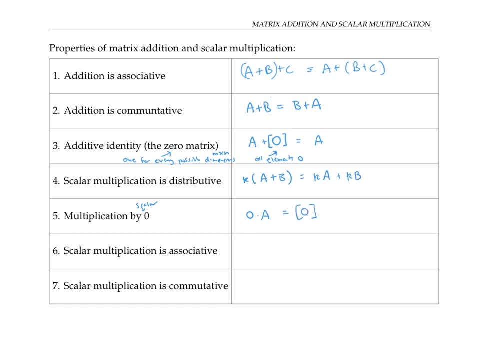 that's going to give me a zero matrix. scalar multiplication is associative in the sense that if you have like k times l and you multiply that by a matrix a, that's the same thing as k times la. And scalar multiplication is commutative in the sense that k times a is the same thing as. 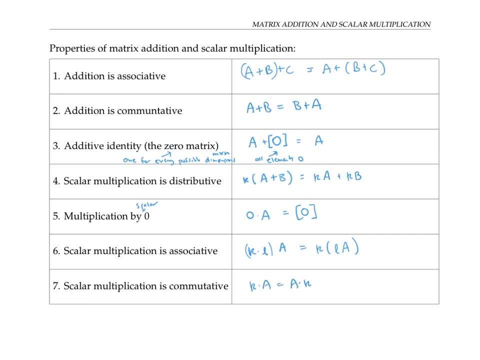 a times k pretty much by definition. So all of the properties that we've mentioned about regular addition and multiplication work for matrix addition and scalar multiplication with matrices. But we'll see in a future video when we talk about matrix multiplication that there are actually some surprises with matrix multiplication. 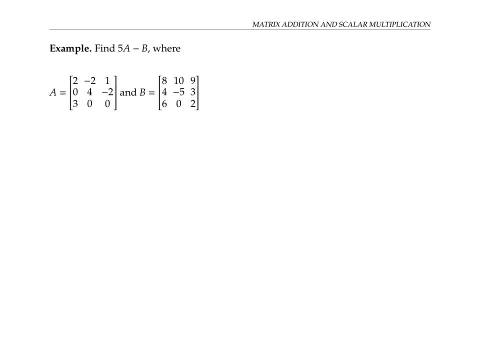 and not all these properties will hold. Let's end with an example finding five a minus B, where a is this three by three matrix and B is that three by three matrix. In other words, I want to take five times this matrix and then subtract that matrix, So to do five. 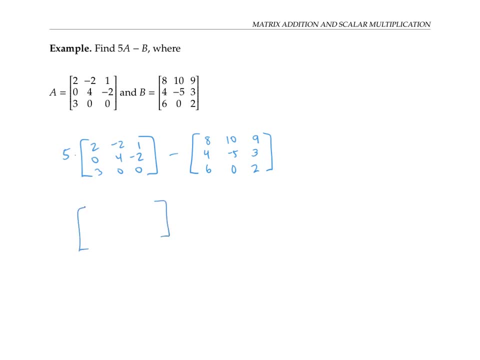 times this matrix. I'm just going to multiply all the entries by five, then I'll subtract this other matrix. So I'll just subtract entries and I get to minus 20, minus four, minus four, 25, minus 1390 and minus two as my finalector of all my 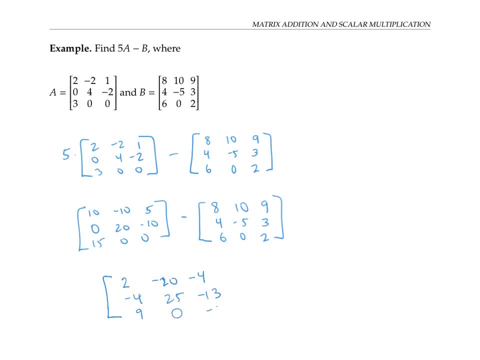 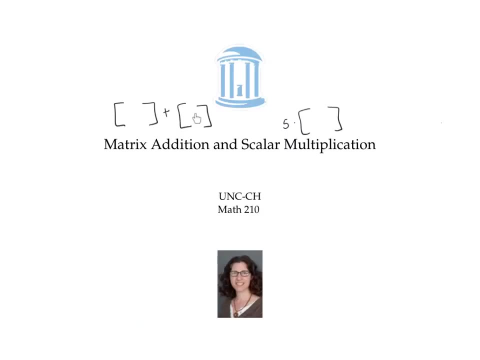 entries. answer. In this video we added matrices together, element by element, did scalar multiplication by multiplying each element by that scalar, And we talked about some of the properties. Previously we defined the sum of two matrices in the simplest, most natural way that we. 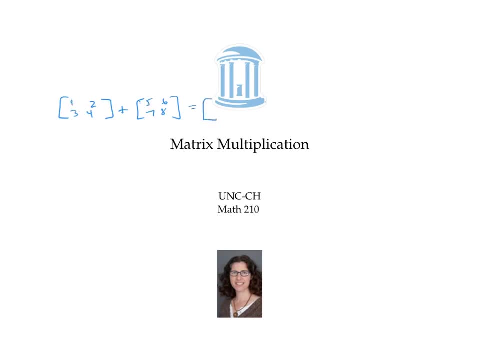 could, simply by adding corresponding elements, it will be possible to invent a matrix multiplication that works similarly, just by multiplying element by element. one times five is five, Two times six is 12. And so on. But we're not going to do matrix multiplication this. 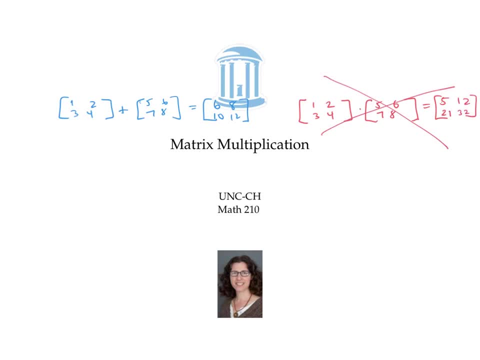 way The standard definition of matrix multiplication. the topic of this video is more complicated. It's also much more useful. So one reason that we wanted to find matrix multiplication in this more and more complicated way Is that when we use matrices to represent transformations or changes in a system, then 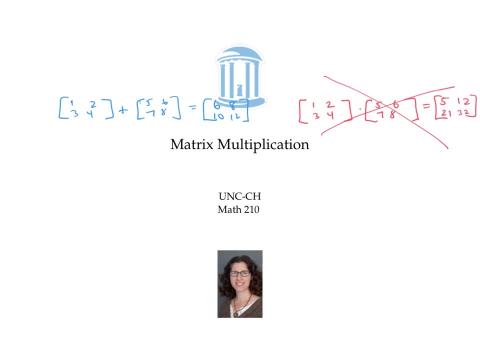 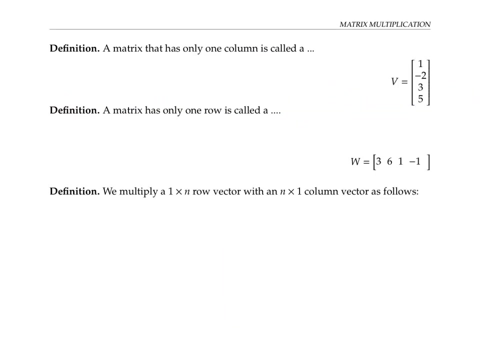 applying two transformations one of the other will exactly correspond to multiplying two matrices in the way that I'm going to show you, And this will allow us to use matrix arithmetic to model complex systems over time. So before we define multiplication for general matrices, we're going to start with very special matrices called vectors. a matrix that has 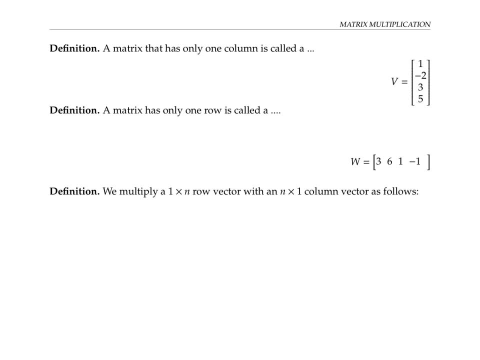 only one column is called a column vector. So this is an example of a column vector. It has four entries all in one column, So as a matrix it's a four by one matrix And in general a column vector is an n by one matrix for some number n a matrix that has. 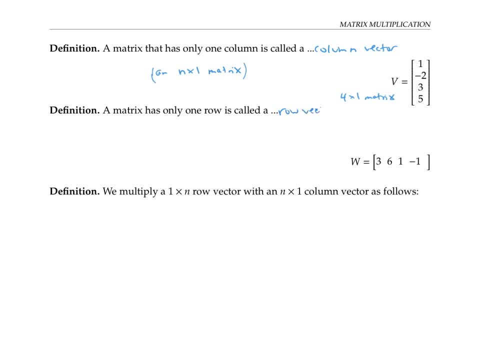 only one row is called a row vector. Here's row vector. it's a length four row vector, or in other words a one by four matrix. And in general a row vector is the same thing as a one by n matrix for some number n I'm. 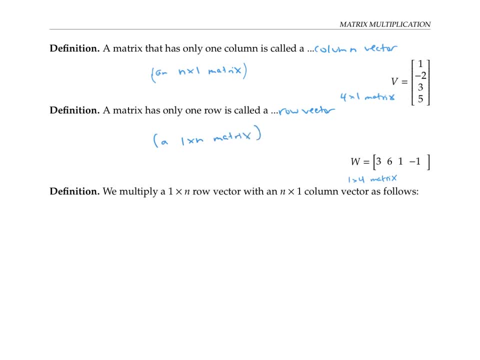 going to show you how to multiply a one by n row vector with an n by one column vector. First, with this example, to multiply this one by four row vector with this four by one column vector. we multiply the first entry of the row vector with the first entry of. 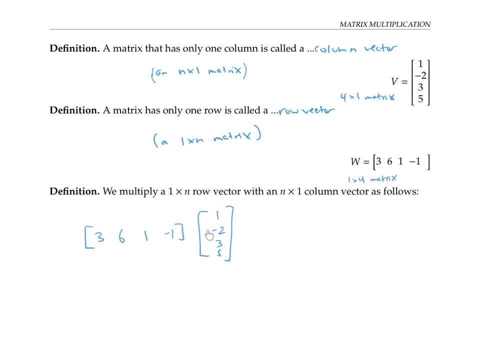 the column vector, the second entry with a second entry, and so on, And then we add those products up. So we're going to do three times one plus six times negative, two plus one times three plus negative, one times five, which adds up to negative 11.. Sometimes I 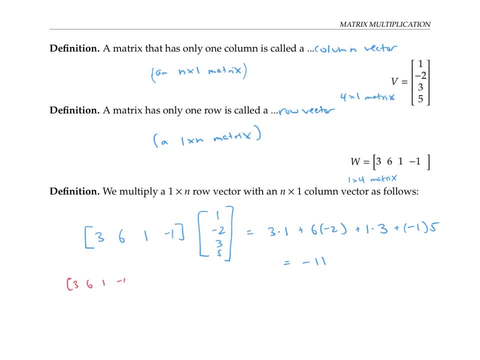 like to visualize this as tipping the row vector on its end And then multiplying numbers at the same height with the column vector and adding them up. Let's write this multiplication process as an abstract formula. Let's write our row vector, say w, and write out entries w, one, w two, w three, all the way through w, n, And then 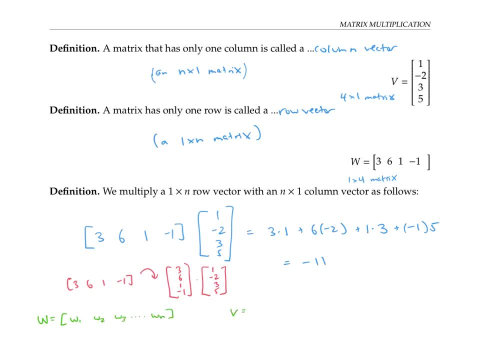 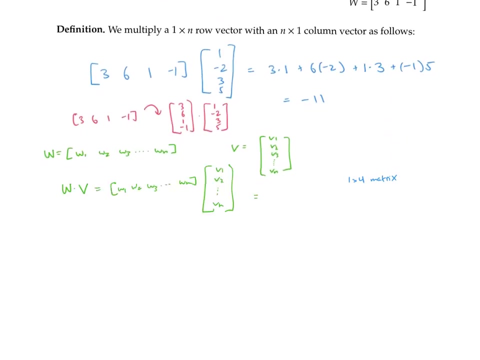 let's write our column vector v with entries v one, v two, v three, all the way through v n. To perform the multiplication of these two vectors w times v, we multiply w one times v one. add that to w two times v two. 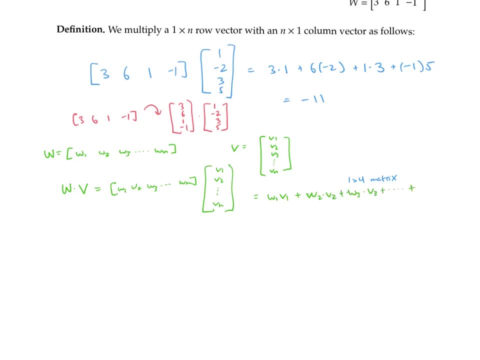 plus w three times v three, and so on all the way up to the last product: w n times v? n. we add up all those terms. If you're familiar with summation numbers, you know what I'm talking about. If you're familiar with multiplication notation written with: 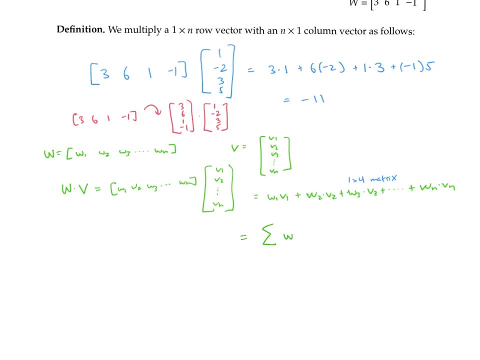 this big letter sigma. this can be written as the sum of wi times vi, where I starts at one and goes through n. Notice that we've only defined multiplication for a one by n row vector times an n by one column vector. It wouldn't make sense to multiply a row vector. 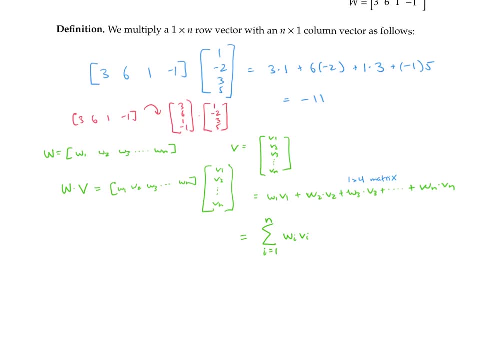 and column vector with different number of entries, because the entries wouldn't line up the way we're using them. It would be possible to define a row vector and column vector with different number of entries, because the entries wouldn't line up the way we're using them. It would be possible. 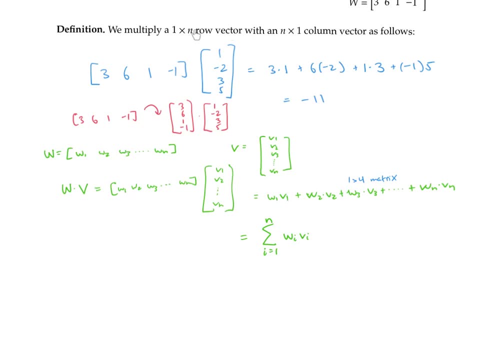 to define multiplying a column vector times a row vector, In that order. there are a couple of ways to define this, one of which may surprise you, But for now we're going to stick with multiplying row vectors times column vectors, in that order, because that's. 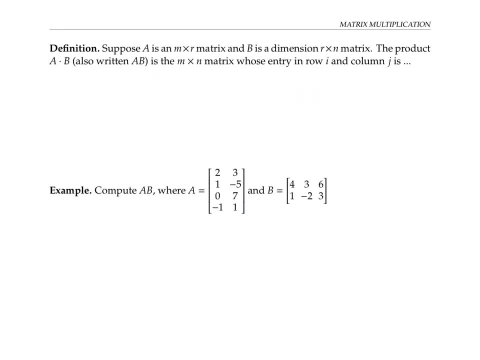 what we need to define more general matrix multiplication. So now let's define matrix multiplication in general. Let's suppose that a is an M by R matrix and B is an R- n matrix. then the product A times B is an M by n matrix And the entry in row I and 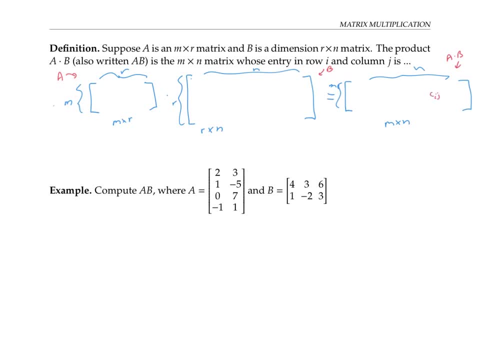 column J is given by the product of row. I have a and a column J of B. Notice that a row of A is a one by r row vector and a column of B is an r by one column vector. So this is just the kind of vector product that we defined on the previous page. I want to emphasize: 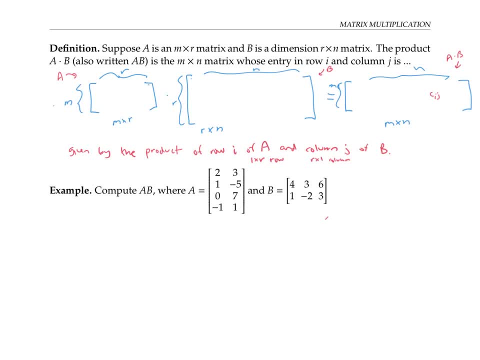 that when we're multiplying two matrices- A times B, in that order- then the number of columns of A needs to equal the number of rows of B. That's the only way that the element will line up when we're doing our vector product And the only way that the matrix multiplication 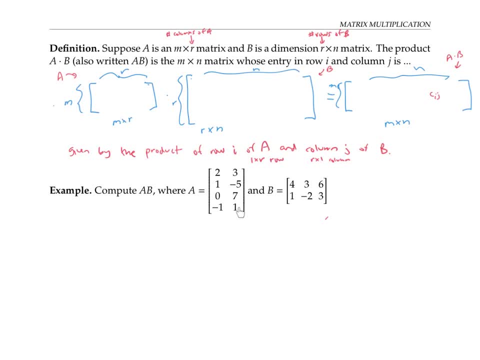 will make sense. Let's look at an example where A is this four by two matrix and B is this two by three matrix. Notice that the number of columns of A is equal to the number of rows of B, So it makes sense to compute A times B in that order, even though it wouldn't. 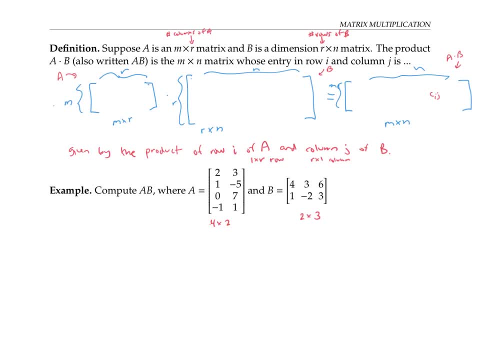 make sense to compute B times A. Suppose we want to compute the product A times B, I'll call that matrix C, And suppose we want to just find like the entry in the second row and the third column, So I could call that C to three. To do that we need to take the second row of A, So that's one. 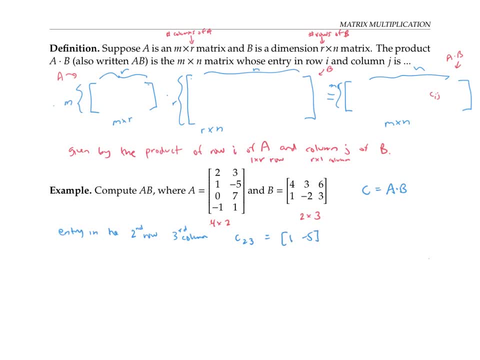 negative five and multiply it by the third column of B, So that's six, three, and we do our vector product one times six plus negative five times three, So that's six minus 15, which is negative nine. So C is going to be. 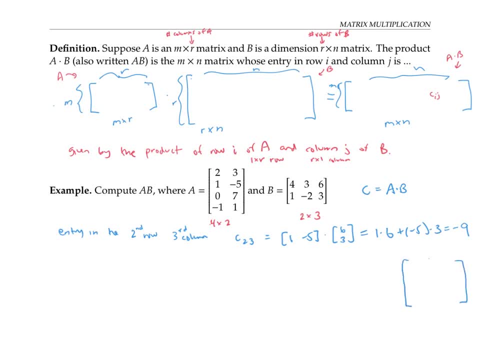 a four by three matrix and its entry in the second row and third column is going to be a negative nine. But in practice we're not just going to want to calculate the number of rows, we're going to want to compute one random entry of our product matrix. we want 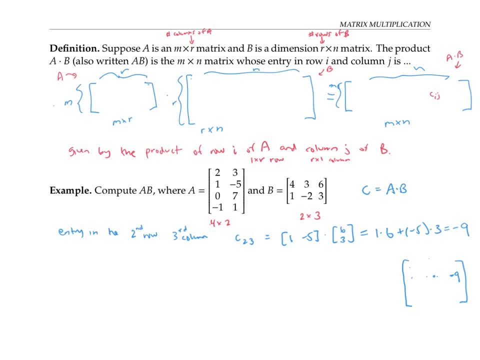 to compute all its entries. So let's do this in a systematic way, starting with the first row and the first column of B to get the entry in the one, one position. Let me rewrite my matrices down here And I'll leave space for my four by three product matrix. So now, 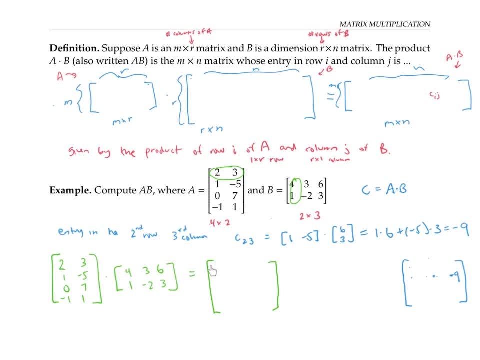 for my entry in the top left position, the first row and the first column. we're going to take the first row of A and multiply it by the first column of B, two times four plus three times one, that's eight plus three, which is 11.. Now let's get the next entry. 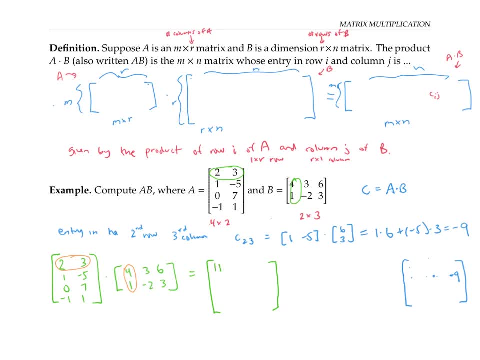 in the first row and the second column. So that's going to be the first row of A and the second column of B. So we'll take two times three plus three times negative two, that's six minus six or zero Moving right along to get the entry here. I'm going to 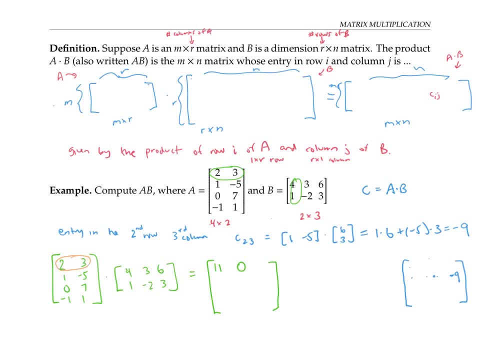 need the first row of A and the third column of B, So that's two times six plus three times three, which is 12 plus nine or 21.. Now I'm ready to move on to the next row of the product. So that's the second row. first column position, So that'll be the second. 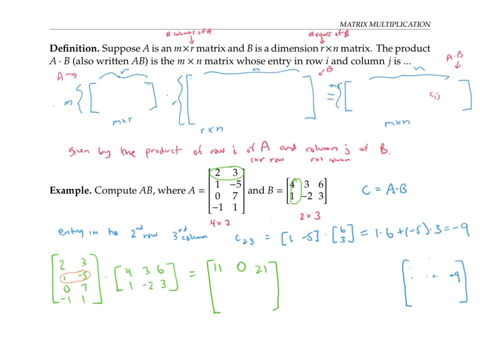 row of A times the first column of B. we have one times four plus minus five times one, that's four minus five or negative one. Continuing like this for the next entry we'll take the second row times the second column. So that's one times three plus negative five. 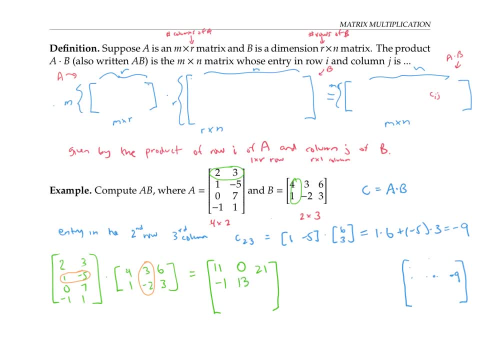 times negative. two. three plus 10 is 13.. And the second row times the third column gives us one times six plus negative five times three. So that's six minus 15, which is negative nine. that's the one we calculated before. The last two rows are similar. For the third row, I need to take the third row. 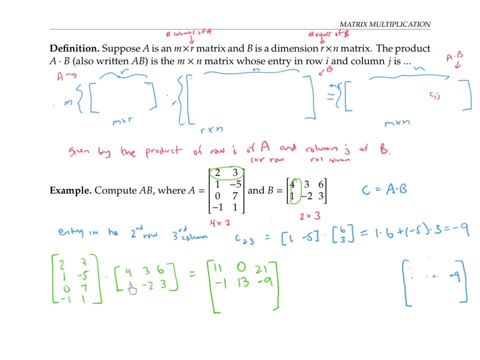 of the product and you take the third row of A and multiply it by each column and turn: zero times four plus seven times one is seven. Zero times three plus seven times negative two is negative 14.. Zero times six plus seven times three is 21.. Finally, we get the fourth and last row of the product by multiplying: 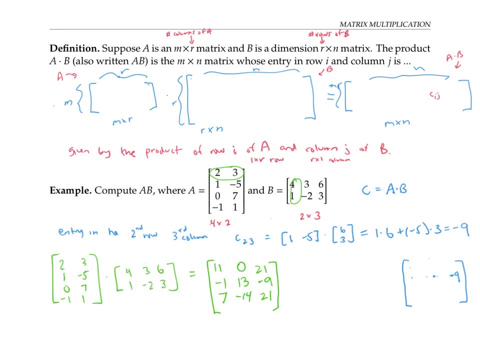 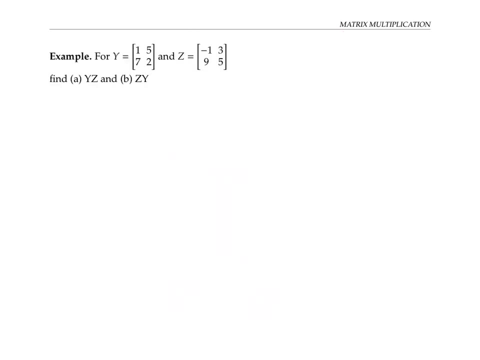 the fourth row of A by each column of B in turn, and that works out to negative three, negative five, negative three And we have our matrix product. Please pause the video and calculate for yourself the product y times z and then the product z times y. Notice: 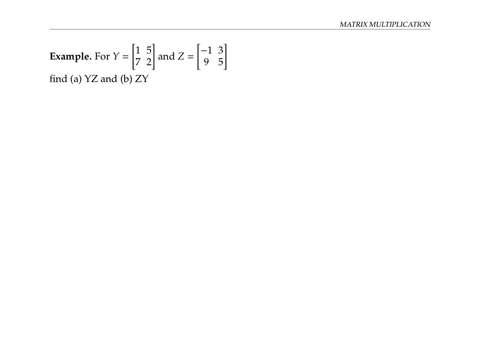 that in this case we can do the product in either order, since each of these is a two by two matrix, So their inner dimensions agree, no matter which order you do the product in. So when calculating y times z, we're going to get the matrix as multiplied in this order And the result should: 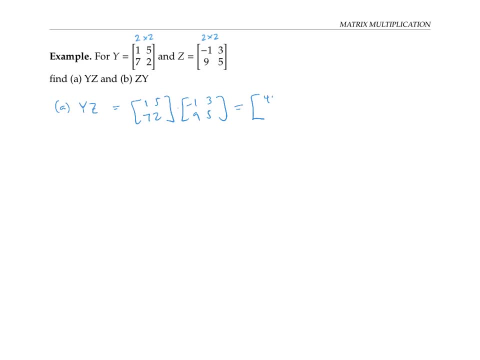 be 4428 1131.. The 44 comes from from multiplying the first row of y with the first column of z. one times negative. one plus five times nine. that's minus one plus 45, or 44.. Multiplying the first row by the second column gives us the 28.. The second row by the first column. 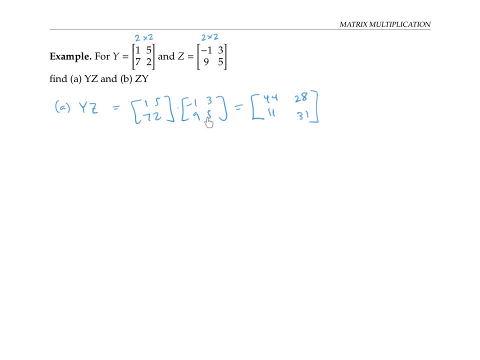 gives us 11.. And the second row by the second column, seven times three plus two times five is 31.. Let's see what happens when we multiply in the opposite order, z times, y. Okay, this time we get 2144 and 55, a completely different matrix, even though one number in 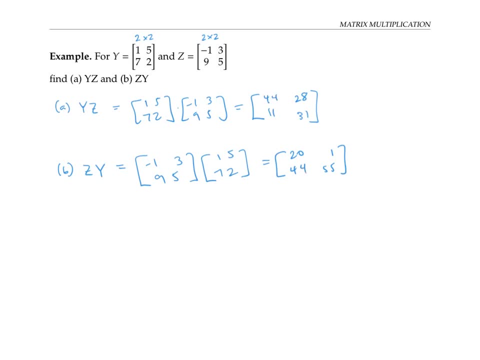 common is just a coincidence. This example shows us that multiplication of matrices is not commutative. y times z is not necessarily equal to z times y. In a future video we'll look at properties of matrix multiplication more thoroughly and figure out what properties 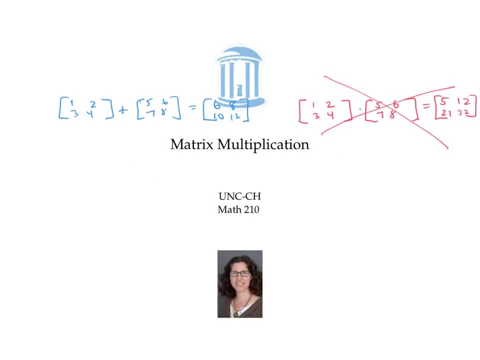 of matrix multiplication we're going to look at in the next video. In this video, we defined matrix multiplication by multiplying rows, times, columns, And we noted that matrix multiplication is not, in general, commutative. In this video, we'll talk about properties of matrix multiplication and compare them to properties of multiplication. 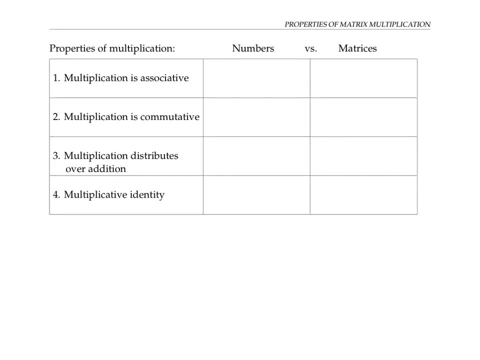 for ordinary numbers. I've listed some properties of multiplication that hold for ordinary numbers. Let's see which properties also hold for multiplication of matrices. Multiplication of members is associative. That means if I multiply a times B and then multiply that by c, that's the same thing. 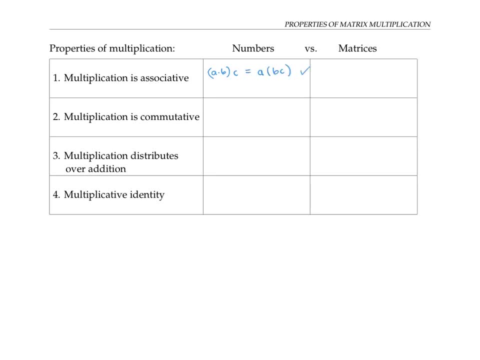 as multiplying A by the product of B and C. It doesn't matter how you group them. It turns out that matrix multiplication is also associative. all right, capital letter to denote the matrices instead of numbers, But the property is this: In this case, I just need to multiply these ones, grandson. 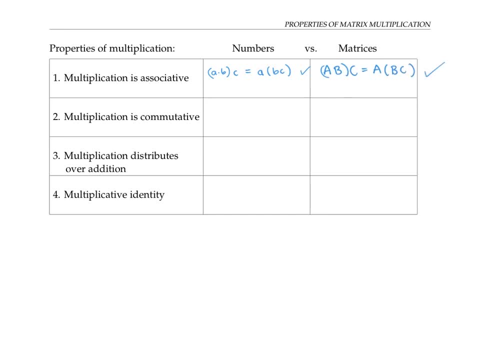 property is the same. There's also a version of associativity that holds for multiplying matrices and scalars together. If I let lowercase k represent a scalar- that's just a number- then I can do. if I do k times the matrix, A recall, that just means multiply every entry. 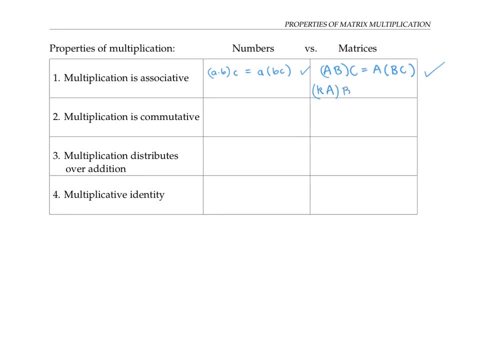 of A by the number k and then do matrix multiplication of that times B. that's the same thing as multiplying A times B first and then multiplying the result by k. In fact it's also the same to multiply A by the product of k times B, Although I won't prove these properties here. 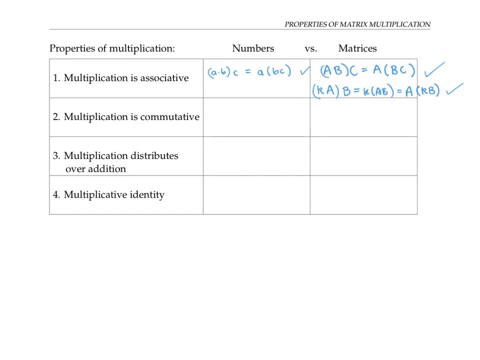 they can be proven by writing out a formula for matrix multiplication in terms of the entries of the matrices and using some algebra. When we're talking about numbers, multiplication is commutative: A times B is the same as B times eight. doesn't matter the order. However, as we saw in a previous 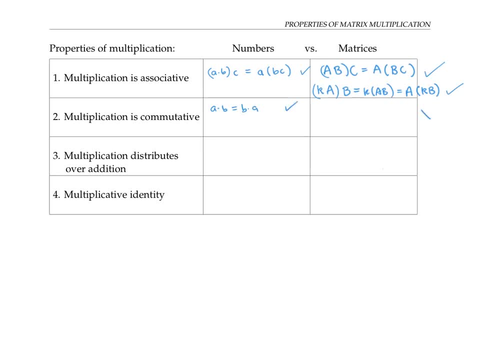 video. matrix multiplication is generally not commutative. A times B is not necessarily equal to B times A. Actually, a lot of times it's not even possible to multiply matrices in both orders. For example, if we have a four by three matrix and multiply it by a. 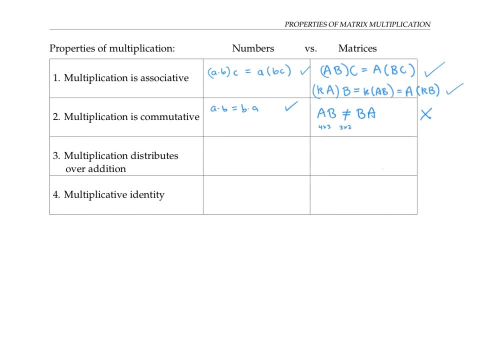 three by two matrix. that's legit because the inner dimensions three and three are the same. But if we reverse the order, so instead of a times B we do B times A, that would end up being a three by two times a four by three, which doesn't make sense. But even when we 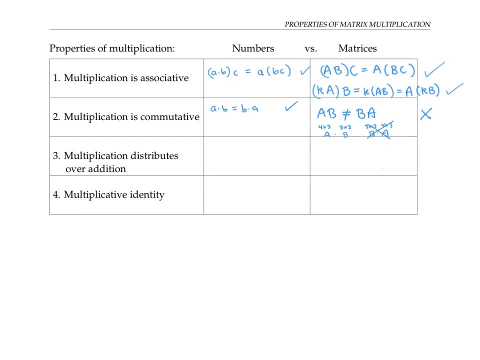 can multiply matrices in both order, for example, square matrices, matrices whose number of rows and columns are both the same, can be multiplied in either order, So like if we have a two by two matrix a and a two by two matrix B. 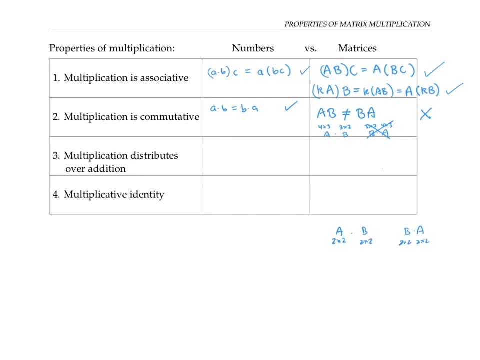 we can multiply them both ways, But most of the time we won't get the same answer. I'll write down a couple of two by two matrices just to show you multiplying in this direction. So row times column gives us negative 11, negative 23.. But multiplying in the other, 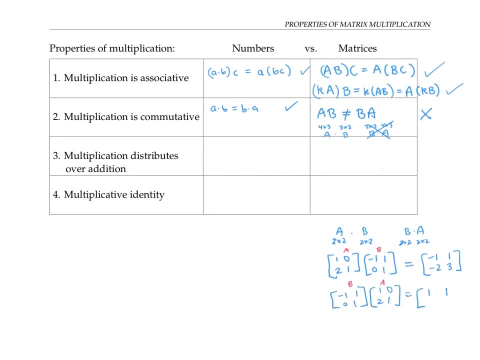 order gives us 1121.. So multiplication of matrices is not generally commutative For numbers. multiplication distributes over addition. That is, if we take A times B plus C, that's the same thing as A times B plus A times C. Also, if I multiply B plus C times A, that's: 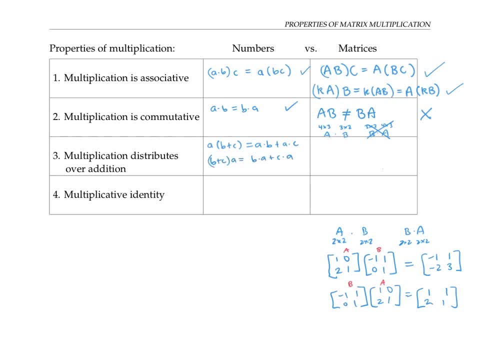 the same thing as B times A plus C times A. Well, the same distributive properties hold for matrix multiplication. I won't prove that property here, But it can be proved by focusing on each row and column separately. Finally, for numbers there's a multiplicative identity. That's the number one. It's called a multiplicative. 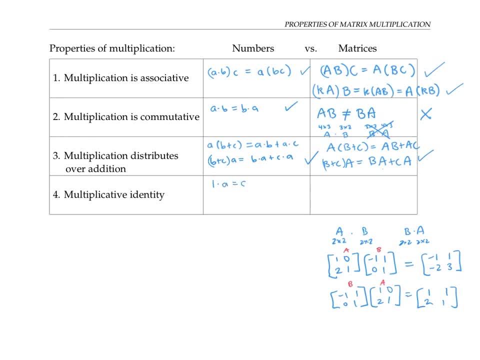 identity because one times any number gives you the same number and any number times one gives you the same number. Is there also a multiplicative identity for matrices, In other words a matrix I for identity such that I times any matrix gives you the same. 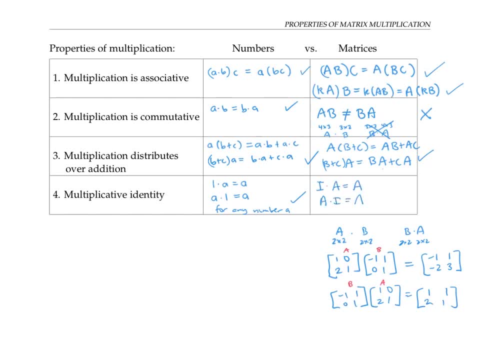 matrix And that matrix times, I gives you the same matrix In fact there is, as long as we restrict ourselves to square matrices, that is, matrices of dimensions n by n for some number, n, the same number of rows and the same number of columns. In fact there's. 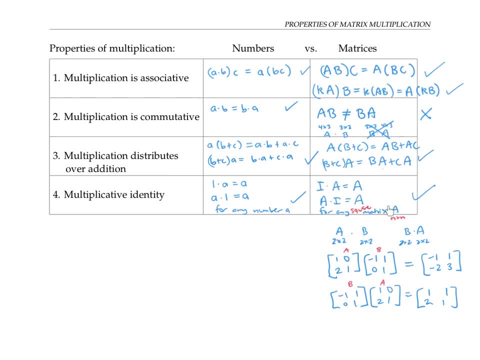 a whole family of identity matrices, One for each size square matrix, one for each number n. So let's see if we can figure out what this identity matrix needs to look like. So I'm just going to write down some random matrix- A, let's say a three by three matrix- And we're going to try to figure out what. 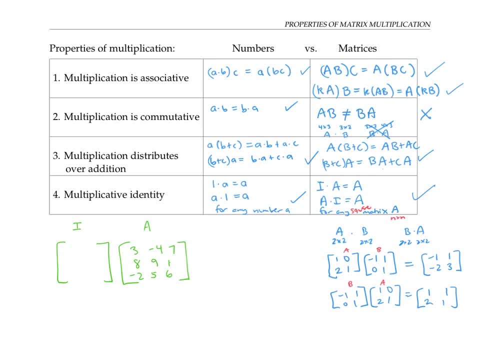 this identity matrix I needs to be in order that we get the same matrix A as the result when we do this product. First of all, we know that I needs to also be a three by three by three matrix for the dimensions to work out. So, thinking about the first row of I 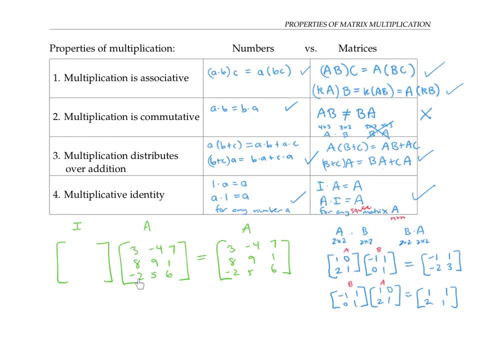 when I multiply the first row of I by the first column of A, I need to get this entry three, So that first row needs to just pick up the number three in this column, If you're thinking that the first row of I should be 100. That's the right idea, Because then when 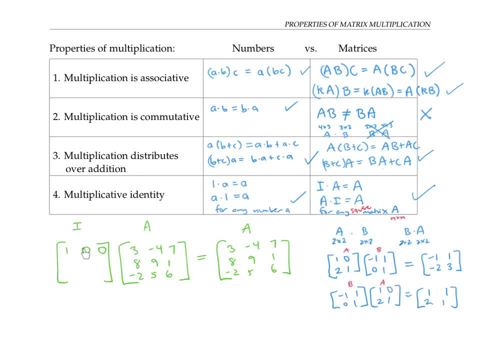 I multiply this row by this column, I'll get one times three plus zero times eight plus zero times three, Zero times negative two, which just gives me the first entry: three. Similarly, if I multiply 100 by the second column of A, I'll get one times negative, 40 times 90 times five. 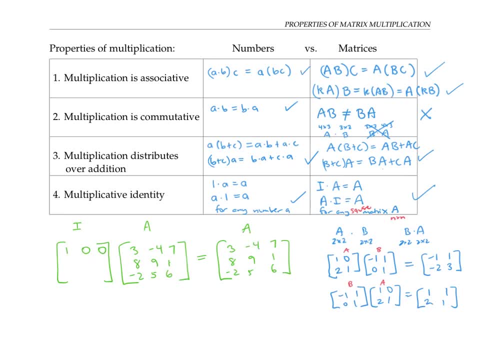 which picks off the number negative. four first row times the third column picks off the number seven. Now, looking at the second row of numbers, when I take the second row of I and multiply it by the first column, I need to get the number eight When I multiply. 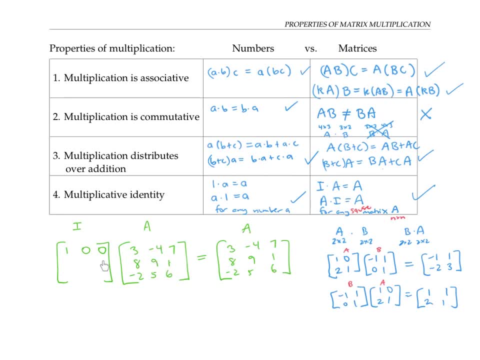 it by the second row of numbers, I get the number eight. When I multiply it by the second column, I need to pick off the number nine. When I multiply by the third column, I need to pick off the number one. Well, I can do that if I make the second row of I be 010.. 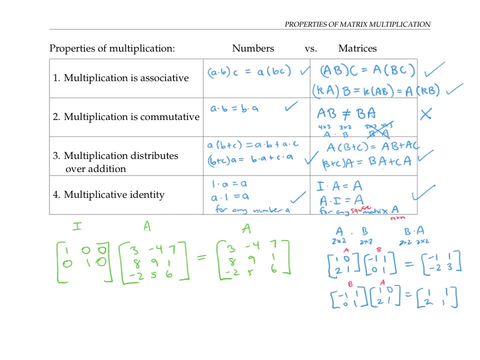 Finally, when I multiply the third row of I by each column of A, I need to pick off these last three numbers. I can do that by letting the third row of I be the row 001.. So this is what my identity matrix needs to look like, And I can check that if I multiply. 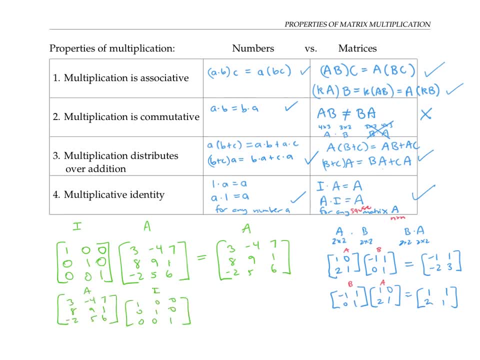 in the other order a times I. I still get back to my original matrix a And there was nothing special about this particular matrix a. if I stuck in any other numbers here, this matrix I would still have done the trick. More generally, the identity matrix for any n by n square matrix will consist of a matrix. 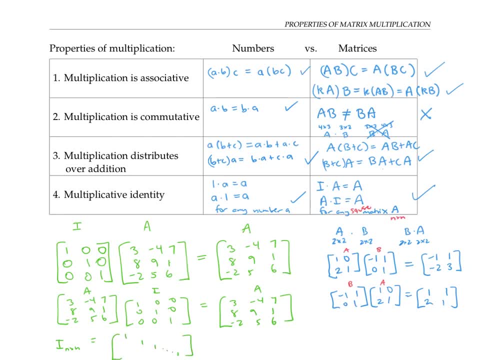 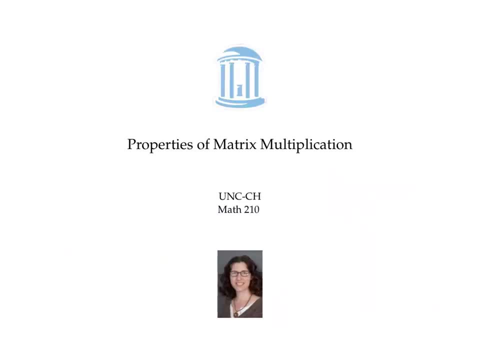 of n ones down the diagonal, with zeros everywhere else. In this video we noticed that matrix multiplication is associative, It is not commutative, It is distributive And there's a multiplication identity. I In a previous video we worked out the mechanics of matrix multiplication. 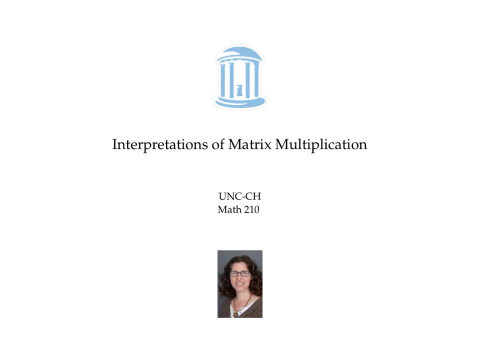 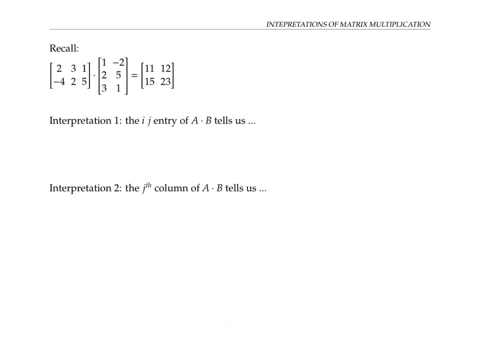 This video focuses on interpretations of matrix multiplication, particularly in terms of the columns of matrices. Recall the mechanics of matrix multiplication. If we multiply a times B to get C, then to get this top left entry, if the answer matrix C, we take the top row of A and multiply it by the left row of B. 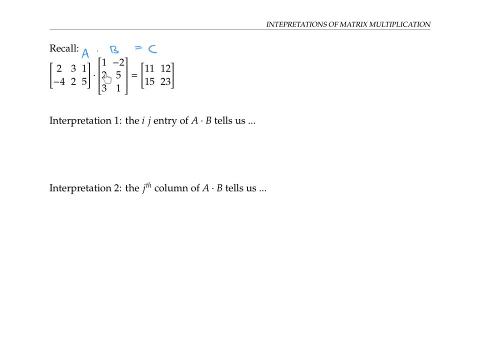 one element at a time. two times one plus three times two plus one times three gives us 11.. To get the entry in the first row, second column, we do the first row A times, second, column B, And in general we saw the IJ entry of A times. 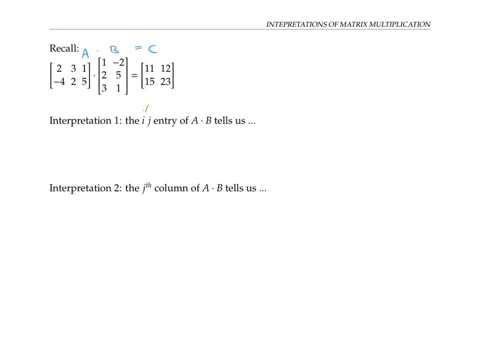 B, But at the top of A times B we have 1 times C. This means that the answer matrix in this: we lift the first row A times the second, column B And we do the first row A times the second. I mean the entry of A times B in row i and column j. we get this by taking the product. 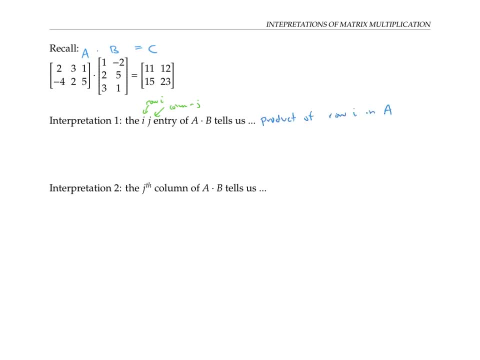 of row i in matrix A and column j in matrix B. Recall that to take the product of a row vector and a column vector, we multiply the corresponding entries and add them up. Sometimes this is called a dot product. But instead of thinking of this matrix product element. 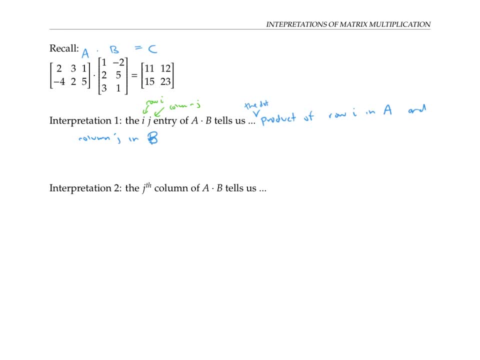 by element. I want to think of it column by column. What does the first column of this answer, matrix C, represent? In fact, this column 1115 comes from multiplying the matrix A by the first column of B. That makes sense if you think about where each of these entries 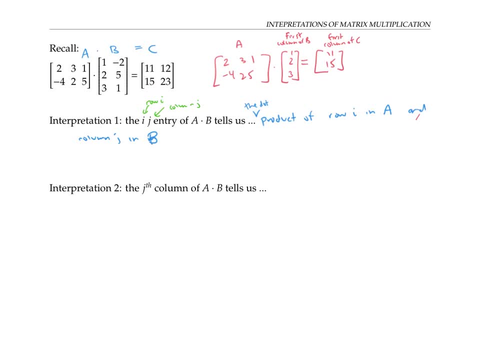 of the first column of C comes from The top entry comes from the top row of A times the first column of B. The next entry comes from the next row of A times the first column of B. All the entries of the first column of C come from multiplying rows of A by the first. 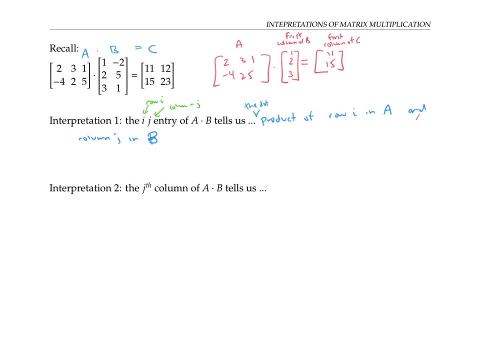 column of B in order. So that's just the same thing as multiplying the matrix A by the first column of B, And similarly, to get the second column of C we can multiply the whole matrix A by the second column of B. So in general we multiply two matrices, A times B, then the jth column. 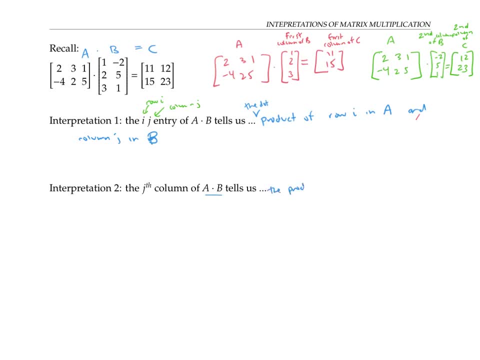 of A times B tells us the product of A with the jth column column of B. One way to write this is if you have a times a bunch of column vectors, I'll call them x1, x2, say x3, x4. In case we have four column vectors and B, then this is the. 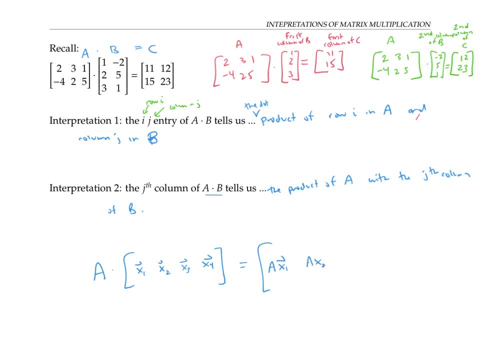 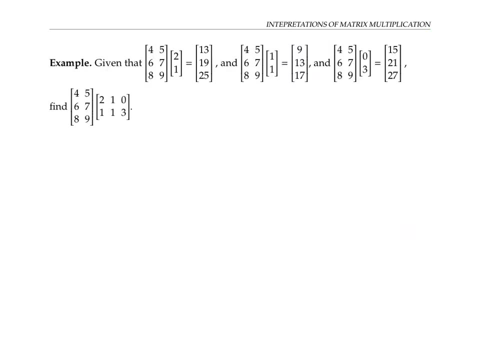 same thing as just multiplying a times each column vector and sticking them together into a matrix. Let's apply this column interpretation in an example. Suppose we know that we have a matrix here- we'll call it a- And we know that a times this column vector gives us this: 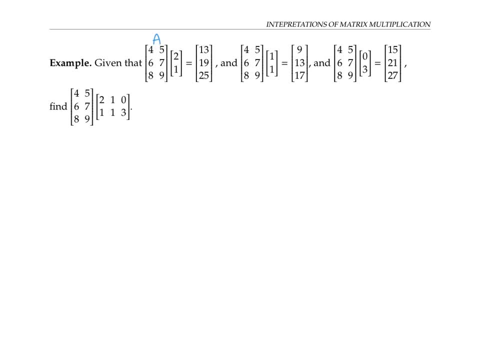 column vector knows the dimensions work out fine And the arithmetic works out fine. And I've also pre calculated that a times this other column vector is this column vector and a times this third column vector column vector gives us this column vector. So now if we want to multiply the same matrix, 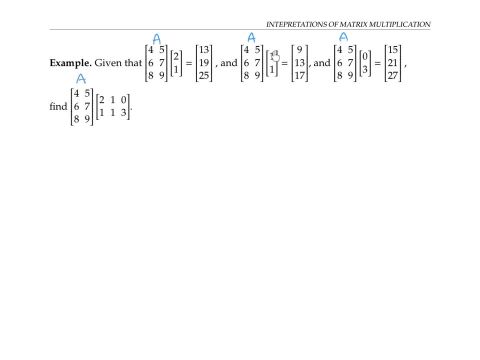 a times the matrix we get by sticking those little two by one column vectors all together into a two by three matrix. that's just the same thing as doing a times two: one as the first column, a times one, one as a second column, a times 03 as the third column, And so it's. 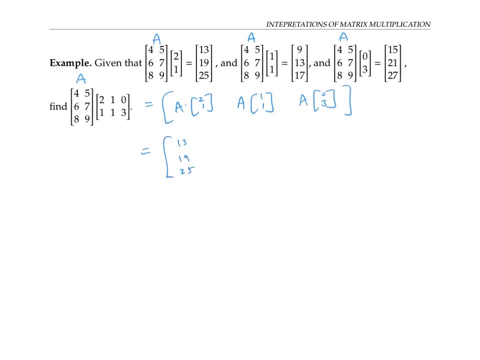 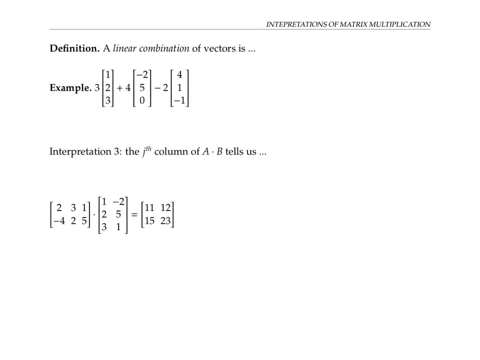 just the same thing as concavity, catenating all those column answers like this. Before I look at the third interpretation of matrix multiplication, I want to define a linear combination of vectors. A linear combination of vectors is just a sum of scalar multiples of the vectors. So, for example, 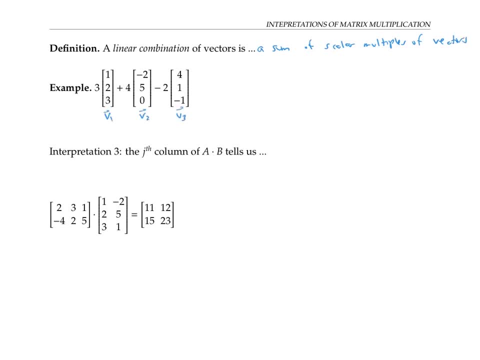 this is our vector: v1,, v2, and v3.. Here we've written down a linear combination of three times v1 plus four times v2, plus negative two times v3. These scalars- three, four negative two- are called the coefficients in the linear combination. So there's a third interpretation. 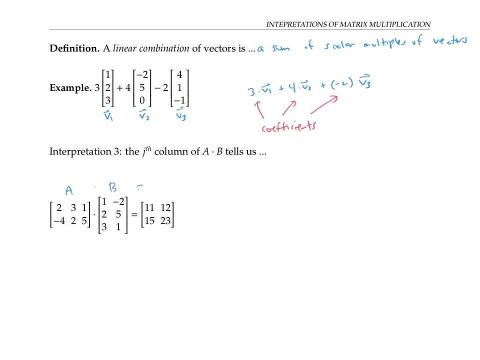 of matrix multiplication a times B equals C. that focuses on the columns of A and B as well as the columns of C. So this interpretation says that the jth column of A times B tells us the linear combination of the columns of A with coefficients given by the entries in. 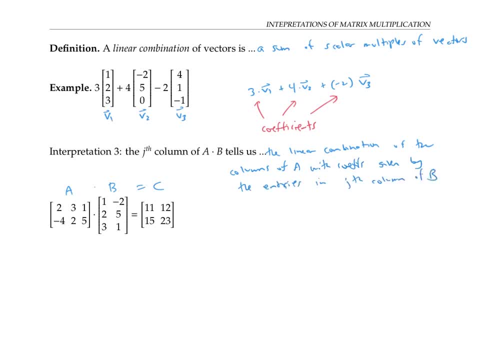 the jth column, column of B. Let me show you what I mean. So to get, say, the first column of C, we're going to use the entries in the first column of B to tell us that we want one times the first column of A plus two times the second column of A, plus three times the third column. 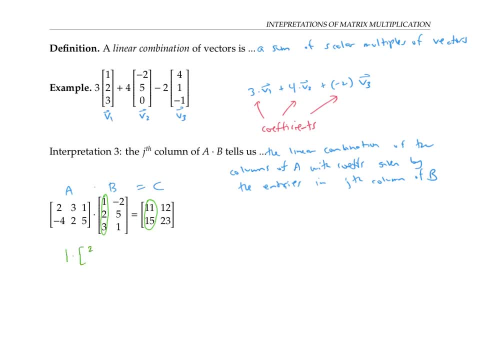 of A, That's one times two negative four plus two times three. two plus three times one five, And you can check that that adds up to the first column of C 1115.. Right, because one times two plus two times three plus three times one, that's. 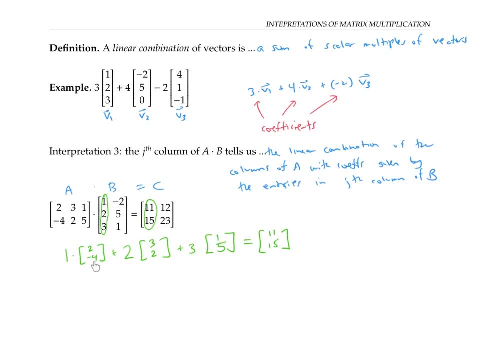 two plus six plus three, which is 11.. One times negative: four plus two times two plus three times five, that's negative. four plus four plus 15, which is 15.. Similarly, to get the second column vector Of C, we can use these numbers in B to tell us that we need the linear combination. negative. 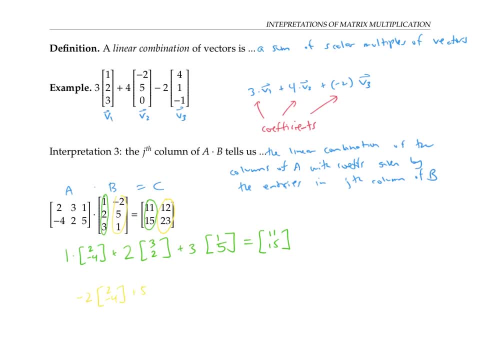 two times the first column of A, plus five times the second column of A, plus one times the third column of A. you can verify. that really does does give us this column of C. it makes sense that this works because we saw before that each column of C just comes. 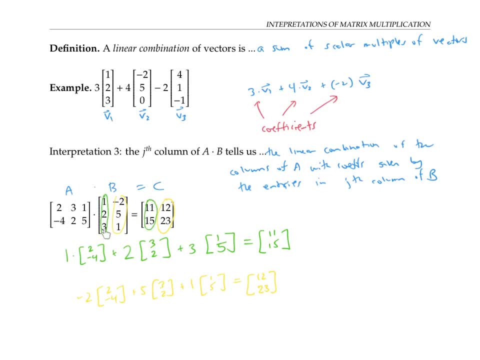 from multiplying a times the corresponding column of B and we multiply a matrix A by the column. then we're doing a bunch of dot products, right, dot product of this with this, and then the dot product of this with this. But each dot product is just the same thing as taking a linear combination. 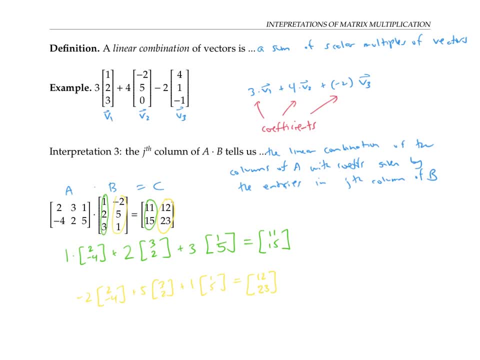 of entries of A, where the coefficients of linear combination are given by the column of B. So we're taking a linear combination of these three numbers sticking in the first entry, linear combination of these three numbers sticking in the second entry. that's just doing a linear combination of. 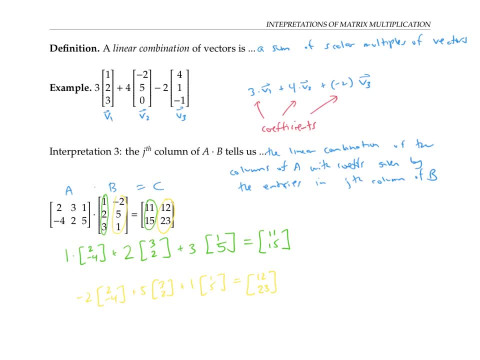 each column and sticking it in the column. If we want to write this out in notation, then if we write the columns of A as say v1, v2, v3, let's use the same matrix B- then the columns of C will be one times v1 plus two times v2 plus three times v3 for the first. 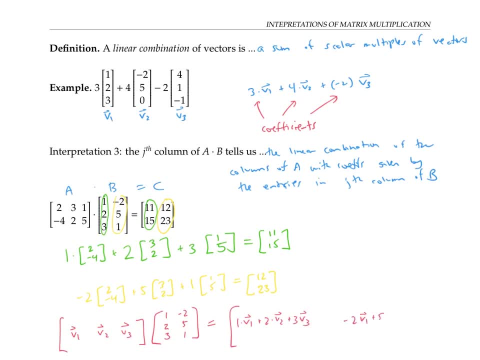 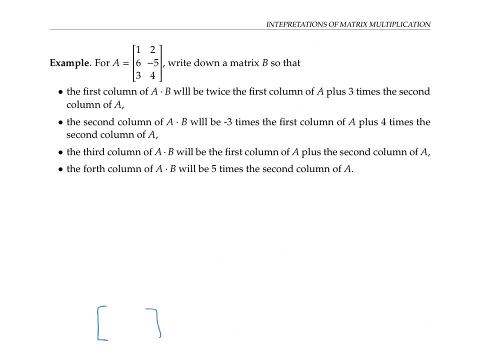 column and negative two v1 plus five v2 plus one times v3. for the second column, Let's do an example in which it's useful to think of the matrix product: a times B equals C in terms of linear combinations of columns of A. So let me copy down my matrix A And I'm going. 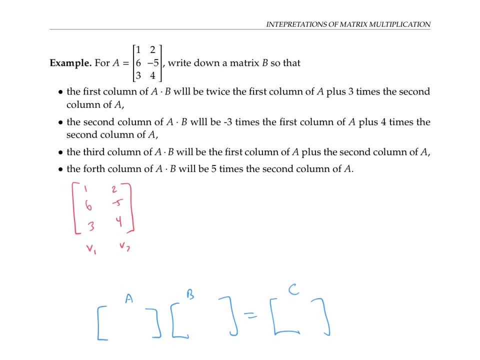 to call its column vectors v1 and v2, I need to multiply it by a matrix B And my answer: matrix is going to have in its first column two times v1 plus three v2.. That's because my first instructions say that the first column of A times B will be twice, or. 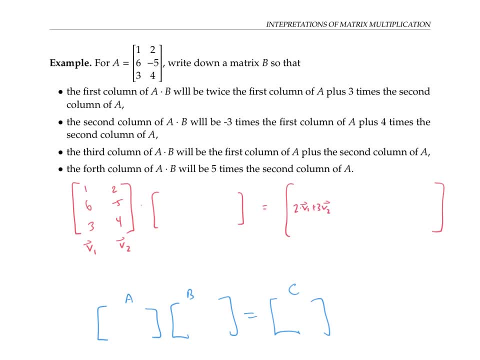 two times the first column of A plus three times the second column of A In its second column. negative three times the first column plus four times the second column. that's going to be negative three v1 plus four v2.. The third column will be v1 plus v2.. And the fourth column five times the second column. 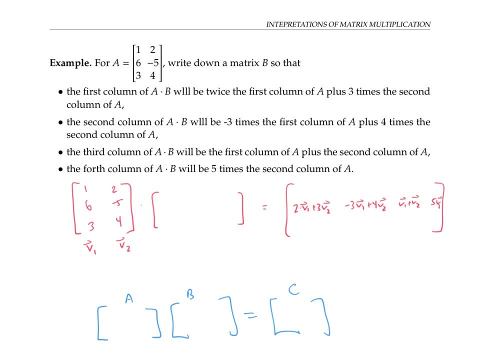 that's just going to be five v2.. Well, we know that we can think of matrix multiplication as each column of B telling us giving us instructions for linear combinations of the columns of A, And so the first column of B has to be instructions: take twice v1 plus three times. 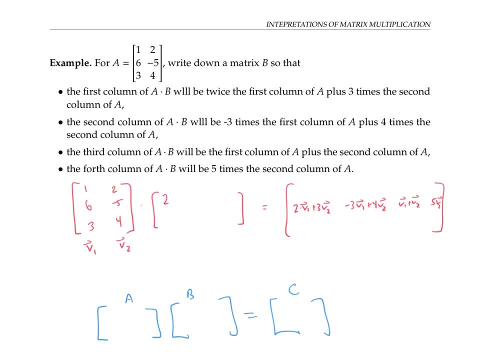 v2.. That means we need an entry of two here and entry of three here, Since the next column of C is supposed to be negative three times the first column of A plus four times the second column of A- our instructions- and B are negative three or four. Similarly, the third column. 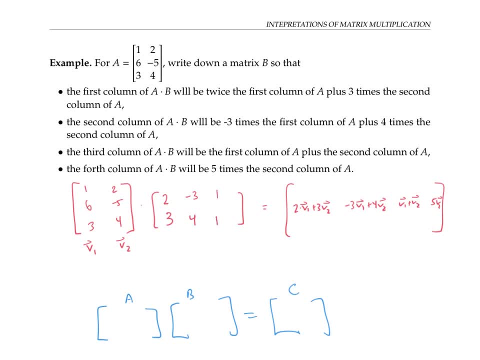 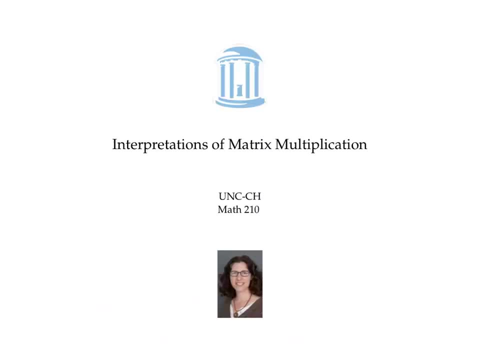 of B needs to be 11.. And the fourth column of B needs to be 05.. In this video we talked about three interpretations of matrix multiplication. The first interpretation is that the entry, the IJ entry, of the product A times B is the. 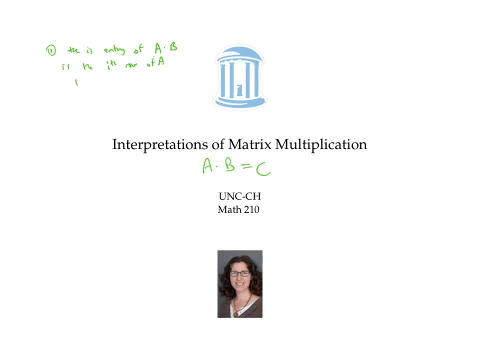 ith row of A times the jth column of B. The second interpretation of matrix multiplication says that we can think about the columns, The columns, The columns Of the answer, as being A times the columns of B. So the jth column of A times B is A. 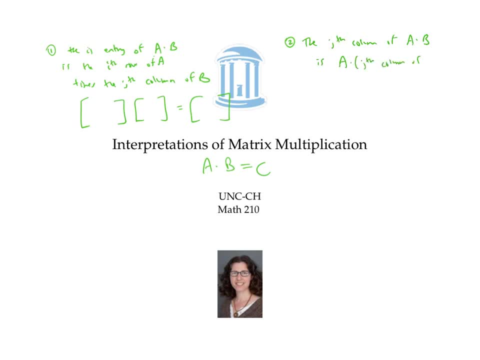 times the jth column of B. Finally, the third interpretation says that the jth column of A times B is a linear combination. Is a linear combination of the columns of A with coefficients given by the jth column of B. There are other interpretations of matrix multiplication as well, But these three will. 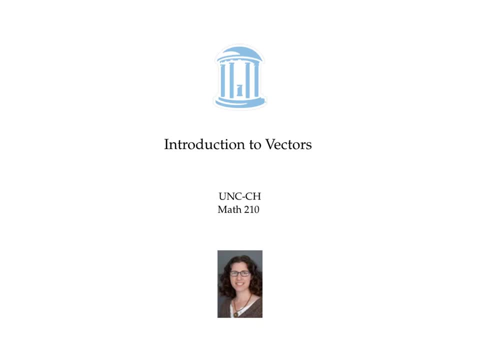 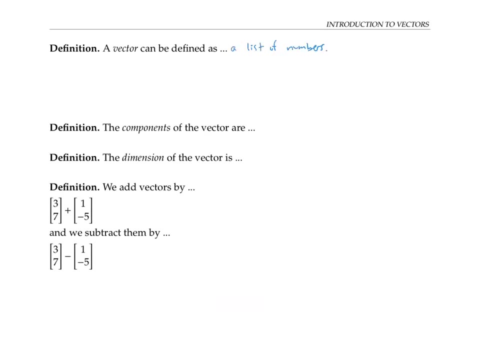 give us the tools we need for now. This video gives an introduction to vectors and basic operations on them. A vector can be defined as a list of numbers. If the numbers are written vertically, then the vector is called a column vector. If they're written horizontally, then it's called 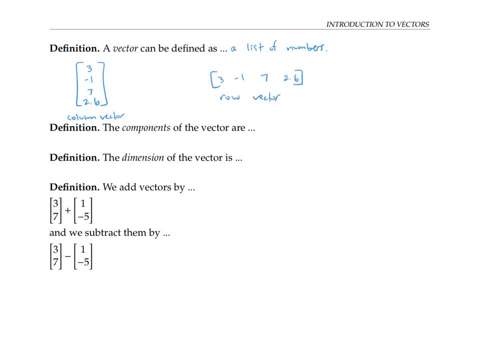 a row vector. We'll be working with column vectors for the rest of this video. I'll use square brackets to surround the numbers in my vector, But you may see other notation elsewhere, such as angle brackets. When I assign a variable name to a vector, I'm going 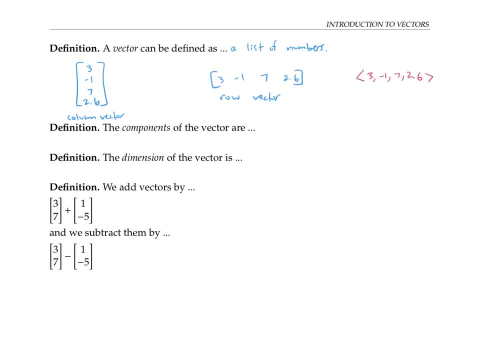 to use a square bracket. I'll put a little arrow above it to signify a vector, But you may see other notation elsewhere, such as boldface or a little hat. The components of a vector are the numbers or entries in the list, And the dimension of the vector is the number of entries. So here my vector. 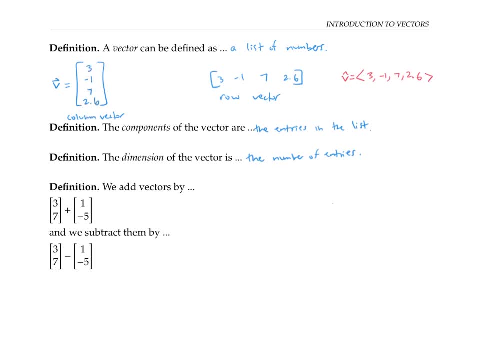 has dimension four because it has four components. The first component is three, the second is negative one, the third component is seven and the fourth component is 2.6.. So the first component is two. For the rest of this video I'll be working with vectors of dimension two, for simplicity. 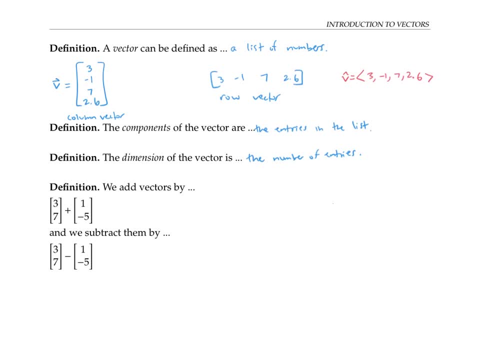 But everything I talked about does generalize to vectors of higher dimensions. We add two vectors by adding their corresponding components. So to add these two vectors, we add three plus one to get four as the first component and seven plus negative five to get two for. 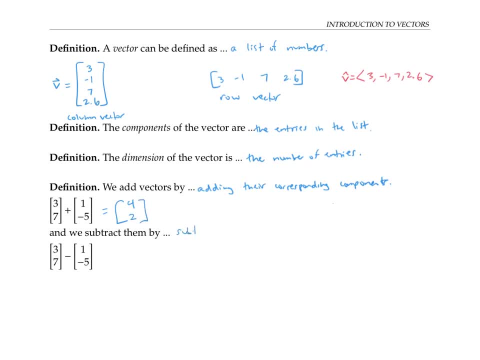 the second component. we subtract them by subtracting their components. So here I do three minus one, which is two, for the first component, and seven minus negative five, that's seven plus five, which is 12.. For the second component, a scalar is another word. 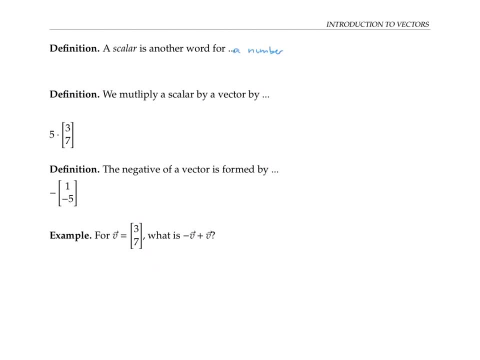 for a number And we can multiply a scalar by a vector by just multiplying each component of the vector by that number. Okay, So here in this example, if we want to multiply five by the vector with components three and seven, we just multiply five times three and five times seven to get 1535.. The negative: 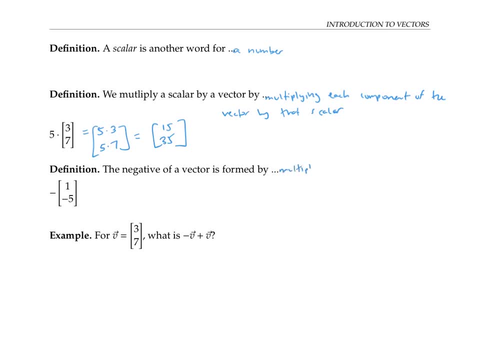 of vector is formed by multiplying the vector by negative one. So here the negative of this vector with components one and negative five will just be negative 15. So say, we have the vector v with components three and seven. what's negative? v plus v. 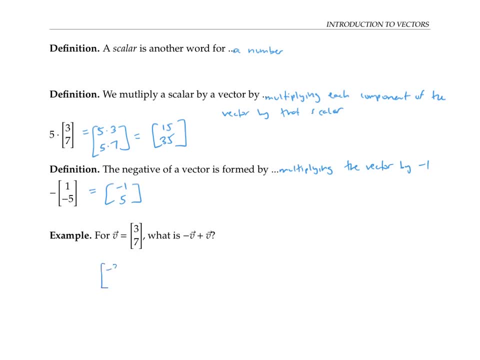 Well, negative v is going to be negative three, negative seven. when we add that to 37, we just get a vector whose components are all zeros. This is called the zero vector, And it's sometimes written as zero with an arrow over it to signify that it's a vector. So 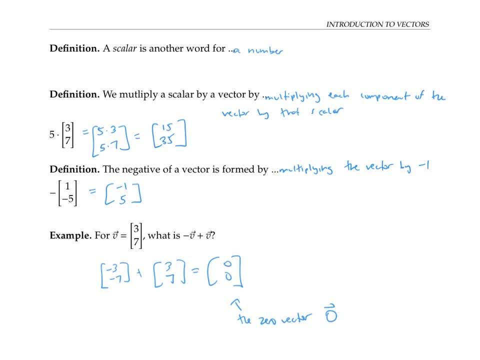 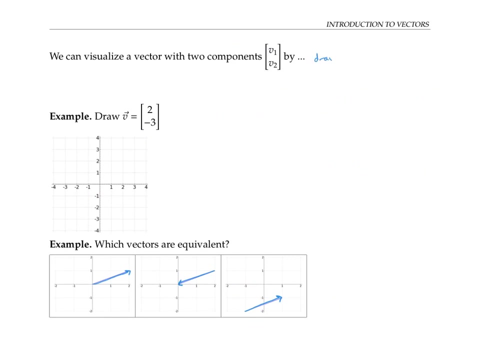 let's say we have a vector with components that are zero and distinguish it from just a scalar zero. In fact, for any vector, v negative, v plus v will give us the zero vector. we can visualize a vector with two components, v one and v two, by drawing an arrow that 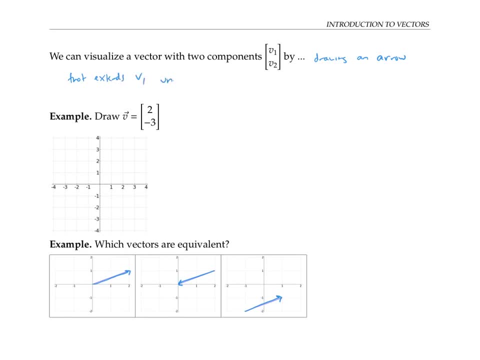 extends v one units horizontally And v two units horizontally Vertically. So, for example, if I want to draw this vector v with components two and negative three, I need an arrow that goes over two units horizontally and down three units vertically. The tail end of the arrow is called its initial point And the arrow. 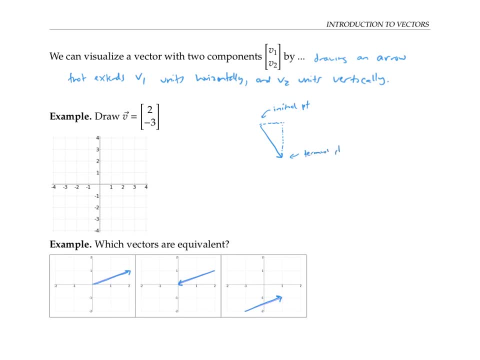 end of the arrow is called its terminal point. It's often convenient to put the initial point, initial point of the arrow, at the origin. So then, going over two horizontally and down three vertically would give me this arrow to represent v, But it's perfectly fine to. 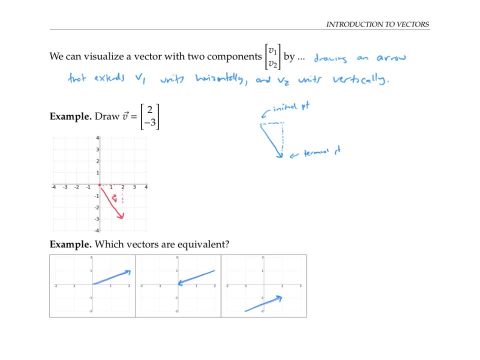 start the arrow anywhere else. So, for example, I could put the initial point here, go over two, down three and get this arrow to represent v, Since it doesn't matter where we put the initial point, only how far over and down we go. we say that a vector has a length and 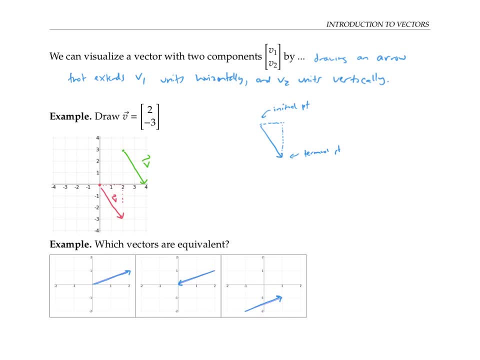 a direction, but not a position. Any two arrows that can be dragged over to lie on top of each other represent the same vector. So which of these three arrows represent the same vector? The first one and the third one? do they both represent the vector with components to one? 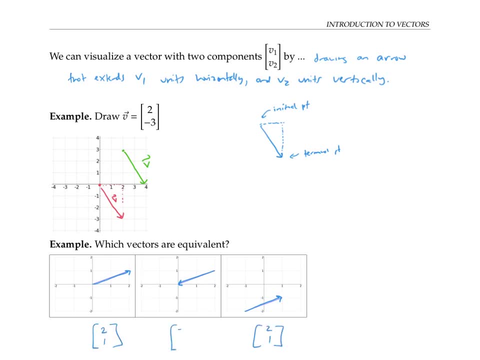 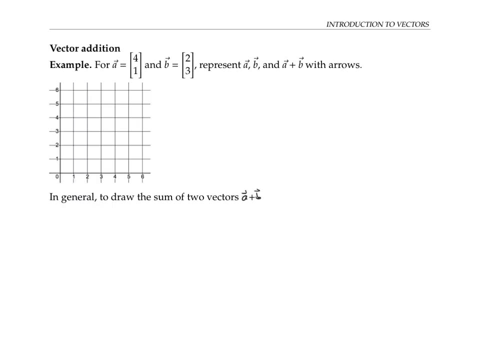 But the middle vector has components negative, two, negative one, So the middle vector is actually a negative one. So the middle vector has components negative, two, negative one, So the middle vector is actually the negative. of the other vectors We've already talked. 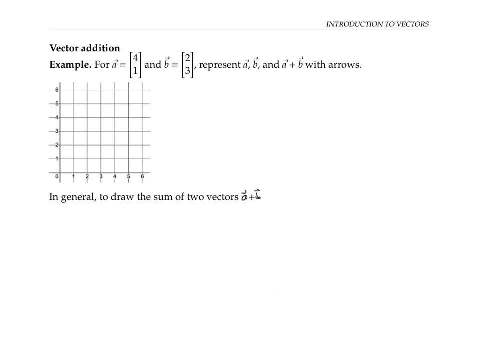 about adding vectors together component by component. But let's see what a vector addition looks like when we draw arrows. First, I'll draw a vector A in blue over four and up one, And I'll draw a vector B in red over two and up three. Now to get the vector A. 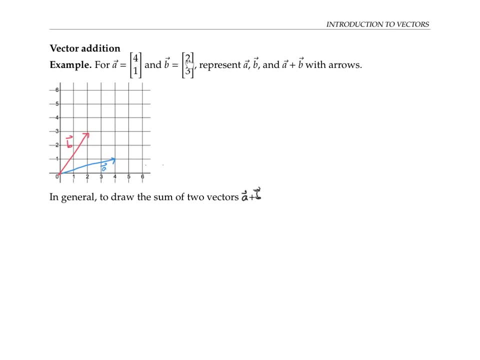 plus B, I have to go over horizontally four plus two units and up vertically one plus three units. So if I start at the origin, where a starts, then my terminal point would be all the way over here at 64. This is exactly the same place I get to if I translate over. 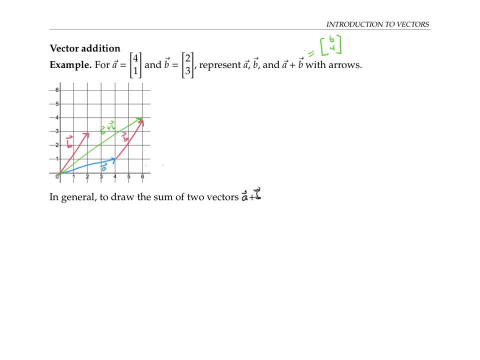 my vector B so that its tail is at a tip, And then draw an arrow from the tail end of A all the way to the tip of B And in general, to draw the sum of two vectors, A plus B. we move the vector B over, So its tail is at A's tip, and draw 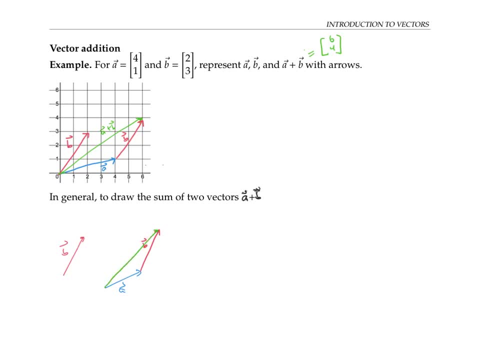 a line connecting the tail of A to the tip of B. It makes sense that this is the same thing as adding component wise, because if the vector A has components A1 and A2, and the vector B has components B1 and B2, then the arrow that I've drawn in green is going. 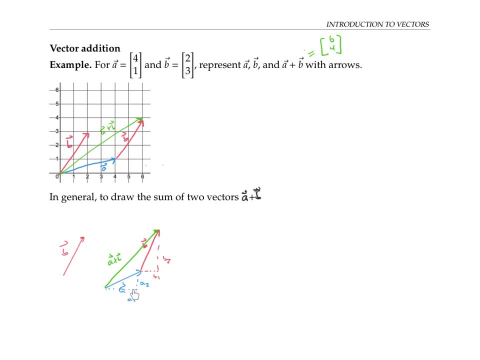 to extend horizontally by A1 plus B1 and vertically by A2 plus B2.. An alternative and equivalent way of drafting back drawing vector addition with arrows is to put the two vectors with their tail end at A1 and B2, and then draw a line connecting the tail end of A to the 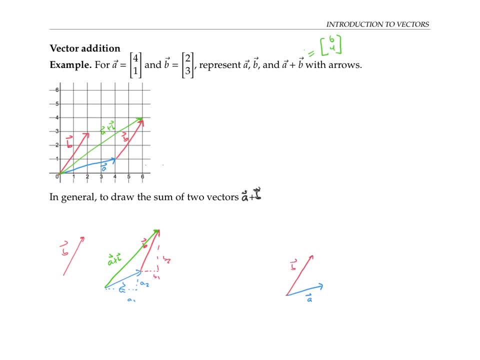 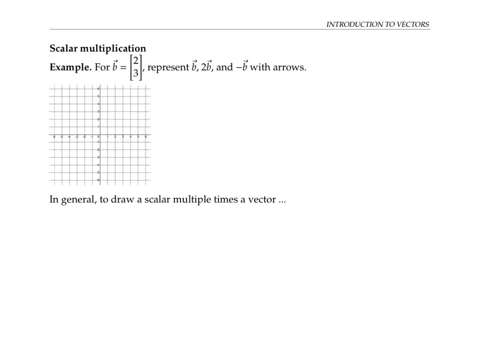 tail's together and form a parallelogram, And now the vector sum is the diagonal of that parallelogram. Next, let's represent scalar multiplication with arrows. Let me draw my vector B for starters. then the scalar multiple to B is what I'm going to call the 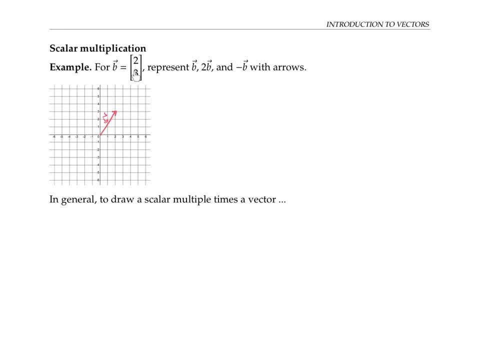 vector B is what I get by multiplying each of its components by a factor of two, So that vector is going to go twice as far horizontally and twice as far vertically. In other words, to B will point in the same direction but be twice as long. The vector negative B will. 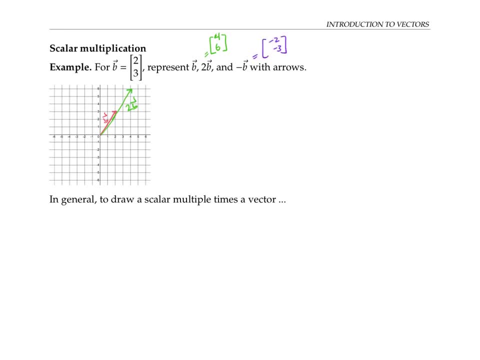 have components negative, two, negative, three, so it will have the same length as B but point in the opposite direction. And in general, to draw a scalar multiple times a vector, say k times v, if k is positive we draw an arrow, k times as long as v, in the direction of v, And if k is less than zero, 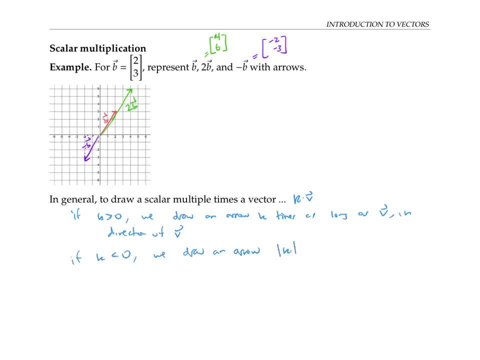 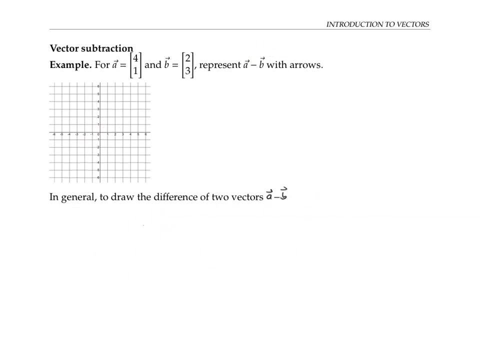 we draw an arrow, the absolute value of k is zero. And if k is less than zero, we draw an arrow, the absolute value of k times as long as v in the opposite direction as v. Finally, let's represent vector subtraction with arrows. Let me draw my vector A and my vector B Now. 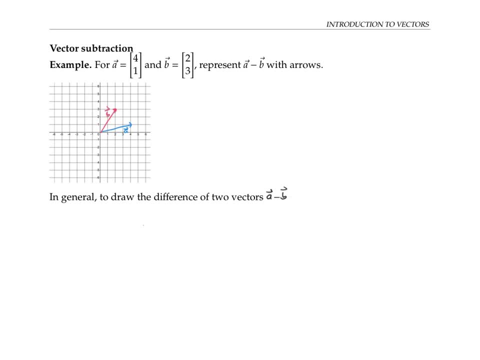 A minus B is the same thing as A plus negative B. So let me draw negative B on here. let's just be going in the opposite direction. So here's negative B, And now I want to do a plus negative B. Well, that's the same thing. 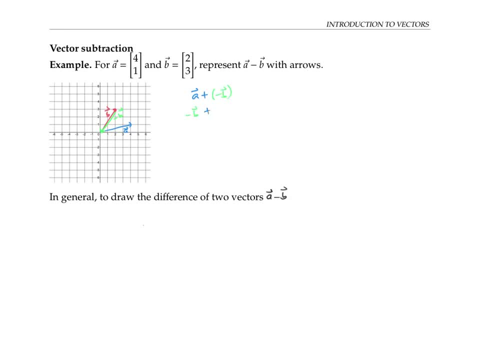 as negative B plus a. Now to do negative B plus a, I just have to put them tail to tip. Well, hey, they're already tail to tip. And then I draw the line from the tail of negative B to the tip of a. this line right here is my a minus B. 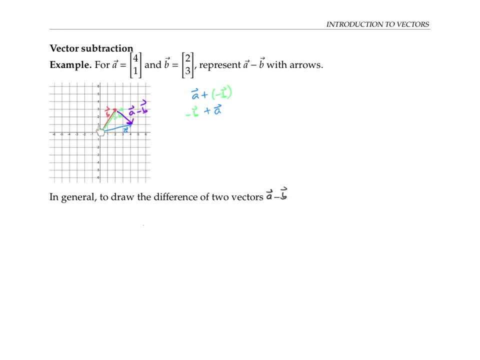 One way to check this is to look at what if we, what happens if we add B plus a minus B? Well, geometrically that means we get this vector right here, which is a, and that makes sense. B plus a minus B should equal a. So in general, let's draw the difference of two. 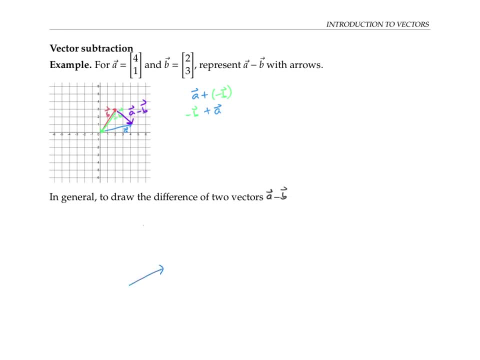 vectors A minus B. One way is to just add a plus minus B, But as a shortcut we could put the two vectors tail to tip tail and then draw a vector from the tip of B to the tip of a. Our last topic for this video is the length of vectors. What's the length of the vector? 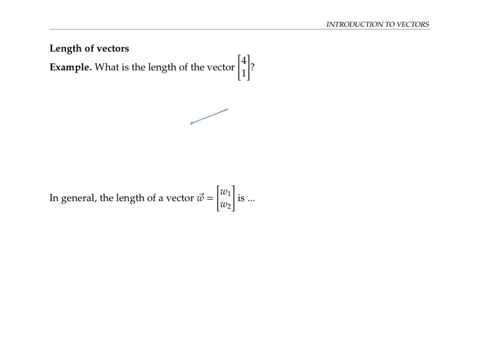 with components four and one. Well, since it goes over horizontally by four and up vertically by one, And this figure forms a right triangle, I can use the Pythagorean theorem to find the length of the arrow which is the hypotenuse of my right triangle: Pythagorean. 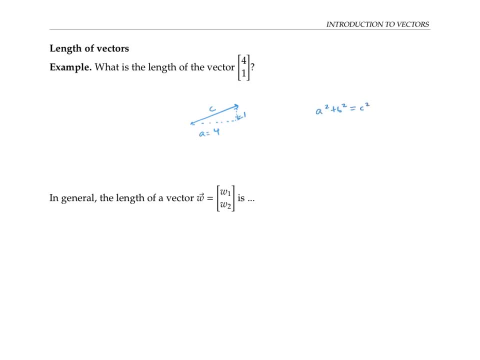 theorem says: a squared plus b squared equals c squared, And so see, the length of the hypotenuse is a square root of a squared plus b squared, or, in this case, the square root of four squared plus one squared, which is a square root of 17.. And in general, to find the length of 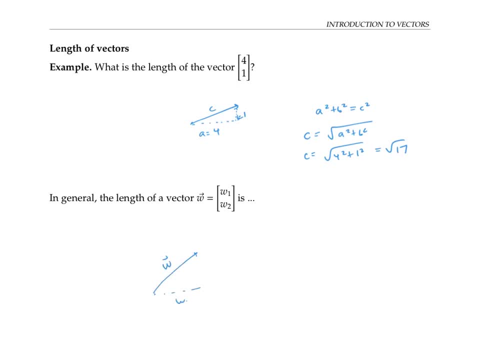 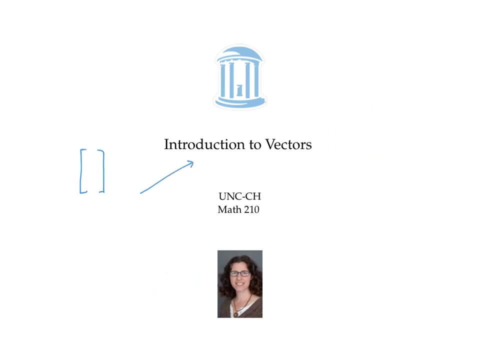 a vector w with components w one and w two. This length, written with absolute value signs, or sometimes double absolute value signs, is given by the square root of w one squared plus w two squared. In this video we've represented vectors with columns of numbers And with arrows. we defined vector addition by adding: 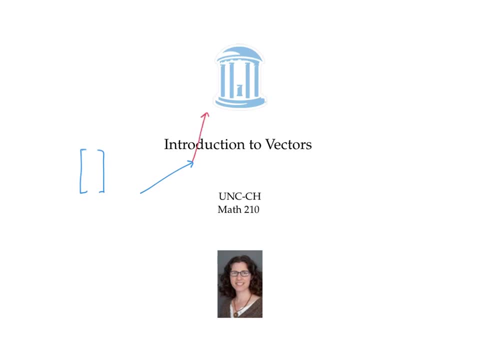 together components and by sticking their arrows tail to tip. And we figured out the length of vectors using the Pythagorean theorem. Although we worked exclusively with two dimensional vectors, vectors with two components that we could draw on the plane, everything we talked about generalizes to vectors of three. 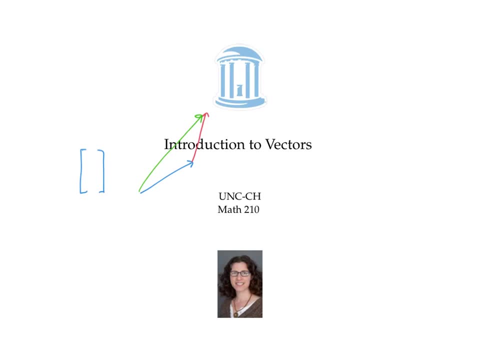 dimensions or higher dimensions. In particular, if we wanted the length of a vector with, say, three components, we would use the generalized version of the Pythagorean theorem: add up all three of its components squared And take the square root of that. This video is about solving the equations of the form. 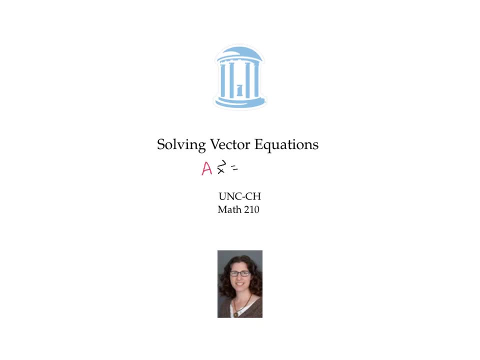 a times x equals b, where a is a matrix, B is a vector And x is a vector that we're trying to solve for. We'll spend a bit of time focusing on equations of the form a: x equals zero, where this is the zero vector. 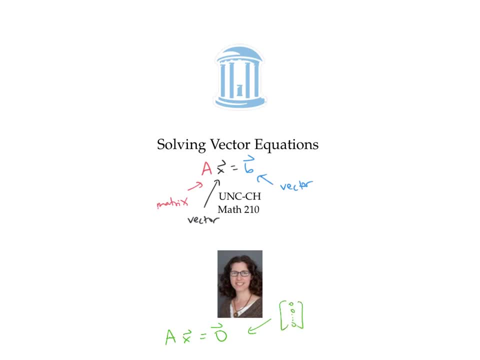 equations of this form where we have all zeros on the right hand side. These are called homogeneous equations. Let's start with this example. we're trying to solve the equation a times x equals b for x, where a is this three by three matrix and B is this length. 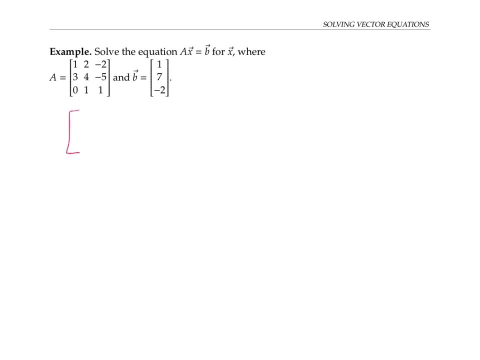 three column vector To make the dimensions work out, I'm going to need my vector a and x to be a three dimensional column vector also. That way, when I multiply a times x to get B, I'll be multiplying a three by three matrix by three by one column vector to get 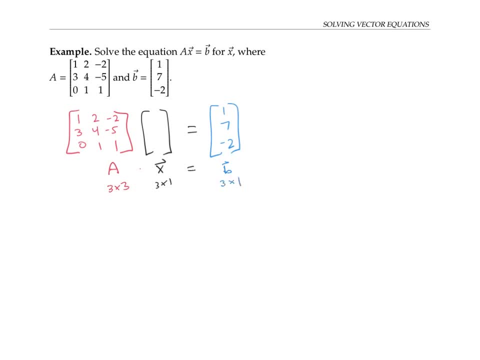 a three by one column vector, as I want to. But this vector x is completely unknown. It's what I'm trying to solve for, Since it has three components, I'm going to use three variables- x, two x three, to refer to those components. And I'm trying to solve for those components. 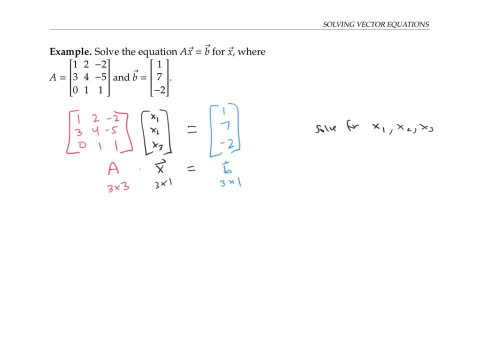 x one x two x three. Now if I work out the matrix multiplication, the left side of this equation becomes the matrix: one times x one plus two times x two minus two times x three. in the first row. three x one plus four x two minus five x three in the second row: 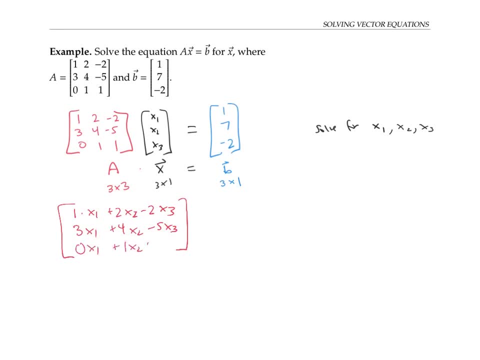 and zero x one plus one x two plus one x three in the third row. So this left side is actually now just a column vector right. there's just one entry in each row and it has to equal this other column, vector 17 negative two. So that's just the same thing as this system. 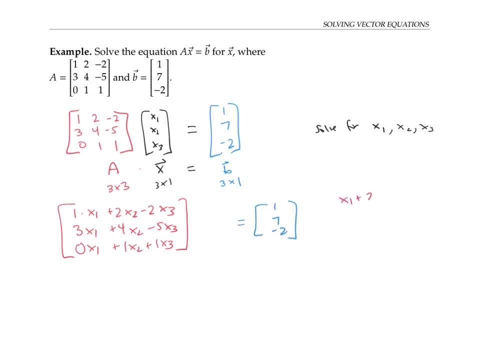 of linear equations: x one plus two x two minus two x three equals one. three x one plus four x three x two minus five x three equals seven and zero. x one plus one x two plus one x three equals negative two. Well, we've seen how to solve systems of linear equations like 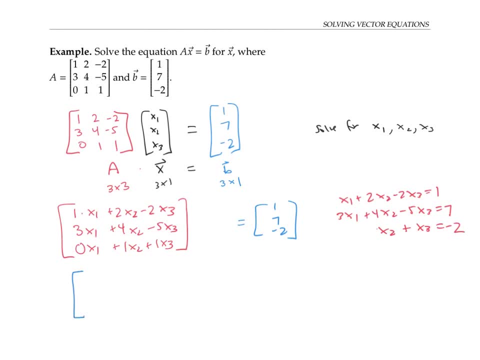 this before. One way is to write it as a matrix 12 negative two. one we're writing out as an augmented matrix where the constants go in the last column of the matrix, Second row. the matrix will be three, four negative five, six, seven, eight, nine, 10,, 11,, 12,, 13,, 14,. 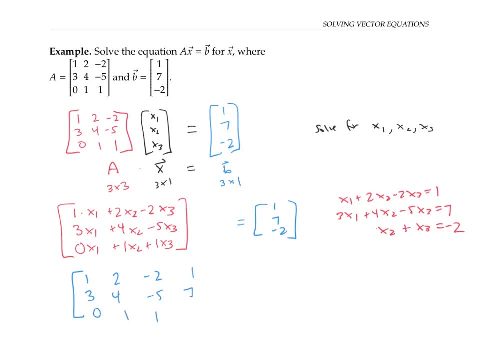 five, seven, and the third row will be 011 negative two. what we'll do is we'll convert this to a reduced row, echelon form, and then we'll be able to read out the solution. Notice that the matrix we're converting is simply the matrix A, augmented with the column B. 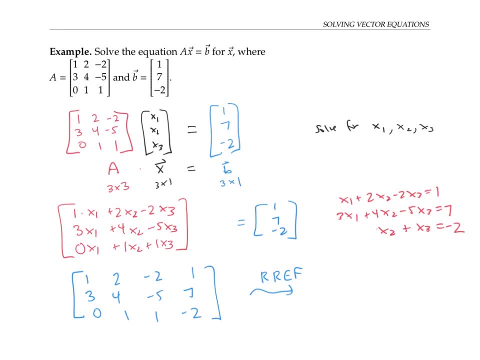 I'll skip the details of converting this to reduce row echelon form, But the final answer looks like this. So we can read off a solution that x one is five, x two is negative two and x three is zero. In other words, there's a unique vector. 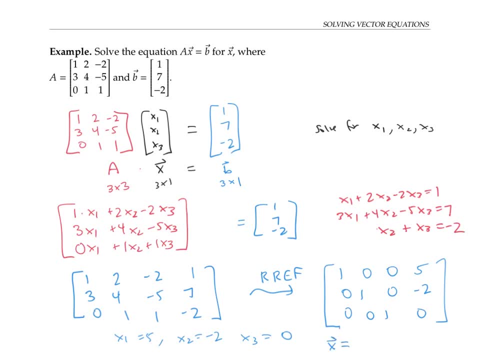 x that satisfies this vector equation And that vector x has components five negative two zero. I'd like to briefly look at a related problem where, instead of solving the equation a times x equals B, we solve the homogeneous equation times x equals zero. Here the zero vector needs to be a three by one column vector. 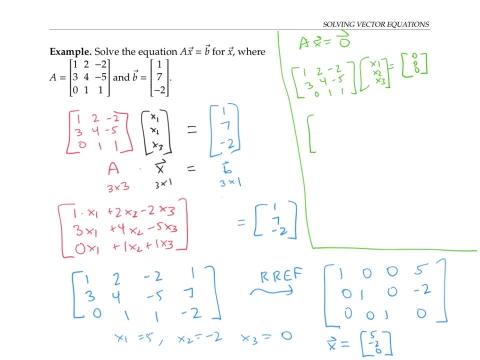 By the same reasoning as before. this amounts to taking the augmented matrix, this time augmented with a column of zeros, and converting it to reduced row echelon form. you can check that when we do this conversion we get this matrix. Therefore, our related vector equation: 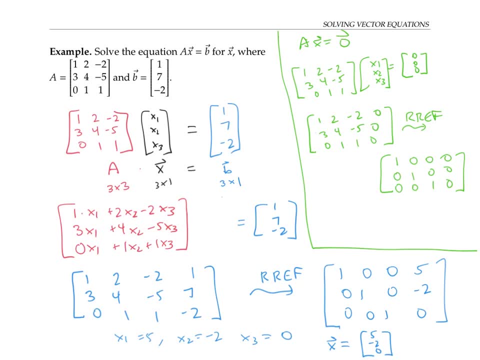 with a zero instead of a B has a unique solution where x one is zero, x two is zero and x three is zero. In other words, the solution is the zero vector. In fact, I could have predicted in advance that the zero vector would be a solution to this equation, with all zeros on. 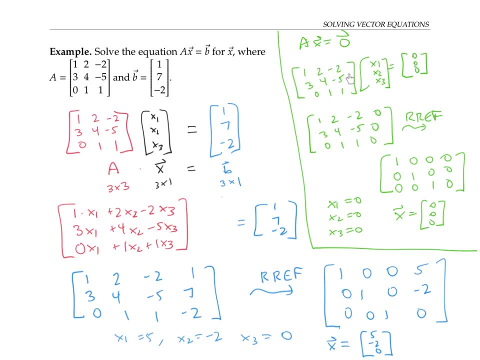 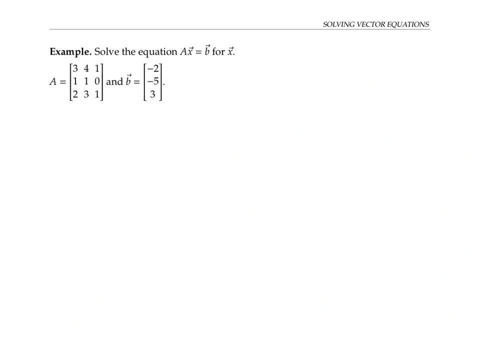 the right side, Because if I multiply any matrix by all zeros, I'm going to get zeros. What I didn't know in advance is that this zero vector is the only solution. That's what working out the reduced row echelon form told me. Let's look at another vector equation Once again. we're. 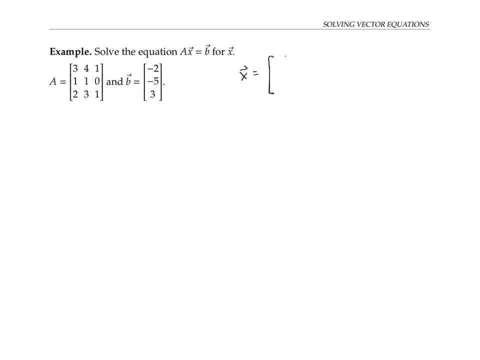 thinking of the vector x as our variable And once again it has to be a three by one vector with three components that I'll call x, one x, two x three. It has to have these dimensions to make the dimensions of the matrix multiplication work. 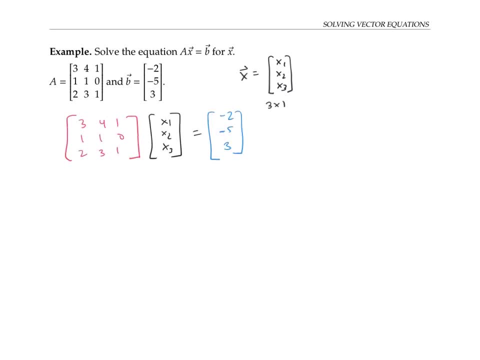 out. This vector equation is the same thing as the system of linear equations And solving the system is the same problem as converting the augmented matrix to reduce row echelon form, where the augmented matrix I can get just by putting a together with the column. 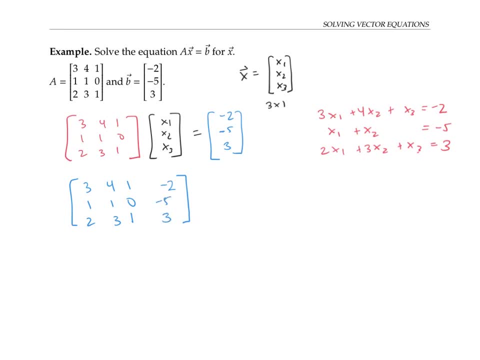 vector B. Once again, we're looking at the linear matrix and we're going to call it this: This vector only has one zero vector, but we're going to make a number of zeros. Once again, I'll omit the details of converting the matrix to reduced row echelon form and 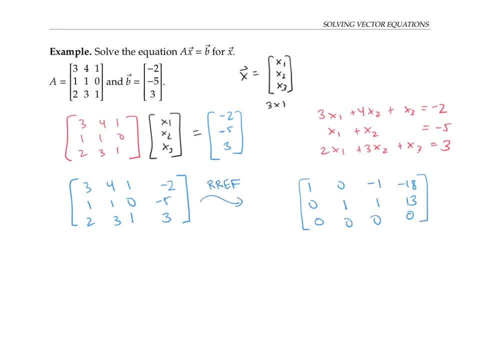 just write out the final answer. In this case, our system of linear equations has infinitely many solutions. I can tell that because I have this column- that's not my augmented constant column- that doesn't have a leading one in it. So this variable x three is a free variable. 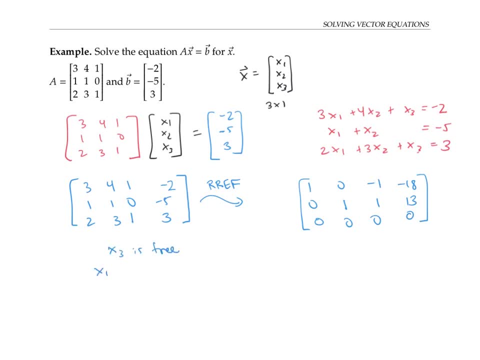 And I can write my other variables, x one and x two, in terms of x three, because x one minus x three is minus 18.. And x two plus x three is 13 comes from these first two rows And therefore I have that x one is x three minus 18 and x two is minus x three plus 13.. 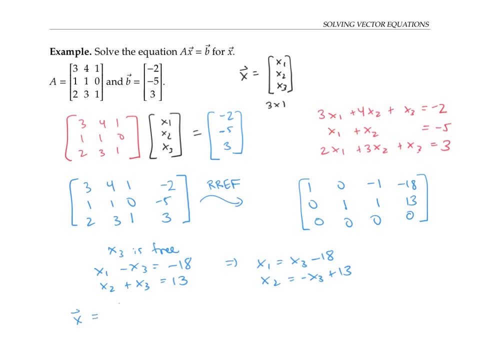 So my vector solutions are of the form x three minus 18, minus x three plus 13, x three, where x three can be anything. I can also write this as a sum of two vectors, one vector that's multiplied by x three. 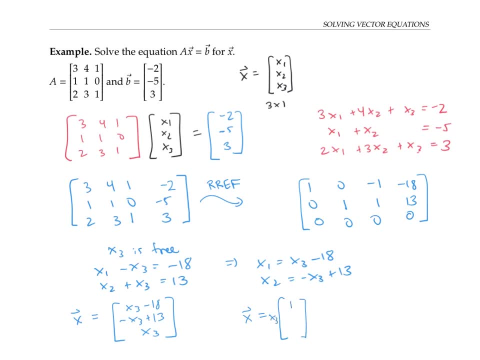 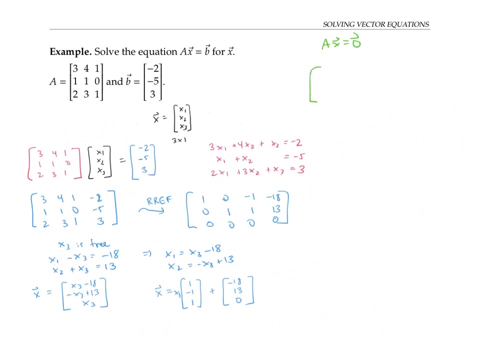 So that'll be x, three times one minus one, one plus a vector that just has constants in it, minus 1813, zero. Okay, Let me once again consider the related homogeneous equation: a x equals zero. solving this vector equation can be accomplished by converting the associated augmented matrix: augmented. 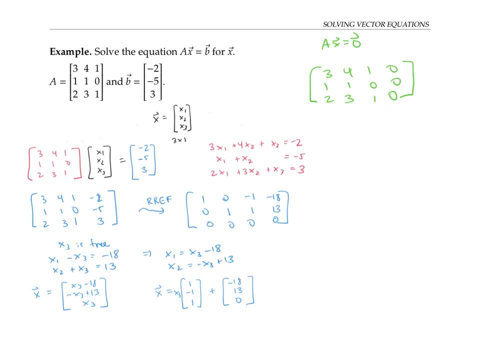 with the zero column vector, converting this augmented matrix to reduce row echelon form. When I do that I get this matrix, The same matrix I had before, just with zeros in the far right column. So the solutions to my a times x equals zero equation are given by x one minus x three. 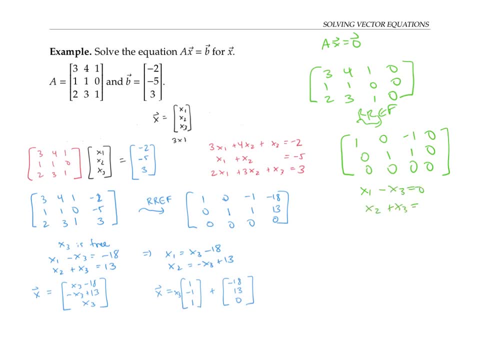 equals zero. x two plus x three equals zero and no conditions on x three. In other words, x one equals x three and x two is negative x three. That's the same thing. I'm saying that the vector x, which originally is x one, x two, x three, is of the form x one. 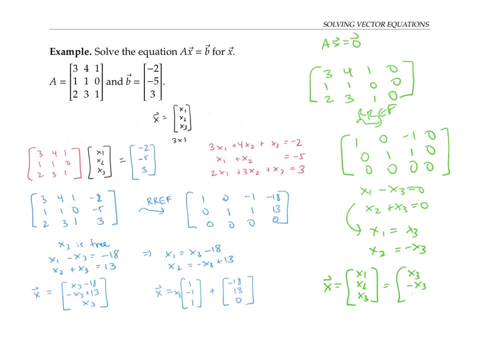 is equal to x three. x two is negative, x three and x three, a free variable, is just itself. So x can be thought of as x three can be anything times the vector, one negative one, one. Notice the similarities between my families of solutions for my two related equations. 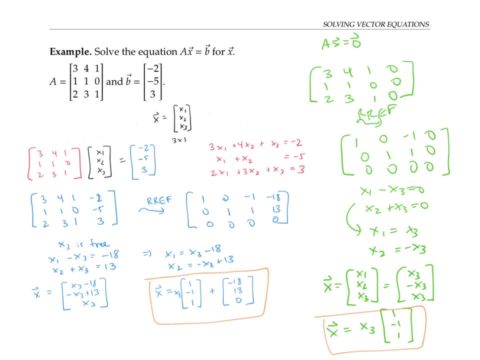 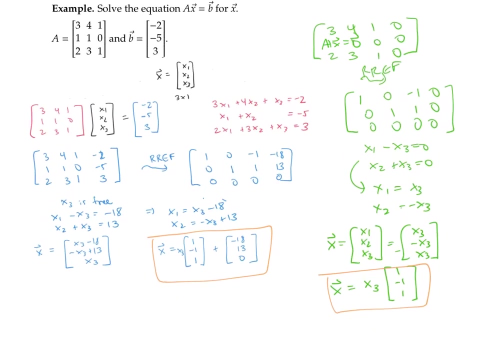 The family of solutions for my equation a times x equals b, is this particular solution negative 1813, zero, plus this expression here, which represents the solutions to my associated homogeneous equation ax equals zero. Another way to say this is that my solutions 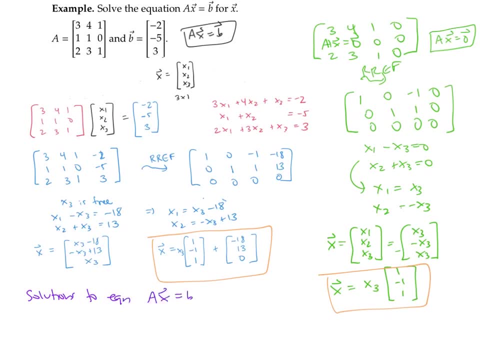 to the equation a, x equals b are of the form: x equals x, three times v plus w, where w is the vector minus 1813 zero. a particular solution to the equation: a: x equals b And v is the vector one. 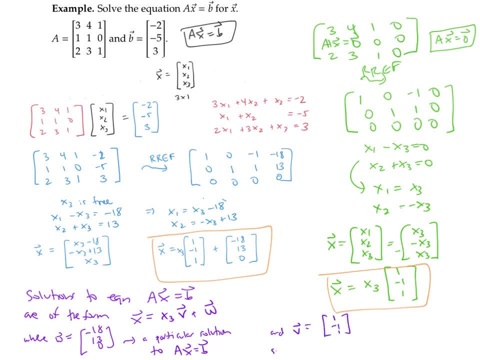 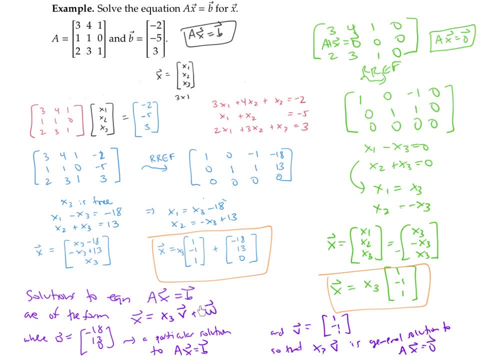 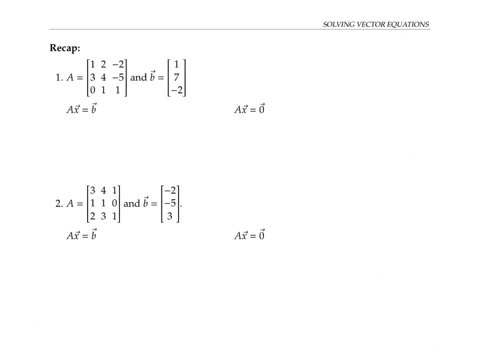 to a: x equals b can be written as a particular solution plus the general solution to the related homogeneous equation: a- x equals zero. Let's recap where we've been In our first example, our homogeneous equation. Let's recap where we've been. 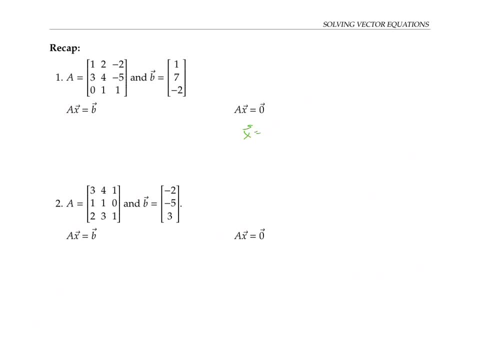 homogeneous equation just had one solution: the zero vector. Our equation ax equals B also had one solution: the vector five negative two zero. In our second example, our homogeneous equation had infinitely many solutions of the form x, three times one negative, one one. 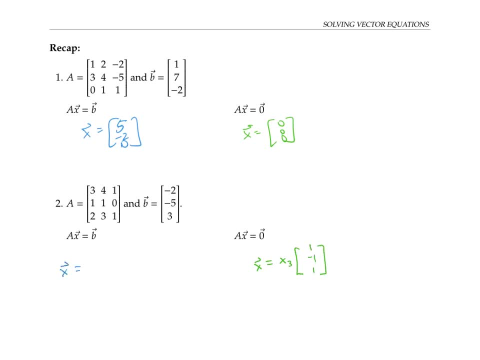 And our original equation ax equals B also had infinitely many solutions of the form negative: 1813, zero plus x, three times one negative one one. These two situations are typical, In fact, if the equation ax equals B has any solutions, in other words, if it's. 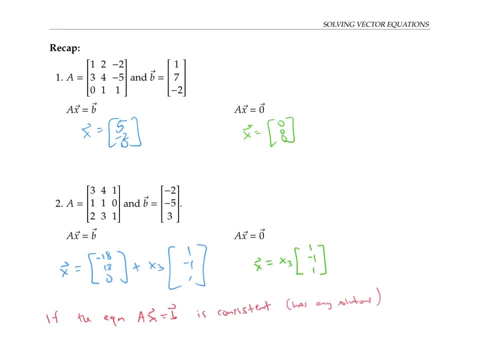 a consistent system of equations, then A x equals B has one unique solution. If, and only if, the associated homogeneous equation ax equals zero has one unique solution, namely the zero vector, and A x equals B has infinitely many solutions. If, and only if, A x equals zero has infinitely 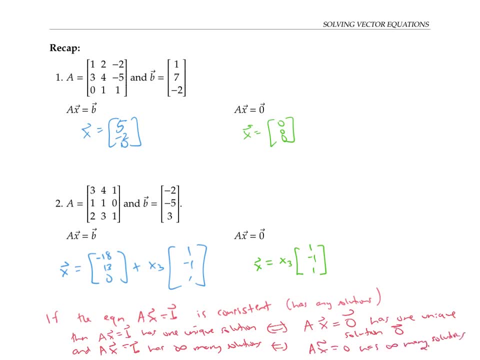 many solutions also. Although I don't have time to demonstrate it in this video, I do want to emphasize that this correspondence only holds if the equation ax equals B is consistent, it actually has any solutions. If this x equals b is inconsistent- no solutions- then anything goes, Well, almost anything. 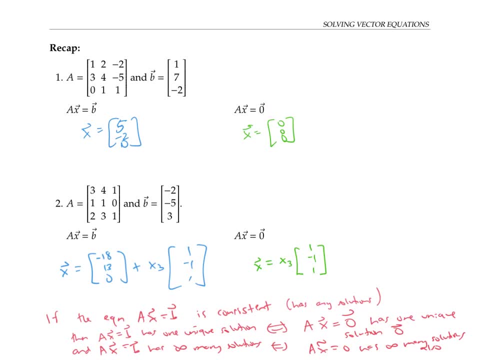 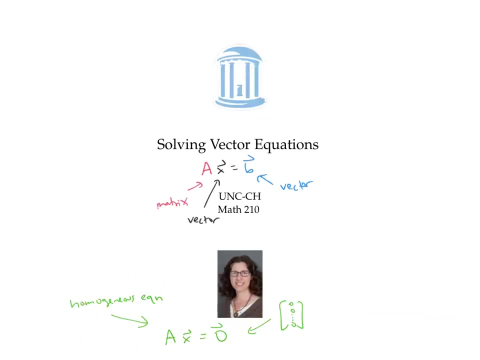 the equation x equals zero will always have at least one solution- the zero vector. but it could have one solution or infinitely many solutions, And this equation x equals b still have no solutions. In this video we solve the equations of the form a: x equals b by 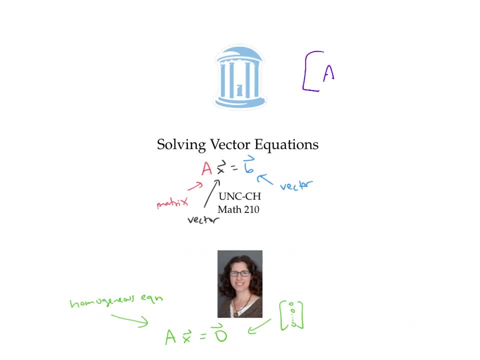 writing down the augmented matrix with a and augmented by B, and then converting it to reduce row echelon form. We also noted that the solutions of a x equals b are related to the solutions of the homogeneous equation a x equals zero, at least as long as the equation. 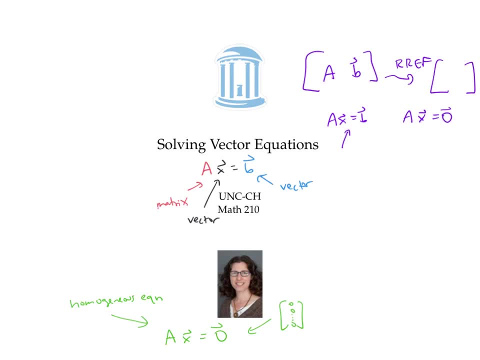 a x equals b has solutions. Specifically, if a x equals b has solutions, then the solution a x equals b has one solution. if, and only if, a x equals zero has one solution and a x equals b has infinitely many solutions. if and only if a x equals zero has infinitely. 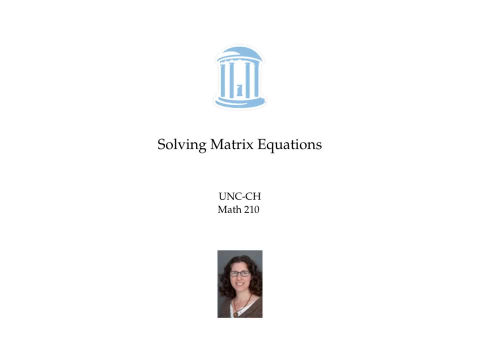 many solutions. In this video we'll solve equations of the form a times x equals b, where a and b are known. In this video we'll focus exclusively on the situation where a is a square matrix- the same number of rows and columns, although x and b might not be square matrices. But 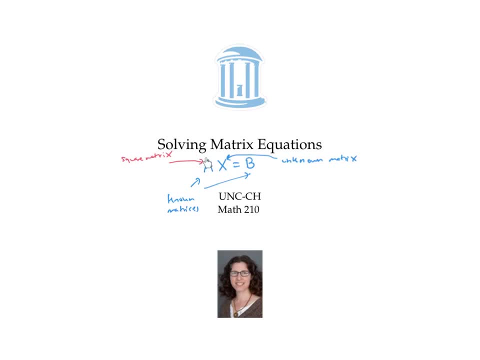 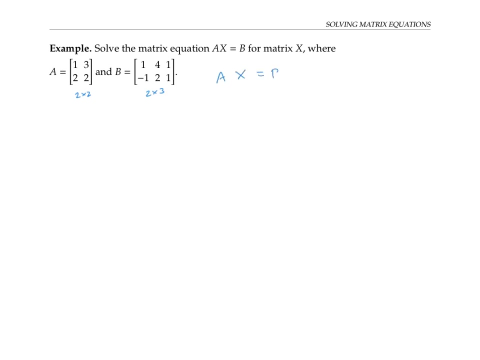 a lot of the ideas will pertain to situations where a is not a square matrix. Let's start with this example: A is a two by two matrix and B is a two by three matrix. So if I want to multiply a times x and get B, what dimension will x have to be In order for the matrix multiplication? 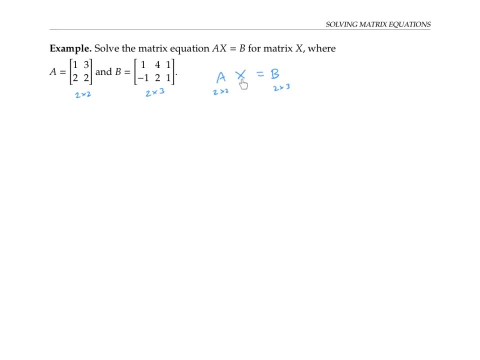 even to make sense, x is going to have to have two rows to match the two columns here of A, And in order to get the right number of columns in the output of B we're going to need A. x is going to have to have three columns. I'm going to call the columns of: 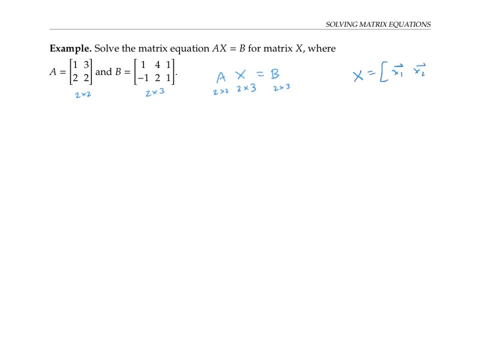 x, x one, x two and x three with that arrow to note that they're column vectors. So we're looking for those column vector so that A times x one, x two, x three is equal to B. In a previous video on interpreting matrix multiplication we saw that when we multiply a matrix we'll. 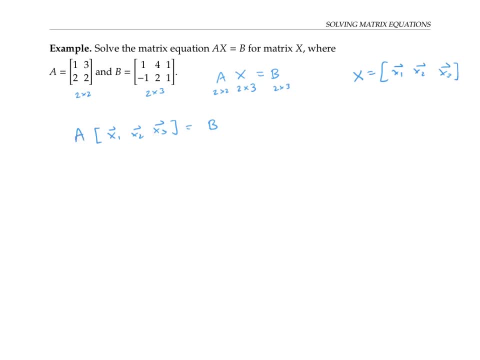 be able to multiply a matrix into two. For matrix multiplication A is a two by three. multiply a matrix by another matrix. we can accomplish that by multiplying the first matrix times each column of the second matrix separately and then just concatenating them together. 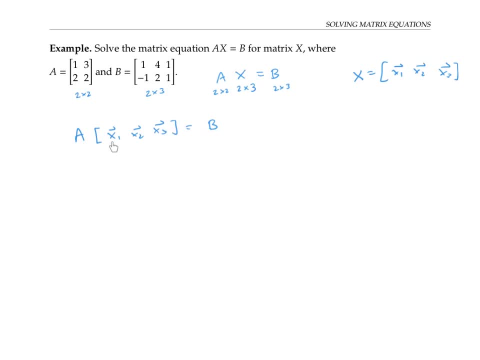 So this expression A times the matrix with columns x1,, x2,, x3, is the same thing, as a result, matrix with columns x1,, x2, x3.. And that has to equal B, which has columns one negative: 14211.. So we know that we need a x one to be the column matrix one negative. 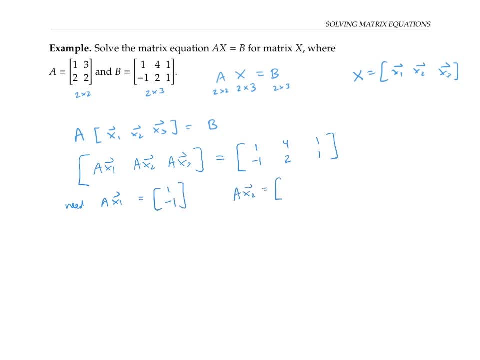 one, a x two to be the column matrix for two and a x three to be the column matrix one. one Hang on a second Back. we've seen how to solve these problems. This is solving a vector equation right: a matrix times a vector is another vector. So all we have to do to solve this first problem. 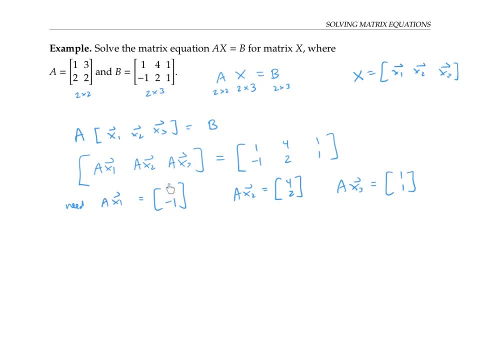 is to augment a with this column, vector one negative one, and put it in row reduced echelon form. to read off our solution. Here's my augmented a. And to put that in reduced row echelon form, I can first leave the first row alone. it's already got a one in the upper left column. 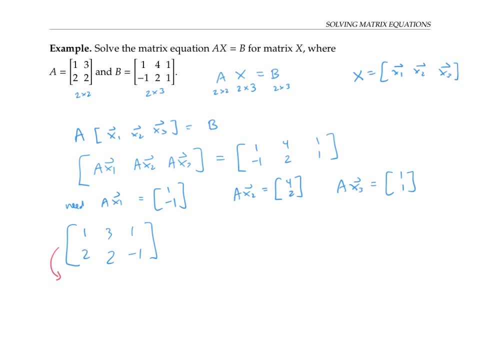 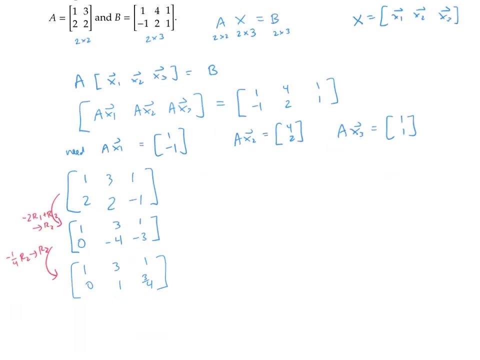 position And I can get rid of this two by replacing the second row with negative. two times the first row plus the second row. Then I can divide the second row by negative four. Finally, get rid of this three by replacing the first row with the first row minus three. 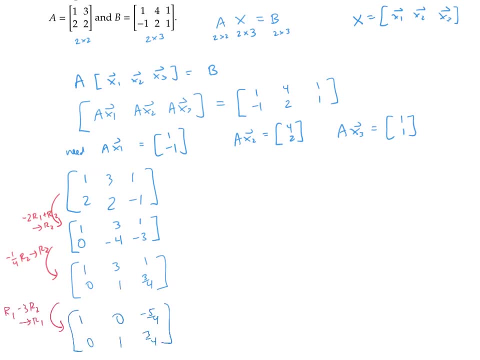 times the second row. Now I can read off the solution. vector x one is going to be the column vector minus five, fourths, three, fourths. Continuing. I need to solve a times x two is a column vector for two, So I'll write down the augmented matrix and start to do. 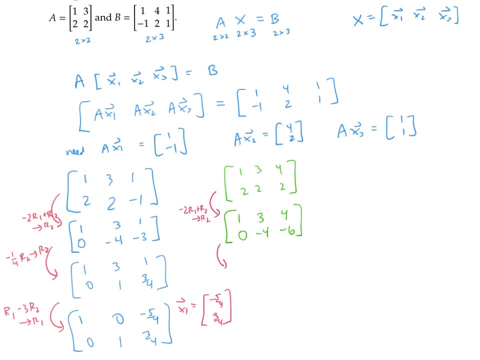 the row reduction. Wait, this is starting to seem familiar. I seem to be going through exactly the same steps as I did before, And that makes sense, Because when I'm doing the steps of row reduction, I'm really focusing on this part of the matrix, trying to get. 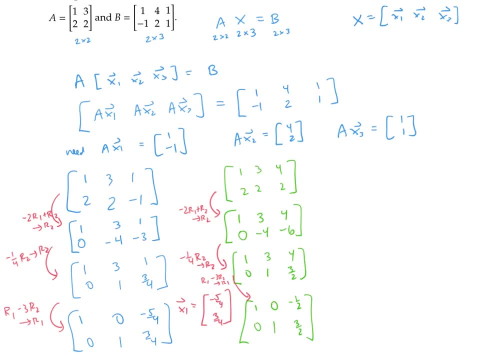 this part of the matrix. It's to have leading ones with with zeros above and below them. This last column just gets dragged along for the ride. So I do get a different answer for my x two column vector. it's going to be negative one half, three halves, But the process I use to get there is the. 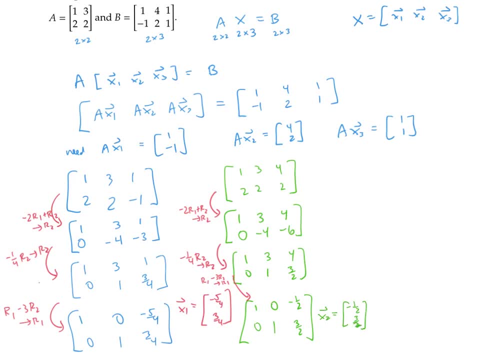 same as what I used for the first column vector, And if I move my attention to solving this third vector equation, I'll go through the same row reduction steps once again. So I'm going to do that. So I have my solution. the matrix x, one x two x three. otherwise, 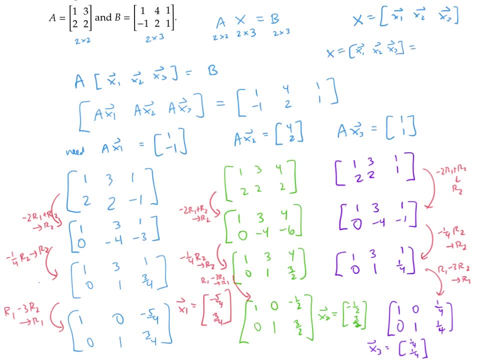 known as x is going to be equal to my three answer vectors strung together. So that's negative five fourths, three fourths negative one half, three halves and one fourth, one fourth. But I also have an idea for how to do this process more effectively, So I'm going 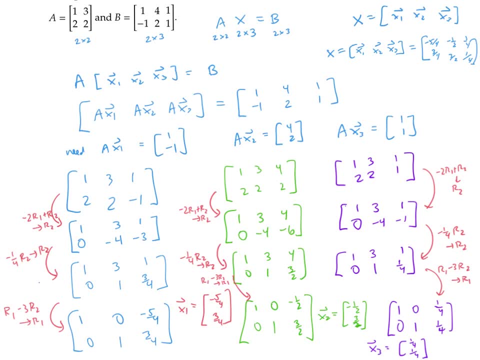 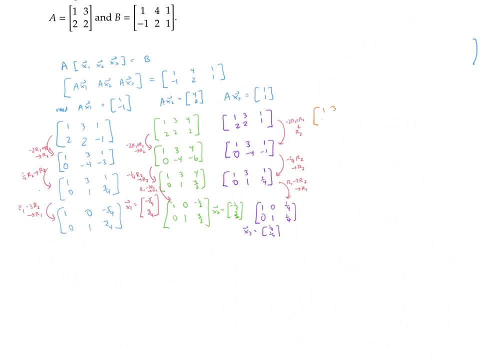 to do this row reduction process three times for the three separate vectors. What if I just string those vectors together and do the row reduction process once? So I'm going to augment a with all three of the column vectors of B And I'll start applying the 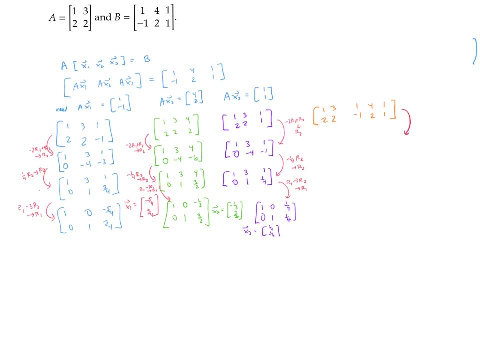 row reduction operations in one fell swoop. The first thing we did was to get rid of that two in the bottom half bottom left corner by replacing the second row with negative two times the first row plus the second row. When I do this, I maintain all the information that I had in the blue. 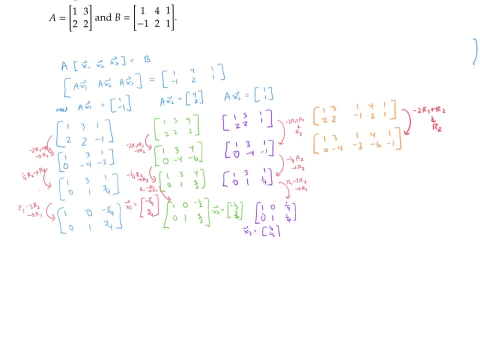 green and purple computations. these first two columns that corresponded to the original columns of a and are the same in the three computations are the same here And then these last three columns are the same as those columns that I did in those three columns And then 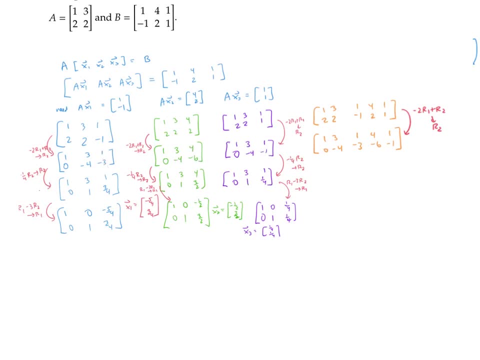 in those three computations before I can also do the next step of the row reduction in one fell swoop And the last step altogether. When I solve the matrix equation in this most efficient way, I can read off my answer: matrix x from the rightmost chunk of my row reduced. 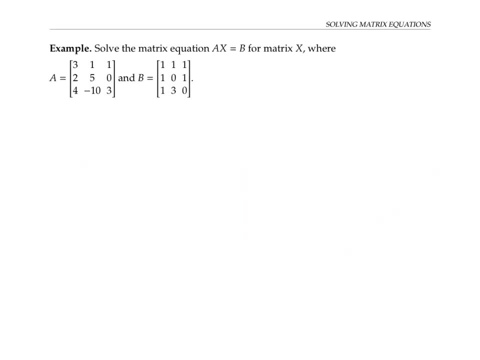 matrix. Please pause the video and try your hand Solving this matrix equation. I'm going to start by writing down the augmented matrix a with B. after it I'll write down the steps of row reduction and leave it to you to verify. 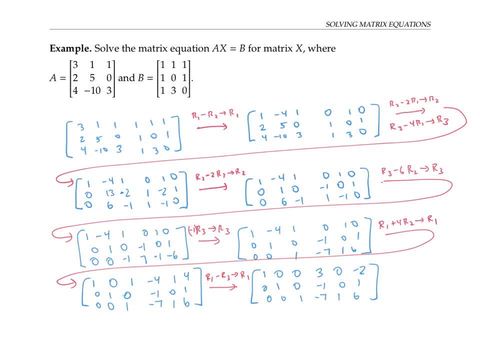 the details. After doing that row reduction work by hand or by computer, we can read off our solution: matrix x. I encourage you to check the work by actually multiplying a times x and verifying that you do get matrix B. I want to point out that the 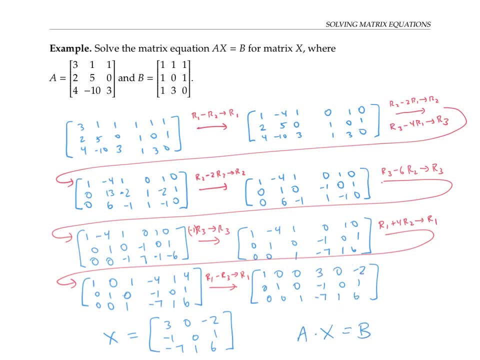 reason we could read off our answer matrix so easily is that after we did the row reduction, the part of our matrix corresponding to a is in a particularly nice form. It looks like an identity matrix with a leading one in each column and no rows that are all zeros If 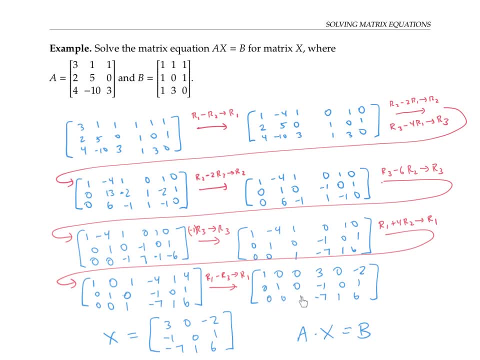 we had gotten, for example, a row of zeros down here and some columns that didn't have leading ones in them, then we would have had to be more careful And we might have ended up with no solution or infinitely many solutions. We'll talk more about those situations in 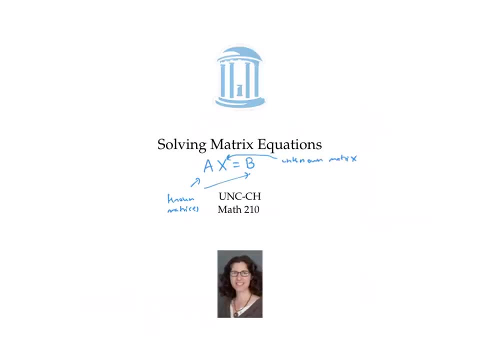 class or in a later video. In this video we saw that solving the matrix equation a times x equals B was equivalent to solving a bunch of vector equations where the unknown vectors x, one through x n, form the columns of the unknown matrix x and the vectors B. 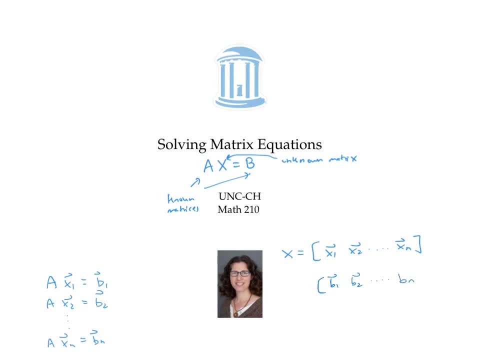 one through B, x, n form the columns of the known matrix B. But rather than solving each of these equations one by one, we saw that it was much more efficient to just augment the matrix A with the matrix B and convert that to reduced row echelon form. When we solve equations with numbers, 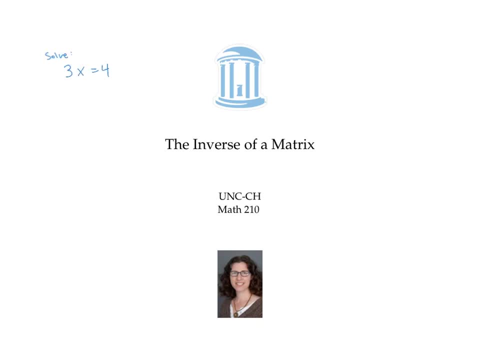 like the equation three times x equals four, we divide both sides by three Or equivalently, we multiply both sides by one third. The number one third is called the multiplicative inverse of three. It's also written as three to the minus one. When 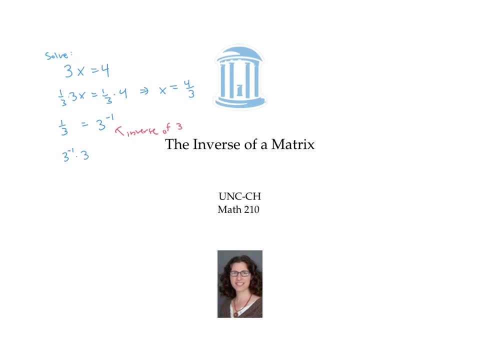 we multiply three inverse by three, we get one, which is why it's so useful for solving equations like this one. If we can find a multiplicative inverse for a matrix, that could give us a good way to solve matrix equations Like a times x equals B, where a, x and B are matrices- a and B matrices that we know. 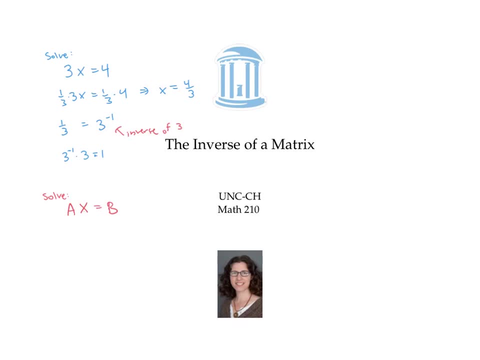 the entries of an X, a matrix we want to find, Recall the matrix I called the identity matrix that has ones down the diagonal and zeros in all its other places. The identity matrix is a square matrix And there's actually one for each dimension, n. So, for example, I three 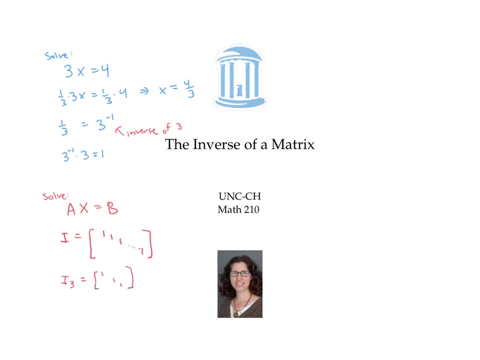 is a three by three matrix that has three ones down, a diagonal and zero as all its other entries, The matrix I plays the role of the number one for matrix multiplication. just like one times any number just gives you the same number itself. If you multiply i by any matrix, you just get. 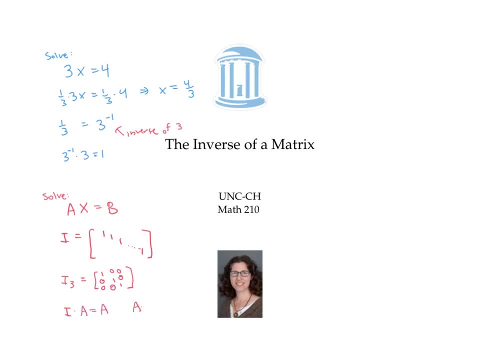 the matrix you started with, And it works if you multiply in the other direction too. So by analogy to numbers, the inverse for a matrix, a matrix, a inverse that multiplies by a to give the identity, It turns out that such a matrix. 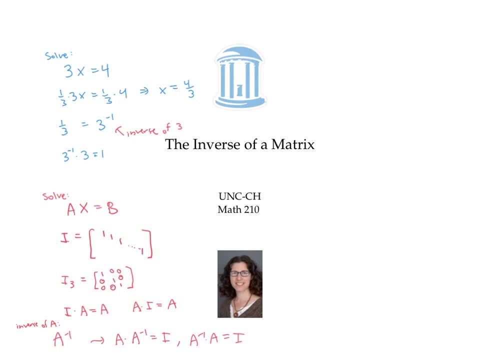 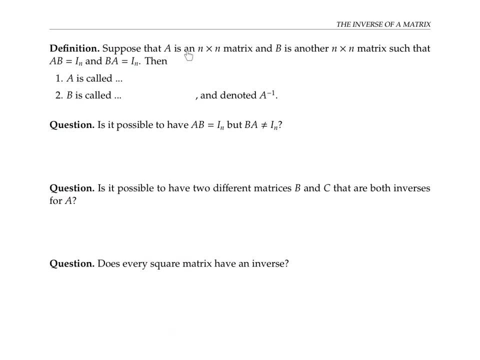 doesn't always exist for every matrix a, but when it does, it's super useful. Let's start with the definition of an inverse matrix. Suppose that a is an n by n square matrix and B is another n by n matrix, So that when you multiply a and B together in either order, 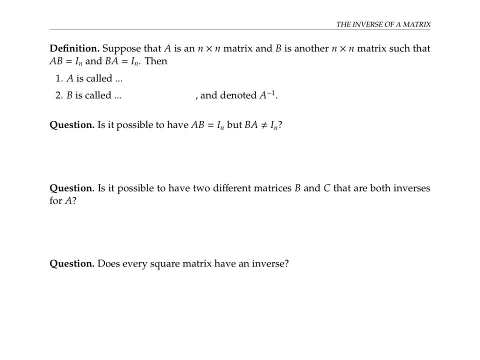 you get the identity matrix, Then A is called invertible And B is called the inverse of a. s can be denoted a to the negative one. we're focusing our attention on matrix A in this definition, But in this situation B is also called invertible and A is going to be the inverse of B. we'll only talk about. 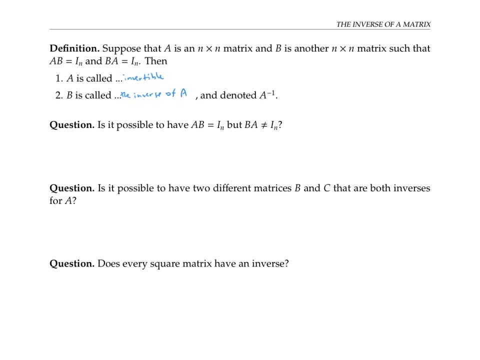 inverses for square matrices And in fact it turns out that it's not possible for pairs of matrices to satisfy both these two conditions if they're not square. You might be wondering: is it possible to have a times B be the identity matrix but not B times a? we've certainly 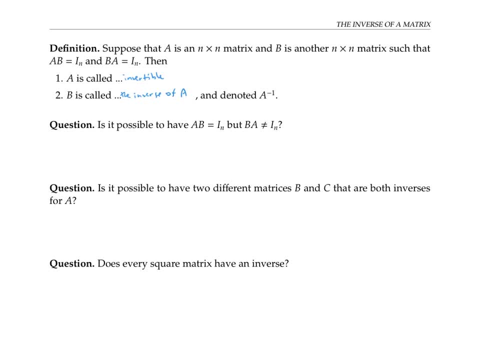 seen that in some cases the product a times B is not the same as the product B times a. matrix multiplication is not in general commutative, But it turns out- although I won't prove it here- that if a and B are square matrices such that a times B is the identity, then 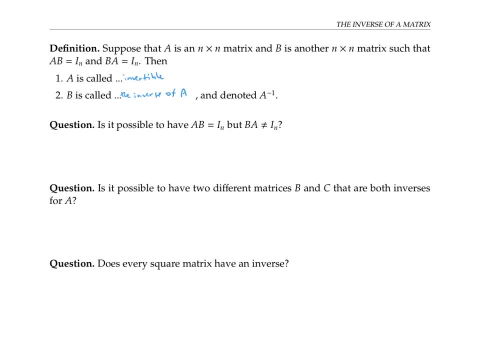 it B times a will also necessarily have to be the identity. So the answer is: is it possible to have the product one way be the identity, but not the other way? The answer is no. this is not possible. You might also wonder: is it possible to have two different matrices? 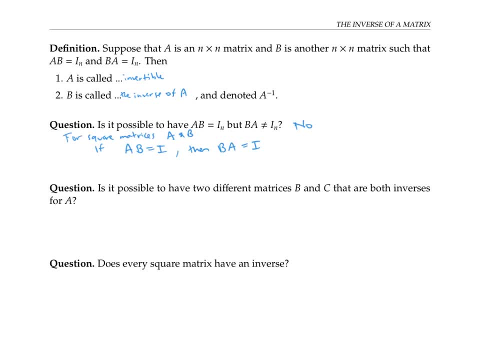 B and C that are both inverses for a. In other words, could we have a times B equals i, b times a equals i, and also have a times C equals i And C times a equals i? Well, suppose I were in this situation and I took the equation. 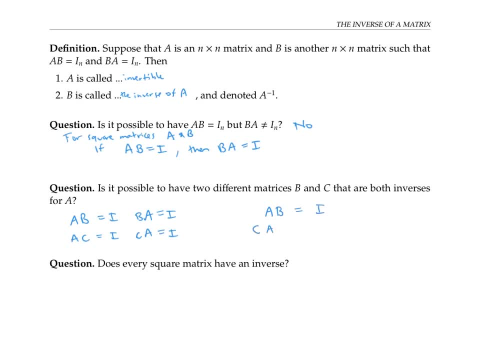 a times B equals i, and I multiplied on the left by C, Since C times a is the identity. this is the identity right here. So this can be. this equation can be rewritten as i times B equals C times i, but the identity times B is just B and C times. you didn't just see? 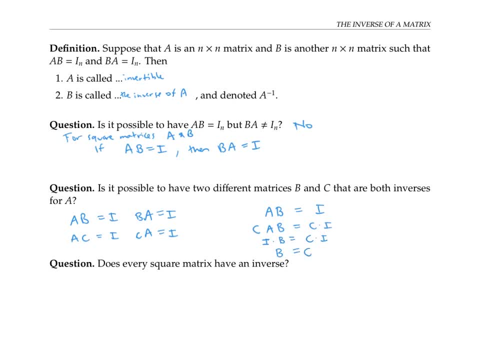 so in fact, B would have to equal C. So the answer is no. it's not possible to have two different matrices, B and C, that are both inverses for a. they would end up having to be the same thing. Another question that comes to mind is: does every square matrix have an? 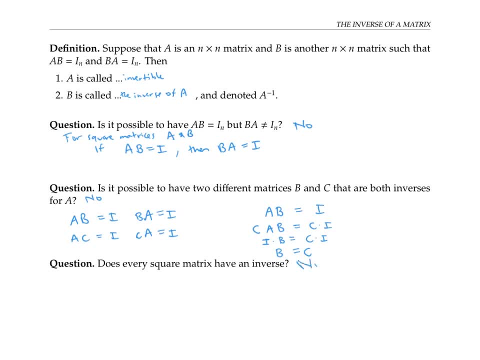 inverse? The answer to this question is also no. For example, let's consider the two by two square matrix 1224.. Suppose we found a matrix. I'll write it entries as A, B, C, D, so that when we multiply together we got the identity matrix. If I 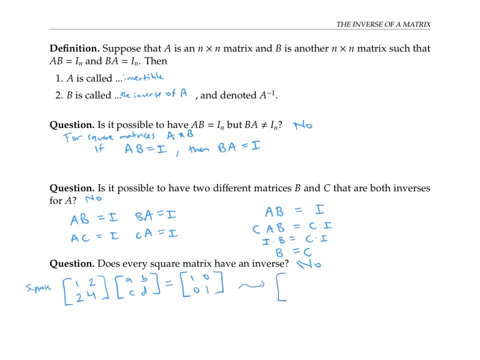 work out the matrix multiplication. I get these entries on the left having to equal the identity matrix on the right, But that means I need a plus two C to equal one and two a plus four C to equal zero. If I take twice the first equation and 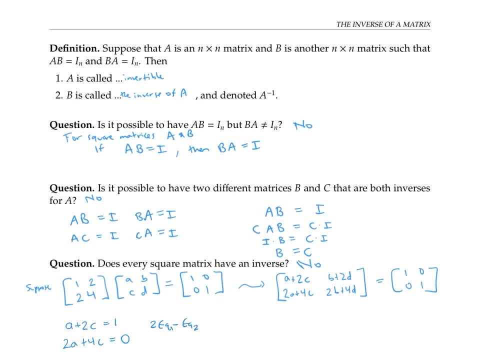 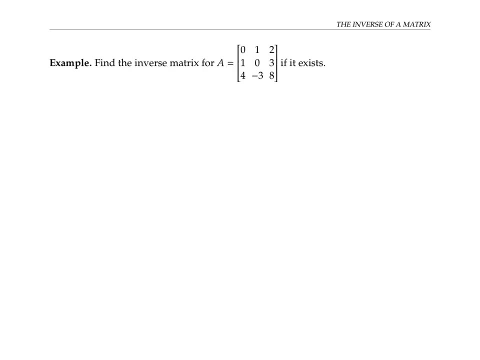 subtract the second equation, I get zero equals two, which is a contradiction. So there are no values of A, B, C and D that would work. There's no inverse to this matrix. If we want to find an inverse matrix for a matrix like this one, that's the same as finding 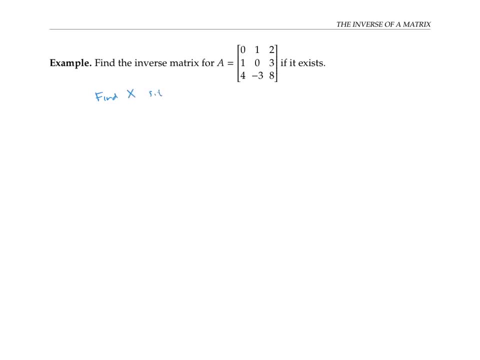 a matrix x, such that a times x is the identity matrix, in this case three by three identity matrix. That's all we have to do, Because we've seen that if the multiplication this way is the identity, then the multiplication in the other direction, x times a, has to also. 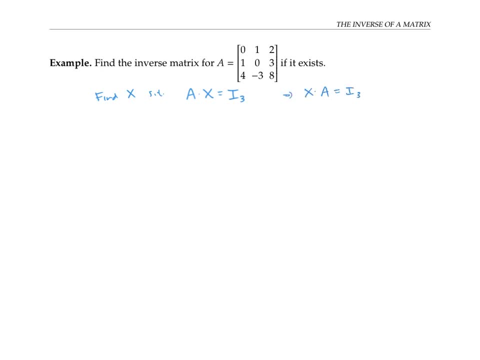 equal the identity. But we've seen how to solve matrix equations like this before. We can do that by writing down the matrix A and augmenting it with the matrix on the right side of the equation, In this case the identity matrix. If we're able to convert this matrix to reduce row echelon form and it works out that the 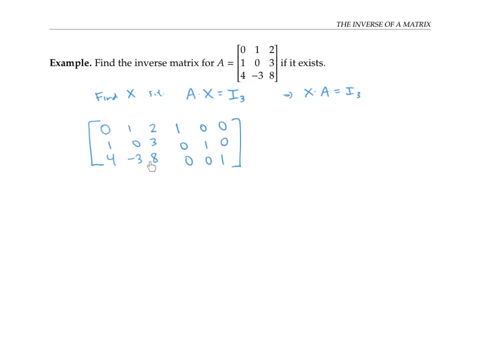 chunk in this part of the augmented matrix turns into the identity matrix, then we'll be able to read off the solution for x in this chunk of the matrix. So let's do some row reducing. I'll swap the first two rows. Use the first row to get rid of the four in. 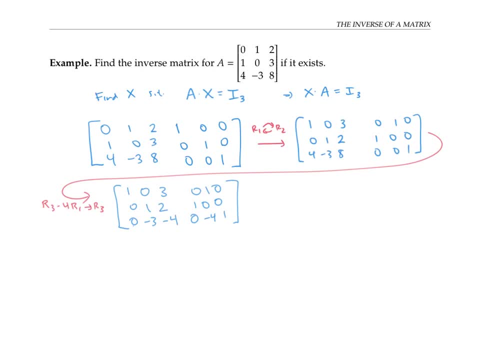 the third row. Get rid of the negative three in this matrix Position and continue. Notice that our row reduced matrix has the identity matrix as a block where the original matrix A used to be. Therefore, we have a solution x that we can read off from the rightmost block of our row reduced matrix. That solution is the inverse. 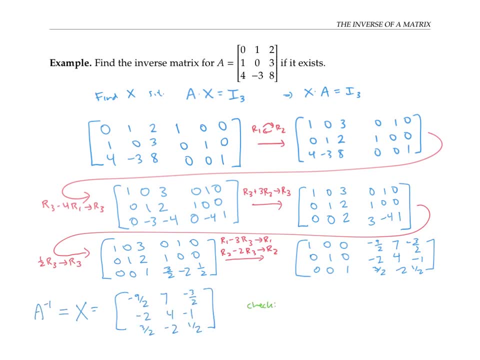 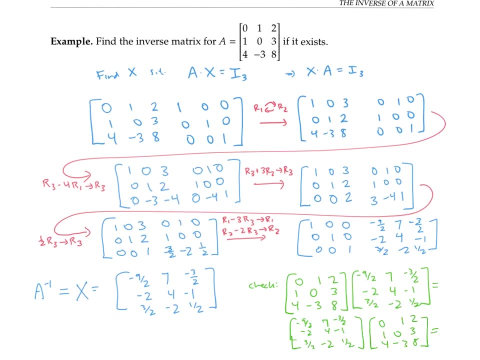 of a And we can check our work by multiplying this matrix by a in either direction and verifying that we get the identity matrix. I want to mention that if we had not gotten the identity matrix as our left hand chunk after doing row reducing, if we had, for example, 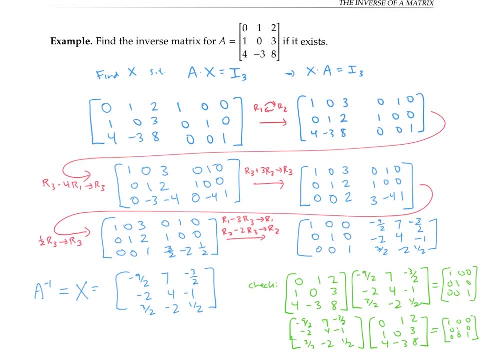 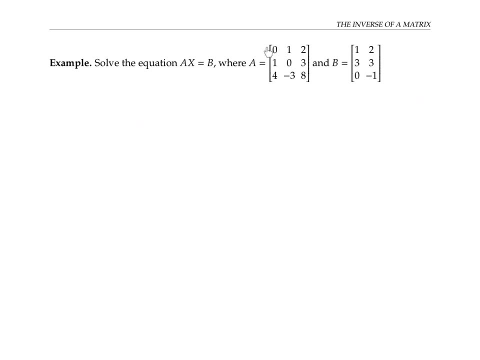 gotten a row of zeros here, then there would not exist an inverse to our matrix A. Now that we've found the inverse matrix- for a notice that this matrix A is the same matrix as was on this previous slide- Now that we've found its inverse, we have an easy way to. 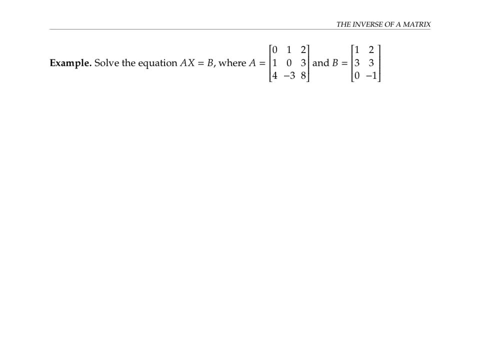 solve the equation a times x equals b. all we have to do is multiply both sides of that equation on the left by a inverse A. inverse times a is the identity matrix And the identity matrix times the matrix x just gives x. So the unknown matrix x will be given by a inverse times. 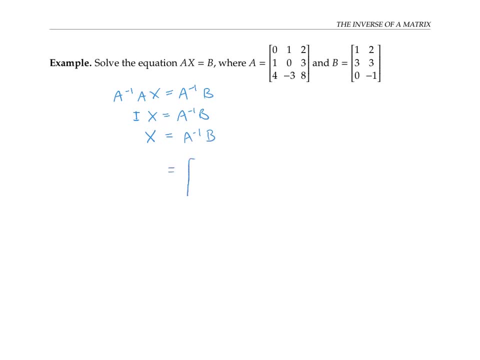 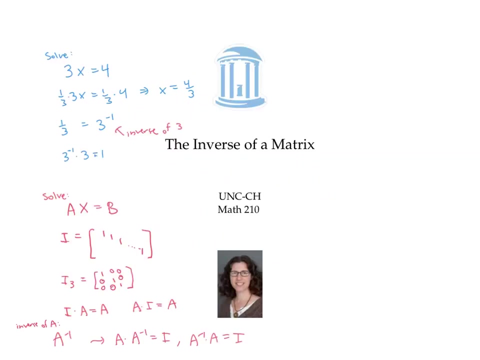 b. I'll copy a inverse from the previous page and multiply it by the matrix B. After some arithmetic this works out to the following three by two matrix: In this video we define the inverse of a square matrix as the matrix that you multiply it by to get the identity matrix. 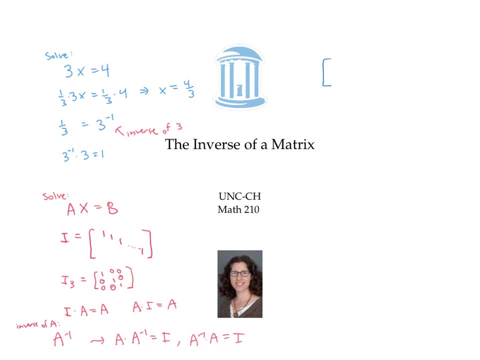 We also computed the inverse of a matrix by sticking the matrix and the identity matrix together And converting this to reduce row echelon form. Finally, once we had the inverse of a matrix A, we used it to solve an equation of the form ax equals B by multiplying both. 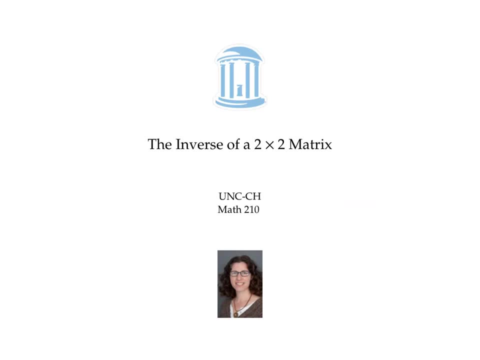 sides by a inverse. In this video we'll compute the inverse of a two by two matrix two different ways: First, by using row reduction and second, using a shortcut formula. As we saw in a previous video, one way to compute the inverse for a matrix is to augment that matrix with the 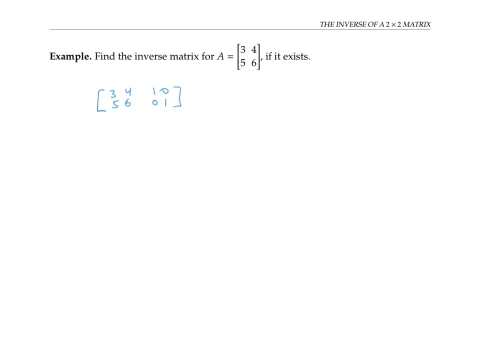 identity matrix and then convert it to reduce row echelon form. I'm going to do my row reduction by first multiplying the first row by one third, then getting rid of this five, then multiplying the bottom row by negative three halves And finally getting rid of this four. 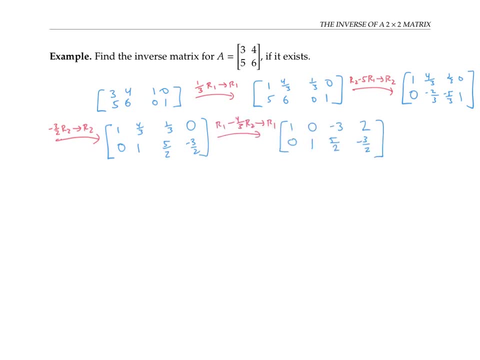 thirds, Since we are able to obtain the identity matrix as our left chunk, after row reduction, the inverse matrix- A inverse- exists and lies in the right chunk. This is our inverse matrix. Next, I'm going to give you a shortcut formula for finding the inverse of a two by two matrix. 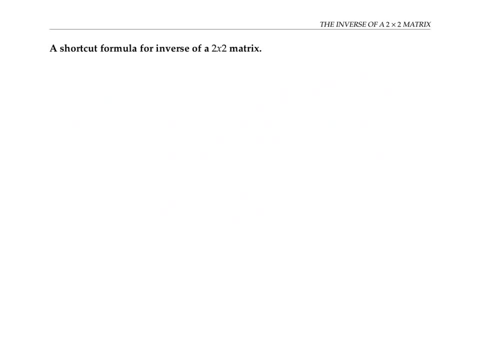 that'll get you the same answer with a little less work. In general, if your two by two matrix has entries- I'll call them little a, little b, little c, little d- then a inverse will be given by the matrix D, negative B, negative C, a multiplied by the scalar one. 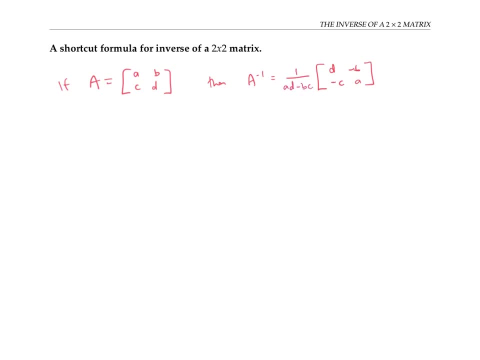 over ad minus BC. To help remember this formula, notice that the entries in this diagonal have been swapped. the entries in that diagonal have stayed the same but gotten negative signs in front of them, And the whole thing is multiplied by one over this crisscross. 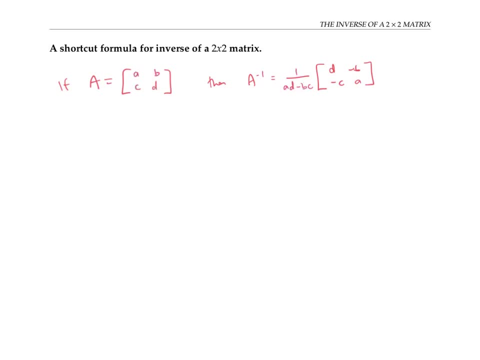 product: ad minus BC. This crisscross product is also known as the determinant of the two by two matrix. Now you might be wondering what if ad minus BC is zero? because then we'd be dividing by zero, And that seems like a bad idea. 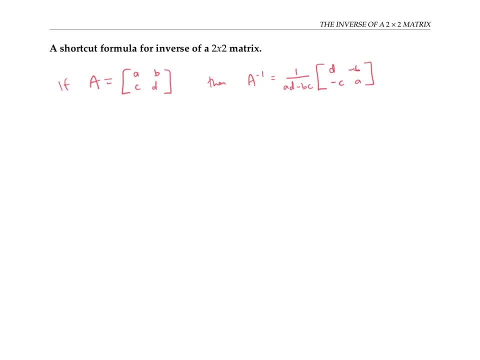 Well, that's a very good thing to point out, And in fact I should be a little more precise and say that if ad minus BC is not equal to zero, then a inverse exists and equals this matrix here, But if, on the other hand, ad minus BC is equal to zero, then it turns out. 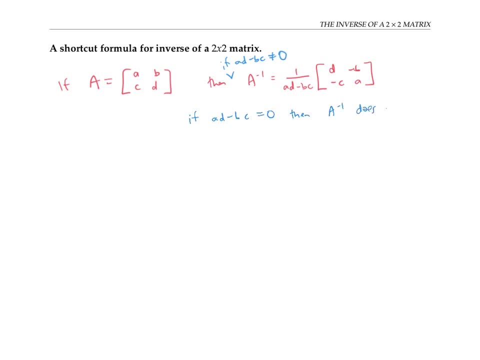 that a inverse does not exist. So let's see why this formula works. We could derive this formula by writing our abstract matrix A, augmenting it with the identity matrix and doing row reduction, But it'll be a little simpler. just to check that it works. 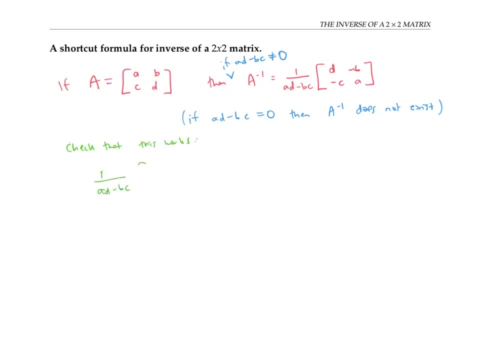 By multiplying our supposed inverse matrix by our abstract original matrix and making sure that we do in fact get the identity, carry down my scalar here. And then I'm going to multiply this row by this column to get AD minus BC This row. 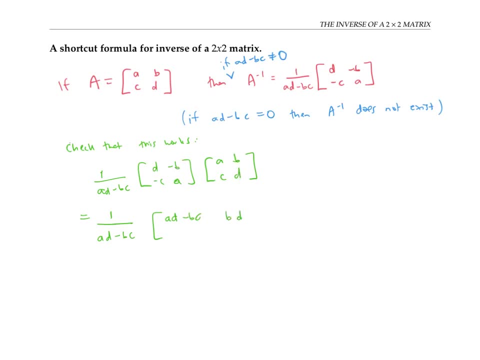 by that column to get BD minus BD, That row by this column to get minus AC plus ABischer's matrix. And then we get A C plus A, Cb, B, d minus. huh, right, an d, right, are we squared? 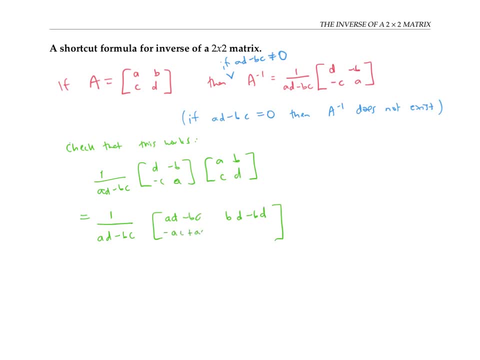 Sounds like a good idea. So we have two odd numbers and two equivalents, right an, d, right an, And then there are two dashes And since we're getting two color and this intense odd, quasi entertained, but AC and that row by that column to get minus BC, plus ad, we can see that this corner is. 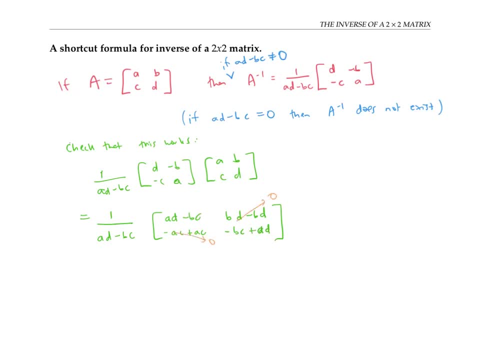 just zero, that corner entry zero. And when we divide these two entries by ad minus BC, we get ones, just like we want the identity matrix. So this matrix must indeed be the inverse of A. So let's go back to our original problem: finding the inverse for this two. 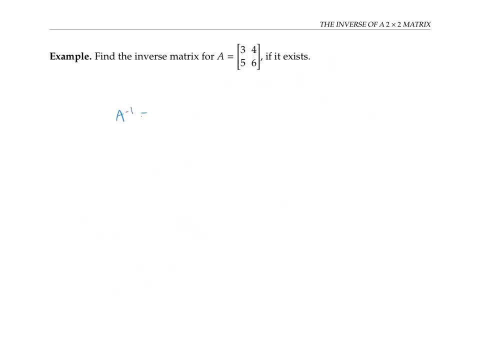 by two matrix. we know the inverse should be what we get when we switch the numbers on this diagonal and negate the numbers on this diagonal And multiply the whole thing by one over three times six minus six, Four times five. So a inverse is one over negative two times the matrix, If I bring. 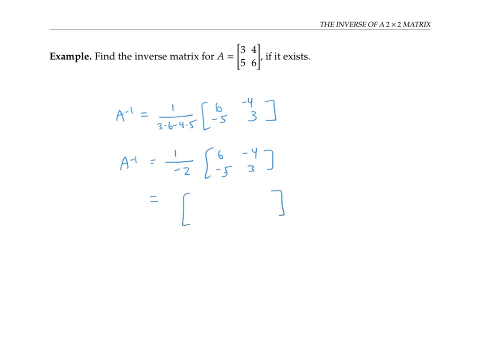 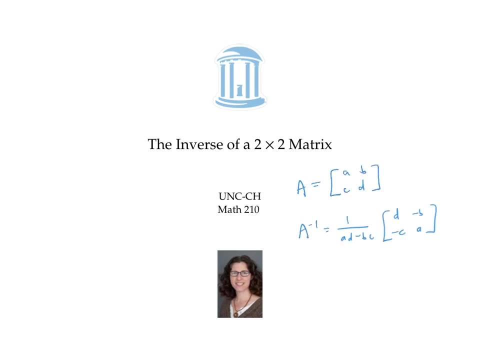 in the one over the negative one half. that gives me negative 325 halves and negative three halves. That's exactly what we got when we solve this problem before. This video gave us a handy shortcut formula For finding the inverse of a two by two matrix. This video gives a bunch of different ways. 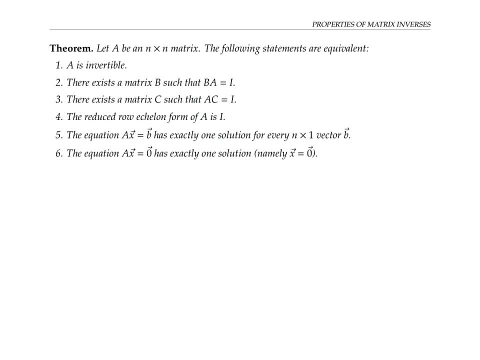 of saying that a matrix is invertible, Let a be an n by n matrix. We call that. we say that a is invertible By definition. that means that there exists an n by n matrix called x, such that a times x is the identity matrix. 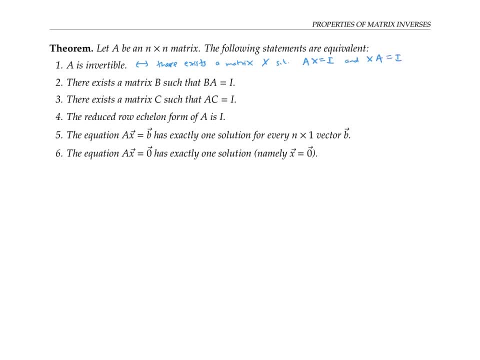 And x times a is the identity matrix. That's the definition of A being invertible. But there are five other properties that are equivalent to this. In other words, if any one of these properties holds about matrix A, then all the rest of them hold also, and if any one of these properties fails to hold, 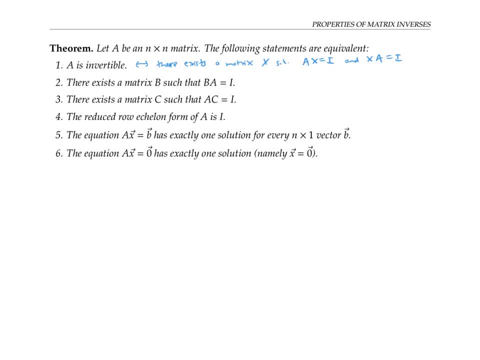 for a, then all the rest of them also fail to hold. I'll talk through these properties, But for a rigorous proof of why they're all equivalent you'll need to look at another video. Statement two says that there exists a matrix B such that B times A is I, So certainly if A is. 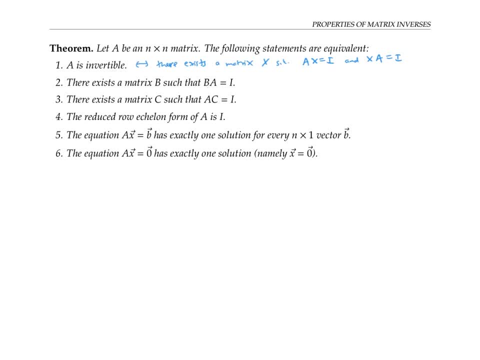 invertible. that's true, right, Because of A is invertible. there's a matrix that we can multiply on the left or the right and get I, and here we just need to multiply on the left to get I. but it turns out that having B times A equals I for square matrices also. 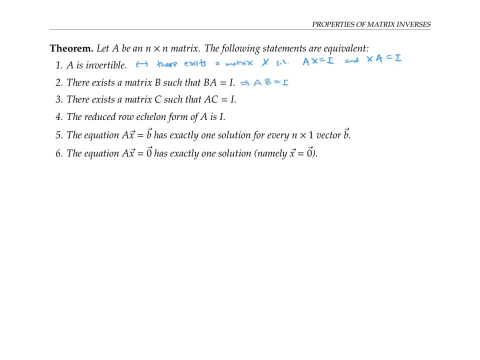 implies that A times B has to equal I, and so if statement two is true, then statement one is also true. Similarly, it turns out that if A times C is I, then C times A is I. So if statement three is true, then statement one is also true. And of course, going the 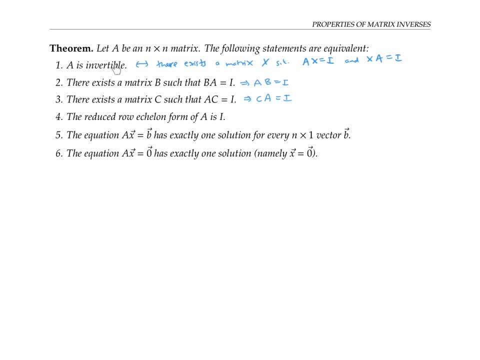 other direction. if one is true- A is invertible- then there certainly exists a matrix C. that's a right inverse. So statements two and three are both equivalent to statement one. Now let's look at statement four and see what that has to do with statement one. Suppose that A is invertible. 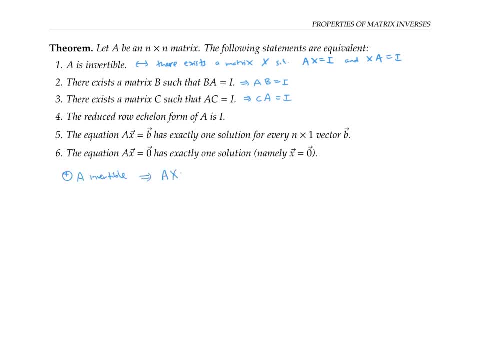 then there's a matrix x that solves the matrix equation. x A times x equals i, And solving this matrix equation is equivalent to taking the matrix a augmented by i and converting it to reduce row echelon form. When we do this, we're really just solving systems of linear equations, one system for each column of i. 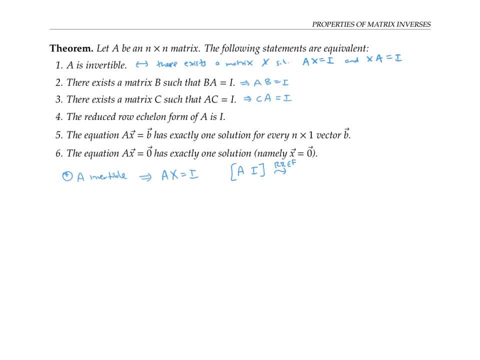 Well, since we know there's a solution, when we do the reduced row echelon form, we know we're going to have to get an eye where a used to be and then some other stuff where the eye used to be If we didn't get an identity matrix on the left hand chunk. it's going. 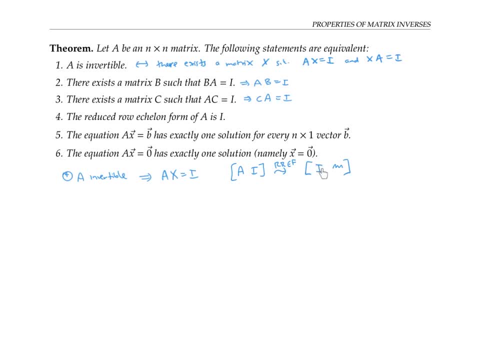 to be the identity matrix on the right hand side. If we got something else, with a row of zeros and some columns that didn't have leading ones in them, then we wouldn't have a unique solution here. we would either have no solution or infinitely many solutions. 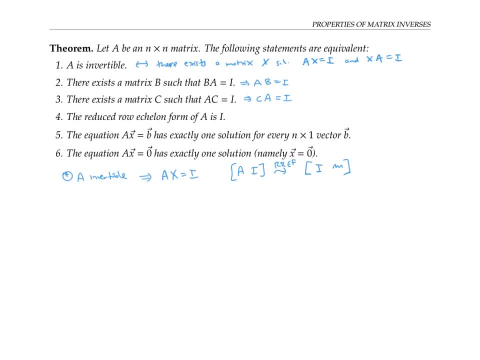 neither of which is possible if A is invertible. So therefore, A being invertible means that the reduced row echelon form of A has to be the identity matrix. And to go the other way: if the reduced row echelon form of A is the identity matrix, then that means that we can solve. 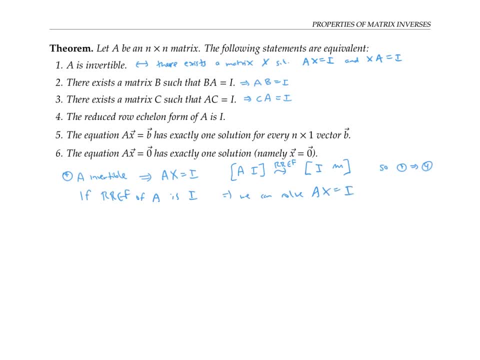 A times x equals i. we can just read off the solution from the right side after we do the reduced row echelon form, And so therefore, we're in a situation of three, which we said was equivalent to situation of one. Now, what about this fifth statement that the vector 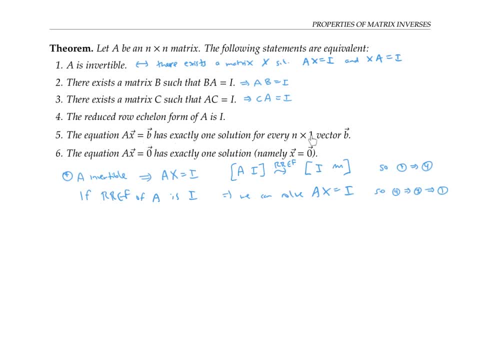 equation ax equals B has exactly one solution for every n by one vector B. Well, if A is invertible, then to solve the equation ax equals B, we just multiply both sides on the left by a inverse and we get that x is a inverse B. So there's definitely 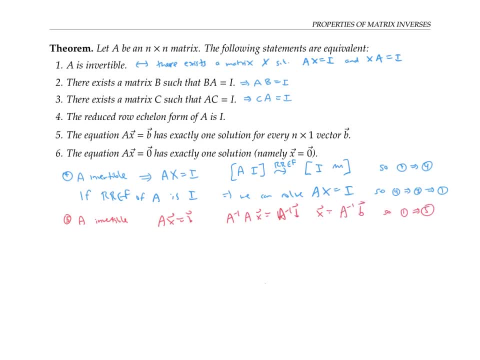 just one unique solution. On the other hand, going the other direction, if ax equals B always has a unique solution, Then when we row reduce any matrix like this, then we end up having a in identity form And we've seen from previous work that that's, that's four, that that implies one, So a being. 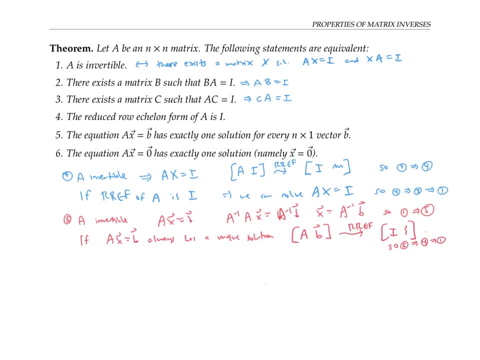 invertible is also equivalent to statement five. Finally, let's consider statement six. Statement six says the equation a times x equals zero has exactly one solution. That solution is necessarily going to be the zero vector, since any matrix times a zero vector is a zero vector. Well, the argument that this is equivalent to a being invertible is: 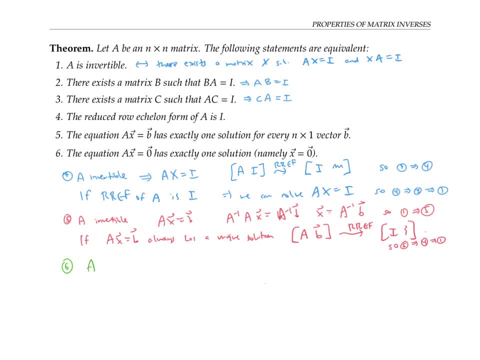 pretty much like the last one. If a is invertible, then the equation ax equals the zero vector can be solved by x. Well, if a is invertible, then the equation ax equals zero has a unique solution. And if a x equals zero has a unique solution, then a similar argument says that a has to. 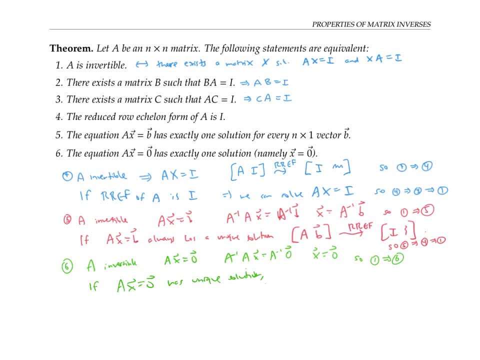 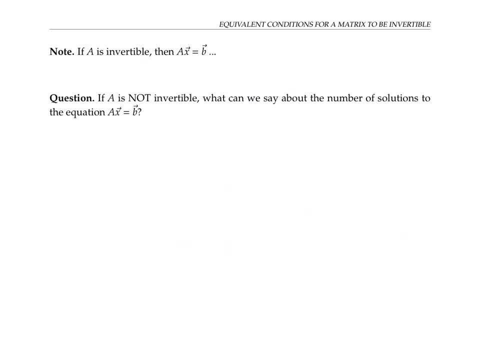 be reduced to the form of an identity matrix and therefore a is invertible. So all of these conditions are equivalent. We've seen that if a is invertible, then a- x equals b- has a unique solution for any vector b. But what about if a is not invertible? What can we say about the number of solutions? 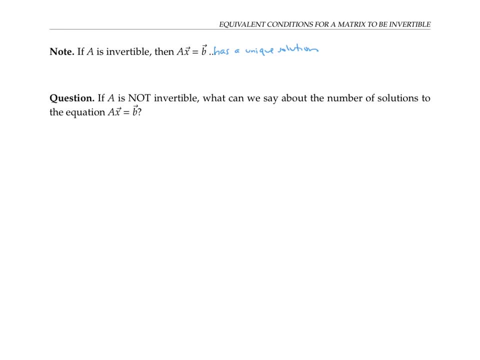 to the equation ax equals b in that case. Well, we know for sure that this equation does not have one unique solution, Since if it did, the same sort of argument we used before would say that a would be reduced to the identity matrix. So if a is invertible, then a is invertible. 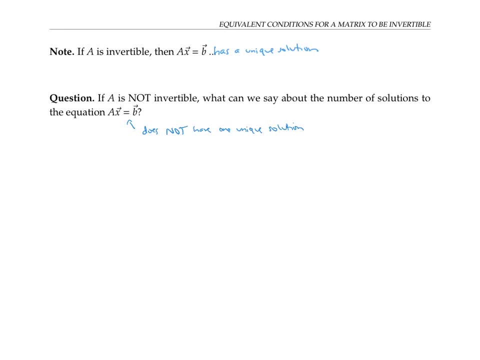 Well, we know for sure that this equation does not have one unique solution, Since if it did, the same sort of argument we used before would say that a is invertible. So if a is invertible, then a is invertible. So this equation cannot have one unique solution. 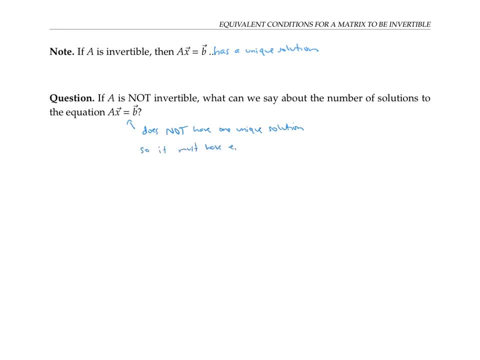 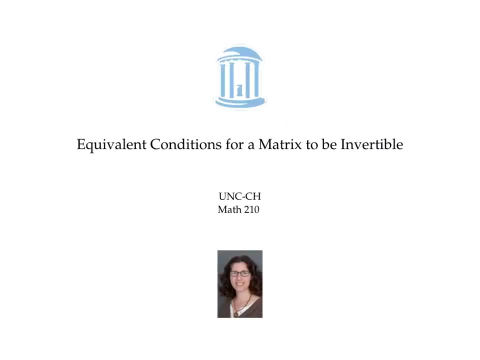 So it must have either no solutions or infinitely many. That's because they're only these three possible options: One unique solution, no solutions or infinitely many solutions whenever we have a system of linear equations, as this vector equation represents. In this video, we saw a bunch of different but equivalent ways of saying that a matrix 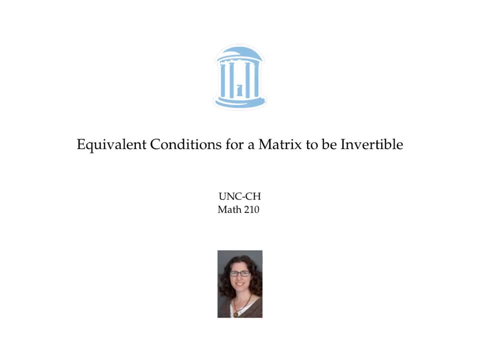 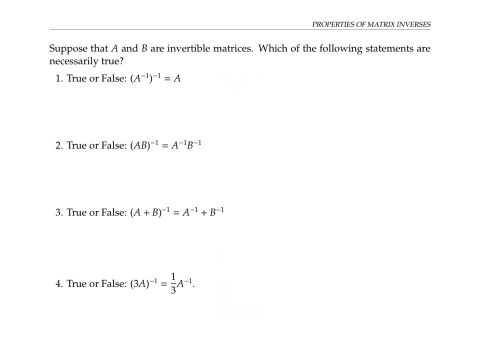 is invertible. A key idea was that invertible matrices were reduced to look like the identity matrix. This video gives some properties of matrix inverses. Suppose that A and B are invertible matrices. I've written down four different properties here And for each of, 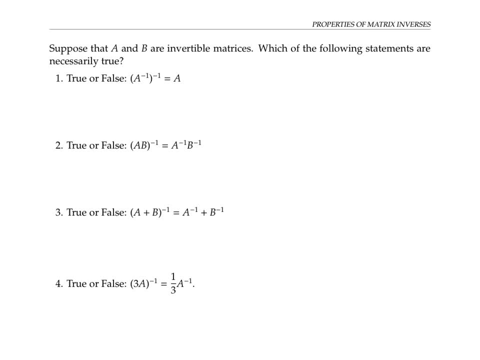 these properties. see if you can figure out if it's necessarily true, no matter what invertible matrices A and B are. You may want to try some examples. Like you could pick a couple simple two by two invertible matrices and test these out. Let's start with statement one. Is it true? 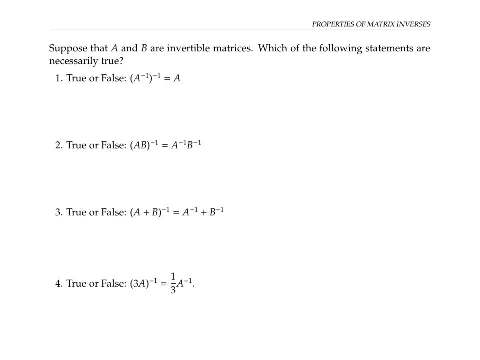 that the inverse of A inverse is A. Well, yeah, that's definitely true, Because A inverse inverse is the matrix You multiply by A inverse to get the identity matrix, But a is also the matrix that you multiply by A inverse to get I. And since inverses are unique, A. 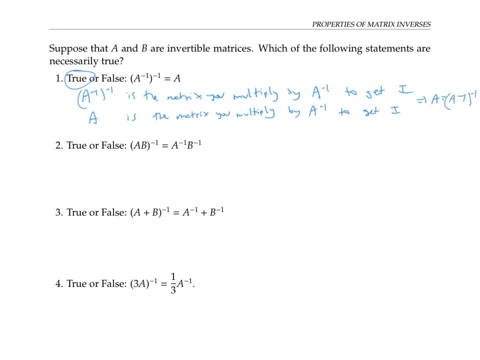 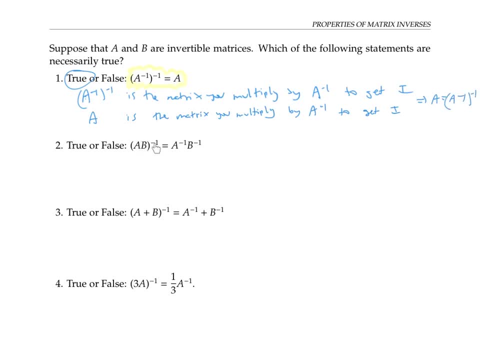 that the if you multiply two matrices together and take the inverse of that, you get the same thing as if you take a inverse and multiply by B inverse. Let's try it out on an example. I'm going to set a equal to the matrix 1327 and B equal to the matrix 23, negative one. 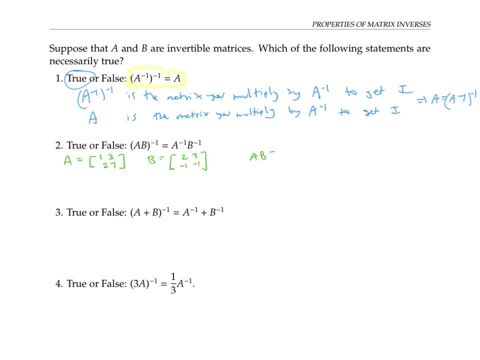 negative one. then you can check that a B is the matrix negative one, zero negative, three negative one. And a B inverse is the matrix negative one, zero, three negative one. Remember there's a shortcut formula that makes it easy to calculate the inverse. 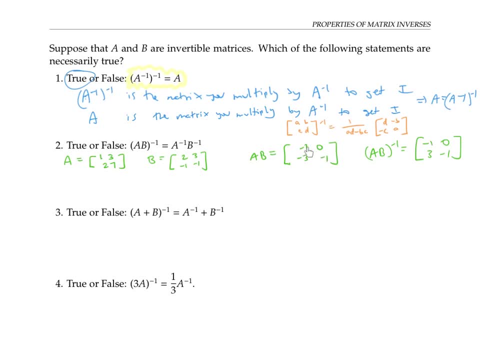 of a two by two matrix. we just swap the entries in these two positions- which doesn't do anything in this case, because the 12 entries are the same- And we negate the entries in these two positions And then we multiply the whole thing by the scalar, that's one over the determinant, which is just this crisscross. 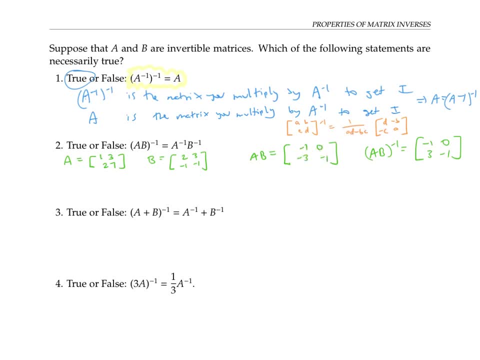 product, this times this minus, this times this, And in this case that determinant is just one. So now let's calculate a inverse Again. the determinant of this example is one, And so I can just swap the seven and the eight, the three and the two. that's my a inverse, And B inverse ends up being 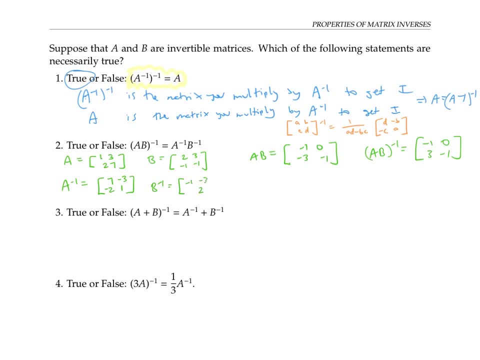 negative one here to here, negative three here and a one here. Once again, the determinant is one. So finally, a inverse, B inverse multiplies out to negative 10, negative 2738, which is not the same as quantity. a B inverse. So this statement is false. We've broken it with our 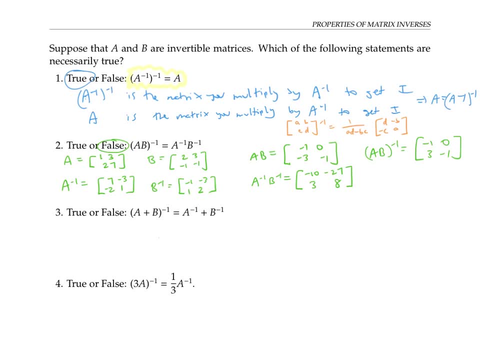 first example. However, there is a related statement. that's true If we do, instead of a inverse, B inverse, we calculate B inverse, a inverse That does give us negative, 103 negative one, just like when we did a B quantity inverse. 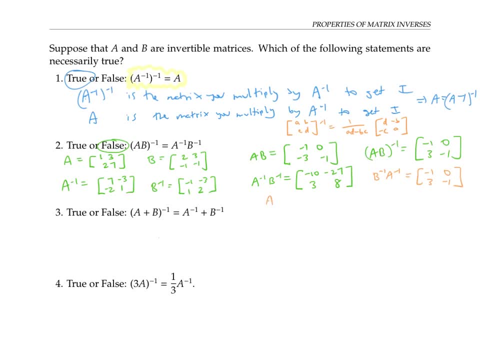 So we have at least one example in which a- B quantity inverse is the same thing as B inverse. a inverse- And in fact this statement is always true- A- B inverse is the matrix that you have to multiply by a- B to get the identity matrix. But if you multiply B inverse, 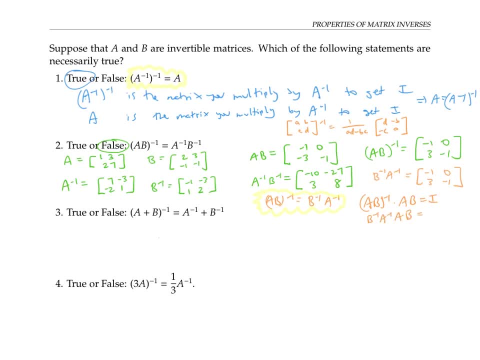 a inverse by a B. the a inverse a becomes the identity A, B becomes the identity A B. Then you multiply the A inverse a inverse by a B. Then you multiply matrix: the IB becomes the matrix B And the B inverse B collapses to the identity matrix. 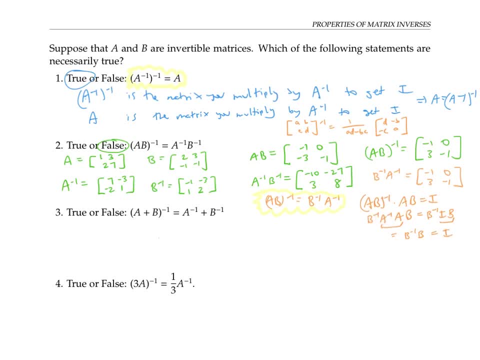 So since B inverse, A inverse times, AB is the identity matrix, B inverse- A inverse must be the same thing as AB quantity inverse. We're using the fact there that inverses are unique. What about this next statement: Is it true that A plus B inverse is equal to? 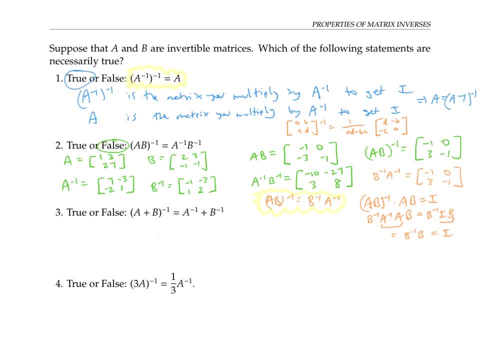 A- inverse plus B- inverse. Again, we can try it out with an example. Let's use the same matrices, A and B. If we compute A plus B by adding together the entries, we get 3616. And if we compute the inverse, 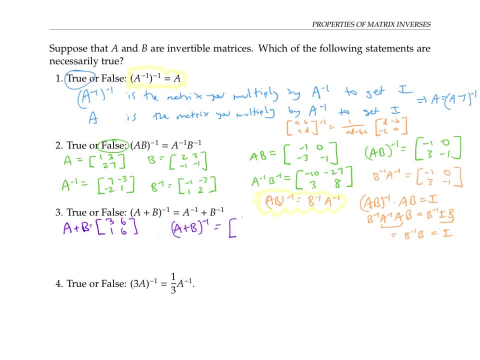 of that, we end up with a matrix- one half negative, one half negative- 112, one fourth, which I encourage you to check. If instead we add together A inverse plus B inverse, which we calculated up here, then we get an answer of six minus six minus 13,, which is: 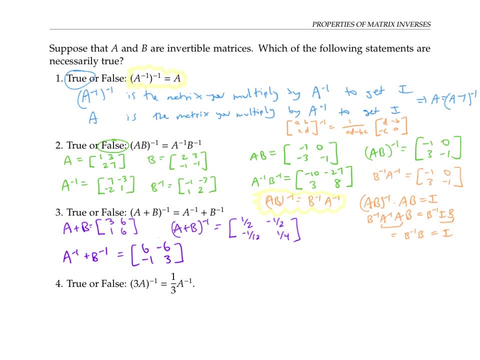 not the same thing as A plus B inverse. In this case, it wouldn't help to switch the order. B inverse plus A inverse is the same thing as A inverse plus B inverse, since matrix addition is commutative. In fact there's. 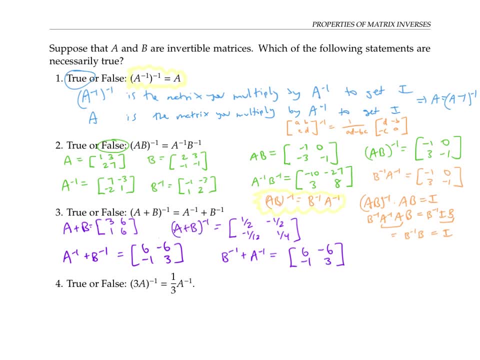 no relationship between A plus B inverse and the inverse of A and the inverse of B. In fact, it's possible for A and B to both be invertible, but A plus B to not be invertible. Finally, let's look at the last true false. 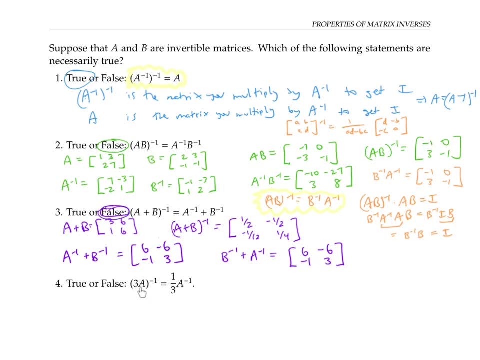 Is it true that the inverse of three times a matrix A is the same thing as one third times the inverse of A? Well, in our example, three A is the matrix 39621.. You can check that three A inverted is the matrix seven thirds minus one. minus two thirds, one third. 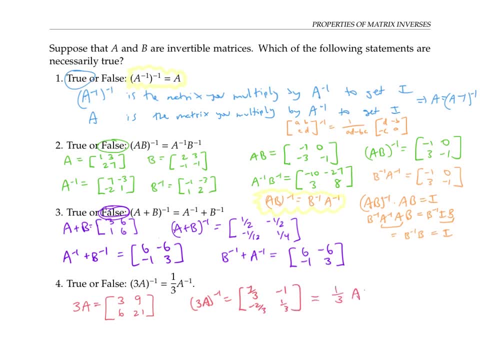 But that's exactly one third times the A inverse matrix that we calculated earlier. So this statement is true for that particular example of A, But in fact it's true for any invertible matrix A and any scalar, not just the number three. 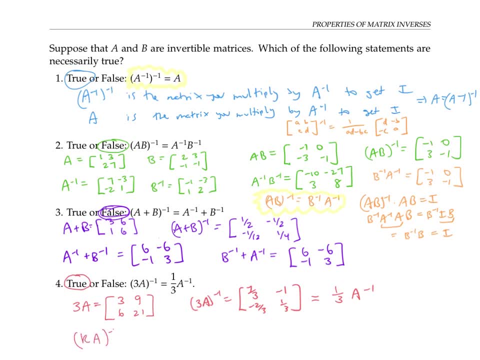 So in general k times A inverse is equal to one over k a inverse for any invertible matrix, A and scalar k- that's not zero- makes sense that this is true because if you take one over k a inverse and multiply it by k a, then pulling out the k you get one over k. 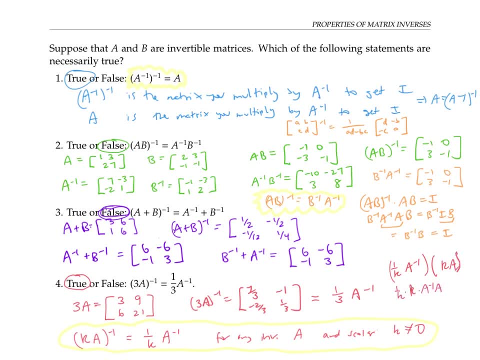 times k times a, inverse times a. well, that's definitely, the identity is one times the identity matrix or the identity matrix. And since we've multiplied two thirds, we get one over k times k times a inverse times a. So if we've put those things together and gotten the identity matrix, the two things, 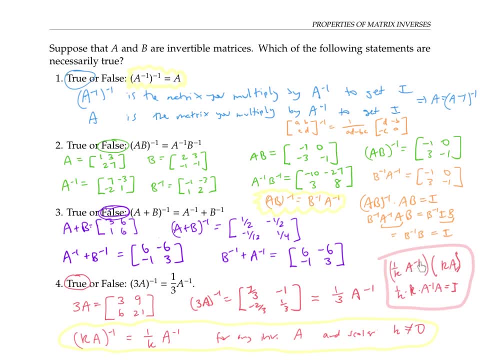 have to be the inverse matrices of each other, So one over k a inverse must be the inverse matrix for k times a. To summarize: if A is invertible, then A inverse is also invertible and its inverse is A. Also, if A and B are invertible, then A times B is invertible and its inverse is B inverse. 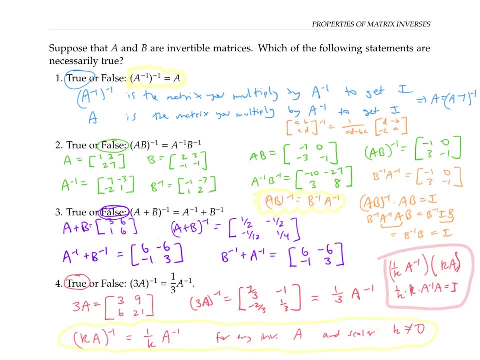 times A inverse. And finally, if A is invertible, then k times a is invertible for any nonzero scalar k and its inverse is one over k times a inverse. There's one more property of inverse matrices that I want to talk about. 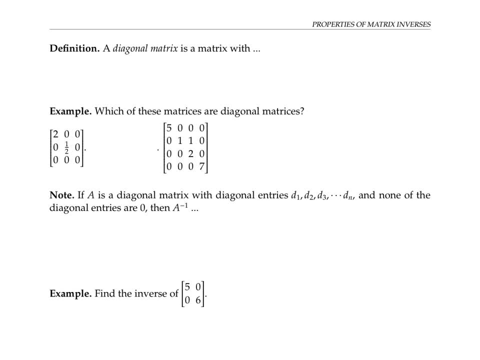 And that's the inverse of a diagonal matrix. A diagonal matrix is a square matrix with numbers on the diagonal which could be zero or nonzero, and zeros in all the other positions. By the diagonal I mean the diagonal that runs from the top left corner to the bottom. 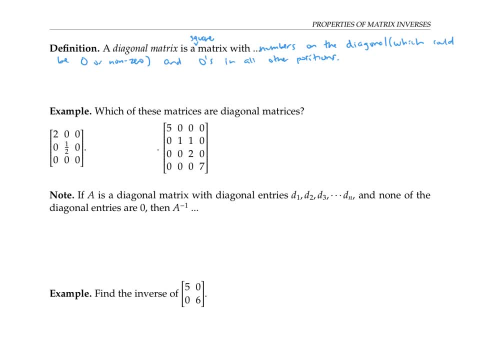 right corner. So which of these two matrices are diagonal matrices? Well, the first one is diagonal, But the second one is not. The first one is diagonal because all the entries that aren't on the diagonal are zeros. it's fine that we have a zero on the diagonal and some numbers that aren't zero on the diagonal. 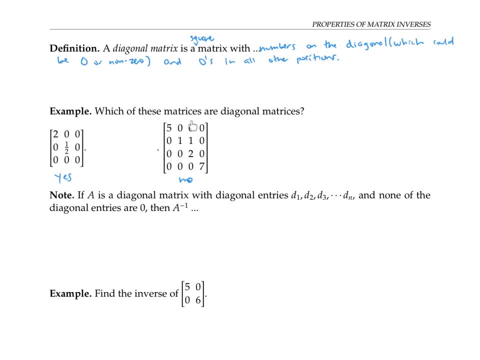 The second matrix is not diagonal because, even though it has zeros most of the places off the diagonal, it still has a one here. So if A is a diagonal matrix with diagonal entries given by the numbers d1,, d2,, d3, through. 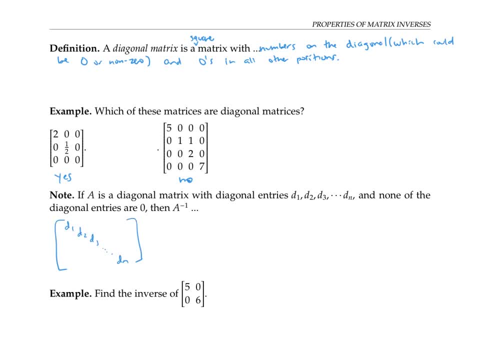 dn and none of these diagonal entries are zeros. I'll put big zeros here to indicate that all the other entries are zeros. then A inverse is also a diagonal matrix. Okay, Okay, Okay, With diagonal entries, one over d1, one over d2, and so on through. one over dn. 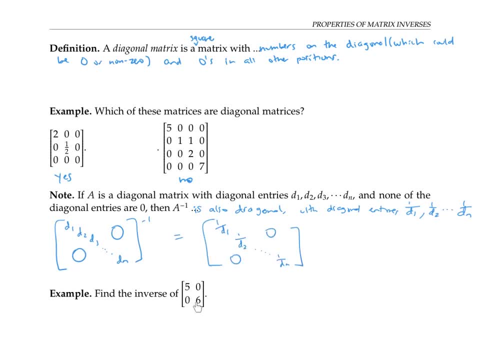 So, for example, if we want to find the inverse of this matrix, with five and six on the diagonal and zeros elsewhere, then we can write it down pretty quickly as one, fifth, 001, sixth. It's not hard to convince yourself that this formula for the inverse of a diagonal matrix 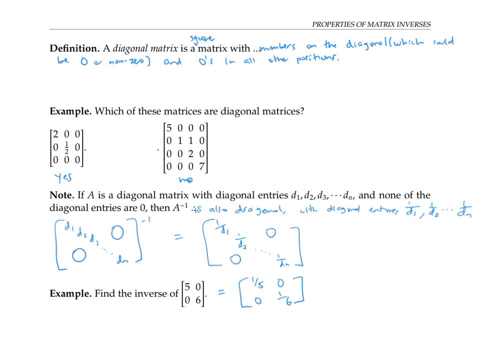 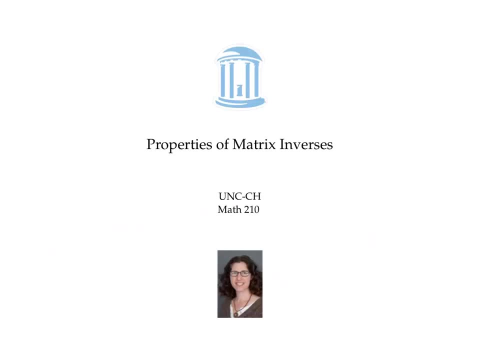 is true. Just take this matrix and multiply it by your original matrix and check that you get the identity. This video showed us how to find the inverses of matrices from the inverses of related matrices. For example, the inverse of a product is the product of the inverses, but in the backwards. 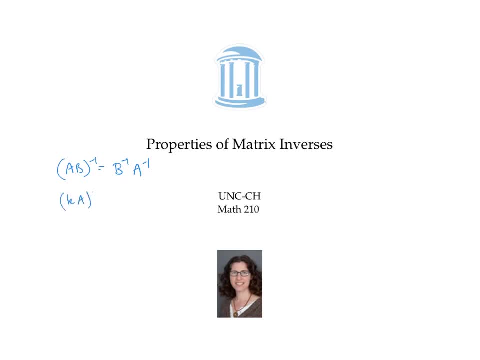 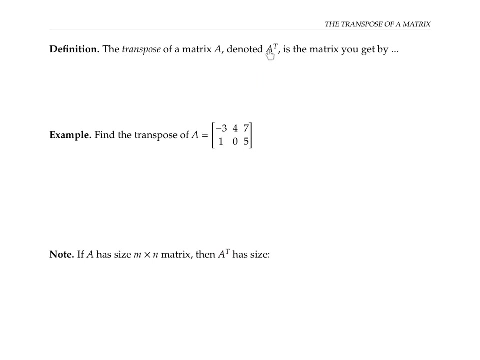 direction And the inverse of a scalar multiple of a matrix is the reciprocal of the scalar times, the inverse of the matrix. This video is about the transpose of a matrix. The transpose of a matrix: a, denoted by a with a little T superscript, is a matrix you get. 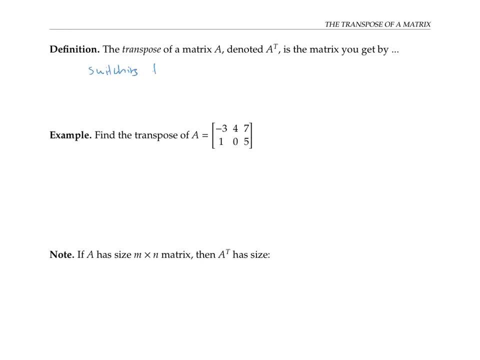 by switching the rows and the columns of a. In other words, the first row of a becomes the first column Of a transpose And the second row of a becomes the second column of a transpose. In this example, notice that we started with a two by three matrix. 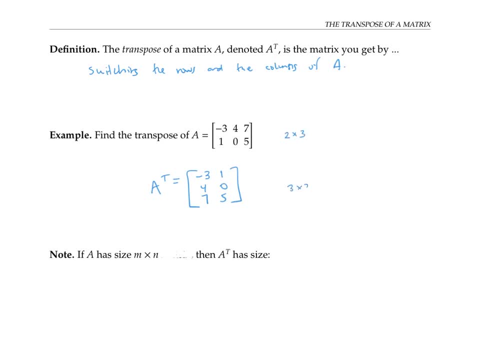 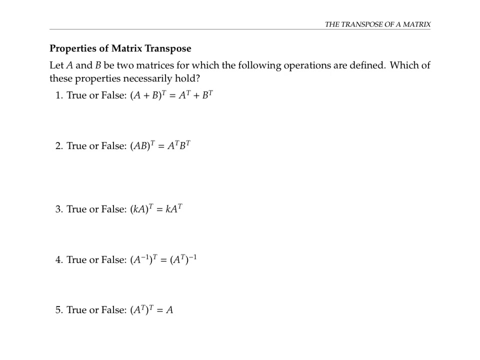 But when we took the transpose we got a three by two matrix And in general if a has size m by n, then a transpose has size n by m. Let's work out some properties of matrix transpose. Let's let A and B be two matrices for which the following operations are defined: 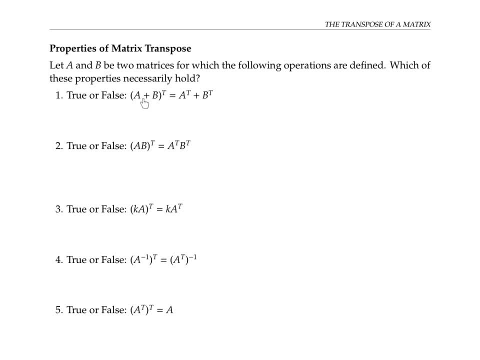 So for property one we need addition to be defined, so we're going to need A and B to be the same size, And for property B we need a times B to be defined, So we need the number of columns of a to be the same as the number of rows of b For property. 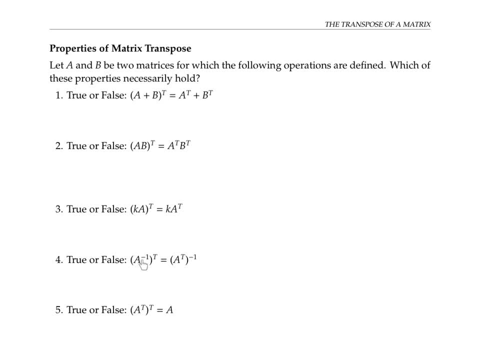 four, we need a to be a square matrix so that we can take its inverse. Please pause the video and try your hand at figuring out which of these five properties holds. you might want to write down some example matrices for A and B and test the property out. I hope you. 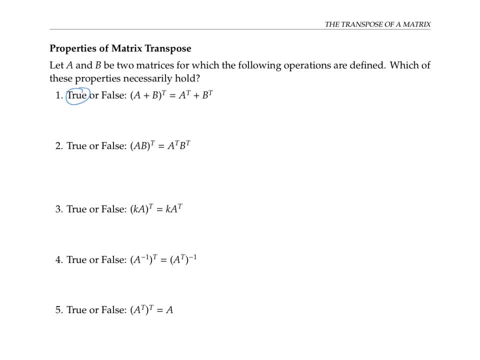 found that the first property is true. If we take two matrices and add them up and then take the transpose, for example, these two matrices, we can think of that as adding them together row by row and then switching the rows to columns, But we'll get the same. 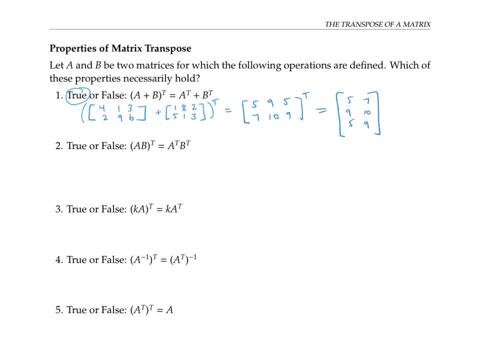 thing: if we first switch the rows to columns and then add them up column by column, What about the next property? Is a B quantity transpose? the same as A transpose times B transpose? Well, thinking about dimension, just because A times B makes sense, dimension wise we're. 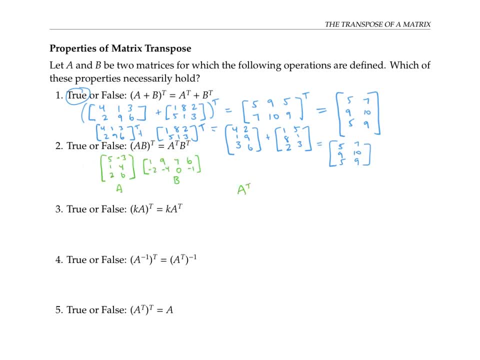 going to have A transpose times B transpose. It doesn't guarantee that a transpose times B transpose will even make sense Here. it doesn't because we can't multiply a two by three matrix times a four by two matrix, And even if we stick with square matrices. so 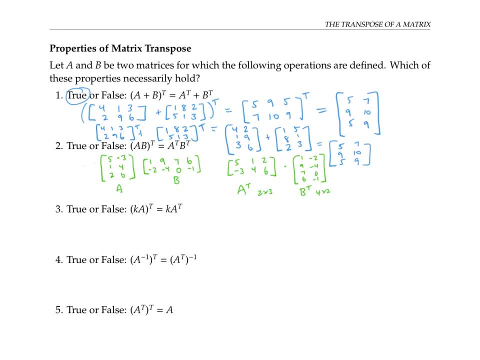 dimensions, not a problem. It's still easy to come up with examples where a, B transpose is not the same thing as B transpose, A transpose times B transpose. For example, we can take a to be the matrix 2317.. And B to be the matrix 234 negative one. then a- B works out to be the matrix 16 330 negative. 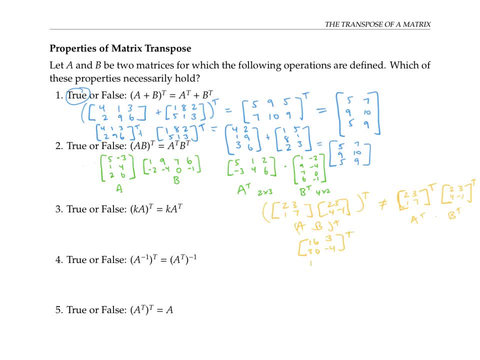 four, And when we transpose that we get 1633 negative four. But if, on the other hand, we transpose a first and also transpose B and then multiply those transposes together, you can check that we get the matrix 777, 27, five, which has nothing. 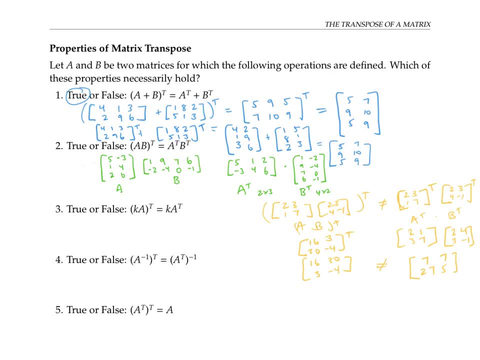 in common with a, B quantity transpose. So this statement as written is definitely false. But there actually is a relationship between transpose and multiplication, Like with inverses if we take the product backwards. so here we do a, B transpose, but on the other side we do B transpose first. 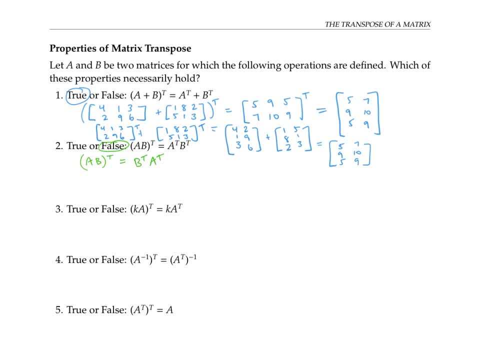 and then a transpose. this does turn out to be true. First of all, we can check that the dimensions will work out. If a is, for example, an M by k matrix and B is a k by n matrix, so that a times B makes sense, then B transpose will be an n by k matrix and a transpose will. 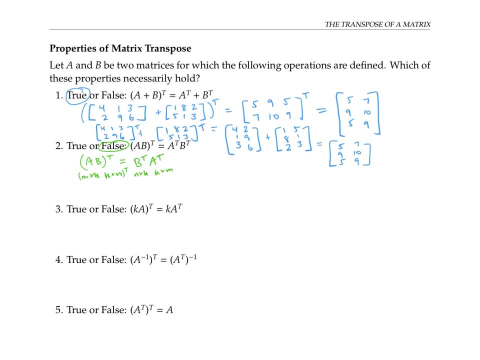 be a k by m matrix, So that multiplication will also make sense And the resulting matrices on either side will be n by m matrices. On this side we get n by m because when we do the multiplication we get m by n, but then when we take the transpose, that switches. 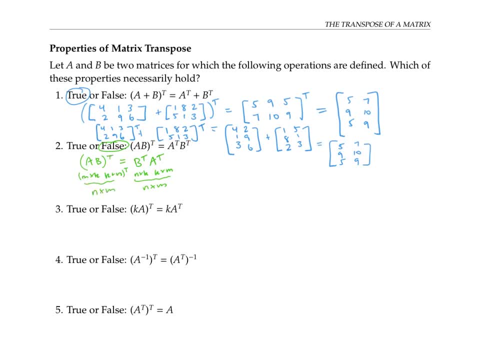 that to n by m. But it's not just that the dimensions work out. These two matrices are actually equal for any matrices- A and B. Let's see how this works In an example. let's say that A is this three by two matrix. 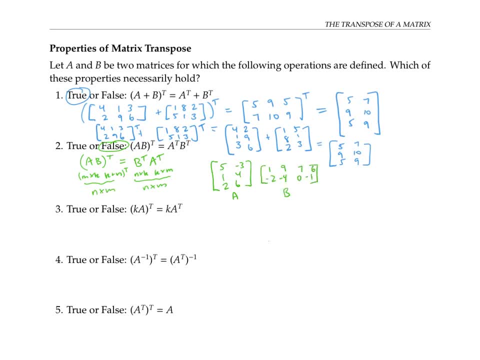 and B is this two by four matrix. then if we want to multiply B transpose times a transpose, the entries of the resulting product matrix will come with from rows of B transpose multiplied by columns of a transpose, For example, the entry in the two, three position of the product. 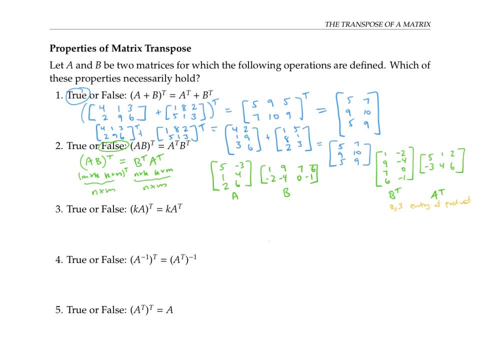 that is the second row. third column of the product will come from multiplying the second row of B transpose with the third column of a transpose. But that's the exact same thing as multiplying the second column of B by the third row of A. So that'll be the three to. 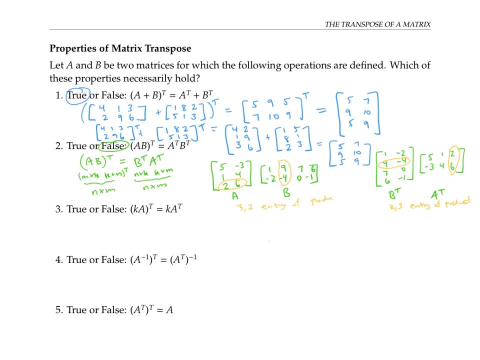 entry of the product a times B, And in general the i- j entry of a times B is equal to the j- i entry of B transpose, a transpose. But that means that the roles of rows and columns is exactly switched between these two matrices. 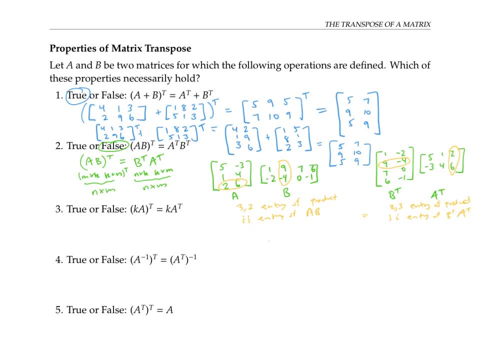 And therefore B transpose. a transpose is going to be the transpose of a- B. So this statement here is a true statement for all matrices, a, B, for which it makes sense. What about this next statement? the transpose of a scalar k times a is the same thing as. 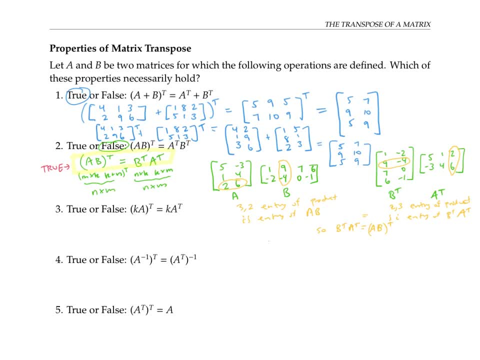 a scalar k times a transpose. it's not too hard to convince yourself that this is true with an example. if we multiply five by the entries of a matrix and then switch the roles of the rows and columns, that's going to be the same thing as switching the roles of the. 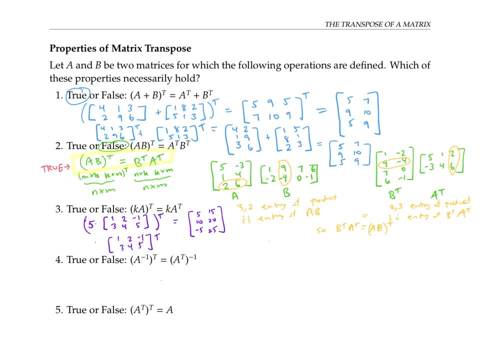 rows and the columns, And then multiplying that by five. What about this next statement? what about this next property? Is it true that a inverse transpose is the same thing as a transpose inverse? It may surprise you that this is true, at least for our square. 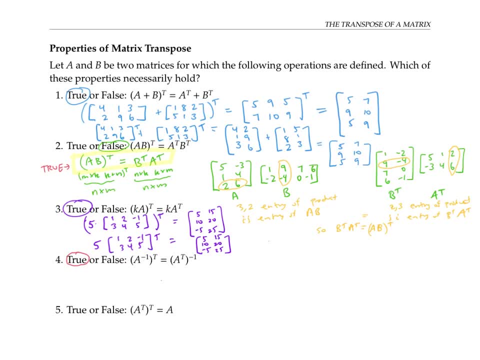 matrices, so that taking the inverse makes sense. One way to show that this is always true is to look at the product, a inverse transpose by a transpose. If we can show that this product is the identity, that will know that a inverse transpose is the inverse of a transpose, which. 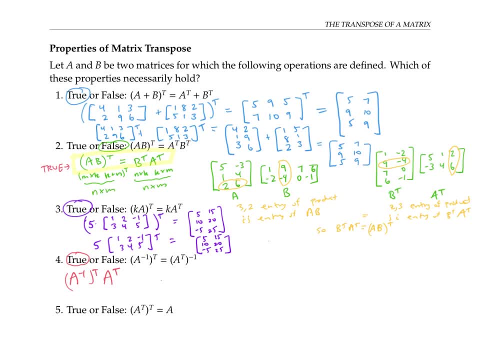 is what we're trying to find on here. So we're going to copy this product And this is going trying to show. But when we take a product of two transposes, we saw from this true property. the product of two transposes is just the transpose of the product in the other direction. 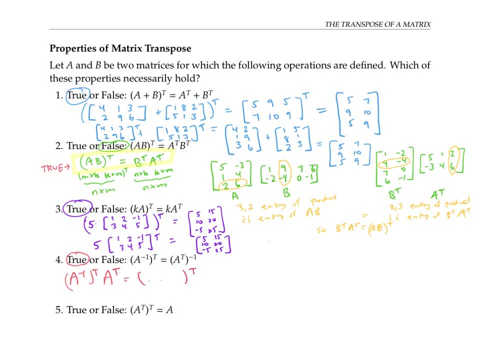 So this is the transpose of the product in the other direction. Hey, a times a inverse is just the identity matrix And we take the identity matrix as transpose and switch the rows and columns, we just get the same thing as the identity matrix And therefore a inverse. 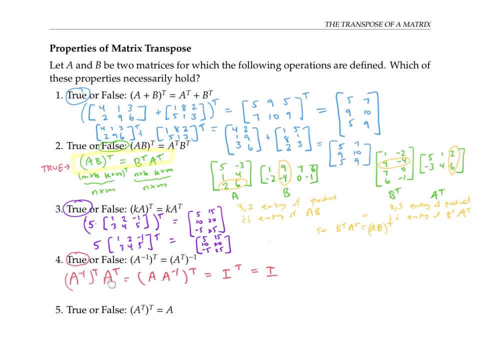 transpose is indeed the inverse of a transpose, like we wanted. Finally, is this last property true or false? Is a transpose? transpose the same thing as a? I hope you're thinking that it's true. It's true Because if we switch the rows and the columns and then switch, 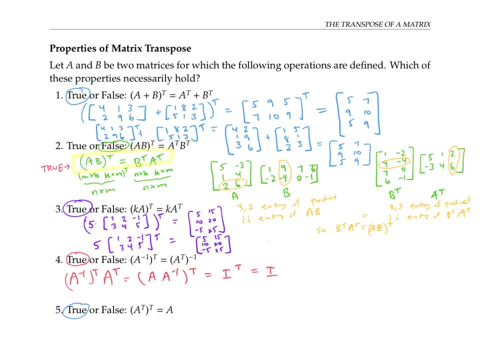 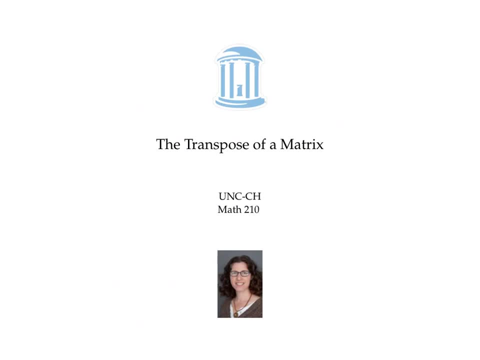 the rows and the columns. again, we get back to the same thing. In this video we defined the transpose of a matrix and looked at how transpose interacts with other matrix operations like multiplication, addition and inverses. This video is about. 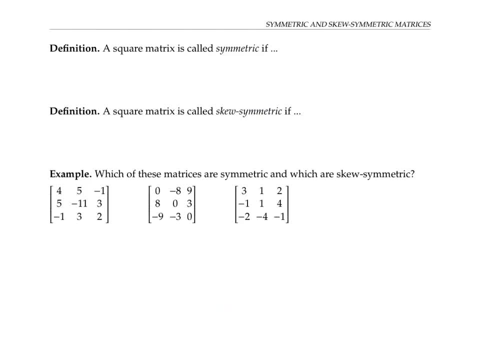 symmetric and skew symmetric matrices. A square matrix, let's call it a, is called symmetric If a transpose is the same thing as a and a square matrix, a, is called skew symmetric If a transpose is the negative of a, that is, its entries are. 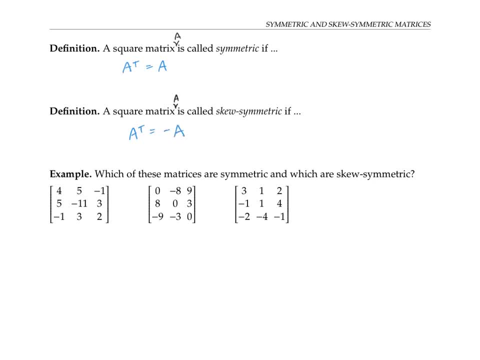 the same as A's entries with negative signs in front of them all. So which of these three matrices are symmetric and which are skew symmetric? If I take the transpose of the first one, I get this matrix And we can see that that's the same as the original matrix. 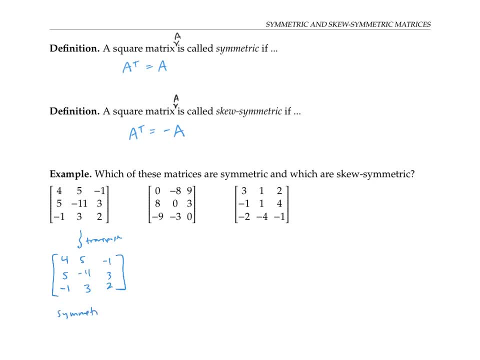 Therefore this matrix is symmetric. Notice how a symmetric matrix has symmetry across its diagonal- the entries. if we reflect them over the diagonal, we get the same thing. That makes sense because taking the transpose is like flipping rows to columns. Let's see what happens when we take the transpose of. 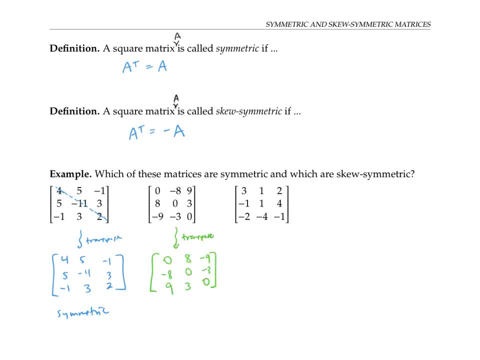 the next matrix. The resulting matrix is exactly the negative of the original matrix, which is skew symmetric. So this matrix is skew symmetric. Once again, it's useful to think about the diagonal. Notice that all the entries above the diagonal if we flip them across. 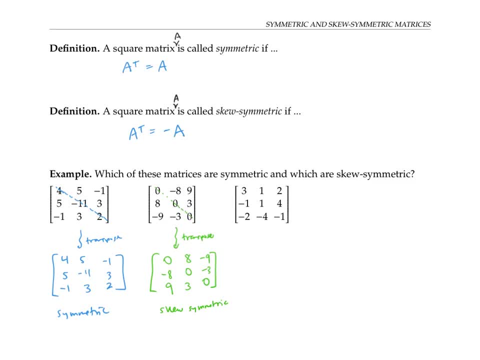 the diagonal. they line up with their negatives on the other side. Notice also that we have zeros all along the diagonal. If a matrix is skew symmetric, it has to have zeros on its diagonal, Because when we take the transpose, the entries on the diagonal stay where they. 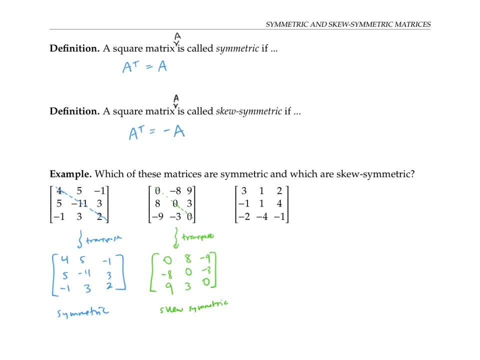 are, And so the only way that an entry can be its own negative is if it's zero. What about this third matrix? What happens when we take its transpose? we definitely don't get the same matrix. For example, this entry here is one, but the corresponding entry in the original. 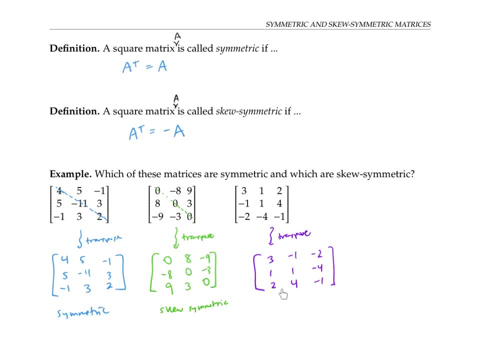 is negative one, So we don't have the same matrix here. So the matrix wasn't symmetric And we don't quite have the. the negative of the original mean most of the entries are the negatives of their corresponding entries, But not the ones along the diagonal, And so it can't be skew symmetric either, This matrix. 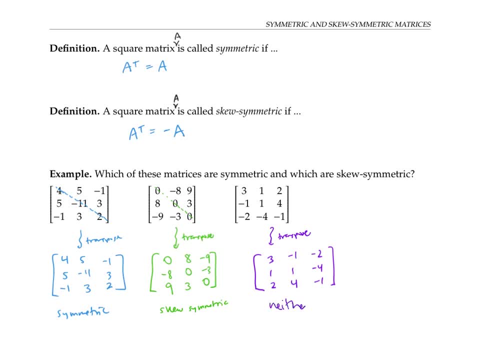 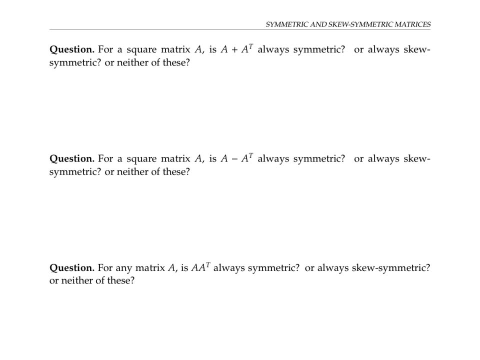 is neither. We know that symmetric and skew. symmetric is related to the idea of transpose. So let's see what happens if we take a matrix and add its transpose or subtract its transpose or multiply by its transpose. Please pause the video and try to answer these three questions. 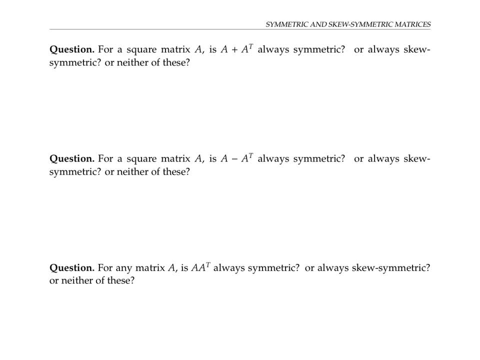 You may want to write out a matrix A and try an example. For a square matrix A is A plus A, transpose always symmetric, skew symmetric or neither of these. If I look at an example, here's an A, Here's its transpose And here's the sum. we get a symmetric matrix for this. 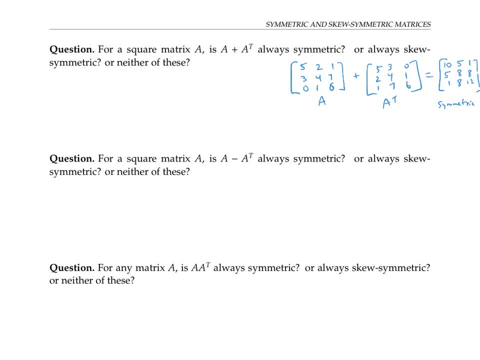 example, And in fact A plus A transpose will always be symmetric. That's because if we take A plus A transpose and transpose it, we saw in the properties of transpose video, this is the same thing as A transpose plus A transpose transpose. 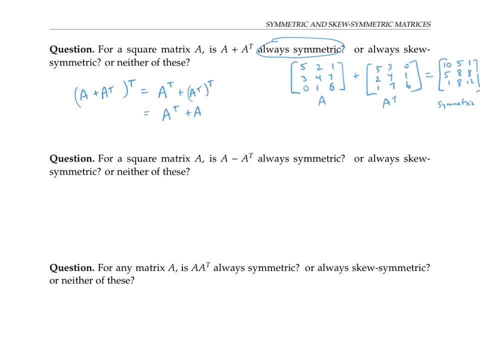 which is the same thing as A transpose plus A, which is the original matrix. Since the transpose of A plus A transpose is the same as the original, the matrix is symmetric by definition. What about A minus A transpose? Again, if we look at an example, and I'll just use the same matrix A, we get a matrix. 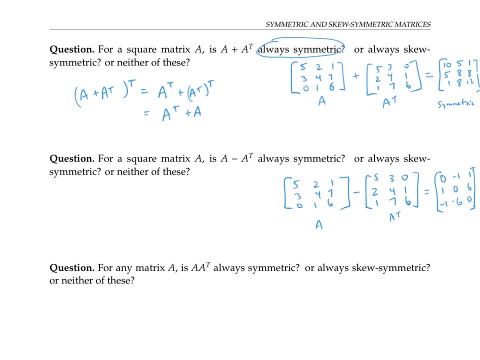 that skew symmetric. Notice how each entry is the negative of its mirror image: entry across the diagonal and all the entries on the diagonals are zero. In fact, A minus A transpose is always skew symmetric. We can write out the argument like we did before. 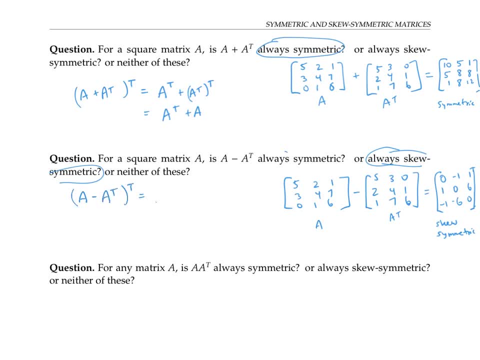 A minus A transpose transpose is the same thing as A transpose minus A transpose transpose, Because subtracting two matrices and then switching the rows and columns is the same: switching the rows and columns first and then subtracting, But A transpose transpose is. 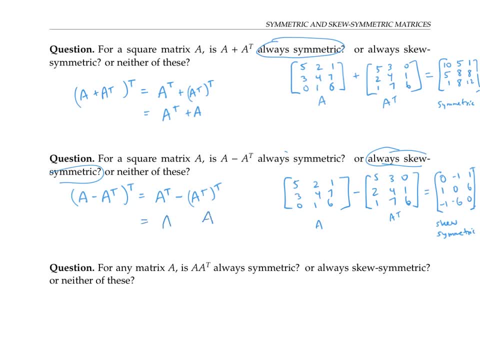 the same thing as A, So this is just A transpose minus A, which is the negative of A minus A transpose. So when we take the transpose of A minus A transpose, we get the negative of the original And that means that matrix A minus A transpose is skew symmetric by definition. 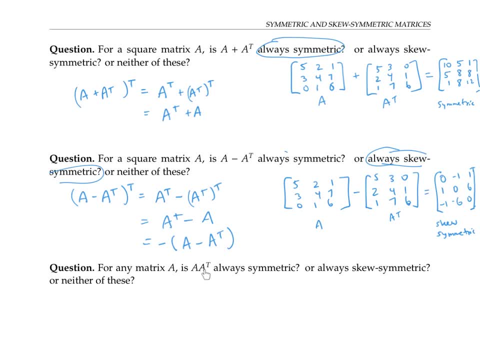 Finally, what about A times A transpose? Here we're taking the transpose of A and we're multiplying on the left by a notice that A times A transpose is always a square matrix, whether or not a is a square matrix. That's because if A has dimensions, m, times and a, 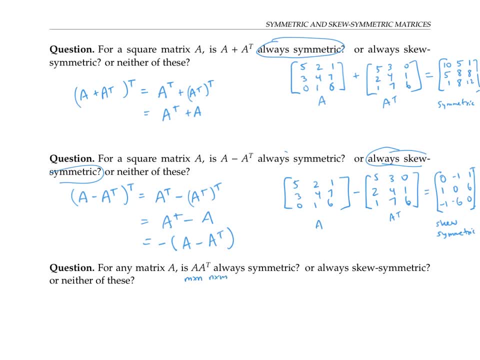 transpose will have dimensions n times m and the product will have dimensions m times m. So it makes sense to ask the question if A times A transpose symmetric or skew symmetric, whether or not a is square, because this will still be square. 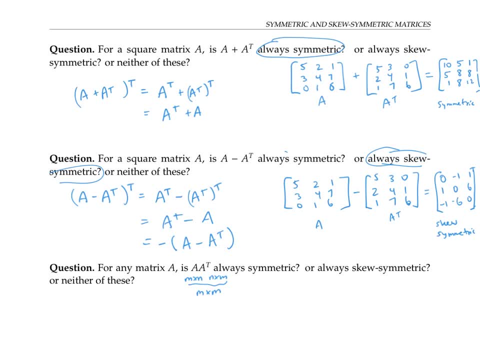 we could write out an example and check it with an example, But I'm going to go straight to writing a a transpose and taking the transpose of that and seeing what I get. Recall that the transpose of a product is the same thing as taking the product of the transposes, where 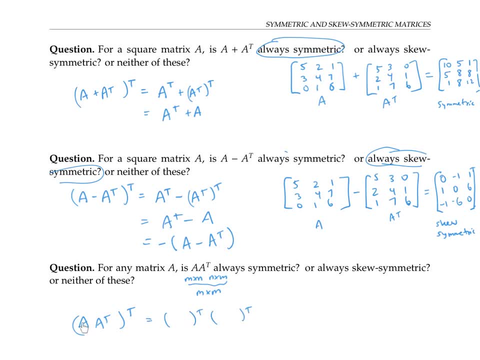 you do the multiplication in the opposite order. So instead of a times a transpose, I'm going to put the second one, a transpose, in the first spot and the first one, a, in the second spot. Well, a transpose, transpose is just a. So this is a times a transpose. 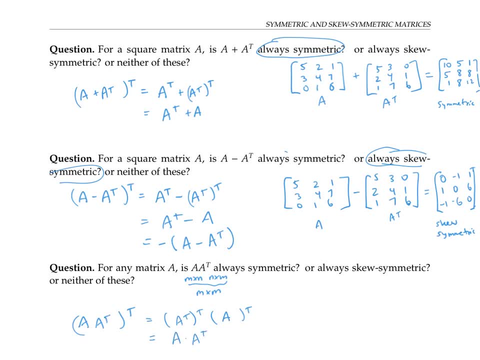 which is the original matrix that we started with, And therefore we have that a times a transpose is symmetric. So we checked that a times a transpose is always symmetric. What about a transpose times a? I'll leave it to you to write out the details and check that this product is also always. 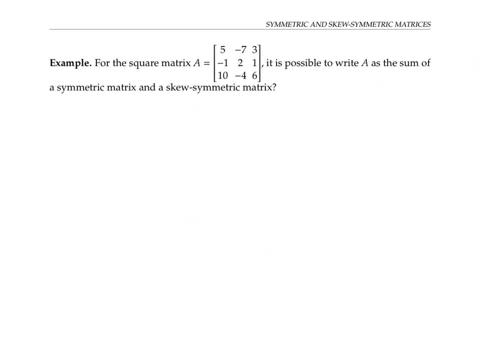 symmetric. Finally, I have a question for you. Is it possible to write this square matrix as the sum of a symmetric matrix and a skew symmetric matrix? Okay, try your hand at it and see if you can do that. It's possible to solve this problem. 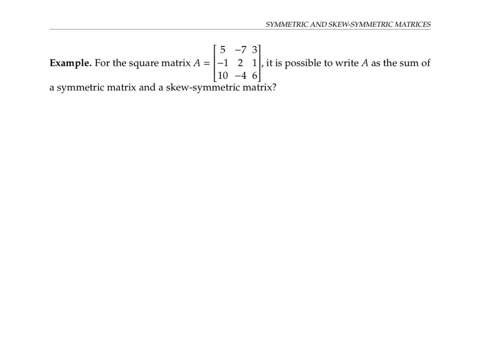 by trial and error, But I'm going to show you a sneaky shortcut. Recall that a plus a transpose is symmetric And a minus a transpose is skew symmetric. But notice that if I take a plus a transpose and add it to a minus a transpose, that's the same thing as a minus. 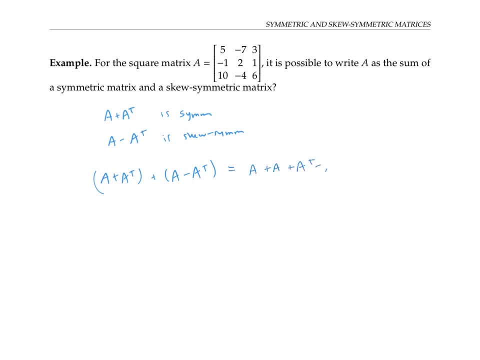 a transpose plus a plus a plus a transpose minus a transpose, But a transpose minus a transpose. when you take a matrix and subtract all its entries, that just gives you the zero matrix, And so we just have a plus a, which is the same thing as to a. So if I take one, 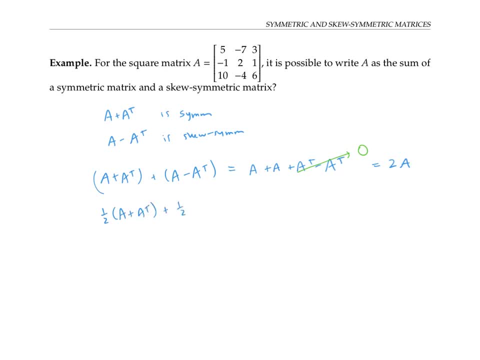 half of a plus a transpose, plus one half of a minus a transpose. these will still be symmetric and skew symmetric, But now they'll add up to one half a plus one half a, which is just a. So a nice trick to solve this problem is to take first a matrix, the matrix, one half a plus a transpose. that's. 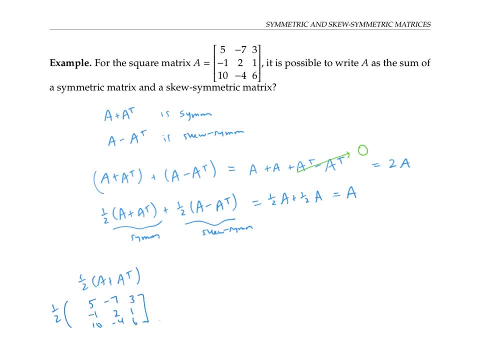 one half this matrix plus its transpose, which works out to one half of this matrix, which simplifies to this. then we'll take one half of a minus a transpose which simplifies to this. Notice that the first matrix is indeed symmetric And the second is skew symmetric. 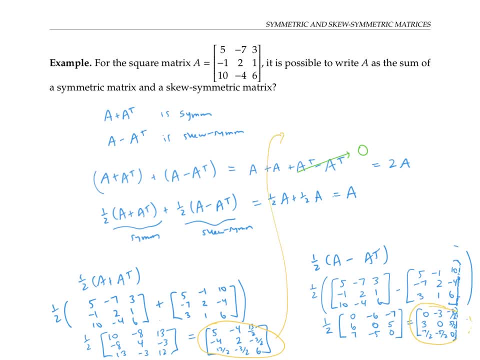 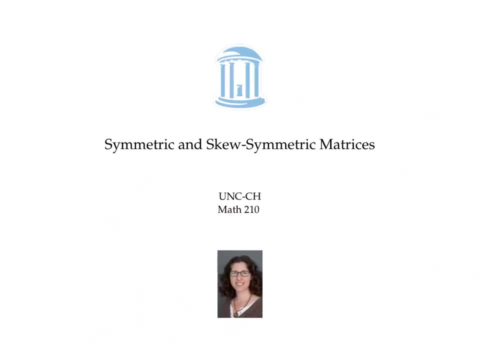 you can check that when we add up these two matrices, we do indeed get our original matrix a. This video was about symmetric matrices, But now we're going to talk about symmetric matrices Which are their own transpose and skew symmetric matrices, which are the negative of the transpose. 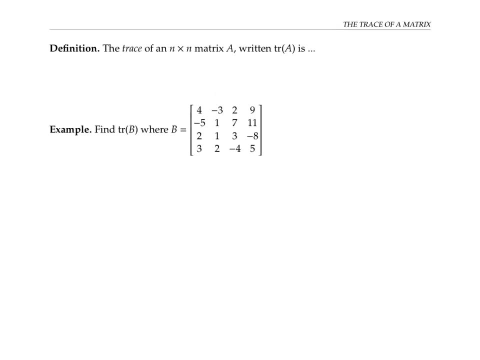 This video is about the trace of a matrix. If you have an n by n square matrix a, the trace of the matrix written t r of a is the sum of the entries on the diagonal. By diagonal I mean the diagonal that starts at the upper left and goes down to the bottom right, And 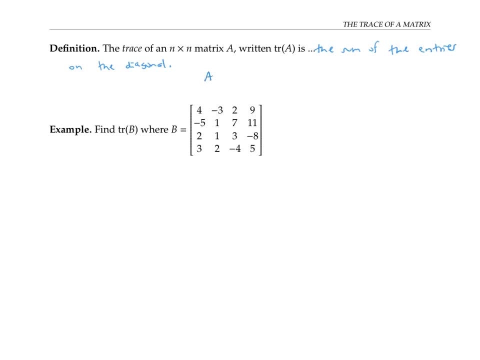 the bottom right In abstract notation, if our matrix A has entries given by a one, one, a one two and so on, through a one n in the first row, a two, one a two, two through a two n and second row, and so on down to a n, one n, two through a n, n in the last row. 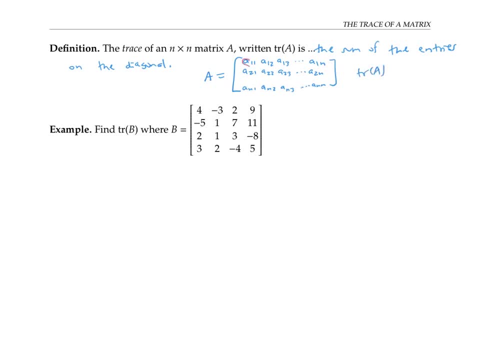 then the trace of a is what you get by adding up These diagonal entries, the entries of the form a one, one plus a two, two plus a three, three, all the way through a, n, n. But it's easier to talk about the trace in a specific 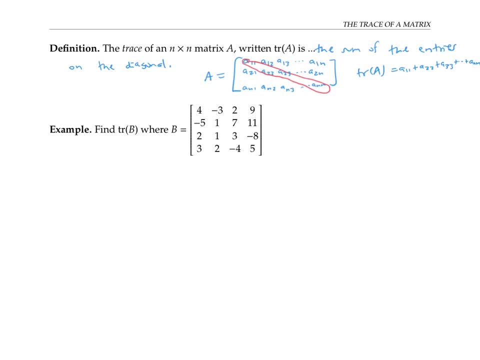 example For this: four by four, matrix B, the trace is what we get by adding up the four numbers on the diagonal, four plus one plus three plus five, and these add up to 13.. Let's see how trace interactions work. Trace interacts with other operations on matrices. Suppose that A and B are two square. 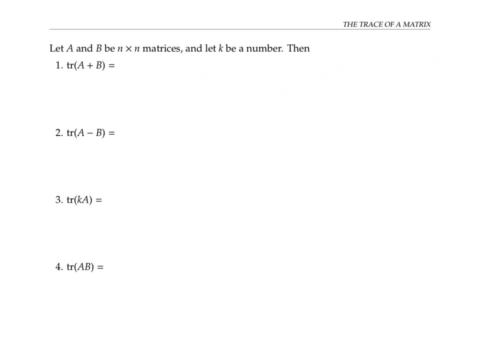 matrices of the same size and by n matrices, And let's let K be a number scalar. then what can we say about the trace of A plus B? Well, if we take two matrices and add them together, we do that by adding corresponding entries. So if we want to take the trace of A plus, 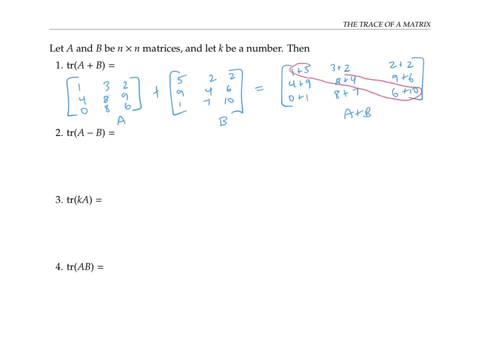 B. we're adding up all those numbers on the diagonal, But that's just exactly the same thing as taking the sum of these three numbers and adding those three numbers. Therefore, the trace of A plus B is the same thing as the trace of A plus the trace of B. Similarly, when we subtract, 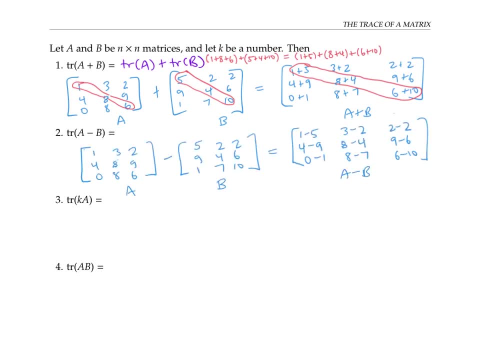 two matrices subtract corresponding entries. so the trace of A minus B, which is the sum of these numbers on the diagonal, is the same thing as taking the sum of these these numbers and subtracting all of these numbers. Therefore, the trace of A minus B is the same thing as. 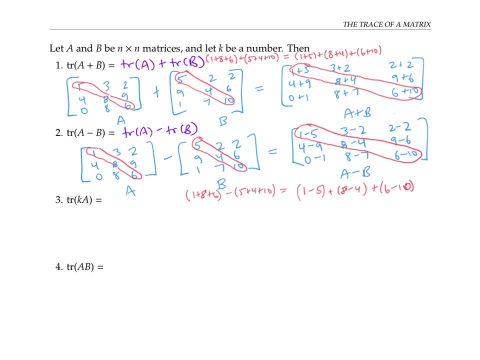 the trace of A minus the trace of B. Let's look at a scalar multiple k times a matrix. I'll use the same matrix. a scalar multiple means I just multiply all these entries by k. So if I want to take the trace of k times a, I'm adding up these numbers, which is: 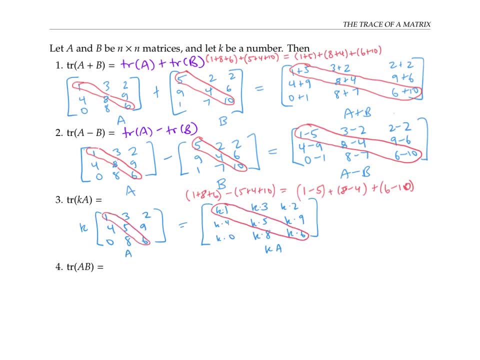 the same thing as adding up these numbers and multiplying by k, since multiplication is distributive. Therefore, the trace of k times a is the same as k times the trace of a. Well, following the pattern here, you might expect that the trace of A times B is: 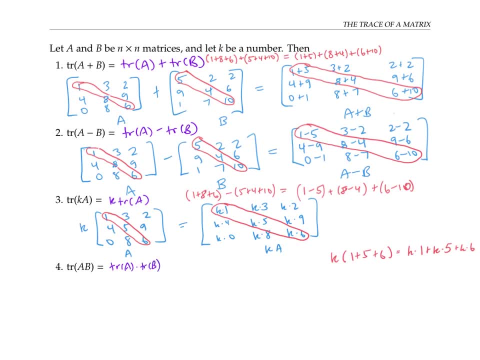 the trace of A times the trace of B. But in fact this is not true. For example, here I have two two by two matrices, both of whose trace is zero. But when I take the product I get a matrix whose trace is definitely not zero. But there is at least one thing we can: 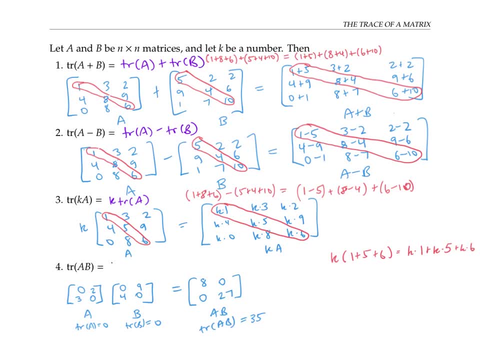 say about the trace of A times B, And that's that it's equal to the trace of B times B. It's certainly true for this example, But it's actually true in general for any pair of n by n matrices. Suppose I have some general matrix A with entries a, one one, a one two. 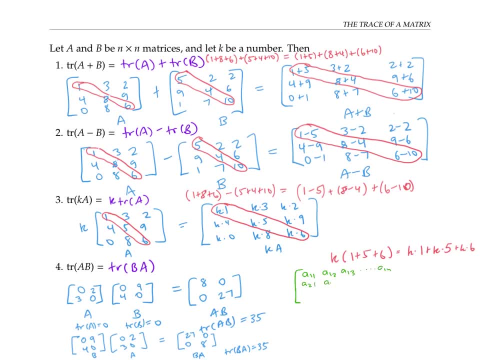 through a one n on the first row, a two one a two, two through a two n on the second row, and so on, And the general matrix B with its entries labeled B one one a two n, and so on. To find the trace of A times B, we're going to have to add up the elements on the. 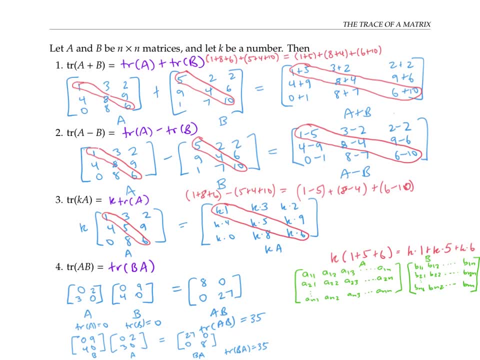 diagonal of A times B. Well, the entry in the first position of the diagonal of A times B is going to be the first row times the first column. So that would be a one, one b one, one plus a one, two b two, one plus a one, three b three, one. all the way through: a one n. 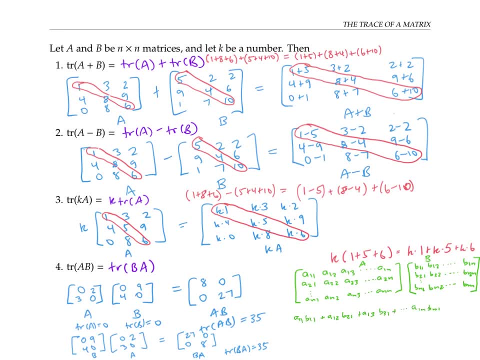 b n one. That's how I would multiply this first row by this first column. So that would be the first entry I add up in the trace of AB. The next entry that I add up in the trace of AB would be the entry that ends up in the second row and second column of the product. 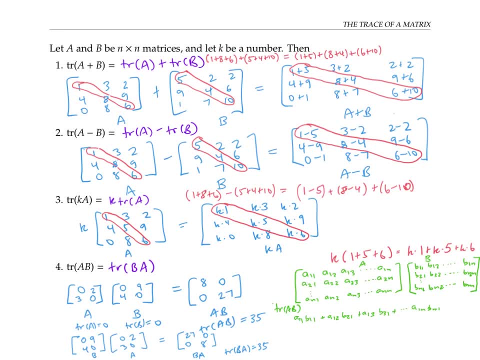 So that's the entry I get by multiplying row two of A by column two of B, So that would have entries a, two, one, b one, two plus a, two, two, b, two, two plus a, two, three, b, three, two, all the way through: a, two, n, b n, two. The next entry of the trace would be the entry. 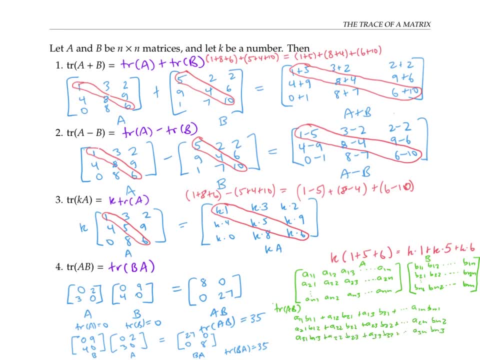 in the third row and third column of the product. I add up more and more entries till I get to the nth row and nth column entry of the product. I'd have to add up all these numbers to get my trace of AB. But what if, instead? 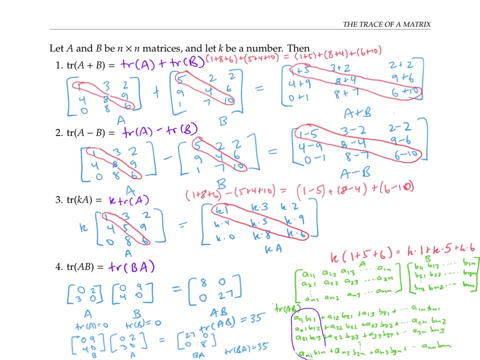 I add up this way, sort of one column of this big mess at a time. This first column of terms actually corresponds. if I added all these up, that would be what I would get. by multiplying the first row of B times the first column of A, right, I get b one one times a, one one b. 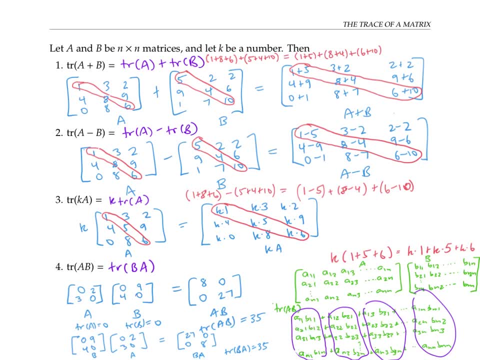 one two times a. two one, that's this. b one three times a: three one. That's this at the end. b one n times a n one. That's this right here. So this column of numbers that circled in purple added up. 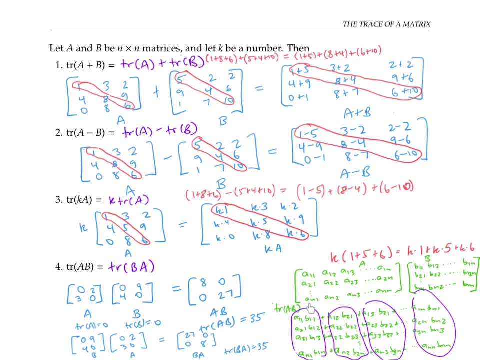 would be the first row of B times the first column of A. the second column added up would be the second row of B times. the second column of a next purple column would be the third row of B times the third row of A, and so on. So each of these purple columns added up is 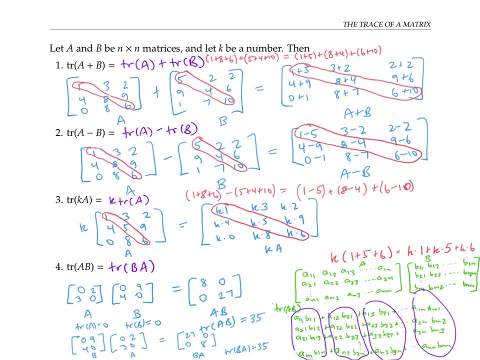 an entry on the diagonal of the matrix B times a, And when I add all these numbers up, I'm really just adding up the trace of B times a. trace of A times B is therefore equal to the trace of B times a. there's just a couple. 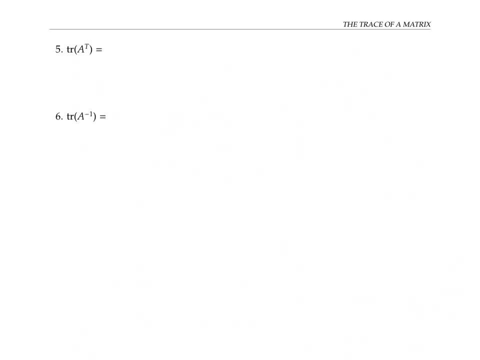 more properties. I want to look at If we have a matrix A and I take its transpose. the transpose doesn't change the entries on the diagonal and therefore it doesn't change the trace. The trace of a transpose is the same as the trace of a. Last of all, what can we say about? 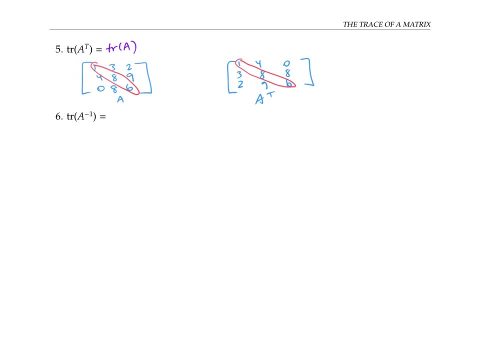 the trace of A, inverse In terms of the trace of A. Well, it turns out pretty much nothing. As an example, suppose I have these two matrices- I'll call them A and B- that both have the same trace, right. 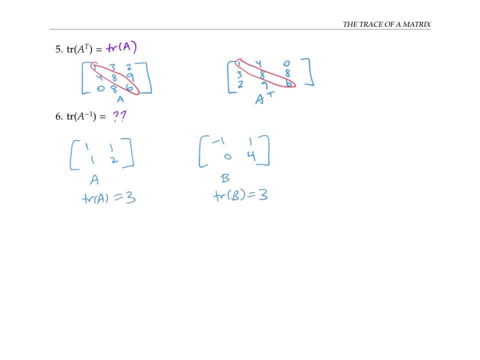 these both have a trace of three, But if I calculate their inverses, the trace of A inverse is three, while the trace of B inverse is negative three fourths. There's no simple relationship between the trace of the inverse matrix and the trace. 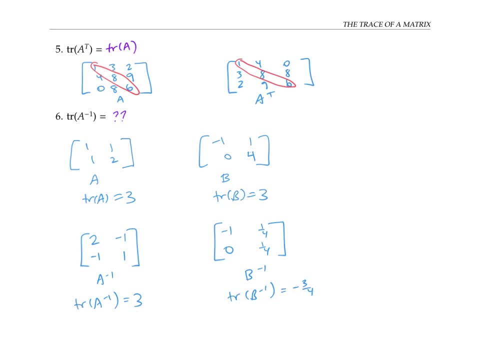 of the original matrix. If you're especially observant, you might notice that for two-by-two matrices there is a relationship between the trace of the inverse and the trace of the original. and determinant of the original, Namely the trace of the inverse, is the trace. 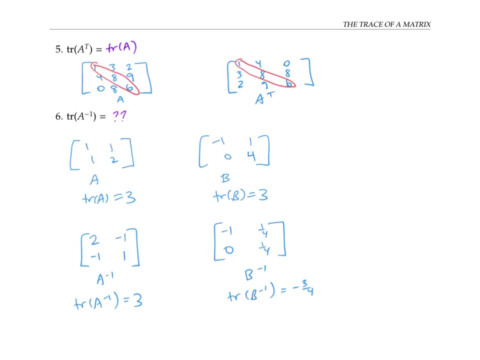 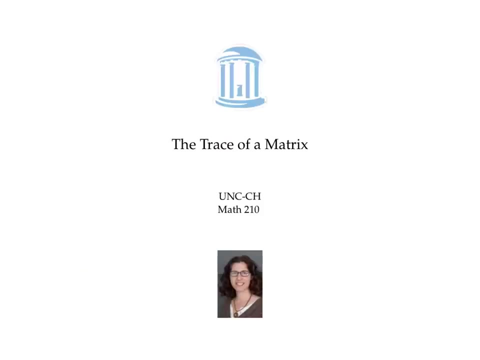 of the Ori Divided by its determinant. But things get even more complicated for higher dimensional matrices and there's no relationship between trace and inverse. This video was about the trace of a matrix and how it interacts with other operations on matrices. I want to remind you that a trace- 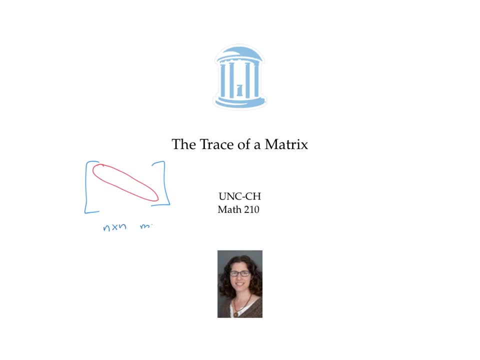 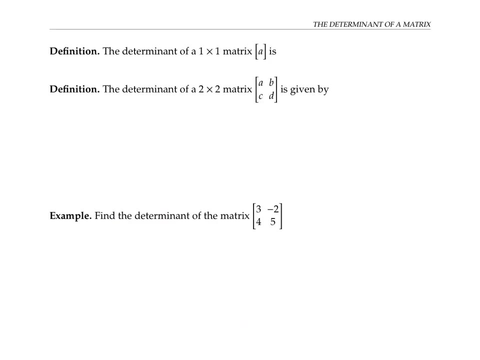 is only defined for a square matrix. This video shows how to calculate the determinant of a matrix. determinants are only defined for square matrices- matrices with the same number of rows and columns. People don't usually talk about the determinant of a one by one. 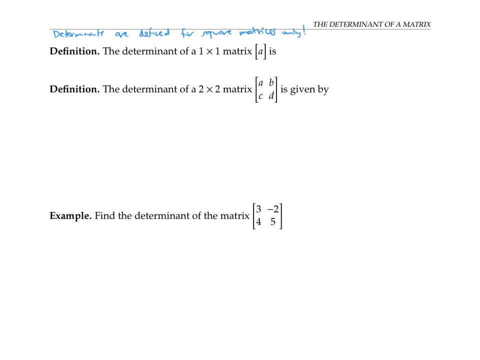 matrix. people don't usually talk about one by one matrices at all, But if, for some reason, you needed to compute the determinant of a one by one matrix, a matrix with only one entry, then that determinant would just be the entry itself. So now let's get to the 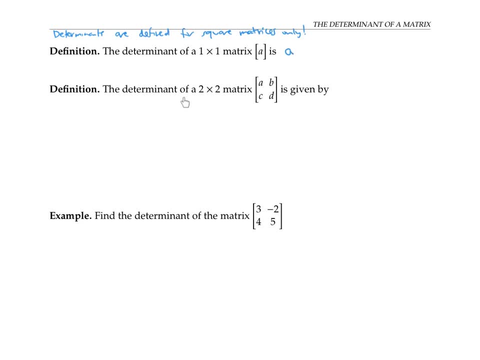 simplest real situation where you'd want to determinant the determinant of a two by two matrix. That determinant is given by this crisscross product: A times D minus B times C. There are a few notations for determinant. Sometimes you might just see the letters det of your matrix, So that means the determinant of the matrix. 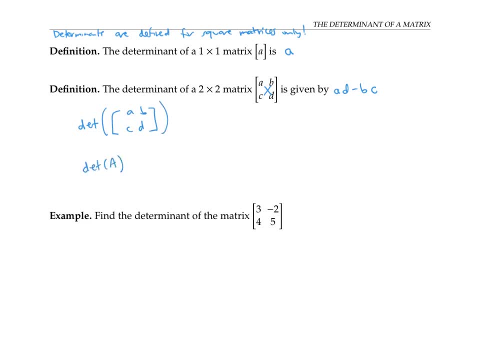 or you might see det of a, if a is the name of your matrix. Another notation you might see is just straight lines, kind of like big absolute value lines surrounding the entries of your matrix. So all three of these are notations for the determinant of a matrix A with entries ABCD. So now let's. 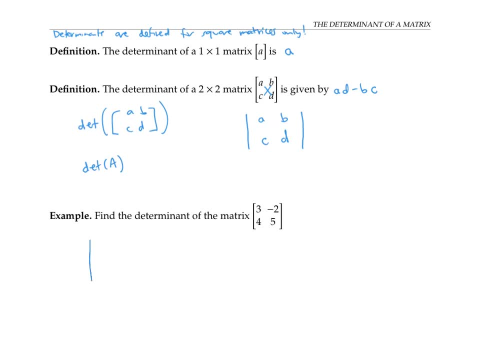 work. an example: we're going to find the determinant of the matrix with entries three negative 245.. So that means three times five minus four times negative two, which is 15 minus negative eight or 23.. Once we go up in size from a two by two matrix to a three by three, 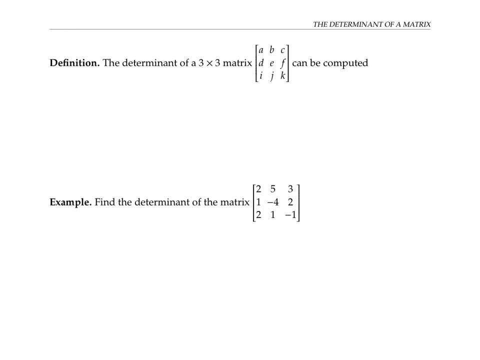 matrix, things get a little more complicated. we can compute the determinant of a three by three matrix by expanding along the first row and computing an alternating sum of entries times determinants of two by two matrices. By an alternating sum of entries we can compute: 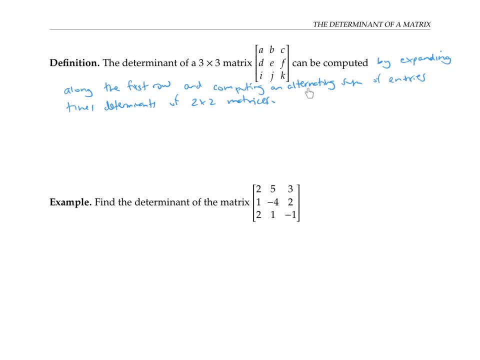 the determinant of a three by two matrices, By an alternating sum. I mean you will alternate adding, subtracting, adding, subtracting and so on. Let me explain more precisely what I mean. Expanding along the first row means we start with the first entry of the first. 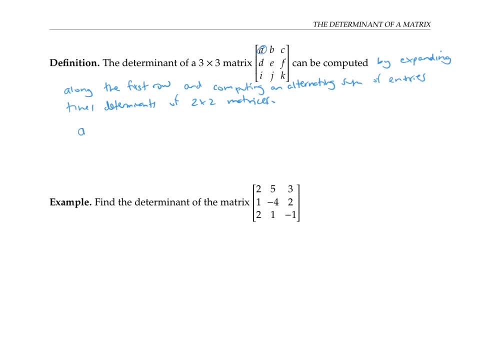 row, so a. And then we take the determinant of the matrix we get by crossing off the row and column that a is in, So that's the determinant E, F, J and N, So that's the determinant JK. Next we take the next entry on that row, B, and we multiply B by the determinant. 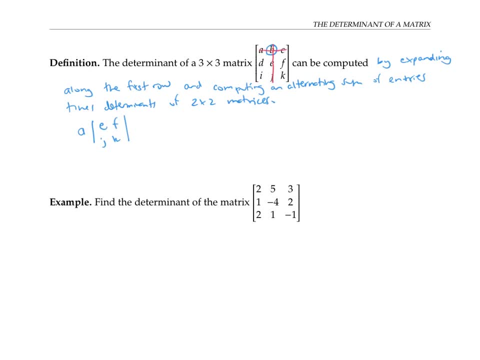 of the two by two matrix. we get by crossing off the row and column that B is in, But we're doing an alternating sum, So we're going to subtract this one B times the determinant of d, F, I, k. Continuing along the first row, we take the next entry, C, and we're going. 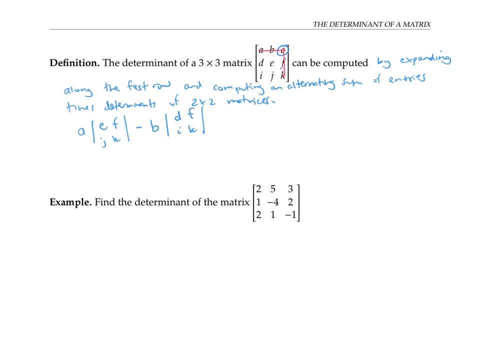 to add C times the determinant of the matrix we get by crossing off the row and column that C is in, So that's plus C times the determinant of D, E, I, J. If you like, we can write all that out as a formula: a times e, k minus j, f minus b times d k. 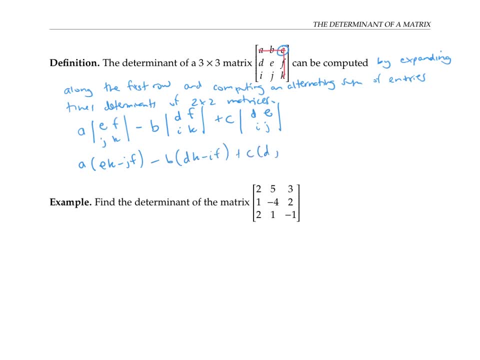 minus i, f plus c, times d, j minus i, e. But I think it's easier just to remember the process rather than some complicated formula, So let's use this process on this example determinant. we're going to expand along this top row, So we'll start with the number two and multiply. 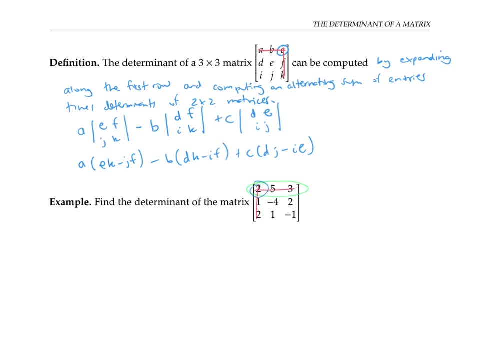 it by the matrix. we get by crossing off the first row and first column two times determinant of negative four to one negative one, then subtract five times the determinant of 12 to negative one, And now we'll add three times the determinant of one negative four to one. that works out. 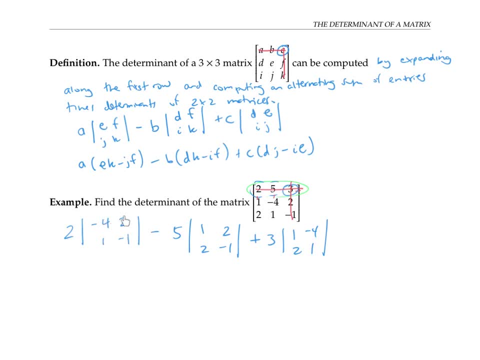 to two times this product minus this product. So two times four minus two minus five times negative one minus four plus three times one minus negative eight, And that all works out to an answer of 56.. Now I have a question For you. What's so special about expanding along the first row? I invite you to try expanding. 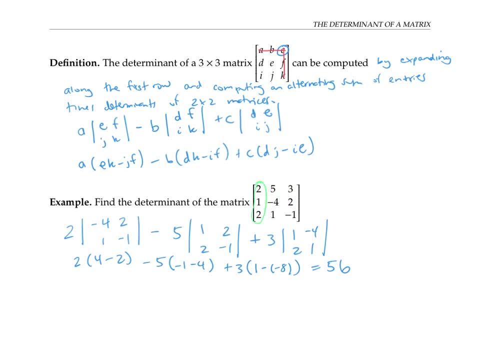 around the first column. instead, do the same sort of process. take one number at a time, cross out the row and column it's in and do an alternating sum That way. when I do that, I get two times the determinant of negative four to one negative one minus one times. 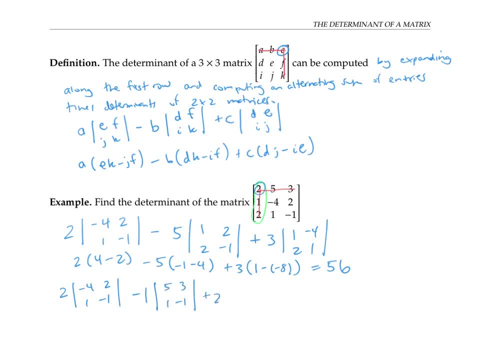 the determinant of 53, one negative one plus two plus two times the determinant of five, three negative 42.. And that works out to 56.. Try using a few more rows or columns. If you use the second row, you have to be careful to. 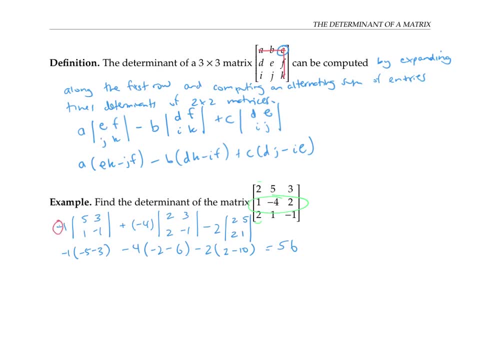 use a negative sign in front of the first entry, a plus sign instead of the second and a negative in front of the third. So it's still an alternating sum, but it's going negative here, positive here and negative here- Same thing if you expand down the second column. 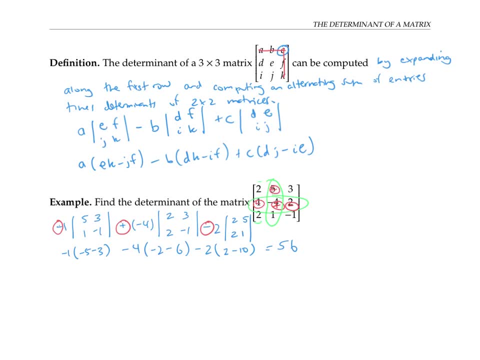 you have to have a negative in front of the five, a positive in front of the four and a negative in front of this entry one. But if you use the third row or the third column, you're starting with a plus again and still doing an alternating sum. 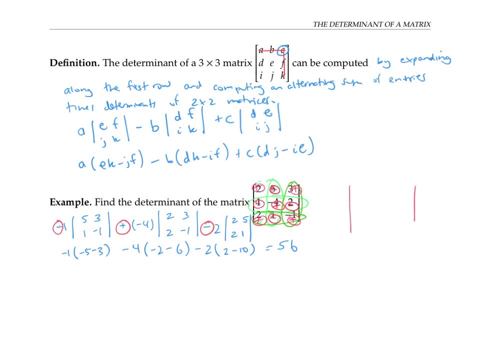 So it's kind of like the matrix itself has a checkerboard of pluses and minuses And when you add up these entries, times these two by two determinants, you just got to make sure you add them with the alternating sum, that that starts with the right negative, or 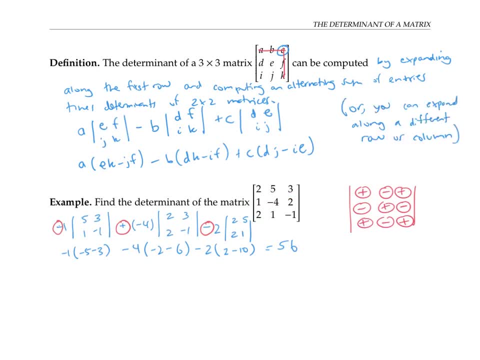 positive sign. I won't prove it here, But it's kind of cool that you get the same answer no matter what row or column you expand along, as long as you start with the right positive or negative sign, And this can also be handy for computation, if there happens. 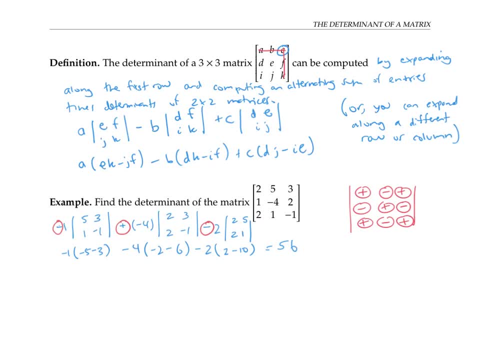 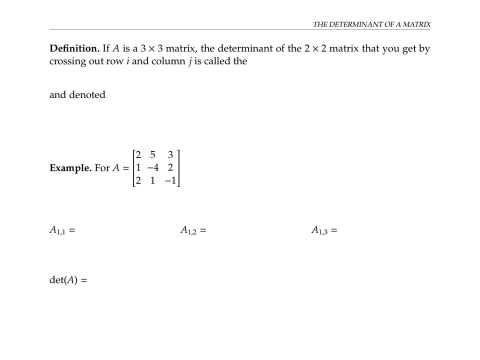 to be a row or a column that has a lot of zeros in it. you might want to expand along that one. to save yourself some arithmetic, Let me revisit what we just did with a little bit of definitions and notation. So for a three by three, matrix A, the determinant of, 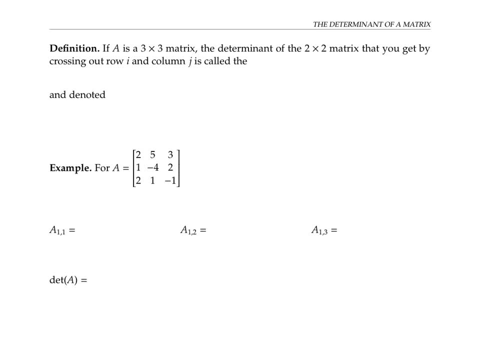 the two by two matrix that you get by crossing out the ith row and the jth column is called the i. j minus Intermediate is a minor and is denoted a ij. So for example, if we want to define the a one one minor, that would be the determinant of the matrix we get by crossing off the first. 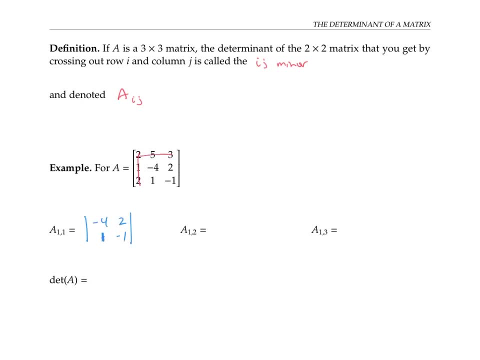 row and the first column, So that would be four minus two, which is two And a one. two is the determinant of the two by two matrix we get by crossing off the first row and the second column, So that would be the determinant of 122, negative one, which works out to negative five. 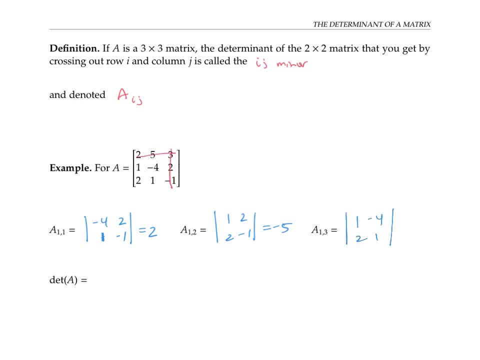 Similarly, a 13 works out to nine, And when we calculated the determinant of matrix A we took the alternating sum of entries times minors. So we took a 11, the entry in the one one position times a 11, that minor minus a little. 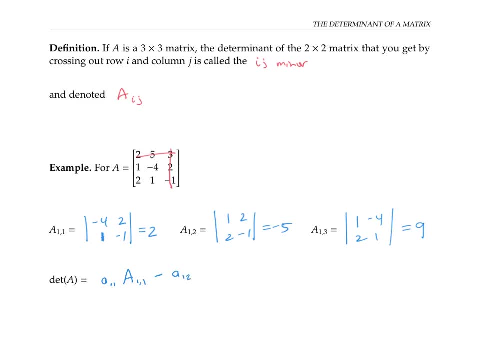 a 12,. the entry in the first row, second column, times the minor, a 12.. And then we added little, a 13 times the determinant of that two by two, matrix a 13.. We also added a 13.. We also saw we could calculate the determinant by expanding along different rows or columns. 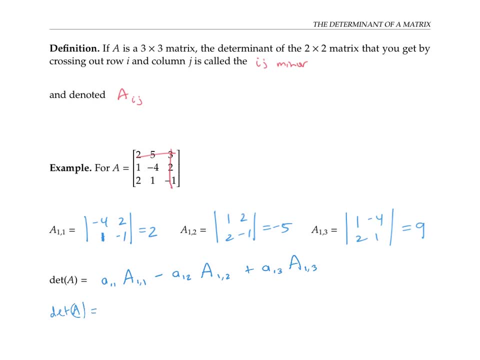 for example, along the third column, would be a 13, capital A 13, minus a 23, capital A 23, plus a 33, capital A 33.. Now that we have this terminology and notation, let's extend this to find the determinant. 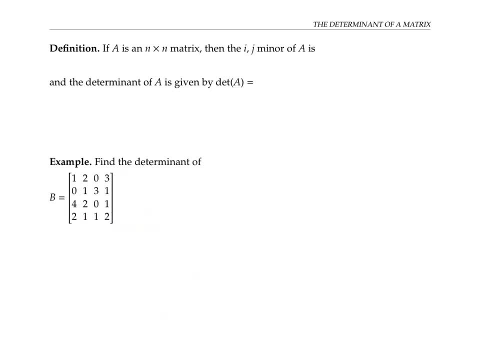 of matrices of higher dimension. So in general, if A is an n by n matrix, the ij minor of A is the determinant of the n minus one by n minus one matrix. we get, by crossing out row i and column j of a, the 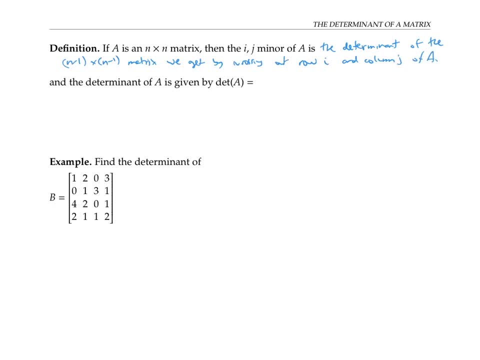 ij- minor of matrix. A is just a, i, j as before, and the determinant of A is given by what we get by expanding along the first row of A and taking an alternating sum of entries times. So in symbols that would be: little a- 11, times. minor. big A- 11, minus. little a- 12, times. 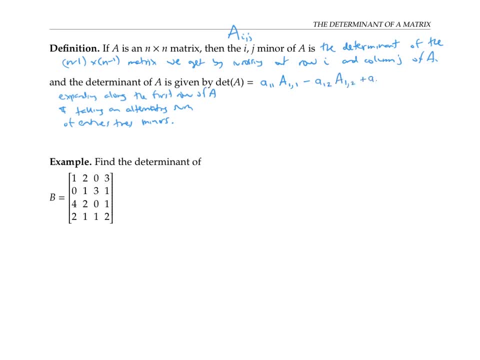 minor, big A 12, plus, little a 13,, big A 13,, minus, and so on, until we finally get to a one n, big A one n, and that will be either a plus or minus, depending on whether n is even or odd. 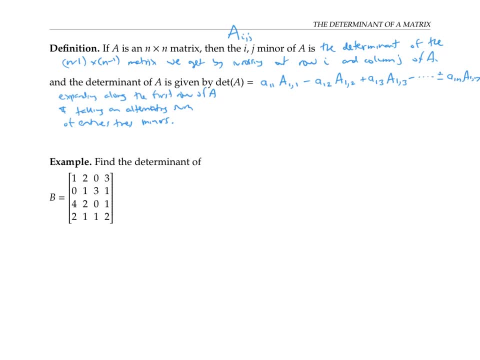 As with the three by three matrices, it turns out that you can actually expand not just along the first row but along any row or column, as long as you start with the plus or minus sign. that corresponds to this checkerboard pattern of plus or minuses, with a plus in. 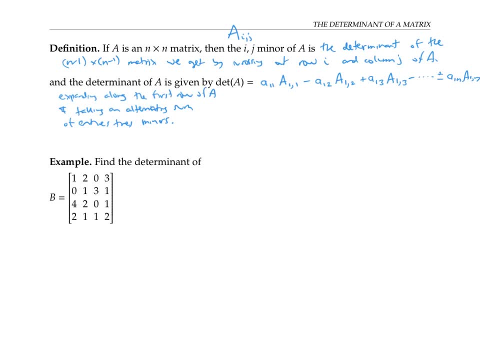 the upper left corner. So please stop the video and use this algorithm to calculate the determinant of this four by four matrix. Beware, it's going to involve a lot of arithmetic. So I'm going to expand along the first row. That means I'm going to start with the one times the determinant of this three by three. 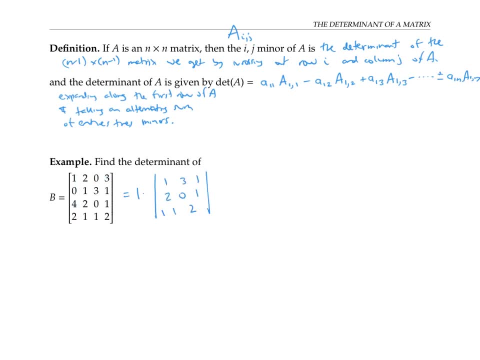 matrix, And I'm going to subtract the two times the determinant of this three by three matrix plus zero times this two by three by three matrix Zeroes. make me happy here we're not gonna have to worry about this, because it's just. 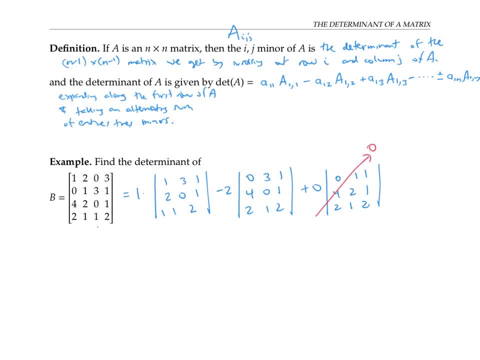 zero. And finally I can subtract three by three. So I'm going to start with the one times the determinant of this three by three matrix. Now I'm going to compute my three by three determinants each separately And I'll just expand each one along its first row. 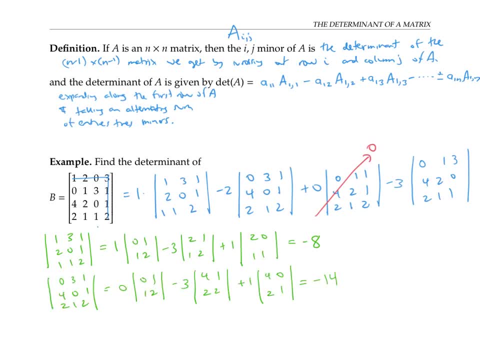 So I get minus eight for the first one, minus 14 for the next one and minus four for the last one. So this all adds up to one times negative eight, minus two times negative 14, minus three times negative four, And the final answer is zero. 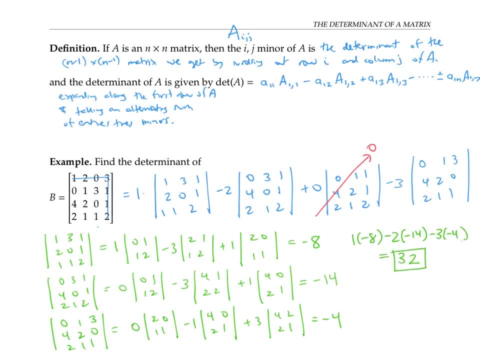 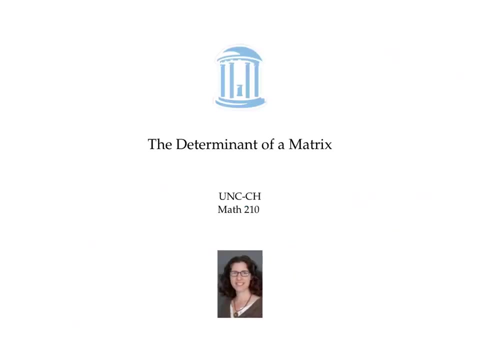 And the final answer for the determinant of this four by four matrix is 32.. And if you chose to calculate this determinant by expanding instead along a different row or column, at any stage of the way, you should still get the same answer. This video showed how to calculate the determinant of a matrix by expanding along a row or column. 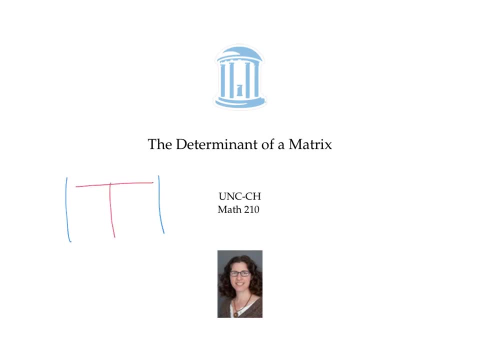 and then using determinants of lower dimension matrices. Thank you. it turns out that when two matrices are related by elementary row operations, like switching two rows or multiplying a row by a constant, then their determinants are also related. This video lays out those relationships Before we get to elementary row operations. 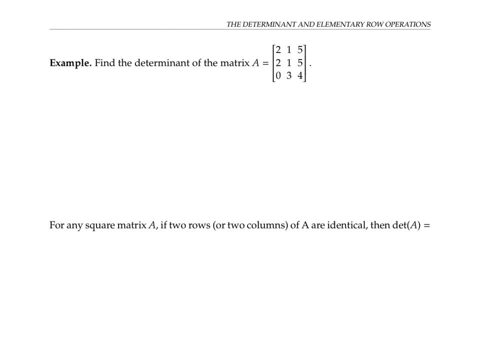 I want to do one warm up example. Please pause the video and see if you can figure out the determinant of this matrix A. I'm going to calculate the determinant by expanding along the first row, So I'm gonna get two times the determinant of 1534 minus one times the determinant. 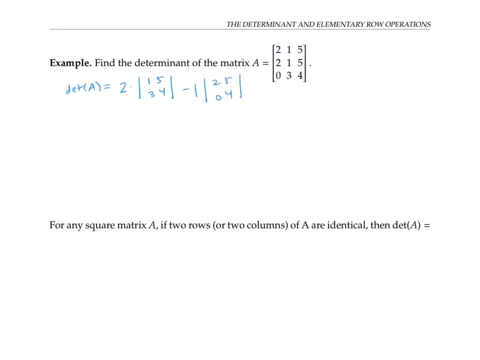 of 2504 plus five times the determinant of 2103.. So that works out to two times four minus 15, minus one times eight minus zero, plus five times six minus zero. If I add that all up, I get minus 22 minus. 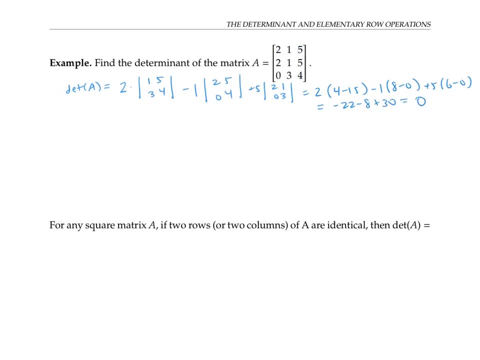 eight plus 30,, which adds up to zero. Is it a coincidence that I got zero? No, actually I could have predicted that before I did any computations. Notice that in this matrix the first two rows are identical. We know from a previous video that we get the same determinant. 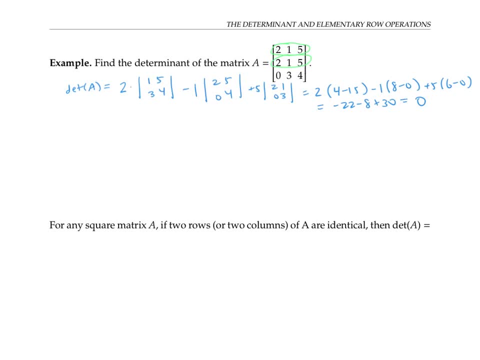 no matter which row or column we expand over. Look what happens if we expand over the third row instead. then we get: the determinant of A is going to be zero times the determinant of the matrix 1515, minus three times the determinant of the matrix 2525.. Plus four times the determinant of the. 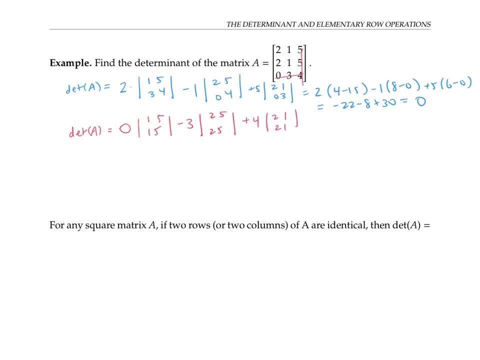 matrix 2121.. Notice that each of these two by two sub matrices has two of its rows, exactly equal, And so when I calculate any of these two by two sub matrices determinants, I'm going to get zero. Therefore, the whole determinant has to be zero. A similar calculation: 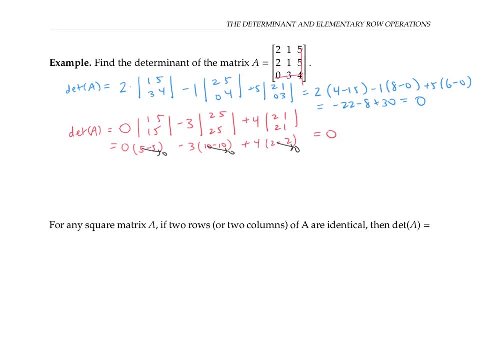 shows that for any three by three matrix that has two rows the same, its determinant will have to be zero. And in fact if we had a four by four matrix x with two rows the same, Here the first and the fourth row are the same. If we expand, 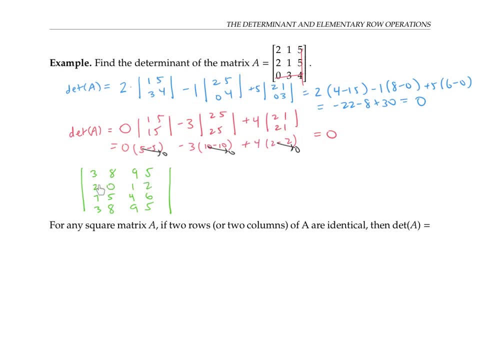 on some row. that's not the first or the fourth, those little three by three sub matrices that we take determinants of. they would have two rows the same, And so they would have all determinant zero. So the ultimate determinant would have to be zero, Using an inductive. 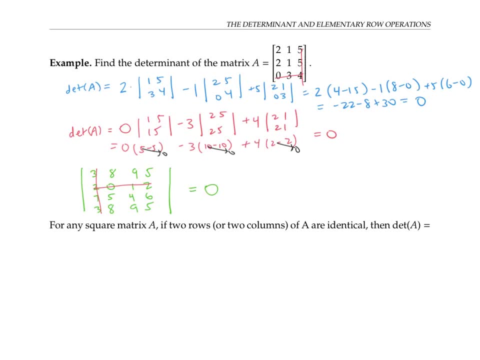 argument like that. going up one dimension at a time, we can see that it seems plausible that for any square matrix A, if two rows of A are identical, then the determinant of A must be zero, And the same thing holds if two columns of A are identical. Now let's 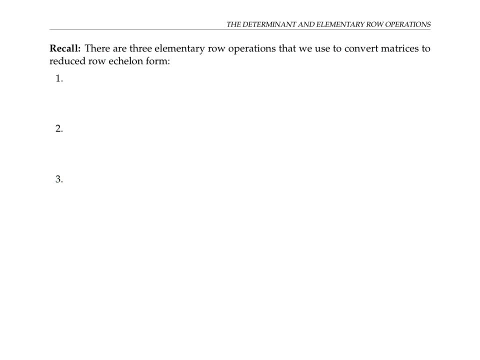 move on to the main topic of this video, the elementary row operations. Recall that there are three elementary row operations that we use to convert matrices, to reduce row echelon form. First, we might switch two rows. Second, we might multiply a row by a number. And third of all, we might 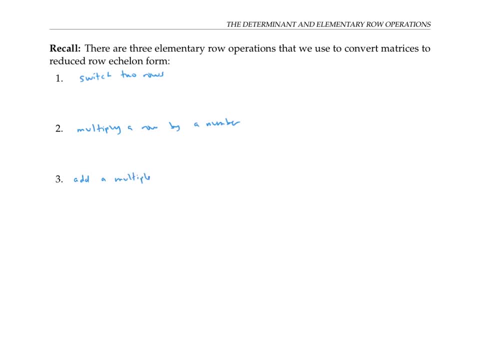 add a multiple of one row to another row, Let's see what those elementary row operations due to the determinant of a matrix. Let's start by just calculating the determinant of this matrix. So I'm going to use the matrix A, So I'll expand along the first row of the matrix. 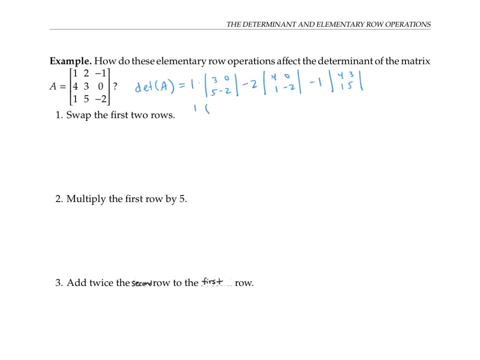 If I work out the determinants of those two by two matrices, I get minus six minus zero, minus eight minus zero and 20 minus three, So that works out to a total of negative seven for the determinant of a. Now let's see what happens if we swap the first two rows. I'll 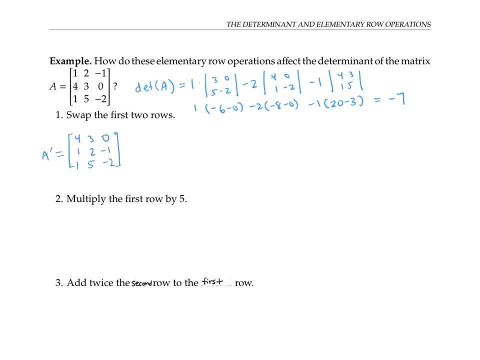 call this new matrix a prime. Well, I could calculate the determinant of a prime by expanding along its new top row, But actually I'm going to save myself some arithmetic by expanding along this middle row, because I've already worked with those numbers before, So I do. 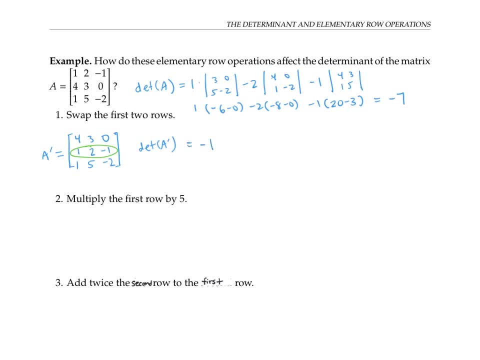 that I have to remember to start with a negative sign. So negative one times the determinant of 305, negative two, I do plus two times the determinant of 401, negative two and then minus negative one times the determinant of 4315.. Do you notice that this computation 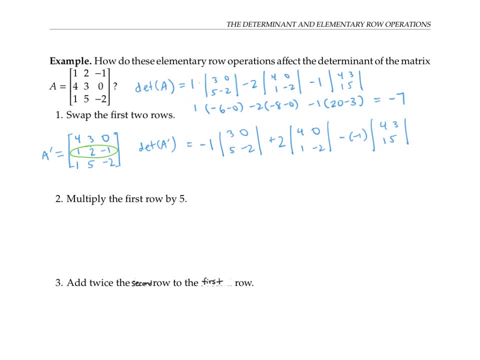 is exactly the negative of this computation right. all of these two by two matrices are the same And I have all the same coefficients. I've just started with a negative instead of a positive, So everything is the negative of what it was up here. Therefore, without having to do any additional arithmetic, I can jump right to 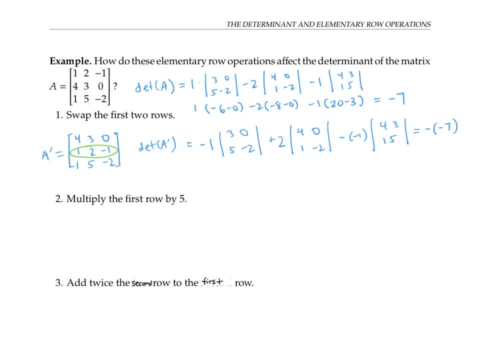 the conclusion that I'm going to get negative of the determinant of what I got before, in other words, seven. In fact, that happens anytime you switch the first two rows of any matrix And, better than that, it happens anytime you switch any two rows. So the fact that 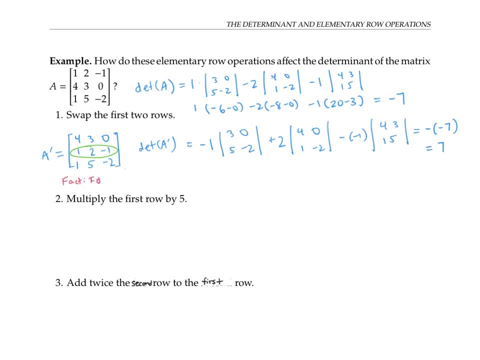 we won't prove here is that for any square matrix a, if we switch any two rows to get a new matrix, a prime, then the determinant of a prime is the negative of the determinant of a Next. let's see what happens if we multiply. 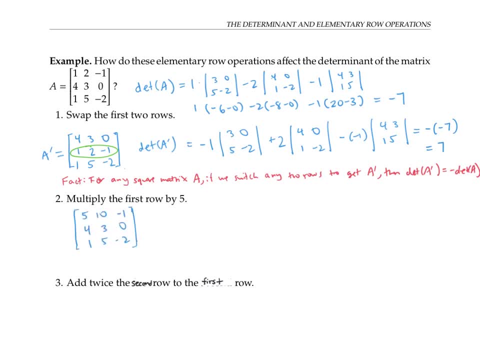 the first row of a by five. I'll call this matrix a tilde. So let me calculate the determinant of a tilde And I'm just going to expand again along the first row. Well, again, if I'm lazy, I don't. 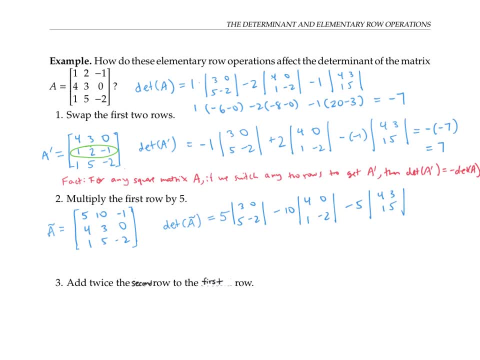 actually have to do any additional arithmetic because I've already computed enough when I first computed the determinant of a. all of these two by two matrices are the same, And these coefficients, which come from the entries in my first row, are exactly five times the corresponding coefficients for the original a, And therefore that when I do this computation, 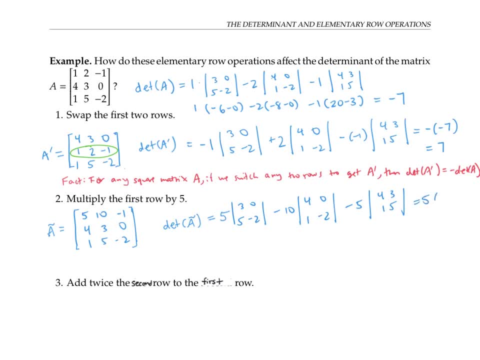 it's got to end up being five times what we got before, five times negative seven or negative 35.. And the same principle works for any matrix a and any scalar multiple and any row that we want to multiply. So the fact is, for any square matrix a and any, 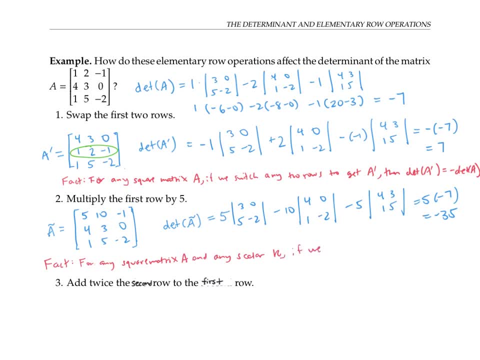 scalar k. if we multiply any row of a by k to get a matrix, a tilde, then the determinant of a tilde is going to be k times the determinant of a. let me point out that we're only allowed to multiply one row by k. 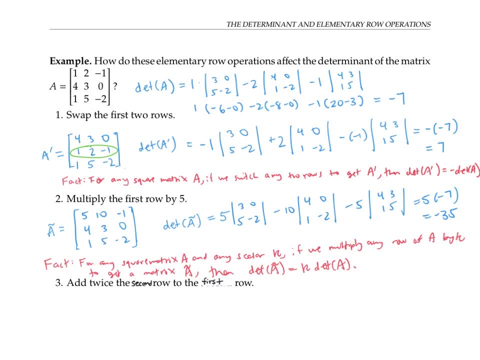 If we end up multiplying two rows by k, then the new determinant would be k squared times the old determinant. And in the case of a three by three matrix, if we end up multiplying the whole entire matrix by k, in other words multiplying each row by k, that would end. 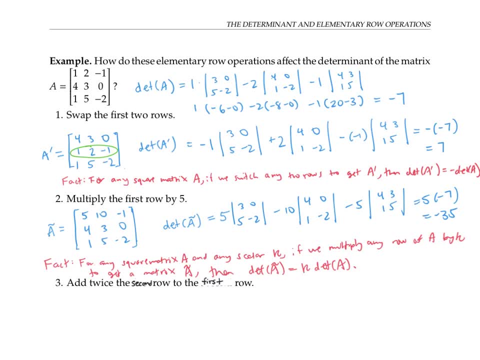 up multiplying the determinant by k cubed. Finally, let's look at what happens to the determinant if we start with the original matrix and add twice the second row to the first row. In other words, we're going to replace the first row with the first row, plus two times. 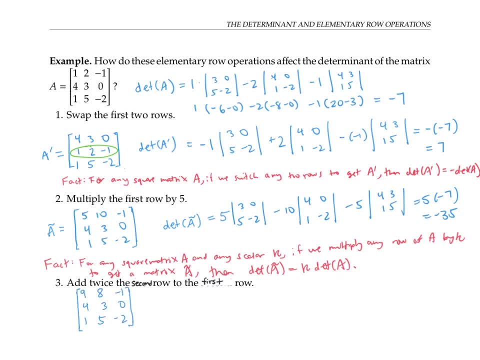 the second row. I'll call this new matrix a hat. I'll expand along the first row again. This one's a little harder to analyze, But if I just work out the arithmetic I see that I get the same answer of negative seven as I did for my original a matrix before This. 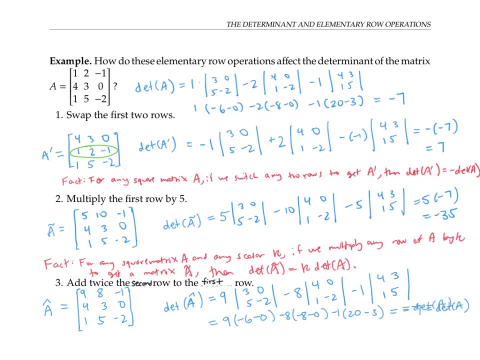 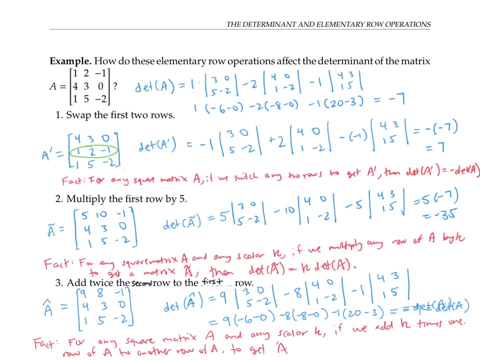 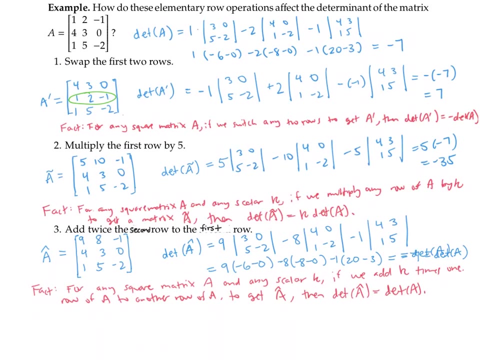 a to get a new matrix- a hat, then the determinant of a hat is exactly the same as the determinant of A. I'm going to try to give you an idea for why this property holds. When I expanded along the first row of a hat to get its determinant, the coefficients in the expansion came from. 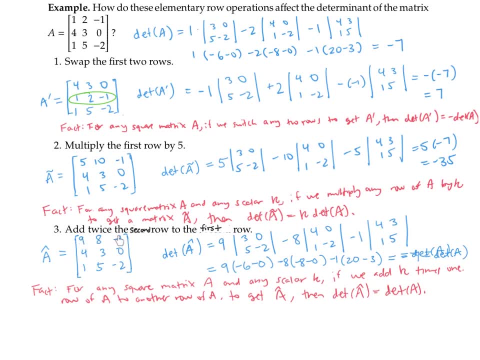 the first row of a hat, but the first row of a hat came from the first row of a, plus twice the second row of a. Let me rewrite my expansion to make that clear. Here I've color coded the part of this coefficient nine that came from the first row of a in green. 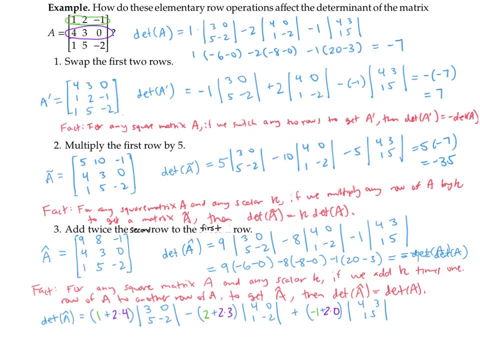 and the part that came from twice the second row I put in purple. Similarly for this coefficient of eight And this coefficient of eight And this coefficient of minus one. Now I'm going to distribute to split out the part of the determinant that goes with the green and the part of the determinant that goes. 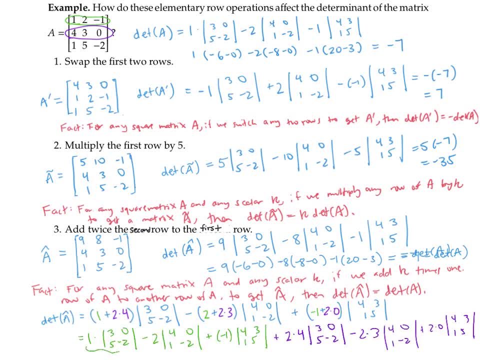 with the purple. Now you can check that this green part is exactly the determinant of a makes sense because these green coefficients came from the first row of the original a. But you can also check that this purple expression is twice the determinant of a matrix with the first two rows identical. Specifically, it's twice. 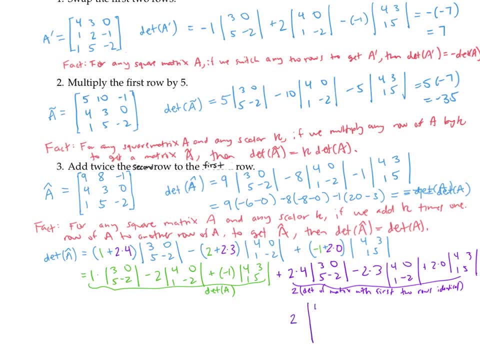 the determinant we get by replacing the first row of a with the second row of a and keeping the second row of a as it is. Well, we saw previously that the determinant of any of a matrix with two identical rows is just zero. So therefore, the determinant of a hat is: 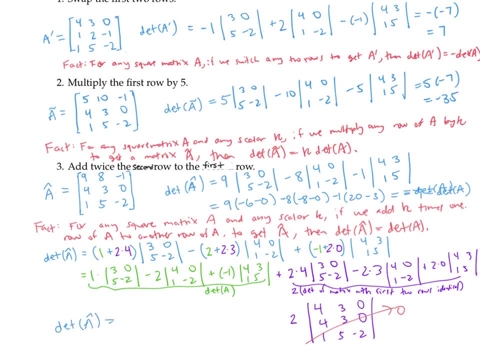 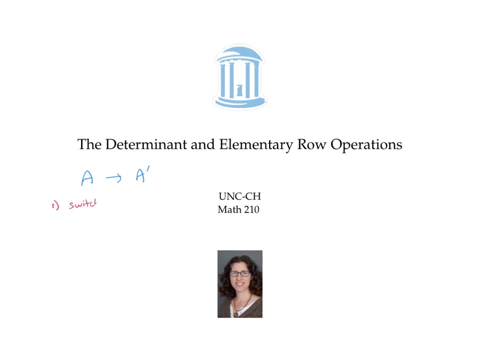 just the determinant of the green part, that's the determinant of a plus zero. In other words, determinant of a hat is equal to the determinant of a. In this video we looked at three elementary row operations: switching two rows. multiplying a row by a number. 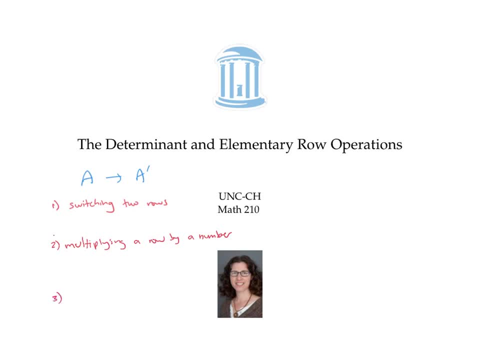 and replacing a row with that row plus a multiple of another row, We found that the third elementary row operation doesn't change the determinant at all. The second one multiplies the determinant by that number And the first row operation switching two rows multiplies the determinant. 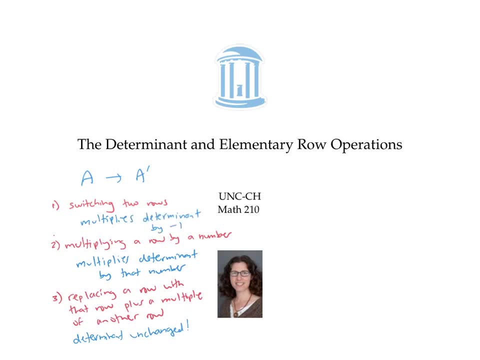 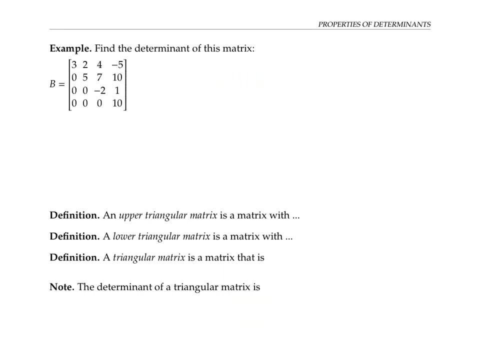 by negative one. We also saw that the determinant of a matrix with two identical rows is zero. This video gives some properties of determinants. I'm going to start with this warm up example. See if you can figure out the determinant of this four by four matrix. One hint is you might want to expand along a row or column. 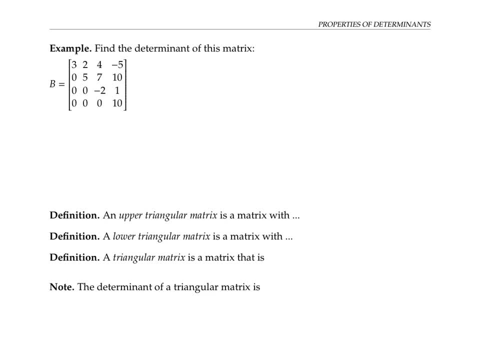 that has a lot of zeros to make your life easier. So I think I'll expand along the first column. then the determinant of B is going to be three times the determinant of this three by three sub matrix minus zero times the determinant of this three by three sub matrix plus zero times this three by 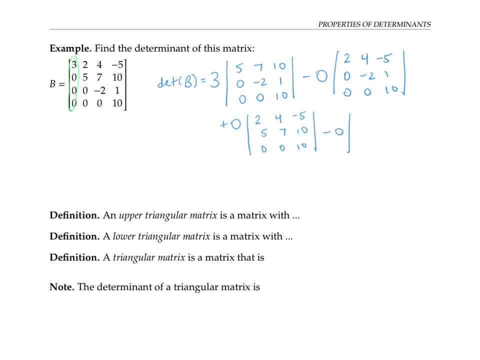 three determinant minus zero times this last three by three determinant. Well, I was kind of wasting my time even writing down all these three by three determinants, because zero times anything is going to be zero. So these last three terms are all just zero And the determinant of B is just three times this. 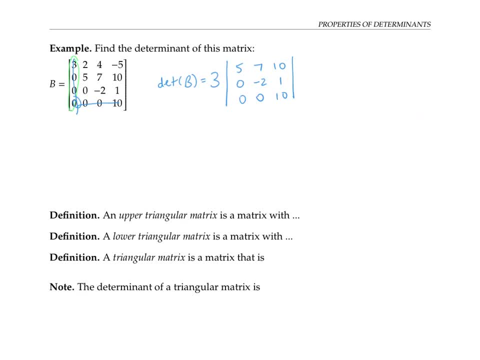 three by three determinant. So continuing. I'm going to figure out this three by three determinant by expanding along its first column, since it has a lot of zeros in it. So let me carry the three and now start expanding. So that's five times a two by two determinant. 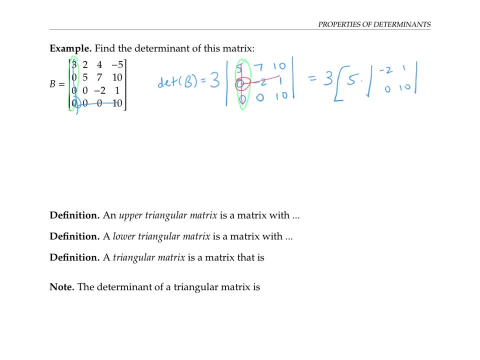 So now I'm going to have a two by two determinant with a plus zero time something, plus zero times something. So those drop out and I just have the three times, the five times that two by two determinant. Finally, I can calculate the two by two determinant as just negative. 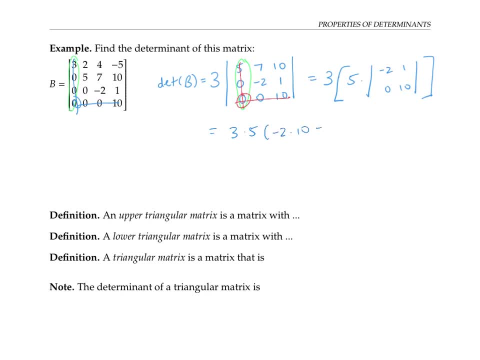 two times 10 minus zero, So I'm ultimately getting three times five times negative, two times 10.. That's negative 300.. But, more interestingly, my determinant is just the product of these entries on the diagonal, And that's no coincidence. that came directly out of expanding along. 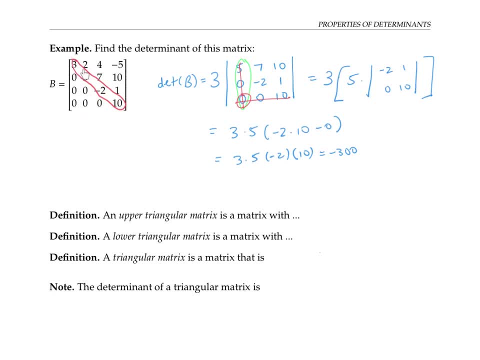 this column with almost all zeros to just get that three times the term of here, and expanding this gives us the five times the term of this, and expanding this gives us the negative two times 10.. So this is an example of an upper triangular matrix And upper 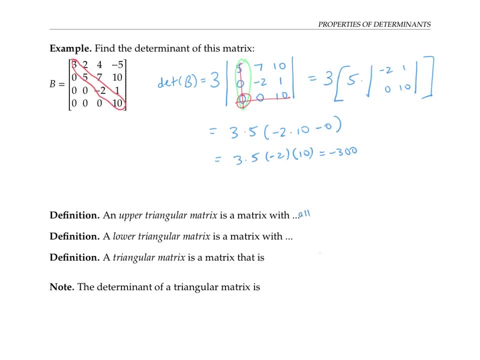 triangular matrix is a matrix with all entries zero below the diagonal. Similarly, a lower triangular matrix is a matrix with all entries zero above the triangle diagonal. I guess the upper triangular refers to the fact that it's only the only non zero entries are in the upper triangle, including the diagonal, and the lower triangular is. 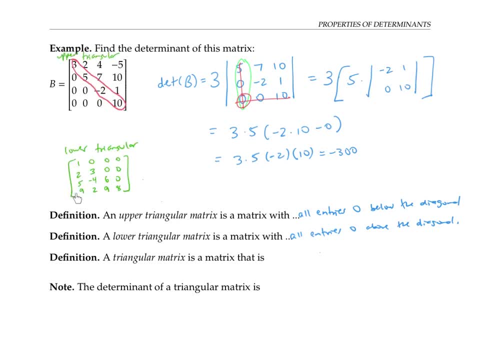 something like this, whose only nonzero entries are in this lower triangle. So a triangular matrix is a matrix that is either upper triangular or lower triangular And, as we saw above, the determinant of a triangular matrix is just the product of its entries on the diagonal. That makes a triangular matrix one whose determinant is: 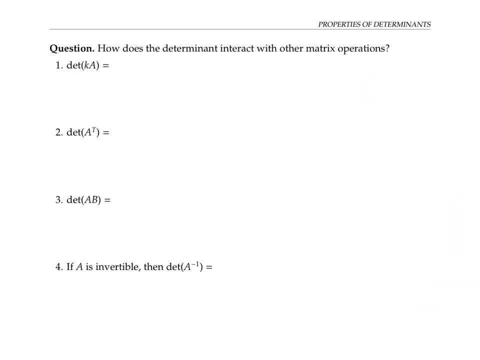 super easy to compute. Now let's go on to our main topic for this video, which is how the determinant interacts with other matrix operations. So let's let A and B, the n by n square matrices and the determinant of q. A transpose the Q times xi, the C, the d ohms, and let's take 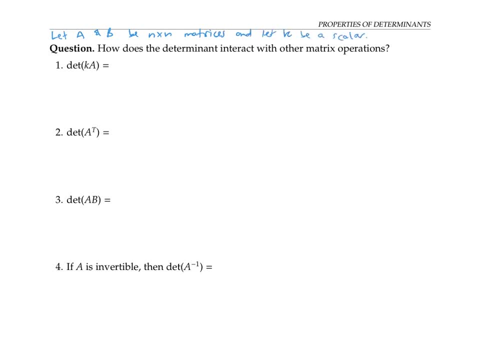 an exponential. cứ cal už diagonal, And let's let K be a scalar. Please pause the video and see if you can come up with any. we'll use for the determinant of K times a. determinant of A. transpose the determinate of A times b. 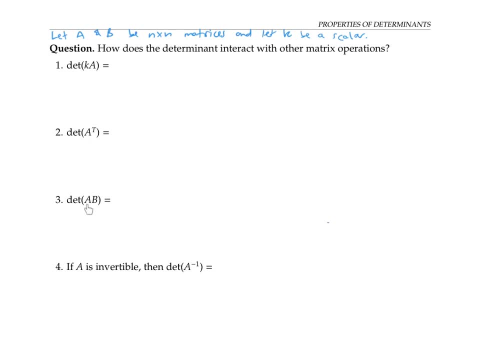 and the only determinant of a inverse for an invertible matrix, determinant of A and B. you might want to write down some example matrices and work out some examples. We saw in a previous video that if we multiply one row of A by k, then 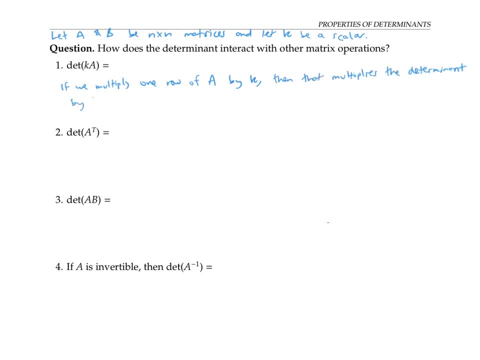 that multiplies the determinant by k. Well, if we're multiplying the whole matrix a by k, that's like multiplying the first row by k and then multiplying the second row by k and all the way through the end row by k. So that should multiply the determinant. 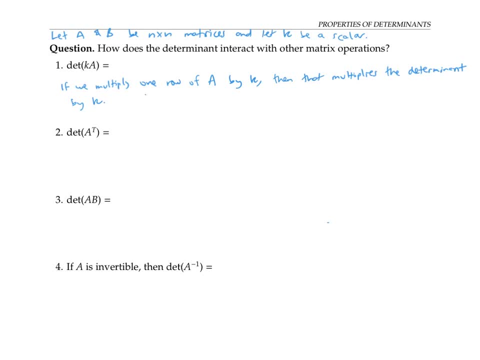 by k, n times. All right, three dots for, therefore, the determinant of k a is going to be k to the n times the determinant of A, where n is the number of rows, Okay, of a, also the number of columns, and say a square. What about the determinant of A transpose? 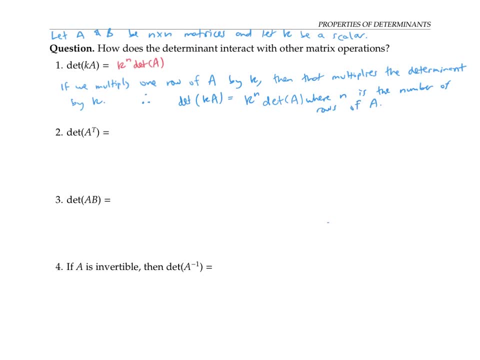 compared to the determinant of A. if you think it should be the same as the determinant of A, you're correct. Certainly it's true for two by two matrices. The crisscross product is the same for the matrix and for its transpose. But if we look at a three by three matrix, 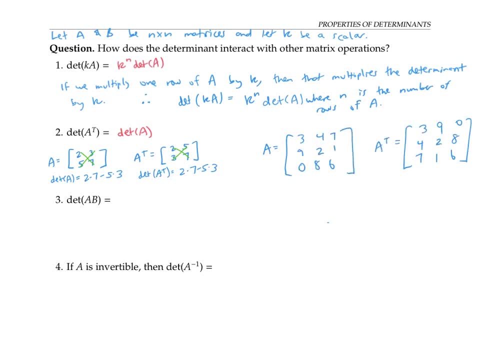 and it's transpose, then Evaluate, Evaluate, Evaluating the determinant of a by expanding along the first row and evaluating the determinant of a transpose by expanding along the first column, gives us two expressions with the same coefficients here: three negative four and seven, and two by two matrices that are the. 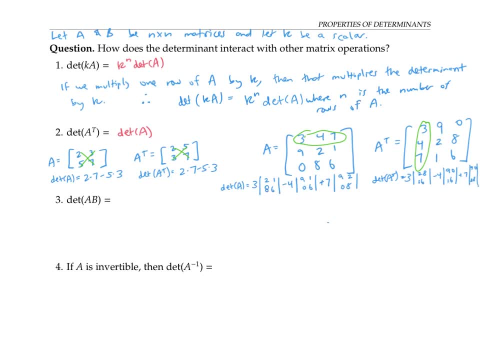 transposes of each other and therefore have the same determinants. And so, therefore, the determinant of a and the determinant of a transpose must be the same. it's the same. computation And inductive argument like that, going up one dimension at a time, will show us that determinant of A and A transpose is also the same. for. 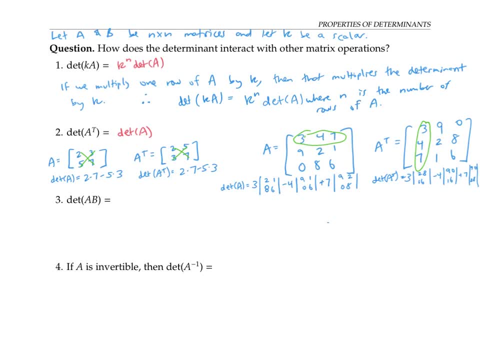 a four by four matrix, or a five by five matrix or any n by n matrix. What about the determinant of A times B? if you worked on an example, you might have noticed that it equals the determinant of A times the determinant of B. 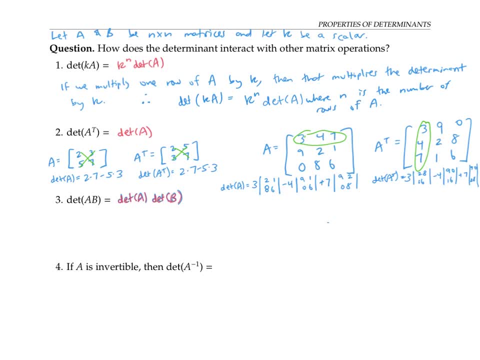 This fact is a little tricky to prove in general, But it's not hard to prove, say, for upper triangular matrices. If you work out what happens when you multiply two upper triangular matrices, you'll see that you get another upper triangular matrix And in addition, 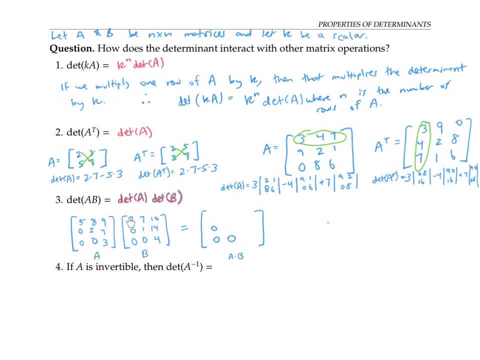 the entries on the diagonal are just the product of the diagonal entries. For example, this entry here where I multiply this row and this column because of these two zeros that hit the eight and the nine. I'm just going to say that the diagonal entries are the product. 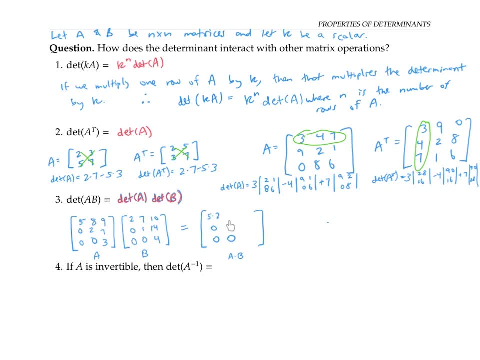 of the diagonal entries, I'm just going to get five times two. Similarly, in this entry that comes from the second row of A times the second column of B, I'm just going to get two times one, since the zero times the seven and the seven times zero are both zero. 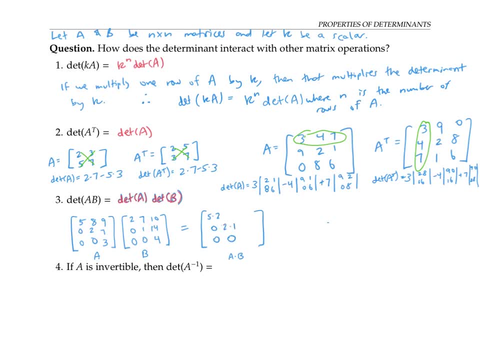 Similarly, this entry here is three times four, And I might get other horribly messy stuff in these positions, But I'm not worried about that because it doesn't affect the determinant. Now we can see that since the determinant of A is the product of its diagonal entries, 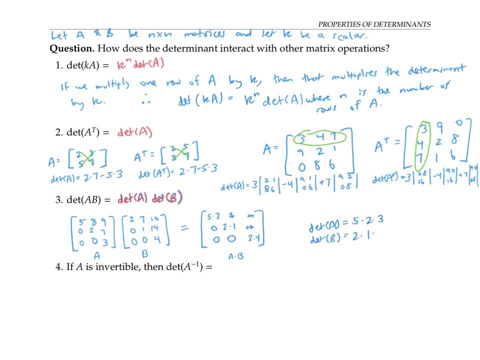 and the determinant of B is the product of its diagonal entries. the determinant of A times B is the product of its diagonal entries. That ends up just being the diagonal entries of A times the diagonal entries of B, or the determinant of A times the determinant of. 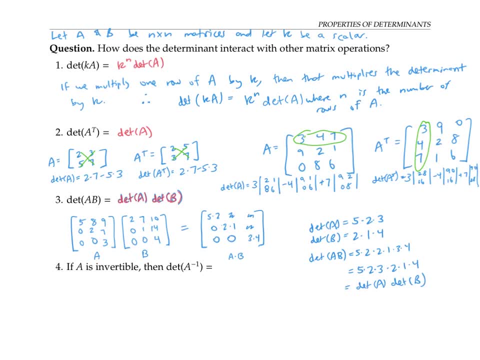 B. So the fact that the determinant of A times B is the term of A times the term of B seems to work, at least for upper triangular matrices, And in fact it turns out to work for all matrices. Finally, if A is invertible, how does the determinant of A inverse compared? 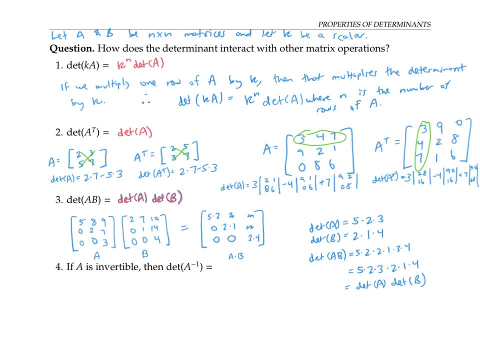 to the determinant of A. Well, we know that A, being invertible, means that A times A inverse is the identity matrix and A inverse times A is the identity matrix Using the. A inverse is the identity matrix Using this multiplication property above the determinant of A inverse times A is the 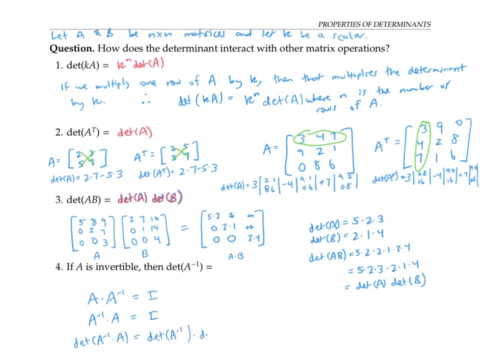 same as the determinant of A, inverse times the determinant of A, But that has to equal the determinant of I, And since I is just a triangular matrix with zeros, it's actually both upper triangular and lower triangular, But in any case it's determined as just the 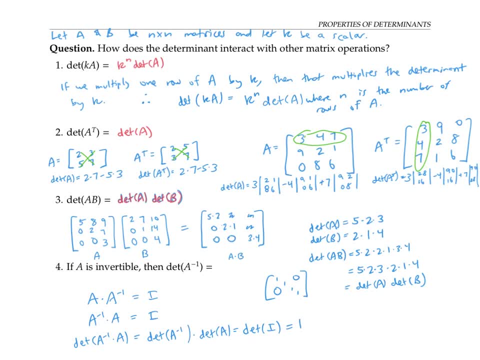 product of its diagonal entries, which is one. Therefore we can solve for determinant A. If you're worried that you might end up dividing by zero here, you don't have to. if A is invertible, the determinant of A can't be zero. it can't be zero because its product with something. 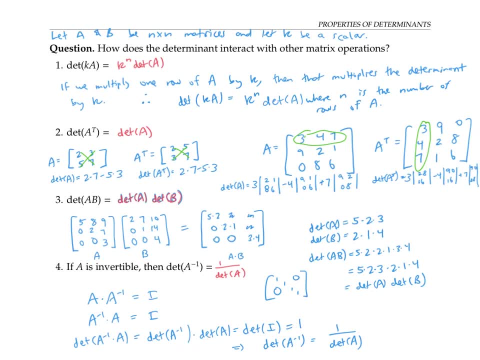 else has to be one. you might notice that I haven't put anything on this list about the determinant of A plus B. That's because there's no relationship between determinant of a sum And the determinant of the two pieces. Let's talk some more about invertible matrices and 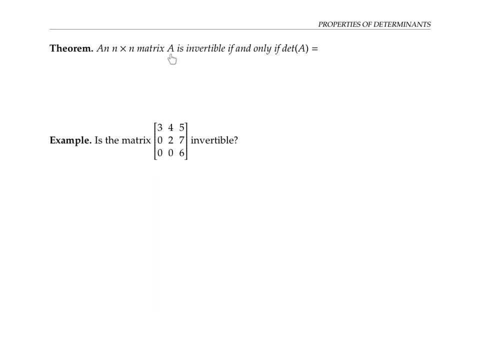 their determinants. We just saw that if a matrix A is invertible, then its determinant is not equal to zero. In fact, this is an if and only if statement. So if it's invertible, then the term is not zero, And if the term is not zero, then the matrix is invertible. 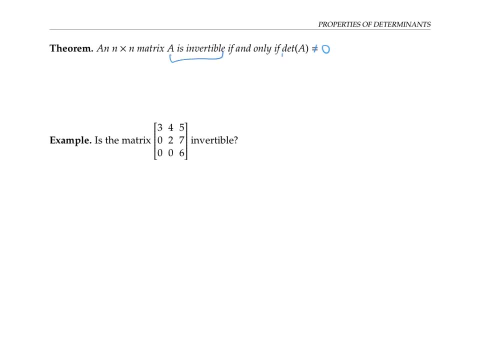 These two conditions: a being invertible and a determinant of a being not zero or equivalent. let's use this equivalence of conditions to check if this three by three matrix is invertible. If we look at the determinant, we can calculate it pretty quickly, Since this is an upper. 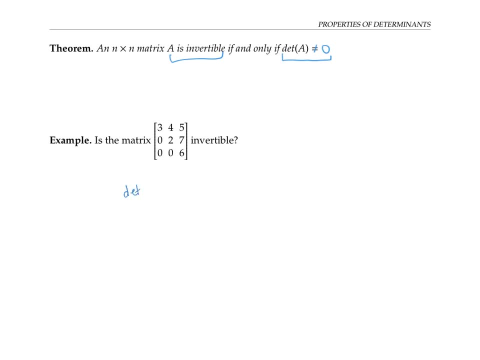 triangular matrix. the determinant of this matrix is the product of its diagonal entries three times two times six or 36.. Which is not zero. Therefore, the matrix is invertible. In this video, we found that the determinant of a triangular matrix is the product of its 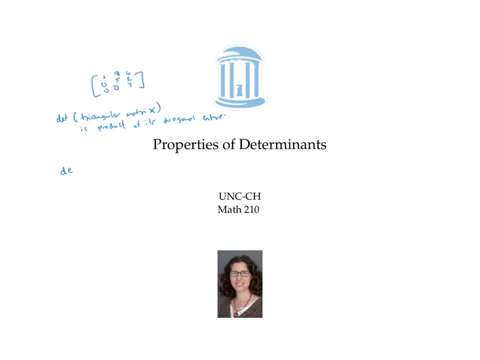 diagonal entries, we found ways to relate the determinant of a matrix A to the determinant of a scalar multiple, of a determinant of A transpose and the determinant of A inverse, if A is invertible. This video also stated the fact that a matrix A is invertible if, and only if, its determinant 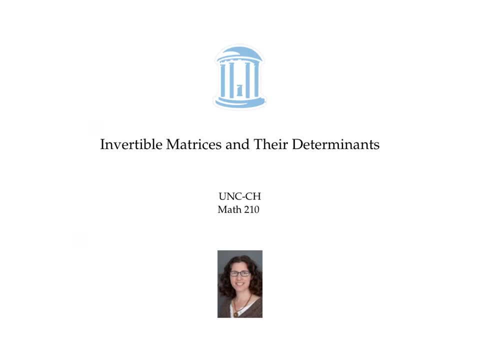 is not zero. Remarkably, it's possible to tell if a matrix is invertible or not just by calculating its determinant. If a square matrix, A, has a determinant that's not zero, then a is invertible. If, on the other hand, the determinant of A equals zero, then A is not invertible. 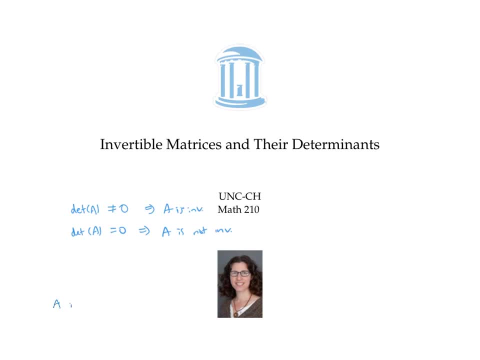 Another way to say this is that a square matrix, A, is invertible If, and only if, the determinant of A is not zero. These two conditions, a being invertible and the determinant of A being nonzero, are equivalent. The purpose of this video. 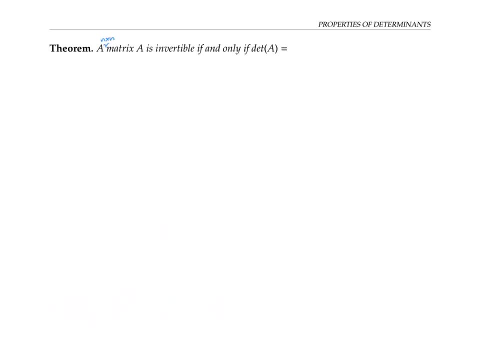 Is to give a proof of this fact. Let's prove the statement that an n by n matrix, A, is invertible if, and only if, its determinant is not equal to zero. To do this, we need to prove first that if A is invertible, then determinant of A is. 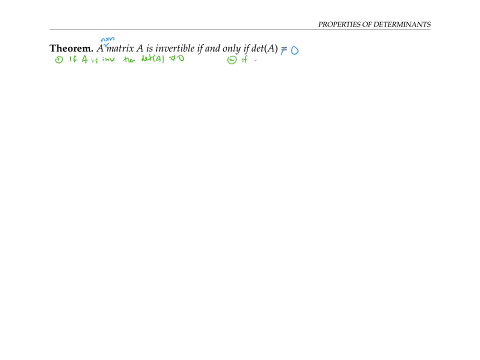 not zero. And second, if determinant of A is not zero, Then A is invertible. Let's focus on this first statement. first, If A is invertible, then we know there's an inverse matrix, A inverse And A times A inverse is the identity matrix. 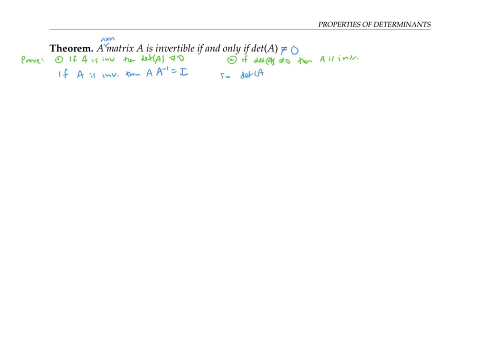 But that means that the determinant of A times A inverse is equal to the determinant of the identity matrix. But the determinant of I Is just equal to one. That's because the identity matrix I has a bunch of ones down the diagonal and zeros and all the other places. 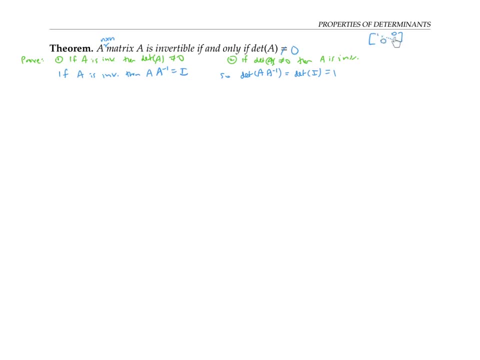 So the identity matrix is an upper triangular matrix. it's also a lower triangular matrix, And we know that the determinant of a triangular matrix is just the product of its diagonal entries, In this case a product of a bunch of ones, which is one. 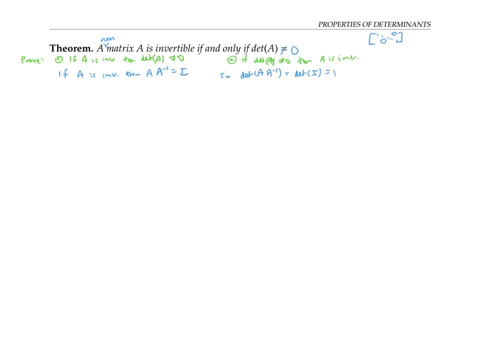 So we have the determinant of A times. A inverse is one, But the determinant Of a product is the product of its determinants. The determinant of A inverse is the same thing as the determinant of A times the determinant of A inverse, And that has to equal one. 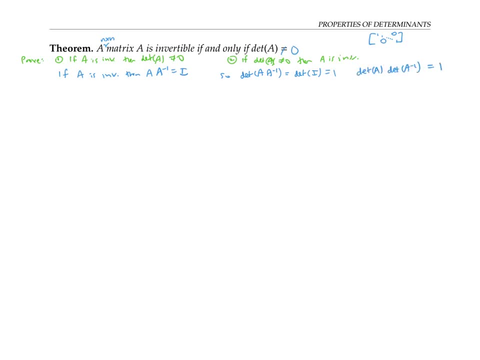 And therefore neither of these two factors can be zero, since you can't multiply zero by something else and get one. In particular, we have that the determinant of A is not equal to zero. That proves the This first statement, And now we need to prove the second statement. 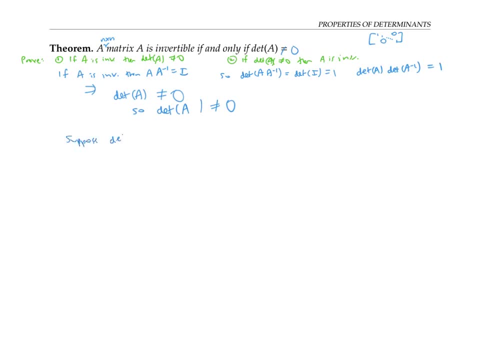 So let's suppose that the determinant of our n by n matrix A is not equal to zero. Let's do some elementary row operations to reduce a, to reduce row echelon form, And I'll call this new matrix a tilde. that is, a tilde is the reduced row echelon form. 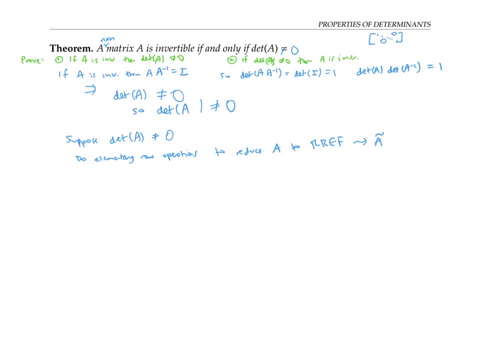 for a. Now we saw in a previous video that elementary row operations change the determinant of a matrix in very predictable ways. Switching to rows of a matrix multiplies the determinant by negative one. Multiplying a row by a scalar k multiplies the determinant by k and finally adding. 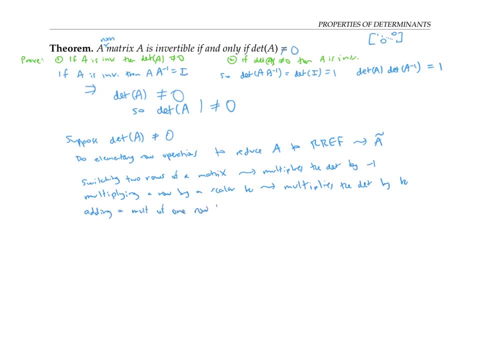 a multiple of one row, Of one row to another row, leaves the determinant unchanged. Well, when we convert a to its reduced row, echelon form a tilde. we perform a series of these elementary row operations. So at each step, we either multiply the determinant by negative one, multiply it by k or leave. 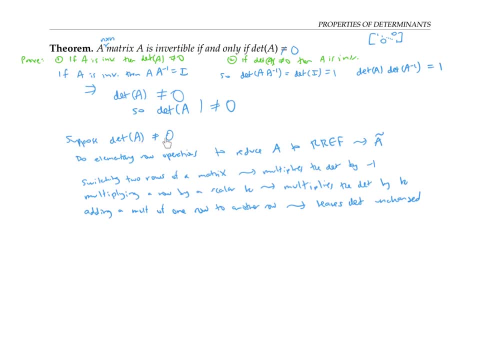 it unchanged. But look at this: we're starting with a determinant of zero. multiply zero by negative one: we still have zero. multiply it by k: we still have zero. Leave it unchanged, we still have zero. Any of these row operations just leaves the determinate at zero. 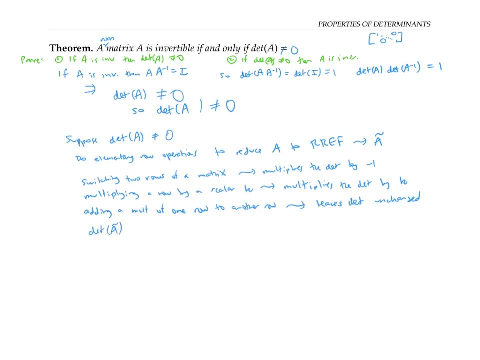 And therefore the determinant of a tilde. our reduced row echelon form version of a must be zero. In particular, this shows that a tilde is not the identity matrix. Since the identity matrix is not the identity matrix, Now let's re-example this. 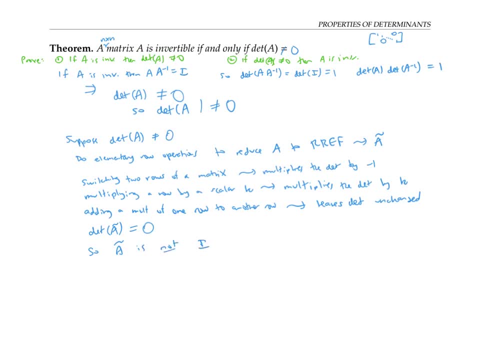 identity matrix would have a determinant of one, And we've seen before that this means that a is not invertible. If it were invertible when we reduced it to reduce row echelon form, we would definitely get the identity matrix. So we've proved that if the determinant of 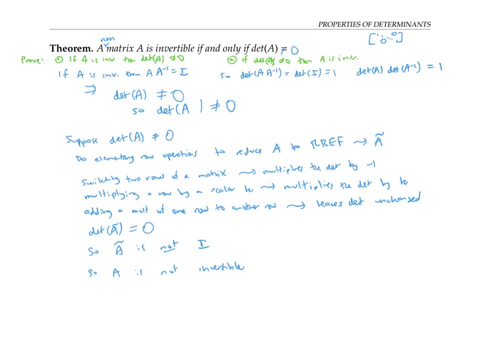 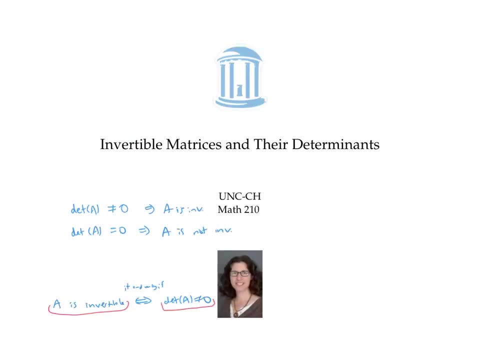 a is nonzero, a is invertible, And that completes the proof of the equivalence of a being invertible and the determinant of a being nonzero. In this video, we proved that a is invertible if, and only if, the determinant of a is not zero. being invertible and having a nonzero, 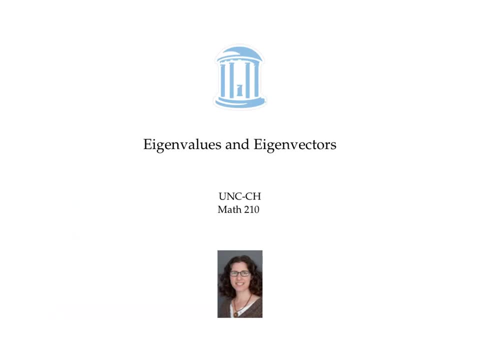 determinant or equivalent conditions. eigenvalues and eigenvectors of matrices have many applications, including to data analysis, where they can be used to simplify and make sense of a multi dimensional data set. This video will define eigenvalues and eigenvectors and explain how. 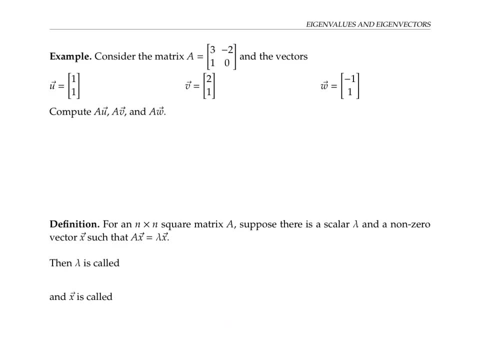 to complete them. Consider the two by two matrix given here and the two by one vectors u, v and w. Please pause the video for a moment and compute a times u, a times v and a times w And see if you notice anything interesting. To compute a times u, we need to multiply our matrix. 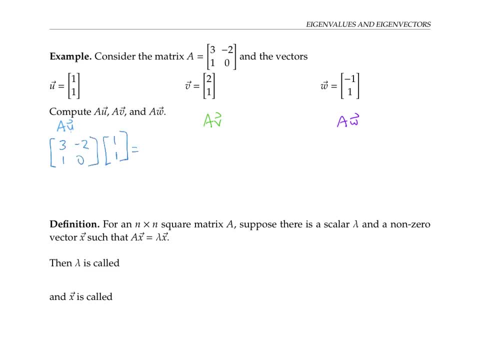 by the vector one one. The result is 11.. Now that's a little weird. We multiplied by this vector u and we got back the same vector u. In other words, a times u is equal to u. Let's see what happens when we do a times V. 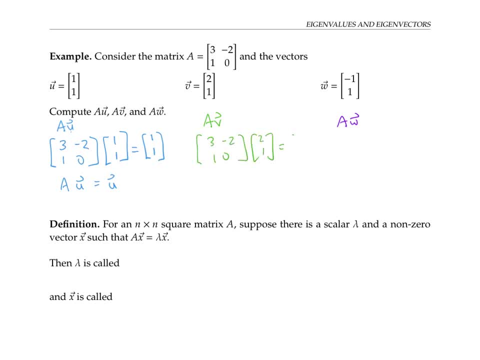 This time we get an answer of for 2.. So when we multiplied by v, we didn't get v back again, But we did get two times v, Because four is twice two and two is twice one. So we have that a times v is twice v. Does that? 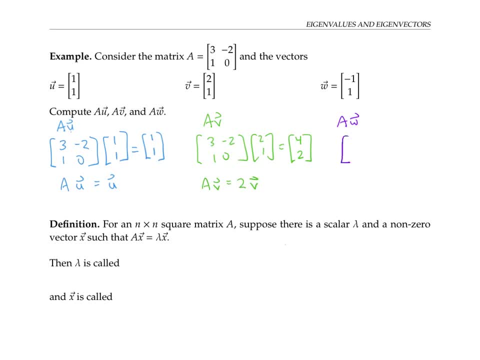 happen for all vectors. Let's try a times w This time our answer: negative. five negative one is not a multiple of the vector w that we started with. So u and v are special vectors for a and that they're stable under multiplication by a. we'll give them a special name. they're. 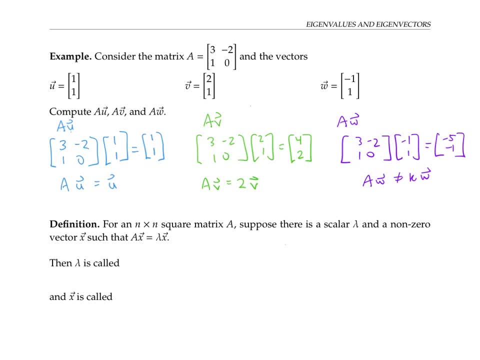 called eigenvectors for a. I'll explain what this means more precisely in the following definition: For an n by n square matrix a, suppose that there's a scalar lambda and a nonzero vector, x, such that a times x equals a. 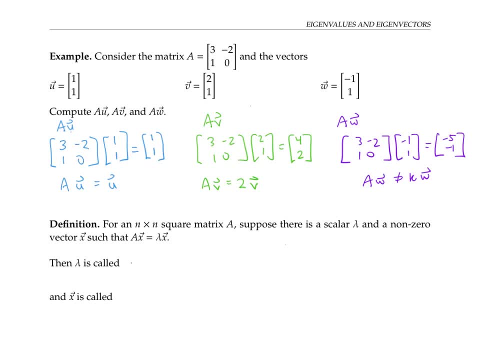 equals lambda times x, then lambda is called an eigenvalue for a and x is called an eigenvector. In the above example we had that a times u was equal to u. I'll write that as a times u equals one times u. And we also had that a times v is equal to two times v, So one. 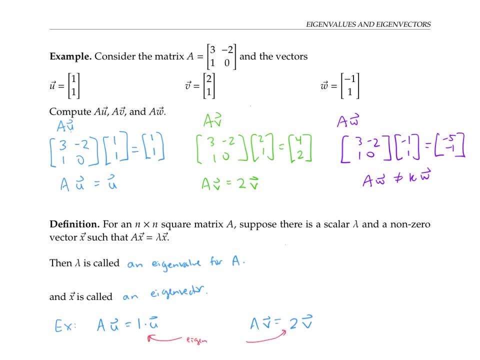 and two, And two are eigenvalues for a And u and v are the corresponding eigenvectors. I want to emphasize that in this definition of eigenvalues and eigenvectors, we need the vector x, the eigenvector, to be nonzero Lambda. the eigenvalue can be zero or a nonzero number, But x is. 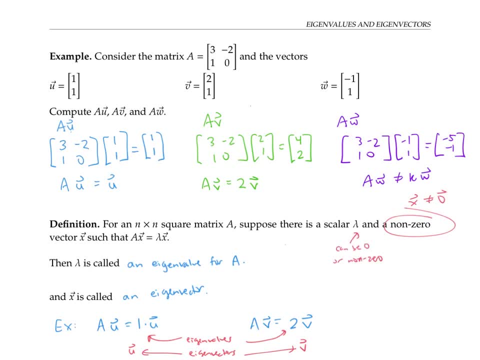 the nonzero number, And so the matrix a can be any matrix a, but x cannot be the zero vector. If x were allowed to be the zero vector, that would kind of be like cheating, because the zero vector is always going to work If you multiply any matrix a by the zero vector. 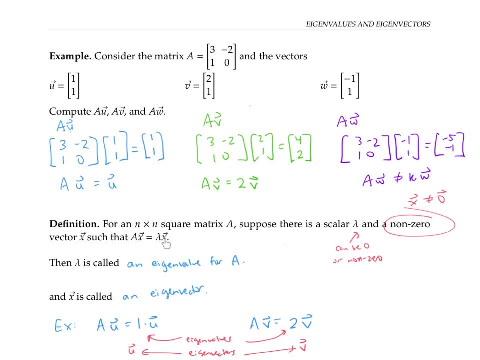 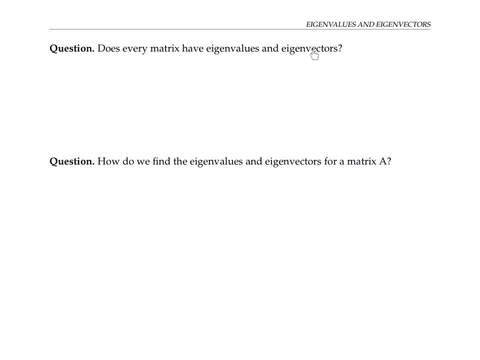 you get the zero vector. if you multiply any lambda by the zero, you actually get the zero vector. So that wouldn't be anything interesting. So does every matrix have eigenvalues and eigenvectors? Is there always some scalar lambda and some nonzero vector x, such that 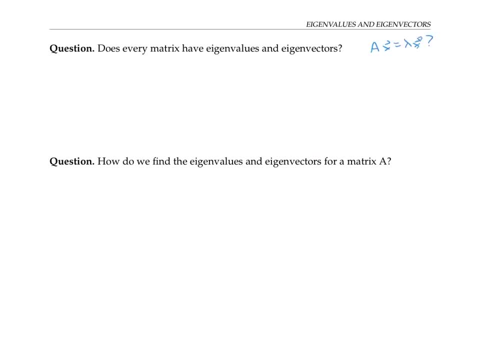 x equals lambda x. Well, if we allow for complex numbers as lambdas, numbers with eyes in them as lambdas, then it turns out the answer is yes. But if we're only interested in real eigenvalues, as we will be in this class, then the answer is no. For example, consider: 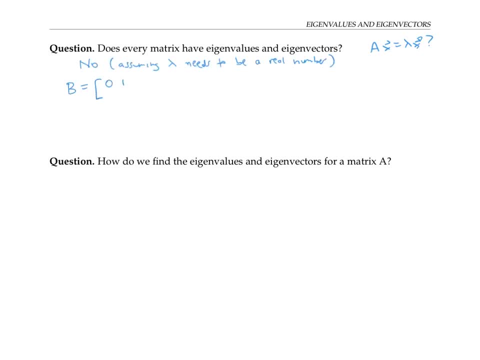 this matrix B with entries 01 negative 10.. If B did have an eigenvalue and an eigenvector, in other words, if there's some x vector such that B times x is lambda times x, then that would mean 01 negative 10 times. I'll write the components of x as x one x two would equal. 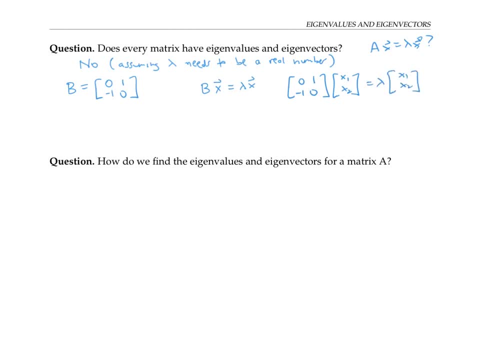 lambda times this vector with components x, one, x two, carrying out the multiplication on both sides of the equation. on the left side we get- let's see this: row times this column is just x two And this row times the column is negative x one. So on the left side we get this vector. 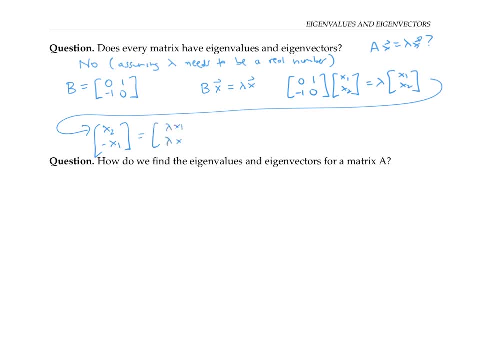 On the right side we get lambda x one, lambda x two. So we would need to have x one x two and lambda satisfy the two equations: x two equals lambda x one and negative x one equals lambda x two If we substitute in x two. 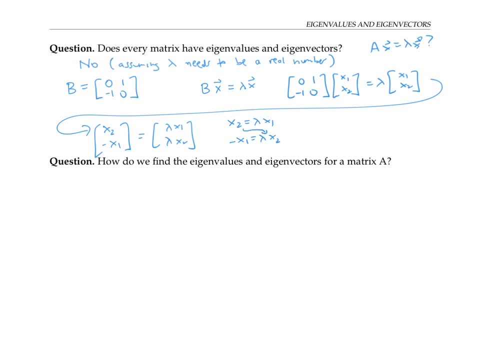 lambda x two, lambda x one from the first equation into x two for the second equation. that gives us minus x one equals lambda times lambda x one. In other words, minus x one equals lambda squared times x one. So that means either x one is zero or if not, we can divide. 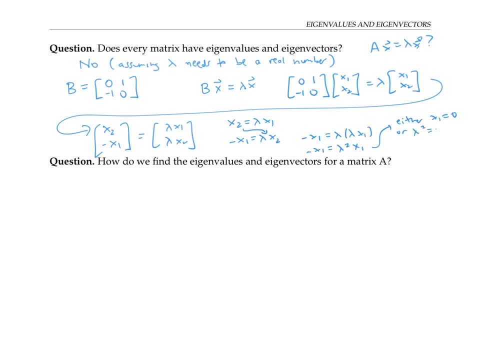 both sides by x one and get lambda squared equals negative one. Well, if we're just looking at real eigenvalues, real numbers for lambda, then x squared cannot equal negative one. there's no real number that you, when you square it, you get a negative number. So x one must equal. 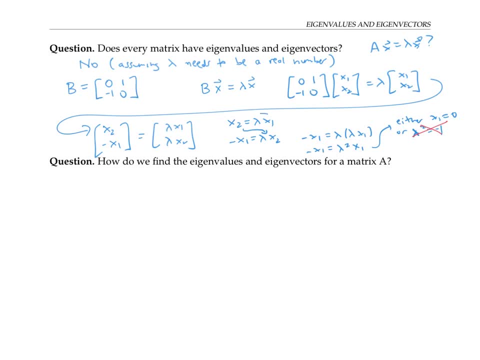 zero. But then, going back to this first equation, that means x two is zero also. So the only way to satisfy this equation is to use a zero vector for x. But as we said before, the zero vector doesn't count as an eigenvector, So we should be able to solve this problem with 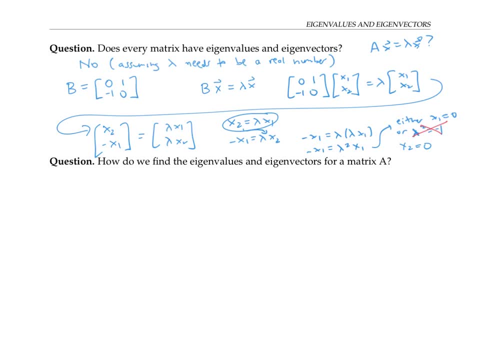 x, but we're going to be doing this later on in the next lesson, So we'll get started. So in fact, there are no eigenvalues and eigenvectors that work for matrix B, But many matrices do have eigenvalues and eigenvectors. So how do we find them Before? 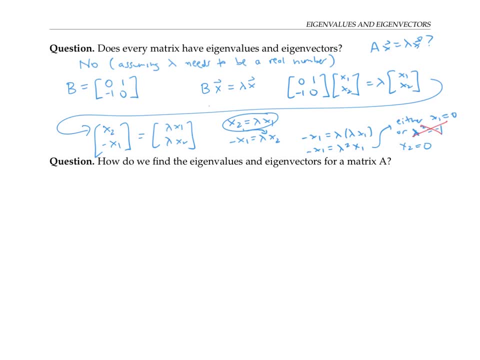 we launch into finding them. I want to remind you of two facts about matrices. First of all, a matrix B is invertible If, and only if, the equation B times the vector x equals the zero vector has no other solutions than x equals the zero vector, which is always going to be a. 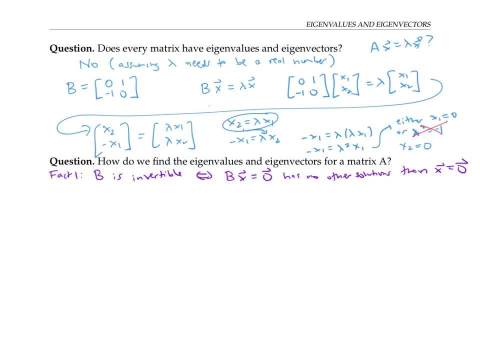 solution to an equation matrix times something equals zero. Since these two statements are equivalent, their negations are also equivalent. So B is not invertible. if, and only if, B- x equals zero- does have other solutions, solutions than x equals zero. In other words, it has nonzero solutions. This is going to be. 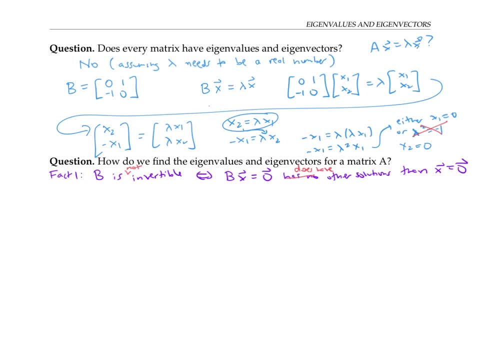 relevant Because when we're looking for eigenvectors, we're also looking for nonzero solutions to an equation. The second fact that I want you to recall is that, be a matrix B is invertible If, and only if, the determinant of B is not zero. Again, we could rewrite this equivalence. 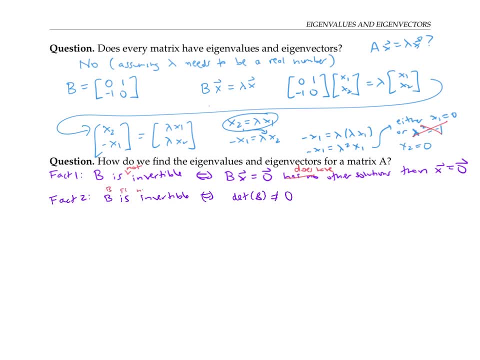 by taking the negations B. B is not invertible if, and only if, the determinant of B is equal to zero. Now let's see if we can figure out how we find eigenvalues and eigenvectors for a matrix A. eigenvalues and eigenvectors correspond to scalars lambda and vectors x that satisfy this equation. 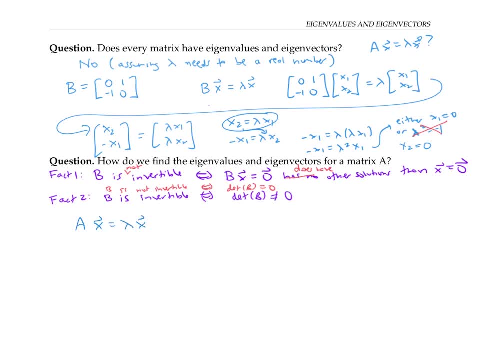 ax equals lambda x. Let's rearrange this equation by bringing everything over to the left side. Now it's tempting to factor out the x and write something like this, But that wouldn't make sense because you can't take a matrix and subtract a scalar from it. 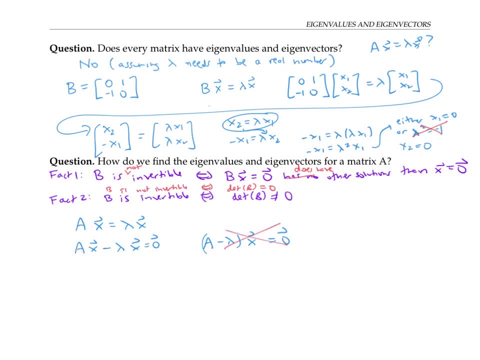 So instead I'm going to rewrite this equation as a times x minus lambda times i times x equals zero, where i is the identity matrix. This equation is the same as the one above it, because i times x is the same thing as x. 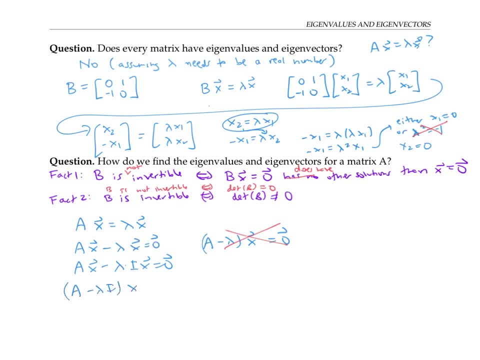 Now it makes sense to factor out the x And to find eigenvalues and eigenvectors for a. we want to find a lambda and a non zero x that satisfy this equation. But fact one says having a non zero solution to an equation of the form B, x equals zero. 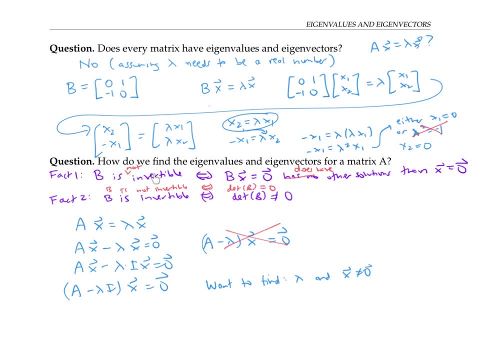 If the equation B equals zero, the matrix B is not invertible. So letting a minus lambda i play the role of b, finding a non zero solution to this equation happens if, and only if, a minus lambda i is not invertible. Now let's look at fact two. 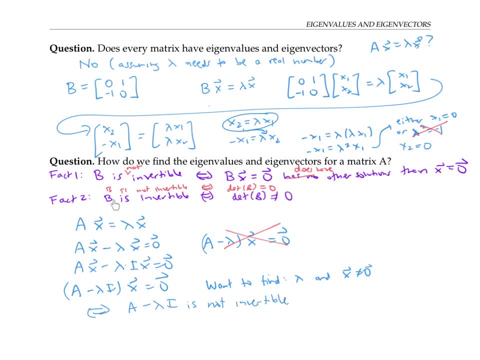 Fact two says a matrix B is not invertible if and only its determinant is può. The rule is neither $ from B to B to dz is zero. So having this matrix A minus lambda i being not invertible, is equivalent to the determinant of A minus lambda i equaling zero. So we'll be able to find eigenvectors solutions. 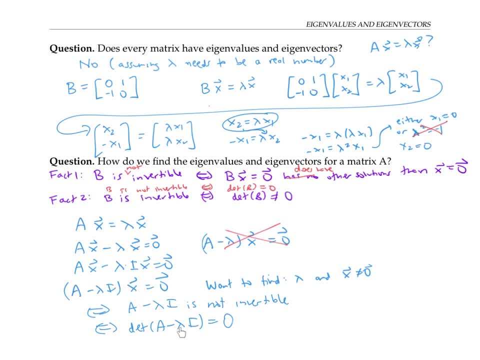 to this equation exactly for those values of lambda that make the determinant of A minus lambda i equal to zero. Now we have a way to find the eigenvalues for a. what we have to do is set the determinant of A minus lambda i equal to zero and solve for lambda Once. 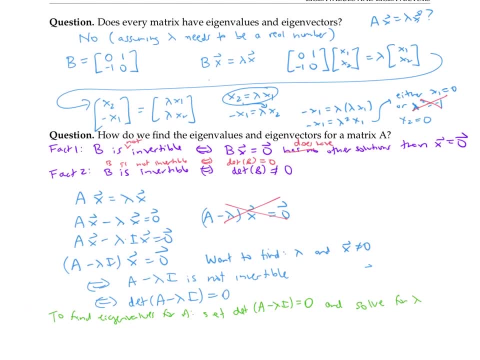 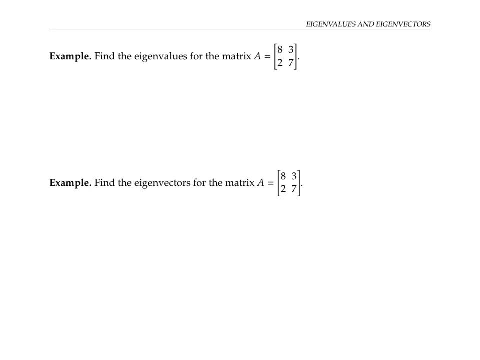 we found the eigenvalues lambda. we can find the eigenvectors by solving this equation for x. Let me show you how this works with an example. So let's find the eigenvalues for this matrix A. what we need to do is we need to figure. 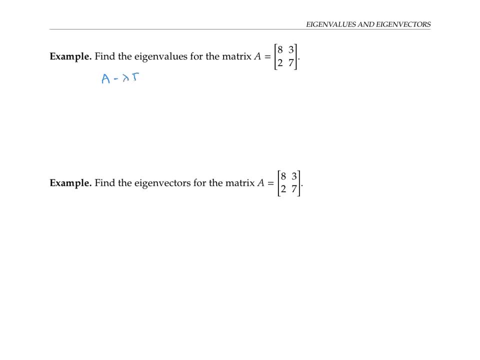 out what lambdas will make. A minus lambda i have a determinant of zero. I'm going to write down A minus lambda i, so that's going to be 8327 minus lambda times 1001.. That needs to have a determinant of zero. I'll rewrite this as: 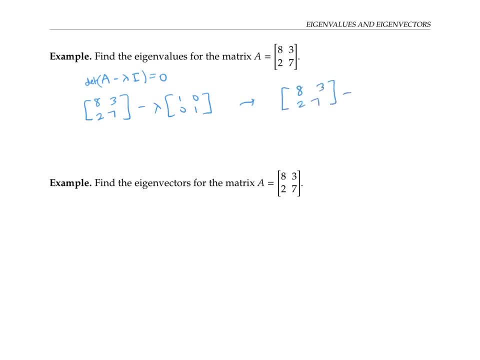 8327 minus lambda, 00 lambda, And I can also rewrite it as eight minus lambda, 327 minus lambda, by subtracting these two matrices, one entry at a time. So I need the determinant of this matrix to be zero. So that means eight minus lambda times seven minus lambda times seven minus. 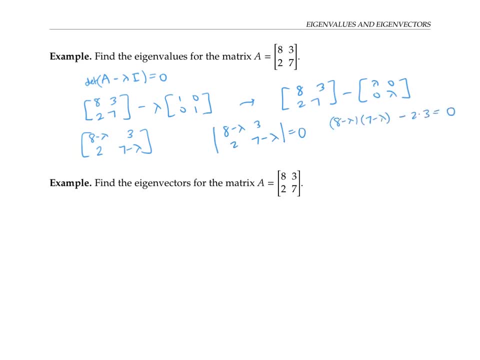 lambda minus two times three needs to be zero. Distributing out, I get 56 minus eight. lambda minus seven. lambda plus lambda squared minus six equals zero. So lambda squared minus 15, lambda plus 50 equals zero And that factors into lambda minus 10, lambda minus five equals. 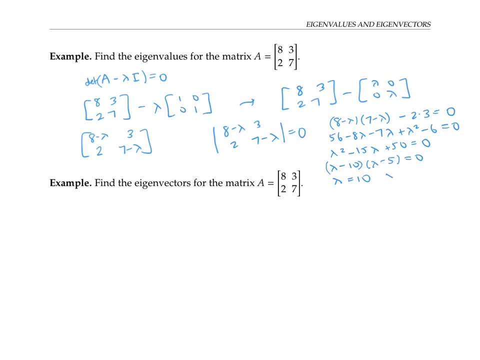 zero. So my eigenvalues are: lambda equals 10.. And lambda equals zero. So lambda equals equal five. now let's find the eigenvectors. So first I'll consider lambda equals 10.. Then I need to solve the equation. a minus lambda i times x equals zero with Lambda equals. 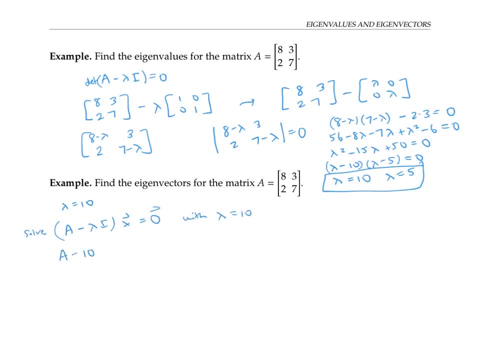 10.. So in other words, a minus 10. I times x equals zero, So let me write that out. So here's a. So here's a, here's 10. I I'll subtract my matrices. So eight minus 10 is minus two, three minus zeros. 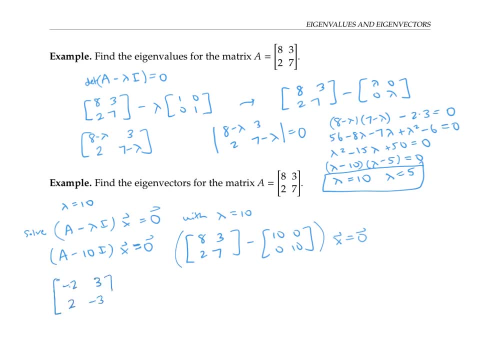 three. two minus zeros. two seven minus 10 is minus three, And I'll write my x in component. Now you might recall that solving an equation like this can be done by writing down the augmented matrix, augmented by the vector on the right side, And converting it to reduce. 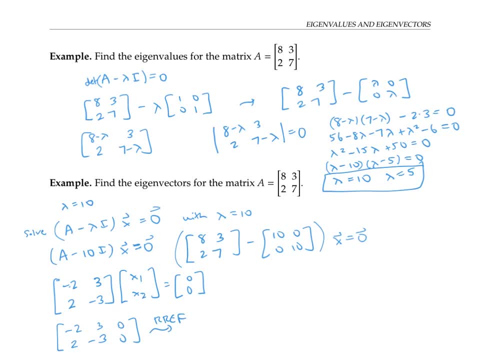 row echelon form. I'm going to do that by adding the first row to the second row and then multiplying the first row by negative one half. Notice that I did not get the identity matrix. when I reduce the matrix to reduce row echelon form, And that's good, That's. 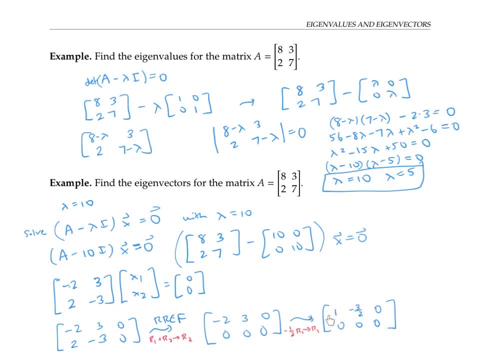 what I expect, Because I expect that the matrix is going to have zero row echelon form. So I'm going expect to get nonzero solutions to this system of equations, and actually lots of them. So to find the solutions, I can set x two to be a free variable, since there's no leading. 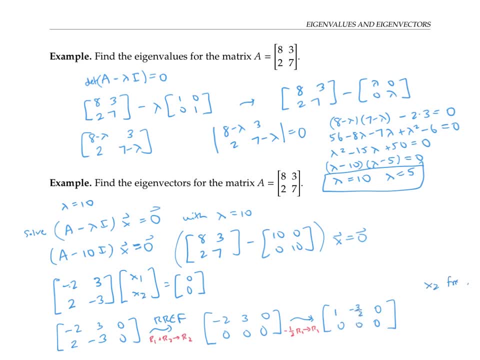 one in the x two position, the x two column, and then I have that x one minus three halves X two equals zero, And so x one is three halves x two. So my solutions are of the form three halves x two, x two, or this can be written as x. 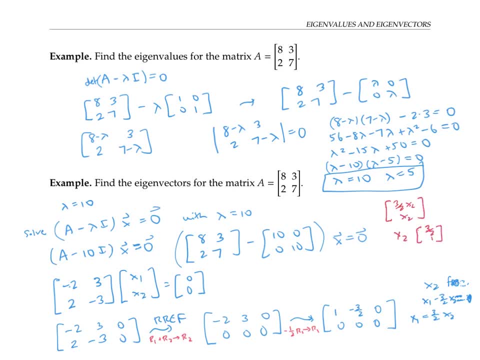 two times three halves one. these are my eigenvectors for the eigenvalue lambda equals 10.. And if I just wanted one eigenvector instead of a whole family of them, I could just pick an easy value of x two like x two equals one. So for example, the vector three halves one is an eigenvector. 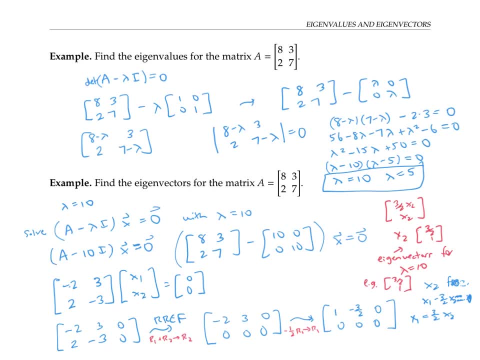 for the eigenvalue, lambda equals 10.. So we're halfway done. Now we need to do the same computation with lambda equals five. In other words, we need to solve the equation a minus five, i times x equals zero. I encourage you to pause the video and try this on your own before. 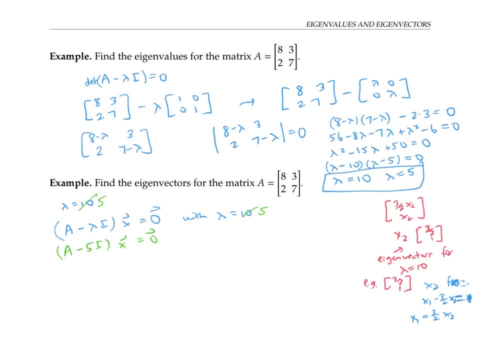 seeing the solution To solve this, I'll write down a minus five. I simplify a little: eight minus five is three. three minus zero is three. two minus zeros to seven minus five is two And I can augment that with the zero vector and convert that to reduce row echelon form. 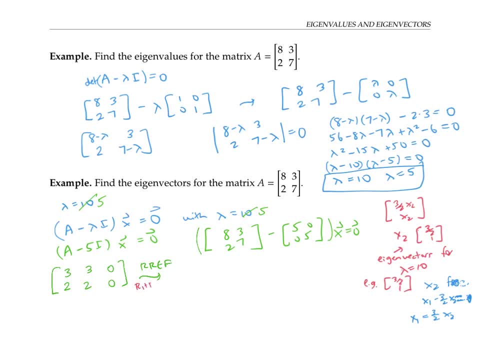 I'm going to add the second row to the first row. Put that in the first row's position. That gives me 110220.. And then I'm going to add negative two times the first row to the second row. That gives me the matrix 110000.. So once again I've gotten in reduced row echelon form and 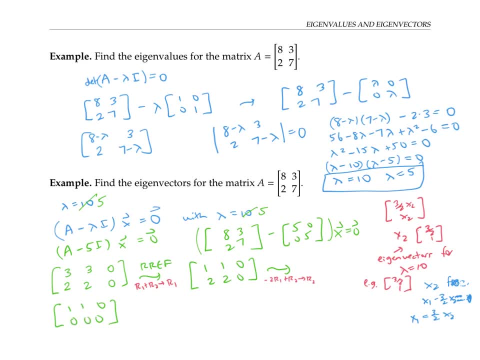 I don't have the identity matrix. I have x two. So I have x two as a free variable And I have x one plus x two equals zero, So x one equals minus x two. So my solution eigenvectors are of the form minus x two, x two, or I can. 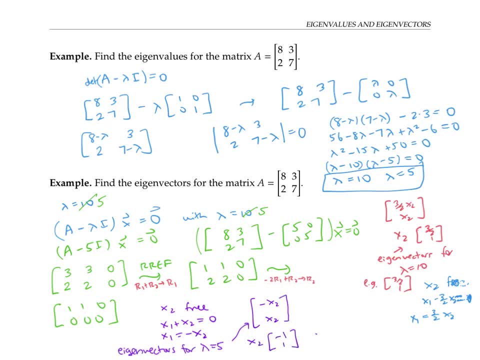 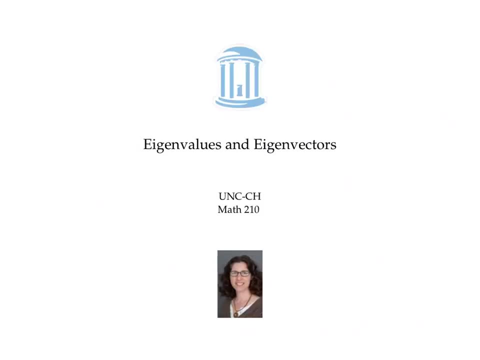 write that as x two times minus one one, And if I want an example I can use minus one one. In this video we found the eigenvalues of a matrix A by setting determinant A minus lambda i, equal to zero, And we found the 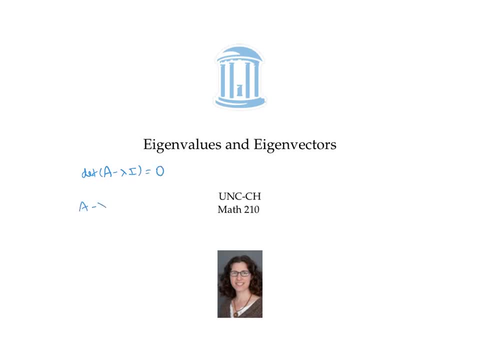 corresponding eigenvectors. by solving the equation A minus lambda i times the vector x equals the zero vector. This expression, the determinant of A minus lambda i, is called the characteristic polynomial of A. This video gives some properties of eigenvalues of matrices. eigenvalues for triangular matrices are especially easy to compute. Let's see what we get when. 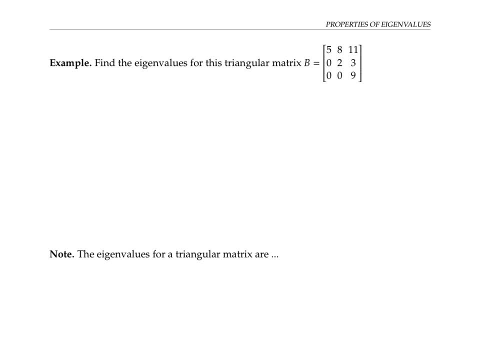 we find the eigenvalues for this triangular matrix B. we can find the eigenvalues for B by computing the determinant of B minus lambda i, setting it equal to zero and solving for lambda, Since the matrix lambda i has lambdas on the diagonal and zeros everywhere. 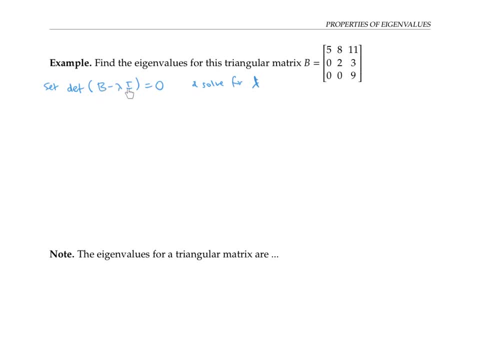 okay, else when we take B and subtract lambda i, we're just subtracting a lambda along each of the diagonal entries. Now we need to take the determinant of this and set it equal to zero. we saw in a previous video that the determinant of a triangular matrix is just 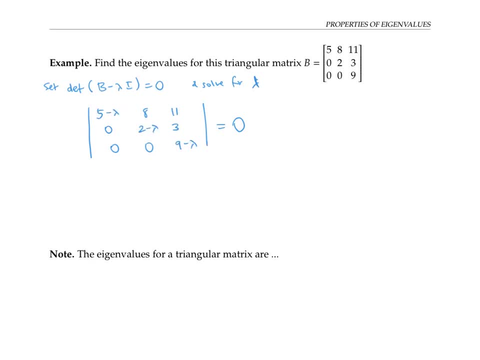 the product of the diagonal entries And since the original B was a triangular matrix, the matrix B minus lambda i is also a triangular matrix. So its determinant is five minus lambda times two minus lambda times nine minus lambda. When we set that equal to zero and solve: 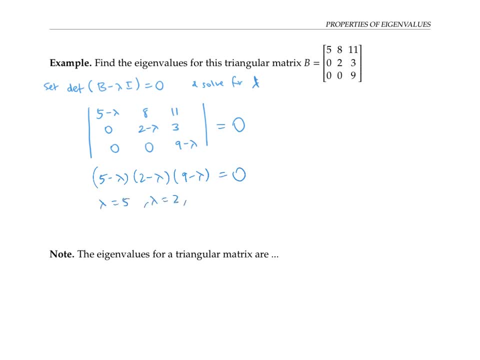 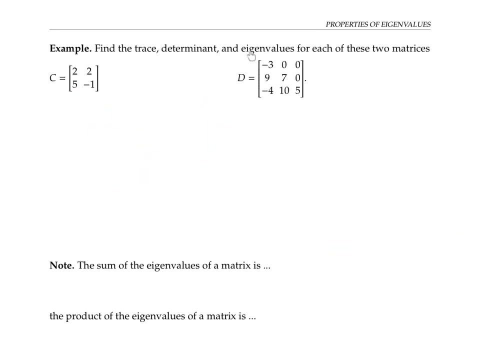 we get that lambda equals five, lambda equals two or lambda equals nine. These are exactly the diagonal entries of B And in general the eigenvalues for a triangular matrix are the diagonal B B entries of the matrix. Next, let's relate the eigenvalues for a matrix to its trace. 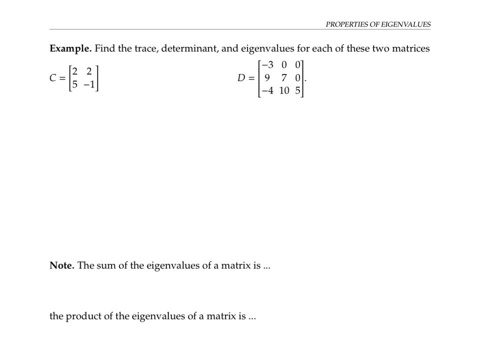 and determinant For this matrix C. the trace of C is two plus negative one, which is one, as determinant is two times negative, one minus five times two, which works out to negative 12.. And then to calculate C's eigenvalues, let's take the determinant of C minus lambda. I So 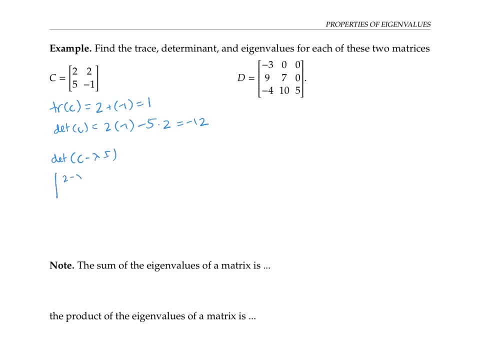 that's equal to the determinant of two minus lambda, two, five minus one minus lambda, which works out to two minus lambda times negative, one minus lambda minus 10.. And we'll set that equal to zero and simplify to get negative: two minus two, lambda plus lambda plus lambda squared minus 10 equals zero. So that means that lambda. 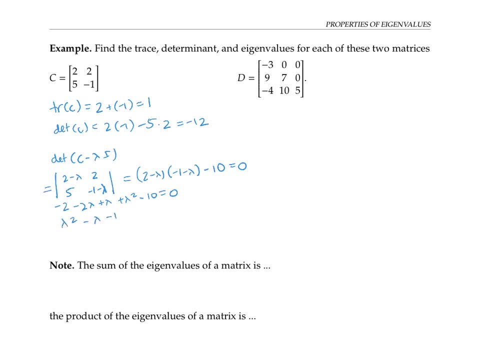 squared minus lambda minus 12 equals zero. we can factor that to get lambda minus four times lambda plus three equals zero. So lambda equals four or lambda equals negative. three are the two eigenvalues. Notice that the sum of these two eigenvalues four plus negative. 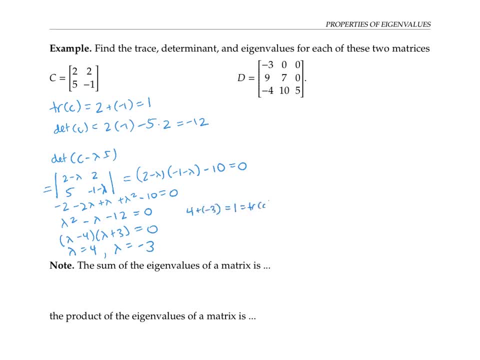 three gives us one, which is the trace of C, while the product four times negative. three gives us negative 12, which is the determinant. Let's see what happens for this three by three. triangular matrix d: We know that the trace of D is the sum of the diagonal entries And 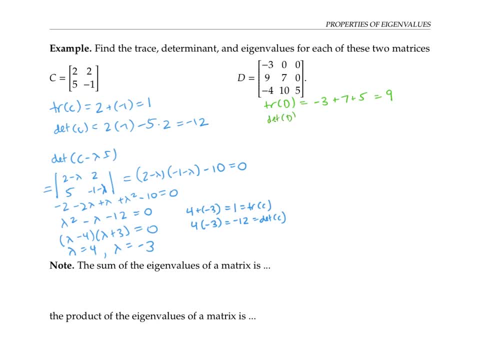 because D is triangular, the determinant of D is the product of its diagonal entries. But as we saw in the consolation제�ector check previous slide, since D is triangular, its eigenvalues are exactly as diagonal entries negative three, seven and five. So the sum of the eigenvalues will be equal to the trace. 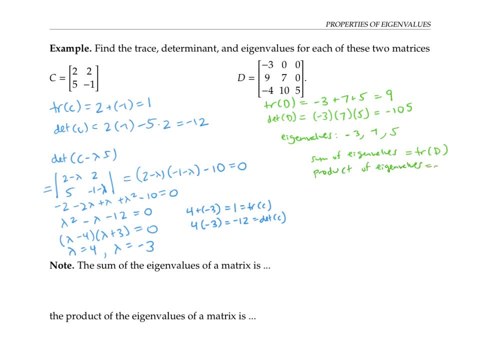 And the product of the eigenvalues will be equal to the determinant. Although I won't prove it here, these facts are true for all matrices, not just two by two matrices and triangular matrix. For any n by n square matrix, the sum of its eigenvalues is equal. 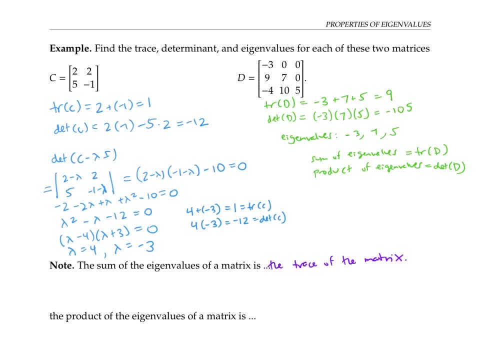 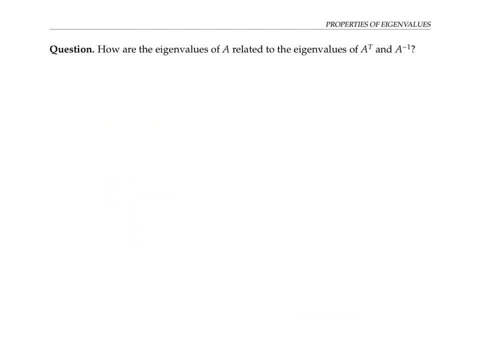 to its trace And the product of its eigenvalues is equal to the determinant. Next let's see how the eigenvalues of A are related to the eigenvalues of A transpose and A inverse. If I want to find the eigenvalues for a transpose, 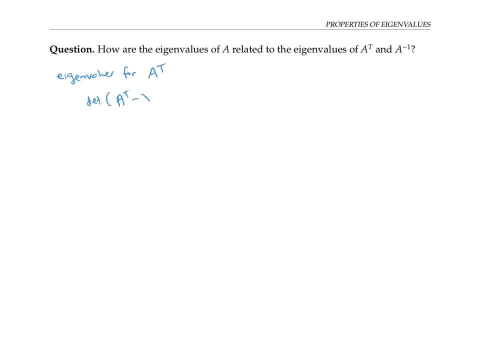 I need to transposed. take the determinant of a transpose minus lambda i and set it equal to zero. The eigenvalues for a transpose are the lambdas that satisfy this equation, But since the identity matrix i is the same as its transpose and in fact lambda times i is the same thing as its transpose, 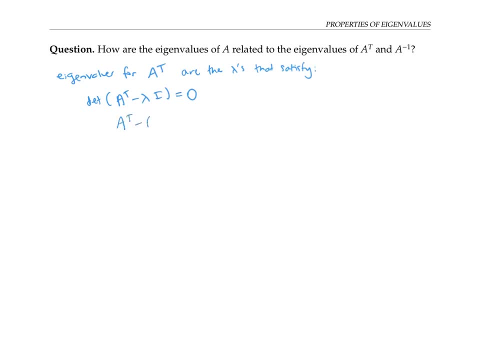 I can rewrite this equation as a transpose: minus lambda: i transpose. Recall that the transpose of a sum of matrices is the sum of the transposes. So I can rewrite this again as the determinant of a minus lambda: i transpose, But recall also the determinant of a matrix. 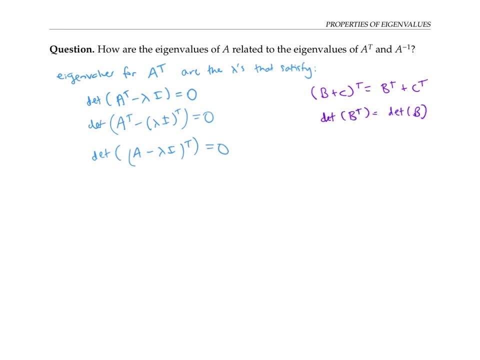 is transpose is the same as the determinant of the original matrix. So I can rewrite my equation as: the determinant of a minus lambda i equals zero, But the eigenvalues of a minus a are the lambdas that satisfy this equation. Therefore, the eigenvalues of a transpose. 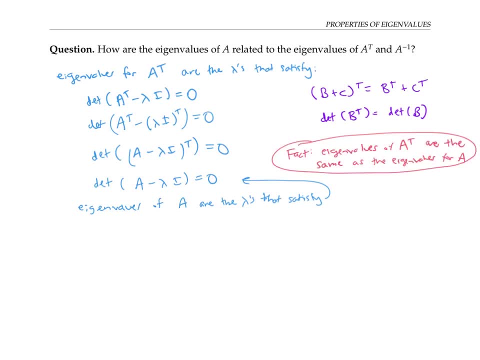 are the same as the eigenvalues of a. Next, let's think about the eigenvalues of a inverse and how they relate to the eigenvalues of a. we know that lambda is an eigenvalue for a with eigenvector X if, and only if, a x equals lambda x, where x is a nonzero vector Multiplying both sides. 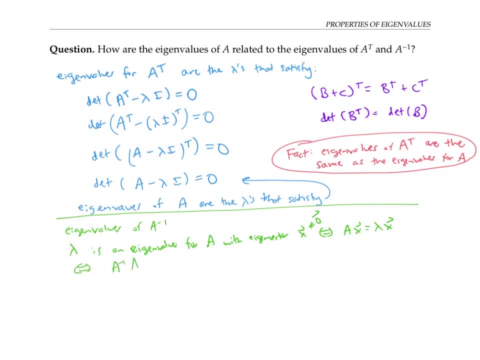 by a inverse. this is equivalent to saying that a inverse a x is equal to a inverse lambda x. Since a inverse times a is just the same as the identity and the identity times x is just x, I can rewrite this left side as just x And the right side. I'll pull the. 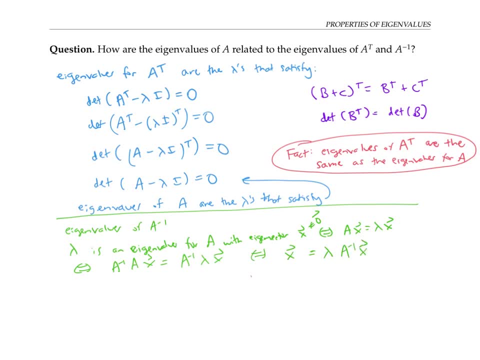 scalar lambda out. Pulling the lambda out is legit, Because if we multiply a inverse by Lambda times x, we get entries that are lambda times as big as if we multiplied a inverse by x. Notice that our lambda cannot be zero, because if it were, this whole right 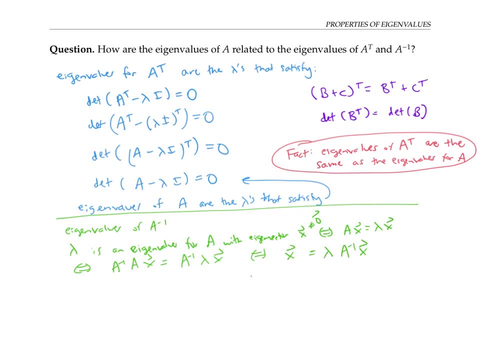 side would be zero and therefore our x vector would be zero And it wouldn't be a legitimate eigenvector. Since lambda is not zero, it's possible to multiply both sides of this equation by one over x, when x equals lambda x, which is equal to x times x, And therefore the 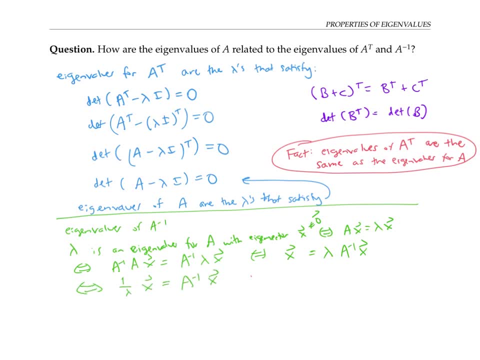 one over lambda. But wait, that's just the equation that x needs to satisfy to be an eigenvector for a inverse with eigenvalue one over lambda. maybe it'll be a little bit more clear if I just switch the order. a inverse x equals one over lambda x. So this is true. 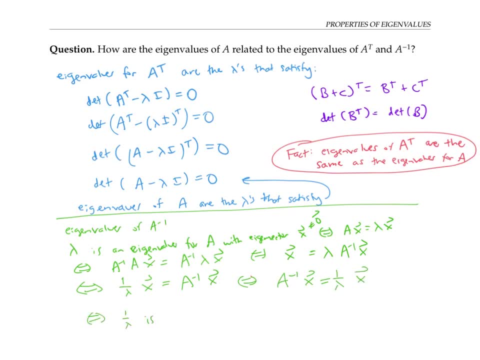 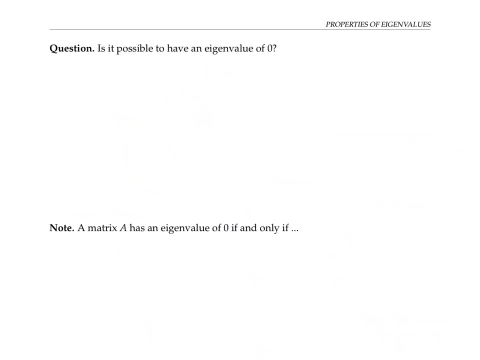 if, and only if, one over lambda is an eigenvalue for a inverse with eigenvector x. So the eigenvalues of a inverse are the reciprocals of the eigenvalues of A And furthermore, the eigenvectors of A inverse are the same as the eigenvectors of A. So is it possible to have an eigenvalue? 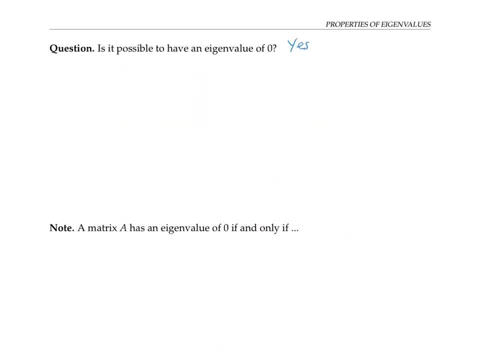 of zero. In fact it is. For example, if we look at the matrix one zero, one zero it zero. then the determinant of A minus lambda i is the determinant of this matrix, which is one minus lambda times minus lambda minus zero. that equation is zero if lambda is. 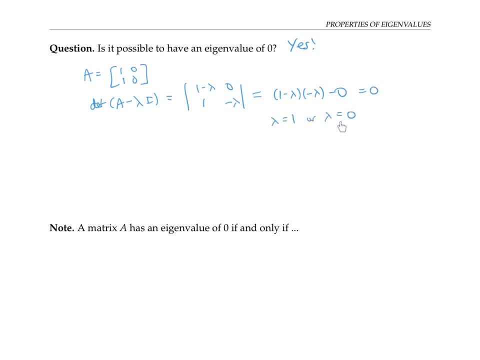 one or lambda, is zero. So we do indeed have an eigenvalue of zero as well as an eigenvalue of one for this matrix, But in fact, this can only happen for non invertible matrices. a matrix A has an eigenvalue of zero if, and only if, A is not invertible. Let me explain. 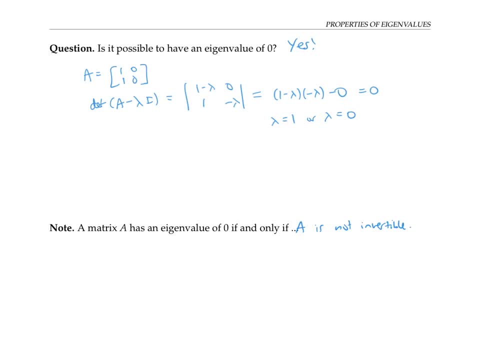 why We saw in a video about invertible matrices that a matrix, A, is invertible if and only if, the equation A x equals zero has only the solution x equals zero. So the negations of these statements are also equivalent. a is not invertible If and only. 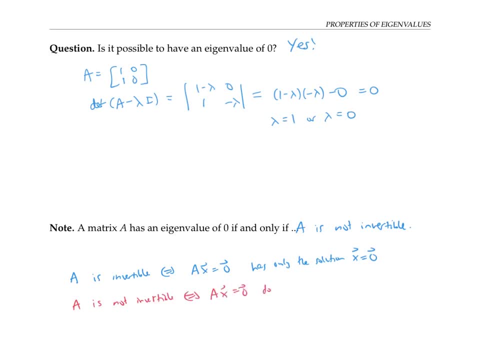 if A x equals zero does not have only one, the one solution x equals zero, x equals zero is still a solution. So this means that there must be some other x. that's not zero, that's also a solution. But the equation A times x is the zero vector. 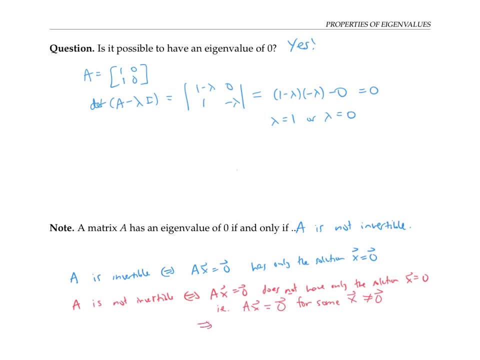 The zero vector is equivalent to saying: a times x is zero times x. since zero times x is the zero vector, That's just the same thing as saying that zero is an eigenvalue for A. So we've shown that A is not invertible if, and only if, zero is an eigenvalue for A. 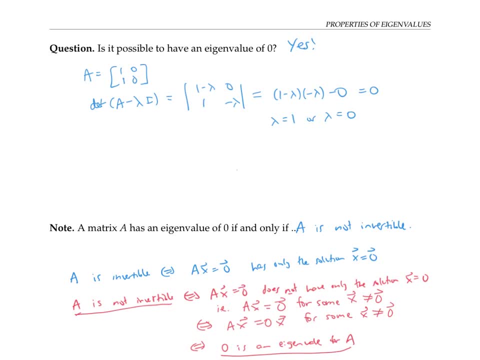 And that's exactly what we wanted to prove. Let me note that an equivalent way of saying this is that a matrix A does not have an eigenvalue of zero if, and only if, A is invertible. In this video, we covered a lot of properties. 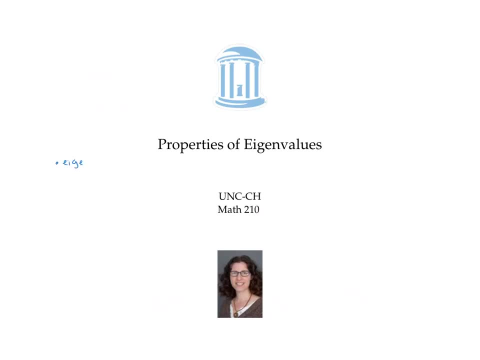 of eigenvalues. we saw that the eigenvalues of a triangular matrix are just the diagonal, right diagonal entries. we saw that the sum of the eigenvalues is equal to the trace of the matrix And the product of the eigenvalues is the determinant of the matrix. We saw that A and 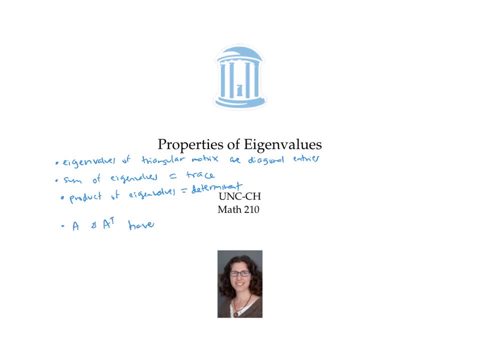 A transpose have the same eigenvalues and the A and A inverse have reciprocal eigenvalues. Finally, we saw that a matrix A has an eigenvalue of zero if, and only if, A is invertible, if and only if A is invertible, if and only 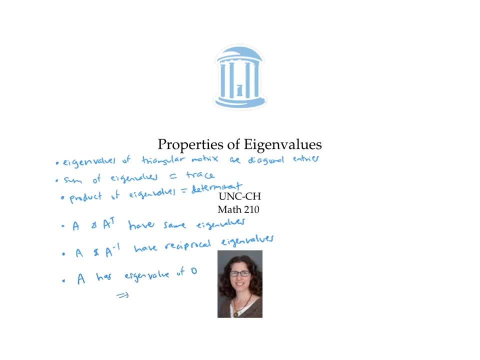 if A is an eigenvalue of zero, if, and only if, it is not invertible. Or, equivalently, A is invertible if, and only if, it does not have an eigenvalue of zero. Recall that a diagonal matrix is a matrix like this one, in which all the non zero entries lie on the diagonal. 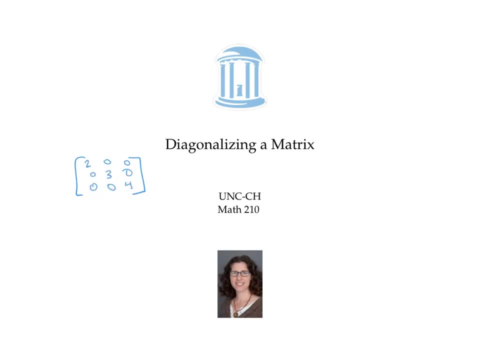 In other words, all the entries that are off the diagonal are zero. Diagonal matrices are much easier to work with than just arbitrary matrices, And for that reason it can be helpful to diagonalize a matrix or relate it to a diagonal matrix when possible. 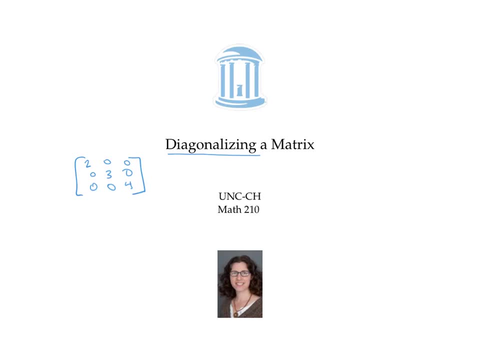 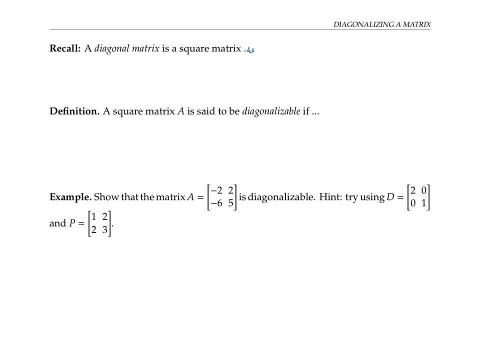 In this video I'll explain what diagonalizing a matrix means and how to do it in some situations, As we just reviewed, a diagonal matrix is a square matrix whose non-zero entries all lie on the diagonal. A square matrix, A, is said to be diagonalizable if A can be written in the form P times D. 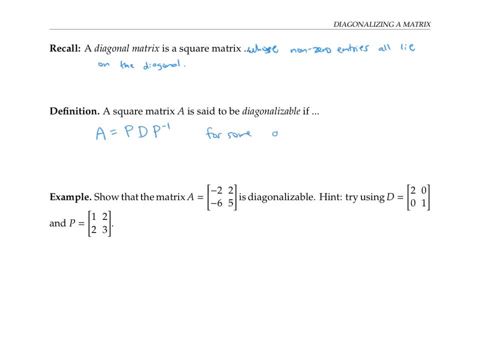 times P. inverse for some diagonal matrix D and some invertible matrix P. So if A is an n by n matrix, then D and P are diagonal. Need to also be n by n matrices to make the dimensions work out. Let's see what this means in an example. 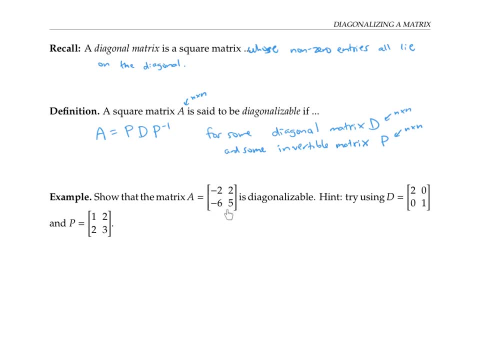 We're asked to show that this 2 by 2 matrix is diagonalizable And we're given a very big hint to use this diagonal matrix and this matrix P, which hopefully is invertible. Recall, there's a nice shortcut trick to finding the inverse of a 2 by 2 matrix. 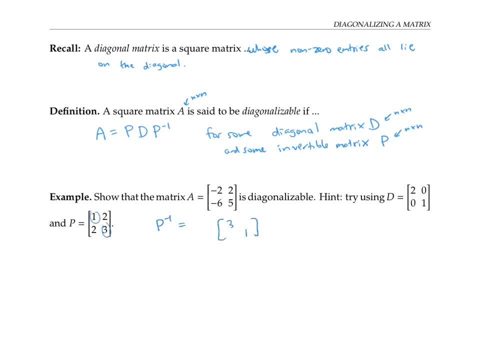 We swap the entries in the diagonal and negate the entries that are invertible And then multiply the whole thing by 1 over the determinant of the matrix. That's 1 times 3 minus 2 times 2, or negative 1.. 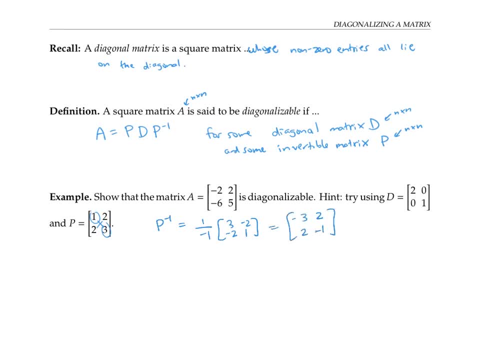 I'll rewrite this by multiplying through by negative 1, and we've got our P inverse. So now we need to check that A is equal to P D P inverse. In other words, we're going to multiply P by D by P inverse. 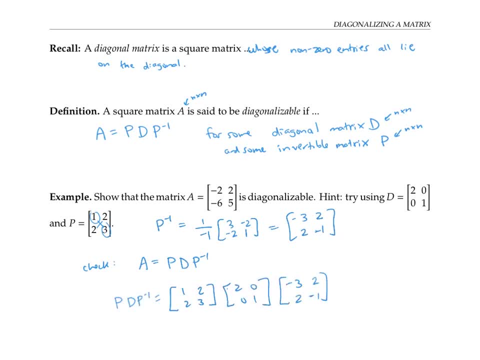 Okay And see if that works out to A. I encourage you to pause the video for a moment and work it out for yourself before going on Now. there's something interesting that happens when you multiply any matrix, in this case P, by a diagonal matrix, in this case D, with a diagonal matrix on the right. 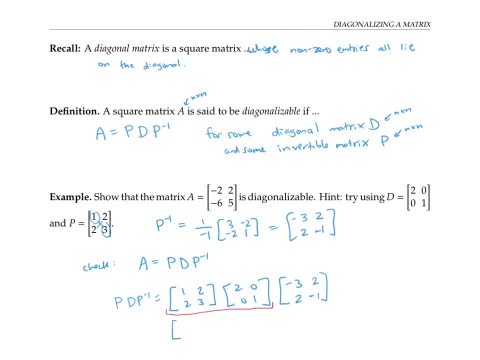 You end up just multiplying the columns of the first matrix by the corresponding diagonal entries. In other words, this is just the same as taking the column 12.. And multiplying them by two to get to four, And then taking this column to three and multiplying it by one to get to three again. 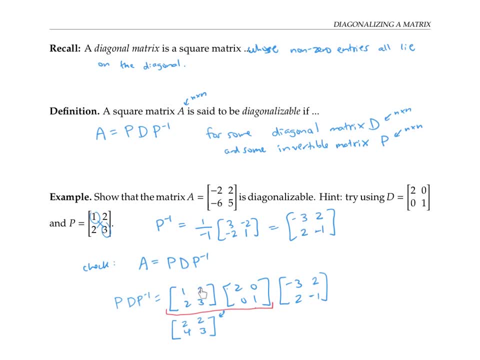 That's the output of that multiplication. Let's just see how that works. We're multiplying to get this entry to. we're multiplying this row by this column, But since there's a zero here, we're just really multiplying this first entry by two. 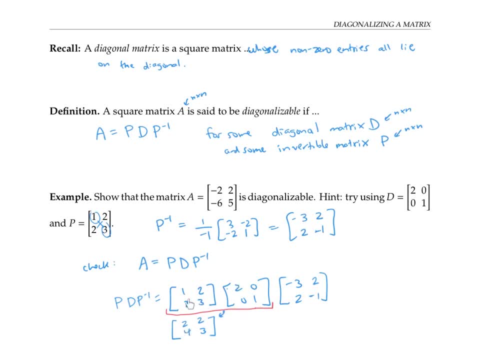 And to get this entry here, we're multiplying this row by this column, which again just multiplies the entry by two. So This column just got multiplied by two to get this column. To get this entry here, we're taking this row, times this column. 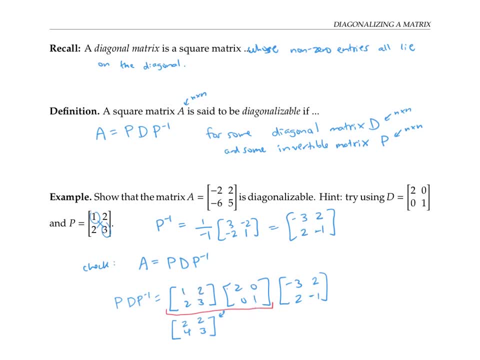 Well, that ends up multiplying this entry by one. to get this entry, this row, by this column, which multiplies this entry by one. So this column gets multiplied by one. I meant that I went through that in such detail because we're going to use this fact in a 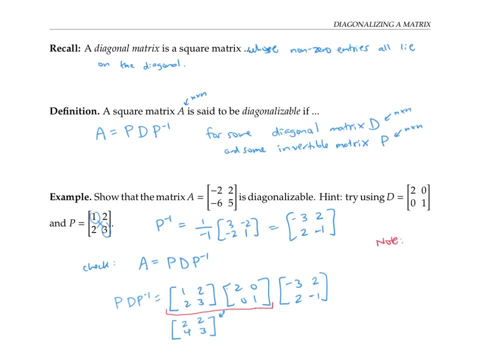 moment. In fact I'll write it out as a little note. So the note is: When we multiply Any matrix, M, by a diagonal matrix, I'll call it E. So M times E. This multiplies the columns of M by the diagonal entries of E. All right, 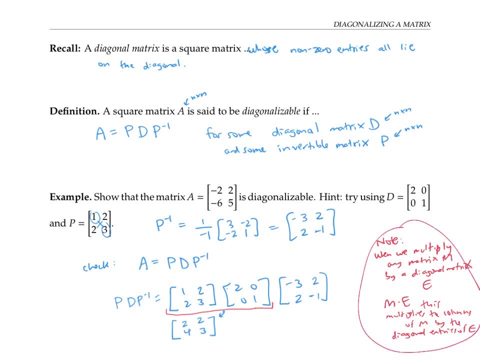 So now that we've got that note tucked away there, let's continue with the problem. So we still need to multiply this matrix by the P inverse matrix And if we work that out we get- let's see: negative two, two, negative six, five, which. 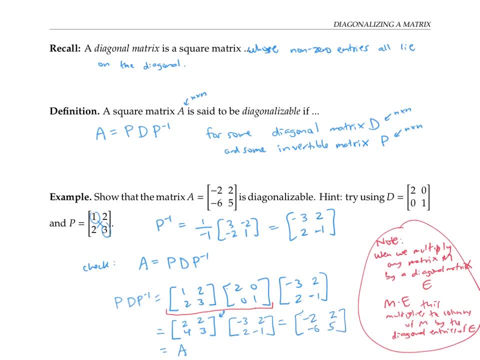 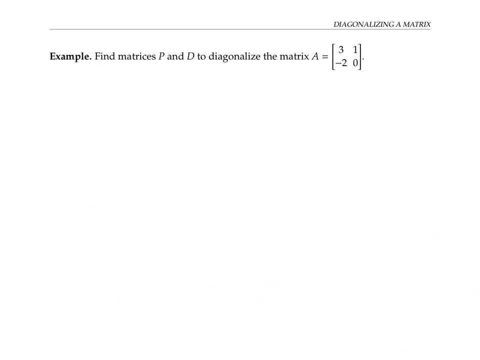 is exactly the A matrix that we started with. So, indeed, the matrix A is diagonalizable, And these are the matrices D and P that do the trick. But what if we want to diagonalize a matrix like this, matrix A, and we're not given the 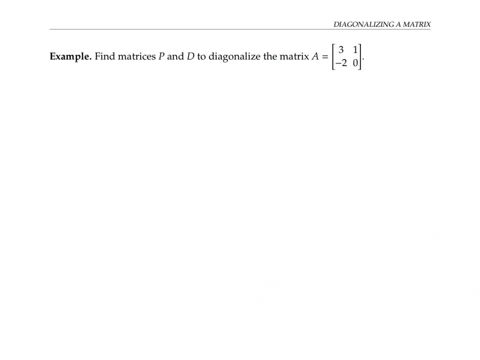 matrices D and P. to do it, we have to find them. In other words, we need to find D, which is diagonal, and P, which is invertible, such that A is equal to PDP inverse. I'm going to rewrite that equation by multiplying everything. 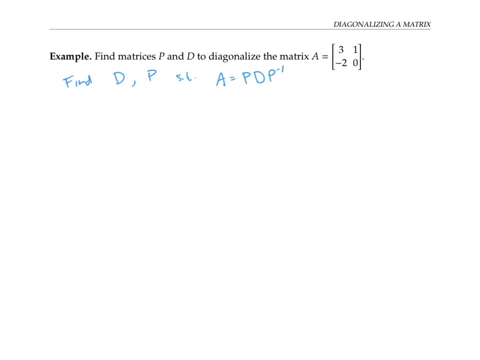 on the right By P. so I get A: times P is P times D, times P- inverse times P. Well, P inverse times P is just the identity, And every anything multiplied by the identity is just the same thing. So this equation becomes A times P equals P times D. I want to focus in on the columns. 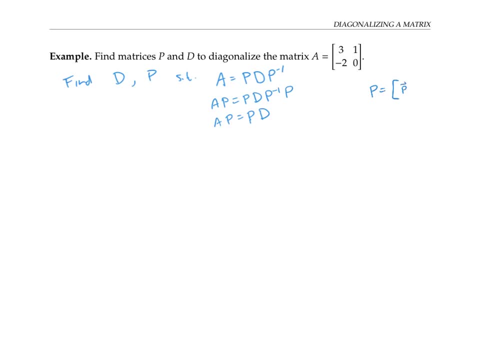 of P, So I'll draw attention to them by writing P as its columns concatenated together. And I also want to draw attention to the diagonal entries of D, So I'll write the diagonal entries of D out like this: So let me bring that notation into my equation: AP equals PD. 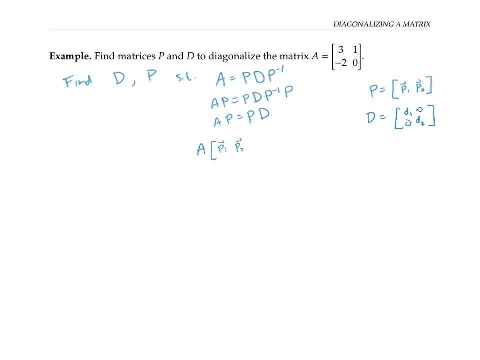 So that's A times the columns P1, P2, equals the columns P1, P2 times this diagonal matrix here that we don't know what B and D are yet, But we do know because we talked about it on the previous slide. 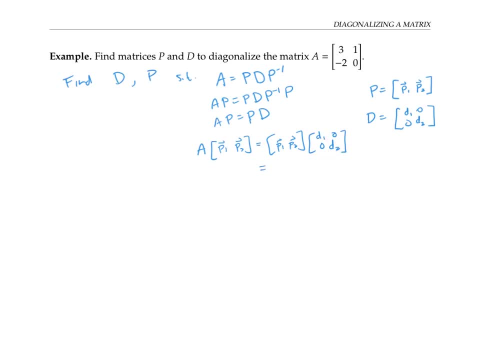 Okay, Then we multiply this matrix by this diagonal matrix. we just end up multiplying these two columns by the corresponding diagonal entry. So this is D1 times the column P1.. And then we have the column D2 times the column P2.. 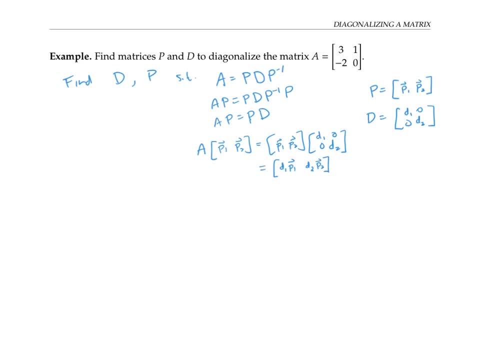 And hopefully you also remember from the video about interpreting matrix multiplication that when you multiply a matrix by another matrix, that's just the same thing as multiplying the matrix by each column. So if you multiply a matrix by each column of the second matrix and stringing them together, 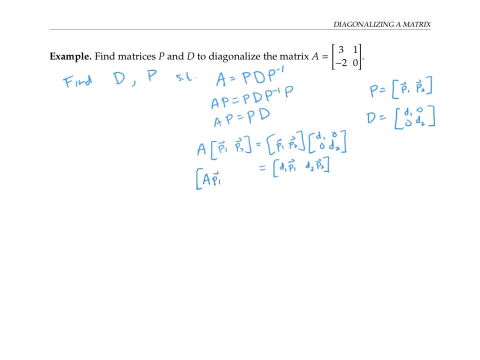 you can just try that out for a couple of matrices and verify it. So this means that we're looking for vectors P1 and P2 and numbers D1 and D2.. So that A times P1 equals D1 times P1, and A times P2 equals D2 times P2, so that these 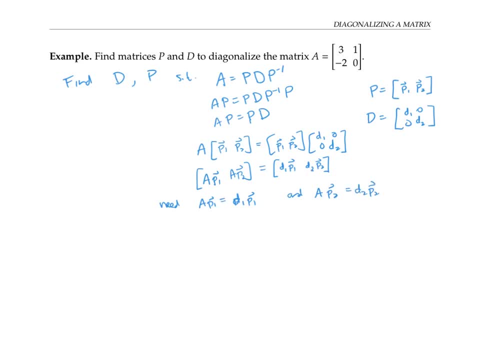 two sides match, So the equation will really be equal. Does that remind you of anything? Because it reminds me a lot of eigenvalues and eigenvectors. This is exactly the statement that D1 is an eigenvalue of A with corresponding eigenvector. 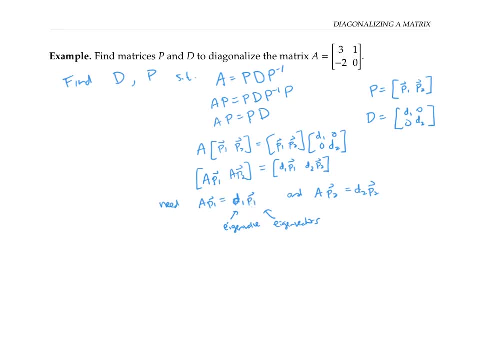 P1. And ditto for D2 and P2.. So we found the key idea for diagonalizing a matrix: We look for eigenvalues. We look for eigenvalues and eigenvectors. That's how we build our matrices D and P. 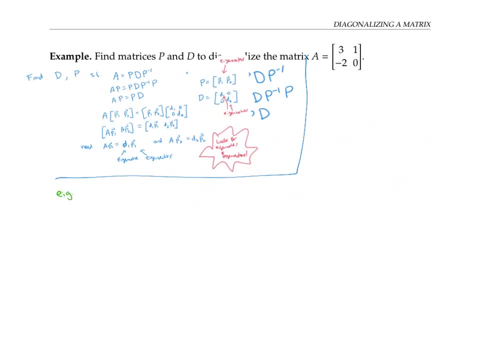 So let's get to work. To find the eigenvalues of A, we need to write down the characteristic polynomial, which we do by taking the determinant of A minus lambda I, So that's the determinant of 3 minus lambda, 1, negative, 2, 0 minus lambda. 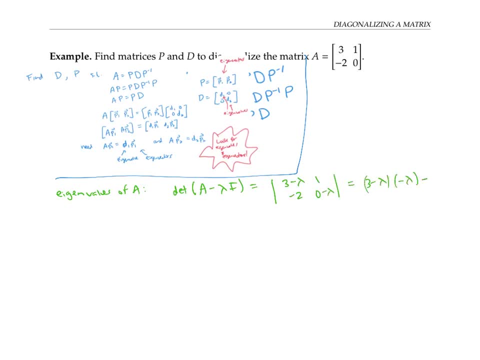 Which is 3 minus lambda times negative, lambda minus negative, 2.. Which simplifies to lambda squared minus 3, lambda plus 2.. And that factors to lambda minus 2 times lambda minus 1.. We set that equal to 0.. We have the eigenvalues: lambda equals 2 and lambda equals 1.. 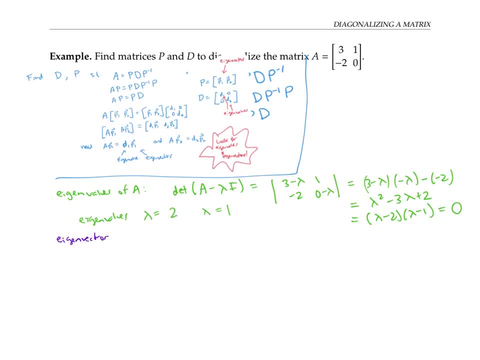 Now to find an eigenvector Corresponding to The eigenvalue lambda equals 2.. We need to solve the equation A minus lambda. I times X equals 0.. For lambda equals 2.. That is, I need to solve the matrix and vector equation. say, when lambda is 2, that gives: 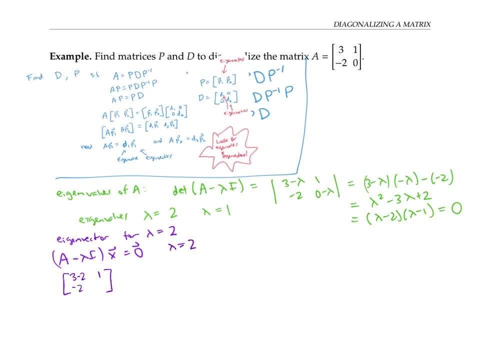 me 3 minus 2, 1, negative 2, 0 minus 2 times X1, X2.. So that's 2.. That's 2.. That's a 0.. That's 0.. Yeah, that's a 0.. 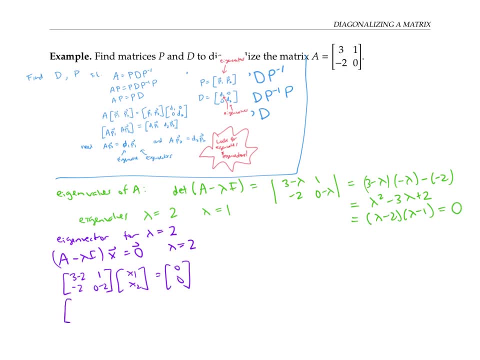 Yeah, So that's 3 minus 2 and it's 2 plus 1 minus 2.. 3 minus 2 equals 0, 0.. And I can do that by writing down the augmented matrix. Let's see: 3 minus 2 is 1.. 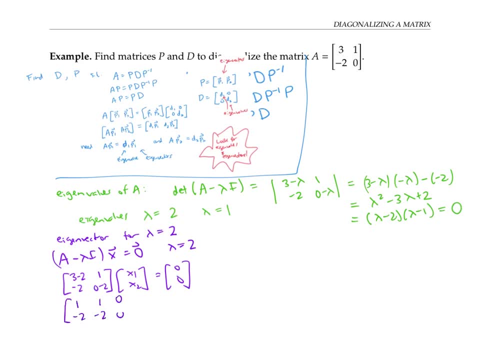 1, negative 2, negative 2.. Augmented by 0, 0.. And I need to row reduce this to reduced row echelon form. This matrix is pretty easy to row reduce if I just take the first row and multiply it. 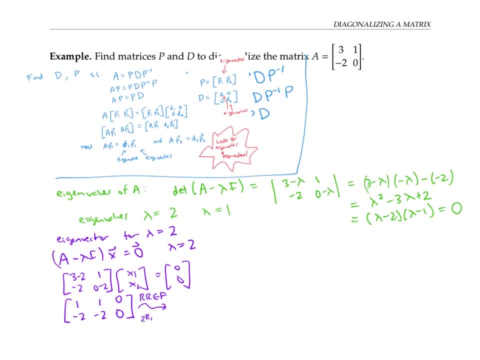 by 2 and add it to the second row, right? So it's going to be 1,, 1,, 0, and 0.. it to the second row and replace the second row with that. I've already got it in reduced. 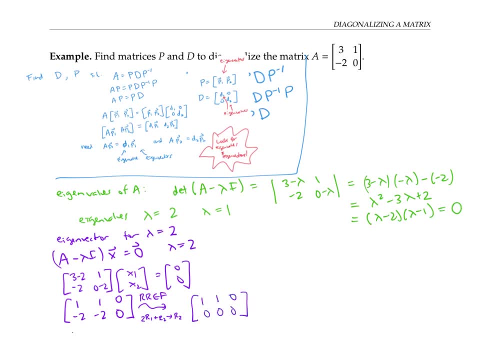 row echelon form. This tells me that x two can be free, And x one plus x two has to be zero. So x one is minus x two. So an eigenvector that I can use is just like any x two and 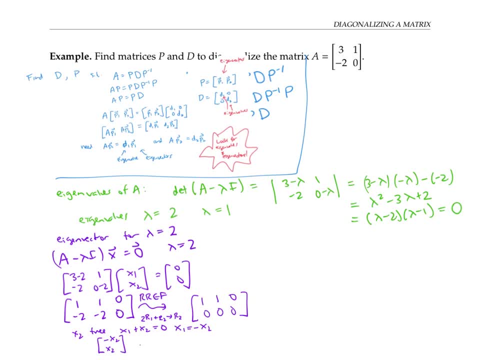 then minus x two here, or in other words x two times the vector minus 11.. So I could just use the eigenvector negative one one. keep things simple Now I'll repeat this process. for lambda equals one, So now I need a minus one times I times x equals zero. So that is. 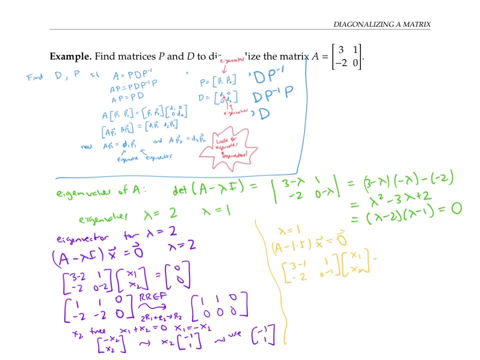 this matrix times the x one x two. vector 21 is equal to the zero vector And I can row reduce the augmented matrix to one negative, two negative one augmented by 00.. This row reduces to this matrix, So I have x two being a free variable and 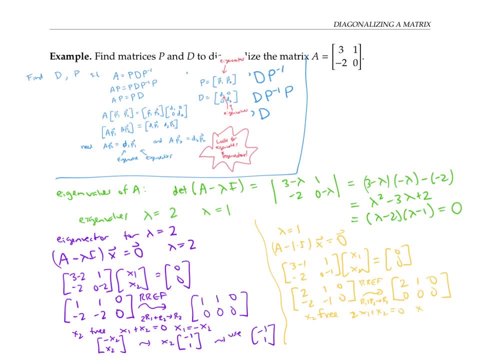 two x one plus x two equals zero, means x. one is negative, one half x two. So my eigenvectors are of the form x, two times negative, one half one, And so I can just use the eigenvector negative one half one as my eigenvector. So now I'm almost done finding P and D. My D matrix is the diagonal. 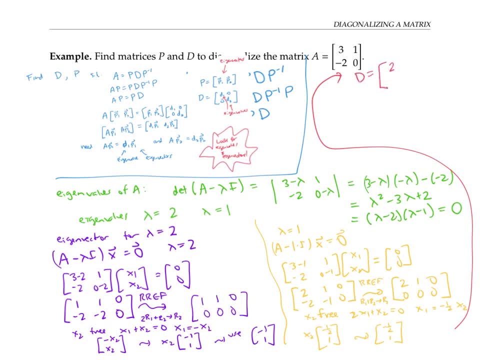 matrix made up of my two eigenvalues, two and one, and my P matrix is made up of the corresponding eigenvectors, negative one, one and negative one half one. notice that the eigenvectors need to be in the same order as the eigen, the eigenvalues. 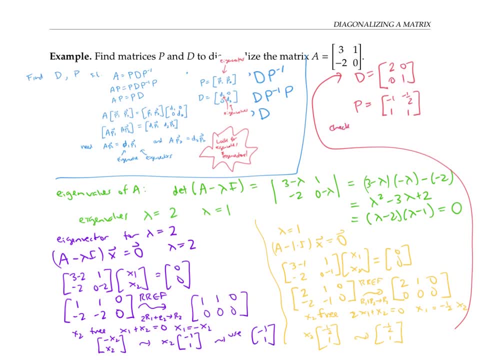 they correspond to. I will leave it to you to check that when we multiply P by D, by P inverse, we get indeed our original matrix A. Here's a little interesting tidbit I want to point out before we move on. The matrices that you use to diagonalize another matrix are not unique. 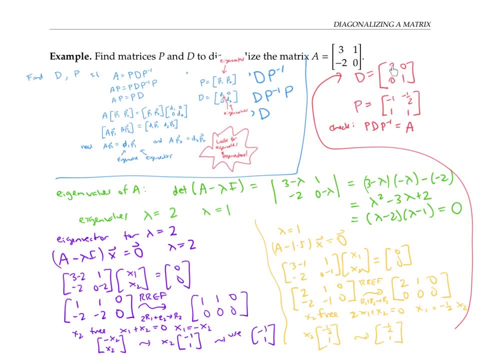 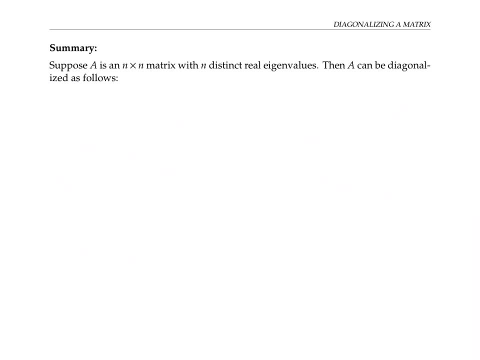 because we could have instead put the eigenvalues in the other order, one and two, And then switched around the corresponding eigenvectors, and that would have worked just as well. So the process we just used for this two by two matrix can be used for any n by. 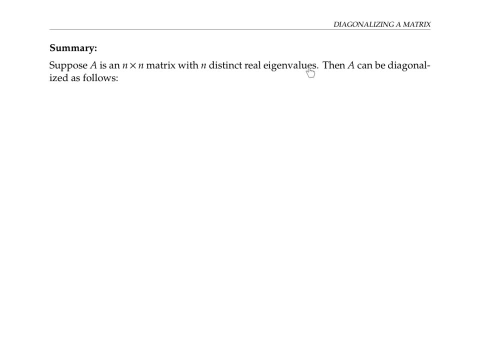 n matrix with n distinct real eigenvalues. The process goes like this: First you find the eigenvalues lambda one through lambda n and you put them in your diagonal matrix D. Then you find the eigenvalues lambda one through lambda n And then you put them in your diagonal 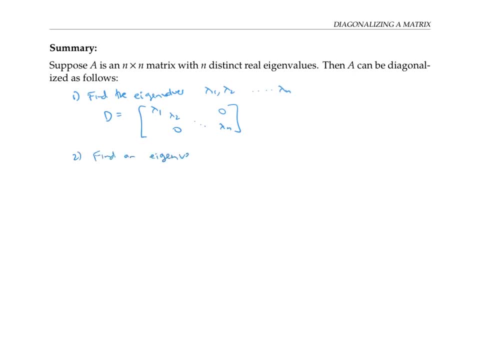 matrix D, And then you find an eigenvector for each eigenvalue. Let's call these eigenvectors V, one through V, n, And we make our matrix P by stringing together those eigenvectors. Now I should point out that it's not always necessary for the matrix A to have the n by 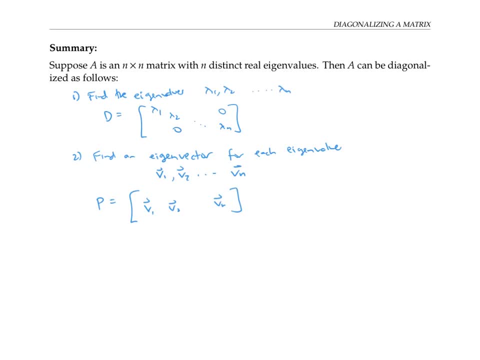 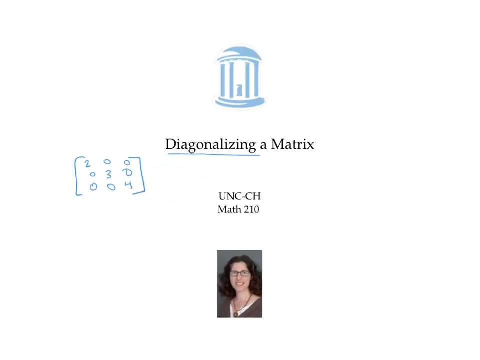 n matrix A to have n distinct real eigenvalues. Sometimes A can be diagonalizable Even if it doesn't have as many distinct eigenvalues as its its dimension, But this situation will cover all the problems that will work in this class. So in this video we defined: 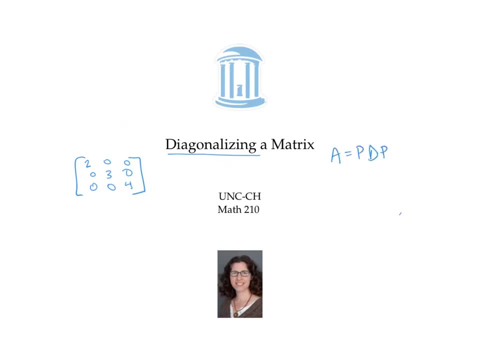 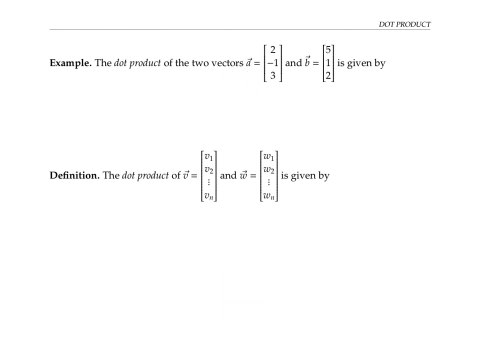 what it means to diagonalize a matrix And we showed how it can be done using eigenvalues and eigenvectors. This video introduces the dot product of vectors. Suppose I have these two vectors, A and B, each with three components. I find the dot product, which is written a. 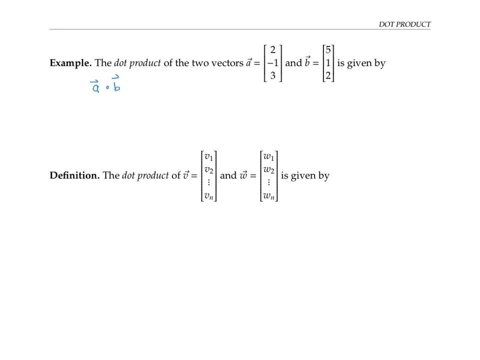 dot B. I usually write it with a little circle to make the dot more obvious. To compute that, we multiply corresponding entries and add them up. So here we do: two times five plus negative, one times one plus three times two, and that adds up to 15.. 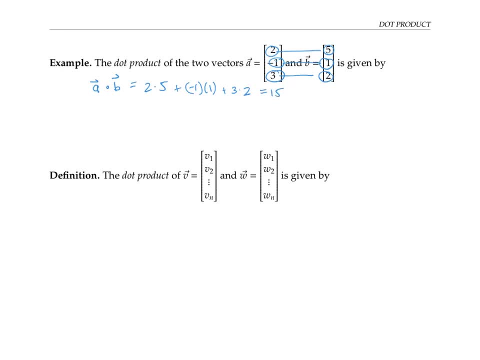 In general, to take the dot product of two vectors, each one with n entries, we again multiply corresponding entries and add them up. So here v dot w would be v one w one plus v two times w two plus all the way through v n times w n. Here are some properties of 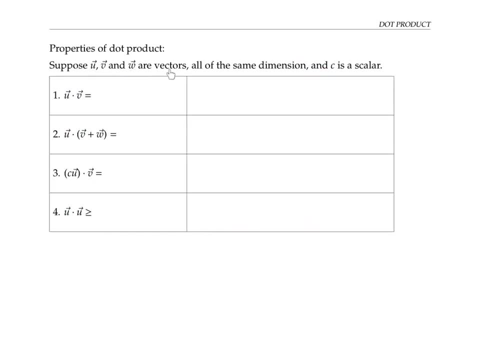 dot product. Let's suppose that u, v and w are vectors all of the same dimension, and by the same dimension I just mean the same number of elements. And let's suppose that C is a scalar. If we don't take the dot product, u, dot v, that's the same thing as doing v. 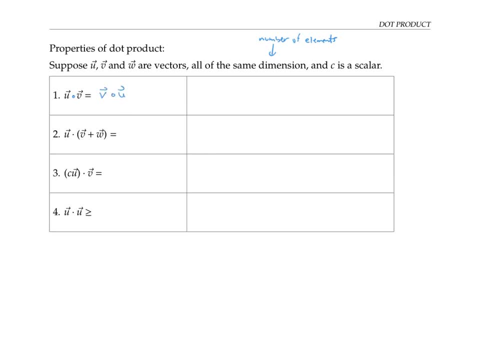 dot u. In other words dot product is commutative. dot product is also distributive over addition. If I take dot u dot v plus w, that's the same thing as doing u dot v and adding u dot w That's distributed in the other direction to. if I take v plus w and dot it with you. 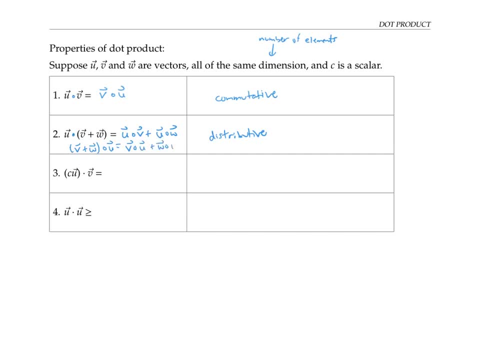 that's the same thing as v dot u plus w dot u. If I do scalar multiplication together with that product, I can move that scale around any way I want. I can rewrite this as u dot C times v, or I can do u dot v first and then multiply that by C. All of those give me the. 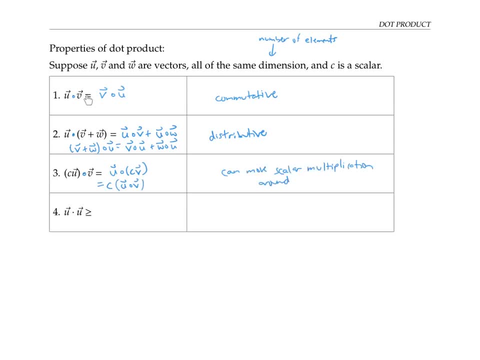 same thing. All of these first three properties can be proved by just writing out that product in terms of the entries and using the commutative, distributive and associative properties of regular arithmetic. For example, if we want to prove that u dot v is the same thing as 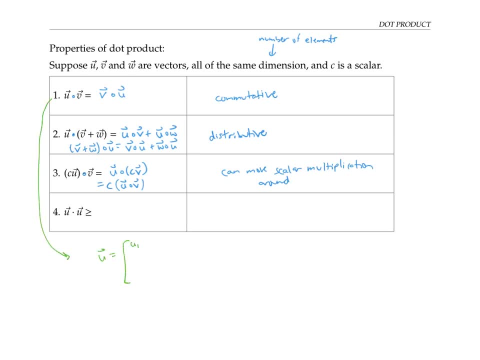 v dot u. if we just write out the entries of a general vector u with n entries and the entries of a general vector v with n entries, We write out u dot u, u dot v. then that string of arithmetic is the same thing as if we switch the orders. 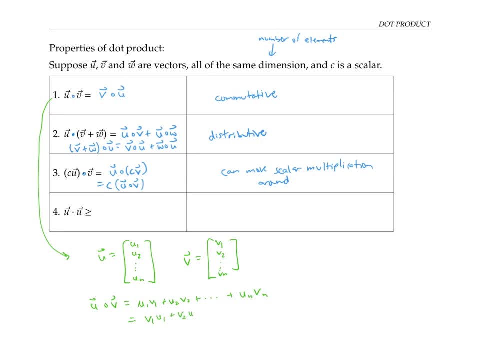 of the V's entries and the use entries, which is the same thing as the dot u, And these other properties can be proved similarly. Finally, last property, if I take you and dot it with itself, then I could get a lot of different numbers, but I'm always going. 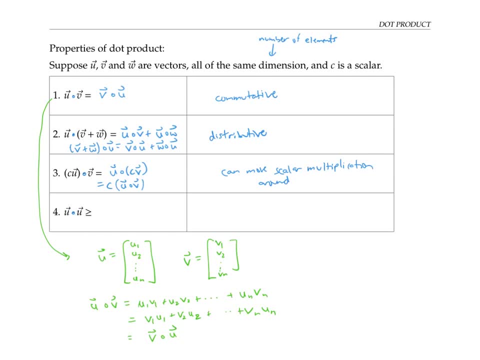 to get a number that's positive or zero. u dot u is always greater than or equal to zero. That's because u dot u can be written in terms of its entries as u one times u one plus u two times u two. keep adding up the entry times itself: un times un, In other words. 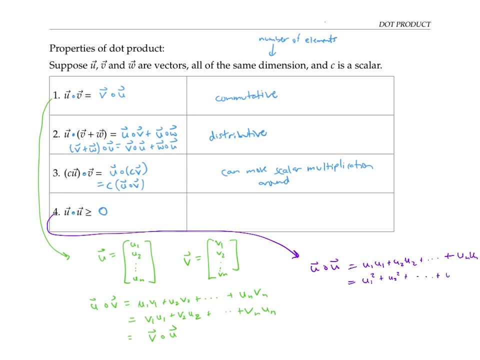 it's the sum of a bunch of squares, And squares are always positive numbers or zero, So therefore this quantity has to be greater than or equal to zero. In fact, u dot u is only going to be equal to zero, can be equal to zero if, and only if, the u, one, u, two and u? n are all zero, even one of them. 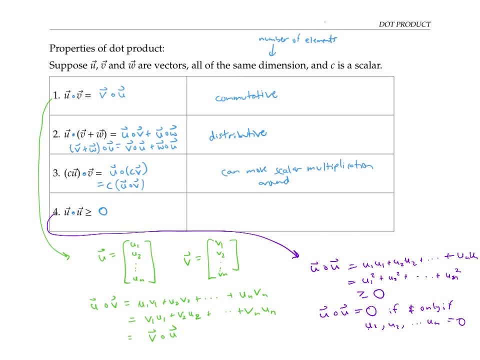 is positive or negative, not zero. when you square it it'll be a positive number. you'll get something strictly positive. So u dot u zero if, and only if, all of these entries are zero, ie u is the zero vector, the property. 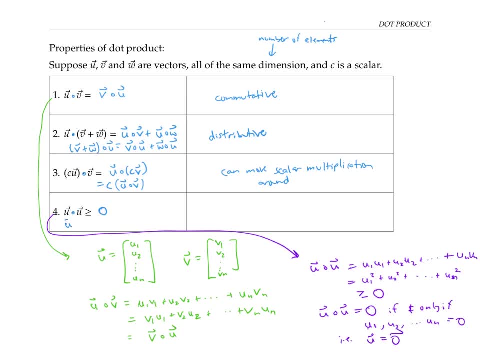 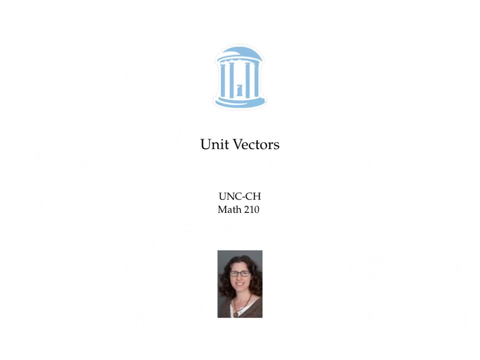 that u, dot u is always greater than or equal to zero and that it's equal to zero if, and only if- u is the zero vector is called the positive definite property. And that concludes this brief introduction to dot product. In this video we'll review how the length of 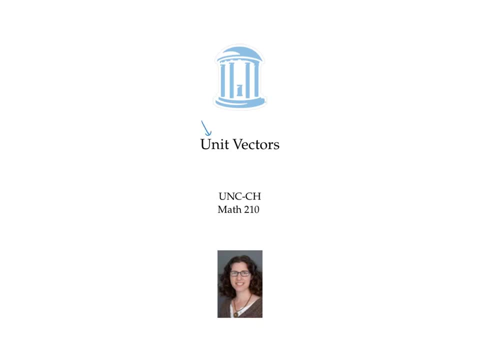 a vector is computed, And then we'll talk about unit vectors, Which are vectors of length one. Our first example is a vector a with two entries, so dimension two, to find its length, which I'll write with double bars, although some people 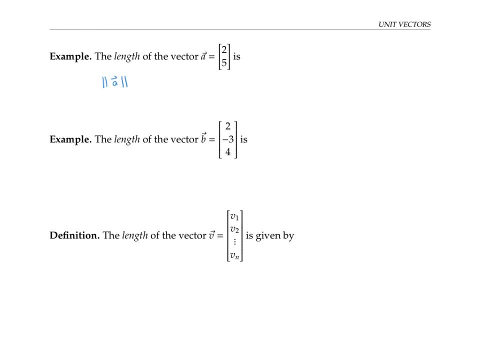 write length of a vector just with single bars. like absolute value, we take the square root of two squared plus five squared, which works out to the square root of 29.. That makes sense because if you draw the vector with its tail end at the origin and then you're 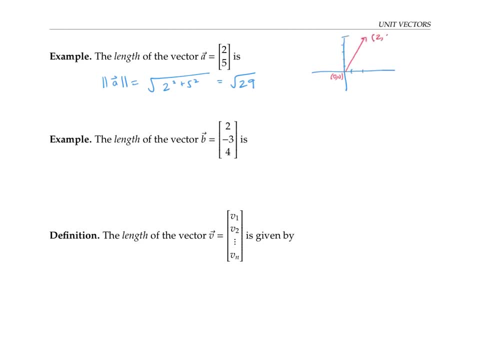 at its terminal point, at the point to five, then Pythagorean theorem says: two squared plus five squared gives us our length squared. If we want to find the length of this three dimensional vector specter with three entries, then we use the three dimensional version. 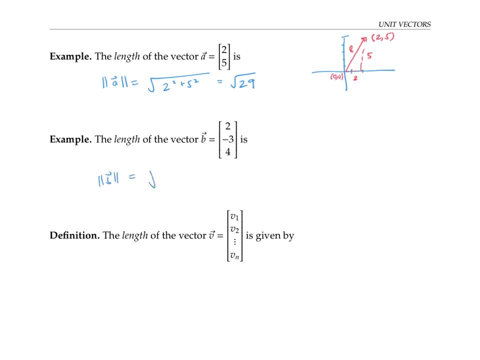 of Pythagorean theorem, the length of B is going to be the square root of two squared plus negative three squared plus four squared. This works out, coincidentally, to also be the square root of 29.. You can also think of this expression for length in terms of the distance formula, If I draw this vector. 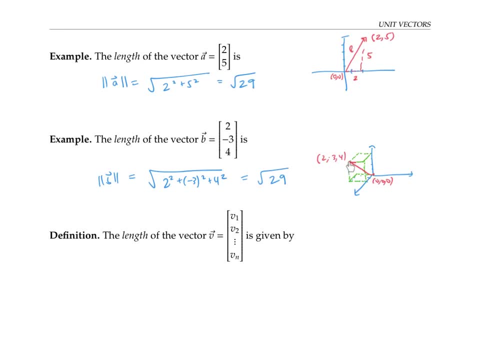 with its tail end at the origin and its tip at the point two negative three, four. then the length of the vector should be the distance between this point and that point, And by the distance formula that's the square root of two minus zero, squared plus negative three. 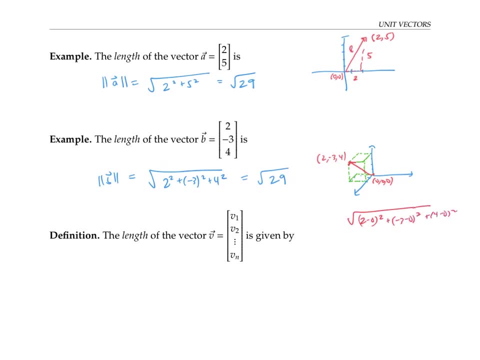 minus zero, squared. plus four minus zero squared. exactly the same formula as we used here In general. the length of a vector v with n entries, v one through v n, is given by taking the square root of the sum of all those entries squared. 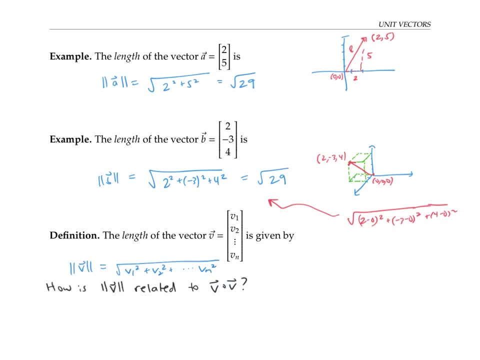 Now it turns out that the length of a vector is closely related to its dot product with itself. Recall that when we compute v dotted with v, we just have each component squared. I'll add it up. If we take the square root of both sides of this equation, we get the square. 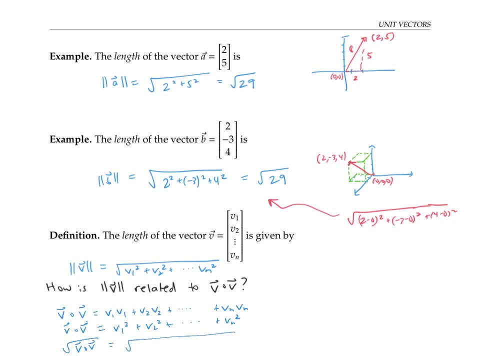 root of v dot. v is the square root of all these components added up, That's just the same thing as the formula for the length of v. So we have that the length of v is the square root of v dotted with itself, or, if you prefer, 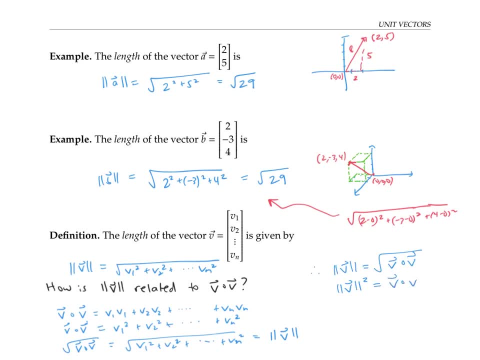 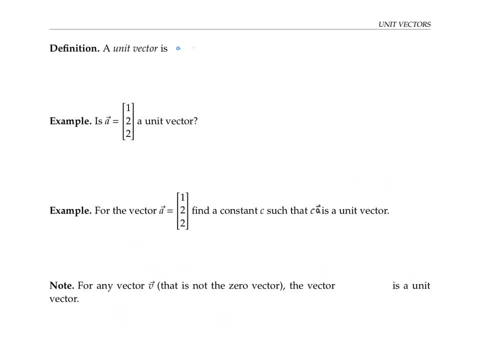 we could write that as the length of v squared is v dot v. This relationship will come in handy in the future. A unit vector is a vector of length one. So let's check, for example, if this vector, a, is a unit vector. we take its length square root of one squared plus. 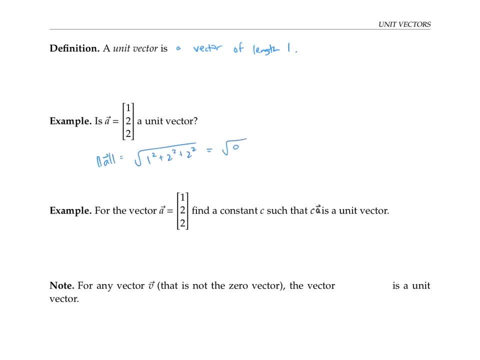 two squared plus two squared, that equals the length of a vector a. So you can use a vector a and you can solve this by taking the square root of a in the future and you we get the square root of nine, which is three, which is definitely not one. So the answer here: 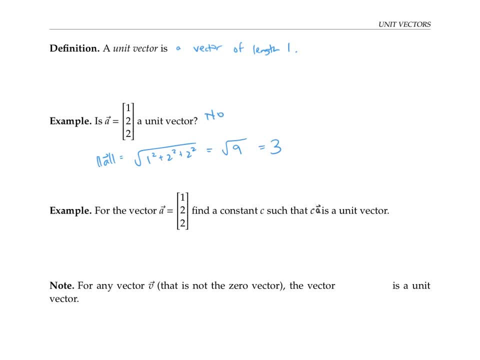 is no. Sometimes it's convenient to take a vector that's not a unit vector and rescale it to be a unit vector. In other words, multiply it by a scalar, by a number, so that that product is a unit vector. So what number would I have to multiply a by to get a vector of length one? 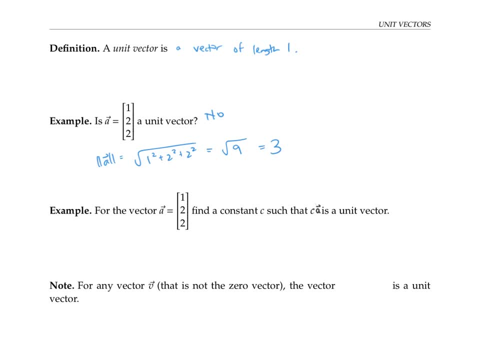 given that its current length is three. If you're saying, multiply it by one third, you're exactly right. Multiplying by one third will shrink it by a factor of three and get that length of three down to a length of one. Let's just check it with some arithmetic: One third times a is one third. 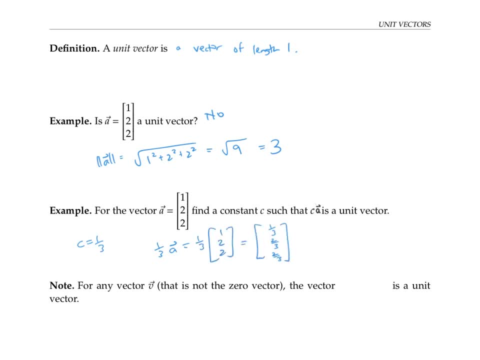 times each of these entries, And so the length of one third a will be the square root of one third squared plus two thirds squared squared plus two thirds squared, which is the same thing as a square root of one squared plus two squared plus two squared over three squared, which works out to one And more generally for any. 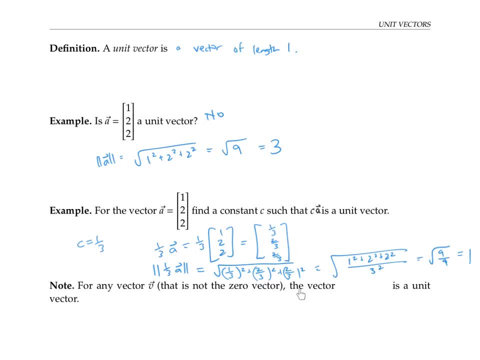 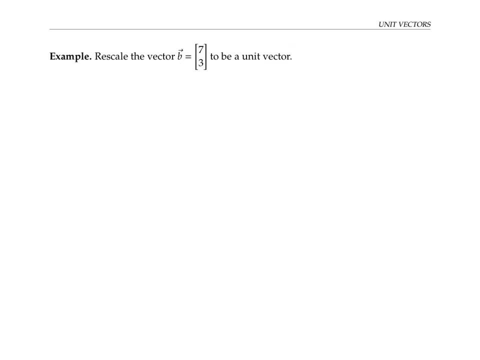 vector v, that is not the zero vector. we can rescale it to be a unit vector by simply multiplying by one over its length. Suppose, for example, we want to rescale this vector by a number of times a v to be a unit vector. Well, the length of v is a square root of seven squared plus three squared. 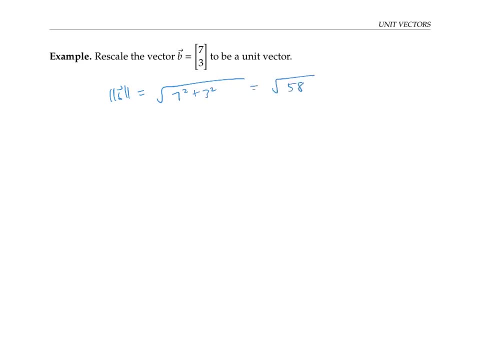 that works out to the square root of 58.. So our rescaled vector is going to be one over the square root of 58 times b, or in other words, seven over the square root of 58, three over the square root of 58.. And that's all for this video on unit vectors. 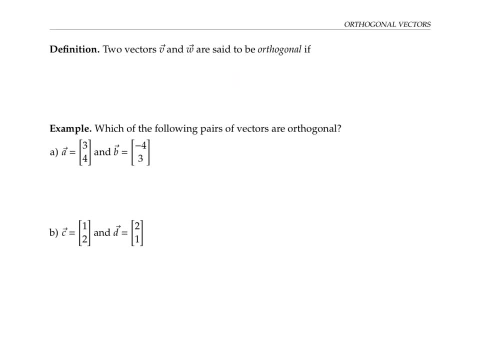 This video introduces orthogonal vectors. Two vectors, v and w, are said to be orthogonal if their dot product is equal to zero. Please pause the video for a moment and see which of these two pairs of vectors are orthogonal. For the first pair, if we take a dot B, that's three times negative, four plus four. 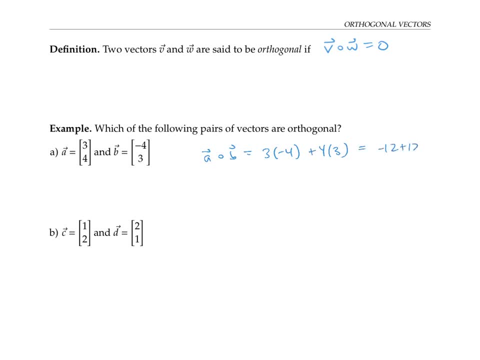 times three. that works out to negative 12 plus 12, which is zero. So yes, they are orthogonal. For the second pair, take c dot D. that's one times two plus two times one, which works out to four, which is not zero. So no, these are not orthogonal. The word orthogonal. 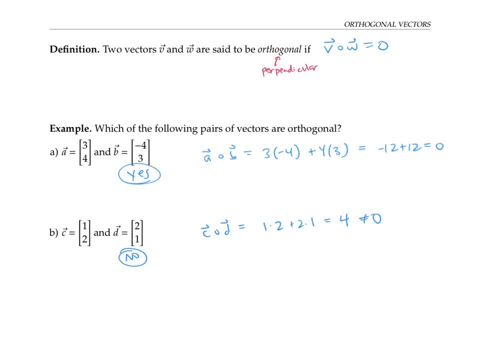 means perpendicular, And in fact it's true that v dot w equals zero if, and only if, v is perpendicular or at right angles to W. And if we draw these two pairs of vectors, we can see, in fact, that the first pair is at right. 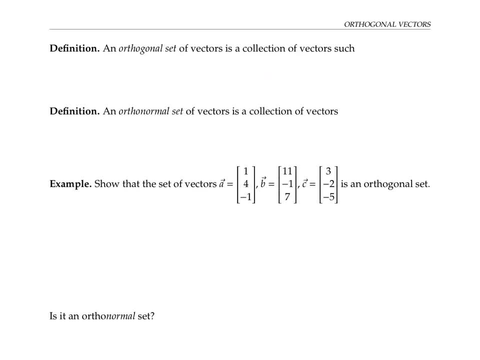 angles from each other and the second pair is not. Let's run through a couple more definitions. An orthogonal set of vectors is a collection of vectors such that for any pair of vectors- v and w in the collection, v is orthogonal. 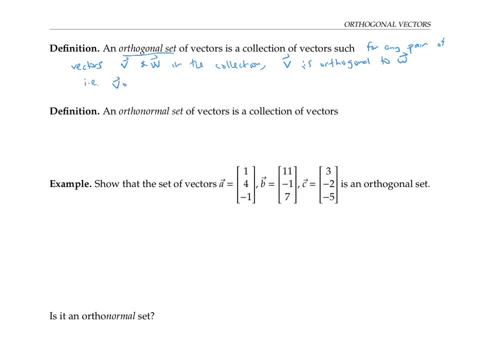 to w. I e. the doc product of V and w is zero. an orphan Normal set of vectors is a collection of orthogonal vectors that are also each unit vectors. In other words, for any vector in the sets, the vector V, the length of V is one. 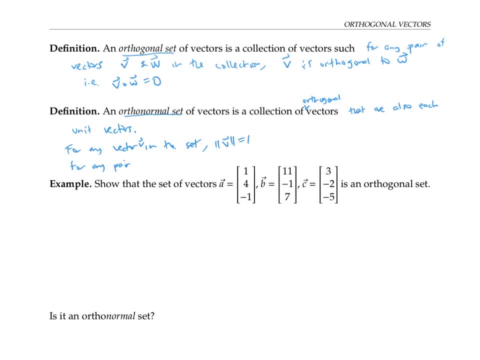 And for any pair of vectors, v and w, v dot w is equal to zero. So let's show that this set of vectors, it's just a set of three vectors: a, b and c. Let's show that it's an orthogonal set. 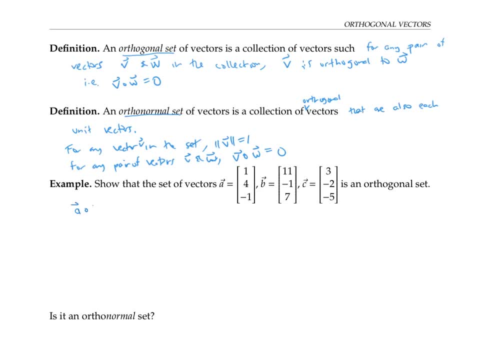 So for any pair there, there are three possible pairs. there's a and b, there's b and c and there's a and c. So let's compute each of these dot products. For the first pair, a and b, their dot product is definitely zero. For the next pair, b and c, I'm getting 33 plus. 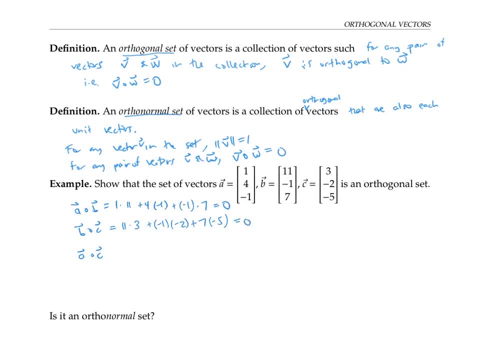 two is 35 minus 35. Yep, that's zero. And finally, for the third pair, a and c: Yep, here I'm also getting zero. So for any pair of vectors in the set, that pair is orthogonal to. 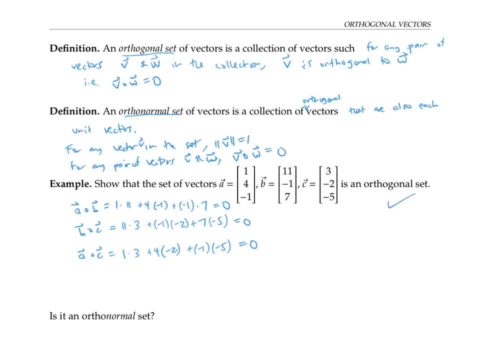 each other And therefore we have an orthogonal set. Is it, however, an orthonormal set? Well, no, because, for example, the length of a is equal to the square root of 18.. The length of b is the square root of 171.. And the length of c is a square root of 38. So this set doesn't have. 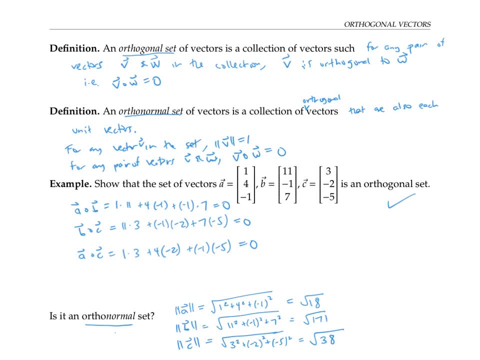 any unit vectors And it needs all of its vectors to be unit vectors as well as orthogonal to each other to be an orthogonal set. So let's show that we have an orthogonal set And therefore we have an orthonormal set. But I can make it an orthonormal set by taking a and dividing it by. 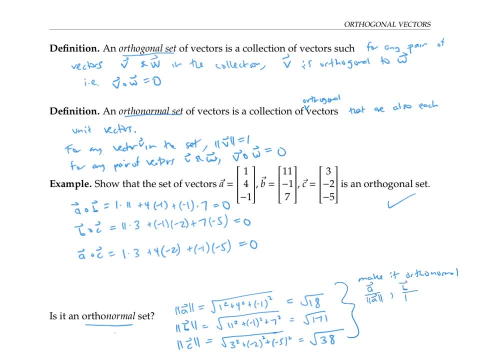 its length. they're multiplying it by one over its length, And same thing with B And same thing with C. those vectors which I'll write out here, those vectors will each be a unit vector and they'll still be orthogonal to each other Because, since they were perpendicular to each 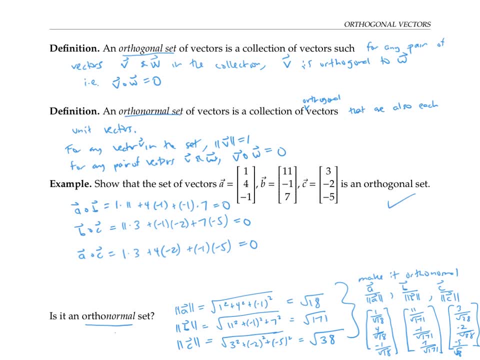 other before we rescaled them. they'll still be perpendicular, they'll still be at right angles to each other after we rescale them by altering their lengths. Another way of seeing the same idea is that, since a dot B was zero, when we take a over its length dotted with B over its length. 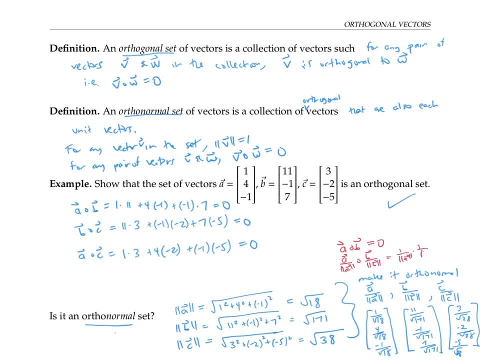 that's the same thing as one over the length of a times one over the length of B, times a dot B. And since a dot B was zero, multiplying it by the length of B, we get a dot B over its length. And since a dot B was zero, multiplying it by a couple of scalars still goes up to zero. So these: 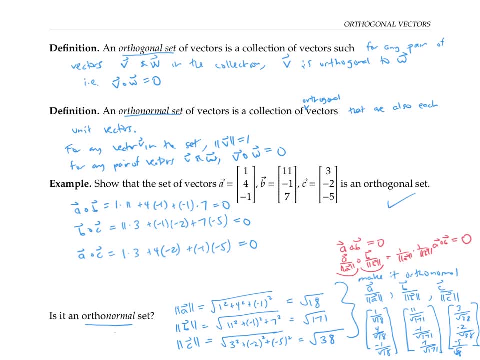 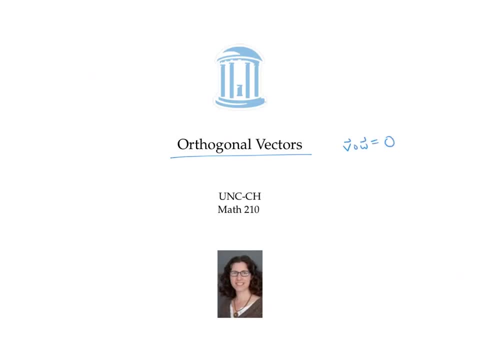 two vectors, once rescaled, are still orthogonal. In this video, we defined orthogonal vectors, vectors who are perpendicular to each other, whose dot product is zero. We also defined orthogonal sets and orthonormal sets of vectors. This video defines orthogonal matrices and give some properties of them. An orthogonal matrix is a square matrix with 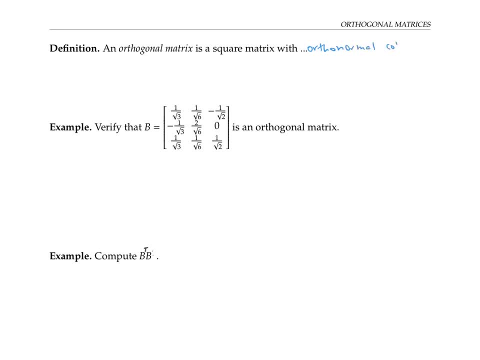 orthonormal and orthogonal matrix, And this matrix is a square matrix with orthonormal and orthonormal column vectors. Recall that a set of vectors is orthonormal. if every pair of Stop Save vectors is orthogonal and each vector by itself has length one, Recall that orthogonal elements. 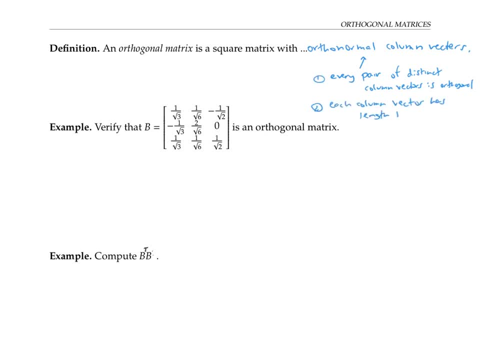 orthogonal means the same thing as perpendicular. it means the dot product of the two vectors is zero. So we could write this first condition in terms of dot product as saying that well, Assumable orthonormal is equal to either of the two vectors, equals to an hypothesis or the second bench Hm. 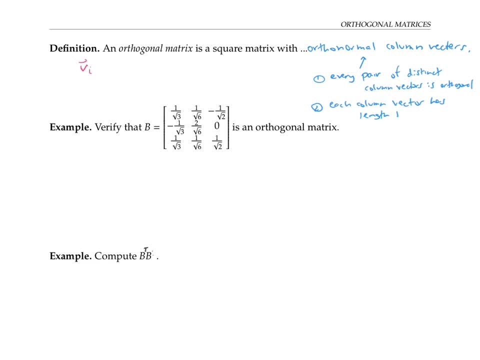 vector is definitely一定要 orthonormal, And what we we're going to do is Legalize these. that vi dotted with vj has to be zero where vi and vj are any two distinct column vectors or the matrix. The second condition: that each column vector has length. one can also be written: 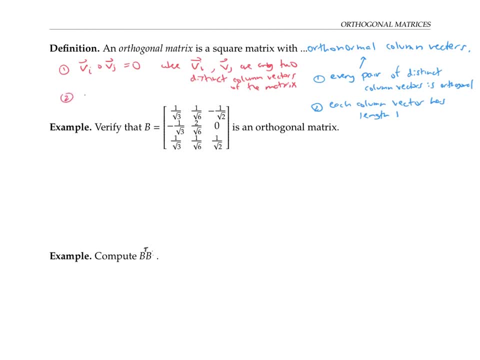 in terms of dot product, since the length of a vector squared is the same thing as the dot product of the vector with itself. So saying that the length has to be one is the same thing as saying that the length squared has to be one, or saying that the dot product 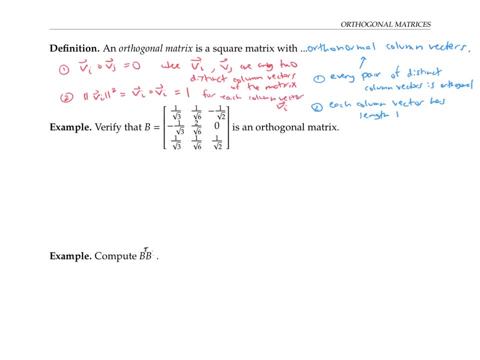 of the vector with itself has to be one. So let's verify that this matrix B is an orthogonal matrix. So first we need to check that each pair of column vectors is orthogonal. So I'm going to give these column vectors names. I'm going to call them: this one at c, one, and. 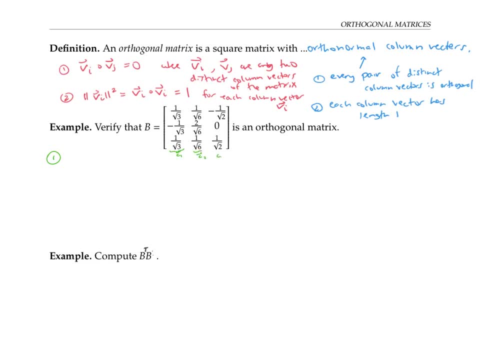 vector. this one I'll call it c two and this one I'll call it c three. So we need to check that c one dotted with c two is zero, that c one dotted with c three is zero and that c two dotted with c three is zero. So, for example, if I want to do the first one, 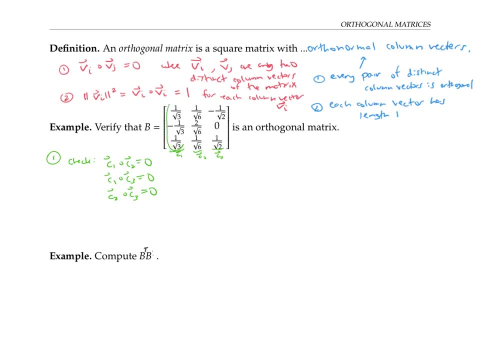 c one dotted with c two is this vector dotted with this vector. So that's going to be c one over root, three times one over root six minus one over root, three times two over root six plus one over root, three times one over root six, which adds up to one minus two plus. 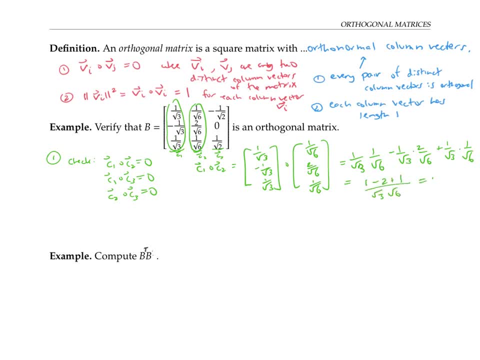 one over root three, root six, which adds up to zero, as we want it to. I'll let you verify for yourself that these other two dot products are also zero. So the column vector vectors are all orthogonal. Now, let's all. let's check that they all have length one. 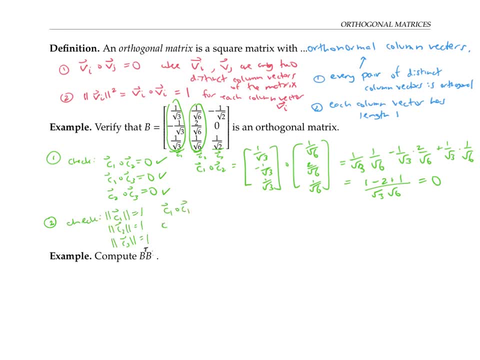 Or equivalently we could check that the dot product of each column vector with itself equals one. For example, if we take c one dot with c one, that's going to be one over root three times one over root. three plus minus one over root, three times minus one. 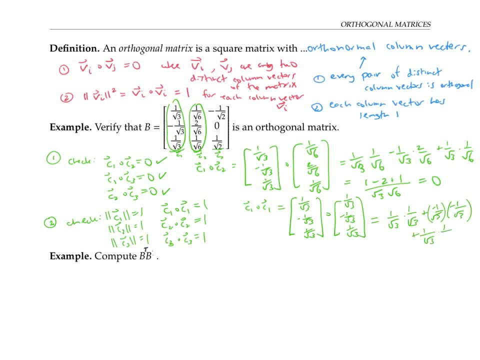 over root three plus one over root three, root three times one over root three, which adds up to one third plus one third plus one third, which is indeed one, And I'll let you verify that the other two columns also have length one. So B is indeed an orthogonal matrix. Let's see what happens when we compute B transpose. 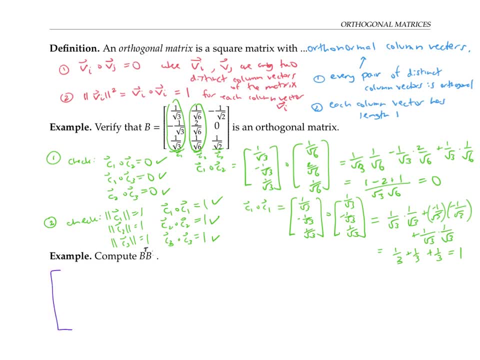 times B. So here's B transpose, where I've turned every row into a column And I'm going to multiply that by the original matrix B. So my answer should be a three by three matrix, And to get the element here in the upper left corner I need to multiply the first row by. 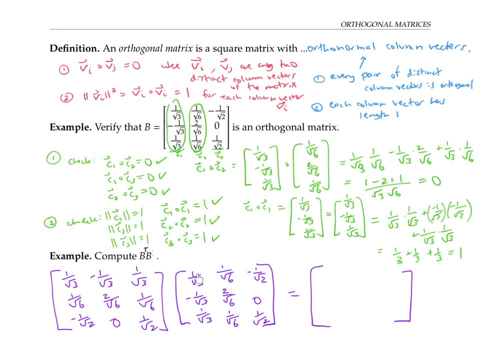 the first column. So that looks like what we just did right when we calculated column one, two, three, four, five, six, seven, eight, nine, 10,, 11,, 12,, 13,, 14,, 15,, 16,, 17,, 18,, 19,, 20,, 21,. 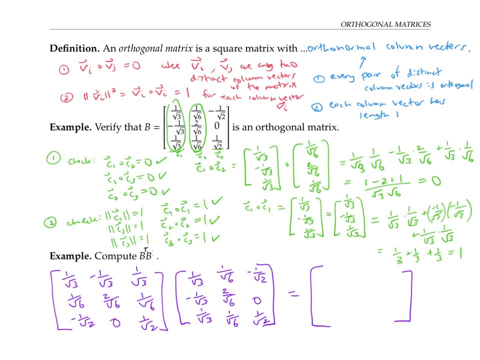 21 times column one. it's the same computation. of course it's the same computation because this row came from it. since this is a row as part of B transpose it came from the first column of B, So we're just doing the first column of B in row form times the first column of B, So that's. 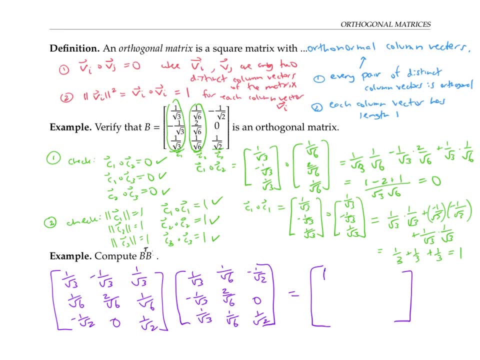 just the computation we did. that has to equal one. Now to get the next entry: entry in the first row and second column of the answer. we're going to do the first row of B transpose times the second column of B, But that's just the same thing as the first column of B right times the second column. 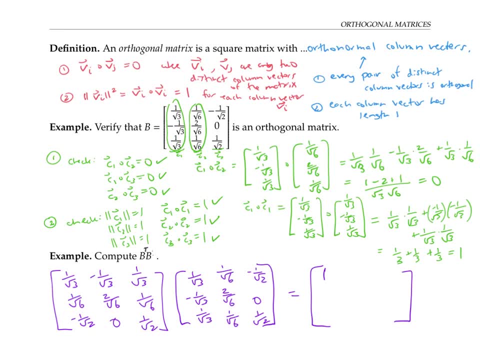 of B. So first column of B times the second column B was zero. The next entry over here is going to come from the first row of B, transpose times, the third column of B. But that's the same as doing the first column of B times the third column of B And since this is an orthogonal matrix, 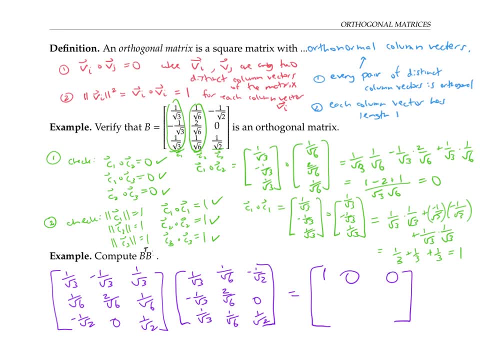 that needs to be zero. If we continue like that, we see that every single entry of this matrix is actually coming from a row of B transpose and a column of B, which is the same thing as coming from a column of B times a column of B, So those are always going to be zero if we're getting it from distinct columns And 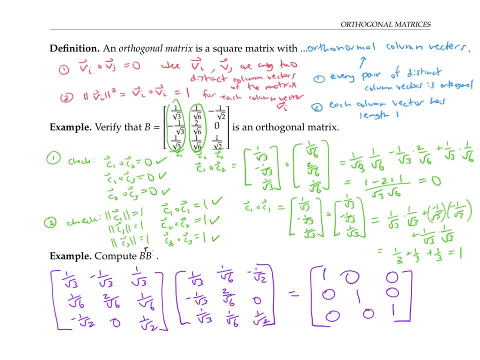 we'll always get one if we're taking the dot product of the column with itself. Therefore, our answer is the identity matrix And in fact the same reasoning shows that for any orthogonal matrix, when we take the transpose and multiply by the matrix itself, we're destined to get the identity. 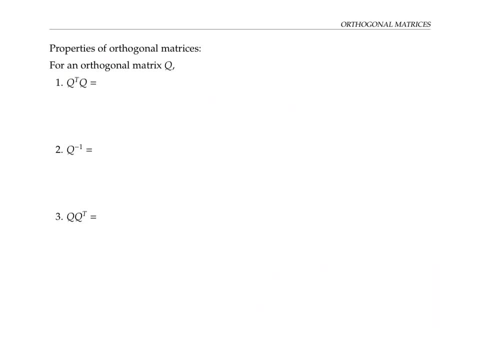 matrix. So that's our first nice property of orthogonal matrices. If we have an orthogonal matrix Q, then Q, transpose by times, Q is going to be the identity matrix. Another way of saying the same thing is that the inverse of an orthogonal matrix is just the same thing. 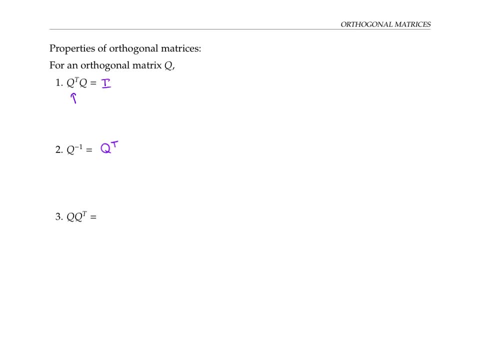 As its transpose right inverses are unique. So if any matrix times Q gives us the identity, that matrix has to be the inverse of Q. Finally, if I take Q times Q transpose the opposite order of what I did up here. that's the same thing as doing Q times Q inverse, And so I'll also get the identity. 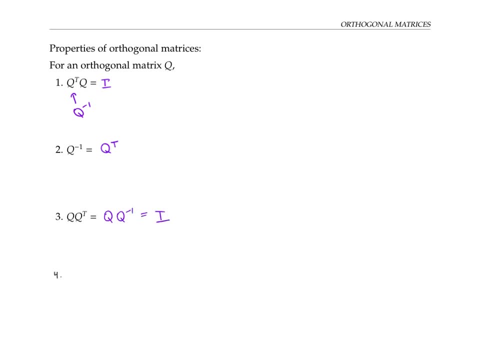 matrix this direction. That last property actually reminds me of one more nice property of orthogonal matrices, So I'll just give you a little hint here, for you to just get an idea why that works. This is the same thing When we take theV, which is the median, and then we multiply it by Q- transpose. 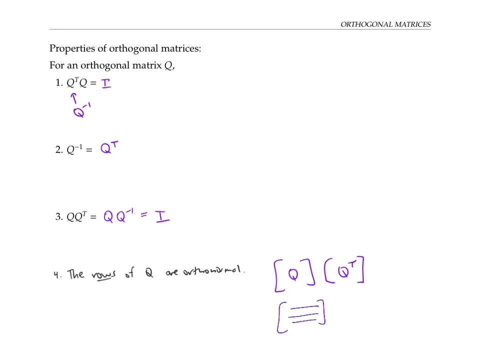 that becomes equal to the value of Q transpose. And you see that the value of Q transpose is equal to the value of the vector, because Q transpose is an orthonormal set and the other thing that happens is that we we think of entropy as a set of intervals. we mistakenly consider that to be the col. So let's say that we take the columns as an orthonormal set, but those columns are also an orthonormal set. That's because when we take Q times, Q transpose, we're multiplying rows of Q by the columns of Q transpose. but the columns of Q transpose are just coming from the rows of Q. Therefore, we're just multiplying the rows of Q by the rows of Q. 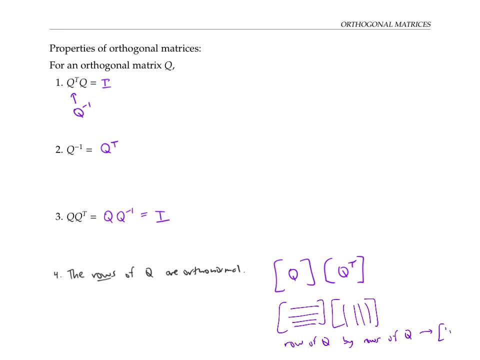 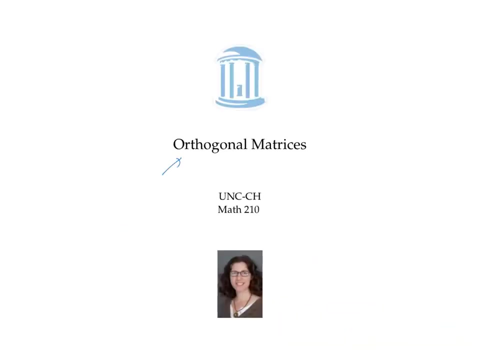 And since we're getting to the identity matrix, that means that each row dot product itself gives us one. each row dotted with a different row gives us zero. So those rows are orthonormal. In this video we saw that orthogonal matrices are matrices whose columns are orthonormal. 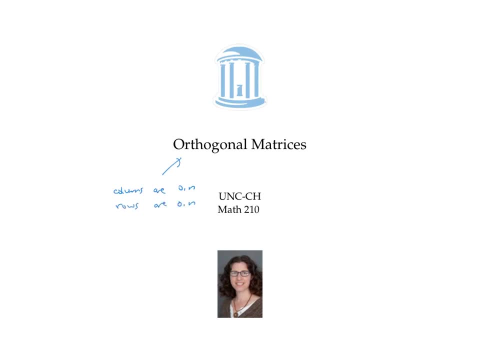 Also their rows are orthonormal. So if you take an orthogonal matrix, times its transpose in either direction you get the identity matrix. In other words, an orthogonal matrices, inverse is just its transpose. This video gives some facts about the eigenvalues and eigenvectors of symmetric matrices. 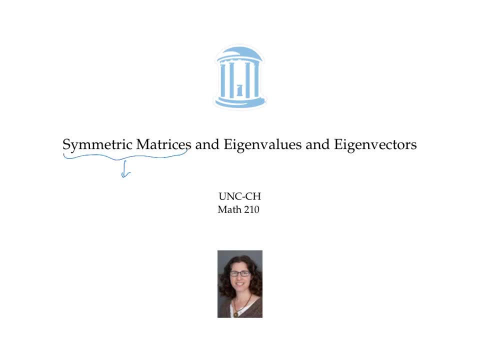 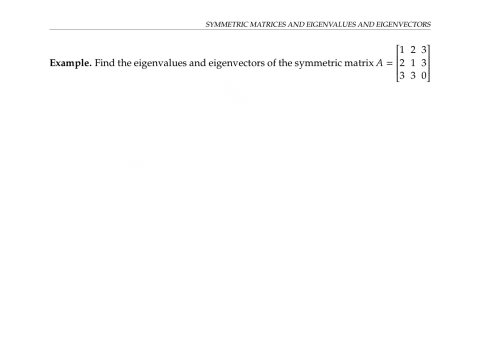 Recall that a symmetric matrix is a matrix like this one, whose transpose is equal to itself. Let's start by finding the matrix, Finding the eigenvalues and eigenvectors of this symmetric matrix. To find the eigenvalues, we'll write down: the characteristic polynomial, the determinant. 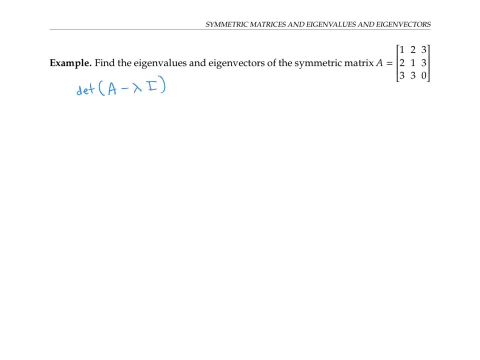 of a minus lambda i, the eigenvalues will be the values of lambda, for which that's equal to zero Lambda times. i is the diagonal matrix with lambdas on the diagonal. So when we subtract that from a, that amounts to subtracting lambda from each diagonal entry. 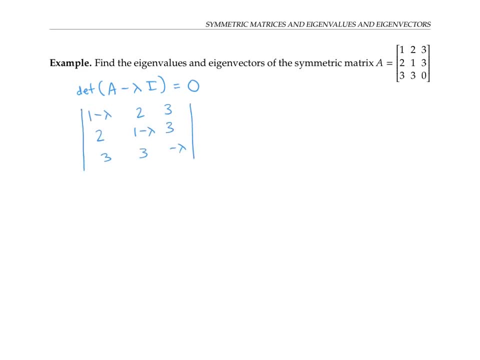 we need to take the determinant of that. So I'll expand along the first row And that works out to this expression which, after some algebra, gives us this polynomial: I'll set this equal to zero and I need to solve for lambda. 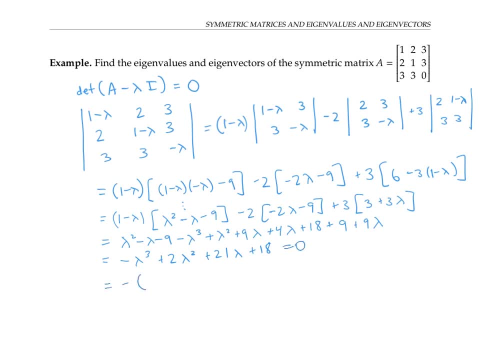 It turns out, this factors into the following expression. I figured this out using Wolfram Alpha and you're welcome to too. You can also figure it out by hand, knowing that the possible candidates for lambda are these roots, these solutions for lambda are going to be, plus or minus, the factors of 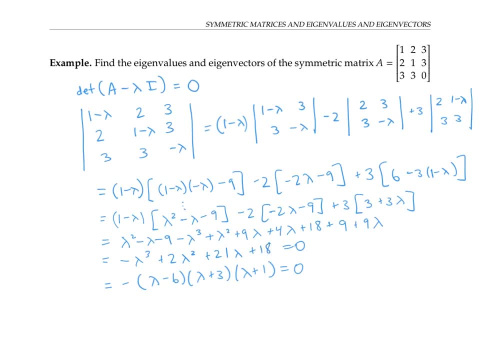 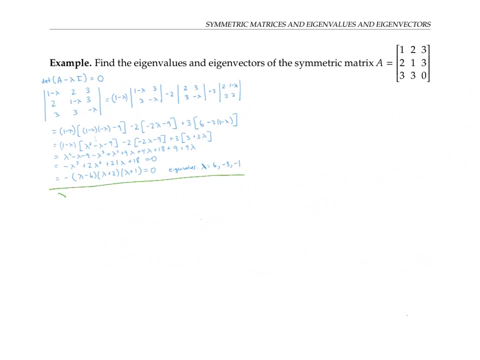 18. And then using long division. In any case, we now know what our eigenvalues are. they're going to be: lambda equals six, negative three and negative one. Next, let's figure out our eigenvectors. For the eigenvalue lambda equals six, we're going to be solving the equation a minus six. 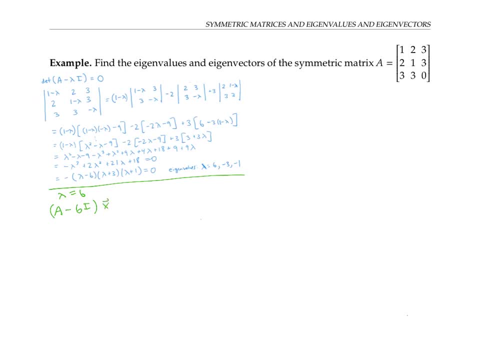 i Time some. vector x equals the zero vector. we can do that by writing down the augmented matrix with a minus six i here and then the zero vector here. So that's this matrix. I can solve by converting this to reduced row echelon form. I'm going 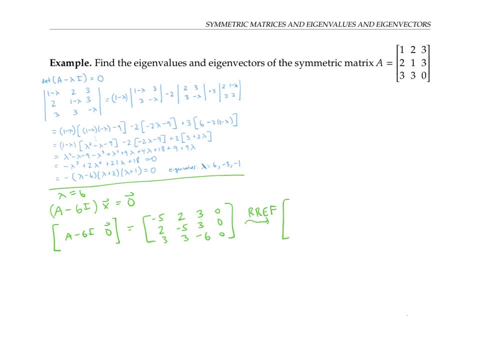 to admit the details. In fact I actually solved this using Python, But this is the answer And from here we can find the eigenvectors. Let's set x three as a free variable. We have x one minus x three equals zero, and x two minus x three equals zero. 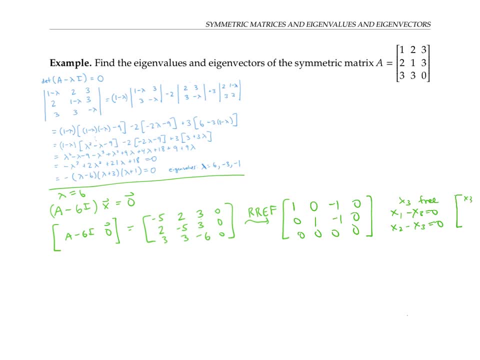 So the eigenvectors are the form x, three x three x three. In other words, they're of the form x three times the eigenvector 111. And I can just use 111 as an eigenvector. A similar computation for lambda equals nine. 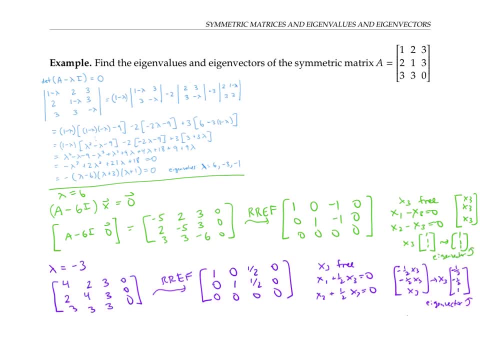 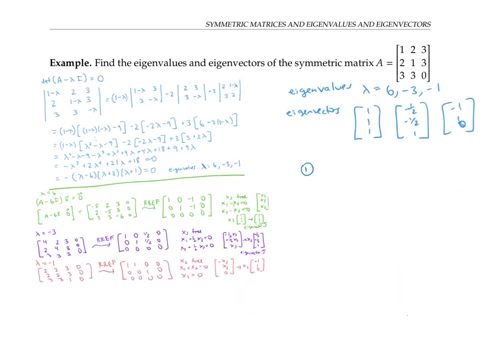 Okay, So negative three goes like this, And a computation for lambda equals negative one goes like this: Let me copy my eigenvalues and eigenvectors here and make some observations. First of all, the eigenvalues for this matrix are all real numbers. 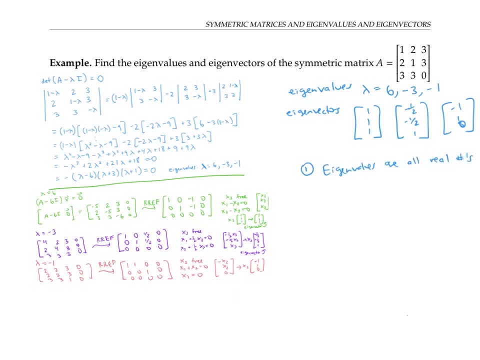 This may not seem so surprising to you, because we've been working with examples, intentionally with real eigenvalues, but it actually is significant. It turns out that for any symmetric matrix, It'll never have complex numbers as the solutions to its characteristic polynomial. it'll always. 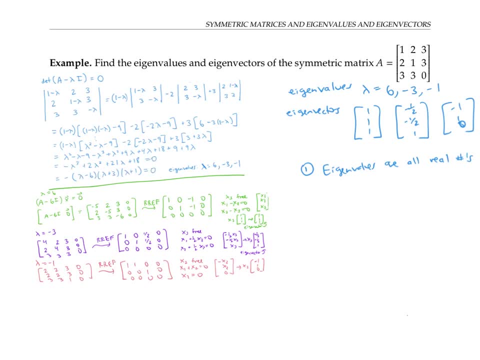 be just all real numbers. So that's the first kind of nice thing about symmetric matrices. The second thing that I want to point out is that all these eigenvectors are orthogonal. Let me give them names: v1,, v2, and v3.. 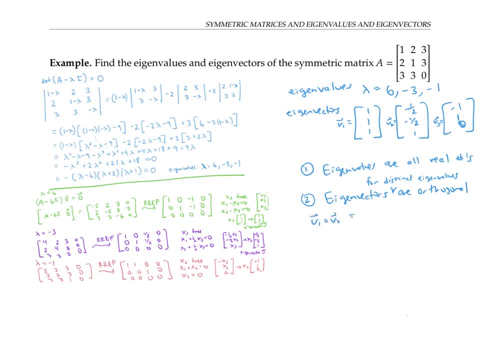 And now if I take v1 dot v2, I get zero. v1 dot v3. is zero, and v2 dot v3 is zero. This is no coincidence. In fact, this is true for any two eigenvectors of distinct eigenvalues for a symmetric matrix. 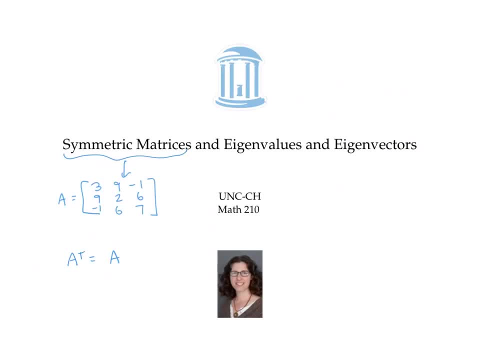 In this video we looked at an example that illustrated two important facts that are true about all symmetric matrices. the eigenvalues of symmetric matrices are always all real numbers- no non real complex numbers at all. And secondly, the eigenvectors of symmetric matrices for distinct eigenvalues are always 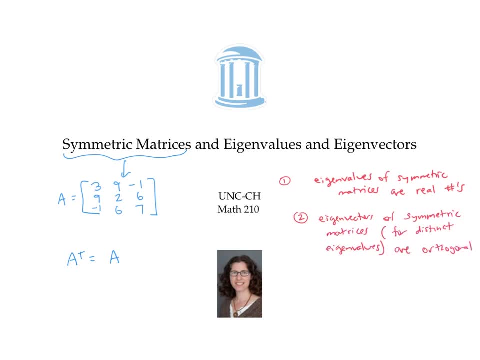 orthogonal. In other words, if v1 is the eigenvector for eigenvalue lambda one and v2 is the eigenvector for eigenvalue lambda two and lambda two, one is not equal to lambda two, then v1 dotted with v2 is zero. 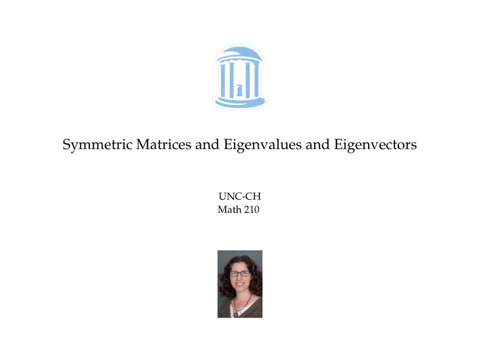 I'll show you the proofs of these facts in a different video. In a previous video, we stated two facts about the eigenvalues and eigenvectors of symmetric matrices. First, we said that the eigenvalues of a symmetric matrix are all real numbers. 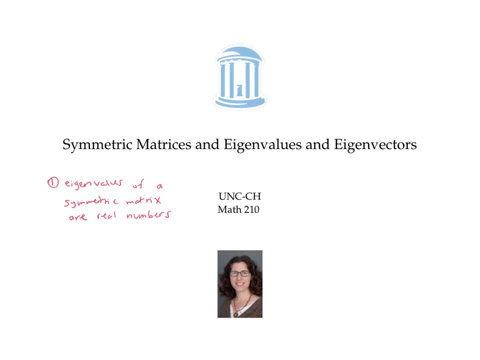 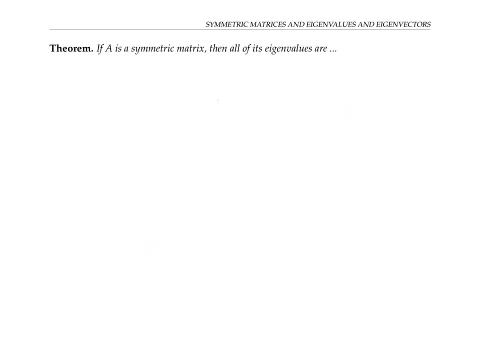 No complex numbers that aren't real occur as the roots of the characteristic polynomial. The second fact that we stated is that the eigenvectors of a symmetric matrix corresponding to distinct eigenvalues are orthogonal. This video gives proofs of these two facts. So the first fact we want to prove is that if A is a symmetric matrix, then all of its 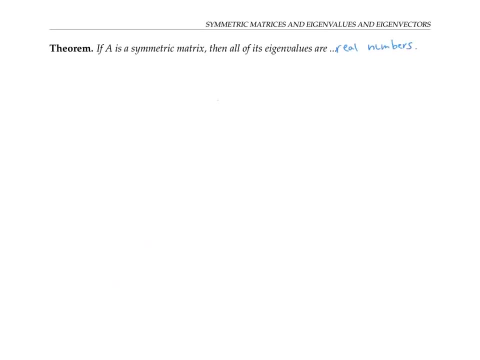 eigenvalues are real. All of its eigenvalues are real numbers. To prove this, let's suppose that lambda is an eigenvalue and v is an eigenvector for that eigenvalue. If we compute the length of A times v squared, remember that's the same thing as A times. 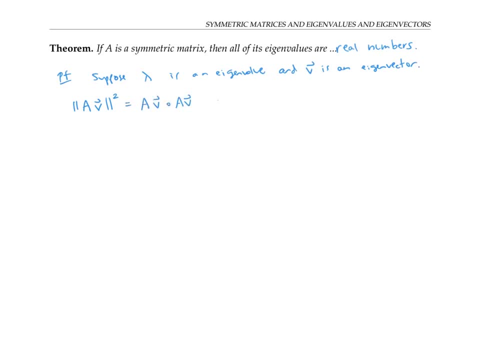 v dotted with A times v, Which is the same thing as taking the A times v vector, which is a column vector, transposing it to make a row vector and then multiplying by AV, which is a column vector, That matrix multiplication also multiplies corresponding entries and adds them up just. 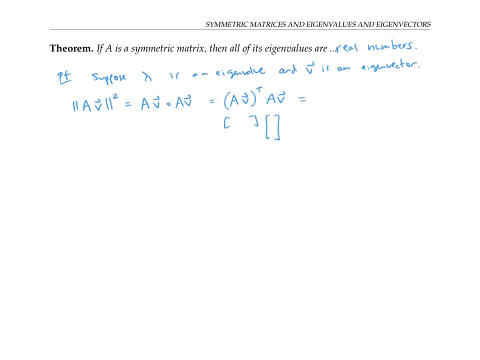 like dot product does. Now remember, when we take the transpose of a product, that's the same thing as doing the product of the transposes in the other order. So I can rewrite this as follows: And since A is symmetric, A transpose is just the same thing as A. Now, since V is supposed, 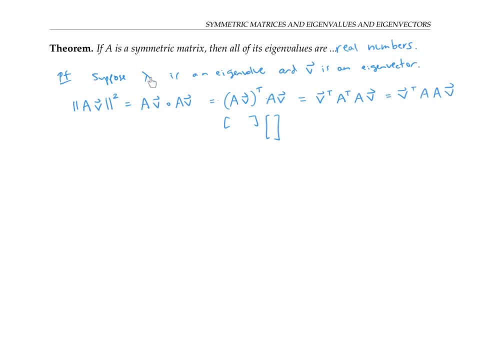 to be an eigenvector for the eigenvalue. lambda for A. A times v is just lambda times v. let me pull the lambda out. And once again, A times v is lambda times v. Once again, pull the lambda out. 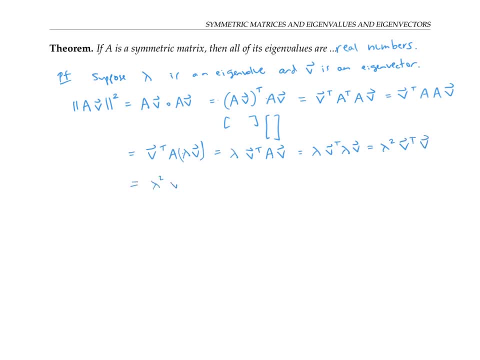 And v transpose times v is just the same thing as v dot v or the same thing as the length of v squared. Therefore, I put the far left side and the far right side of this string of equations together, I get the length of AV squared is lambda squared times the length of v squared. 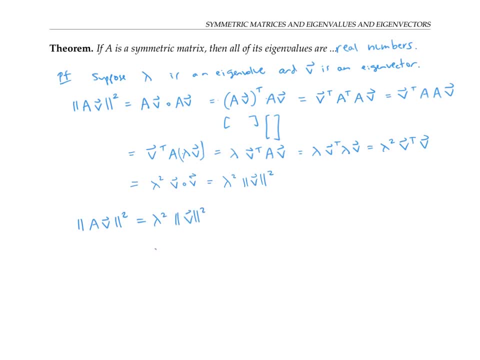 In other words, if I divide by A times v, I get lambda squared times the length of v squared. And if I divide by the length of v squared, I'm getting that lambda squared is the length of AV squared over the length of v squared. notice that it's legit to divide by the length. 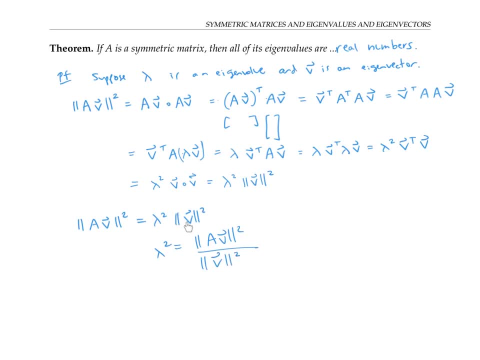 of v squared, because v is supposed to be an eigenvector, So it can't be the zero vector, So it can't have length zero. So then, not dividing by zero here. in fact, I have something on the numerator, that's. 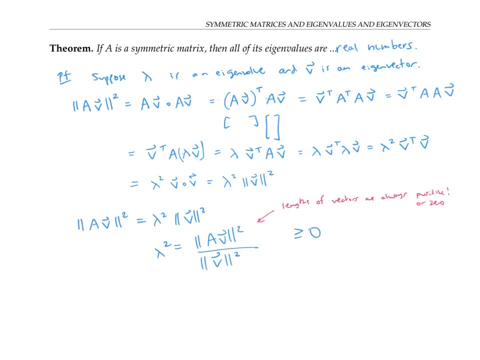 got to be positive or zero. A times v could actually be the zero vector if- if lambda is is a zero eigenvalue. And then on the bottom I have something that's just got to be strictly positive. When I divide something greater than or equal to zero by something greater than zero, I 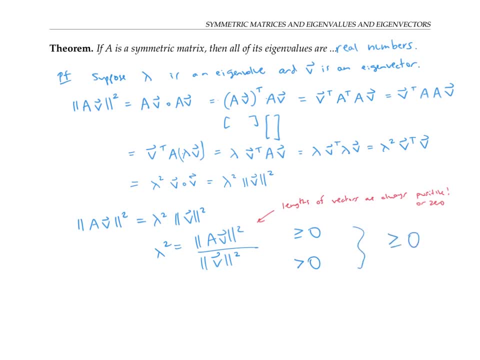 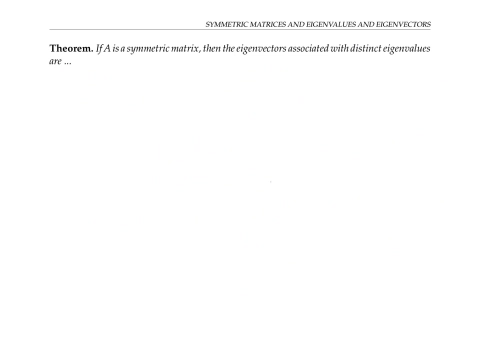 get something that's greater than or equal to zero. So lambda squared is greater than or equal to zero, which means I can take the square root of it And lambda is a real number. Next let's prove that if A is a symmetric matrix, then the eigenvectors associated with 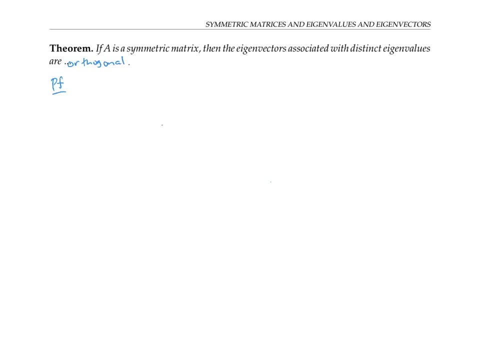 distinct eigenvalues are orthogonal, So let's take lambda one and lambda two to be distinct eigenvalues And as they're different numbers, So and let's let v one and v two be eigenvectors, for lambda one and lambda two respectively. 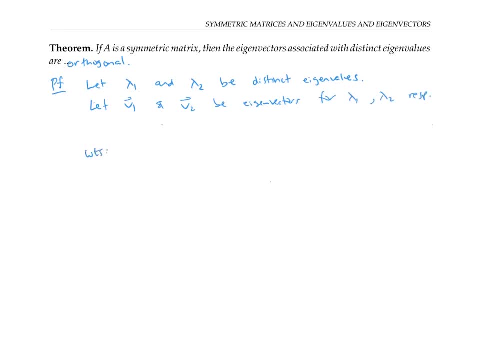 Okay, so what we want to show is that v one dotted with v two is zero, but I'm going to start instead by looking at lambda: v one dotted with v two, So that's the same thing as the matrix A times v one dotted with v two, which is the same. 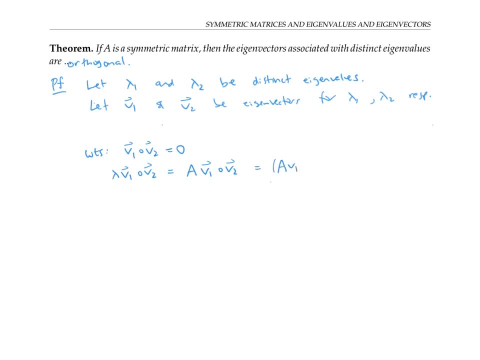 thing as taking a times v one, that column vector, transposing it to a row vector and multiplying, doing matrix multiplication with v two. Now I'll rewrite that transpose As v one: V one transpose, a, transpose v two. but a transpose is the same thing as a, since a is symmetric. 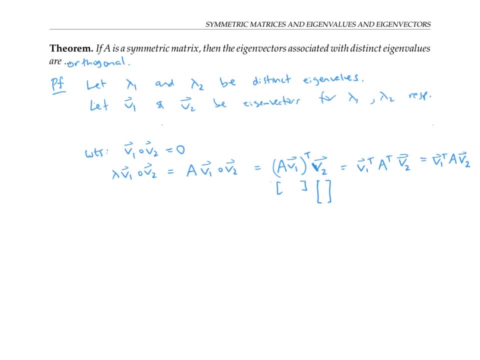 And since v two is an eigenvector of a with eigenvalue, lambda two, that's the same thing as v one transpose lambda two v two. So if I pull out the lambda two, v one transpose v two, that's the same thing as lambda two. 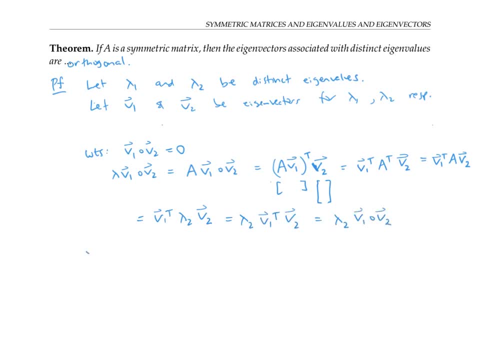 v one dotted with v two. Therefore I have lambda one times v one dot v two is equal to lambda two. v one dot v two. if I pull everything over to the left side and factor out the v one dot v two, I know that lambda one minus. 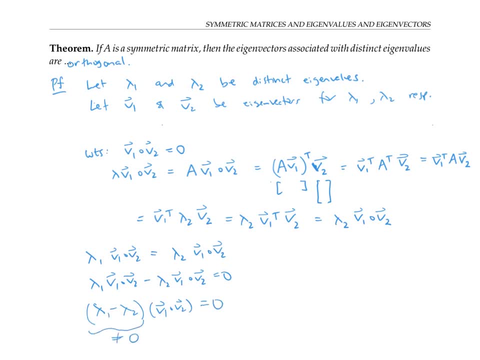 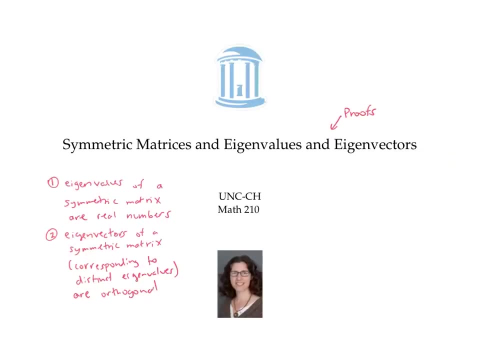 lambda two is not zero, since lambda one and lambda two are distinct and therefore v one dot v two must also be zero. So we've now proved these two facts about the eigenvalues and eigenvectors of symmetric matrices. The key components for the proof were the definition of eigenvalues and eigenvectors. 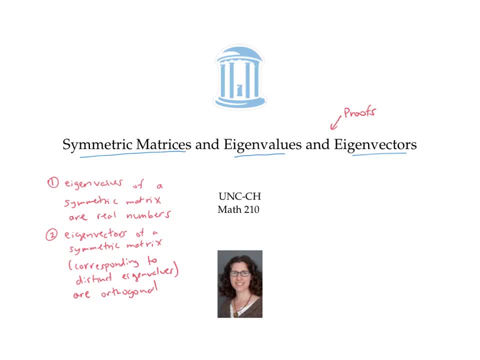 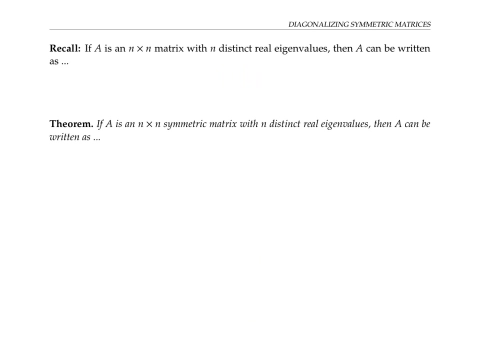 the definition of symmetric matrices and this key idea of rewriting dot product in terms of the transpose of the first vector to turn into a row vector matrix multiplied by the second vector, column vector. This video is about diagonalizing symmetric matrices. In the video about diagonalizing matrices in general, we saw that if we have a matrix, 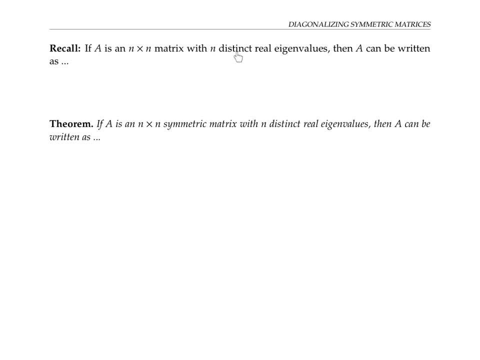 A, that's an n by n matrix with n distinct real numbers as our eigenvalues, then a can be written as a product of matrices: p times d times p inverse, Where d Is an n by n diagonal matrix And p is an n by n invertible matrix. 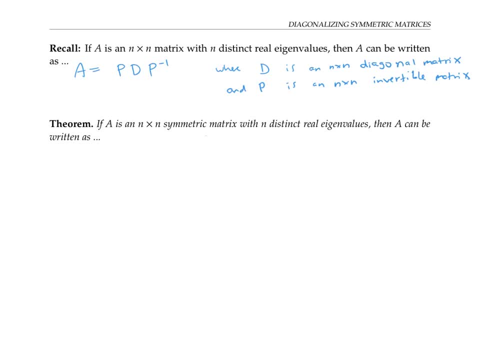 Writing a in this form is called diagonalizing a. we constructed the diagonal matrix D by stringing together all the eigenvalues of a and we constructed the invertible matrix p By stringing together eigenvectors for each of these eigenvalues as the column vectors. 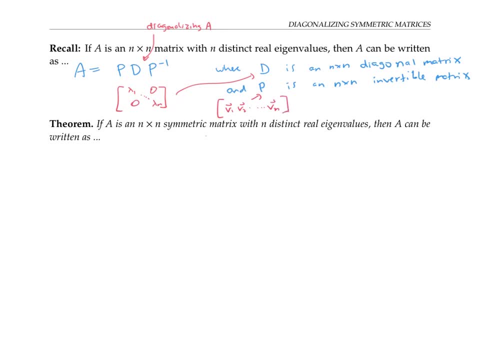 for p. Now suppose we add the condition that a is a symmetric matrix. That means that a transpose is the same as a. we still assume that it has n distinct real eigenvalues. then a can be written as a product of p times d times p inverse, where 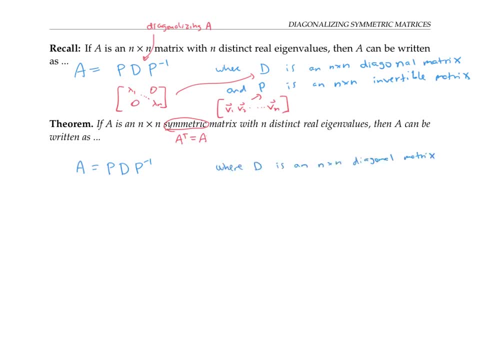 d again, is an n by n. diagonal matrix And p, this time is an n by n. orthogonal matrix. Recall that an orthogonal matrix is a matrix whose column vectors form an orthonormal set. Recall that an orthogonal matrix is automatically invertible because its inverse is given by: 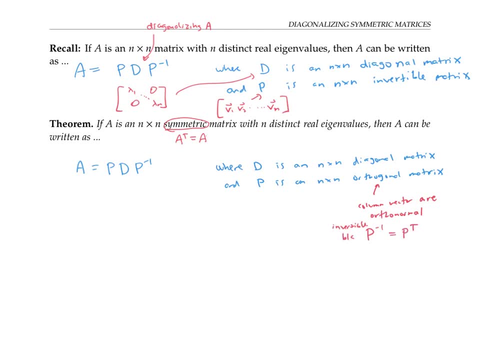 its transpose. So by starting with a symmetric matrix, a matrix with a little bit extra structure, then in our diagonalization we get p to be an orthogonal matrix, a matrix with also a little more structure. So how do we know that this is possible? 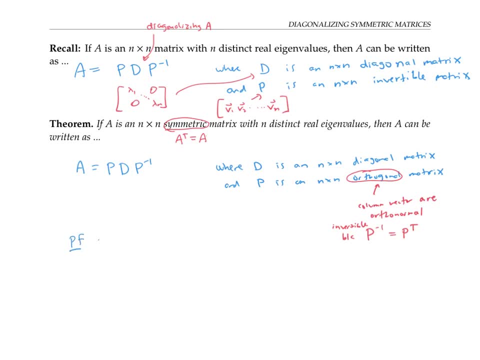 Well, we're going to use pretty much the same construction as we did before. We'll let D be the diagonal matrix, whose entries on the diagonal are the eigenvalues of a. Let's call those eigenvalues lambda one, lambda two through lambda n. 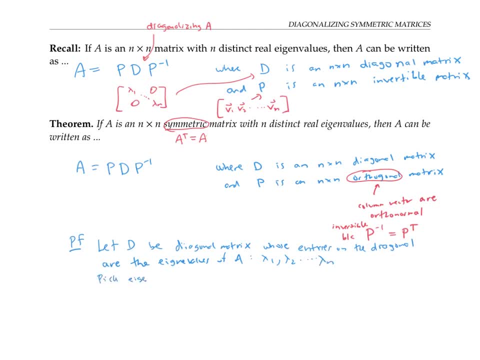 Now we'll pick an eigenvector for each eigenvalue And I'll call those v1, v2 through vn. So v1 is an eigenvector for lambda one, and so on. From the previous video on symmetric matrices and their eigenvalues and eigenvectors, we 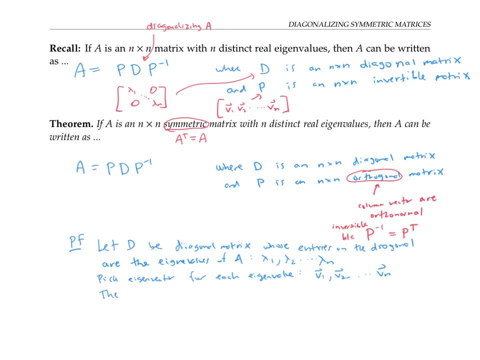 know that the eigenvectors, Okay, v1 through vn, are all orthogonal to each other. Well now, they might not be worth a normal, though they might not have length one. but let's just take w one to be v one divided by its length, and w two to be v two divided. 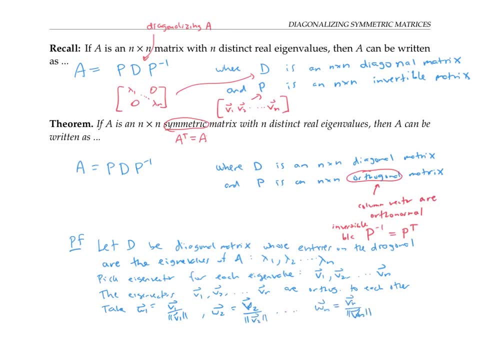 by its length and so on. Then the w ones through w, n's: Okay, Okay, Okay, Okay, They'll still be orthogonal, but they'll also have length one, So they will be an orthonormal set. If you're worried about why they're still orthogonal to each other, just consider, say: 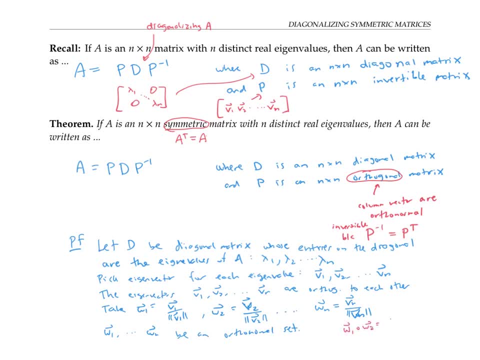 w one dotted with w two. that's v one just rescaled, dotted with v two rescaled. and if you pull out the scalars then you just have a real normal set. So you have a real number times: v one dot v two. 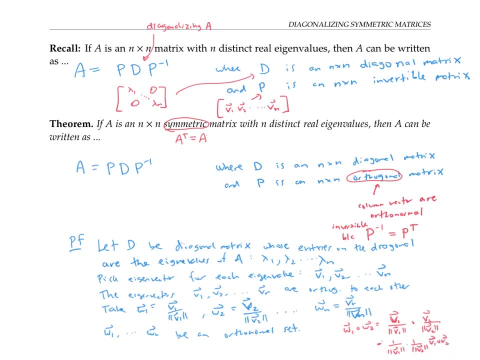 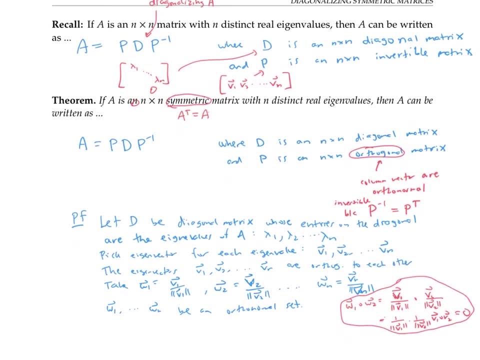 And since these were already orthogonal, their dot product is zero And therefore the dot product of w one and w two is still zero. So now we're going to take this orthonormal set of vectors, w one through w n, and we're 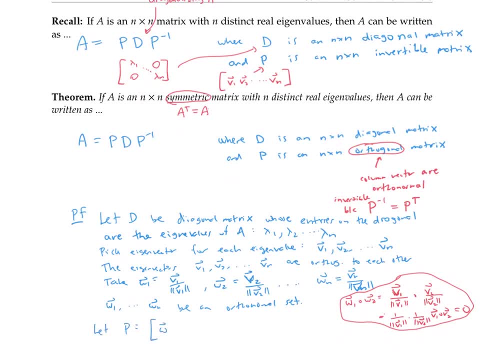 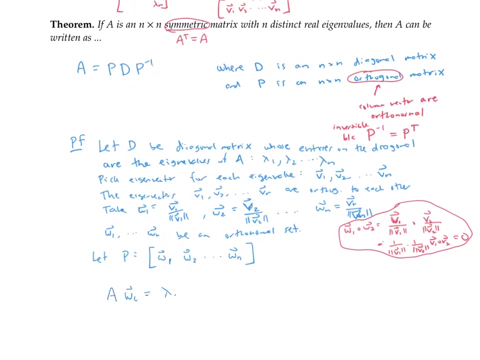 going to let p be the matrix we get by putting those column vectors together into an n by n matrix. Since we have that A times any of the w eyes is equal to lambda i times wi. We know that a times the matrix of the w eyes all stuck together is going to be this matrix. 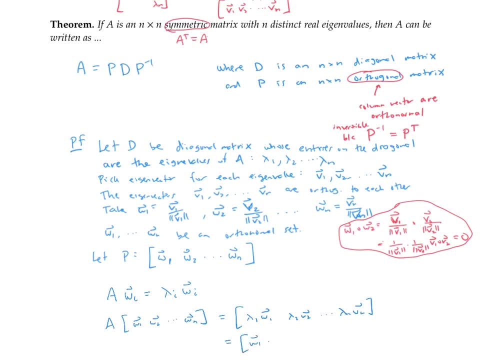 But the matrix on the right side is just exactly what we get by taking the matrix with columns w, one through w, n, and multiplying it by this diagonal matrix. If you think about what happens when you compute each entry of this product, you'll see that. 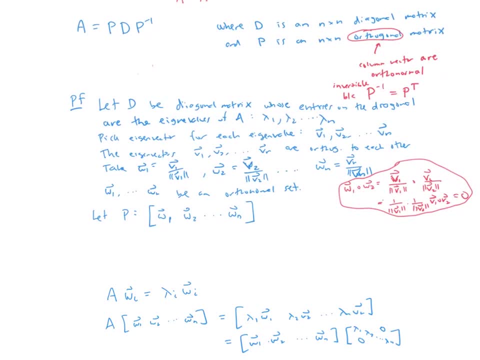 this is what you get. So now we have that a times p- because this is our matrix we called p- is equal to p times d, our diagonal matrix, And therefore a is equal to p times d times p inverse. Multiplying both sides of this equation by p inverse on the right: 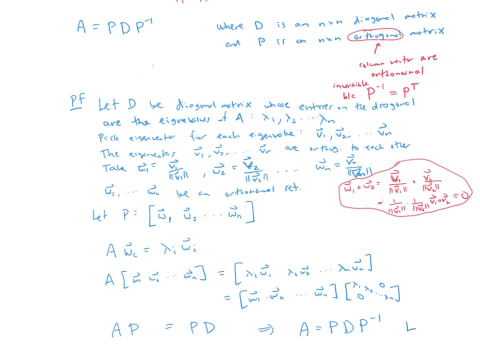 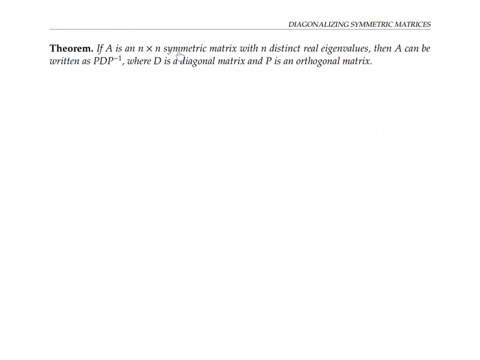 So we've diagonalized a, And because we started with a symmetric matrix and just made sure our eigenvectors were rescaled to be length one, we ended up with an orthogonal matrix for p. So this is what we just proved: if a is an n by n, symmetric matrix with n distinct real. 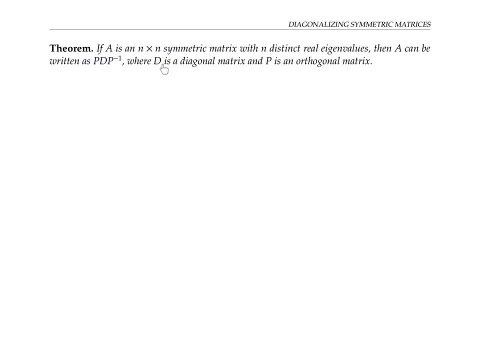 eigenvalues, then a can be written in this form: D is a diagonal matrix, P is an orthogonal matrix, But in fact, as you might have noticed, we don't actually need to state that these eigenvalues for a are real, Because if a is a symmetric matrix, its eigenvalues are automatically real. 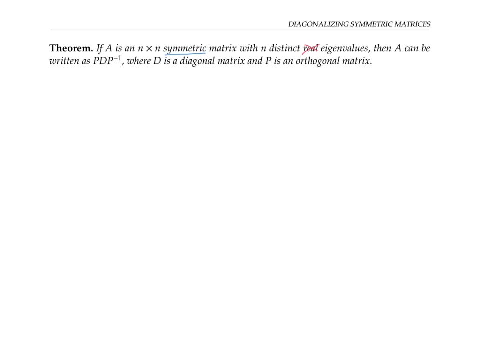 So that was kind of a redundant statement there. In addition, it turns out- although I won't prove it here- that we don't even need to know that a has distinct eigenvalues. it could have the same eigenvalue repeated, Okay. 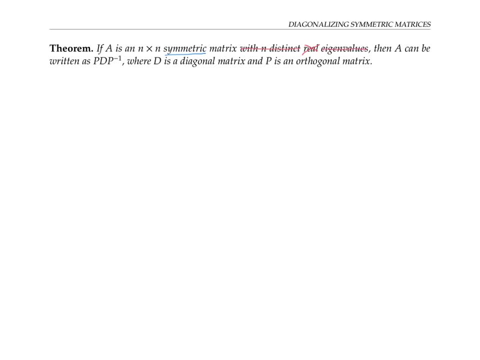 It could be repeated twice or more like that could. that eigenvalue could be a multiple root of the characteristic polynomial And we would still be able to write a. diagonalize a in this way. Let's finish with an example. Let's orthogonally diagonalize the matrix given here. 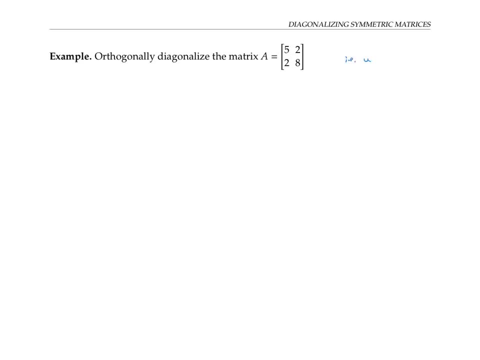 Orthogonally. diagonalize means we write a as p d. Okay, So we're going to write a as p d. Okay, So we're going to write a as p d. p inverse, where this is a diagonal matrix And this is an orthogonal matrix. 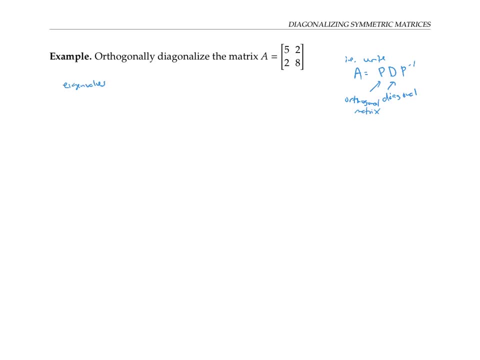 So to do this, we need to start by finding the eigenvalues, since that's what's going to go into our diagonal matrix D. So I'll write down the characteristic polynomial That determinant works out to this expression, which factors into lambda minus nine times. 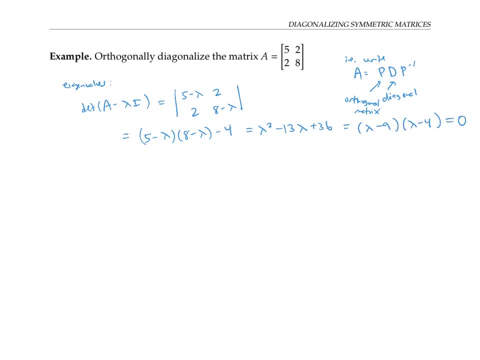 lambda minus four. Okay, So if that equal to zero, I see that my eigenvalues are going to be nine and for next I'll compute the eigenvectors for each of these eigenvalues. So for lambda, one equals nine. I'm solving a minus nine. i times some vector equals a. 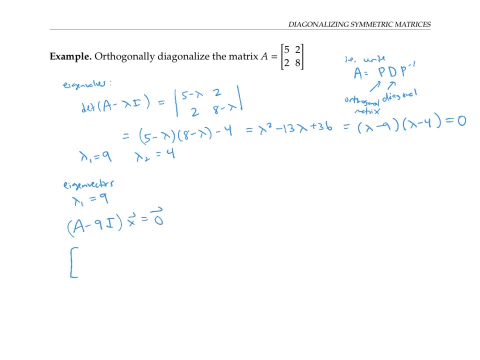 zero vector, the matrix a minus nine. i is this matrix which I'll rewrite as an augmented matrix and row reduce as follows: I'll let x two be a free variable And I know that two x one minus x two is zero. So x one is one half x two. 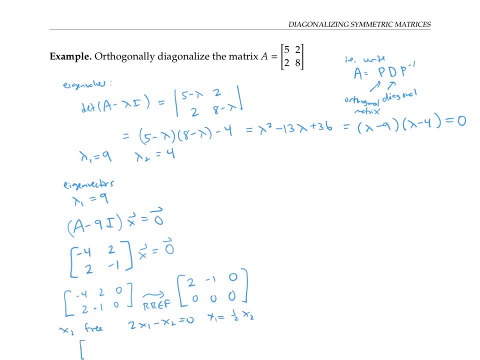 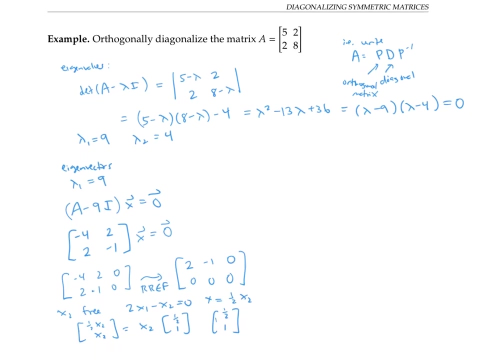 So I have eigenvectors of the form one half x two x two, or that is x two times one half one, And so I can use one half one as an eigenvector, except I want all my eigenvectors to have length. 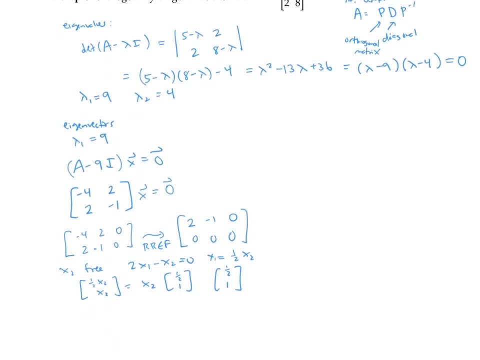 one. So there'll be an orthonormal set And the length of this eigenvector, I'll call it v one. length of v? one is the square root of one half squared plus one squared, the square root of five fourths, or the square. 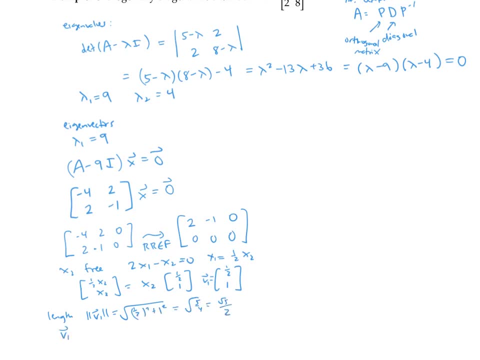 root of five over two. So I need to use v one over its length, which works out to: let's see one half divided by square root of five over two and one divided by square square root of five over two. that simplifies to one over square root of five and two over 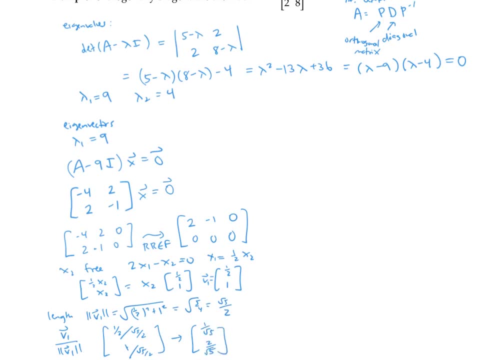 square root of five. Notice that this rescaled eigenvector is still itself an eigenvector. It's like using this eigenvector where x two was one over square root of five over two, I can find the eigenvectors for the eigenvalue lambda. two equals four. 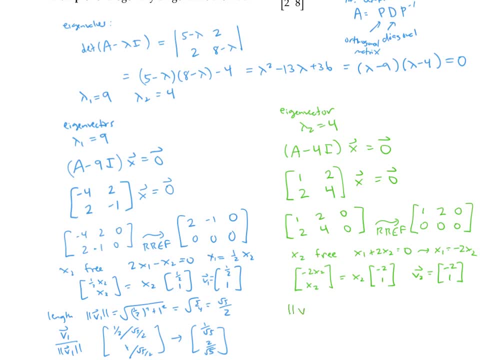 Once again, the length of the eigenvector that I found is not equal to one. in this case, its length is equal to the square root of five. So, as before, I just rescale my eigenvector by dividing by its length. 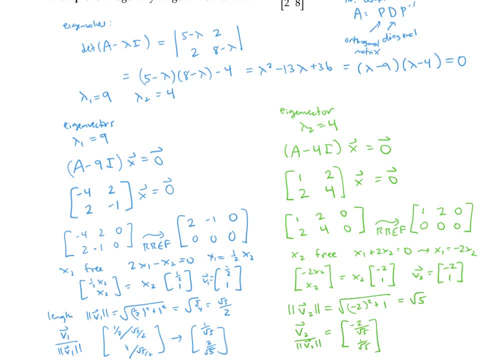 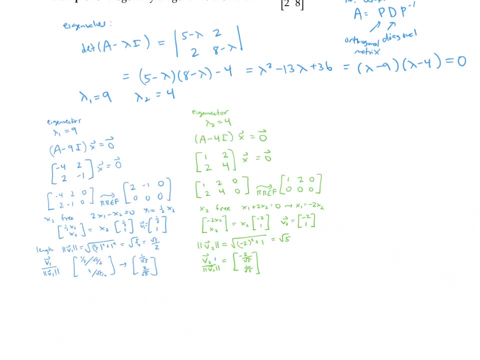 Now that I find found my eigenvalues, found corresponding eigenvectors and made them length one, I'm ready to construct my matrices D and P. The diagonal matrix D- Okay, We'll have its diagonal entries from the eigenvalues And the invertible matrix P will have its columns from these length one eigenvectors. 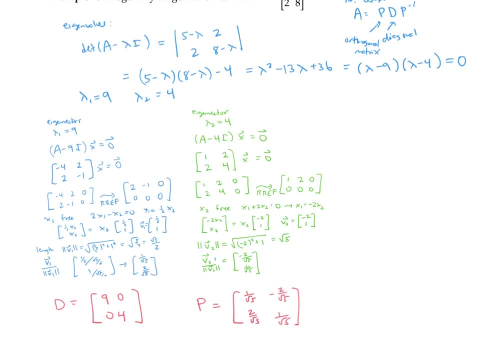 that we just found. I invite you to check that this matrix P really is an orthogonal matrix And that if you find its inverse, which is just its transpose, and then take P D- P inverse, you get back to the original matrix A. In this video we worked out how to diagonalize. 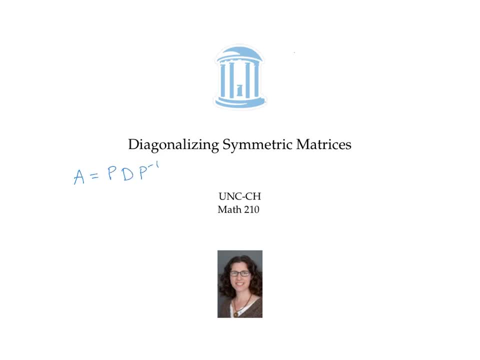 a symmetric matrix A by putting the eigenvalues of A into the diagonal matrix D and putting eigenvectors of A as the columns of the matrix P after short, first making sure to rescale those eigenvectors to have length one. When we do that. 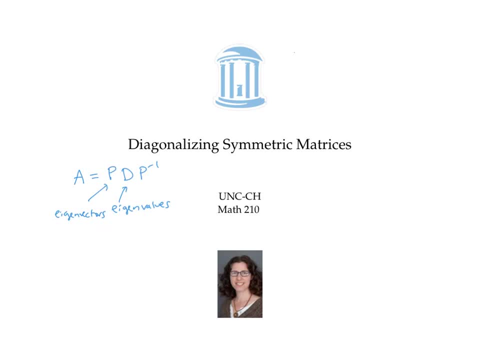 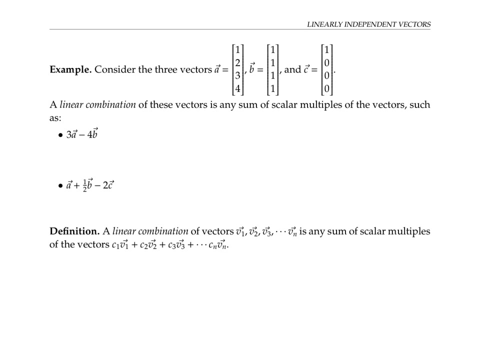 We end up with a matrix for P that's not only invertible but actually orthogonal. This video is about linearly dependent and linearly independent vectors. Consider these three vectors: A, B and C. A linear combination of these vectors is any sum of scalar multiples of the vectors, such as three times A minus four times B. 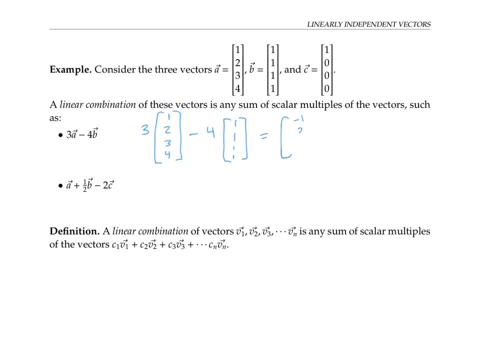 which works out to the vector with entries minus one, two, five, six, seven, eight, nine five, eight. Another linear combination would be: A plus one half, B minus two, C, which works out to the vector with entries minus one half, five halves, seven halves, nine halves. 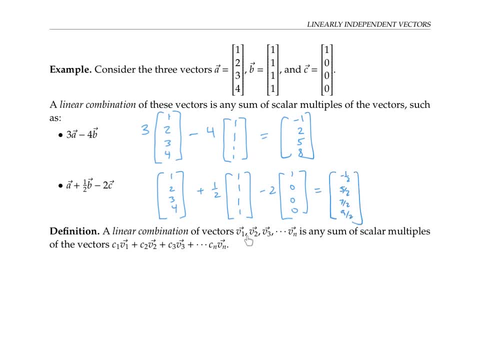 And, in general, a linear combination of vectors- v one through v- n is any sum of scalar multiples of the vectors. we can put in any real numbers for C one through C n, including zeros and including negative numbers, which is why we could think of this subtraction as really. 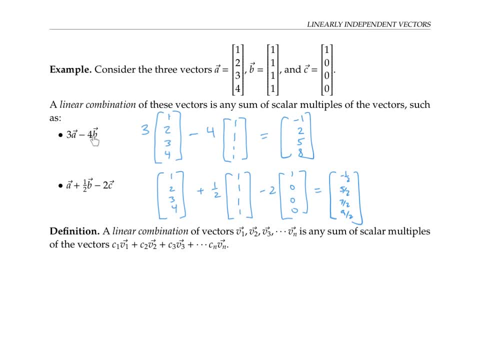 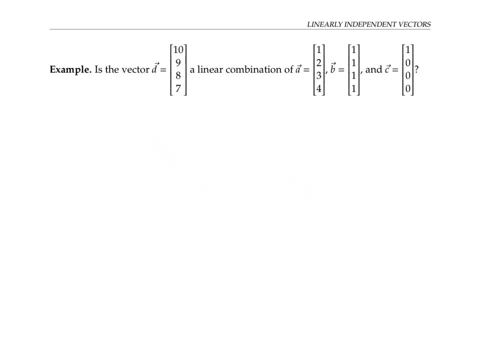 a sum where one of the coefficients is negative four. So let's try to figure out if this vector D is a linear combination of A, B and C. In other words, can we write D as some like x one? some number x one times a plus x two? 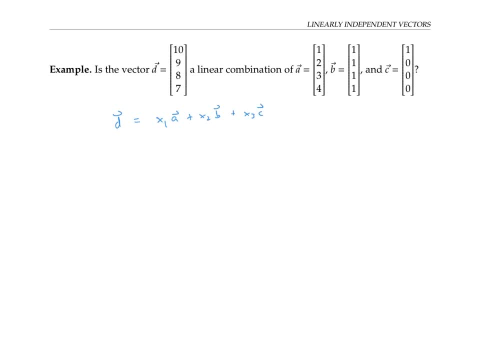 times B plus x, three times C. we could write this out as follows: Or we could even write it out as a system of linear equations. Recall that solving a system of linear equations like this can be done by row, reducing the augmented matrix, where we augment by the constant terms that here we're on the left. 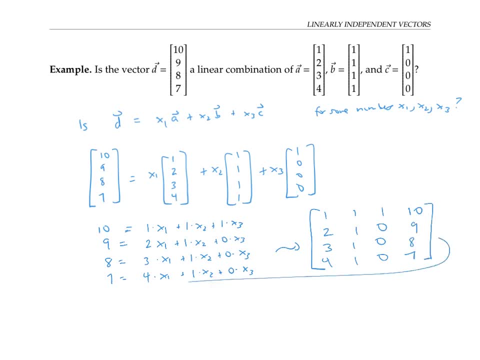 side of our equations. I'll omit the details of row reducing and just write down the final form, which tells us that we can indeed solve this system of linear equations with x one equals negative one, x two equals 11. And x three equals zero. 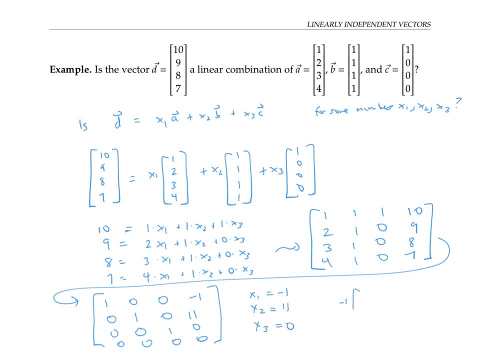 As a check, if we write down negative one times the vector A, plus 11 times the vector B, plus zero times the vector C, we do indeed get the vector 10987.. So D is indeed a linear combination of A, B and C. 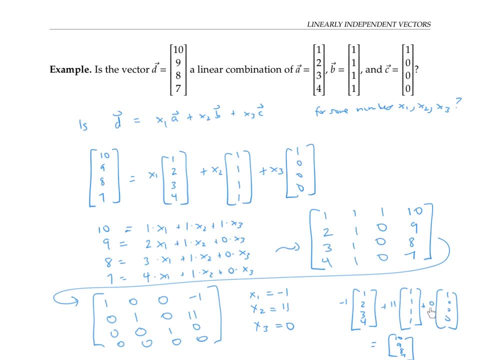 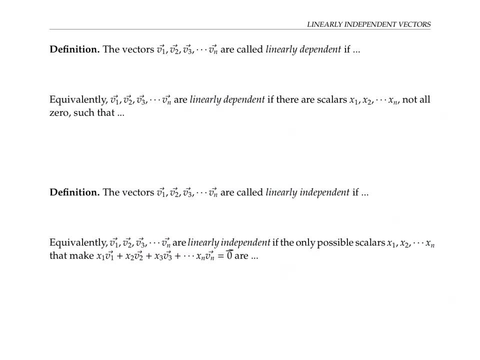 In fact we do. We didn't even need C. the coefficient of C ended up being zero. The set of vectors v1 through vn are linearly dependent if at least one of the vectors can be written as a linear combination of the others. 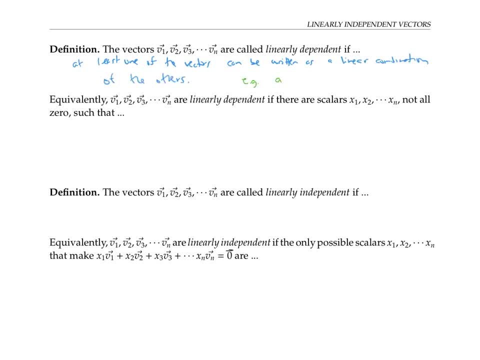 So in the previous example A, B, C and D were linearly dependent because vector D could be written as a linear combination of the others. Equivalently, we can say that v1 through vn are linearly dependent If there are scalars x, one through x, n, not all of them zero. 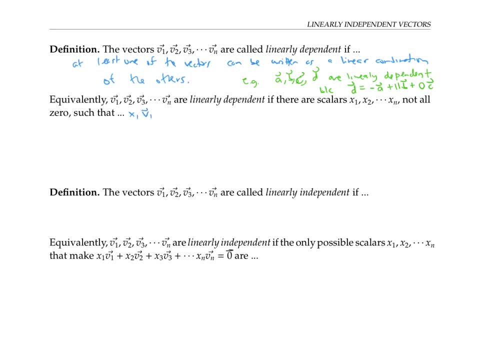 Such that x one times v one plus x two times v two plus all the way through x n times v n is equal to the zero vector. specifying that the x- i are not all zero is important because we could always make the sum equal to zero just by making the x's all equal to. 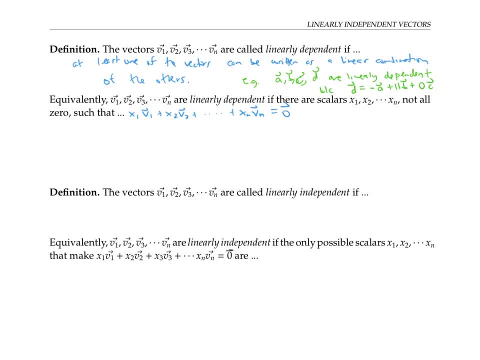 zero. Let's see why these two definitions are equivalent. Suppose we have the statement of definition one that one of the vectors can be written as a linear combination of the others. let's say say, for example, v3 can be written as: 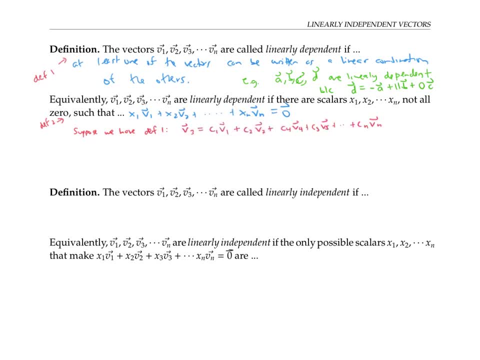 a linear combination of the other vectors, then we can get an expression like the one in definition two just by subtracting over v3 to the other side. So we have exactly the expression from definition two, with the C's functioning as the x's and. 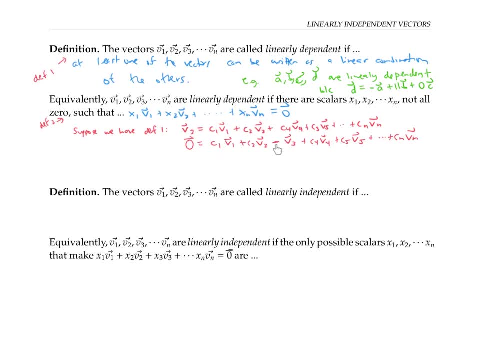 notice that the these x's are not all zero, because the coefficient of v3 is negative, one, which is not zero, And conversely, suppose we have the condition and definition two. So we have an expression like this, where all the x's aren't zero but the sum is zero. 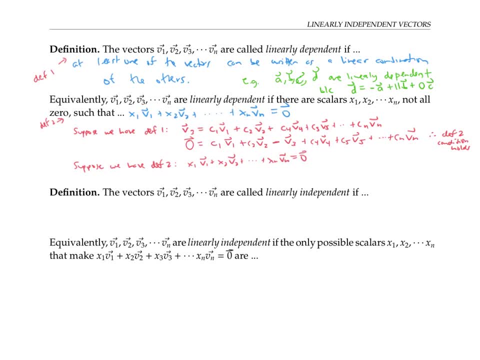 then we can just find an x that's not zero. let's say say x four is not zero and use that to solve for v four in terms of the other V's. So we can write x four times v four in terms of all the other V's, and then just divide. 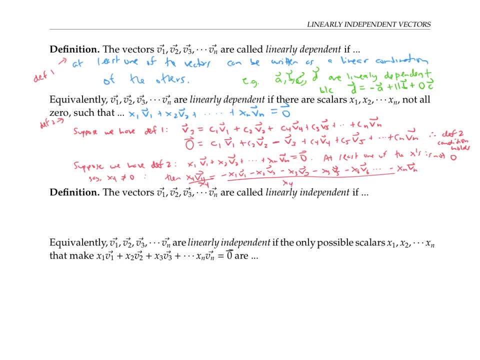 both sides by x four, Which is a number that's not zero, to isolate v four and get v four as a linear combination of the other vectors, which is exactly the condition we need for definition one. So enough about linearly dependent vectors, let's talk about linearly independent vectors. 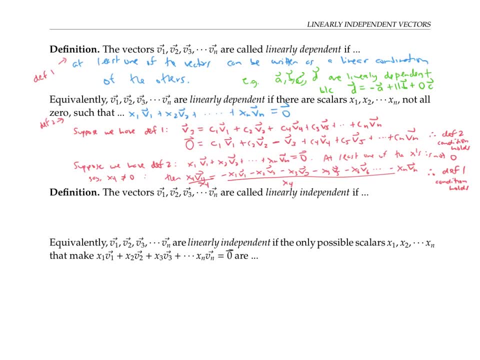 Well, there are vectors that are not linearly dependent, In other words, in terms of definition, one, the vectors v. one through v n, are called linearly independent If it is not possible to write any one of the vectors As a linear combination of the others, or thinking in terms of definition to the vectors. 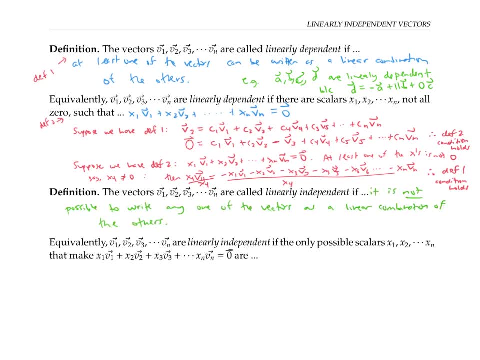 v one through v, n are linearly independent. If it's not possible to write an expression like this one, where multiples of the vectors add up to zero, except for if those coefficients, x, one through x n, are all zeros, So the vectors are linearly independent. the only possible scalars x, one through x n, that 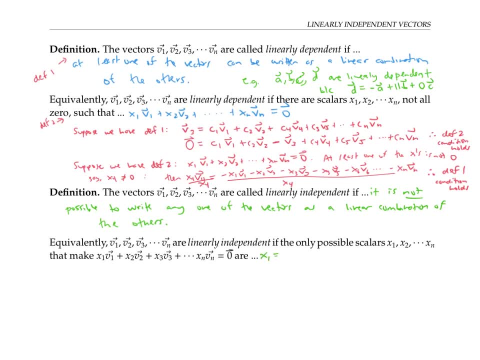 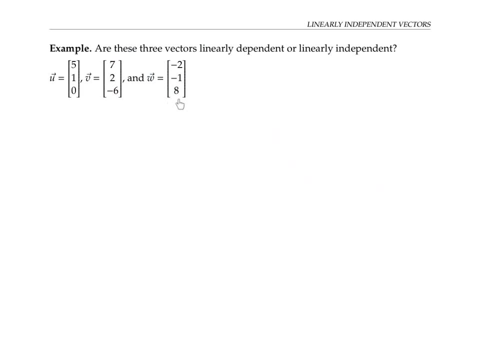 make this expression. zero are x one equals zero, So x two equals zero and all the x's are zero. So let's see if these three vectors are linearly dependent or linearly independent. One way to do that is to write down the equation: x one times u plus x two times v plus x three. 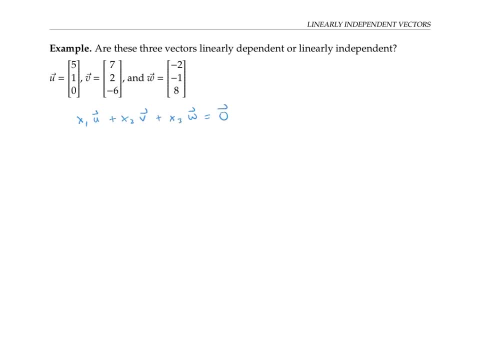 times w equals the zero vector- and see if we can find solutions for x one, x two and x three that are not just all zeros. I can rewrite this equation as follows, Or I can write it as this: system of linear equations: Solving the system of linear equations can be done by writing down the augmented matrix. 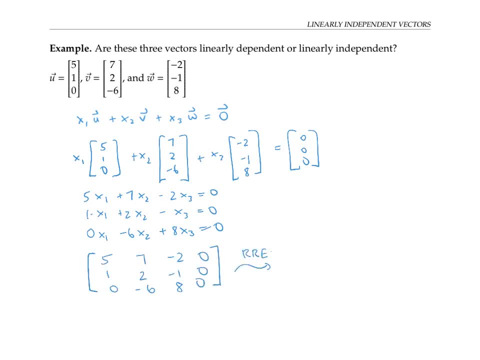 and converting it to reduced row echelon form. Once again, I'll omit the details of row reducing it, and just write down the final answer. From this matrix we can see that the only solution is that x one is zero, x two is zero. 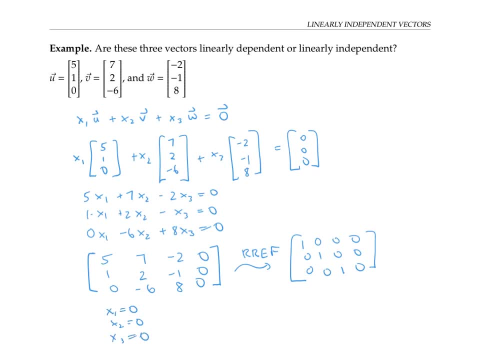 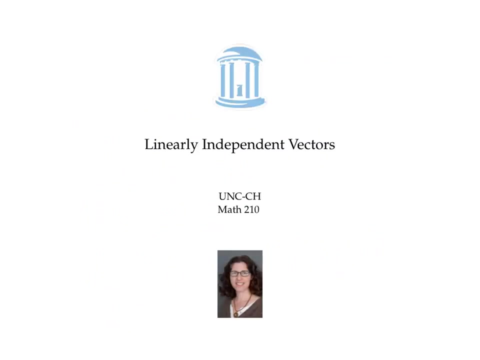 and x three is zero, So there are no other solutions Besides the x's all being zeros. So that means that these three vectors are, in fact, linearly independent. In this video we defined linearly dependent and linearly independent vectors. 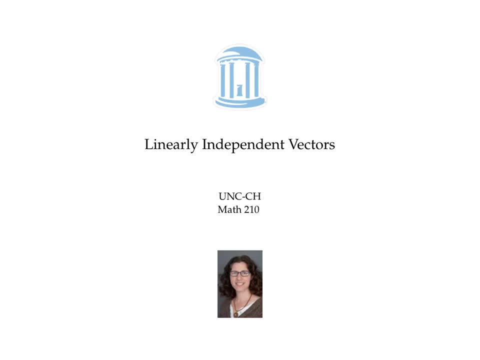 Linearly dependent vectors are redundant. in some way you can find a vector in the group that can be written as a linear combination of the other vectors, Whereas you can think of linearly independent vectors as all being necessary for the collection. you can't write any one of them as a linear combination of the others. 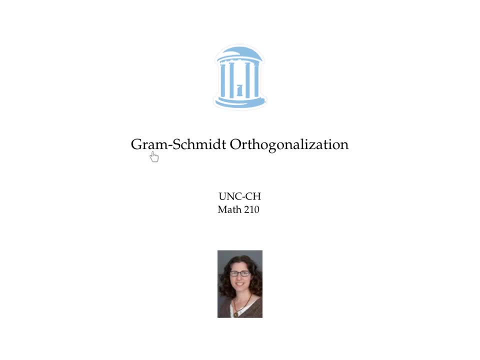 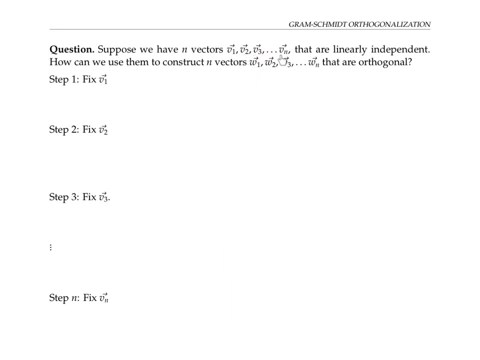 This video gives an algorithm known by the name of Graham Schmidt to convert a set of linearly independent vectors into a related set of orthogonal vectors. So suppose we have n vectors, v1,, v2,, v3, all the way through vn- that are linearly independent. 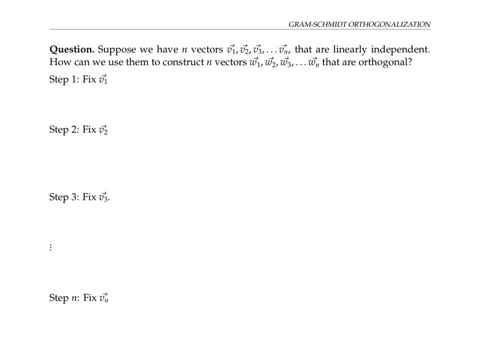 Recall that this means that none of these vectors is a linear combination of the others. How can we use them to construct n vectors, w one through w n, that are orthogonal? Recall that two vectors are orthogonal if their dot product is zero. So I'm going to show you an algorithm to do this. 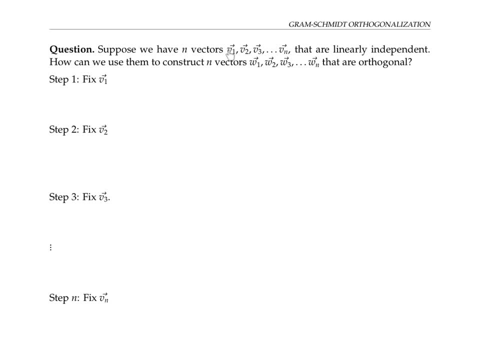 And this algorithm basically replaces one vector at a time, building up a bigger and bigger collection of orthogonal vectors. So we'll start with v one. we don't actually need to fix v one, we'll just let w one- Okay, be exactly the same thing as v one. 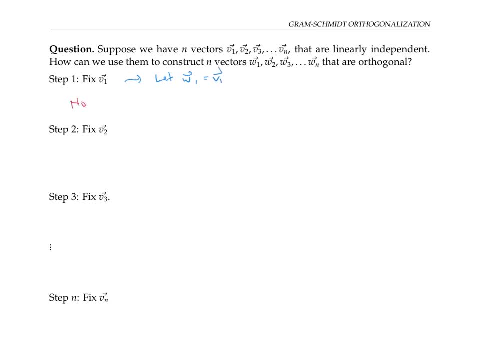 I want to note, because we're going to need to use this in a moment. I want to note that w one is not the zero vector, or in other words, v one is not the zero vector, And that's because we assume that we started with a bunch of linearly independent vectors. 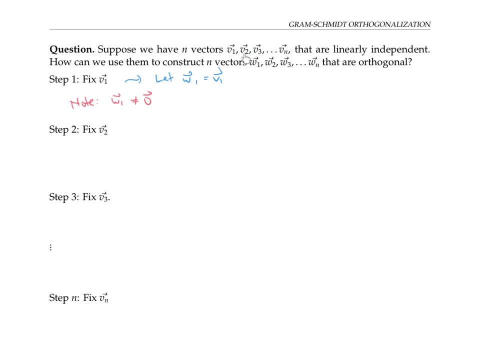 If this first one were the zero vector, then this set of vectors wouldn't be linearly independent, because you can always write zero as a linear combination of a bunch of others things, just by letting the coefficients all be zeros. Okay, so now I've hopefully convinced you that w one is not the zero vector. 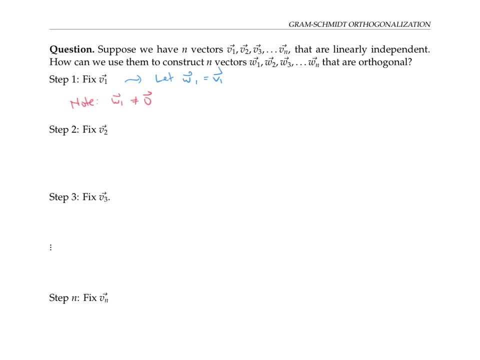 And we're going to go on to the next step, which is to fix v two. v two might need some fixing because it's not automatically going to be orthogonal to v one unless we modify it. So here's how we're going to modify it: we're going to let w two be the same thing as v. 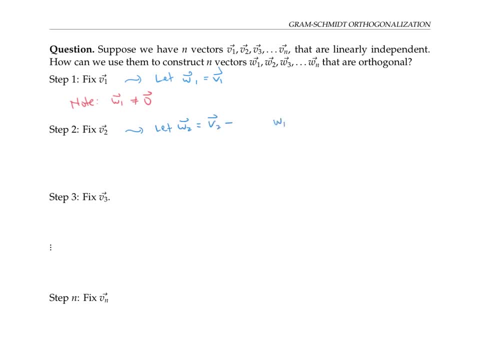 two minus some multiplications. Okay, So v two is going to be the multiple of w one, And that multiple is going to be given by v two dotted with w one divided by w one dotted with w one. notice that this expression here is a scalar, because dot products give us scalars. 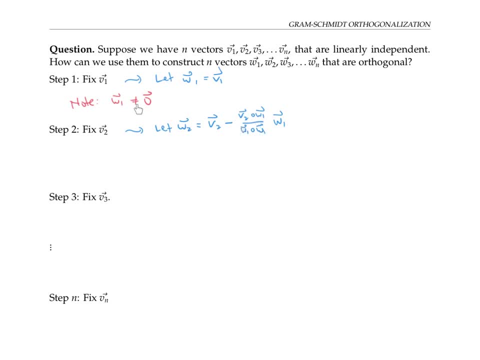 And we didn't divide by zero, because w one is not the zero vector, So it's dot product itself can't be zero, So w two is a legitimate vector. And now Let's see what happens when we take w two and dot it with w one. 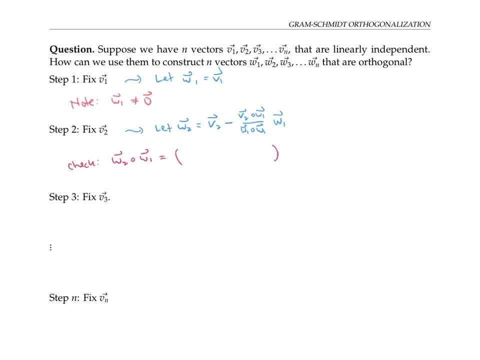 That's the same thing as taking this expression for w two and dotting it with w one. Let me distribute the dot product And now the w one, dot w one is going to cancel out And I'm left with this expression: v two, dot w one minus. v two, dot w one. 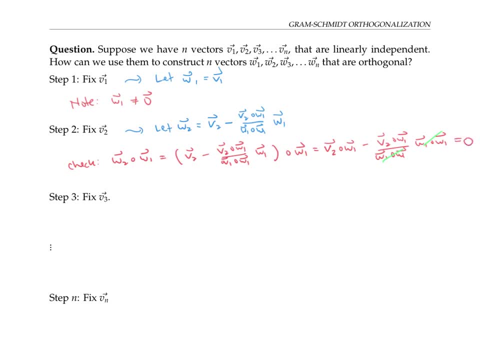 So that's going to go to zero. Therefore, w two Is orthogonal to w one, And we've made a good start. we now have two vectors- w one and w two, that are orthogonal to each other. Note also that w two is not going to be the zero vector. 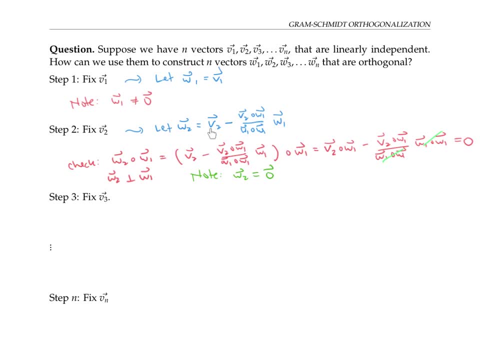 That's because w two is a linear combination of v two and w one, w one being the same thing as v one. So w two is a linear combination of v two and v one And since these v vectors are linearly independent, we can't get a linear combination of them. 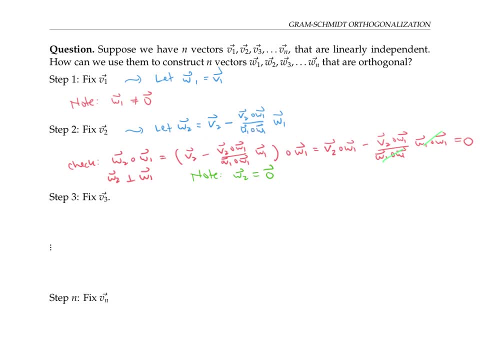 equaling zero, unless the coefficients are all zero, and the coefficient of v two is one, not zero. Let's continue by fixing up v three using the same ideas. So we're going to let w three the v three minus a multiple of w one minus a multiple. 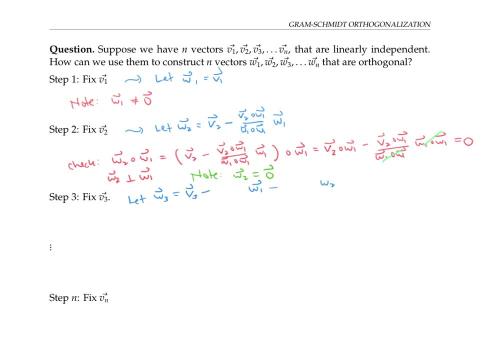 So we're going to let w three be v three minus a multiple of w one minus a multiple of v one. The multiple of w one is going to be given by v three dot w one over w one dot w one And the multiple of w two is going to be given by v three dot w two divided by w two dot. 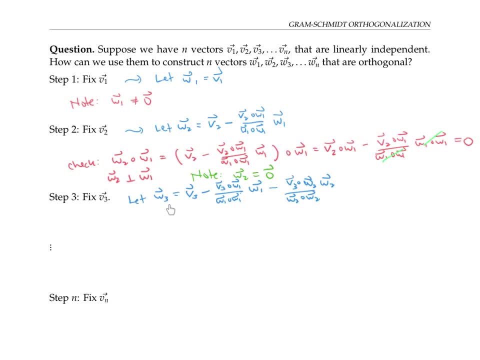 w two, w three is a legitimate vector because it's just a linear combination of other vectors. And notice that w one dot w one can't be zero, since w one is not the zero vector. And also w two dot w two can't be zero. 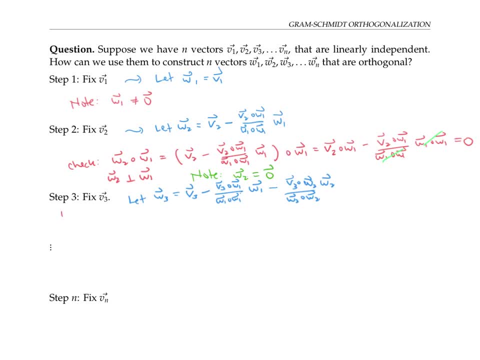 So we're not dividing by zero here. Now I claim that w three is going to be orthogonal to both w one and w two. If I take w three dot w one and distribute the dot product, I get a w two dot w one, which 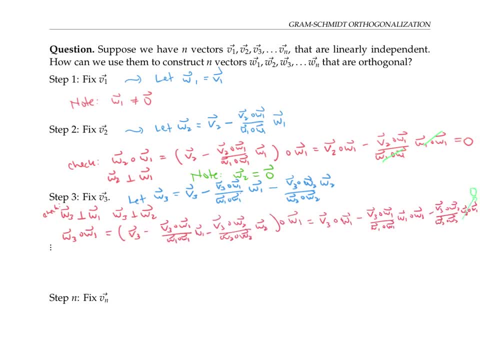 I already know is zero, because w two was orthogonal to w one And after canceling some w one, dot w ones, I get an expression that's equal to zero. Similarly, if I dot w three with w two, I get now this middle term goes to zero, since 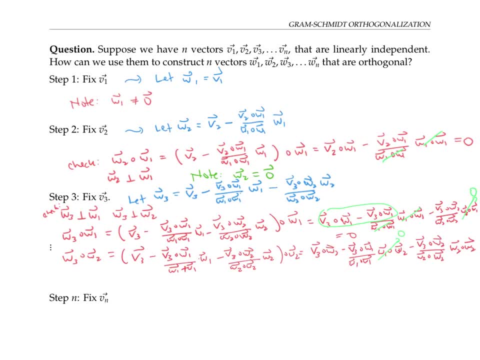 w one dot. w two is zero, And now this third term cancels with the first term to give us zero. Okay, So w three, indeed, is orthogonal to both w one and w two. The same argument as before tells us that w three cannot be the zero vector. 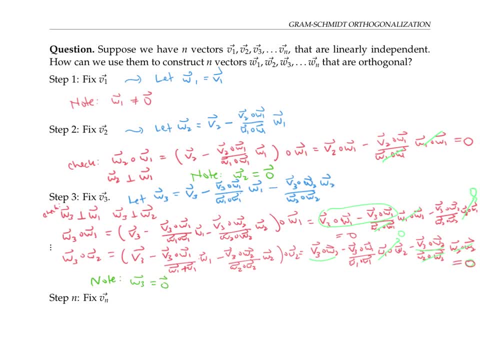 It's a linear combination of v three, w one and w two, but w one and w two are themselves linear combinations of v one and v two. So w three is really a linear combination of v three and some v ones and v twos, whose 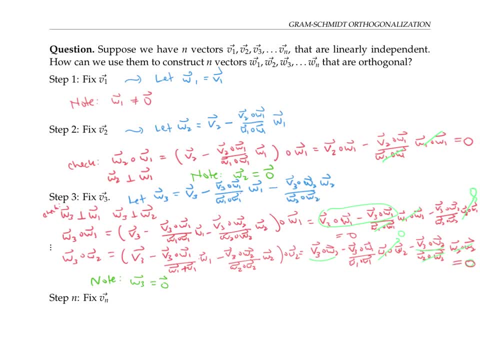 coefficient of v two is zero, The coefficient of v three is one, And so linear independence says that can't give us the zero vector. So we continue in this way, fixing up v four, then v five, and so on. Finally, the last vector, v n, we'll replace with w n, which will be v? n minus a multiple. 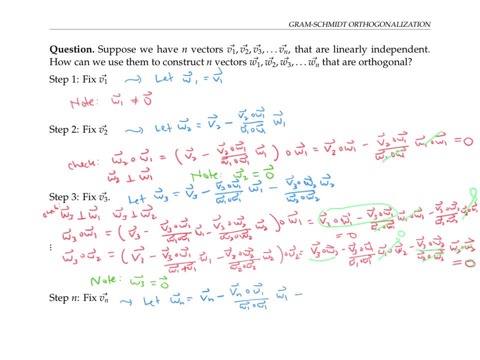 of w one minus a multiple of w two, and so on, until finally we subtract a multiple of w n minus one. Anytime I dot product this with a previous w vector, I'm going to get zero. For example, if I dot product it with w three, then all of these terms would go to zero, because 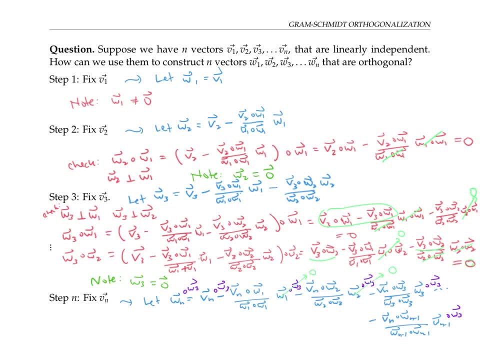 all the previous w's are orthogonal And the w three dot w three would cancel and I'd be left with v n dot w three minus v n dot w three, which would give us zero. Okay. A similar argument shows that w? n dotted with, say, w four or any other of the w's would 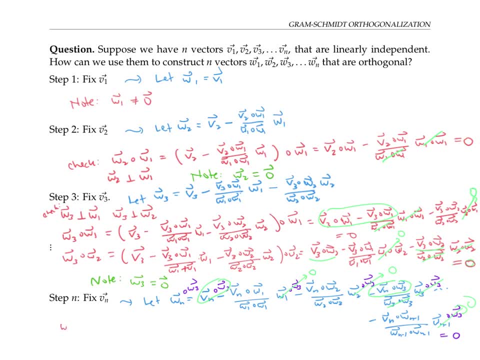 give us zero. So in the end we have w one through w n. all orthogonal vectors And arguments like we made previously can be used to show that they're all nonzero vectors. to question: are these new vectors, w one through w? n, still linearly independent? 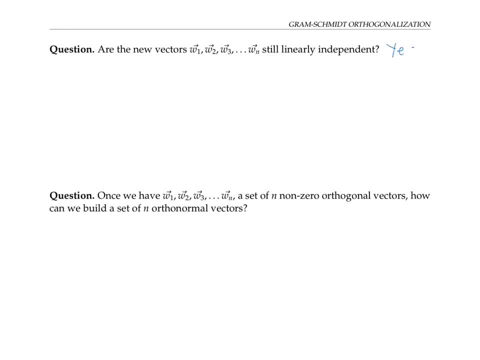 Okay, In fact they are. in fact, any set of orthogonal vectors, none of which is the zero vector, will be linearly independent. That's because if we take a linear combination- x one w one plus x two w two, so on through. 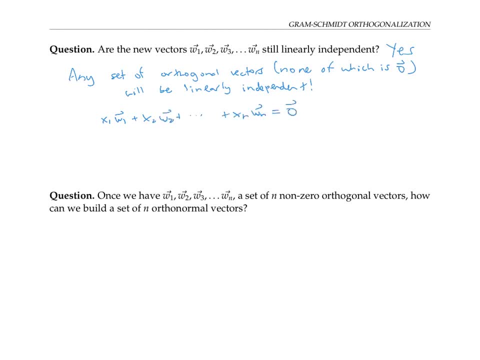 x, n, w, n. And if that's equal to the zero vector, then look at what happens. If we dot product both sides with, say, w, one on the right side, we'll get zero, since the zero vector- dot with anything- is zero. 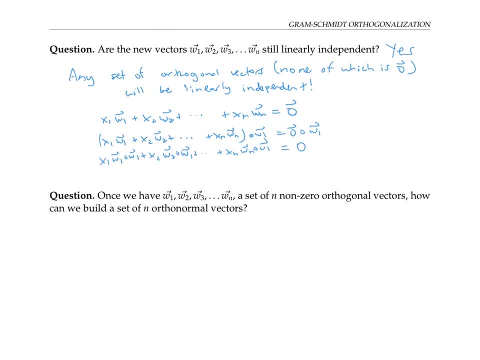 And on the left side, after we distribute the dot product, we'll get a bunch of zeros everywhere, since we've got a bunch of orthogonal vectors and we'll be left with just x one times w one dot w one equals zero And since w one is not the zero vector, 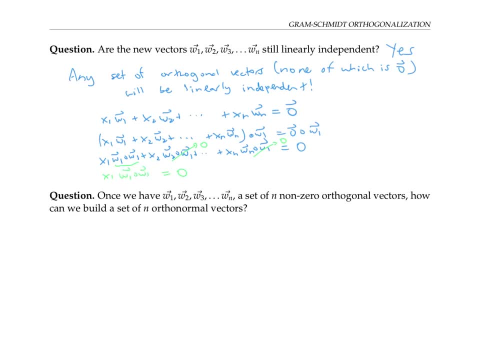 So it's dot product can't be zero. This means that x one must be zero. So dotting with w one shows that x one is zero. If we dot with w two instead, the same argument will show us that x two is zero. 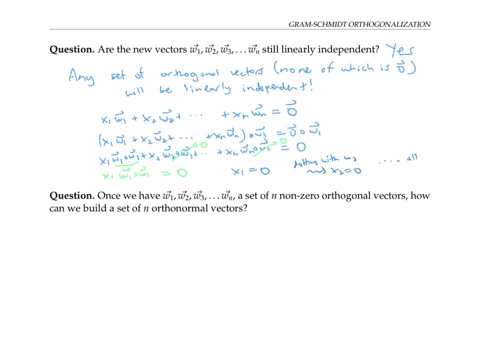 And so on. we can keep going to show that all the x, i's are zero. Therefore these orthogonal vectors, w one through w n, must be linearly independent. So one last theory question before we get an example: if we have these w one through, 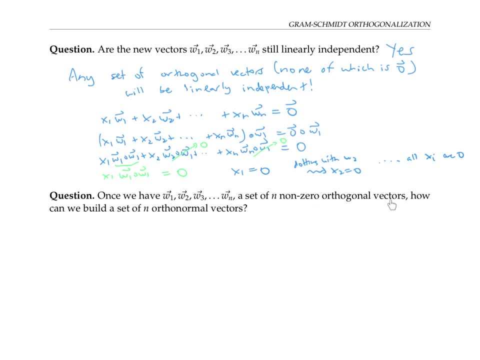 w, n now a set of nonzero orthogonal vectors. how can we build a set of n orthonormal vectors? Remember, orthonormal means they're not only orthogonal to each other, but they each have length, one. Well, fortunately that's pretty straightforward. 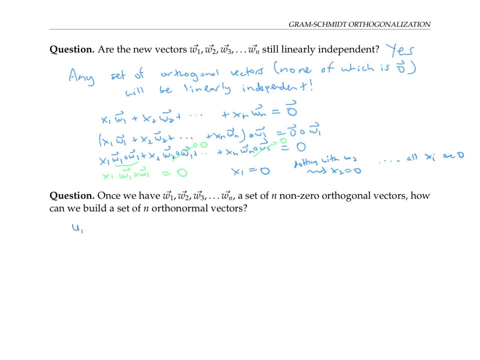 All we do is I'll call the new set of vectors by us. I'll let you one b w one over its length, you to be w two over its length, and so on, up through u? n, which is going to be w? n divided by its length. 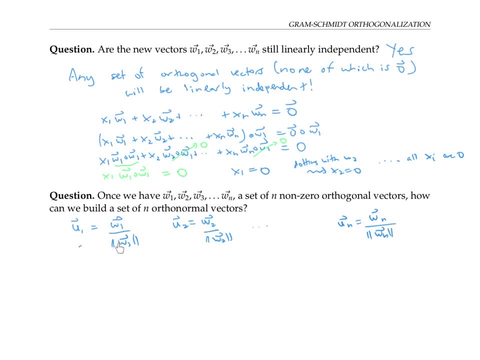 Each of these us is just a w rescale to be length one, So they'll definitely all be length one, And I'll also still be all orthogonal. For example, if I take u two and dot it with u three, That's gonna be the same thing as w two over its length, dotted with w three over its length. 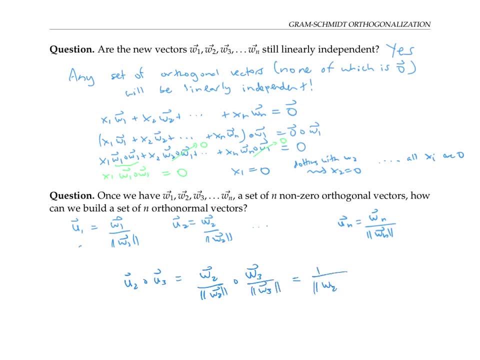 And if I factor out the one over the length of w two and the one over the length of w three, I'm just going to get that scalar times w two, dot w three. well, this is going to be zero, since the original W's were orthogonal and therefore the dot product of the use. 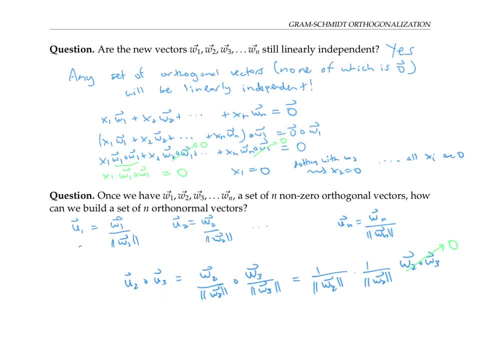 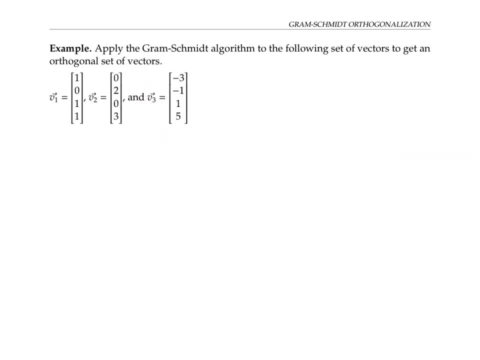 is zero, the user orthogonal. So we have a straightforward method of converting nonzero orthogonal vectors into orthonormal vectors. So let's conclude with an example. Let's apply this algorithm to convert this set of three vectors into an orthogonal set of vectors. 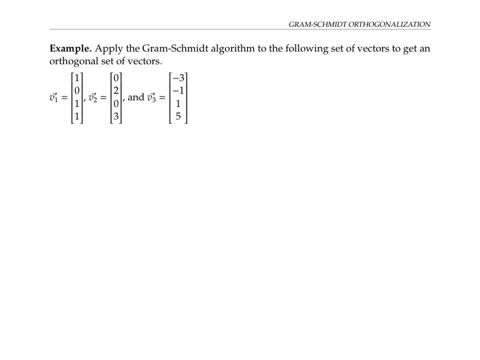 I'll let you check on your own that this is in fact a set of linearly independent vectors, or you can take that on faith. So our first vector w one is just going to be the same thing as v one. Our next vector w two is going to be v two minus v two. dot w one over w one. dot w one. 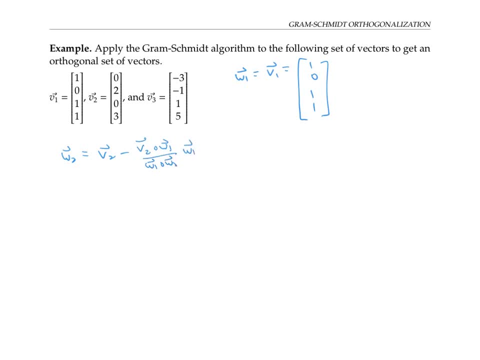 times w one. Let's do some scratch work on the side. v two, dot w one. that's the dot product of these two vectors which works out to three, while w one, dot w one is the dot product of those two vectors, which also works out to three. 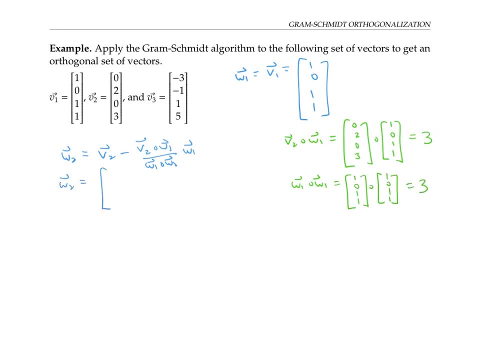 So w two is going to be v two minus three over three times w one. that works out to the vector with entries negative one, two, negative one, two. Now we need to build the vector w three. that's going to be v three minus v three dot w one. 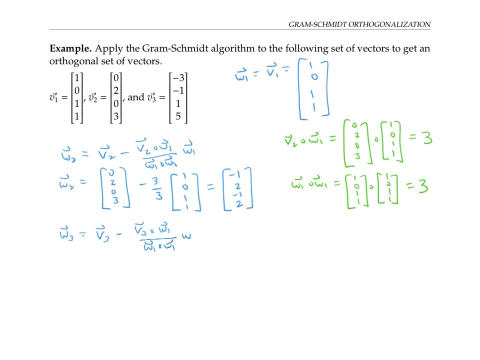 over w one dot w one times w one minus v three dot w two over w two dot w two times w two. again, I'll do some computations on the side, And so we end up with this expression, which works out to minus three minus 312.. 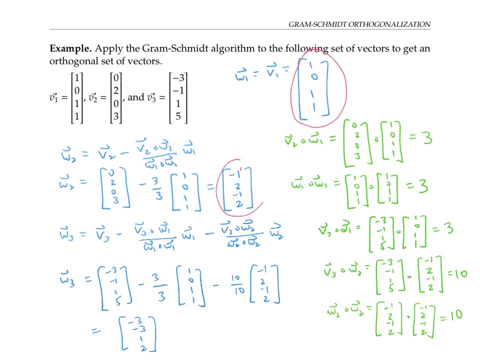 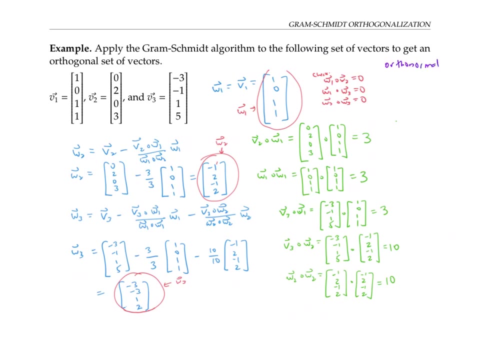 So these are our new vectors w one, w two and w three, And you can check That they're, in fact, all orthogonal to each other. If I wanted to go one step further and get a set of orthonormal vectors, I could just. 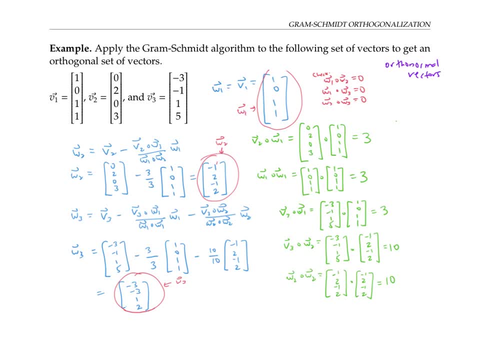 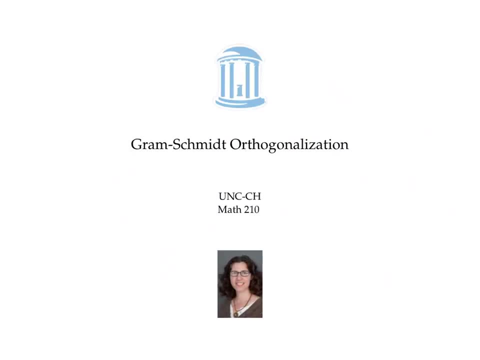 divide each of w one, w two and w three by its length. This video gives an algorithm for turning a set of linearly independent vectors into a set of orthogonal vectors And, if we want, We can go one step further and turn them into a set of orthonormal vectors. 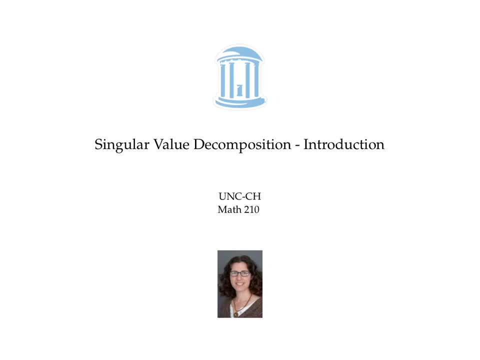 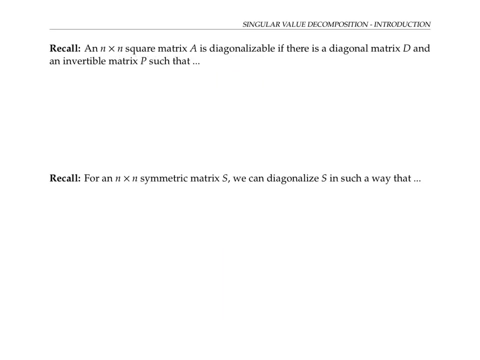 This video introduces the idea of singular value decomposition, a powerful way of rewriting matrices that has important applications to real world problems like image compression and data simplification. Recall that an n by n square matrix A is said to be diagonalizable if there's a diagonal. 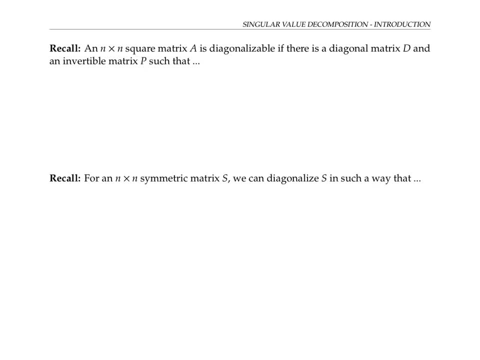 matrix D, An invertible matrix, P, such that a can be written as P times D times P inverse. Recall also that if we start with an n by n symmetric matrix, let's call it s. then we can diagonalize s in such a way that P is an orthogonal matrix, the singular value. 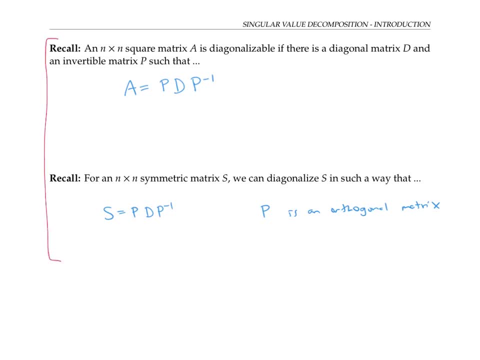 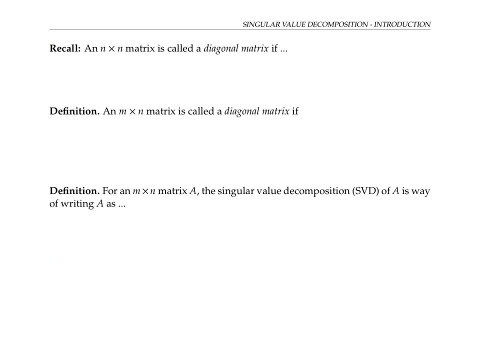 decomposition generalizes these ideas. The singular value decomposition generalizes these ideas To a general matrix A that need not even be a square matrix. In order to generalize this idea of diagonalization to matrices that aren't even square matrices, we first need to generalize the idea of a diagonal matrix. 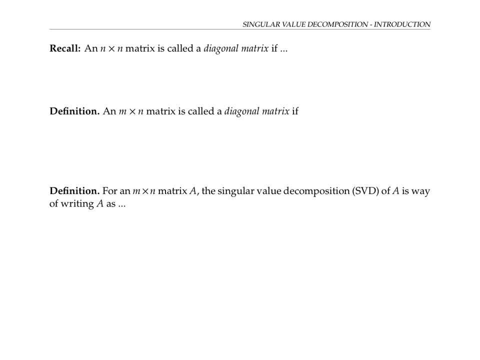 So up to now we've only talked about n by n, square matrices being diagonal matrices, And we said that a square matrix is a diagonal matrix if all of its nonzero entries are nonzero entries and all of its nonzero entries lie on the diagonal. 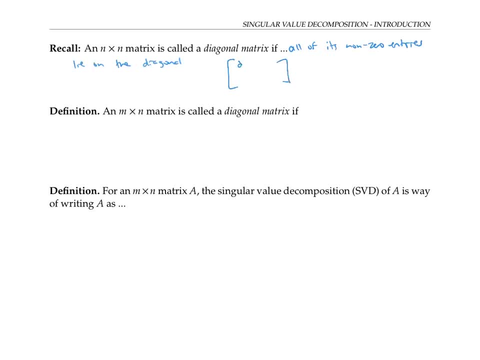 So we have some, we might have some nonzero entries here, And then we have zeros everywhere else. So we'll say that an m by n matrix, where m and n might be different, is called a diagonal matrix if all of its nonzero entries lie on its diagonal, where the diagonal entries are. 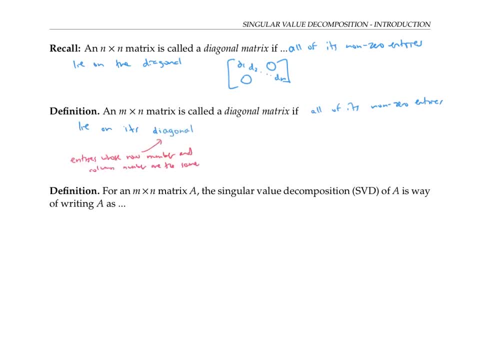 the entries whose row number and column number are the same. So, for example, here's a four by two diagonal matrix And here's a three by five diagonal matrix For an m by n. matrix A. the singular value decomposition, abbreviated SVD, of A is a way 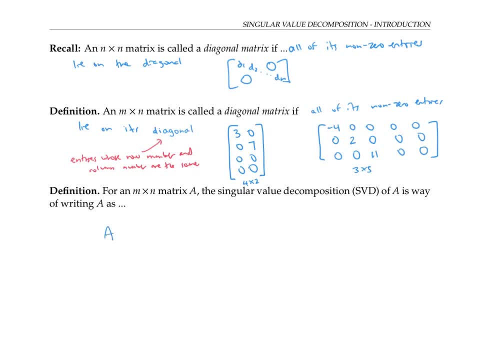 of writing A as a product of a matrix, U, a matrix sigma and a matrix V. transpose: Where sigma is an m by n- diagonal matrix, V is an n by n- orthogonal matrix And U is an m by m- orthogonal matrix. Let me draw these matrices with squares and rectangles to illustrate the dimensions. 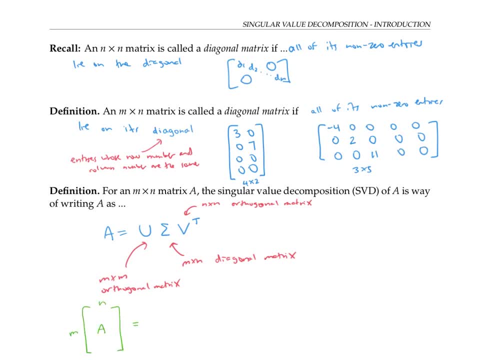 So here's A an m by n matrix, Here's U an m by m square matrix. Sigma is an m by n matrix, just like A And V. transpose is an n by n matrix, And actually V is also n by n. 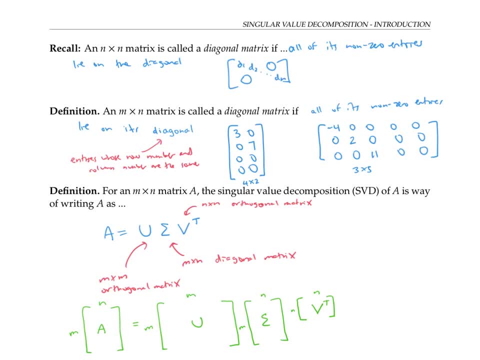 The singular value decomposition has some features similar to the diagonalization of a matrix, then, namely that the middle matrix sigma is diagonal And then it's a product of three matrices. In fact, since V is orthogonal, V transpose is the same thing as V inverse. 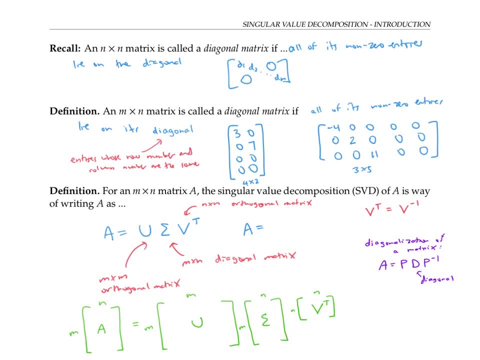 So we could make this look even a little more like a diagonalization by writing this as U times sigma times V, inverse. Also like the diagonalization of a symmetric matrix, the singular value decomposition uses matrices on the outsides that are orthogonal. Okay. 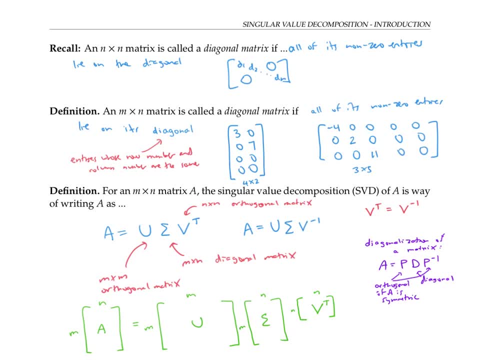 But the singular value decomposition is different from a diagonalization in that U and V may be different matrices. In fact, if m and n are different numbers, if we have a purely rectangular matrix, not a square matrix, then U and V have to be different matrices because they've got different dimensions. 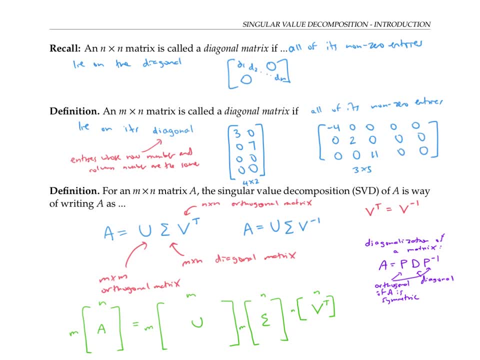 A singular value. decomposition has a lot of the same power as a diagonalization does, namely the power to write a matrix A In terms of a much simpler diagonal matrix, which is why it has important applications, as we'll see in future videos or in class. 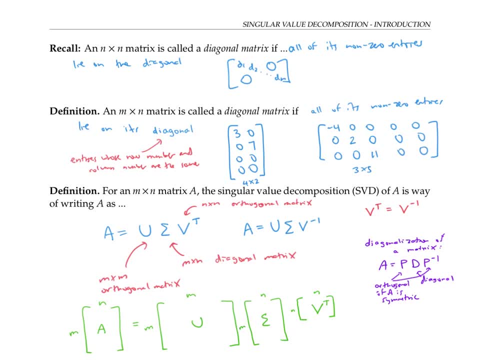 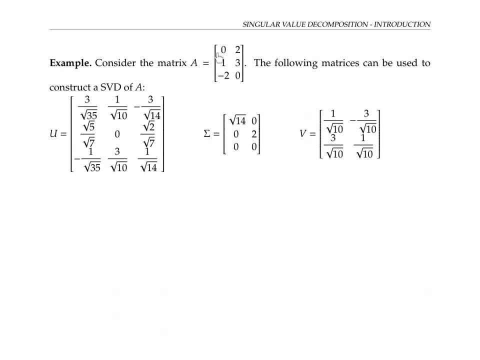 For now let's look at an example of a matrix and its singular value decomposition. Here's an example of a singular value decomposition. We have a three by two matrix, A, and it turns out that we can write A as U times sigma times. 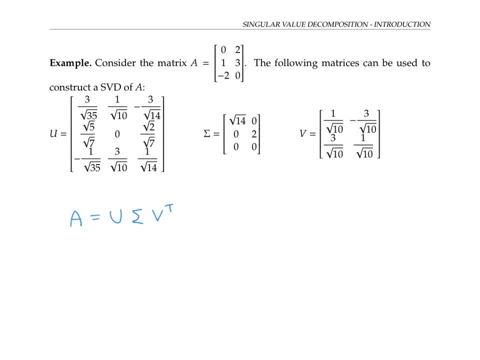 V transpose Using these given matrices. Notice that this last matrix needs to be V transpose, not the original V. It's clear from looking at it that sigma is a diagonal matrix. I'll leave you to check, if you want to, that the matrices U and V are both orthogonal matrices. 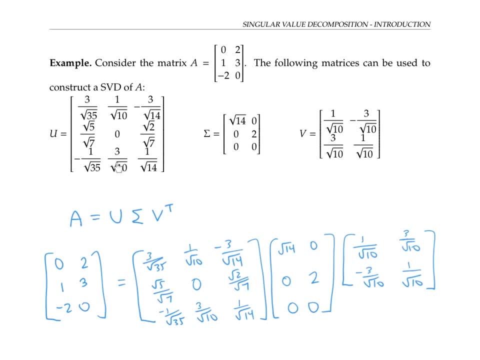 In other words, each pair of columns of U has a dot product of zero, And if I dot product any column by itself, I get one and same thing for V. I'll also let you check, If you're interested, that this product really does work out to the original A. 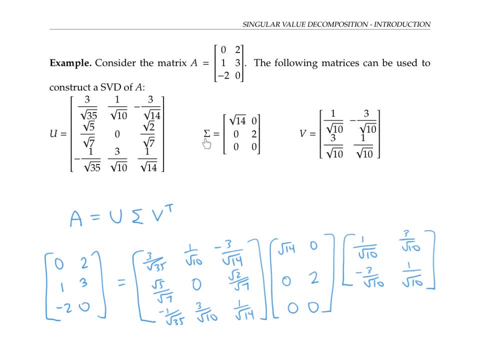 Now you may be wondering how did I come up with these matrices U sigma and V that work Well? to be honest, I use software, but there is a method, an algorithm that will allow us to do a singular value decomposition for a matrix A like this: 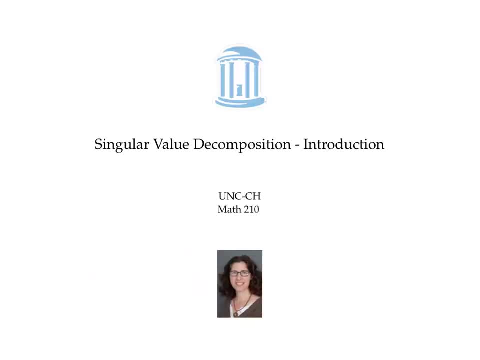 And I'll show that to you in another video. In this video we introduced the idea of a singular value decomposition and compared it to diagonalizing a matrix. In future videos we'll look at how to do a singular value decomposition, In other words, how to find U, sigma and V, and what some of the applications are. 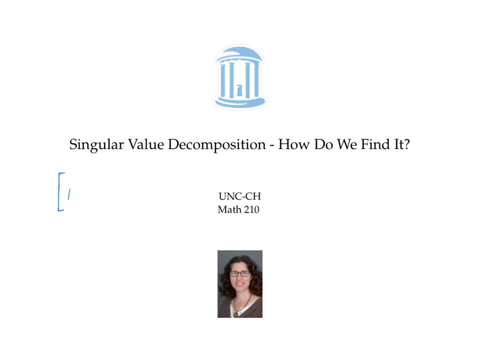 Recall that a singular value decomposition for a matrix A is a way of writing A as the product of three matrices: a square matrix- U- that's actually an orthogonal matrix. a rectangular matrix- Sigma- the same dimensions as a- that's actually a diagonal matrix. and a square matrix V transpose. 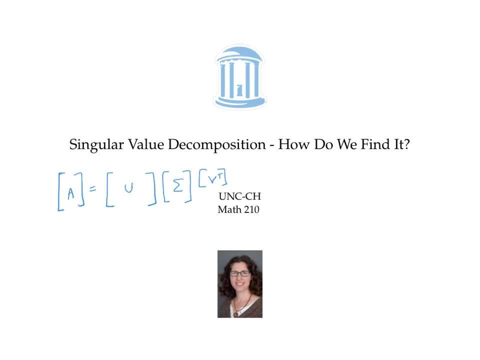 where V and V transpose are both square matrices and orthogonal matrices. In this video I'll walk you through an algorithm to start with a matrix A and find these three matrices: U, sigma and V. I'll also do one example, but I'm going to postpone to another. 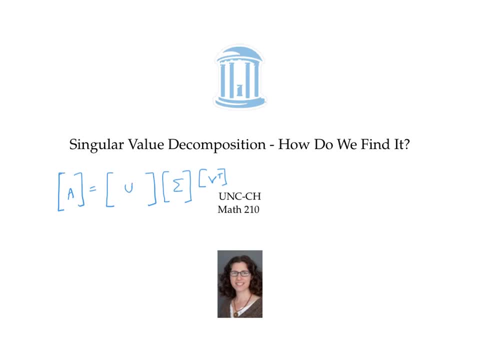 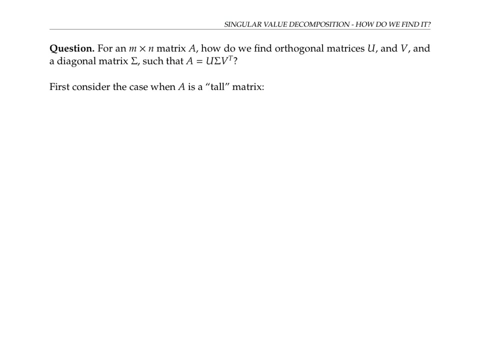 video I'll explain why this algorithm actually works, Why at the end of it we actually get matrices whose product is A, and why the matrices U and V that we get are actually orthogonal. So, for an M by N, matrix A, how do we find orthogonal matrices U and V in a diagonal? 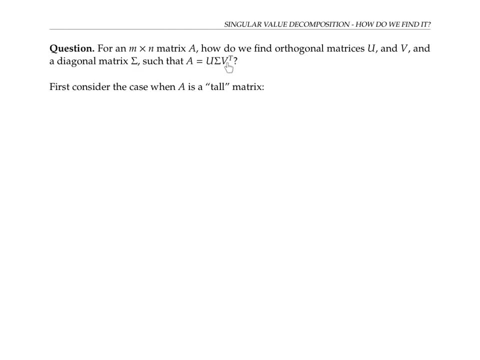 matrix sigma such that A is equal to U. sigma V: transpose: First let's consider the case when A is a tall matrix. In other words, when M is a tall matrix. In other words, when M is a tall matrix. 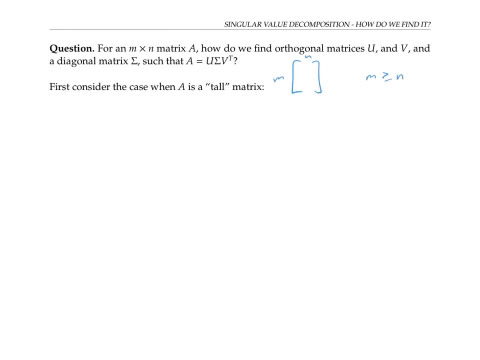 In other words, when M is a tall matrix, A is greater than or equal to n. First we're going to find the matrix A transpose times A. notice that that will be an N by N matrix And it'll actually be an N by N symmetric matrix. 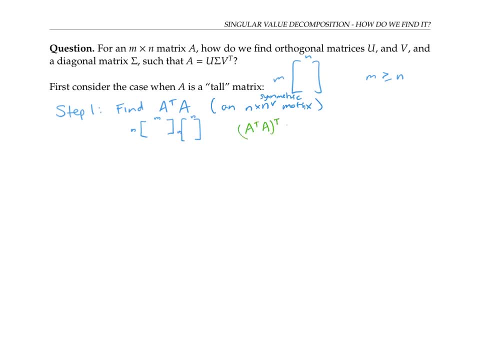 Since the transpose of A transpose A is a transpose, A transpose transpose, which is A transpose A thing. as we started with, we're going to find the eigenvalues of A transpose A. Since A transpose A is symmetric, these eigenvalues are all real numbers. But even better, as 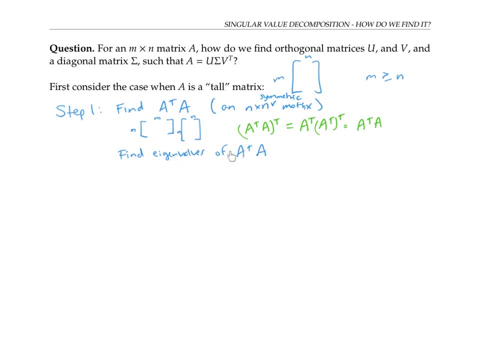 a previous video shows any matrix of the form A transpose A has eigenvalues that are actually non negative real numbers. So we have that these are all real numbers greater than or equal to zero. Now, in this class we'll only work with situations when all the 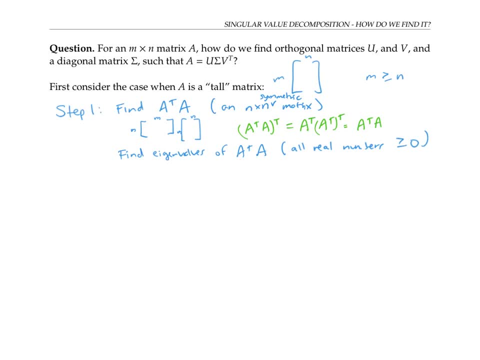 eigenvalues of A transpose A are distinct, So I can call them lambda one through lambda n, And I'm going to order them in such a way that lambda one is bigger than lambda two is bigger than lambda three, and so on. More generally, in some examples the eigenvalues won't all be distinct numbers sometimes. 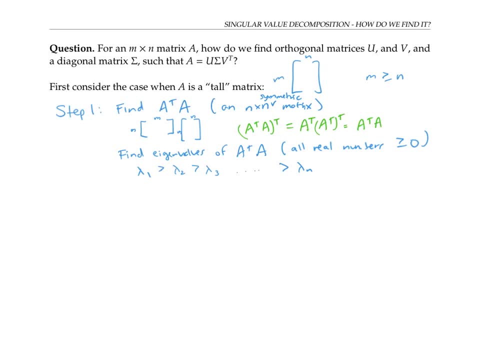 there'll be a root of the characteristic polynomial that's repeated, And so, if that's the case, we'll still write them all down, And if the root of the characteristic polynomial has a multiplicity three, we'll just write it down three times, And so, in more generality, 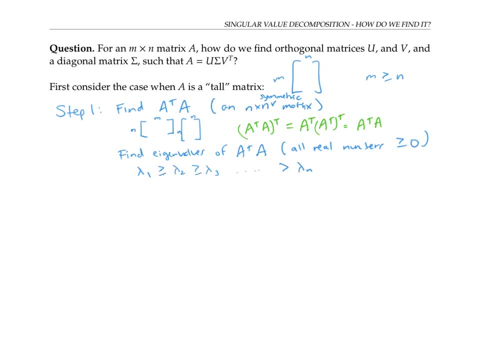 we'll just be able to say that lambda one is greater than or equal to, because there might be some repeated eigenvalues. Now, when we were diagonalizing a matrix earlier, we just used the eigenvalues of A transpose A and A transpose B, And so we're going to. 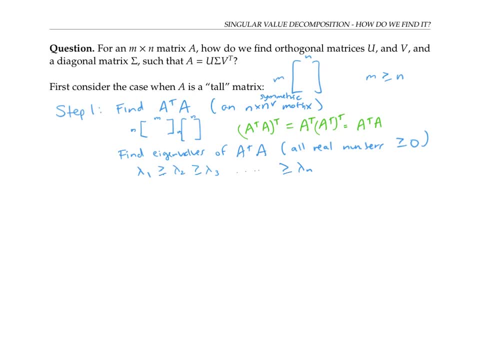 use those eigenvalues for the matrix as our diagonal entries. But this time we're going to do something a little bit different. we're going to use the square root of our eigenvalues as our diagonal entries. So I'm going to call the square root of lambda i. I'm going to 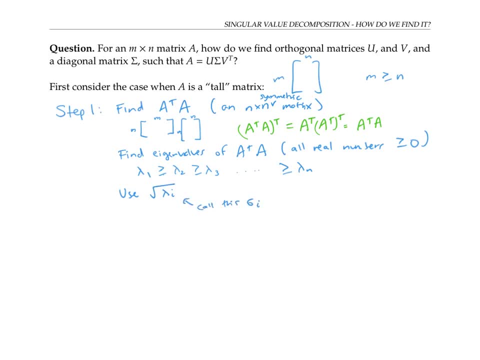 call this sigma i. notice that it's no problem taking the square root of lambda i, since lambda i is going to be greater than or equal to zero. Notice also that we still have the sigmas in descending order. These numbers, sigma one through sigma n, are called the singular. 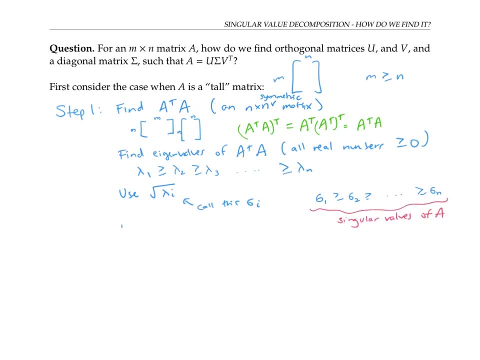 values of A. And now I'm going to build the rectangular diagonal matrix sigma by taking sigma one through sigma n along the diagonal and filling the rest in with zeros. If m is bigger than n, then sigma n is greater than or equal to zero, And if m is greater than 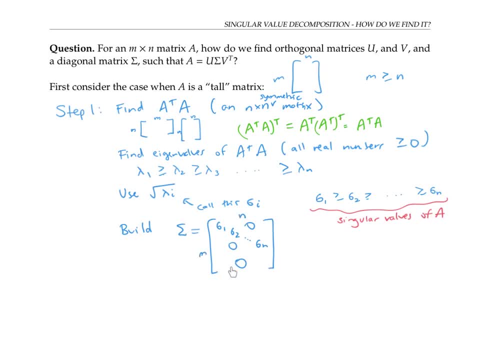 n, then the last few rows of sigma will all be zeros. To me it kind of makes sense. we want to use the square root of lambda i instead of lambda i, because lambda is the eigenvalue for this product, which is kind of almost like doing a squared. So makes sense, the square. 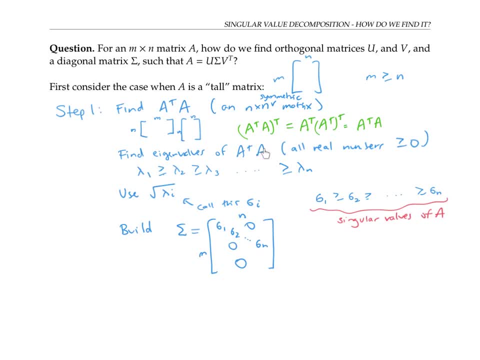 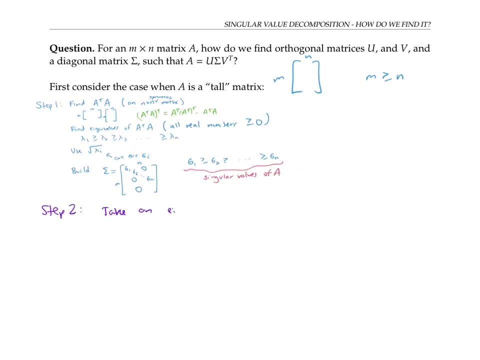 root of lambda, i would be more related to just a itself. Okay, so now we've got sigma, the middle matrix of the three. Next let's work on v. So for step two we're going to take an eigenvector v, one for lambda. 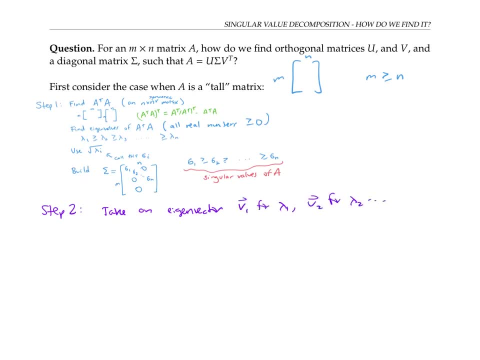 one v two, for lambda two, etc. Each of which has length one. If the first eigenvectors we pick don't have length one, then we can just rescale them by dividing by their length to get an eigenvector of length one. 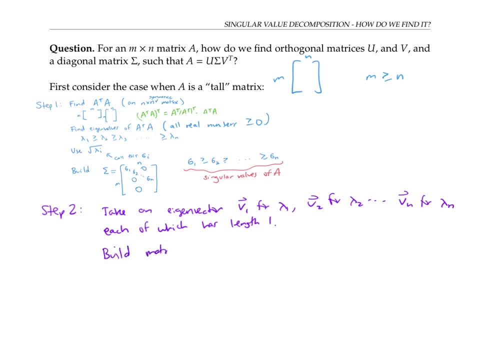 Now we're going to build the square root of lambda i, and then we're going to take the square root of lambda i, and then we're going to build the matrix v using v one through vn as its column vectors. Again, for our class, we'll only ever consider the situation where 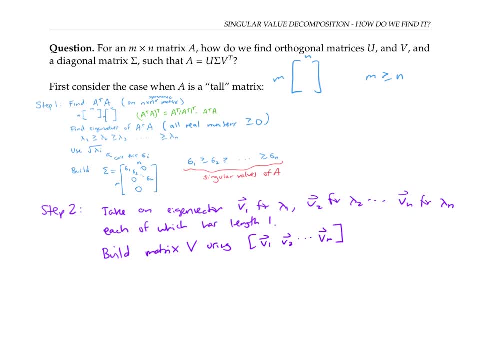 the lambda eigenvalues are all distinct and we just take one eigenvector for each of them. If you were to consider a more general situation, when maybe, say, the first eigenvalue was really repeated, so lambda one and lambda two were the same, then you would end up having to. 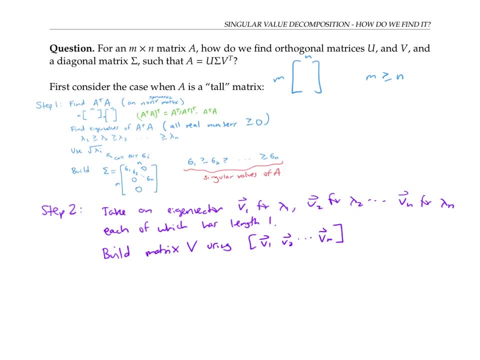 choose two eigenvectors for that eigenvalue in such a way that those two vectors were not only length one but also orthogonal to each other. And it turns out that this is possible, since these eigenvalues came from a symmetric matrix. but that's beyond the. 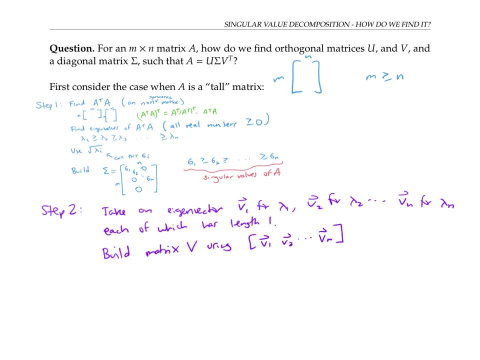 scope of our class. Okay, so now we have built our matrix v, from which we can easily get v transpose. notice that these eigenvectors are eigenvectors for the matrix a. transpose a, which is an n by n matrix, So these vectors have dimension. 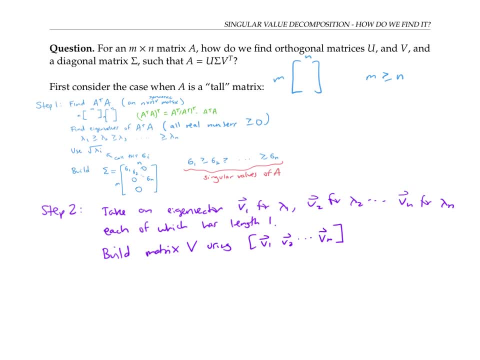 n, And so the matrix v will be an n by n matrix, And the last thing we need to do is to find our matrix u. So to find u, we're going to compute. So to find u, we're going to compute a times vi over sigma i, for each non zero number, sigma i, Since the matrix a is an. 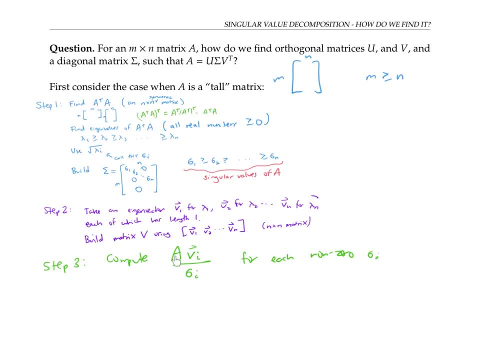 m by n matrix. when we multiply a by the n dimensional column vector, we're going to get an m dimensional column vector. dividing it by the scalar, it'll still be an m dimensional column vector. We'll have no more than n of these column vectors. it would be exactly n, except for: 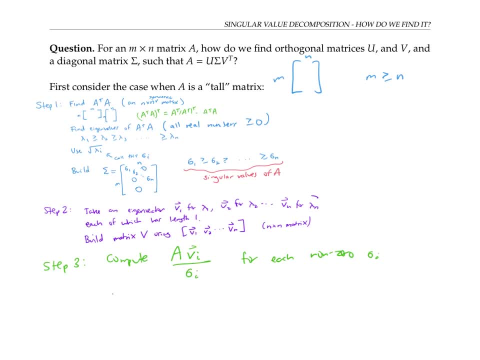 some of the sigma i's might be zero. So I'm going to call these column vectors, u one through u, r, say where r is less than or equal to n, And I'm going to start building you, the matrix, you, by stringing these column vectors together. Ultimately, I want to know: 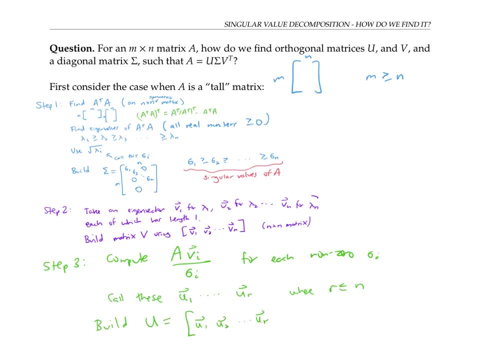 how long the two行r specialyl and r specimen report. I want U to be an m by m matrix And I might not have enough columns to do that, So I need to fill out my matrix U with some more columns, m minus r of them, To be exact. There are a few ways to do this, But in practice 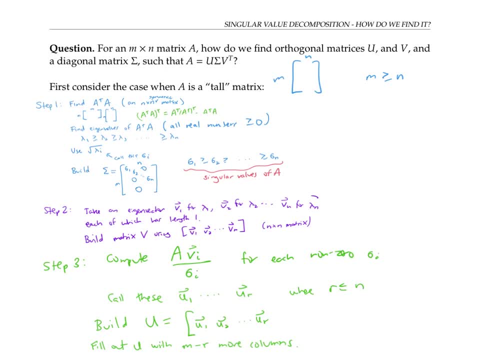 the simplest thing to do is usually just to pick some M minus r columns at random and then using the Gramm Schmidt orthogonalisation algorithm to make them orthogonal to each other and to the original U1 through UR columns and dividing them by their lengths, if necessary to make. 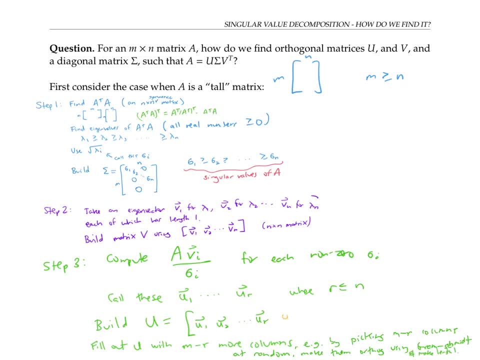 them length one, So I'll call these extra columns after we orthonormalize them. I'll call them UR plus one through UM. There are a few details here that I'm sweeping under the rug. In particular, in order to do the Gram-Schmidt orthonormalization process, we need all of 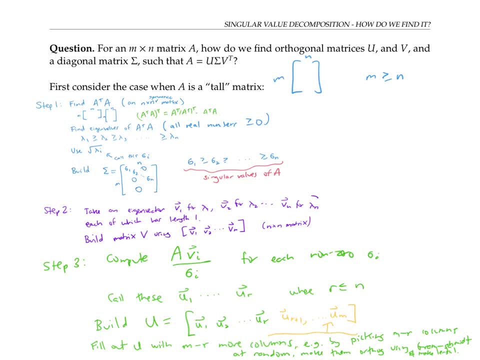 our columns together to be linearly independent, Turns out, if you pick columns at random, usually you will get things that are linearly independent. If you have bad luck, you might have to do some re-picking. There are some other ways to fill out the matrix U, but in the interest of keeping things, 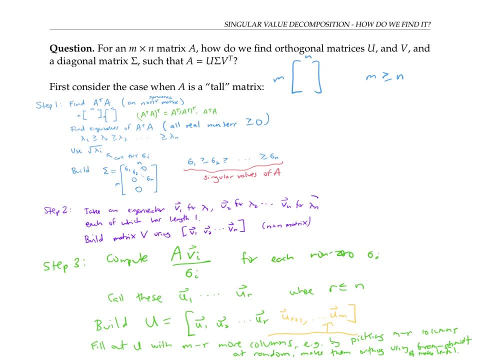 short and simple. I won't go into those details here. In addition, as you'll see in the applications video, it doesn't actually matter a whole lot what the end of this matrix looks like. Okay, so to summarize, we build the diagonal matrix sigma using the eigenvalues of A transpose. 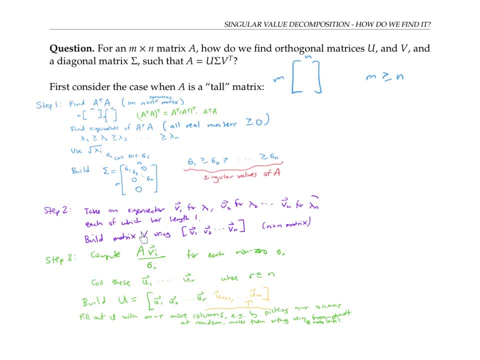 A and taking their square roots. Then we find V by using the eigenvectors for A transpose A. And then we find U by computing A times those eigenvectors divided by those singular values and filling out the matrix one way or another. I want to remind you that we haven't yet verified that this matrix is a linear matrix. 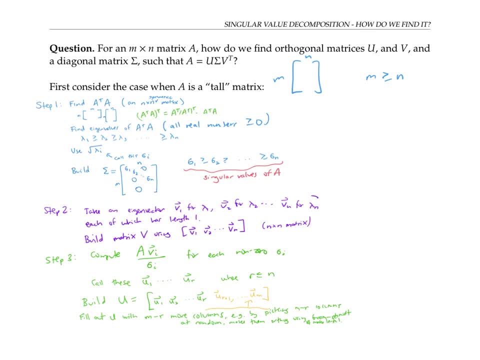 This process actually gives us a singular value: decomposition, That is, we haven't verified that U and V are actually orthogonal matrices and that the product U sigma V transpose actually gives us A. That'll happen in the next video. I wanted to do this for a tall matrix first, where M is greater than or equal to N, because 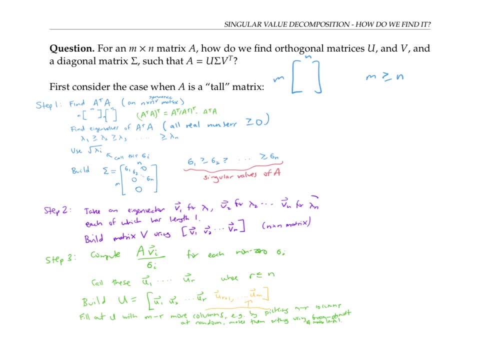 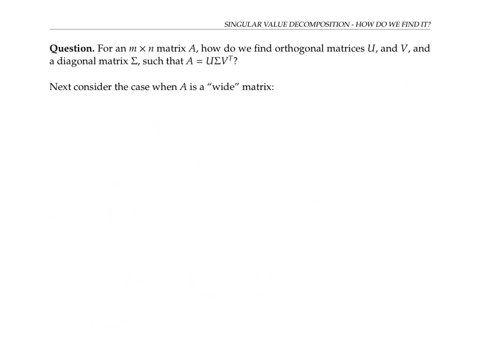 that way we could be sure that the number of eigenvalues we'll get for A transpose A and eigenvalues would be small enough to fit into our rectangular matrix sigma. Next we'll look at the case of a wide matrix, Although it turns out that a similar process could be used when A is a wide matrix. 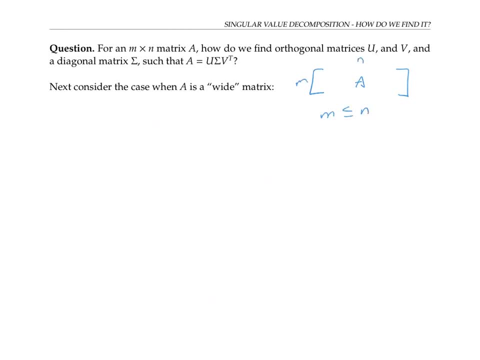 That is, when M is less than or equal to N. Instead, I'm just going to repeat what we did on the previous slide for the tall matrix B, which is given by A transpose. that'll give us B As a product of some U times, some sigma times, some V transpose, where the dimension of B 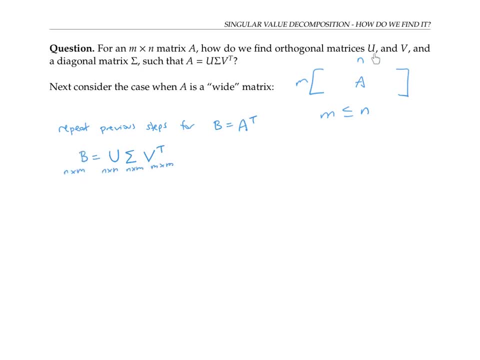 is n by m, since it's the transpose of A and mentions of U, sigma and V are as follows: Now I can write a, which is B- transpose, as U sigma, V- transpose, transpose, which is the same thing as V- transpose, transpose, sigma transpose, U transpose, or V- sigma- transpose, U transpose. 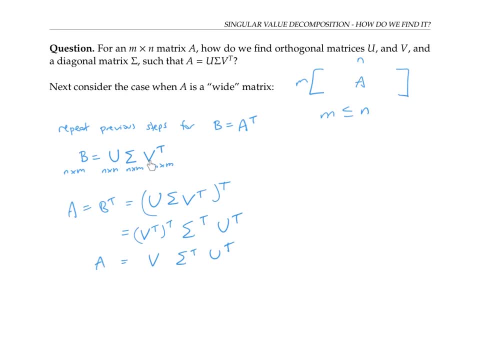 And since V and U were orthogonal matrices and sigma a diagonal matrix, I'll still have orthogonal matrices here and a diagonal matrix here, all of the correct dimensions. Let's do an example and find the singular value decomposition For this three by two matrix. 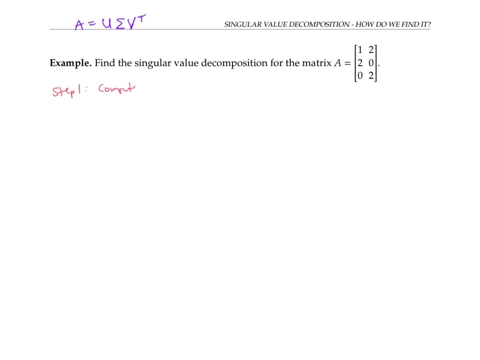 Step one is to compute A transpose A and find its eigenvalues. A transpose A is this product which works out to this two by two symmetric matrix. To find the eigenvalues, let's write down the characteristic polynomial which is given by the determinant of the matrix, with entries five minus lambda, two, two and eight minus. 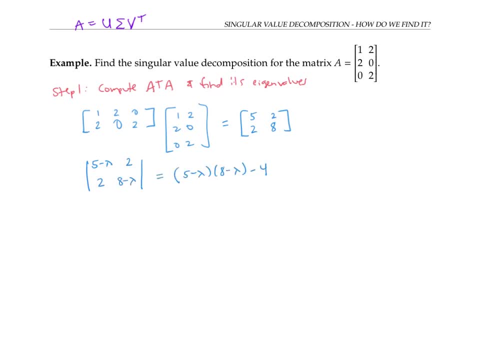 lambda. Here's the determinant which simplifies to: lambda squared minus 13, lambda plus 36.. When I factor this and set it equal to zero, I get that the eigenvalues of A transpose A are: lambda one equals nine and lambda two equals four. 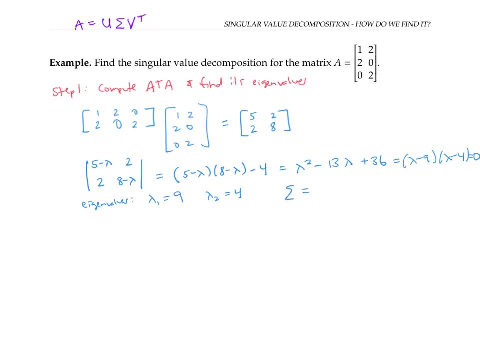 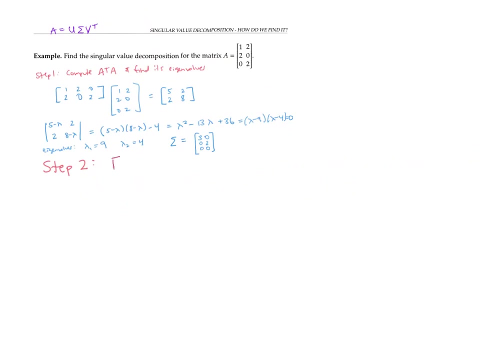 So now I can write down my diagonal matrix sigma, which should also be a three by two matrix. Notice, recall that the diagonal entries, the sigma eyes, are given by the square roots of the lambda eyes. Now let's move on to step two: finding the eigenvectors for A, transpose A and building. 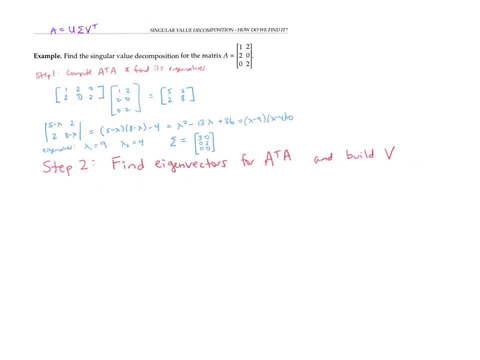 V with them. I encourage you to pause the video and work this out for yourself before going on. Here's what I get. So for eigenvectors, I have the vector one, half one, and the vector negative two, one, But aren't length one. I'm going to want to rescale them by dividing by their lengths. 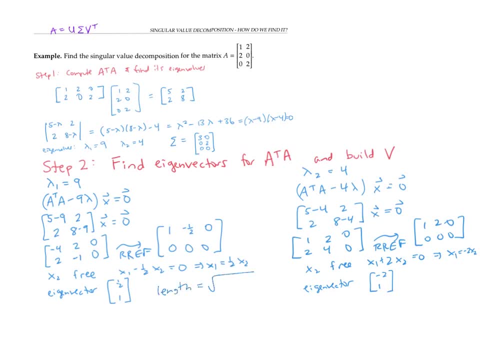 The length of this first eigenvector is the square root of one half squared plus one squared, That's the square root of five fourths or the square root of five over two. So I'm going to take the eigenvector and divide by that length, which gives me the length. 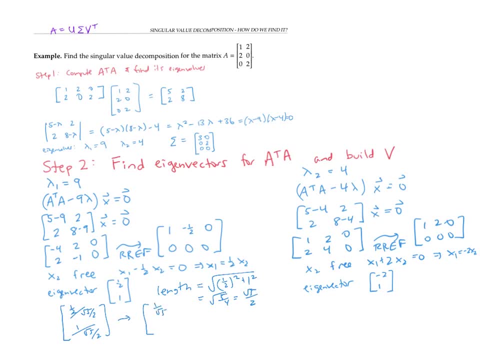 one eigenvector, one over square root of five, two over square root of five. For the other eigenvector, Its length is going to be the square root of five, And so I can divide by the square root of five. Now I can build my matrix V by using these two length one eigenvectors as my columns. 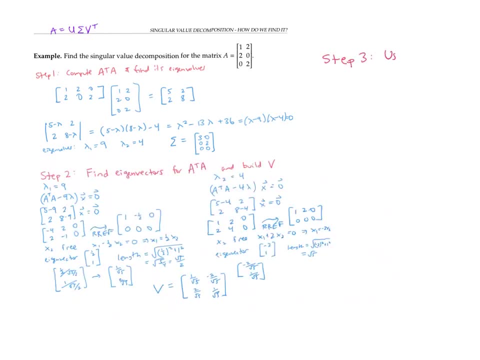 And I'm ready to go on to the third step, which is using the column vectors a, vi over sigma i To build The matrix. you hear, the vi are the column vectors of V. So let me write down a v one over sigma one and a v two over sigma two. 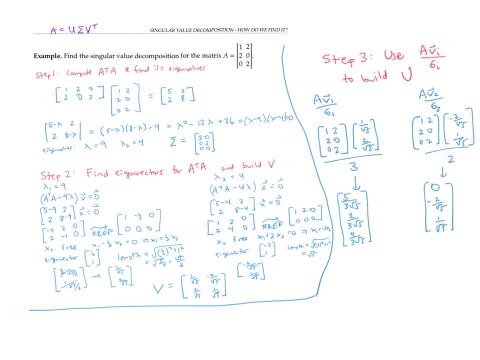 Those work out to these vectors. These will be my first two columns of you, And you might notice that they're already length one and orthogonal to each other, But I need to fill you out with a third column that's also length one and orthogonal to these. 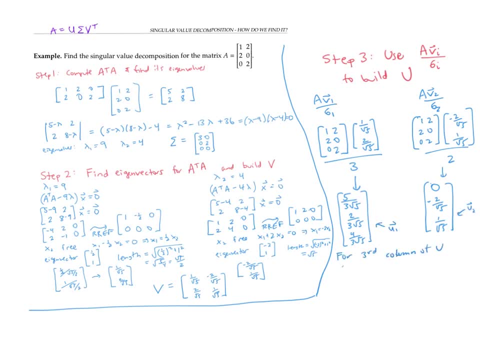 first two columns. For this third column, I'm going to start with the column vector one, zero, zero- although any column vector that's linearly independent from these two would do- And then I'll apply the Gram Schmidt or the normalization process to make it orthogonal. 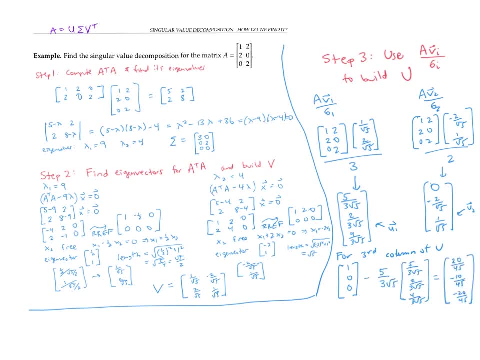 to you one and you two. I'll omit the details, But this is the vector I get which is in fact orthogonal to both you one and you two. It's not length one, So I'll just calculate its length And divide by it to get my last orthonormal vector, u three. we put these three columns. 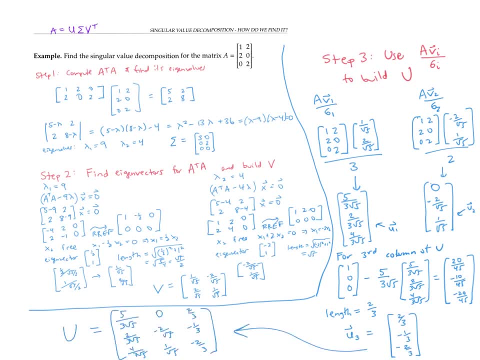 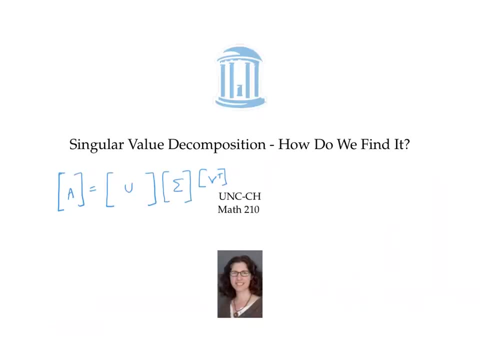 together and we have our matrix, you and we finished our singular value decomposition using these three matrices. This video gave them methods for finding a singular value decomposition. It was a complicated process, but it will prove to have powerful applications. In a previous video, 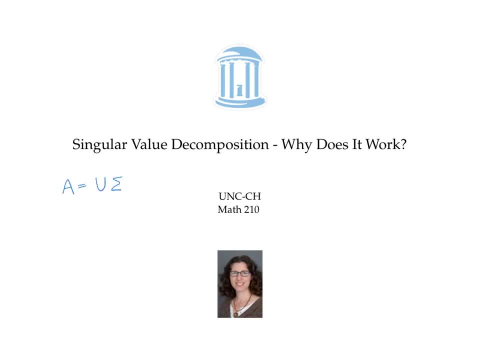 We walked through an algorithm for finding the matrices u, sigma and v used for a singular value: decomposition. In this video we'll go through some of the theory behind it to explain how we know that the u and v, that we found our orthogonal matrices and how we know that when we multiply. 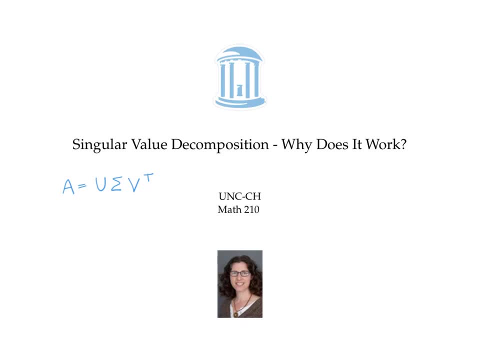 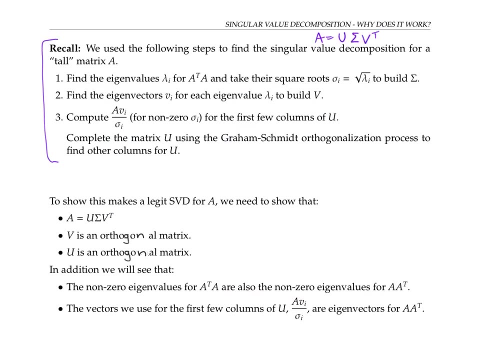 these three matrices together we actually get back to a. here are the steps we used to find the singular. First we found the eigenvalues for the product, a transpose times a, and we took their square roots to get our singular values. sigma sub i. we put those sigma sub i's down the diagonal. 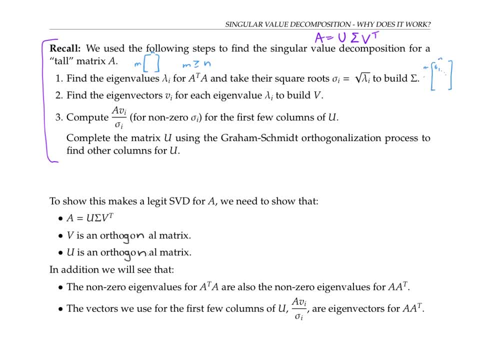 and m by n matrix to get our matrix sigma. Next we found length one eigenvectors for a transpose times a and use them as our columns for the matrix V. The simplest situation is when a transpose a has all distinct eigenvalues, So we can just take one eigenvector for each eigenvalue. 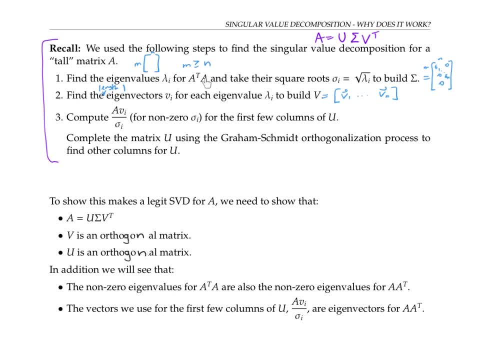 It's a little more complicated if a transpose a has repeated eigenvalues, and I didn't go into those details. Finally, we computed the first few columns of the matrix u by taking a times V sub i over sigma sub i for the nonzero singular values: sigma sub i. 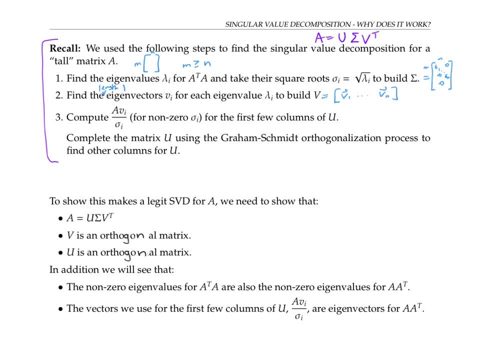 And we got the rest of the columns for you by choosing linearly independent vectors, using Graham Schmidt To orthogonalize them and dividing by their lengths to make them length one. it's clear from the construction that we get a diagonal matrix for sigma. 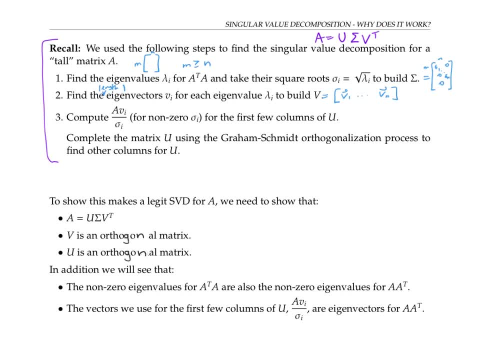 But here are the other details we need to check to make sure we have a legitimate singular value decomposition for a first need to check that when we do this process and then multiply u times sigma times V, transpose, we actually do get the matrix a back. 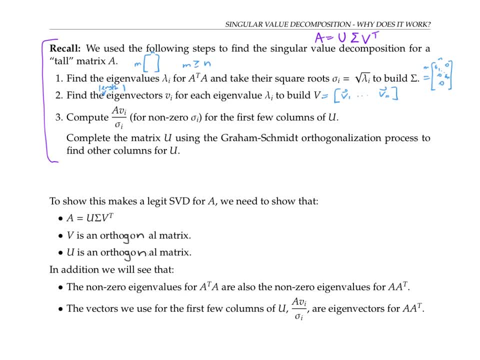 And then we also have to check that V and U. Okay, So our honest to goodness orthogonal matrices. In addition, it's interesting to note that the nonzero eigenvalues for a transpose times a end up also being the nonzero eigenvalues for a transpose. 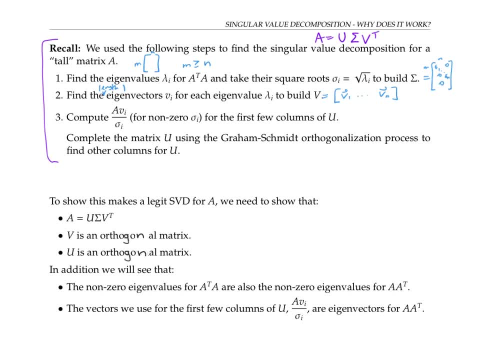 And it's interesting that the vectors we use for the first few columns of you, these vectors of the form a times V sub i over sigma sub i, are actually eigenvectors for a transpose. So we'll also look at why these two facts are true. 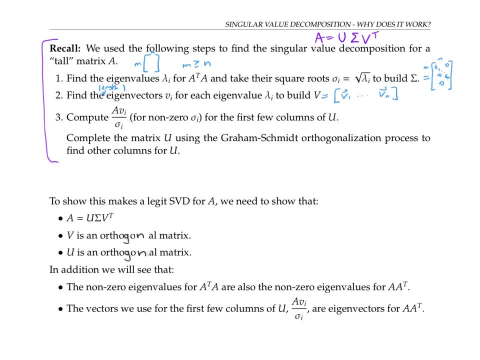 These facts show that, even though we build our matrices, use sigma and V and sort of an asymmetric way, focusing on a transpose, a instead of a transpose, and using eigenvectors to get V, but doing something entirely different for you, Even though we use an asymmetric method, we there is in fact a symmetry to how you is. 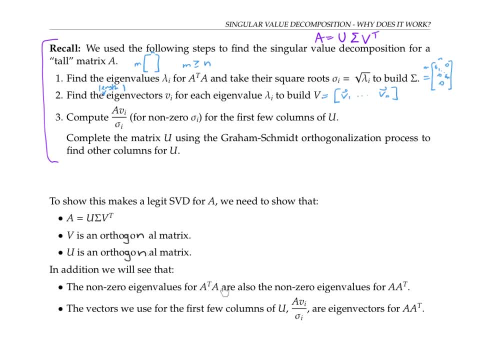 formed, V is formed And The choice of doing a transpose, a instead of a transpose. I'm going to start by showing these two matrices are orthogonal, then I'll show that a is the product we think it should be, And then I'll show these additional facts. 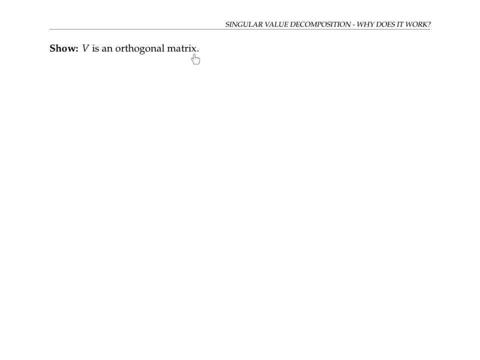 I'm not going to say very much about why V is an orthogonal matrix. Recall that the columns of V are eigenvectors for a transpose a. So that's just so. it's probably not necessarily stretching the useful values for your matrix. On the whole, we would do the same thing over here, which isLI. 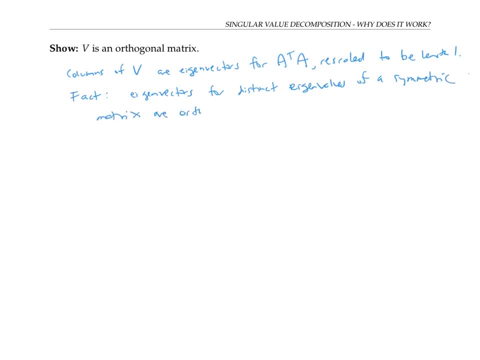 And four times V for me is going to be bra ka, which is drop down here, and B for me. Remember, if H is an orthogonal matrix, both sources are orthogonal, So that it's definitely empathic. Both of these are actually symmetries. 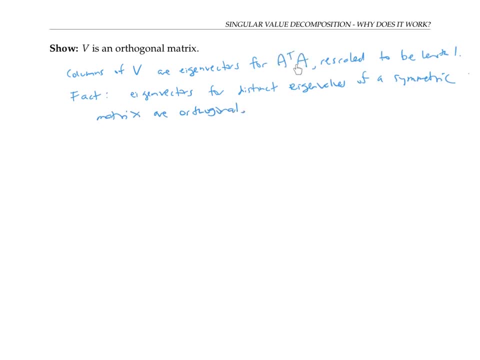 at least in the case when it has distinct eigenvalues. we're going to get orthogonal eigenvectors And so rescaling them will mean they're orthonormal and our matrix will be an orthogonal matrix. It turns out that when A transpose, A doesn't have distinct eigenvalues, 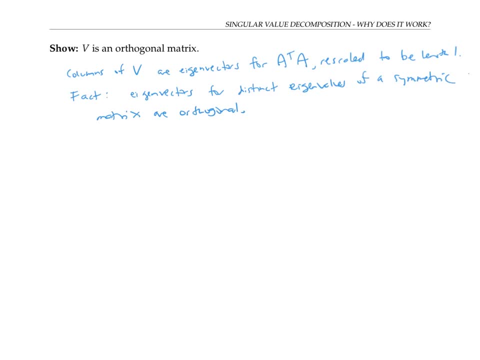 it's still possible to choose eigenvectors in such a way that they're orthogonal to each other, And so rescaling them will still give us an orthonormal collection of vectors to make an orthogonal matrix V. Next, let's convince ourselves that U is an orthogonal matrix. 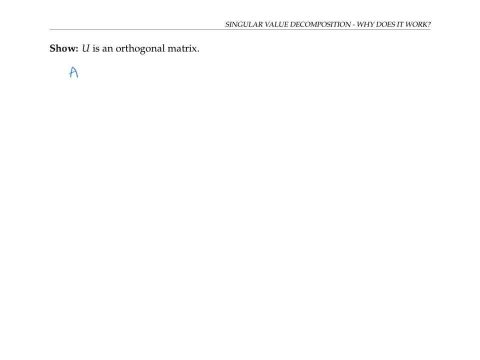 The first few columns of U are of the form A times VI over sigma i, where VI is one of the column vectors of V. So if we take two of these column vectors, two different ones, say AVI over sigma i and AV j over sigma j, And we want to check if these are orthogonal. 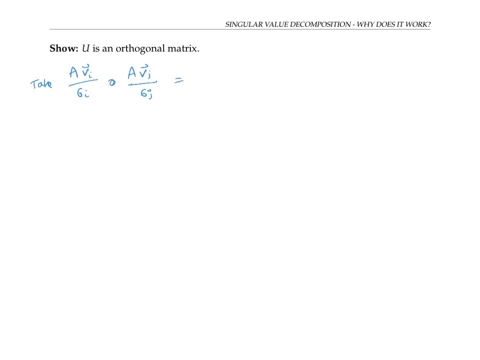 we're going to take the drop product. Well, that's the same thing as taking the first vector, transposing it and doing matrix multiplication with the second vector. I can pull these scalars out And now I have a VI: transpose matrix multiplied. 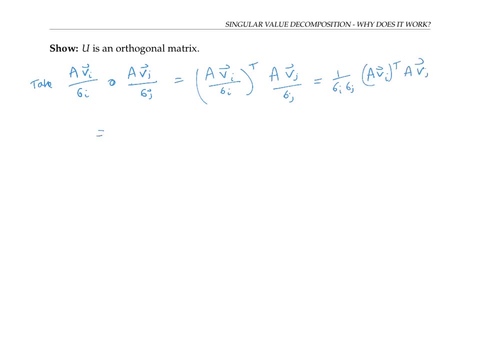 by a VJ Using transpose rules. This is the same as this expression, Since when we take the transpose of a product, it's the product of the transposes in the opposite order. Now VJ, remember, is an eigenvector for A transpose A. So when I multiply A transpose, A times VJ, I'm just going. 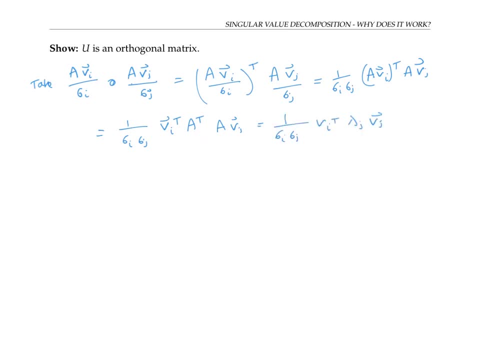 to get lambda j times VJ, Let me pull out the lambda j, But VI transpose times VJ. I'm going to vj is the same thing as doing the dot product of vi and vj And if i and j are different. 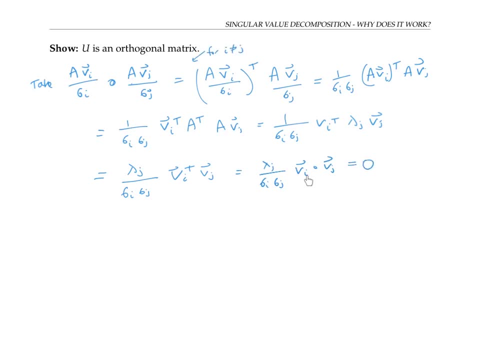 then this is just zero, because my matrix v, we already showed was orthogonal. So the dot product of distinct columns of you in those first few columns of this form are all going to be orthogonal. And furthermore, if I take something of the form a, vi over sigma, 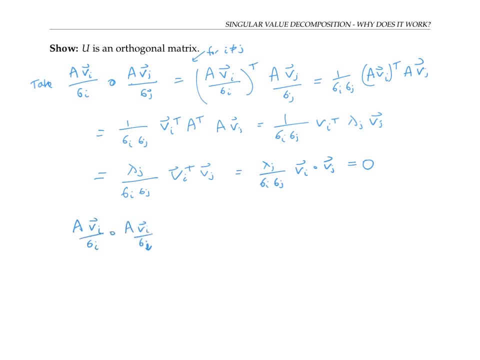 i and dot it with itself, then this exact same computation is going to get me down to lambda i over sigma i. sigma i vi dot vi. Since sigma i is the square root of lambda i, this quotient of scalars is just equal to one. And since the matrix V is an orthogonal matrix, 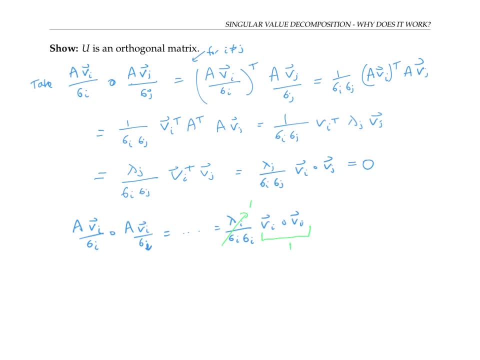 this dot product is equal to one, So this whole expression evaluates to one. Therefore, the initial columns of the matrix U, the ones of this form, form an ortho normal set. But when we added on some more columns to you to complete it to an M by M matrix, we did so in a way to ensure those last columns. 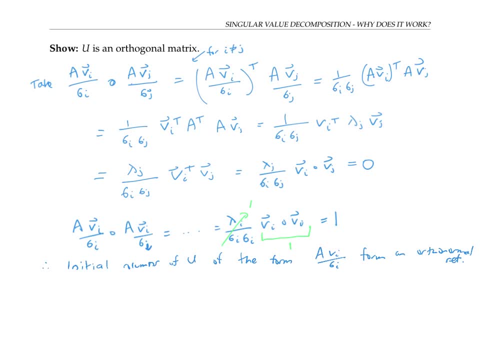 would be orthogonal to each other and to the first columns because we used the Graham's Schmidt orthogonalization process And we also made sure they were length one by dividing by their lengths if needed. Therefore, all of the columns of U are an ortho normal set. 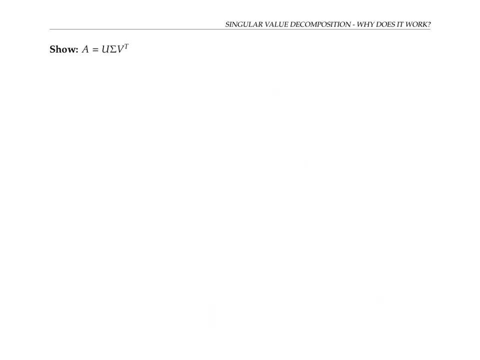 and U is an orthogonal matrix. So now let's show that a really is equal to u times sigma times V transpose. Since V is an orthogonal matrix, V transpose is the same thing as V inverse, So we need to show that a is equal to u sigma V inverse, or equivalently that a times. 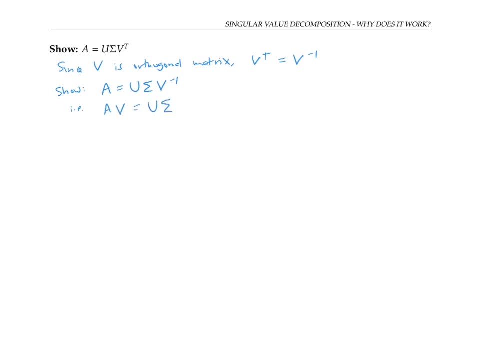 V is equal to u times sigma. Well, when we multiply two matrices together, that's the same thing as multiplying the first matrix by each column of the second matrix and then just concatenate those columns together. I'll write this down. And when we multiply a matrix, 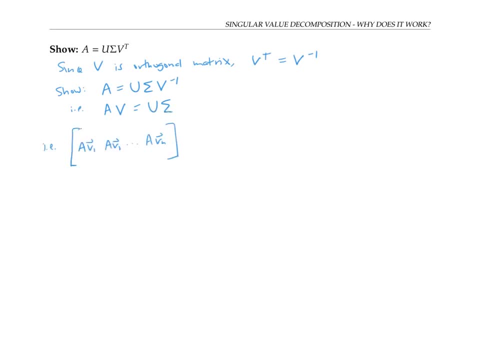 by a diagonal matrix on the right. that's the same thing as multiplying each column of the first matrix by the corresponding diagonal entry. I'll write this down. Notice that if u is an m by m matrix and sigma is an m by n matrix, with m bigger than n, then the last. 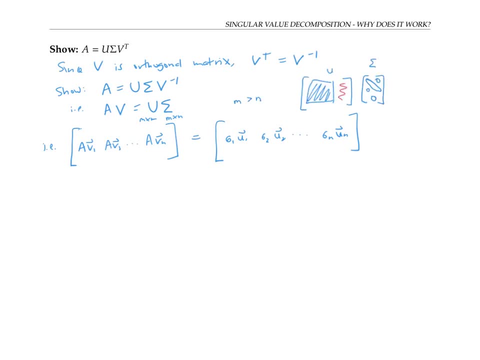 few columns of you. they don't even appear in this expression. they're completely irrelevant, because all the entries in those last few columns just get multiplied by the zeros down at the bottom of sigma. So this is what we're trying to show. In other words, we need 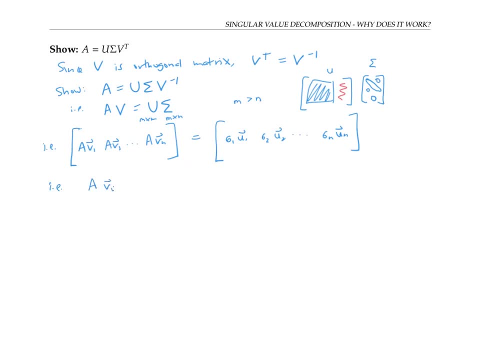 to show that a times vi is equal to sigma i. times u i for i between one and n For sigma i, not equal to zero. we know that u? i is defined as a times vi over sigma i, And so sigma i u i is going to be sigma i. a vi over sigma i, canceling out the sigma is. 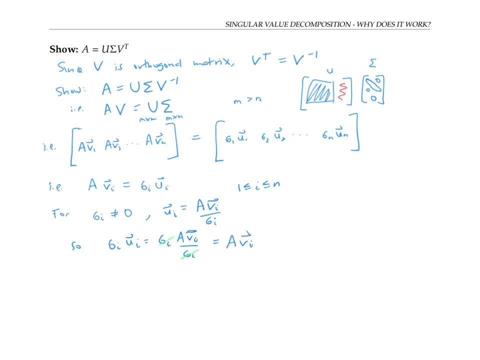 we get the equality that we're looking for. And if sigma i is equal to zero, then sigma i, u i is just zero. But lambda i, which is sigma i squared, is also zero, zero. So a VI is also going to be zero times VI, which is the zero vector also. So we have 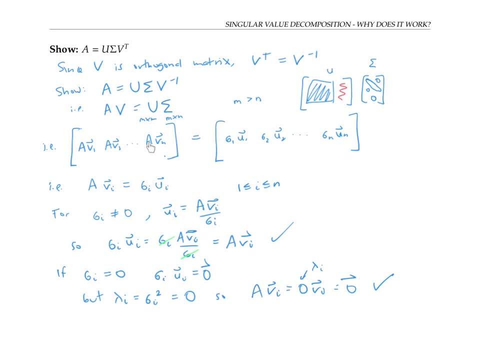 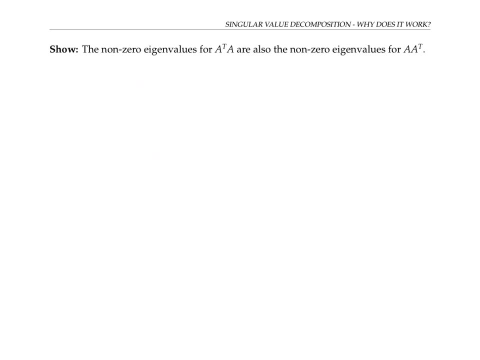 the equality of matrices, that we need to prove that a is equal to u times sigma times v transpose. Next, let's show that the nonzero eigenvalues for a transpose a are also the nonzero eigenvalues for a transpose. Suppose that lambda sub i is a nonzero eigenvalue for a transpose. 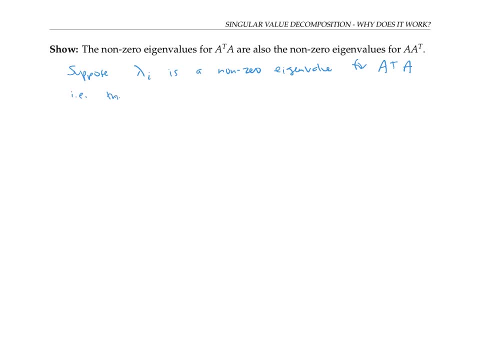 a. In other words, there is a nonzero vector, say x- i, such that a transpose a times x i- x i is equal to lambda i times x i. Let's multiply both sides of this equation on the left by the matrix A. That gives us a transpose a x i equals a lambda i x i. If I pull out. 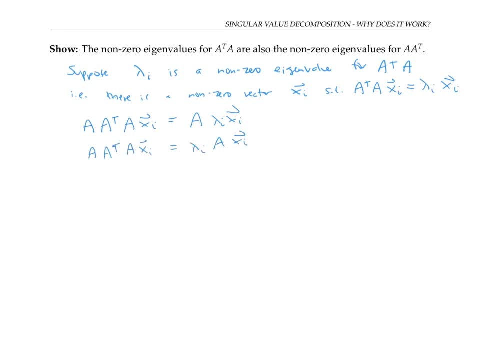 the lambda i on the right side. give the vector a x i a name, say y i, then I have the equation a x i a. transpose: y i is equal to lambda i, y. i Note that y i is not the zero vector Because 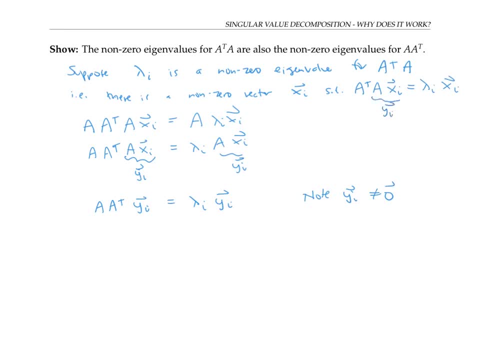 if it were, then a transpose times y i, in other words, a transpose a x i, would be a zero vector, which would mean that lambda i would actually be a zero eigenvalue. Therefore, we know that y? i is an eigenvector for a transpose with eigenvalue lambda i, So lambda i is. 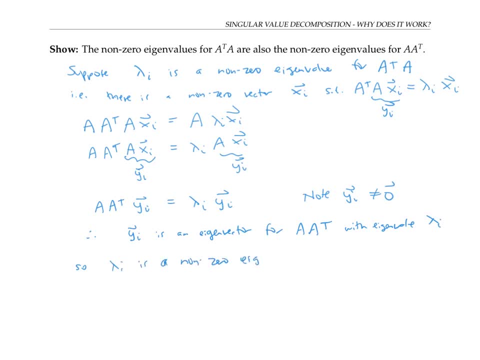 a nonzero eigenvalue for a transpose. Conversely, lambda i is a nonzero eigenvalue. Now let's If mu i is a nonzero eigenvalue for a transpose, ie a transpose times. some say z i is equal to mu i times z i. then the same kind of argument, multiplying both sides on the left by a transpose. 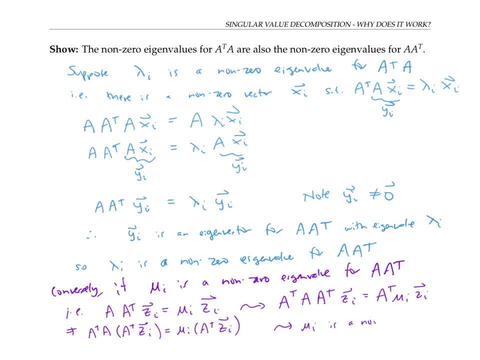 will show that mu i is a nonzero eigenvalue for a transpose a. So the nonzero eigenvalues for these two matrices- a transpose a and a transpose- are exactly the same. And when we're doing the singular value decomposition, even though we build the matrix sigma in. 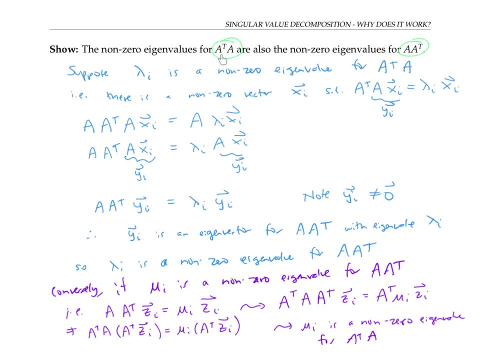 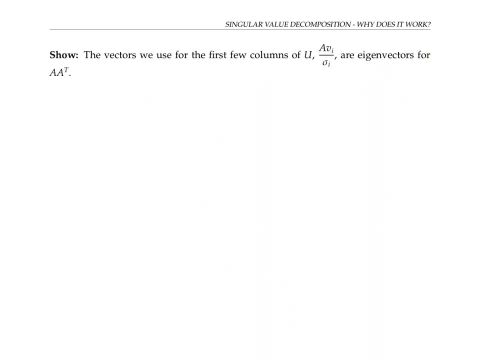 terms of the eigenvalues for a transpose a. we could just as well have built them in terms of the eigenvalues For a transpose. Finally, I want to show that the vectors were used for the first few columns of u, the vectors of the form a times vi over sigma i, where the vi are the eigenvectors. 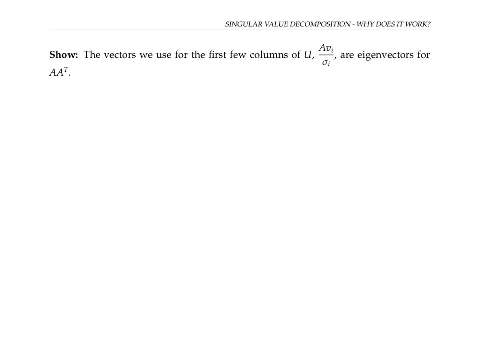 for a transpose: a, the columns of the V matrix and the sigma i are the singular values and nonzero singular values. I want to show that these first few columns of u are actually eigenvectors for a transpose. This shows that u and v have a lot more in common than we might first have realized. 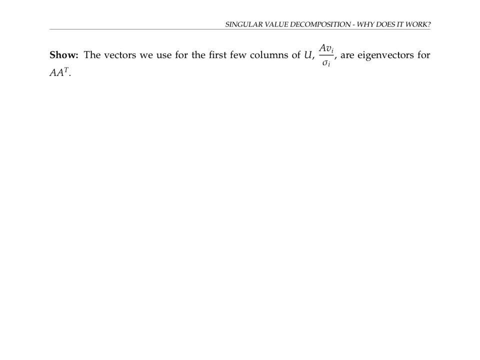 They're both built out of eigenvectors. So to prove this, let's take a transpose and multiply it by a V sub i over sigma i. I'll pull out the one over sigma i. And now, since V sub i is an eigenvector for a transpose, a with eigenvalue lambda i, I can rewrite this: 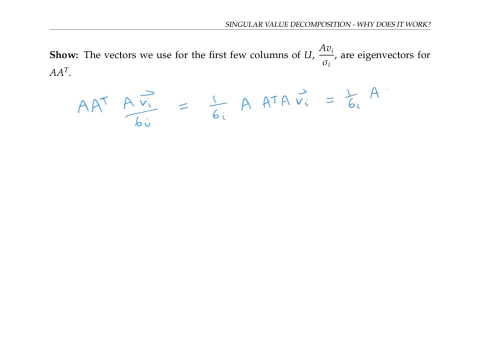 as one over sigma i times a times lambda i, V sub i. Now let me pull out the scalar lambda sub i and rewrite things a little bit, And we see that this vector a V sub i over sigma i, when we multiply a transpose by it, we just get the same thing as lambda sub i times it. 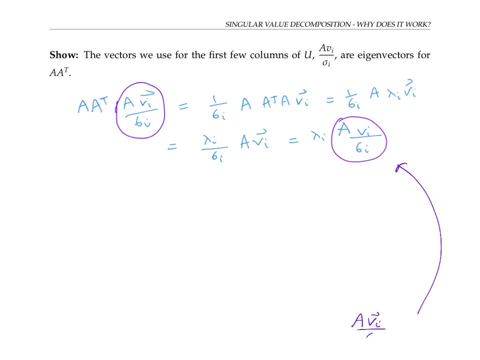 Also this vector, a V i over sigma i, is not equal to the zero vector, Because if we multiply a, transpose a V sub i over sigma i, then that gives us lambda i, V sub i over sigma i, which is not zero, because we're assuming sigma i and therefore lambda i are not zero. Therefore, 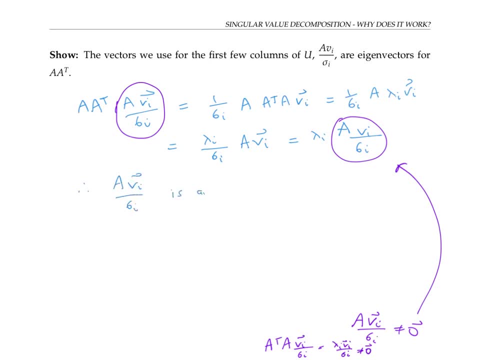 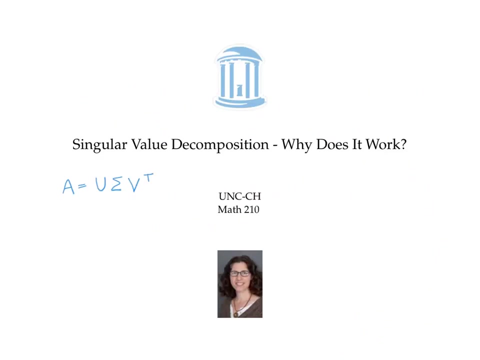 a V sub i over sigma i is an eigenvector for a transpose with eigenvalue lambda sub i. This video squared away a lot of the details about singular value decompositions. The matrices u and v that we built really are orthogonal. When we multiply u times sigma times v transpose, we really do get back a.